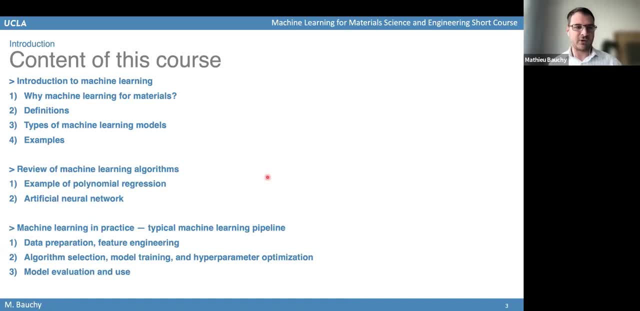 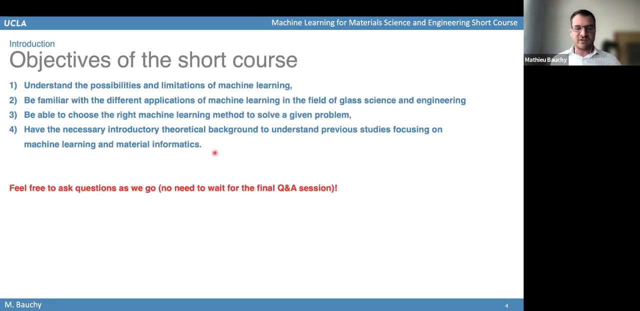 I don't think we have to wait for the end to ask questions. I'd rather you just ask me questions as you go, So either by raising hands or just by opening your mic and just asking questions. So feel free to interrupt. In terms of the objectives of this course, 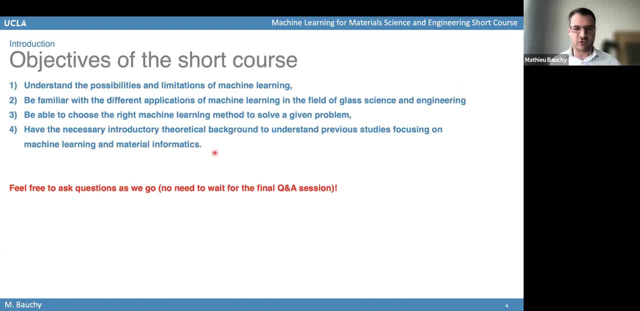 So of course it's still like a pretty short course, so we cannot go through everything, But what I would like to really have you get out of this course is understand what can be done with machine learning and what cannot be done. So understand both the potential possibilities but also the limitation of what we can do using machine learning for materials. 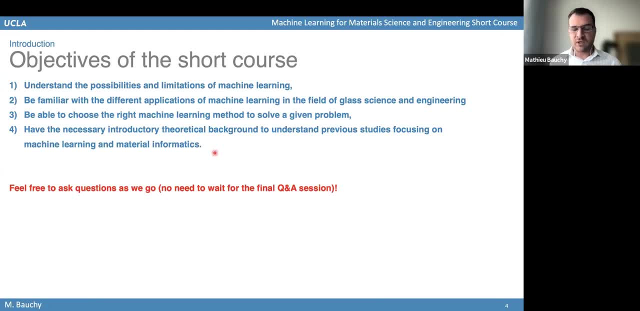 And another thing is to be to get a first taste of what are the different aspects of machine learning, And another thing is to be to get a first taste of what are the different potential application of machine learning in the field of materials. In this presentation I'll focus a little bit more on glasses. 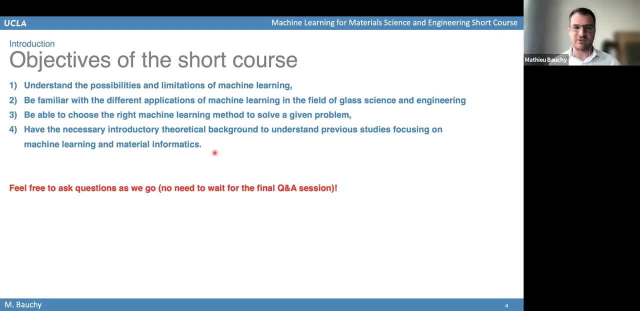 So I'll take glass as an example of materials, because it's a good example of a material that you can really optimize or understand better using machine learning. But everything that I present is also general to any kind of materials. And then the next thing is that, when it comes to machine learning, there is really many methods available. 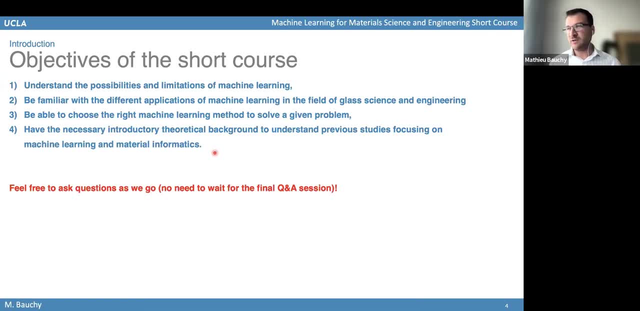 And to some extent, if you want to work in the field of machine learning, the difficulty is not necessarily to use a given machine learning tool, because most of those tools they are available, They are free to use. There are a lot of tutorials online. 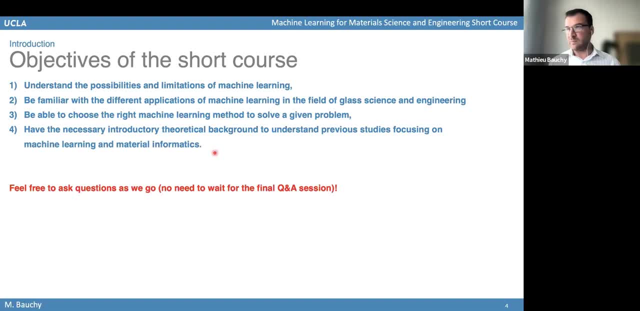 And it's typically not available. It's typically not that difficult to use. I think the real difficulty is how to choose the right tool, Like if you have thousands of machine learning packages available, how to choose the right one, how to choose the right algorithm to solve a given problem that you have. 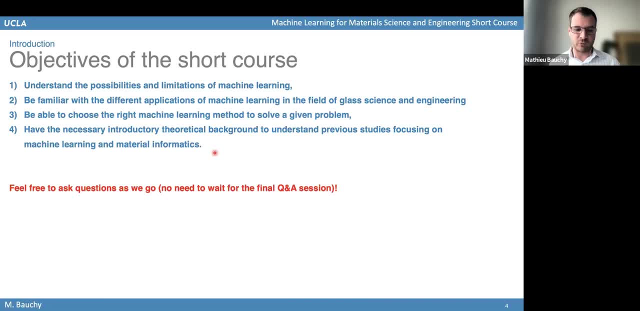 So I think this is more where the difficulty- and this is more what will distinguish somebody who has more experience in machine learning from somebody who doesn't have so much experience- is how to choose the right tool to solve a given problem, And so what I hope also is that after this course, you would be able to understand better. 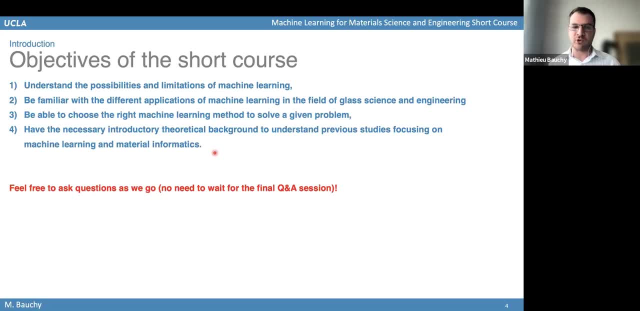 Like if you are reviewing a paper involving machine learning for materials, then you would be in a better position to understand the content of this paper, the potential limitation, or use this paper to inform your own research as well. So, yeah, as I mentioned, feel free to ask any question as we go. 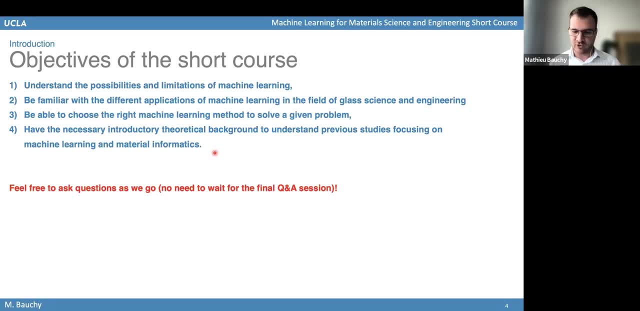 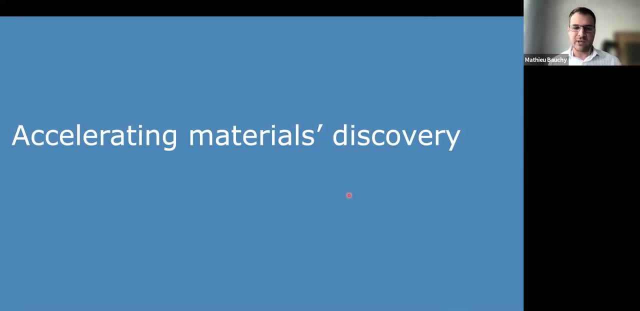 Thank you, So just turn on your mic and feel free to ask if there is something that is not clear, or if you want more details about something in particular, Yeah, so let's get started then. So the first thing I'd like to talk about is how do we discover materials in general, and how machine learning can help discover new materials more efficiently. 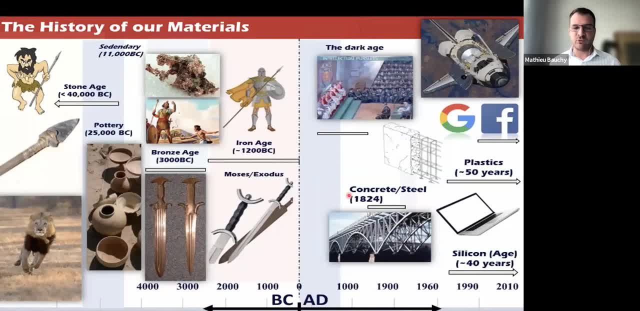 So the reason that we need to discover new materials is really about, like the story of mankind, Like, if you think about, like the story of human as a civilization, like the progress of humans are really linked to the discovery of new materials, And most of the progress that we have seen over the past centuries is very often linked to discovering a new material that unlock a new functionality that we didn't have before. 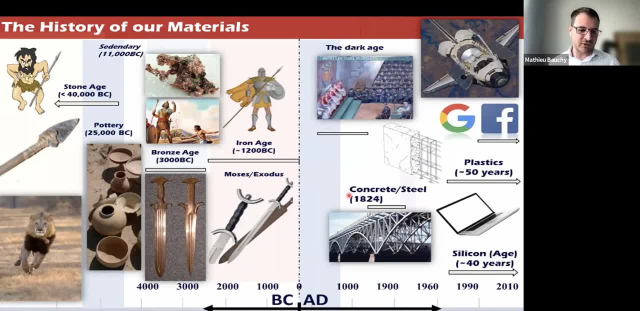 Right, And so this is true to the point that, like you know, the big ages in mankind are often named after materials Like, for example, you have the Stone Age, the Bronze Age, the Iron Age. So those are all ages that have been named after the material that enables some key advances in the story of mankind. 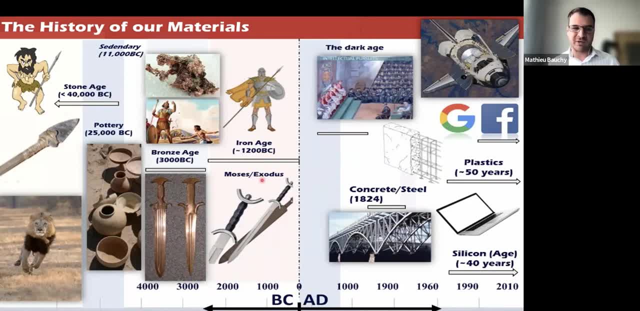 And so, when you think about everything that materials have been enabling, right? so the ability to use materials to build weapons in order to, well, to be able to eat, the ability, of course, well, everything involving material is very often linked to wars and to making weapons. 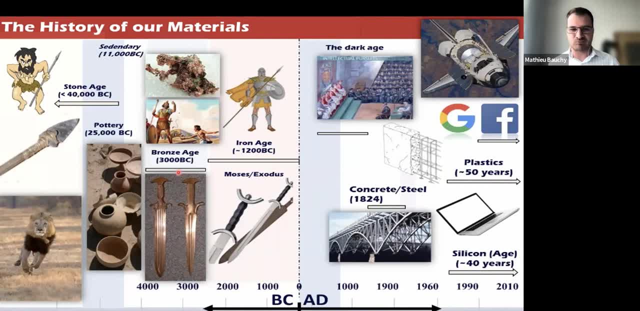 So that's not necessarily the most happy example of materials, But still that's a pretty important part of discovering new materials that enable, you know, to enable military application And then, more recently, like the discovery of concrete about two centuries ago, has really enabled like modern infrastructure as we know it today. 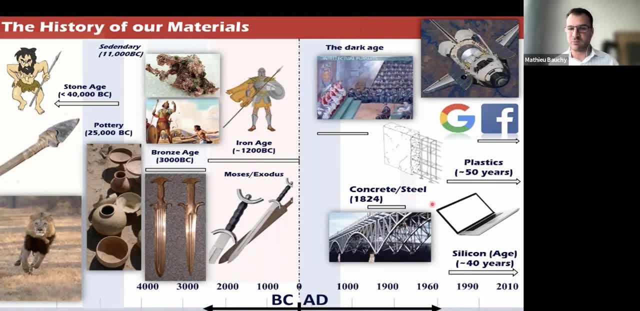 The discovery of steel also, is really what has enabled, like the construction of structure, that were not possible before. More recently over the past century, plastic. the discovery of plastic has enabled a whole range of new items that were not possible before And to some extent now we are still living in the silicon age, where the you know, 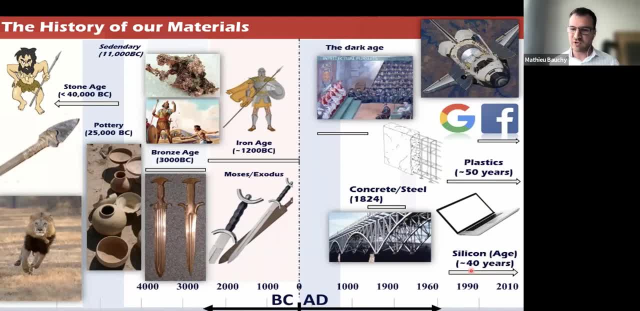 everything revolving about transmitting information or computing, everything relies on some silicon for chips And so over the past year, like the discovery of silicon and the ability to build silicon chips with very fine resolution, has really enabled, like the modern information age, where you can process a lot of information. 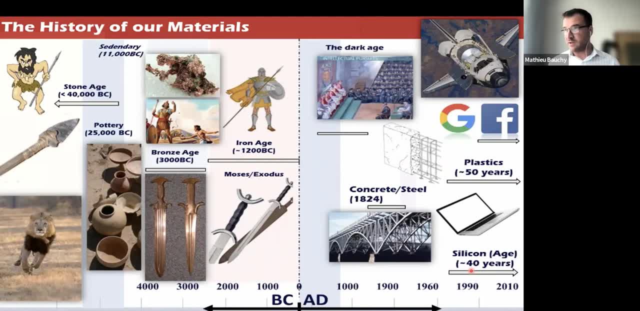 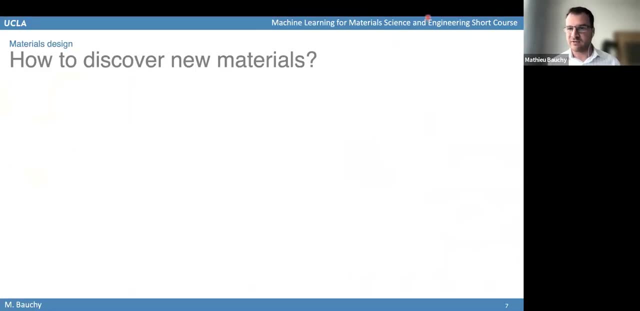 share information and use this for communication or processing information, things like that. So the modern world as we know it today. So, before we go any further, I'd like to maybe ask you like, and so I think that would be good if you could. 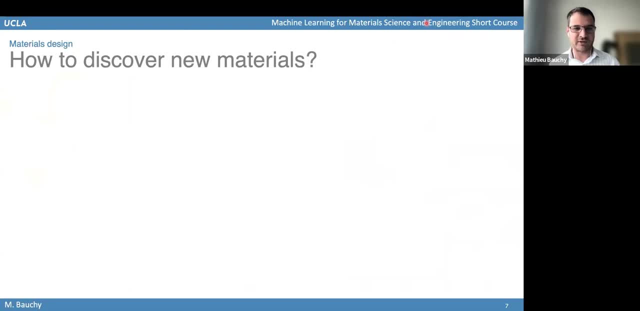 if you can also be active during this course, so that it's not just me talking and also you can participate. So, like my first question here would be: all of those progress that I just mentioned. So they all rely on the discovery of new materials. 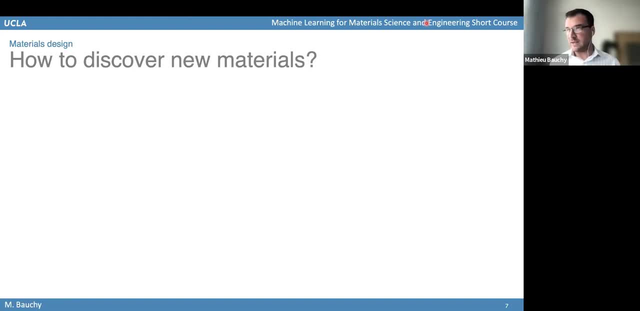 So the question is, if we want to continue making progress, like we need to continue to discover new materials that have new functionalities, that enable new things that were not possible before. So the question is: how do we discover those materials? So if it was easy to discover new materials, then we would have discovered them all already. 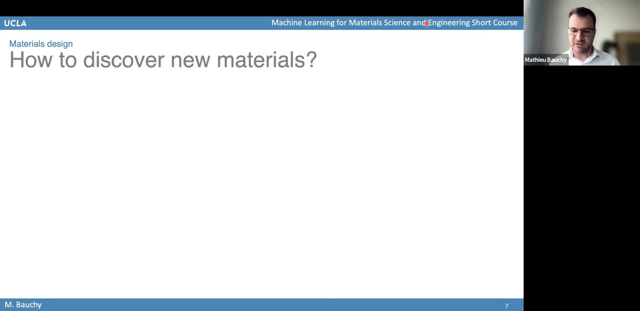 But we know that we keep discovering new materials all the time, which means that it's not an easy process. So, like the first question that I would like to ask you is if you want to discover a new material either, like a completely new types of material. 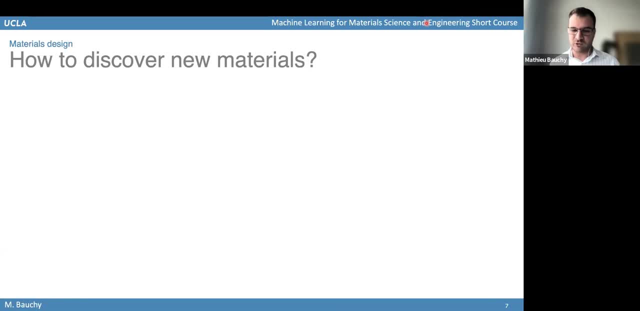 a family of materials, or simply a material that would be part of an existing family of material but that you want to optimize like. you have a given material and you can change its composition, you can change its structure, you can change its processing temperature, pressure, whatever. 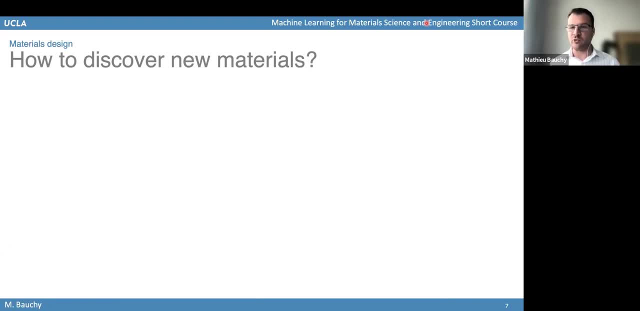 How would you discover? what would be your process to discover a new materials that has desirable properties or desirable behaviors that existing materials don't have? So, like what would be your process to discovering a new material? Does anybody has any idea on that? Like what? How would you discover new materials? 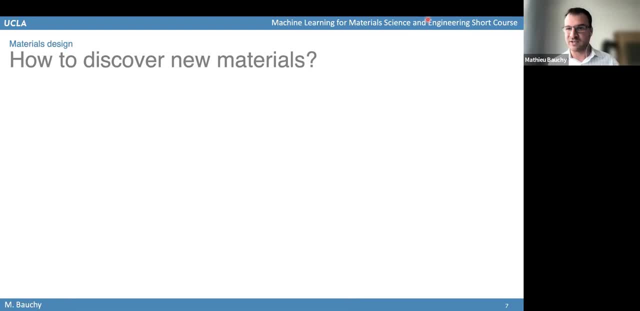 So let's see who is going to be the first to speak today. Usually, we always have a big embarrassing silence until somebody volunteers to turn on his mic. So let's see who is going to be the brave person to speak first. Anybody like? how would you, what would be your process to discover new materials that do not exist yet? 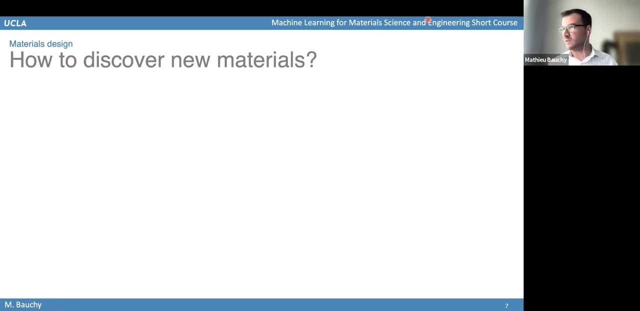 Or do you have any example of materials that have been discovered over the past centuries and how those materials were actually discovered? Anybody, Okay, Hello doctor, Hello, Hello. My name is Rita. I am studying my PhD. In my case, I am working about that- could be discovering a new material. 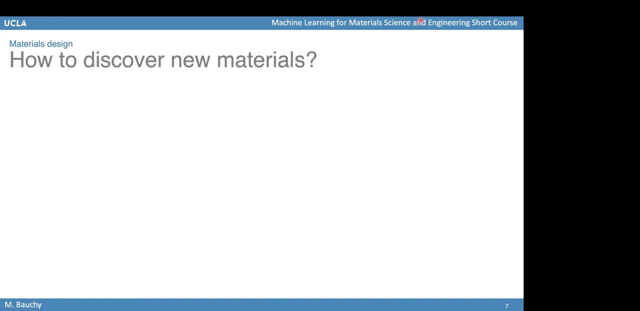 For example, in my case, I want to meet elastomer materials with the other materials- materials in chain, memory, alloys, or could be a different material in silicon Could be- Is considered how to discover new materials. Yeah, So what would be if you want to have, let's say, a new elastomer material that would have like different properties? 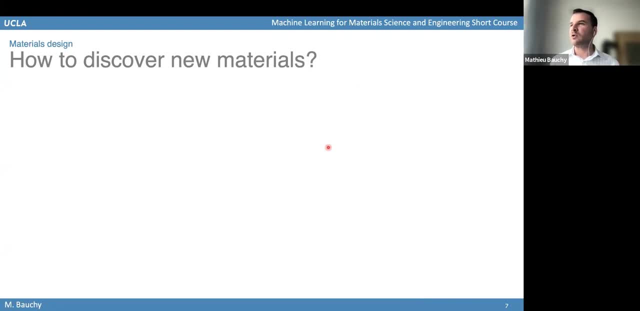 than the one that presently exists, like what would be your process to optimize these types of materials, to enhance, to increase Or decrease a given property of this material? Okay, In my case, I want to implement or application these materials in robotics because I am working in about the construction. 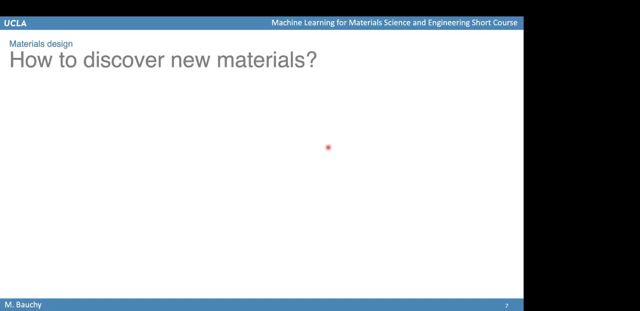 and design the different robots and, for example, prototypes or artifacts. I want to design the different actuators with these materials. Okay, I need to reduce the designs for my actuators. Yes, Okay, So like so a common process to do that right? 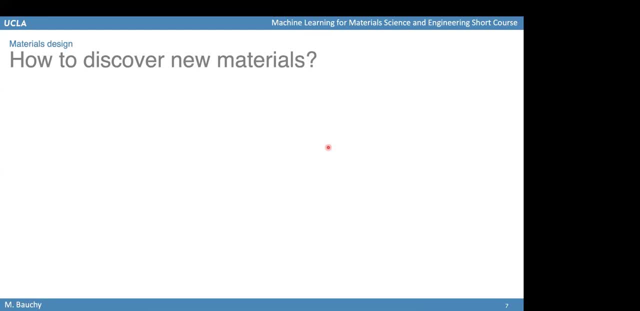 So if I mean- and it's very common in research that you try to understand some physics or some chemistry governing material, right, Right, So if you can understand the some fundamental knowledge of what dictates the property of a given material, then you can use this knowledge to try to change something in this material, like either it's processing. 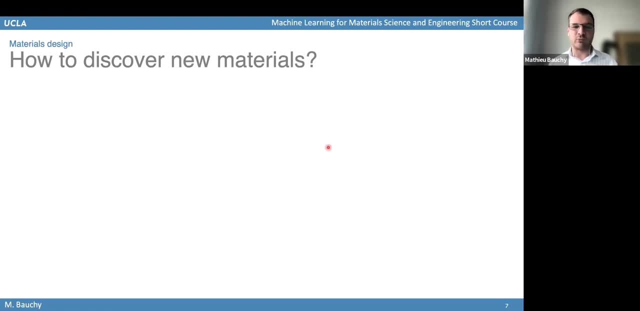 either it's chemical composition to try to improve its property right. So a very common approach when it comes to discovering new material or optimizing new material is to try to understand the fundamental physics that governs those materials, or to try to understand, to establish some laws, some relationship between the parameters of this material and its property. 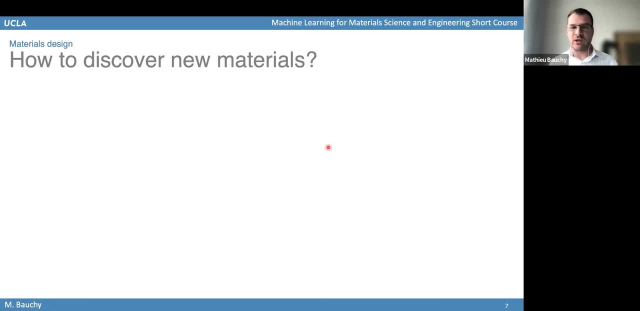 and then use that, use that knowledge to change materials, to adjust materials' properties, depending on the application that you have in mind, right? So that would be one way of discovering new material. One way of discovering new materials it's to try to use to develop some knowledge. 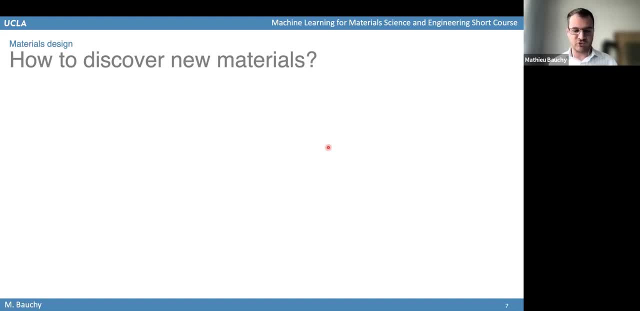 some physical knowledge or some chemical knowledge and to use that to optimize materials. Do you have any other example, like maybe anybody has, any example- of another way where you can discover materials without necessarily having some knowledge- some physical or some chemical knowledge- about how materials behave and why they behave the way they behave? 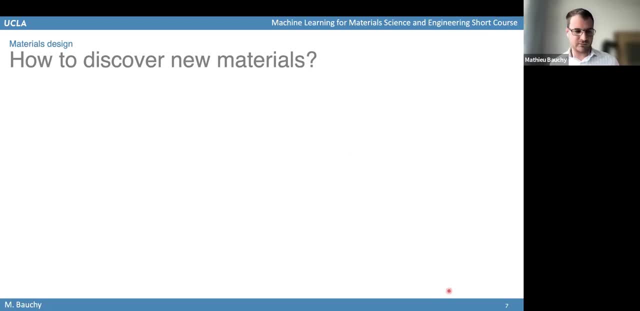 Anybody else has any idea regarding this. Do you have maybe something? Yeah, go ahead, You can repeat the question, please. Yeah, so what I was mentioning is so. one way to discover materials is to understand more- more about their physics or about their chemistry. 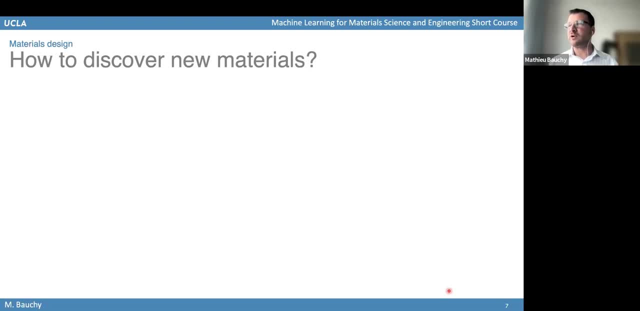 Like: if you understand some fundamental knowledge about why materials behave in a certain way, then you can use this knowledge to optimize materials, to try to change something in materials, like, for example, their chemical composition, in order to change their behaviors, change their functionalities, change their properties. 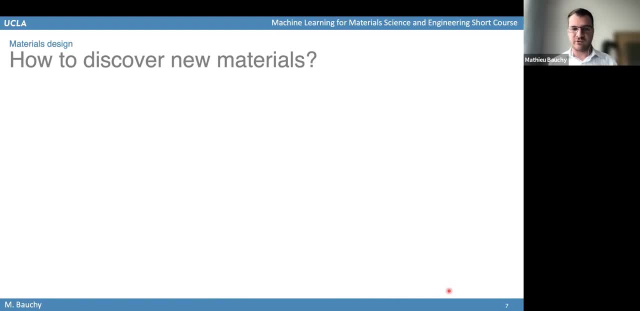 So that's one way of discovering new materials. Another way is to use some knowledge to develop some knowledge. Can you think of another way to discover new materials that would be different from that, Like when you don't know anything about a given material? 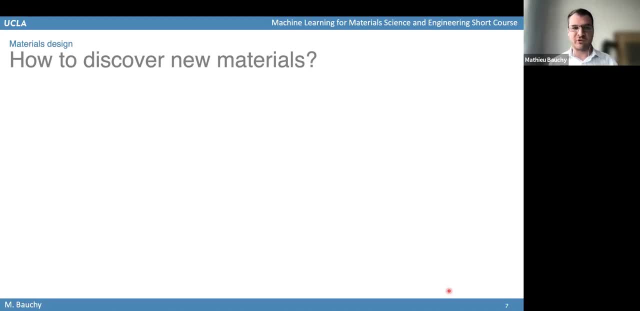 you don't know anything about the physics or the chemistry that governs the behavior of these materials, like: how would you discover new materials? How would you optimize materials? How would you change materials to enhance their properties? Any other idea? What could be other types of discovery process for materials? 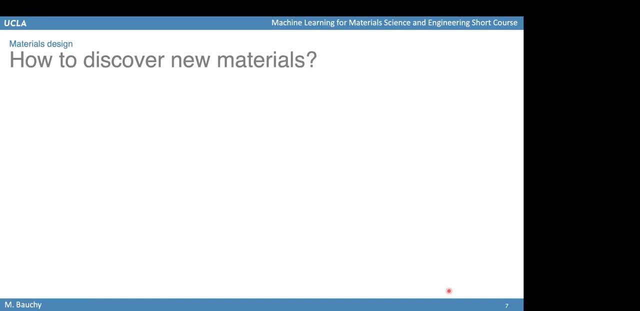 Yeah, Hello, Mario Avila, from Optical Research Center in León, Guanajuato. I'm postdoc, I think so I remember from my master's degree in France. we have to start with oxy-sulfur metal synthesis. 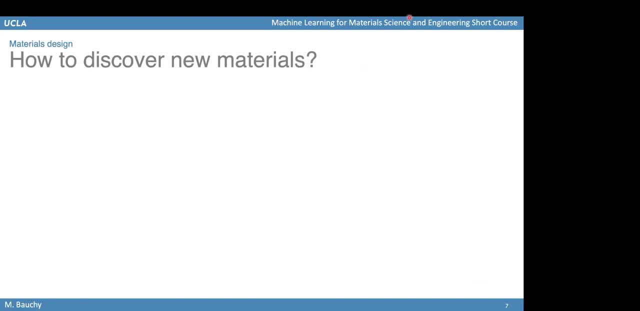 It was kind of new. Normally it was for catalysis, but it was not sure- And we start to synthesize from different elements And after that we have to analyze all the synthesis, the properties of the synthesis, the temperature, reactions, temperature, everything. 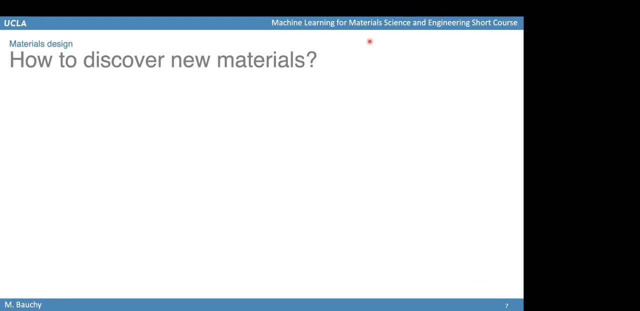 And after, with studies in physical chemistry, we discovered we have properties for the catalysis, also for imagining properties for the cancer Tumors, for cancer, something like that. It was something pretty new because it was only exist in the micro, macro matter. 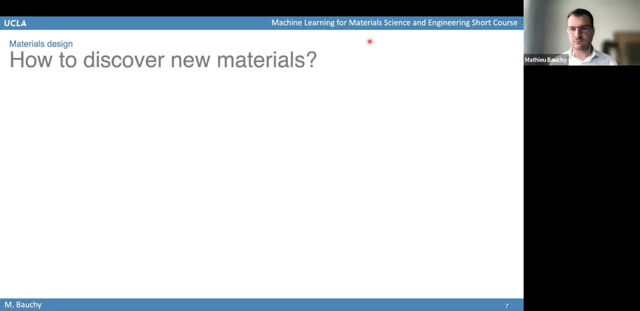 And it was very new for the nanometer. It was only to start with one article. We start to synthesize from the nanometer, We synthesize from the nanomaterials. We try with first the reaction after: If you use one solvent, we use another solvent. 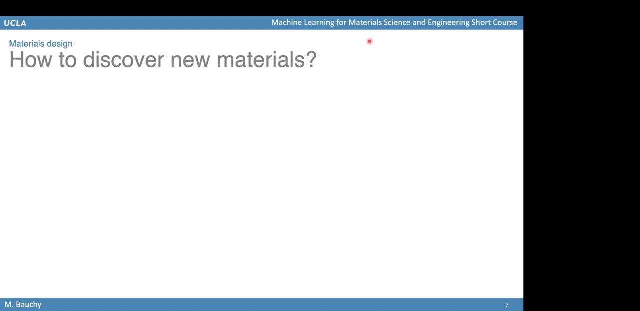 We use one. how do you say one reactive metal reactive or other metal reactive? What is the property, What is the difference between one and another? And I think so you have all the data they give us. I think so you have something for understand all the chemistry. 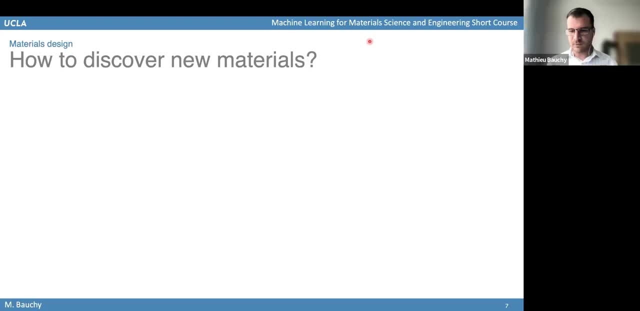 and the physics of this new material. Yeah, I think that's a great example. So I think this is a good example for when you start exploring a new type of material or new types of process for which you don't yet have some knowledge. 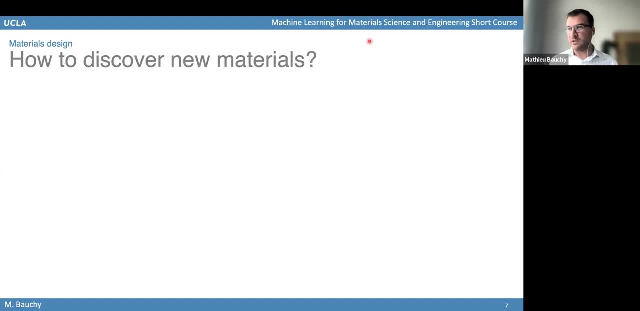 And then a very common way, as you just said, for example, in your case you just try different types of solvents, et cetera. A very common way in that case to discover a new process or new material is just to try everything you can think of. 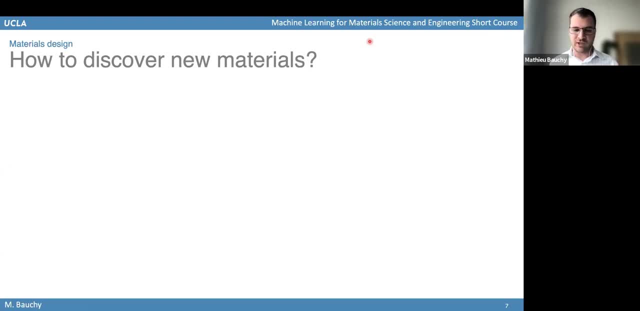 So if you have a list of solvents that you can use, for example, then one very common way to optimize this process is trying all the solvents that you have at your disposal and see which one will give you the best properties at the end, right? 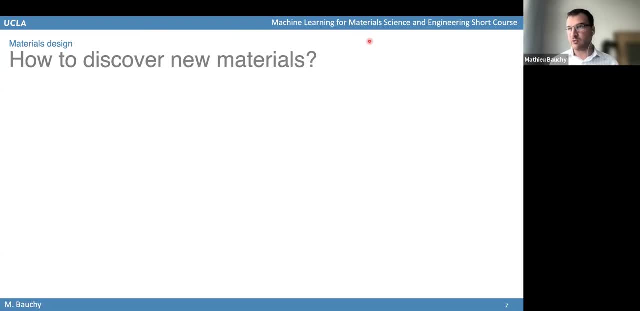 So this would not. in that case, this would not really be a process that is based on knowledge, because we don't really have knowledge initially when we start to study a new material. It would be something that we would call like a systematic exploration or a high-throughput exploration. 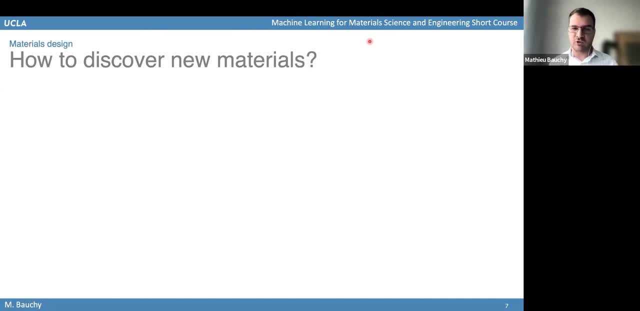 where you have a list of potential candidates, So that can be candidates, in the sense of you have a list of solvents that you can use. Or maybe you have a list of condition, like I don't know, like the temperature, the pH, et cetera. 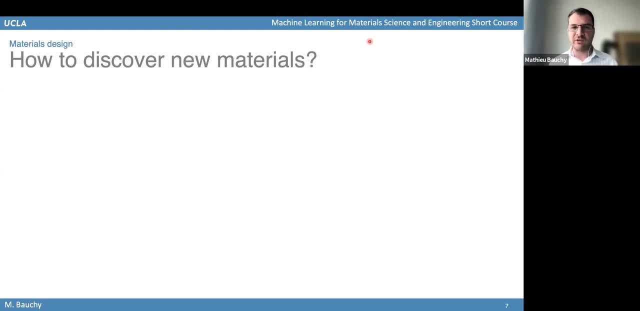 So those are a list of candidates that you can choose from, And if you don't know initially what are the best candidates for a given application, then you just a common strategy is just to try them all and see which one is the is going to perform the best right. 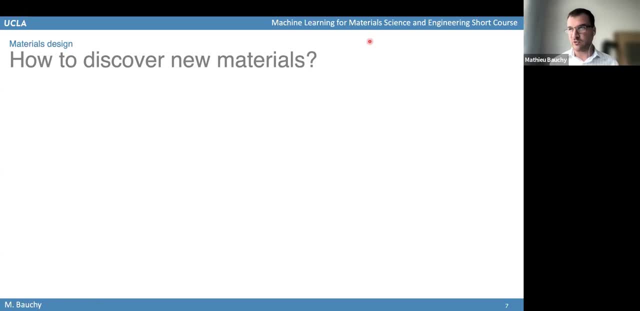 So that would be another types of discovery process where you just explore systematically all the parameters that you have at your disposal and you will see at the end which one performs the best. So that would be like a systematic exploration of all the degrees of freedom that you have at your disposal. 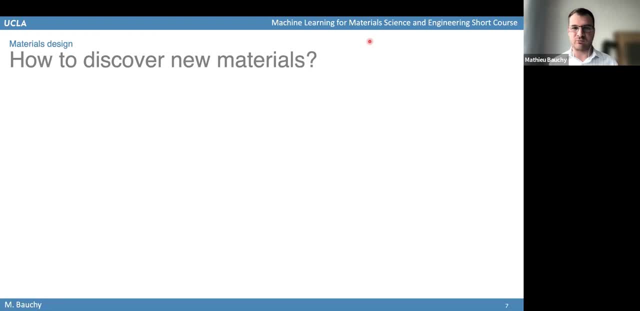 and see at the end which one gives you the most desirable properties. So that would be a very common second way of discovering new materials. Does anybody else has any other ideas Like besides using knowledge to discover new materials or besides just trying a lot of different condition? 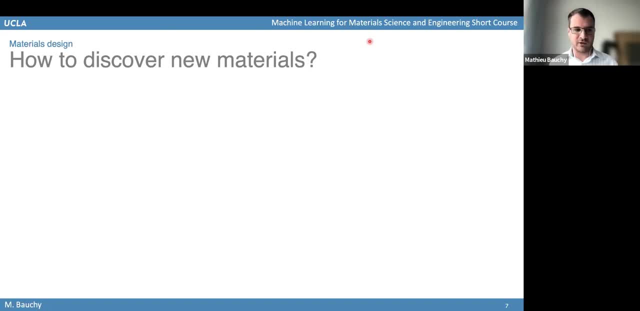 and see which one gives you the best material at the end, like any other ideas on how to discover new materials. Okay, So let me review a little bit like what I think are like the main ways of discovering new materials. So one thing: when you discover new materials, 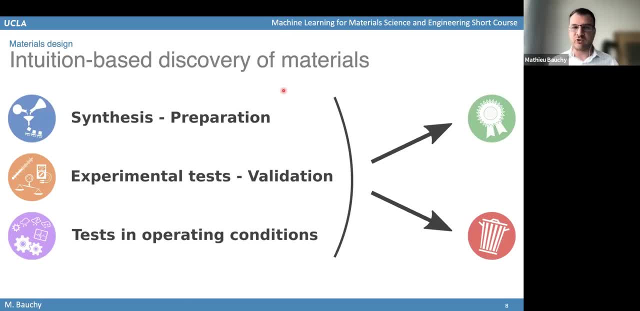 is. a lot of these things sometimes rely on intuition, especially when you have worked with a given types of material already. In many cases, you already have some intuition about what are going to be the right condition- the right, the most promising condition or the missing condition- to make a given material. 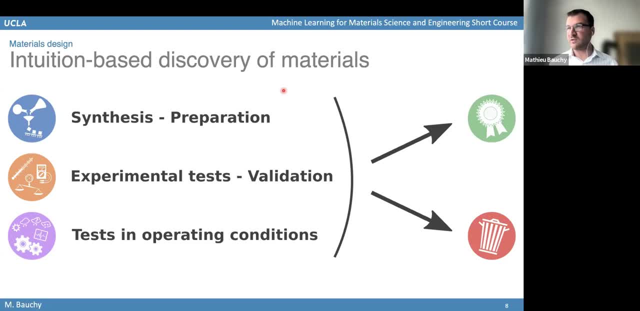 So in many cases, like if it's a scientist is trying to optimize a given material, he's going to use his previous experience, use his intuition and use this knowledge to optimize materials, And in that case, a very common process would be: first you try. 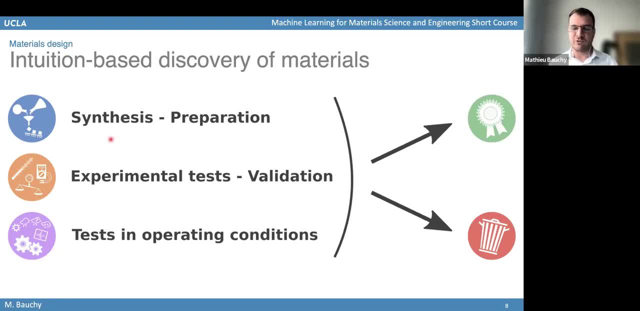 So you synthesize this material, So you follow a given recipe to prepare a given material. Then, based on that, you are going to experimentally test this material, So you are going to measure the performance of this material And after that, either the material will pass the test. 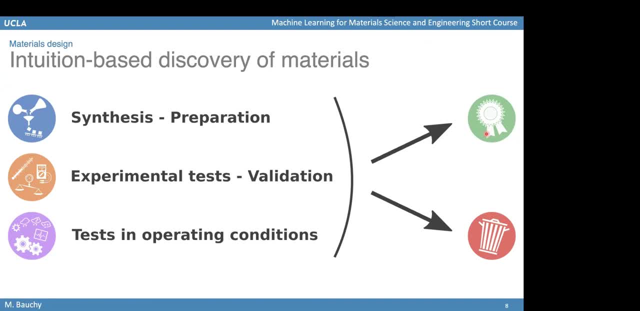 So either it will show some properties that are the one that you expect, either it will not, And so if it passes the test, then you can keep this material and you have successfully discovered a new material, Or if it doesn't pass, as the text. 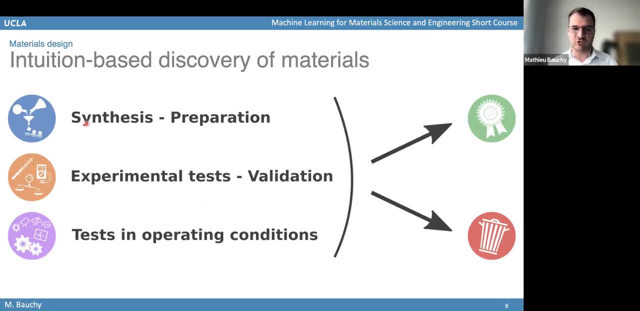 then you have to try again, right? So you have to try again. You have to change something in your recipe, change something in the way you are preparing this material. Try again and see if the change in your recipe has improved the priority of the material. 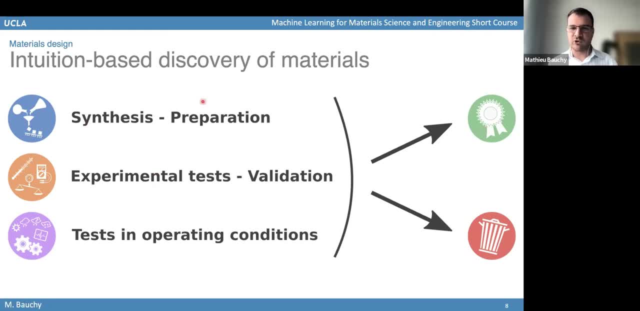 And if now it meets your condition, And so you will repeat that iteratively, And every time that you fail in your experiments you will try to use this material, And you will try to use those failures to build your intuition about what are the right conditions to prepare new materials. 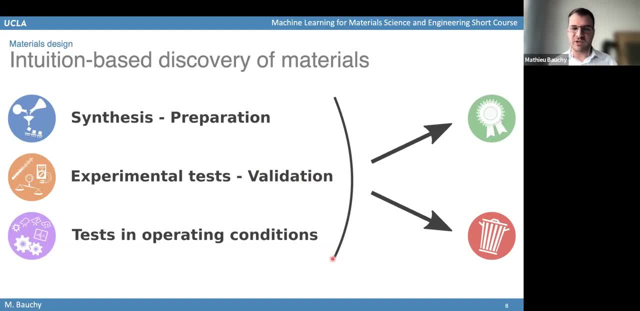 And at the end, once you have found your material, then you will. usually it's one thing to test it in the lab, but you will also want to test it in an operating condition, like to test it in real life, to see if what you tested in the lab also translates to operating conditions. 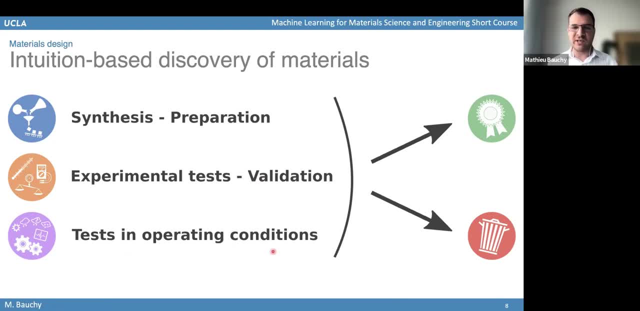 And if the material performs well in an operating condition, then you have found the material that you wanted to find, And if not, again you need to go back to change something in the way you prepare this material until you have found the material that performs as expected. 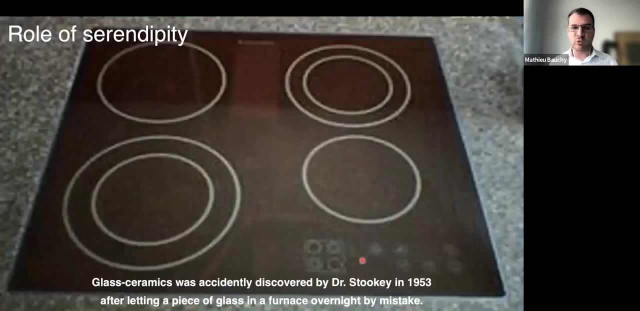 So a very other common way that you have not mentioned but is actually very common is: very often materials are just discovered by chance. It can be either due to some mistakes that you make or just like purely by chance by just trying a lot of conditions. 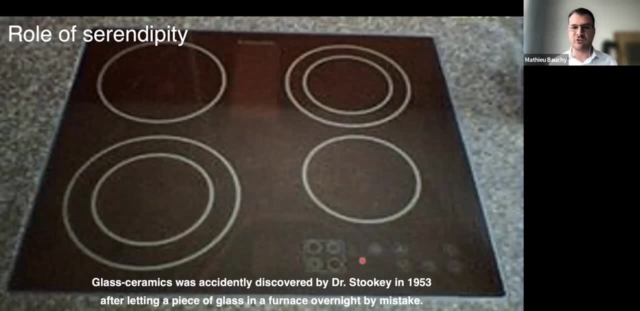 until you find like a set of conditions that gives you something unexpected, like a new types of material that you were not expecting. It's very common, for example, that scientists would try to change something in a material to optimize it And, in the process, either due to a mistake, 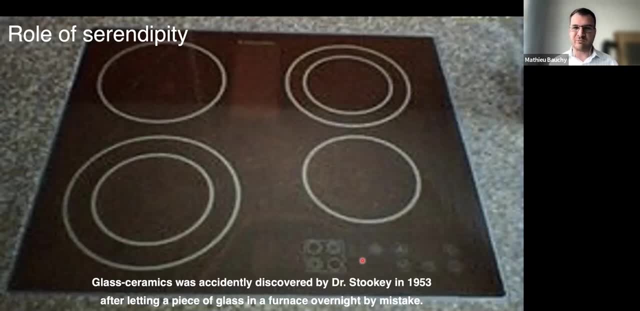 either, due to luck, they will discover a completely new types of materials that they were not necessarily expecting So like, for example. one example is the material like of glass ceramics. So this is the material like vitro ceramics like this that is used on certain types of cooking station like this: 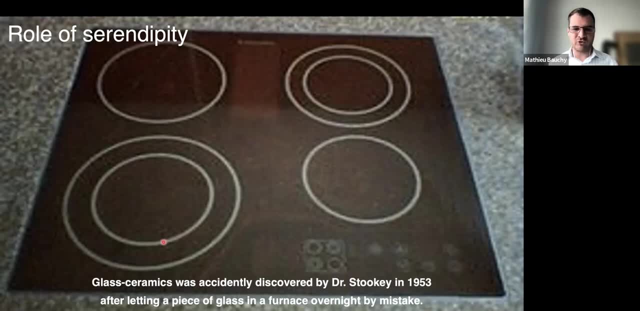 It's a metal that can sustain, like very high temperature or very rapid changes in temperature. It can go from very cold to very hot very quickly without breaking, unlike glass that would be subject to thermal shock. So, like this is an interesting material, because it was in this case. 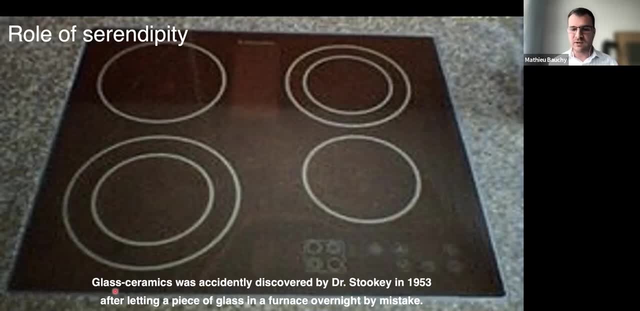 this glass ceramics completely discovered by chance. So it was discovered, like about 50 years ago, by Dr Stuckey, who was a scientist at Corning, which is a company that makes a lot of glass and a lot of ceramics, And so the way it happens is that 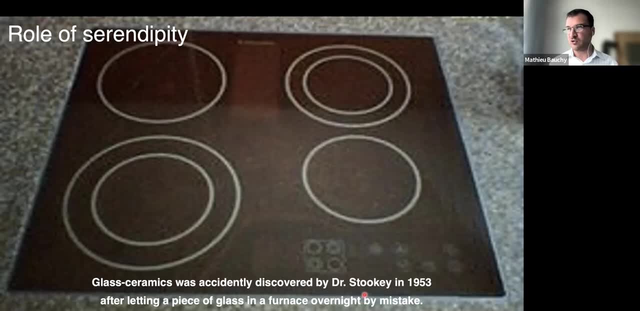 so this scientist, Dr Stuckey, was trying to discover new glasses, and the way to make glasses is to melt something in a furnace and then to quench it very quickly to prevent any crystallization and to form an amorphous glass. And so what it did, by mistake, is that he left a piece of glass in a furnace. 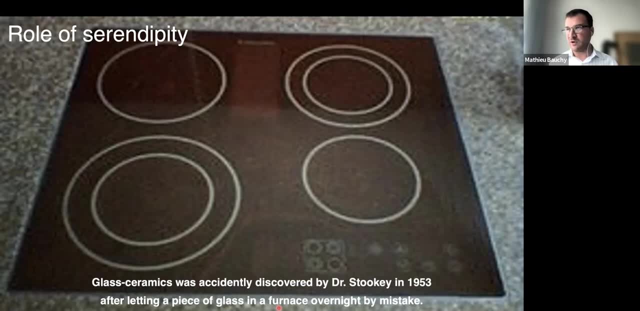 and just left it like all night long and forgot to remove it from the furnace before he left, And so what he discovered in the next morning when he came back to the lab is that this material that he has left in the furnace overnight was not transparent. 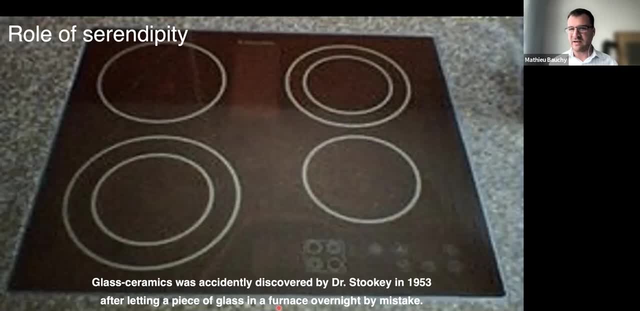 like you would expect for a typical glass. So it became like a pretty dark, So like, basically, this material had crystallized overnight, like it was not amorphous anymore, And so what he did is that then he just realized his mistake and just take this piece of material and just throw it in the trash. 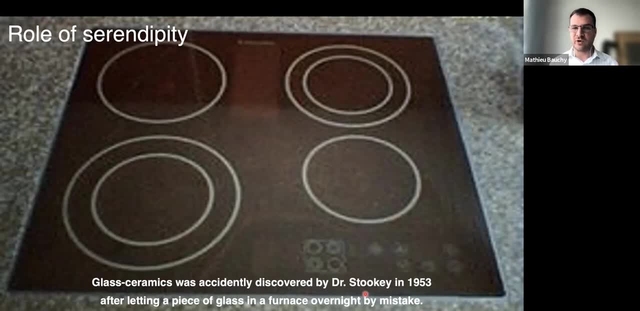 and then realize that, after throwing this metal in the trash, that this metal actually did not break, Like if you take a typical glass and if you drop it, this piece of glass is going to fracture because it's a very brittle material, But this material that he had synthesized like was very tough. 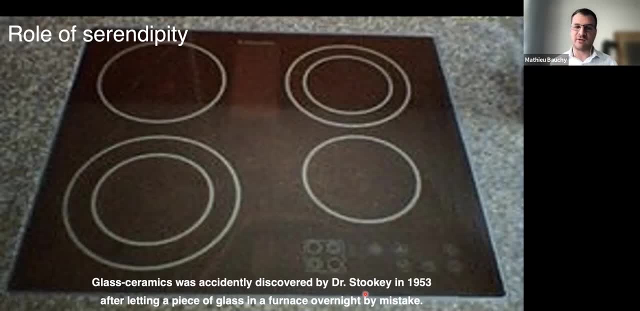 and actually didn't break when he just threw it in the trash. So then, that's the point that he realized that actually he had discovered, like something, a new way to synthesize material that can result in material being very, very tough, So material that can be used for application. 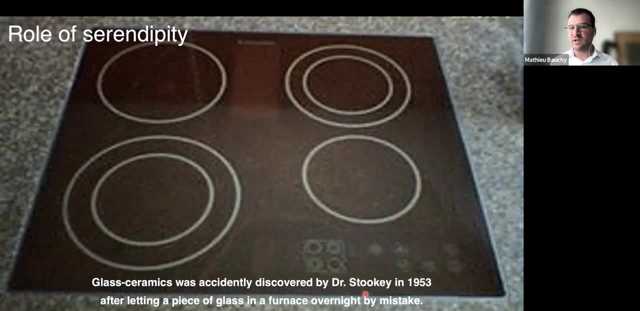 where you don't want the material to break. So that's one example where sometimes you just do a mistake or something happens by luck and you can discover this new family of materials, this glass, ceramics, that did not exist. So discovering material by luck is actually something. 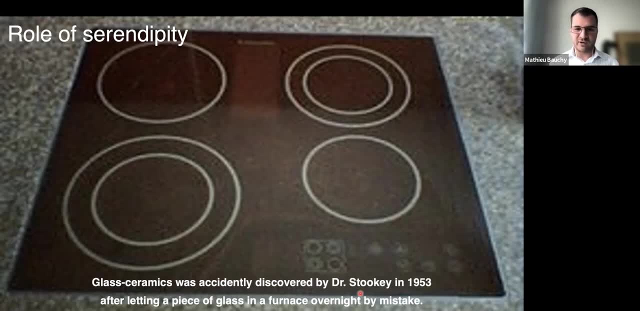 that is a pretty common way of discovering new materials, especially when it's material that you did not really envision, that you had no idea could really exist. Then it's very hard to discover those materials because you don't have any intuition about how those materials would work. 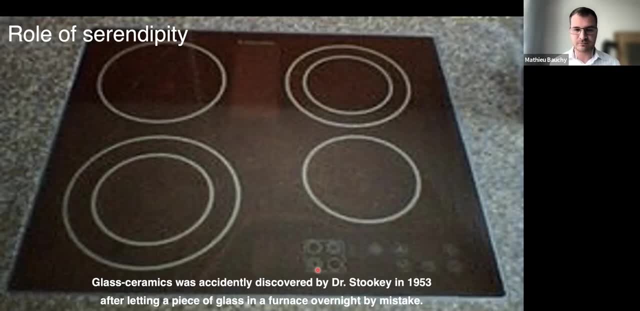 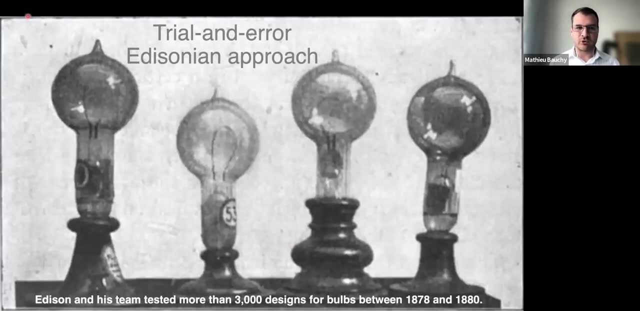 So in that case, it's very common that they are discovered just by chance. Another way of discovering new materials would be more like a trial and error approach, And so that's actually the way that Edison invented the light bulbs, And so, in this case, like what Edison wanted to have. 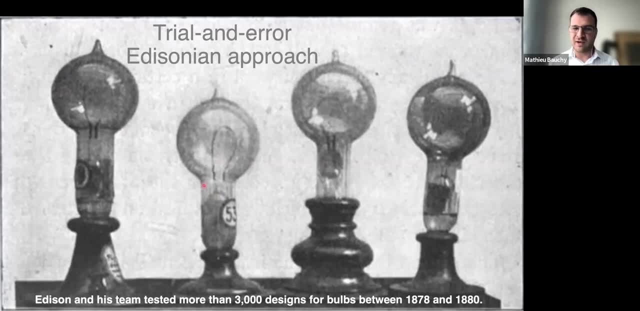 is to create a type of glass that can be used for a light bulb where you have like that you can use for light And in this case, like the type of glass that were existing before they were, they could not sustain the change in temperature. 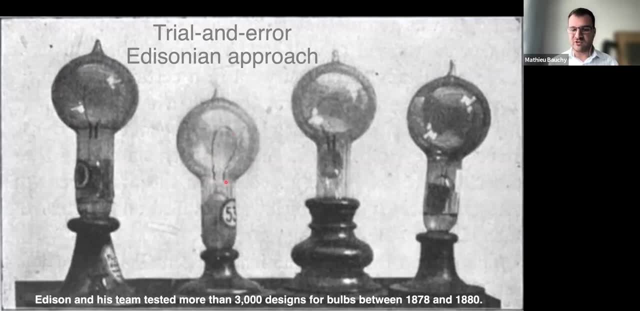 when the bulb is initially off And when you turn on the lights, like the temperature inside the bulb will increase a lot very rapidly, And most of glasses that existed at this time- if you increase the temperature too fast then that will cause the glass to break. 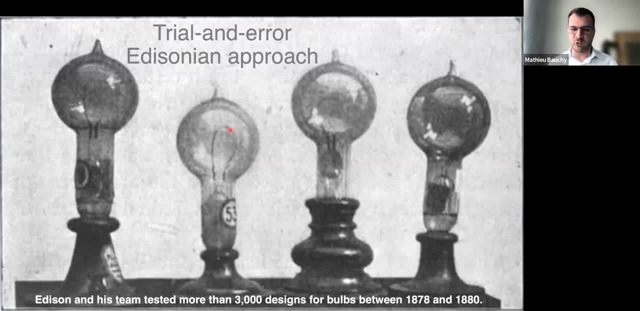 And so, in that case, to enable the design of those light bulbs, what Edison had to do is really to try a lot of different glasses, And actually, in this case, Edison did not really have any good intuition of what would be the right type of glass for this application. 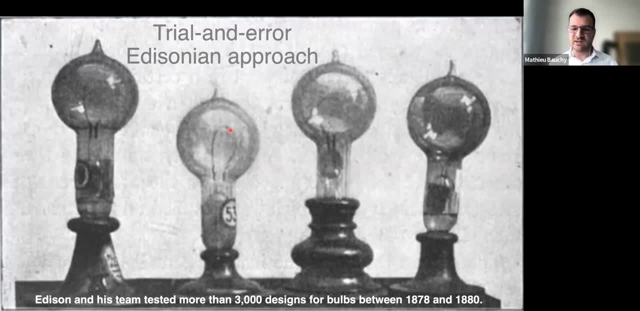 So what it simply did is just to try a lot of them. So what they did is like they spent like two to three years just trying thousands of different glasses, thousands of different design, until they can find the one that works. So in this case, so that's what we would call like now. 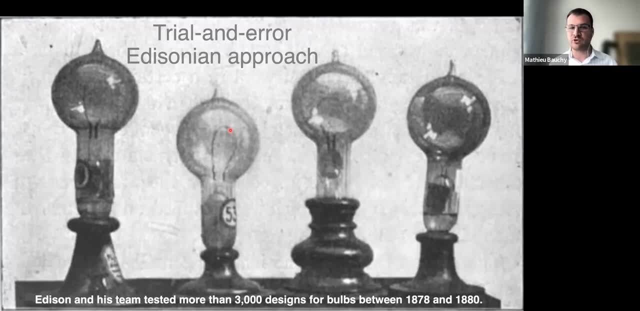 we would call it an Edisonian approach, where you just try everything, You try to change all the condition. like you try to make a new material, you change its composition, you change the processing of these materials and you just do this by trial and error. 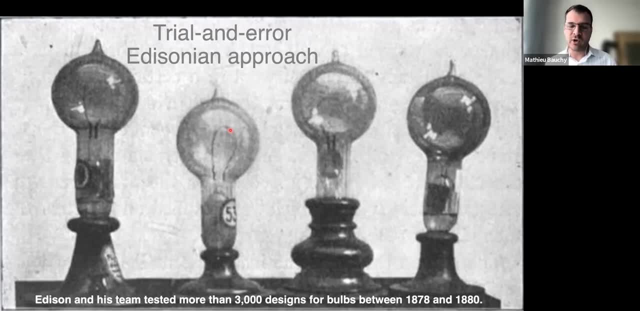 like pretty randomly, you try a lot of different combination until you can find the one that works for your application. So that would be a process that can be pretty long, But if you just try enough for a very long time, ultimately you will be able to find the material. 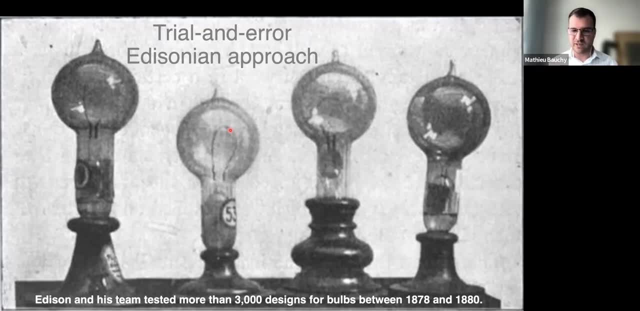 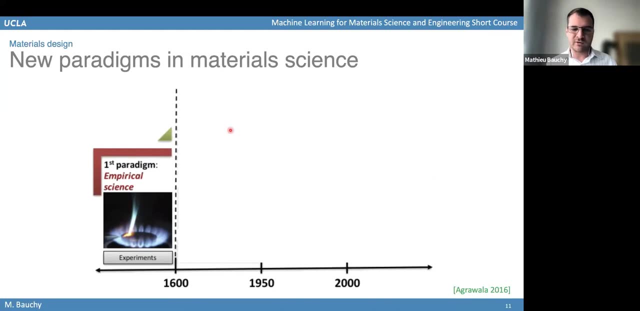 that works for the application that you have in mind. So if we want to summarize what are the different ways that you can discover materials, I would say like they can be classified in terms of four big paradigm. And so the first thing, the first paradigm, 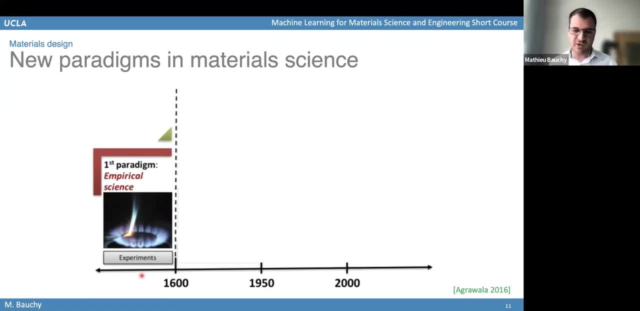 and that's the way material used to be discovered before, I would say, the 15th century- is relying on empirical science, And in that case it means that at this time, the knowledge of, for example, of thermodynamics, or the knowledge of physics, 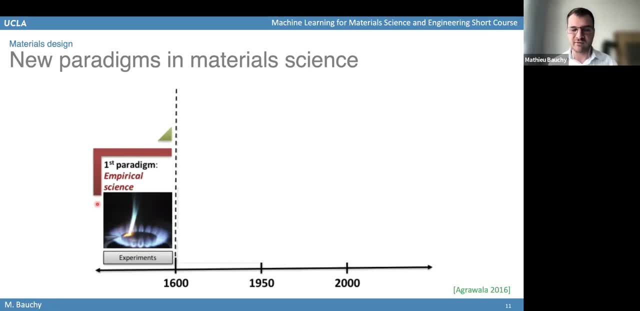 and chemistry governing materials was very limited. So in that case, at this time, we didn't have really a lot of knowledge about materials And in that case the main way to discover new materials was just to rely on empirical observation, like just to try different things. 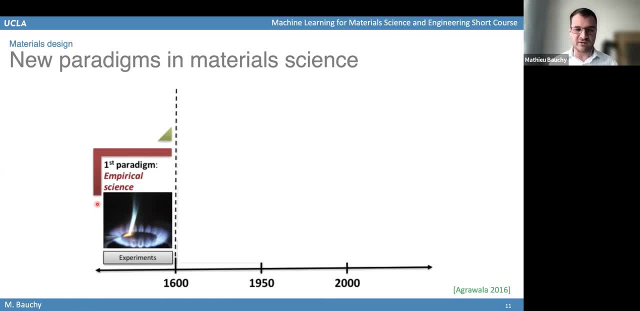 see what works, see what doesn't, and build on this experience to discover new materials, even though we don't really understand why they behave the way they behave. And that's the way materials were discovered initially, like the discovery of glass initially by the Egyptians. 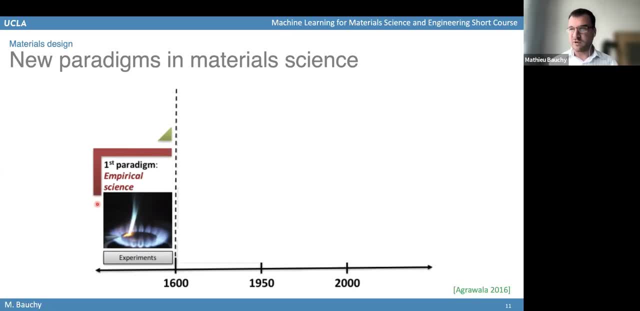 was purely based on empirical knowledge, Like they didn't have any idea of what governs the formation of a glass, but they just were able to make it, just based on their own experience, The discovery of concrete, like the, for example, Romans. 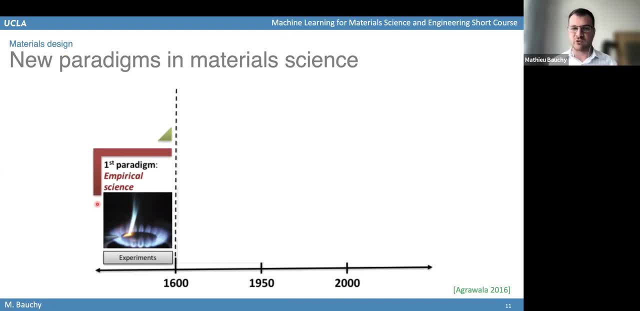 the Roman empire used a lot of concrete, like to build big structures, And this again like they had no clear idea about why concrete can initially be some kind of slurry and then gradually turn into a stone that can be used to make some construction. 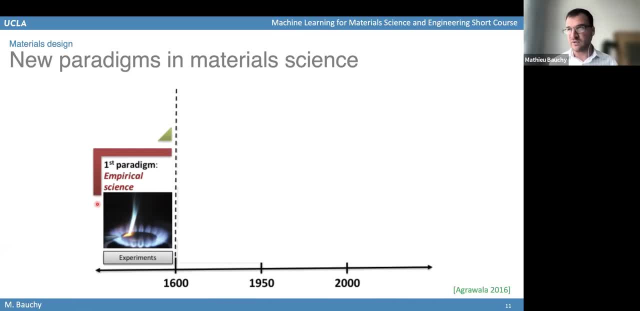 They just know it works and that's enough to use it. But they don't really understand, they don't have a clear knowledge about why concrete can gain some strength over time. So those are some examples of material that were discovered, just based on empirical experience. 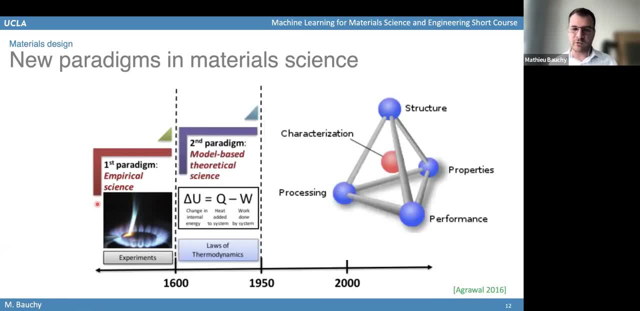 not based on knowledge. At some point, like over the more recent centuries, then there has been more progress in science, and especially more progress in thermodynamics, And so this knowledge has been used now to discover material that are based on science. So, if you're able to, for example, 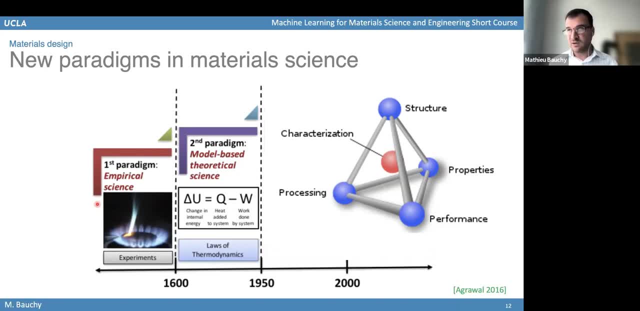 develop an equation of state for a given material. if you know how the property of a material changes as a function of temperature, as a function of pressure, then you can use this thermodynamical knowledge to discover new materials that have properties that you want. 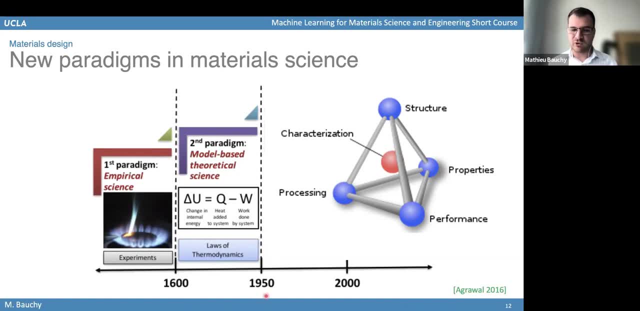 So this is more like between the 1600 to like the 20th century. there has been more knowledge being knowledge being generated by scientists, Knowledge that can be used, for example, to understand how the relationship between the structure of a materials 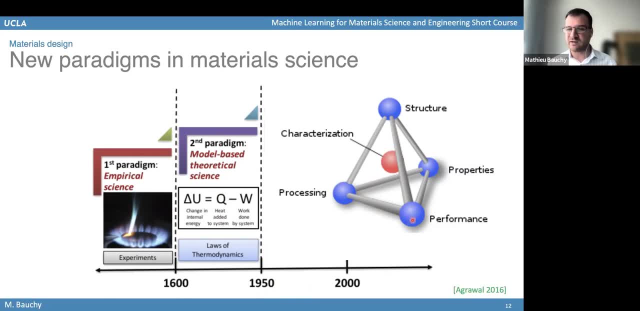 the processing of a materials and how does it impact its properties. So, like understanding those relationship between the characteristics of the materials and its property. that's something that you need, some theory in order to understand that. So that's the second paradigm in the material discoveries. 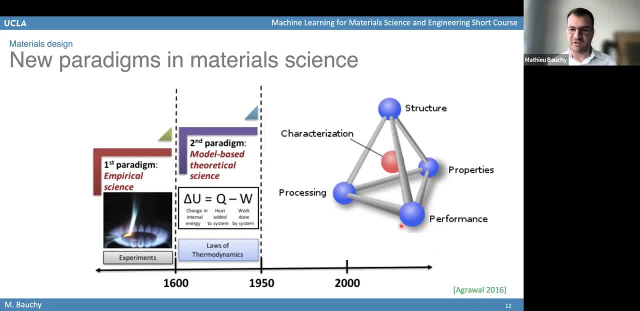 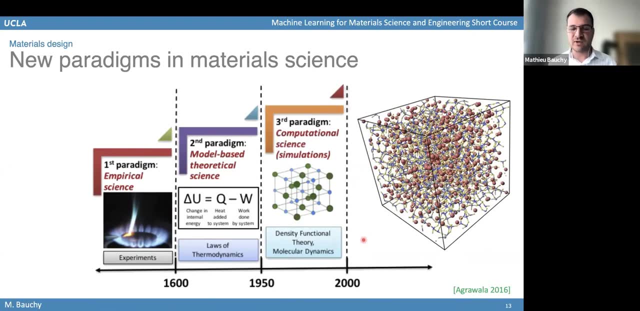 to use knowledge to discover those materials. Then a third paradigm that is more recent, like especially over the past 50 years, is to use simulation, to use computational material science, And that's something that has really been enabled over the past decades by the fact of having 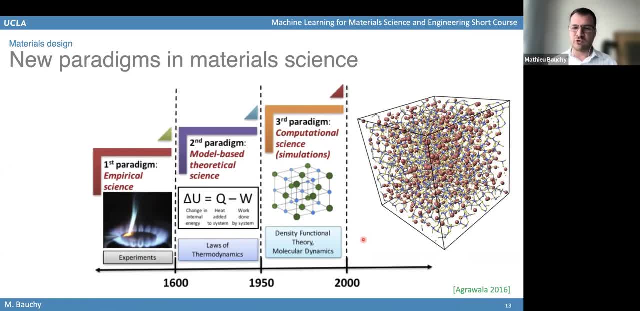 more and more powerful computers. Now we can use those computers to simulate materials, And that way it can make it much faster to discover materials, because it means that you don't have to necessarily synthesize a lot of materials and then test them in order to find the material that you want. 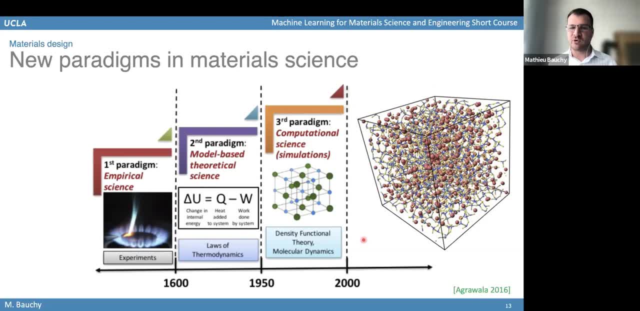 You can simply simulate them. So you can simulate them on a computer and use this computer to compute what would be the property of different material that you are simulating And then, based on that, you can use the simulation to really pinpoint what would be the most promising materials. 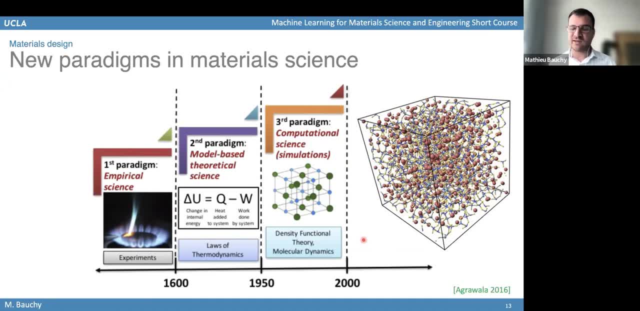 without having to test them in practice. So that can really accelerate the process of discovering new materials. because rather than just synthesizing thousands of different materials, then it's much easier, much faster and much cheaper to just simulate thousands of materials and really limit. 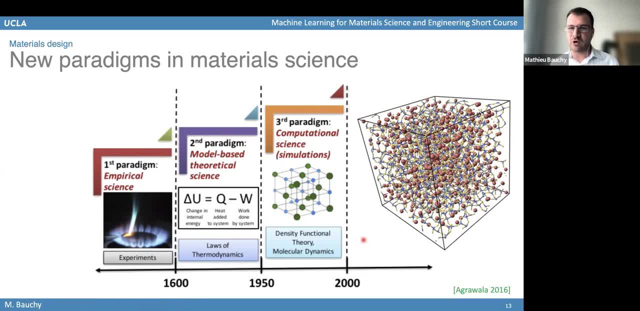 the experimental synthesis of materials to a lower number of materials that you have found to be promising, based on some simulation. So this would be the third paradigm of material discovery: It's using simulation, using computational material science. So, when it comes to computational material science, 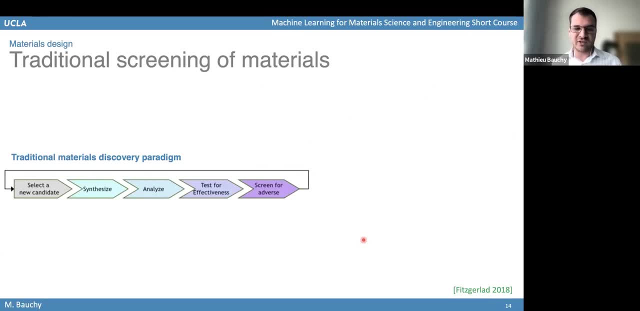 and using simulation. the big advantage of this is that you can bypass the traditional material discovery pipeline. So, like the traditional way to discover materials, as we mentioned before, is that you just select a candidate, So you select a given composition, You select some given condition. 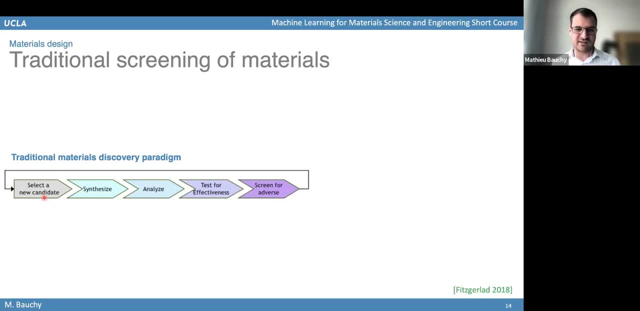 like the temperature, pressure, pH, et cetera. And then you try synthesizing this material. You measure a property and then you test if the property meets your constraints, meets your objective or not. And if it meets your objective, 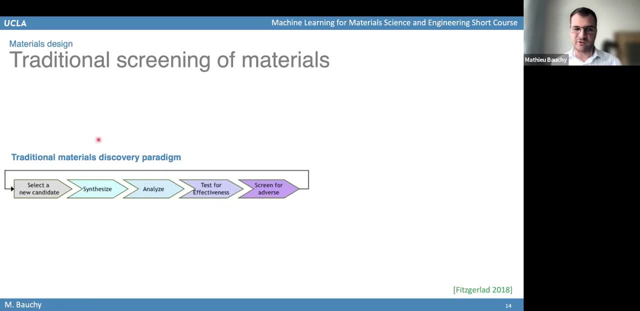 then you're going to keep this material. If not, then you're going to go back, loop back to change something in the way you make this material. So that's the traditional way to discover materials. But what can be different if you use simulation? 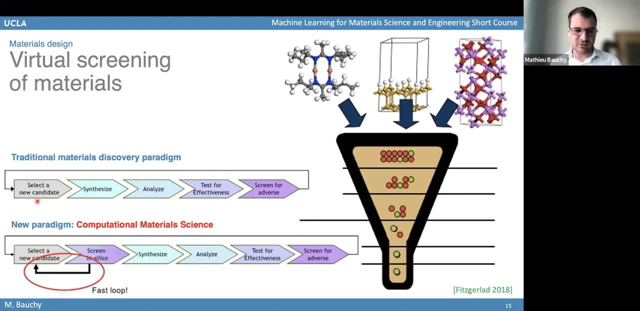 is that you can iterate much faster Like, rather than going for this entire route here, which takes a lot of time and will take at least several hours before you can select a new candidate, just because synthesizing a material is long and testing a material also takes a lot of time. 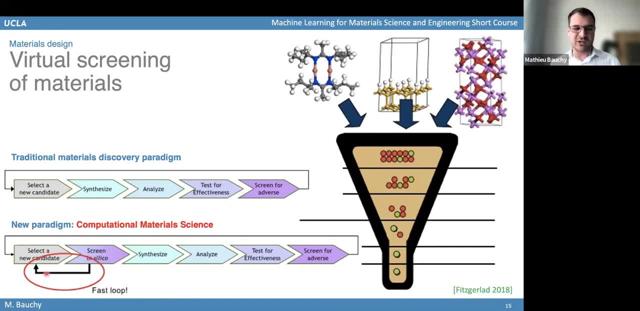 So this loop would be pretty slow, But if you are simulating a material, then it becomes much faster because you can again select a given candidate. So select a given set of condition or a given composition for your materials, And then you can directly simulate this. 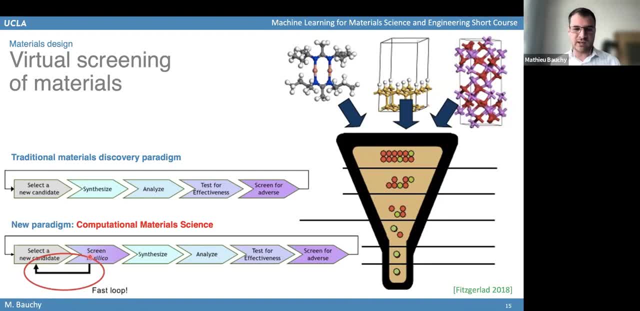 So you can simulate this material and quickly figure out if this material looks promising or not. If this material doesn't look promising, then you know, you don't need to synthesize it, You can directly move to a new candidate. But if the simulation predicts, 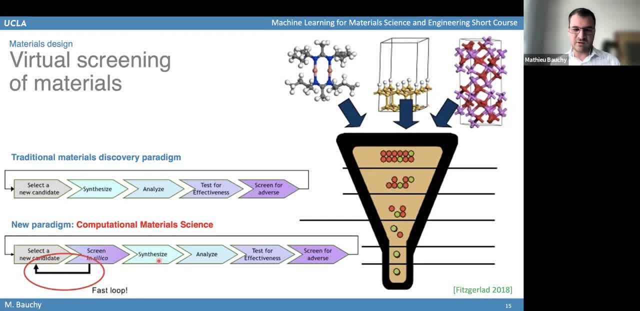 that this material looks promising, then you will synthesize it and test for its property and decide if you want to keep it or not. So by having the ability to simulate materials you can really accelerate the way you discover materials, because you don't have to synthesize materials all the time. 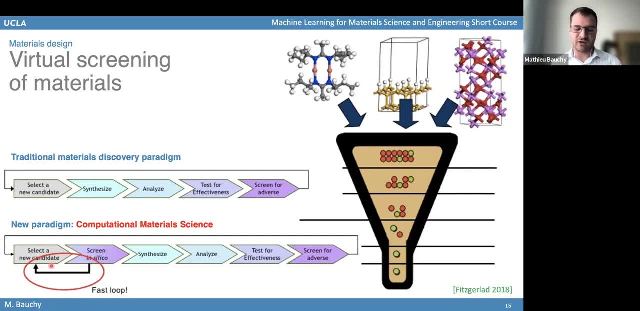 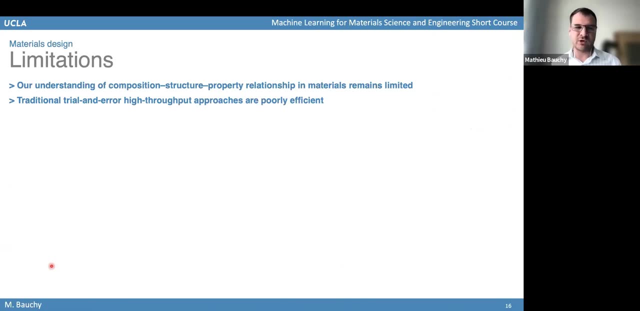 You can just disregard very quickly materials that are not going to be very promising, So you really focus your experiments on the most promising materials. So, even though that sounds good, there's still some limitation behind this, because the first thing is that if you want to use knowledge to discover materials, 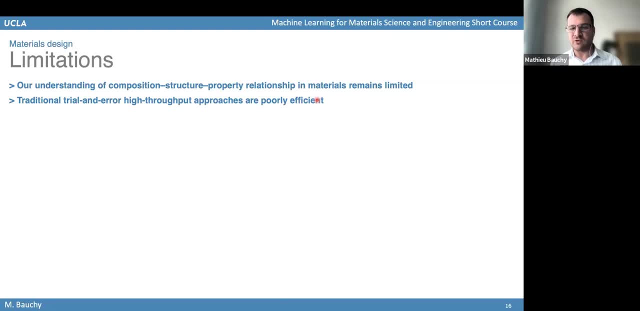 then well, sometimes you don't have this knowledge, So this knowledge is not always available. So if you don't have enough knowledge about how the composition or the structure of a material impacts its property, then you cannot use this knowledge. And when you don't have this knowledge, 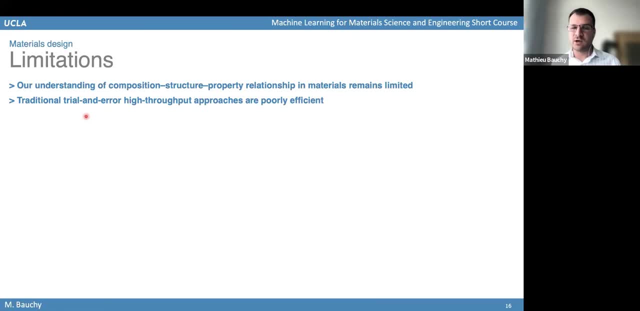 and if you just want to use trial and error, so just try a lot of potential candidates and see what works and what does not. this is something that can still take a lot of time because, like if you, for example, if you want to discover a new glass- 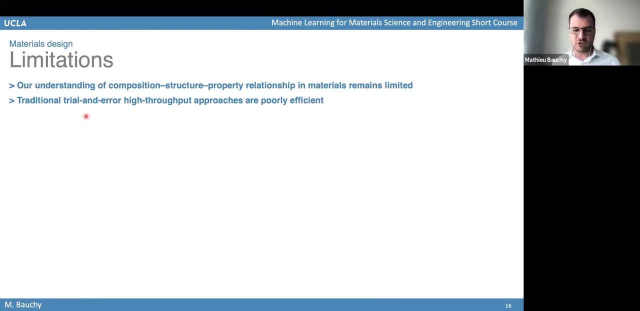 and you are going to try different potential composition for this glass, like different oxides that you are going to melt in your glass, then you really have a lot of choices, Like you can pretty much put the entire periodic table inside your glass. 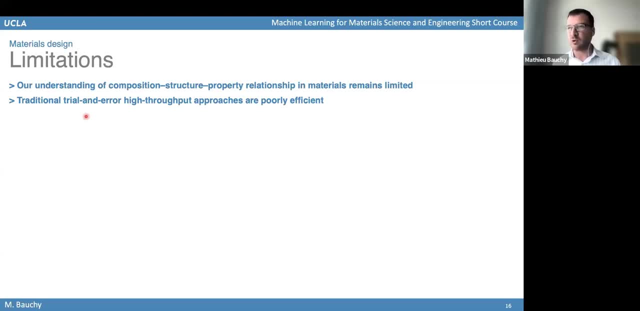 That would be a very, very high number of potential combination, potential composition for your glass. So you would have like billions of possibilities. So you cannot just try all of them one by one. That would take a lifetime and probably more to come up with the best solution. 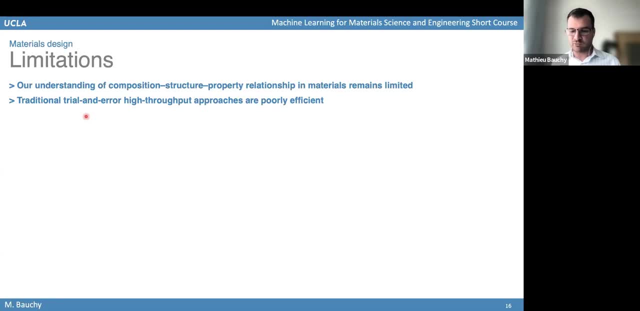 So if you have a very small number of parameters that you can change in the way you make a glass, then it's okay to just to try all of them and just to see which one works, which one does not. But if you have more parameters that can change, 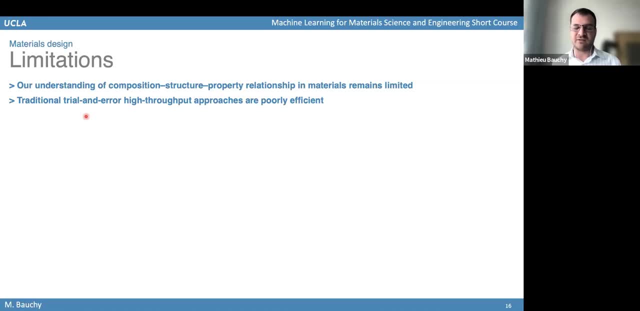 then just using this traditional, like Edisonian approach and trying all the possibilities would be a very slow process, very poorly efficient process. So we need to find some other ways of discovering new materials And well, as we would see, machine learning will be a very efficient way. 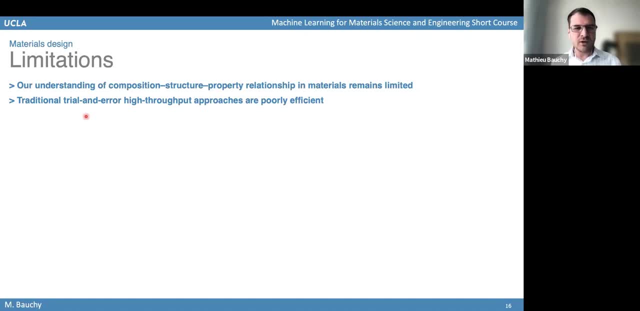 to accelerate this process. So let me illustrate this. So let's assume that you want to discover a new material. So if you want to either find a material that will have the best possible properties or just discover a brand new material that you have never worked with before, 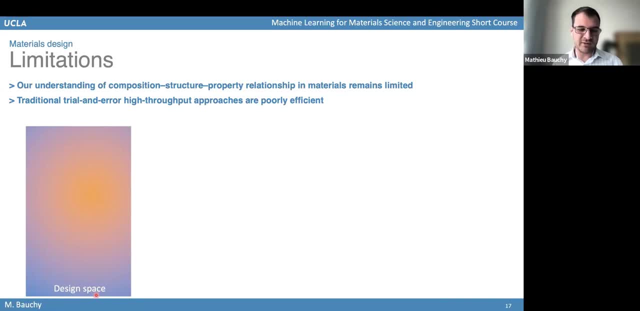 the way you have to do that is, you have to explore a given design space. So what I mean by design space is the design space is going to be the list of all the parameters that you can change in the way you make a material, So you can think of the fact of making a material. 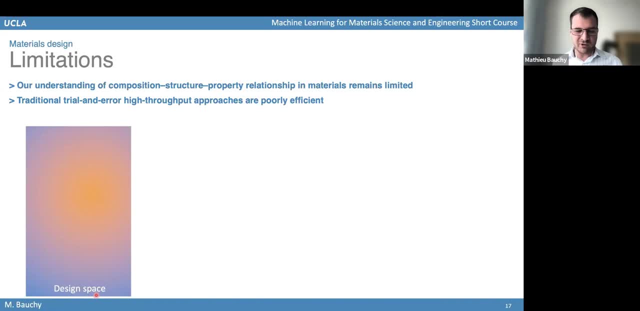 it's the same as cooking a cake. You have a given recipe to make this cake, So the recipe will involve, like, some raw materials, like, for example, you can put some flour, some milk, some butter, et cetera, So you have different ingredients. 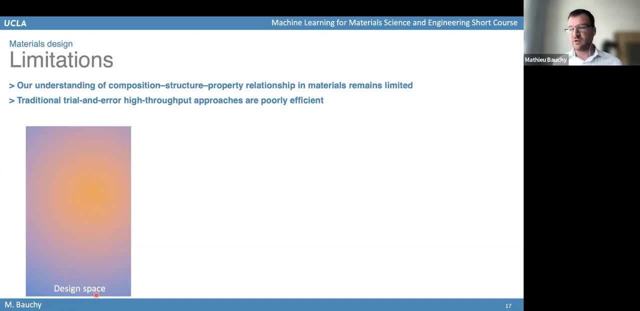 that you can put. So, in that case, the parameters that you can change is: what are the ingredients that you are going to put inside your cake And what are going to be the fraction of all those ingredients? Like are you going to put, like, more milk? 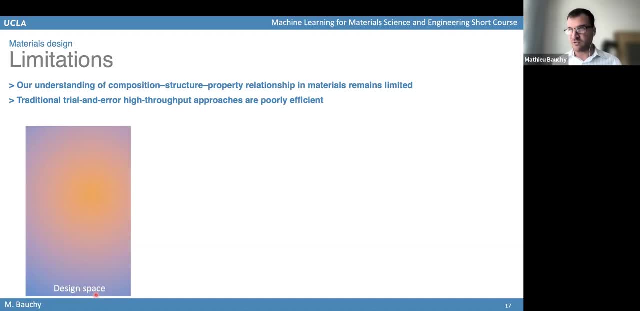 less milk, et cetera, more salt, more sugar, So you can change the fraction of the materials that you can put initially in your recipe. So that would be one example of design parameter, And then you can change the parameters and you can change the processing. 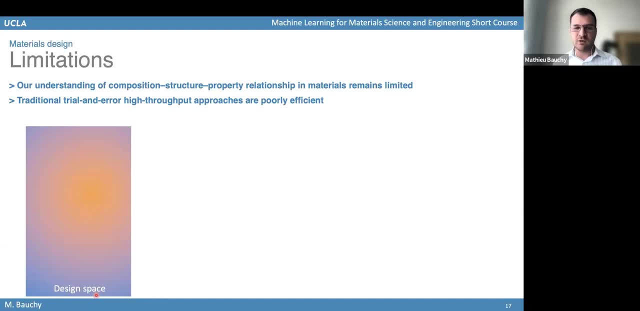 You can change the temperature at which you're going to cook your cake, You can change how long you're going to cook your cake, et cetera. So you can change when it comes to material, you can change the temperature, you can change the duration of the processing. 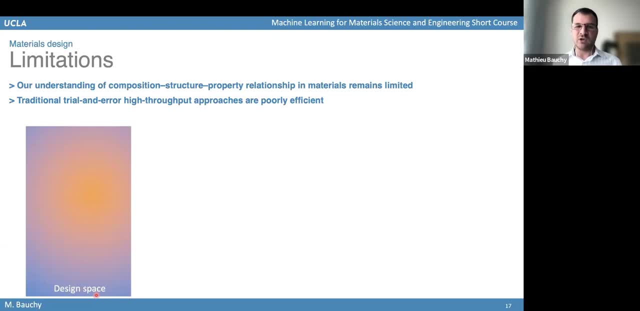 of the annealing. you can change the pressure, et cetera. So you have a lot of parameters that you can change. So the design space would be the list of all of those parameters, either the composition of the material that you're going to use. 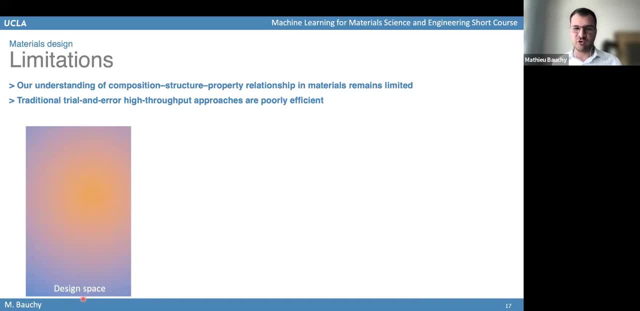 or the processing temperature, processing pressure. So this is a list of different parameters that you can change, And so this can be represented as a space where the axis of this space would be the parameters, would be the composition, would be the pressure, et cetera. 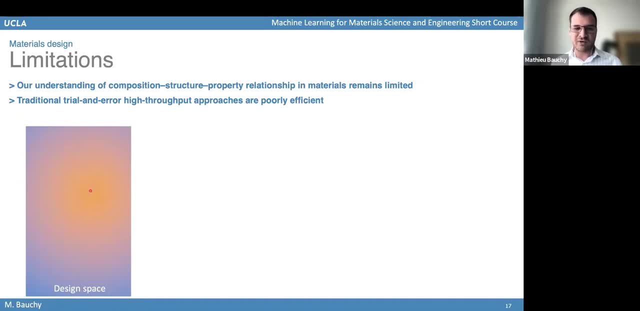 And so what you want is to explore this space to find what would be the combination of all of those parameters that will give you the best possible material. So it's like you are: you have a given space. In this case, it's a pretty highly dimensional space. 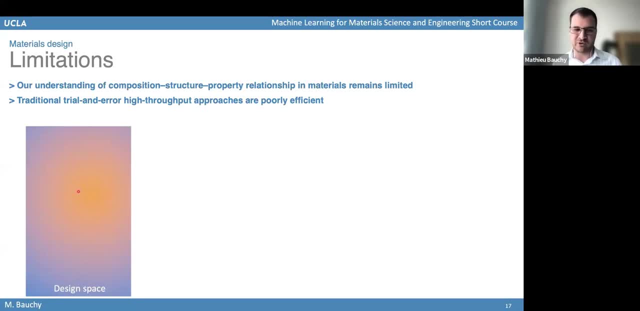 It's not simply a three-dimensional space, because you have a lot of parameters that you can change And you want to explore this space in order to find somewhere here, like this orange area would be, for example, the position in this space where the material will have the best possible properties. 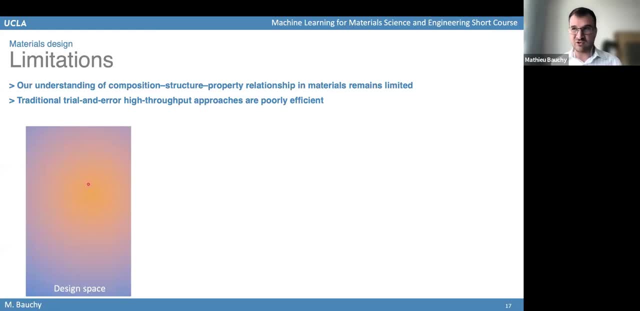 And so the question is: how do we explore this space as efficiently as possible? How do we find the sets of parameters that will give you the most promising material? So one first way to do that is to find this optimal material here, which I represent as a star here. 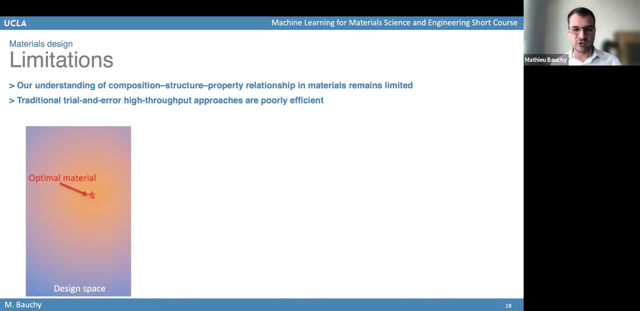 So this is the optimal material. Initially, we don't know where this material is. We want to explore this space to find this star material here, And so one first way is to just do this, this onion approach that we talked about, this trial and error approach. 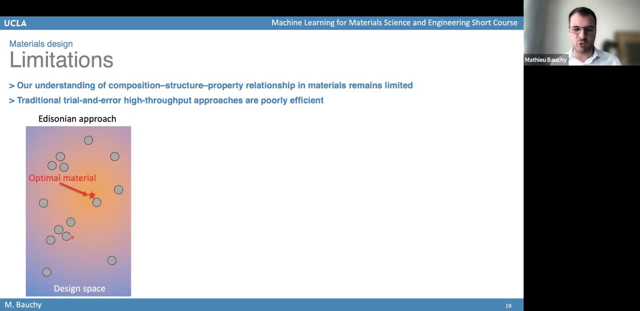 And in that case what you will do is just a lot of random trials. You will explore randomly this design space and try many combination of your design parameters until you can find one combination of parameters that will give you something that is close to the optimal material. 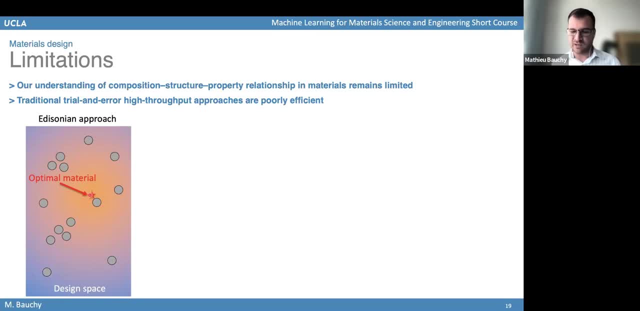 So that's one potential way to explore the design space is just by trial and error, just trying, trying, trying until you find the right combination, And so this process eventually is going to work if you are just very patient And if you try for a very long time. 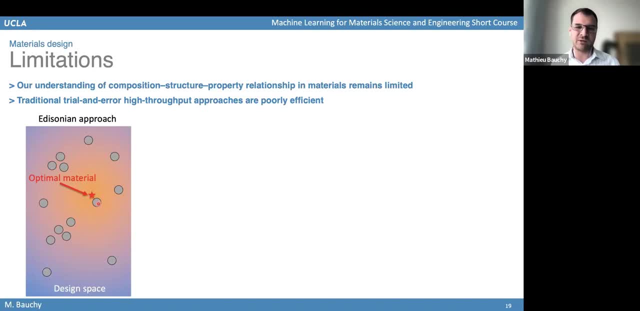 at some point it's going to work, you will find the optimal process, But that can be something that can take a very long time. It can take many iterations, like thousands or millions of iterations, until you find the right material, The other approach. 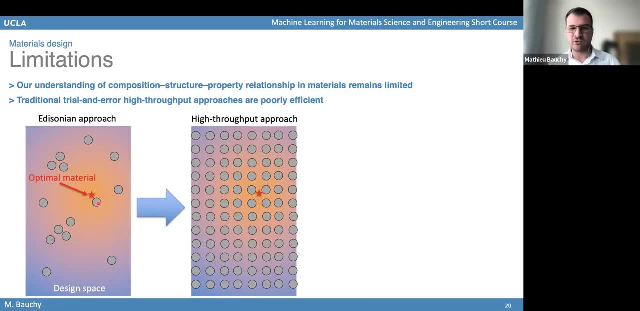 and especially that's something that you typically do when you do simulation- is to do a high throughput, high performance approach where, rather than randomly exploring your design space, you are going to systematically explore it, So you're going to fix all the parameters. 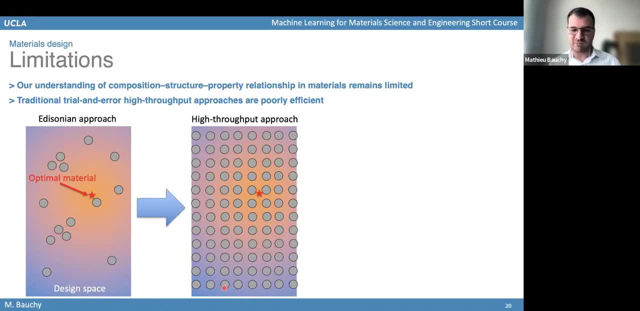 and take one parameter and change it systematically. For example, you will fix everything but just change the temperature at which you're processing the glass, And after that you will keep all the parameters fixed and you will start changing something else. So you will start changing the pressure. 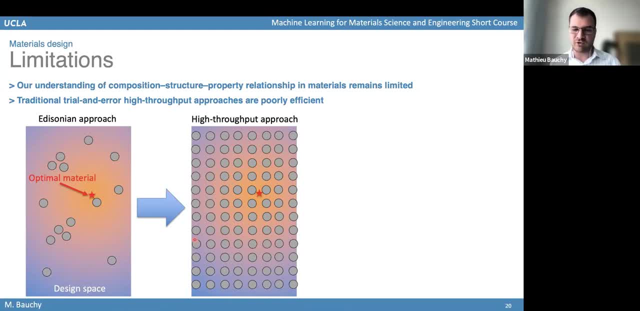 where now you will fix the temperature and change the pressure that you use when you synthesize your materials, And then you will repeat that, where you iteratively either change the temperature or the pressure, and you will do that for every possible combination of pressure and temperature. 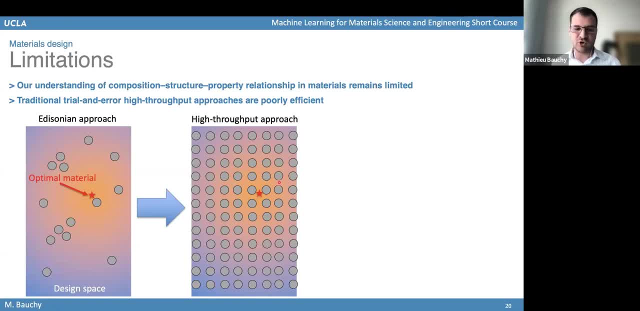 or every combination of composition, or you will just change all the parameters in your design space in this high throughput fashion And you just try all the possible combinations until you find the material that you were looking for. So in that case that's also a process. 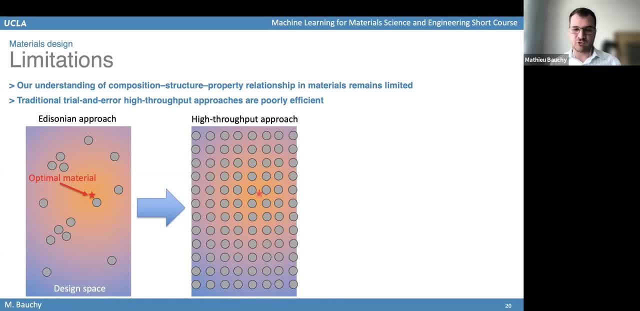 that eventually is going to work Like if you just try every combination, then necessarily at some point you will find the best combination. But this again is something that can take a lot of time because you really have to try many, many combinations. 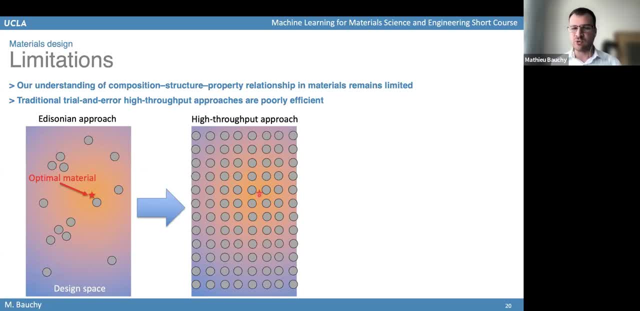 until you find the best material. So that's something that you can do if you are using simulation, because using simulation we can really simulate thousands or maybe even millions of potential candidates in a very fast fashion. But if you are going to do that experimentally, 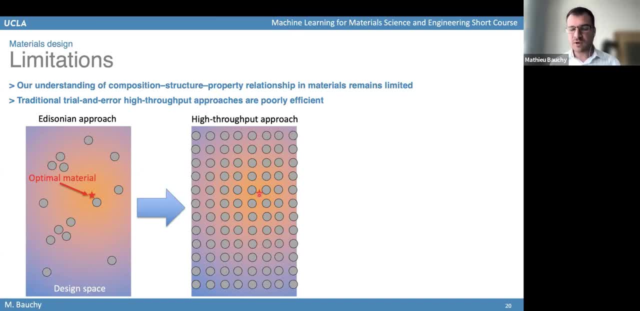 then that would really take a very long time. So the last option is: what is the promise of machine learning? The promise of machine learning is that you can accelerate the way you design materials. You can use the knowledge that you generate as you design new materials. 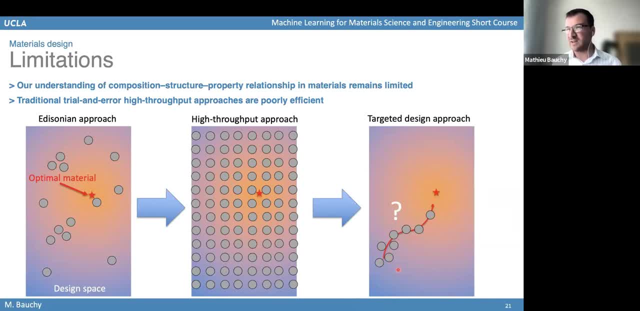 and use this knowledge to discover new materials. So in that case, the promise of machine learning is that, rather than just exploring randomly or systematically your design space, then machine learning will tell you in which direction you should go to find, as efficiently as possible, your optimal material. 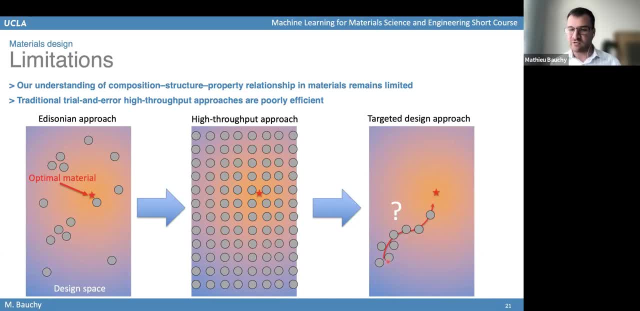 And in that case the main idea of machine learning is that you will start initially to try different materials pretty randomly And as you make those materials you will generate some data. So you will generate some data sets about four different materials. You will have both their design parameter. 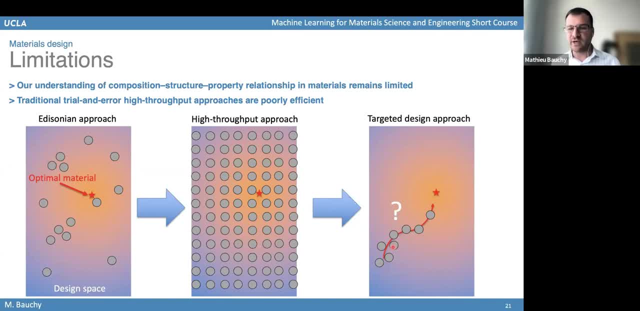 like the temperature, the pressure, the composition, etc. together with the measured property. So you will have more and more data about those materials as you generate them, And then what you will do is use this data and use this data to train some machine learning model. 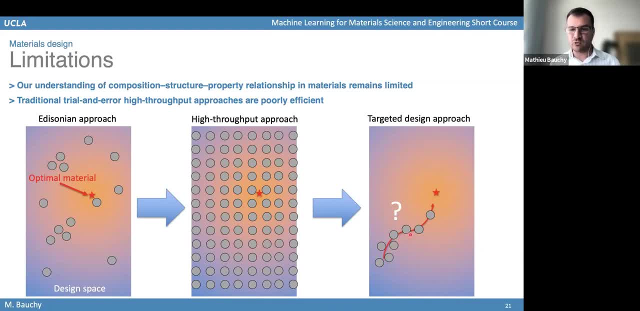 And the machine learning model will tell you what should be the next material to try. So, in that case, that's the promise of machine learning- is that it will tell you which material to try next, based on all the data that you have accumulated so far. 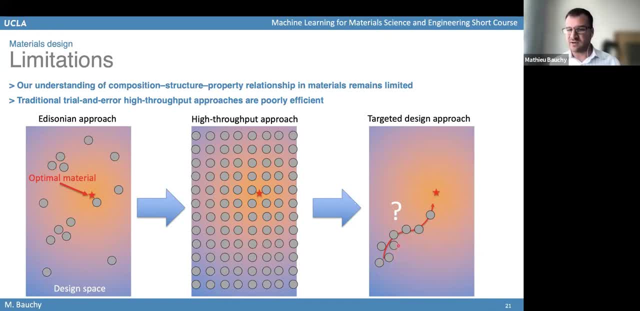 And in that case so that's an efficient process because it can guide you towards the most promising materials by minimizing the number of experiments that you need to get there. And that's also a very powerful process, because this process of discovering materials with machine learning. 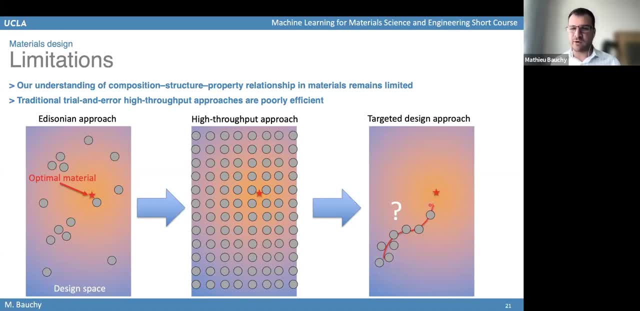 does not require knowledge. It doesn't require you to understand some physics or some chemistry about the material. You just need some data. You just need to start synthesizing materials, measure their properties and then use this data with some machine learning to predict what should be. 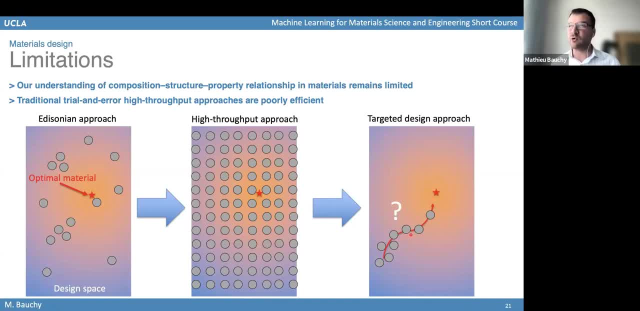 the next material that you are going to use, And that's something to try. So it only relies on data, not on knowledge, And that's something that makes it very efficient, especially when you don't know yet any knowledge about materials. So that's mostly. 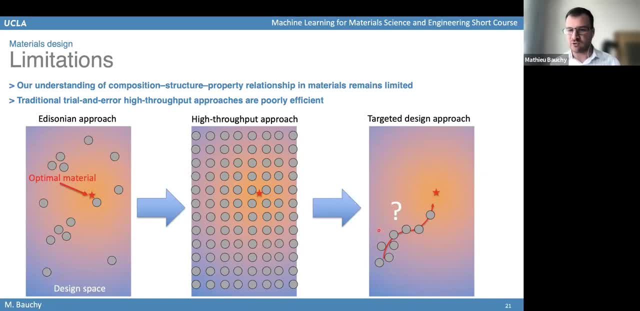 what we are going to talk about today is how we can use these types of machine learning techniques to discover new materials or optimize materials or find materials with optimal properties as quickly as possible, without having knowledge or without having to just simulate all the potential combination of materials. 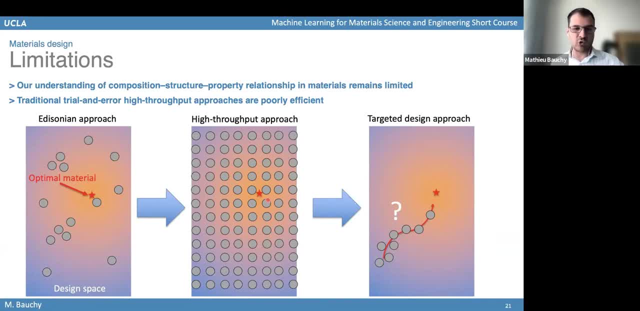 that you can have. Do you have any questions so far? Okay, So just as a reminder, if you have any questions that come in, just feel free to ask as we go. You don't need to wait for me to stop talking or anything like that. 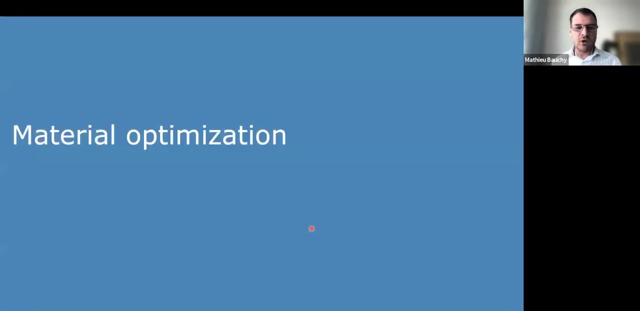 Just feel free to ask questions. Okay, So now let's go to a new part, which is: like: how do we use machine learning for the process of optimizing a material, So like in this case, like the idea is that you want to come up. 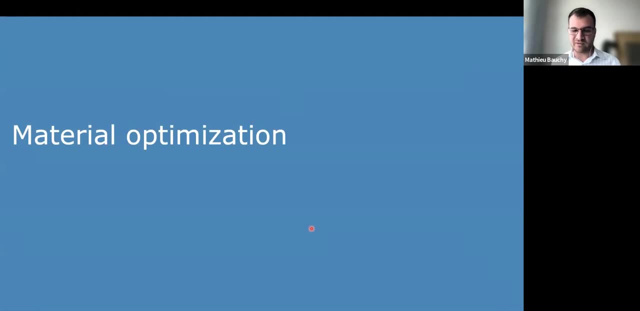 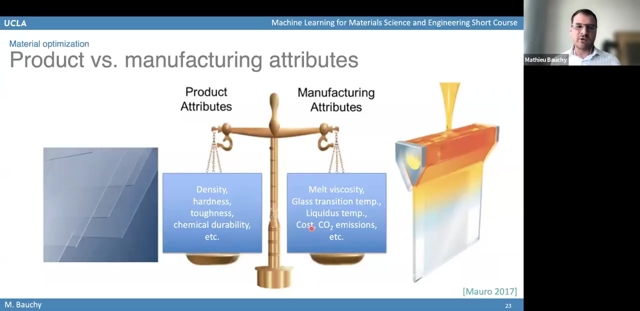 with a new material that has better properties than existing material, And in this process is called material optimization. You want to optimize something in a given material, And the question is how to do this as efficiently as possible. So when it comes to optimizing a material, 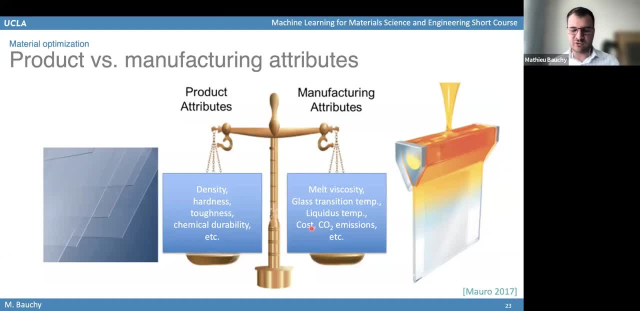 there is always a balance between different things. So here I'm taking an example of a glass, but this is true for any types of materials is, if you want to change a given materials to make it more appropriate for a given optimization, you have a balance. 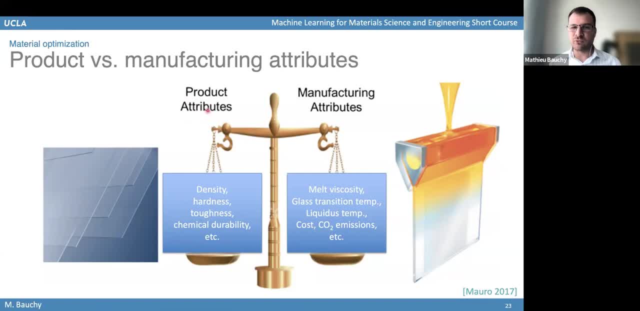 between two things. First, you have the product attributes. So the product attributes are going to be the properties of the materials that are going to be, that are going to make this material useful for a given application. So, for example, if you come up with 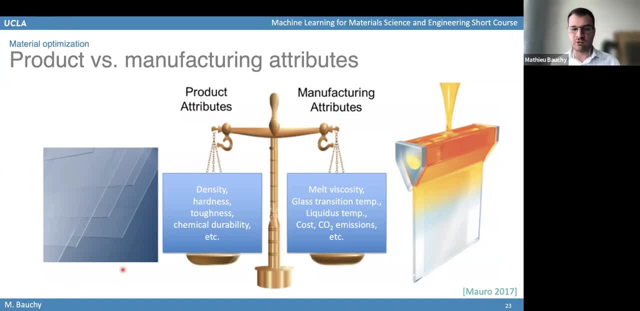 for example, let's say you want to come up with a new glass that you can use to make a screen for your smartphone. So in that case, as a consumer or as a glass producer, you will want this glass to be as light as possible. 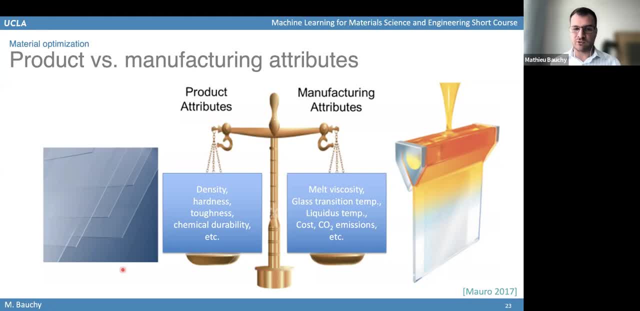 so that it doesn't make your phone too heavy. So you will want to potentially minimize the density of the glass. So in this case, you may want to have a glass that is as hard as possible so that it's hard to scratch Like you cannot scratch. 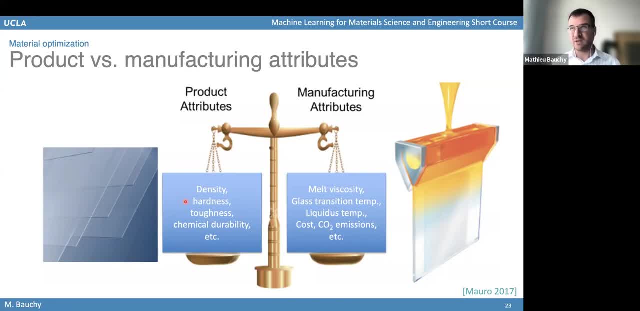 this glass and make some big scratch if you put your phone and your keys in your pocket, Like you don't want the keys to scratch your phone. You want the glass to be as tough as possible, Like if you drop your phone. ideally you don't want. 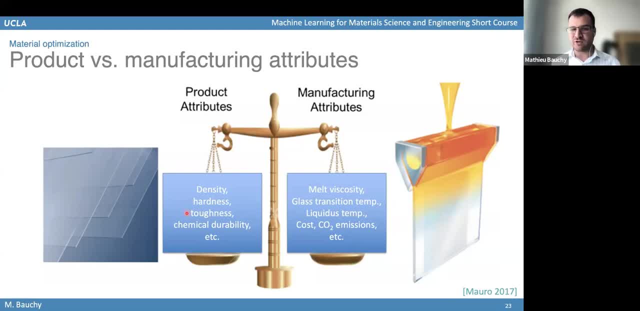 the glass to break, So you want to have a toughness that is as high as possible, And you want like also a high chemical durability. You don't want the glass on your phone to start dissolving if it starts raining, So you want to have 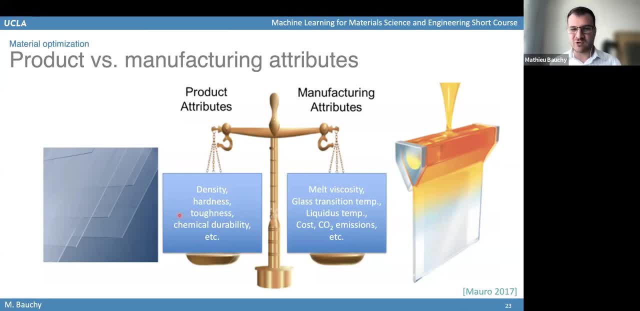 a good chemical durability. So those are the attributes about the product itself. Like a given material will have certain types of performance attributes which will make it possible to use these materials for different applications. So those are the properties that dictate the performance of the materials. 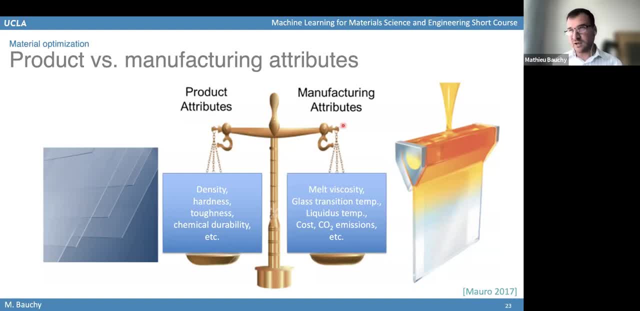 for a given application. But then, even if you have a material that has a very high performance, you still need to be able to manufacture this material. So this is going to be the second type of attributes. Those are the manufacturing materials. So, those manufacturing materials, 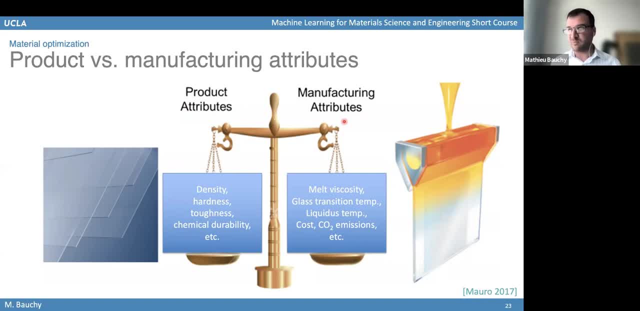 they do not dictate the performance of the materials, but they dictate whether in practice, you can manufacture these materials or not, Or they dictate how expensive is it going to be to make these materials. So, for example, when you make a glass, there's a couple of things. 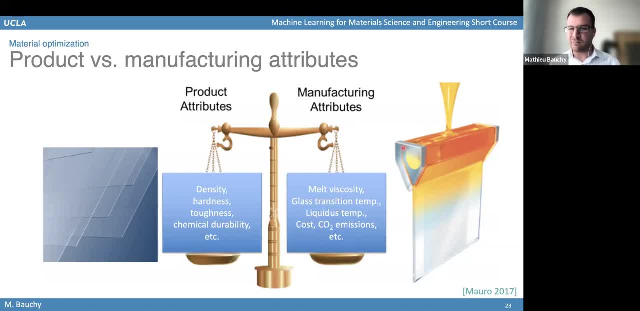 that are very important, like the viscosity of the melt at a given temperature, the glass transition temperature, the liquidus temperature, like the temperature at which you need to heat material to melt them. So those are all properties that, as a consumer, you don't care about. 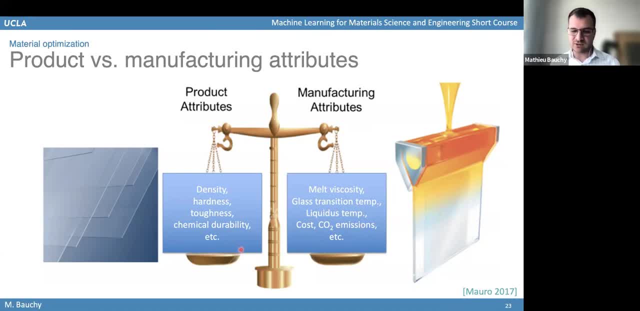 Like, if you want to just make a glass to use as a smartphone screen, you don't care about the glass transition, temperature or things like that, But still, if you want to be able to make this material, then you need to make sure that this material 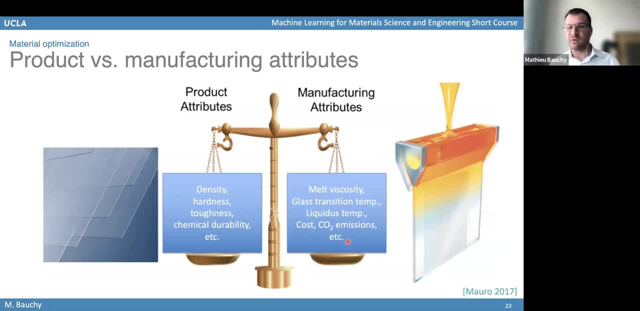 will be able to be made. So you need to make sure that this material will be processable, that it won't be too expensive to make this material, or that you can make it using the material that you have at your disposal, So when you want to come up. 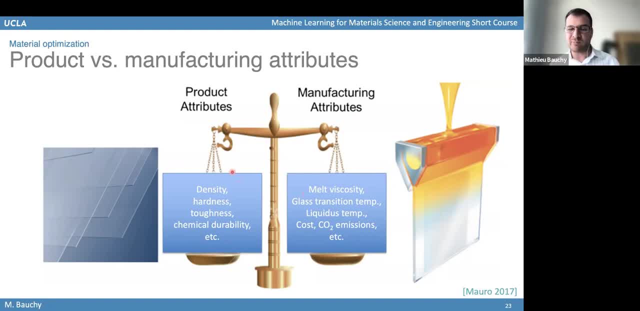 with a new material. very often you will have to find the right balance between maximizing the performance of the materials, but also ensuring that these materials can be made in practice and that it won't be too expensive to make these materials. And very often, 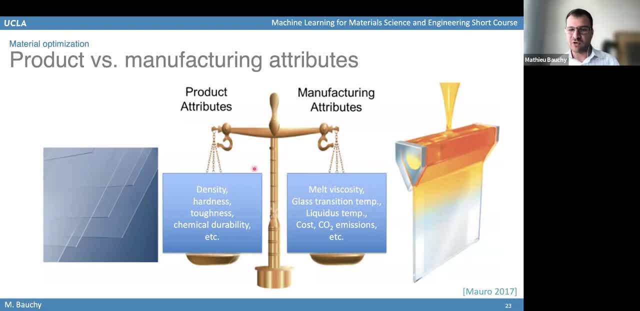 it's a competition between those two things, because usually when you increase the performance of the materials, then it means that it's going to be more challenging to produce these materials. So very often you will have to find the right balance between those two things. 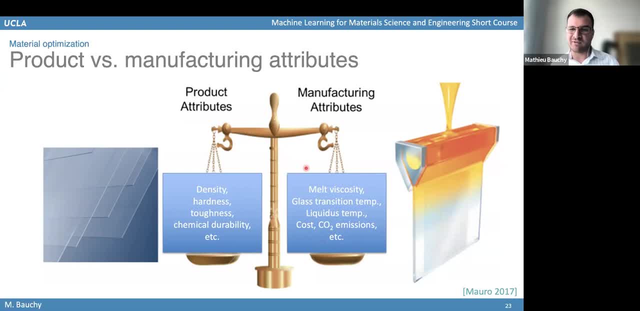 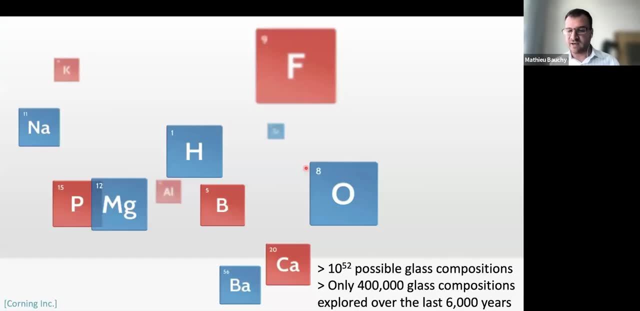 So finding the right balance between the performance of the materials and whether these materials can easily be manufactured or not, that you can summarize this as an optimization process. So, for example, if I again I take an example of glasses, is you want to come up? 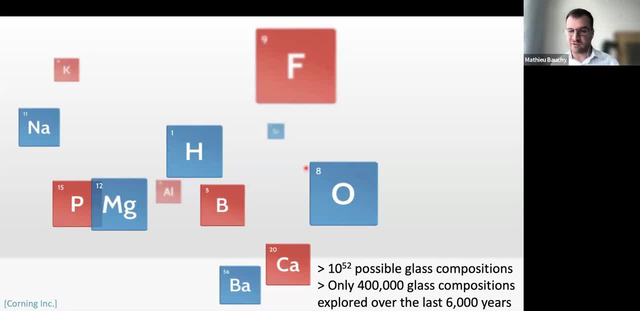 with a new glass that will be very tough, like a glass that would be very resistant to fracture, And in that case what you can do to change a given glass is change its composition, So you can change. you can take pretty much any element of the periodic table. 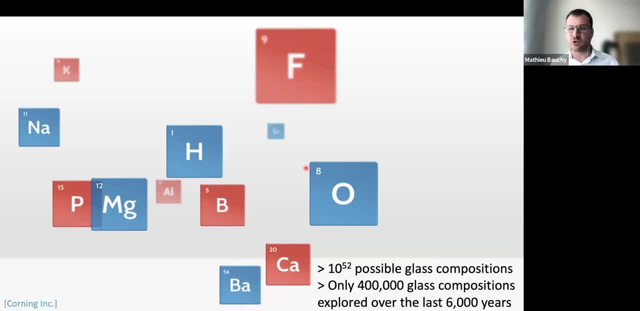 put it in a furnace and melt it and then quench it very fast and form a glass out of this. So you can take all the elements of the periodic table, pretty much mix them with different fraction and form a glass out of this and see then if the glass 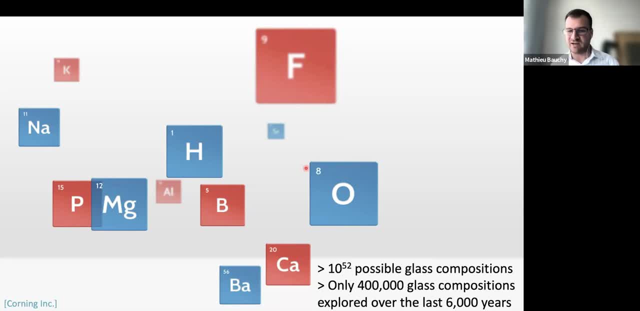 is going to be performing as you want, or if the glass is going to have a high toughness, for example. The problem with that is that, like there is a very large number of possible composition, For example, if you just take glasses and if you just assume, 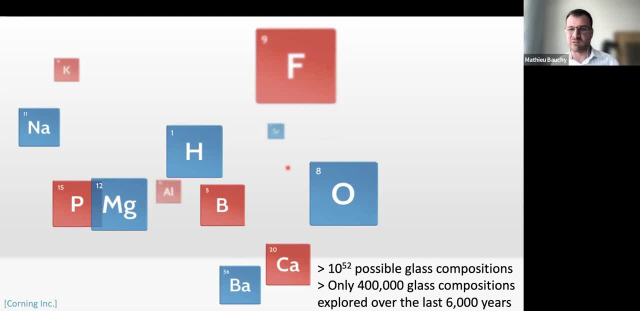 that you can just put all the elements in the periodic table into this glass. then you have like this very astronomical number, like 10 to the power of 52 possible glasses. So that's a very high number of possible glasses that you can make. 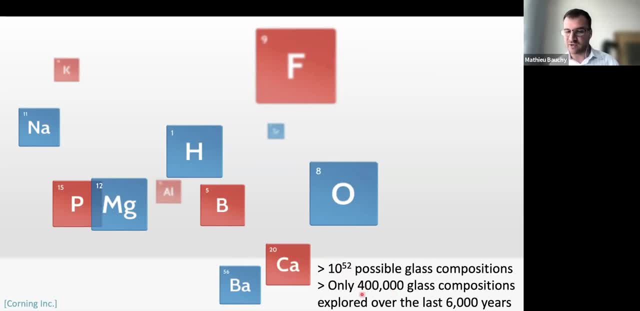 And so far, like even since the beginning of history. like the number of glasses that humans have been making over the past centuries is really a very small fraction, Like the number of glasses that have been made is probably around 400,000, which is a pretty high number. 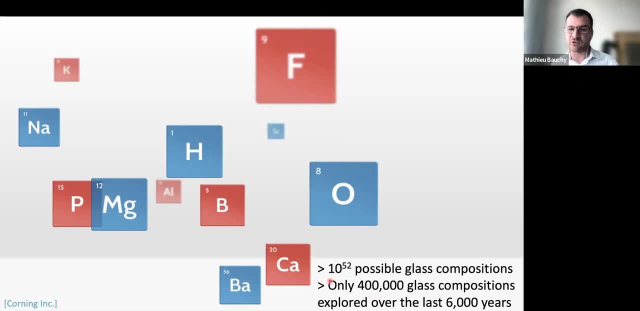 but it's still like very, very small as compared to the number of all the possible glasses that can theoretically be made. So it means that there is still a lot of room to discover new materials, because the types of material that we have been exploring so far 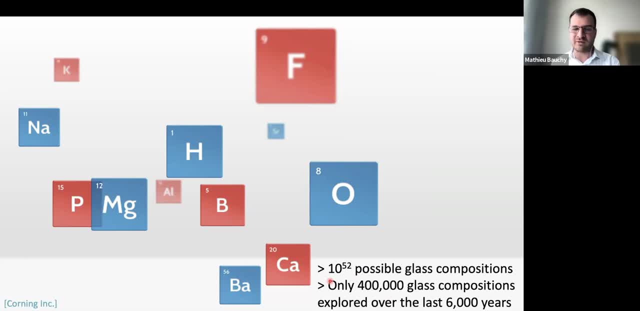 it's really a very small fraction of all the material that you can think of that can possibly theoretically be made, But like there is so many possibilities that it's a very complicated process to discover new materials because you don't know necessarily where to start because there's so many. 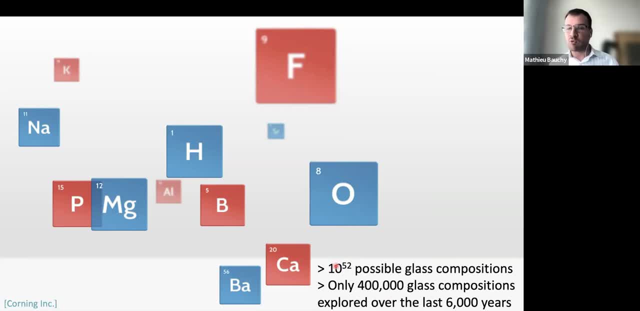 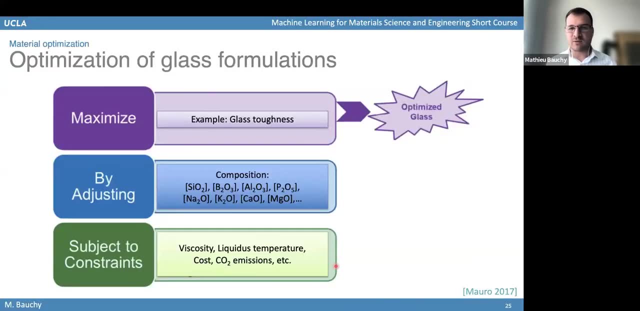 different possibilities that it's very hard to know where should we start when discovering a new material. So this can be formulated like, more mathematically speaking, as an optimization process. So, for example, if I come back to the example of glass, you have a given objective. 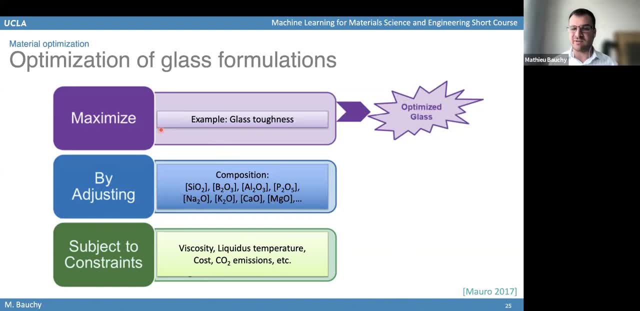 that's the objective of, like the material that you want to discover. Like, for example, you want to discover a glass with a very high toughness, a very high fracture toughness. So in that case, that would be your objective. You want to maximize. 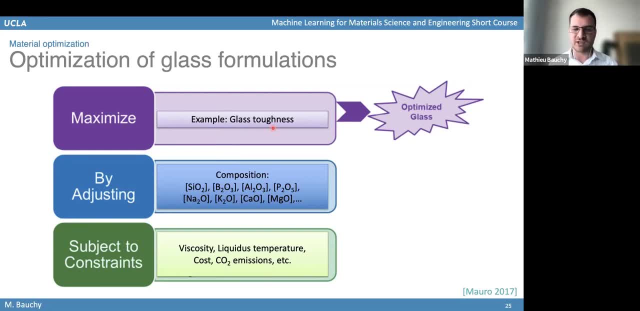 the fracture toughness of your glass. So that's the objective function of your optimization. Then the way you can maximize this is by changing some degrees of freedom. So, for example, in the case of glasses you can just take different oxides like silica, B2 of freedom. 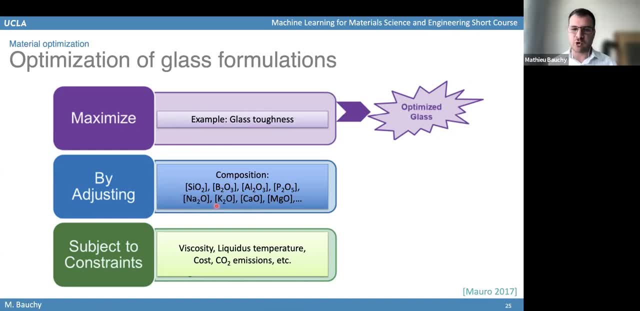 et cetera, and change the fraction or change the oxide that you use for the glass. So this is going to be the degrees of freedom. It's like the variables in the function that you can change, And your goal here is to find. 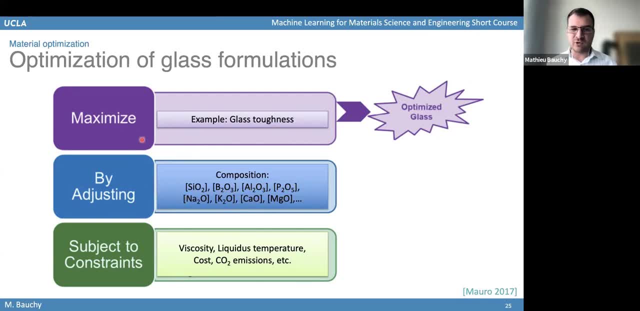 what is the optimal variables here that will give you a maximum of a given function? So you have a function which in that case would be the fracture toughness. This fracture toughness is a function of certain variables, Where the variables here are the composition of the glass. 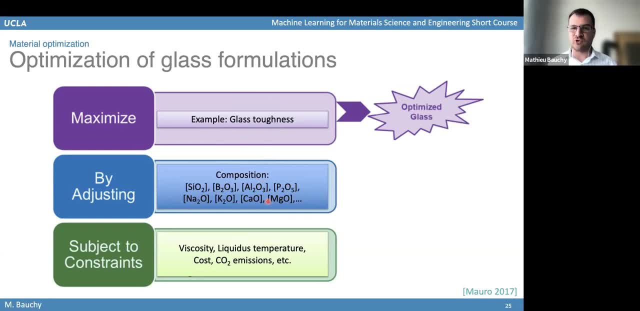 for example, And just like in mathematics, you would want to find what are the variables that will give you a maximum for a given function. Then here the goal is again, like, you have some degrees of freedom. the glass composition, for example. 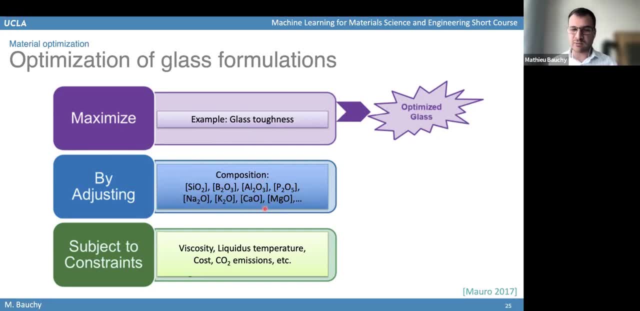 and you want to find what are going to be the optimal combination of composition here that will give you a maximum for this priority, for the glass toughness, for example. So, as you do that, you will want to change the composition until you find the maximum in the glass. 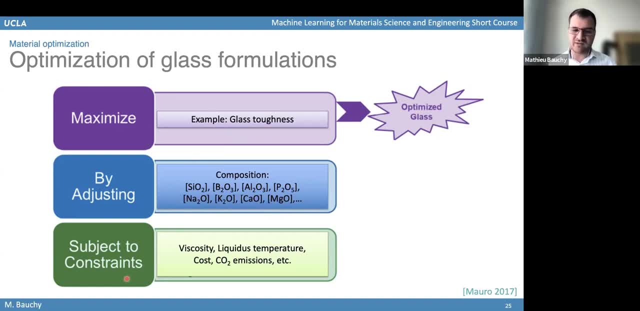 priority here. But as you do that, you always need to obey certain constraints. So it's not simply about finding the composition that will maximize a given priority. You also need, at each step, to ensure that certain constraints are satisfied. So those constraints are the manufacturing constraints. 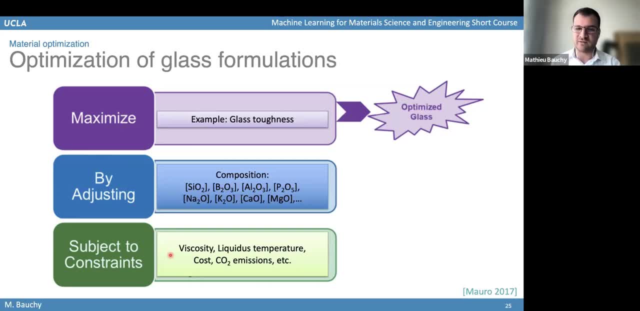 This is to ensure that the material can actually be made in practice. So, altogether, like you have those three things, You have the objective that you want to achieve. So this is the performance of the metal that you want to achieve. You have the degrees of freedom. 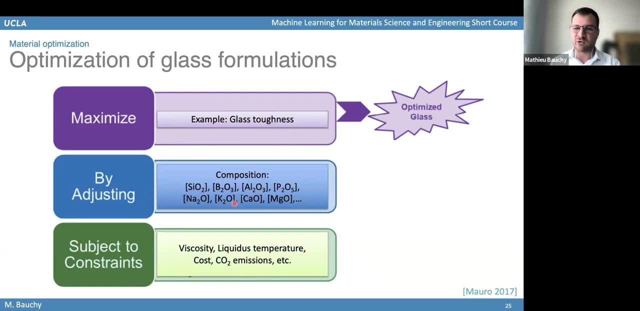 that can be changed. So those are the design parameters that you can change, And then you have the constraints to ensure that the material can be made in practice And, if you are able to find an optimal set of design parameter that can maximize the property, 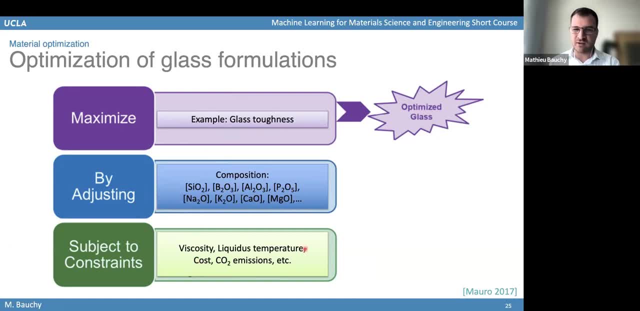 while obeying certain constraints, then you have achieved what you wanted. You have discovered like the optimal material or the optimal glass for the application that you want, And it's going to be a material that can still be manufactured because it obeys the manufacturing constraints. 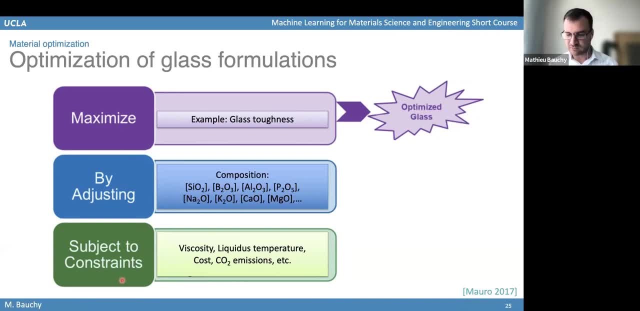 that you would have enforced during the optimization process. So this is exactly the same as a manufacturing parameter in the mathematical optimization process, where you want to maximize or minimize a function by changing some variables, but you have certain constraints on those variables. So this is very similar. 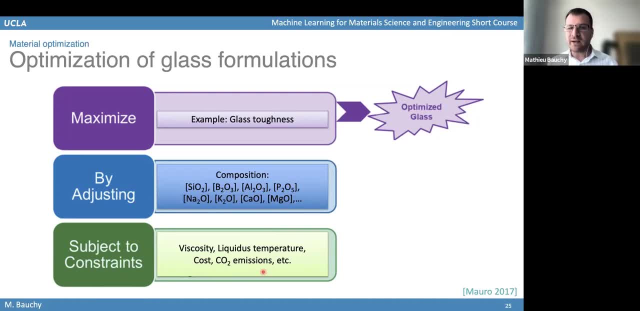 to an optimization process in mathematics. So the way that you can solve these steps of optimization process is by finding some relationship here. Like those arrows here, they symbolize some relationship between the design parameters and the properties, or the design parameters and the constraints. 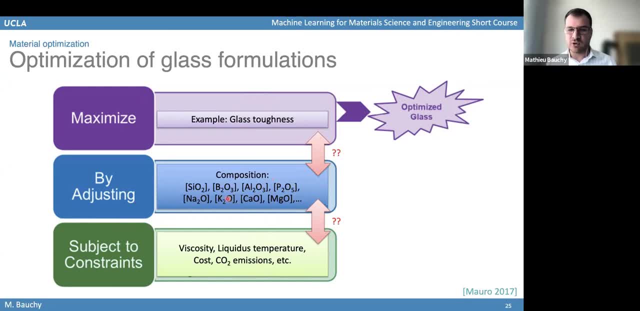 For example, if you have a model here that can tell you the relationship between the glass composition and the fracture toughness, and if you have another model that will tell you the properties between the composition and the viscosity liquidus, temperature, et cetera. 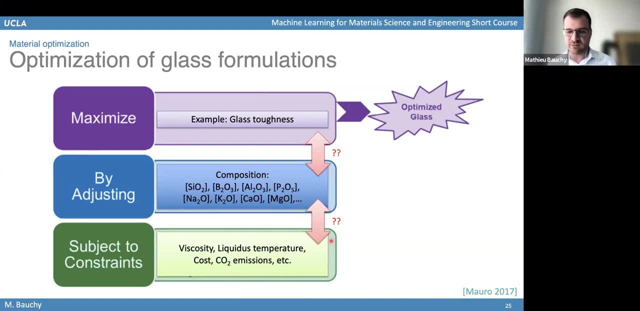 then you can use those models to very efficiently solve optimization problem. You can use those relationship here to quickly find what is going to be the best composition that will maximize a given property while ensuring that certain constraints are met. And if you don't have those models here, 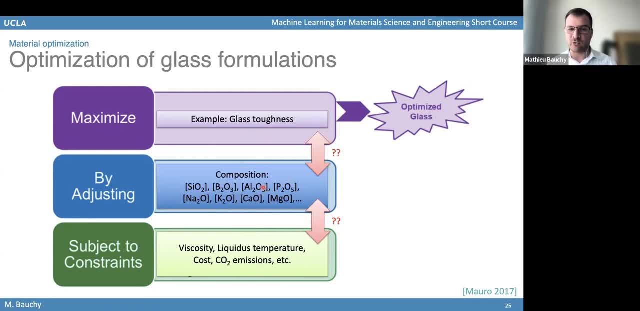 that tell you the relationship of how composition is affecting properties, of how composition is affecting your constraints, then it's something that would be very difficult to solve. So here, one of the main objectives that we would want to achieve using machine learning is to build some models. 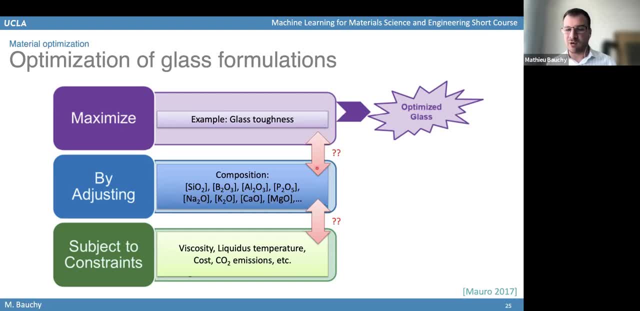 that can tell you those relationship here, A machine learning model that would be able to use as input, for example, the composition here or the temperature or the pressure, and use this as input for a model that can then predict how those inputs 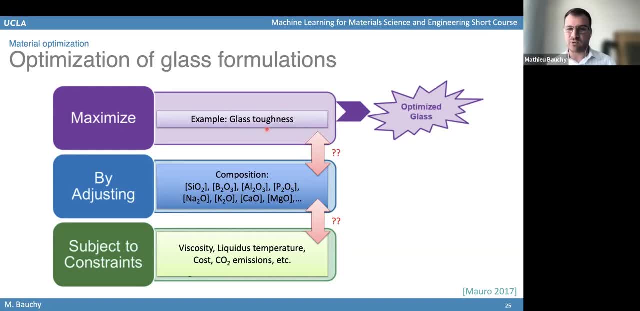 will affect a given property. So this is what we hope to do with machine learning- is to find a model that can be used to transform some design parameters into some properties. If we have this model here, then it makes it very efficient to solve these types. 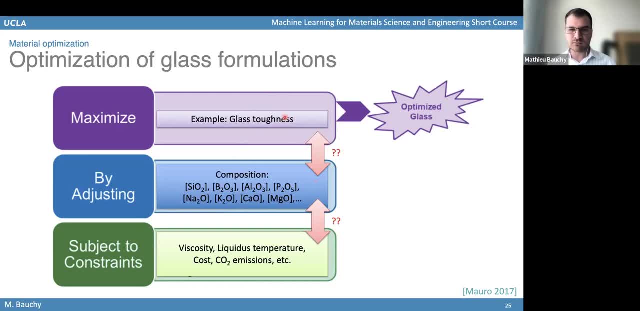 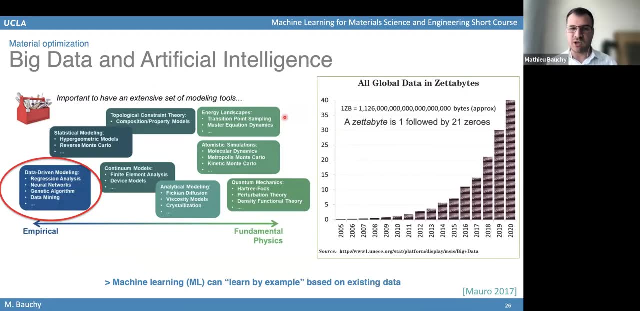 of optimization process. So for this we need some models. We need some models that we can use to map some design parameters to some properties. So we need to find some models that can take as input some design parameter like the temperature or the pressure. 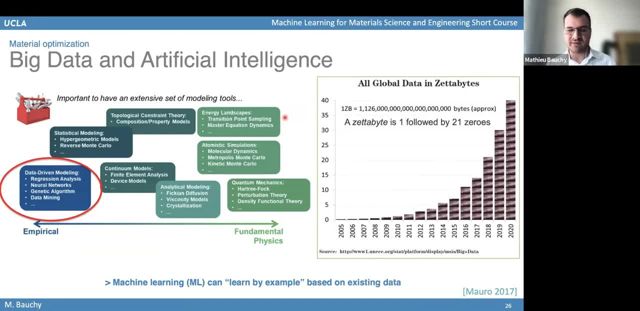 of the processing, And this model will then predict what would be the performance of the material as a function of the design parameter. So for this, when it comes to developing new models like this, there is various models that are available, or various families of models. 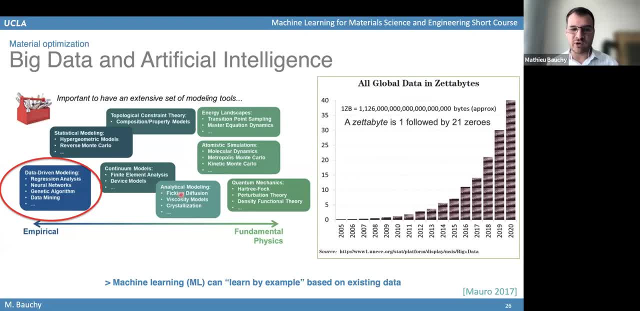 So you can either use what you know about the physics or the chemistry of those models. So those are the models that are rooted in physics, for example. So if you understand enough about the physics of the material, then you can develop a model that is based. 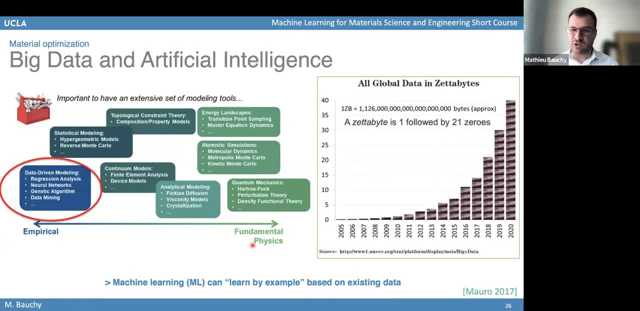 on physics and will relate composition, pressure, temperature to the properties of the materials. Or, on the other hand, sometimes you don't know anything about the physics of those materials, So then you will need to follow like purely empirical approach, And so this is where 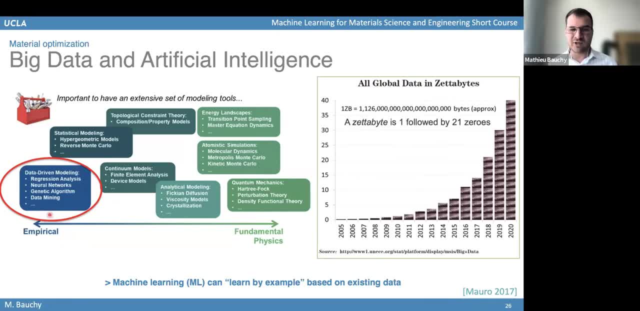 machine learning will go. So this is where, if you don't have any physical or chemical knowledge about the materials, then you can use machine learning. If you have some data, then you will use those data to train some models that can learn based on those data. 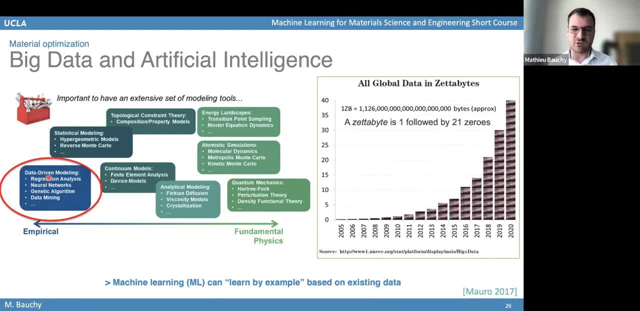 to find a relationship between the design parameters and the properties of your materials. So here, in this case, like this family of models, those are the models that are based on data only, Rather than being based on knowledge, based on physics or chemistry. 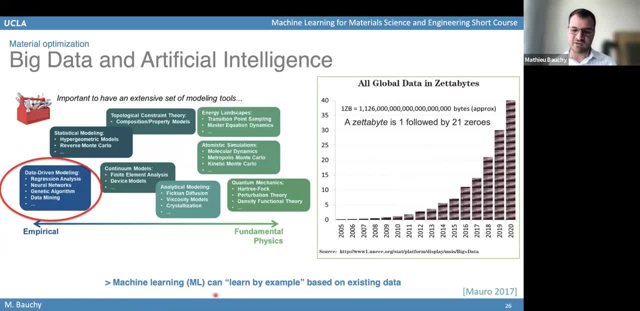 those models will be based on data, And so the main idea of machine learning is that if you have data, then the machine learning model will look at those data and try to learn by example how to use those data to develop a model, And that is. 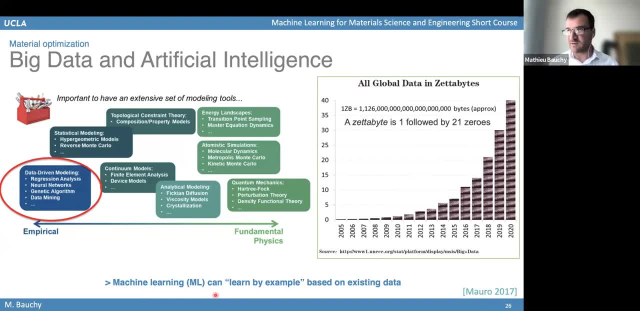 very similar to the way human learn in practice, Like if you are a child, and the way you discover how to do certain action, like how to eat, how to walk. it's very often, if you discover how to walk as a kid, it's not because 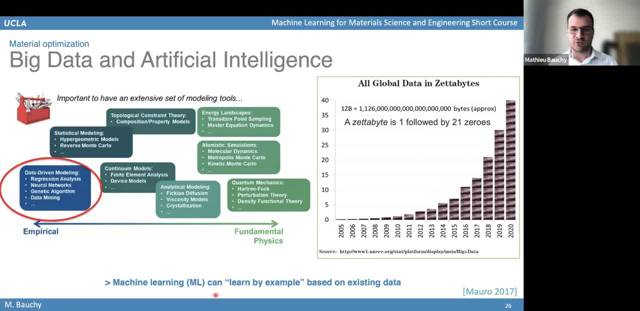 you understand the physics of equilibrium, of how to stand on equilibrium on your legs. It's not based on knowledge that you learn how to walk. You learn how to walk by watching other person walking, or you learn how to walk until you find the right way. 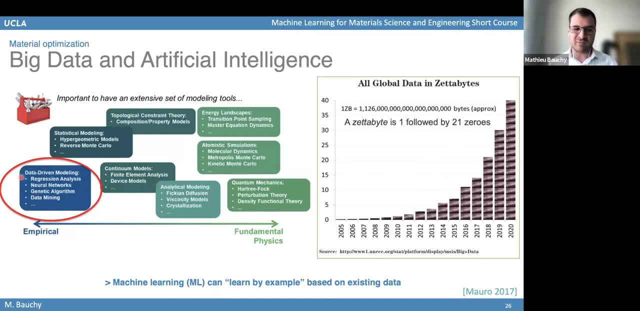 of walking. So in this case that's a very similar process. of machine learning is that you will learn relationship between material parameters and material properties simply by observing. simply by observing many materials with many different features, many different design parameters, combination, and observing how those design parameters 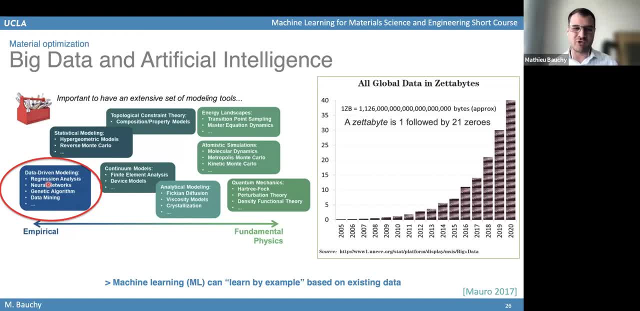 change the properties of materials and then, by observing previous data that you have, then machine learning will be able to develop some models that can relate those design parameters with the properties of those materials. So in that case machine learning they really learn by example. You have some. 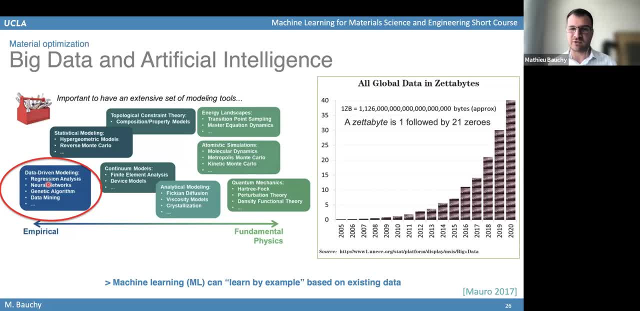 example of materials and machine learning will learn from those examples without learning anything. like we learn as a when we are kid, like we learn everything simply by observing, not really by understanding the fundamental knowledge governing the action that we do. We mostly observe all the person and mimic. 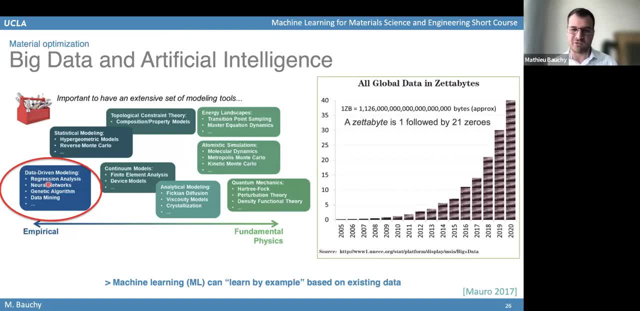 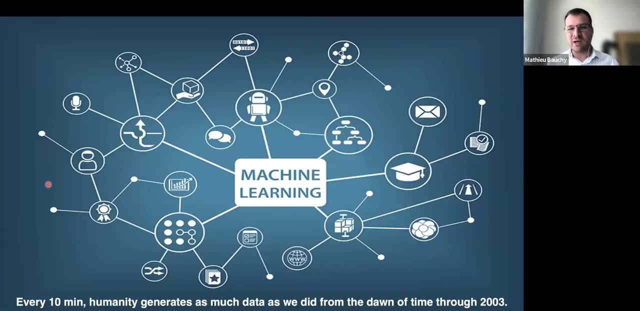 what they are doing, rather than understanding the fundamental reason of why we do things in a certain way. So this is really what machine learning has become more popular over the past decades: is that machine learning is only based on data. Machine learning models will learn some. 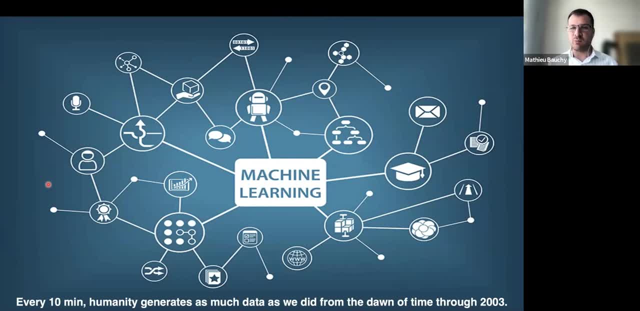 relationship based on existing data, and the main reason we use machine learning more now more than ever is because we have really a lot of data. We produce much more data than we used to. This is also because we have much more computing power than before. 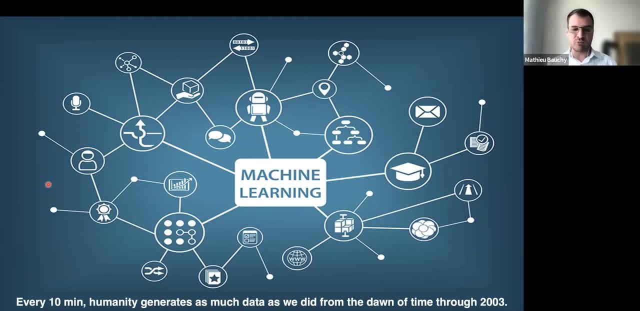 So it makes it possible to really generate much more data than before, But now, every year, we produce much more data than the year before. This is really this accumulation of a large number of data, and we are not possible before just simply because we did not have. 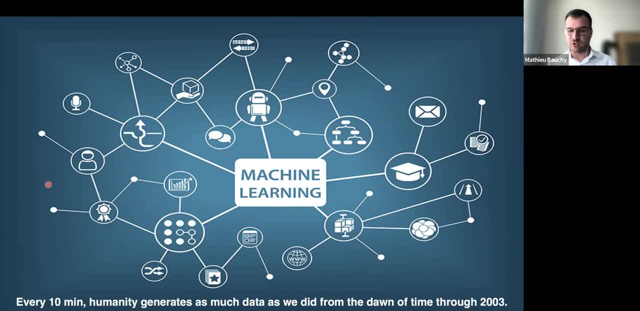 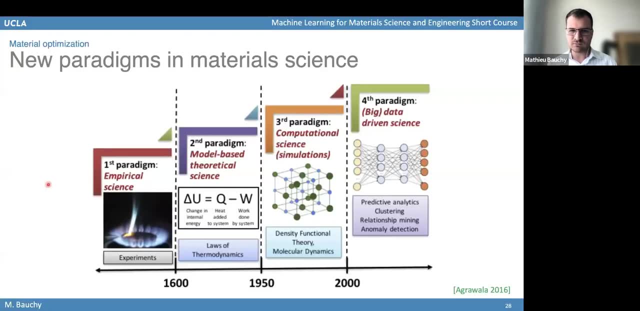 enough data available. So now there is more and more of those data, and more and more of those data becomes available to everybody. So this is really what has enabled the development of machine learning over the past decades, And so this is what we have been. 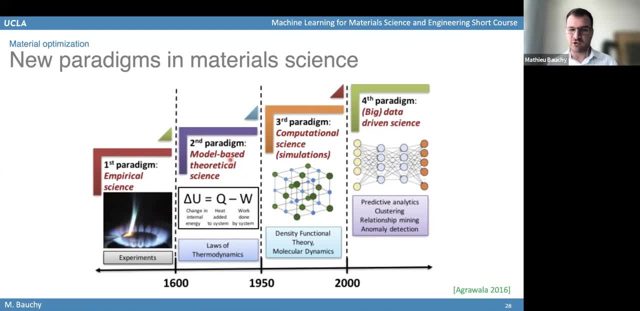 doing for the last 20 years. So this is what we have been doing for the last 20 years. So this is what we have been doing for the last 20 years And in that case, in this case, the process of discovering. 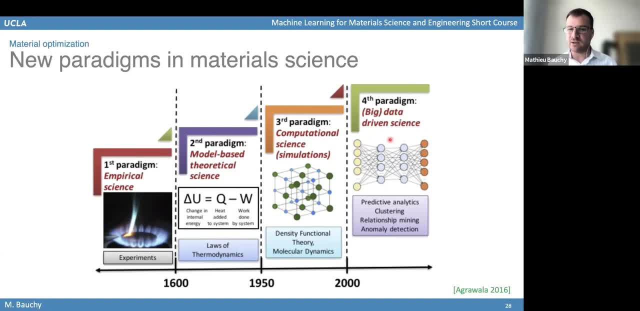 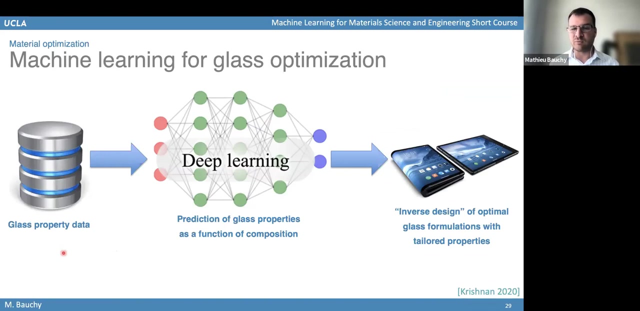 new materials has been really changed by machine learning, Because in this case you can just use data to discover new materials without necessarily having some knowledge about materials and without having to simulate a very large number of materials. So this is the fourth paradigm in material science. 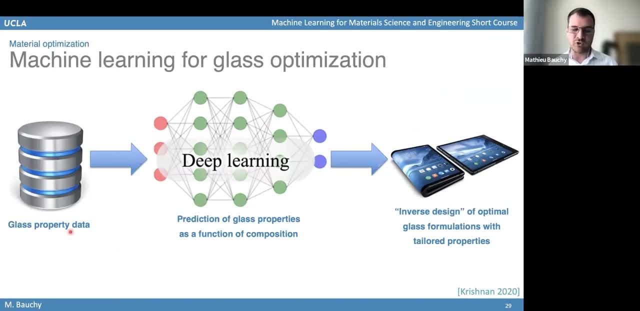 and engineering. So like just to give you an idea. So in this case, if you want to use this model for some inverse design, you can use this model for the optimization process that I previously described. You can use this model to find what will. 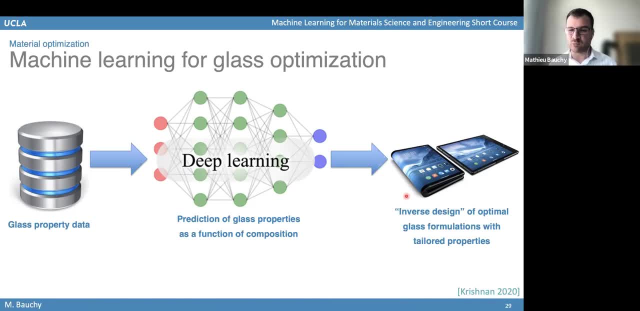 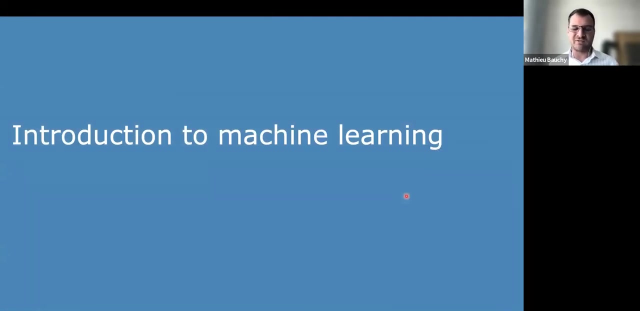 be the optimal glass composition that will give you the highest toughness while meeting certain requirements, So you can use this knowledge to design the material that you want with the optimal properties that you are interested in, depending on the application that you have in mind. Okay, 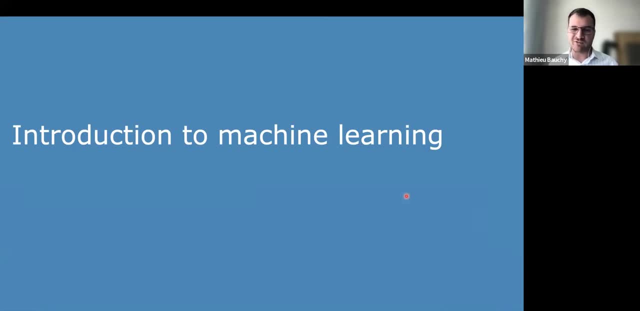 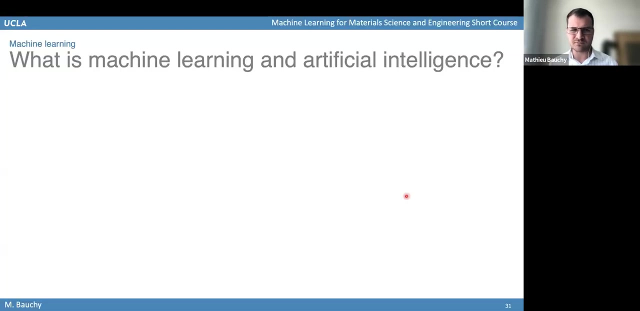 so let's jump now to more specific introduction to machine learning. So the first thing you need to do to use machine learning is really to find what is the best way to define machine learning. what would be the best possible definition of machine learning and how. 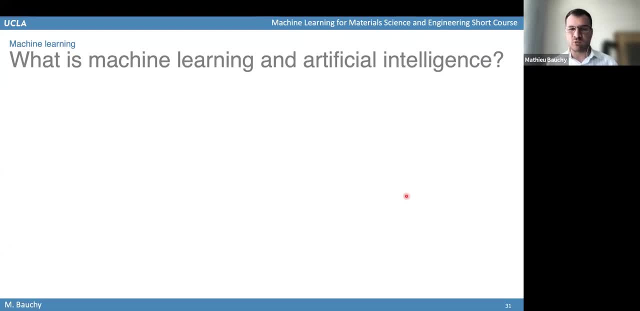 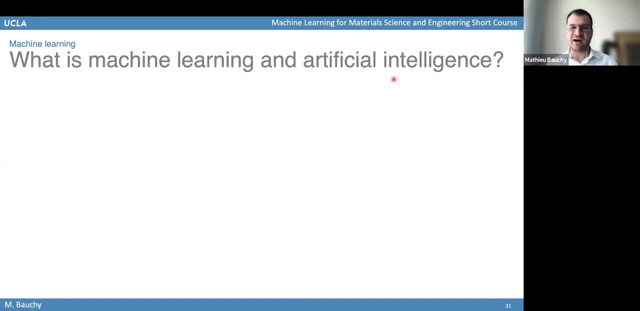 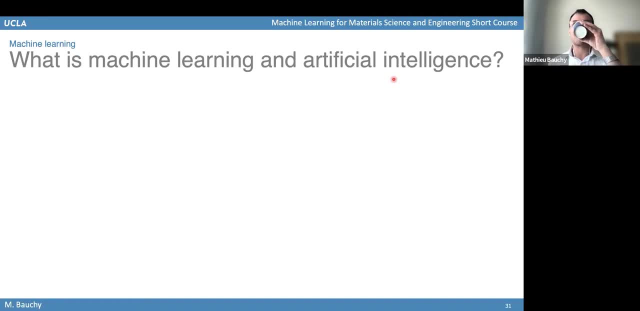 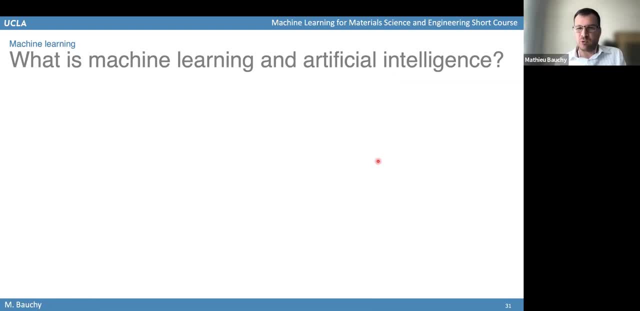 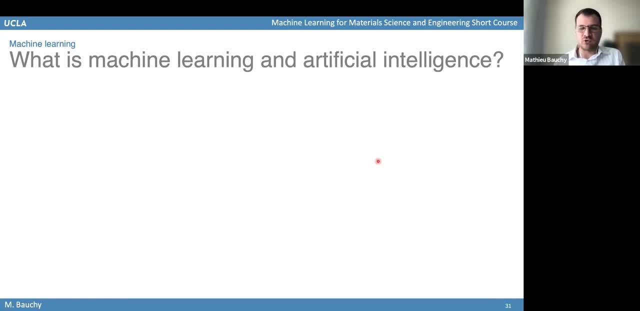 find is what machine learning really is and what it can do and what is the main idea behind machine learning. So do you have any idea of, like a definition of machine learning either based on machine learning? So let me tell you what I think would be. 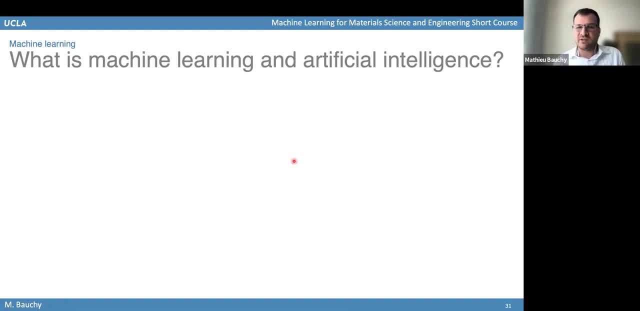 my definition of machine learning, and for this we can use an example and to try to understand, based on this example, what would be a machine learning way to understand what machine learning is. So the first thing you need to think about is what machine learning is. 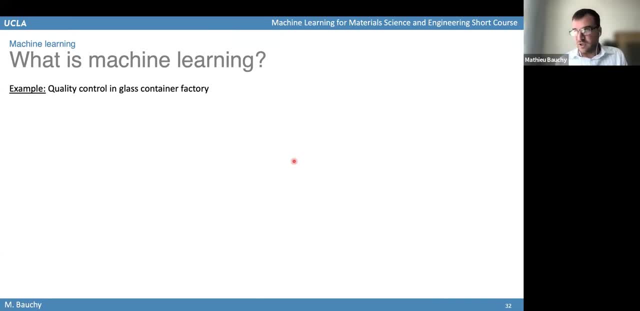 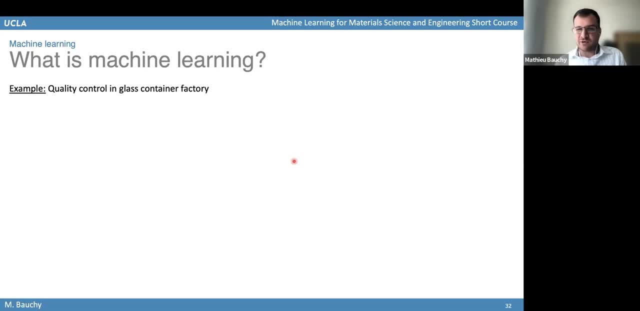 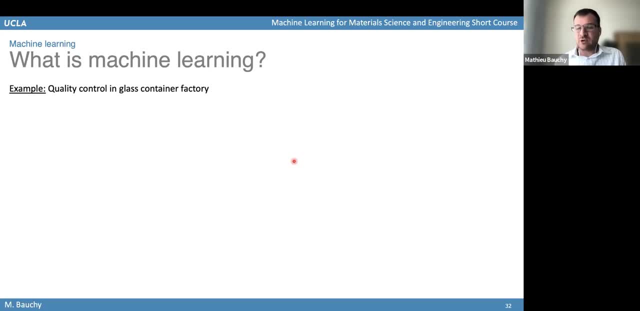 learning is. So the first thing you need to think about is what machine learning is. So the second thing you need to think about is what machine learning is So the first thing you need to think about is what machine learning is So. the second: 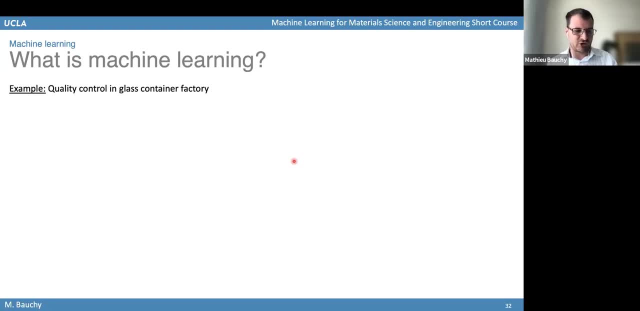 thing you need to think about is what machine learning is. So the first thing you need to think about is what machine learning is. So the second thing you need to think about is what machine learning is. So the first thing you need to think about is: 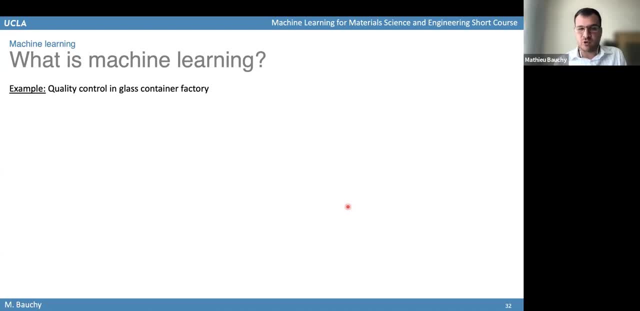 what machine learning is. So the second thing you need to think about is what machine learning is. So the first thing you need to think about is what machine learning is. So the second thing you have to think about is machine learning. And then you. 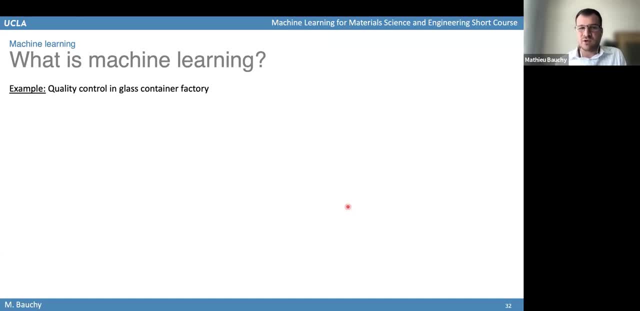 need to think about what machine learning is. The third thing you need to think about is the fact of seeing some cracks in your glass means that the glass doesn't meet the quality that you want. Then you will use this knowledge to decide that I should disregard this glass container. 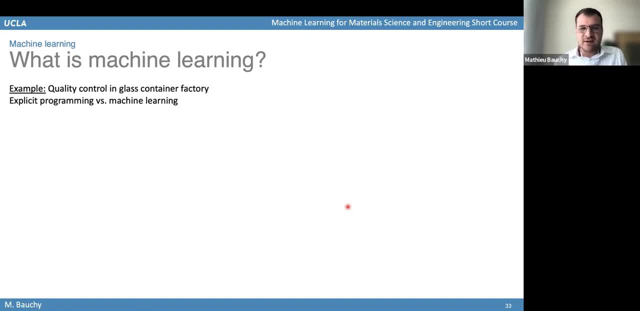 So that would be a first way, And this is what I would call explicit programming. Like you can, if you want to optimize this process, then you can take a picture of this glass and then use this picture and put this picture to a program. 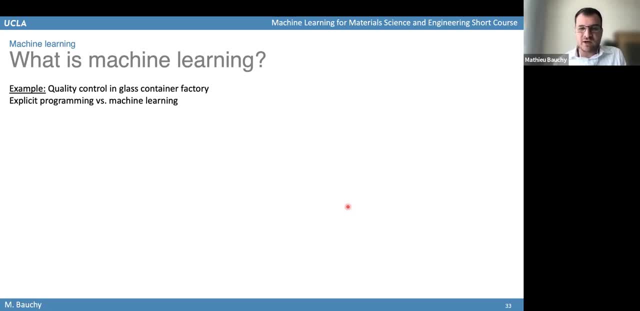 and this program will try to see: is there a crack in the glass, Is the glass transparent or not, Is there some bubbles in the glass or not? And based on those conditions, you will have a given algorithm that will say: if I can see some cracks, 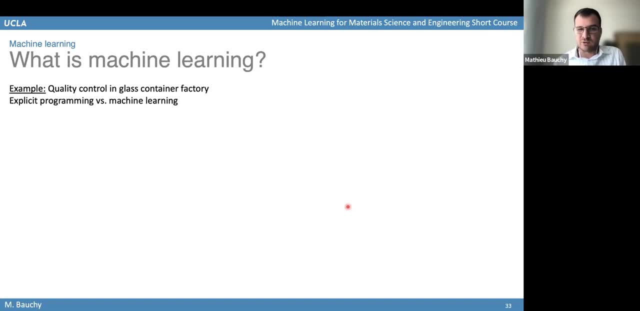 then the glass doesn't meet the quality. If I can see some bubbles, then the glass doesn't meet the quality requirements. So this would be explicit programming, because you would explicitly code in your program what are the conditions that distinguish a glass that meets the quality requirement. 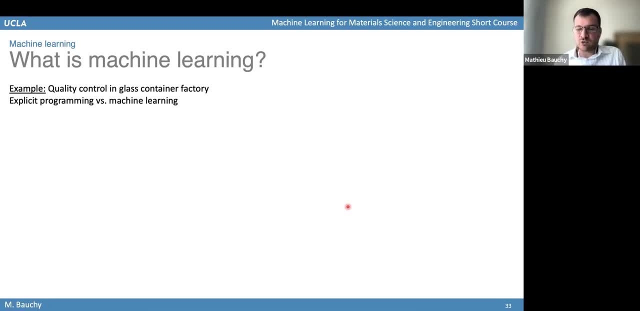 from a glass that doesn't meet a quality requirement. So that would be the first way to develop a model is that you will write the condition explicitly. You will explicitly write in your program what are the conditions that makes a glass container satisfactory and what are the conditions. 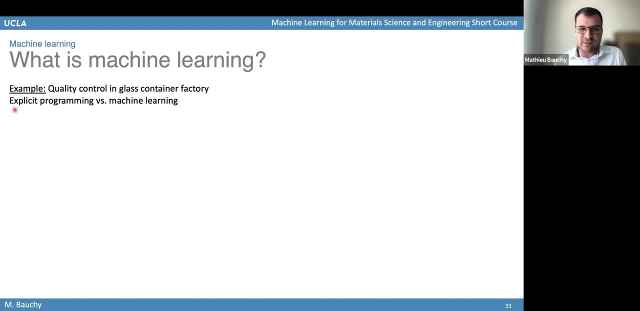 that makes it non-satisfactory. So that's what we call explicit programming. because we don't have to do that, We explicitly give to the program the rules of what distinguishes a good glass from a bad glass. But then there's an alternative way. 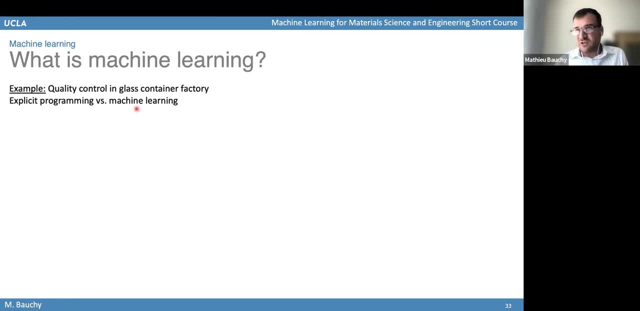 which would be to use machine learning. If you use machine learning, then it means that you don't necessarily already know what is the difference between a good and a bad glass. You don't know how to distinguish it yet, But what you know is that you have some example. 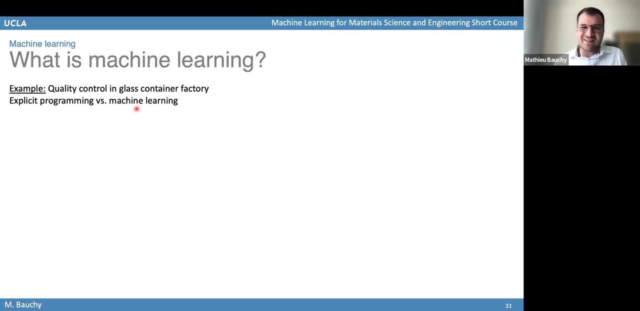 You have some example. For example, you have some example of 1,000 glasses that you know meet quality requirements, and you have another 1,000 example of glasses that do not meet quality requirements, And so this is what you have already. 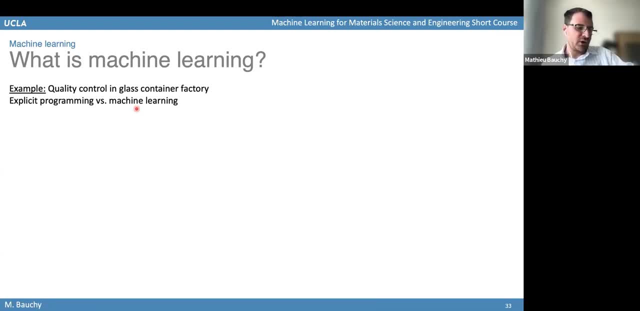 So you have, for example, you take 1,000 pictures of example of glasses that meets requirement, quality requirements, and you have another 1,000 of glasses, one other example of pictures of glasses that do not meet quality requirements, And then you will use those example of pictures of glasses. 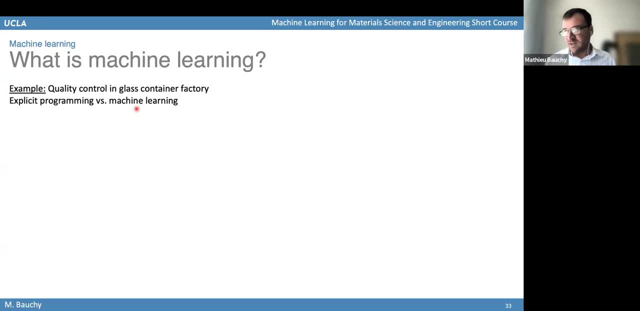 and you will give that to a machine learning model, And then what the machine learning will do is to analyze those pictures, analyze those example of pictures of glasses that either meet quality requirements or do not meet quality requirements. And by analyzing those example of pictures, 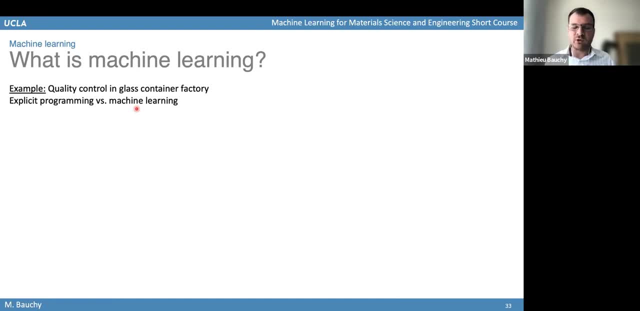 the machine learning model will train, Try to understand what are the rules that distinguishes good glass from bad glasses. So in this case it's a very different process. When you do explicit programming, then you already know the rules of what distinguishes. 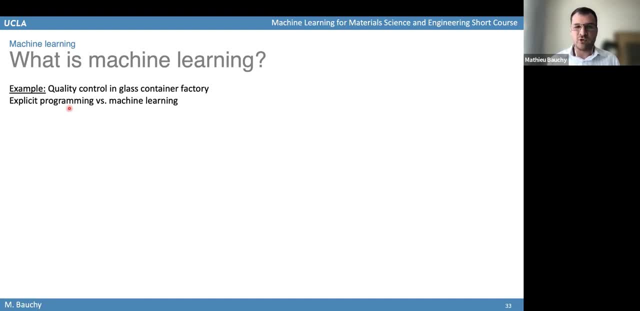 a good glass from a bad glass and you will use those rules to build your program. In the case of machine learning, it's exactly the opposite. You don't know what are the rules that distinguishes good glass from bad glass. All you have to do is some example. 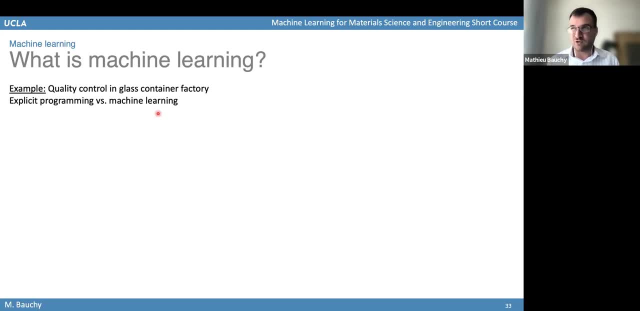 All you have is some example. You have some example of pictures of good glass, some example of pictures of bad glass, and you will use those examples to teach a machine learning model how to recognize what is a good glass from what is a bad glass. 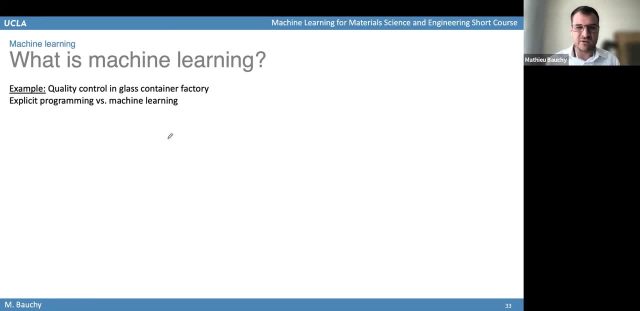 So one way that we can summarize this is: if you want to write a given software that can recognize what is a good glass from what is a bad glass, There are two ways you can do that. One would be this explicit programming. So that's the first option here. 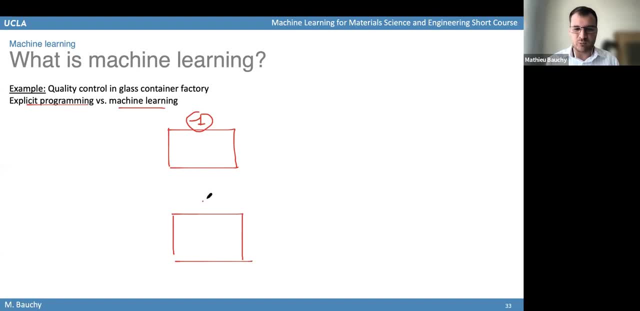 And the other one would be the machine learning option, And in that case, the idea behind this would be very different. In the case of explicit programming, what you need to come up with is some rules, So you need to come up with an algorithm. 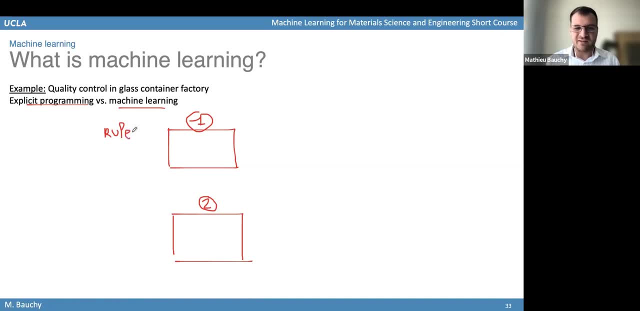 So, for example, you need to come up with some rules that if I see some crash, then the glass is not satisfactory. So in that case, that's what you need to provide first, And you need to provide some rules, And then your software here will use those rules to decide if the glass is satisfactory or not. 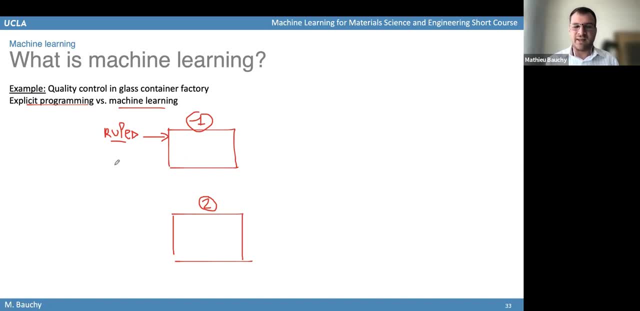 So that would be the first way, And then, once you have those rules, then you can put some inputs. So the inputs would be the picture of a new glass, And then what this program will do is to analyze this picture and then use the rules that you came up with. 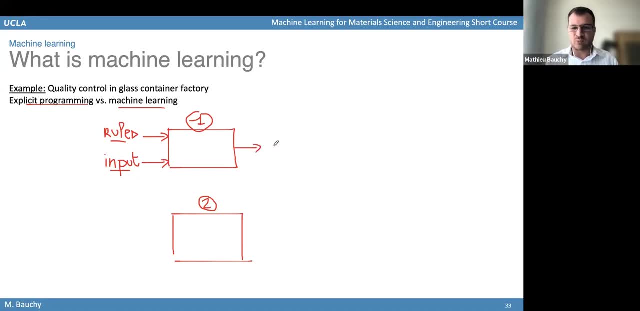 And, based on those rules, the program will tell you an output, And this output will be: either it will be like you can have two options as an output, which be either the glass is satisfactory or not satisfactory. Either it meets quality control. 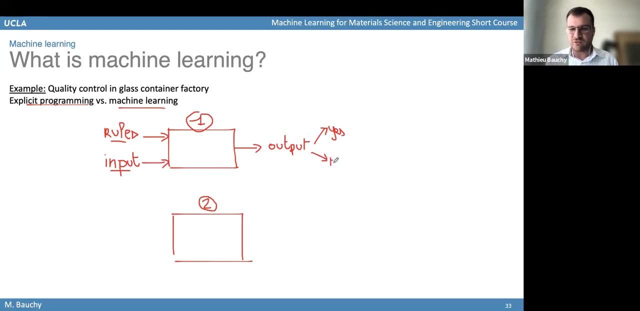 Condition or it does not. So in that case, that's the first way to come up with a software that would check the quality of a given materials. You provide the rules explicitly, then you provide an input. So in that example, this input would be just a photo of a given glass. 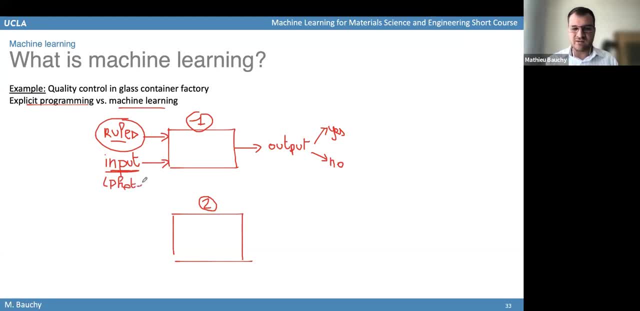 And then the program analyzes this photo, Check The rules that you imposed and then, based on those rules, will tell you if this glass is either okay or not okay. So that would be explicit programming. That's option one. Machine learning is very different. 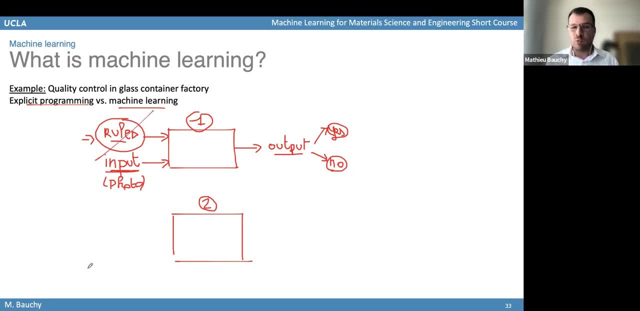 In machine learning. you don't know those rules, So you don't know what distinguishes a good glass from a bad glass. All you have is some example. So it means that you have some example of inputs. So you have some example of. 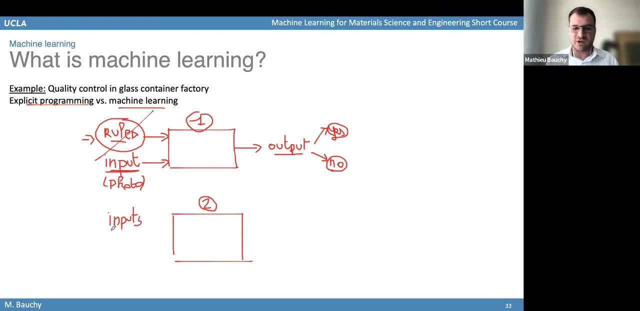 you have some example of photos, that of glasses, and for those glasses you already know the output, So you know already if this glass is satisfactory or not. So in this case that's a completely different approach where rather than providing the rules- if you don't know the rules- then you will kind of do it in the completely reverse way. 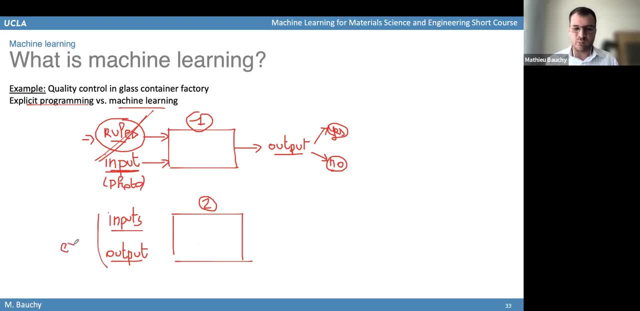 where you use some example. So here that would be some example. So here that would be some example. So here that would be some example of glasses where you both know the input, So you have some example of photos of this glass, but you also know the output. 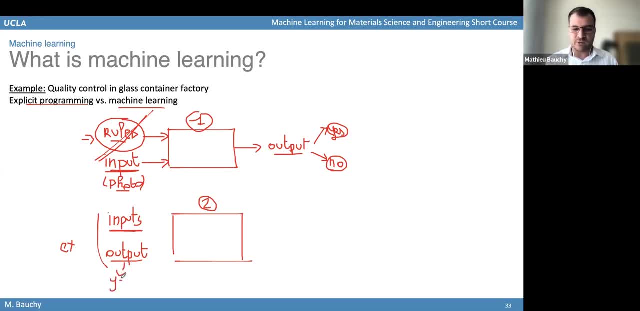 So you know if this glass either meets quality requirements or it does not meet quality requirements. So in that case, that's where you start from. That is what you're providing to the machine learning model, And the main difference here is that then machine learning. 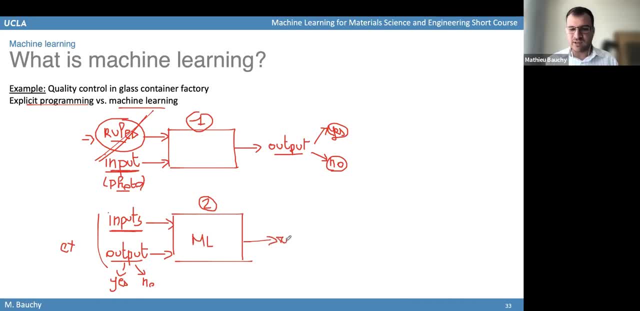 model. as an outcome of the machine learning model, it will give you the rules. It will give you the rules on how to distinguish a good glass from a bad glass. So the machine learning approach is completely the opposite of explicit programming. Usually, you know the rules that govern the given materials. 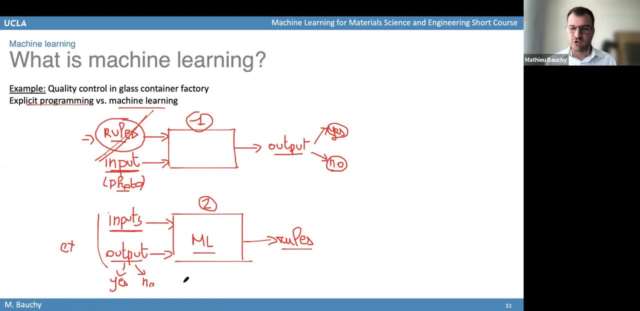 But in the case of machine learning it's exactly the opposite. You don't know the rules, you just know some example, know some example of materials That are either good or bad. You use those example, you feed them to a machine learning model. 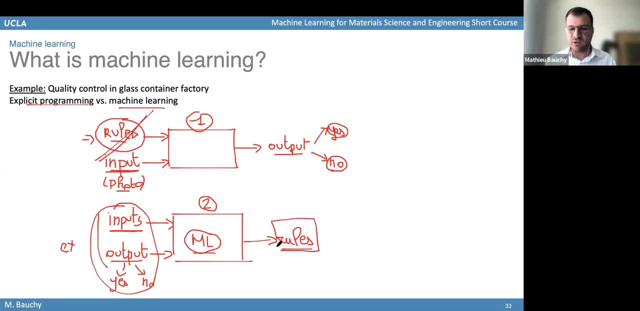 And then the machine learning model tells you, as an outcome, the rules. So it's going to learn, for example, that if it sees some cracks in the glass, then it means that the glass is not satisfactory. It will learn, by example, that if it sees some bubbles, then the glass is not satisfactory. 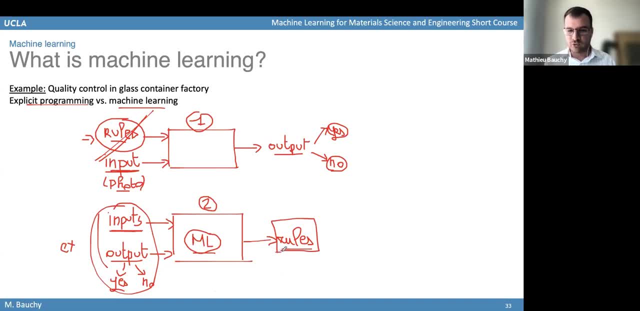 So here it's exactly the opposite. You get the rules that distinguish a good glass from a bad glass As an outcome of the machine learning model. Rather than having the rules as an input, Here you have it as an output. This is what the machine learning model tells you. 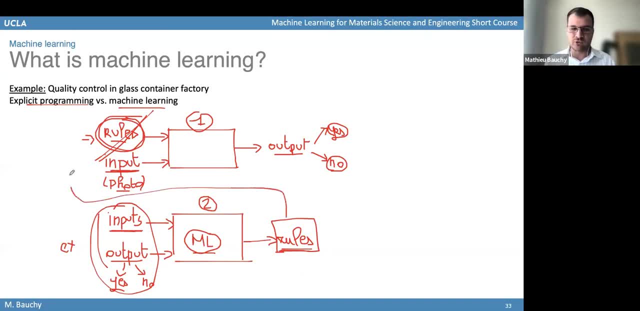 And once you have those rules, then you can use those rules to come back to a more traditional approach, Where you will use those rules And, based on that, analyze new photos of new glasses And, based on those rules, You can decide if the glass is satisfactory or not satisfactory. 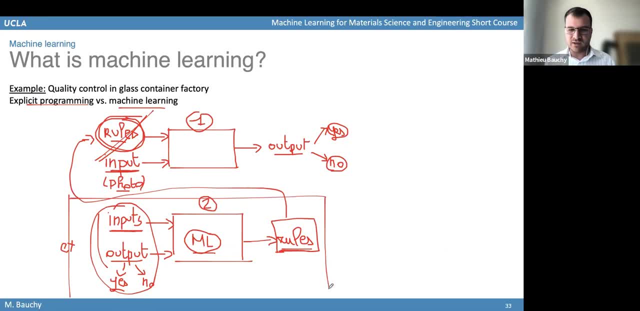 So this process here is the machine learning approach. This is where you don't know the rules. that dictates the materials behavior. But you have some example of materials And you will use those examples to teach some machine learning model To try to come up with the rules. 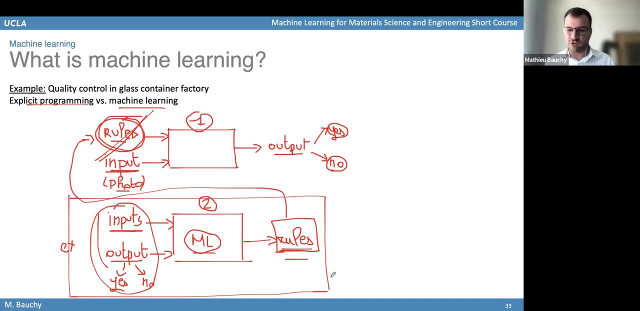 So that's completely the opposite of the traditional way of Studying materials. Rather than using some rules to make some prediction, Here you just start with some example And the machine learning model will give you the rules Rather than the opposite. So that's a completely reverse way of approaching materials. 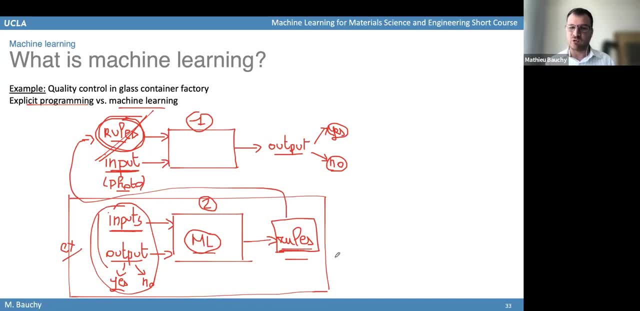 You just approach it based on examples, Based on data, Rather than based on rules, Rather than based on knowledge. So to some extent, In the traditional way, You use some knowledge To make some prediction. Now, in machine learning, that's completely the opposite. 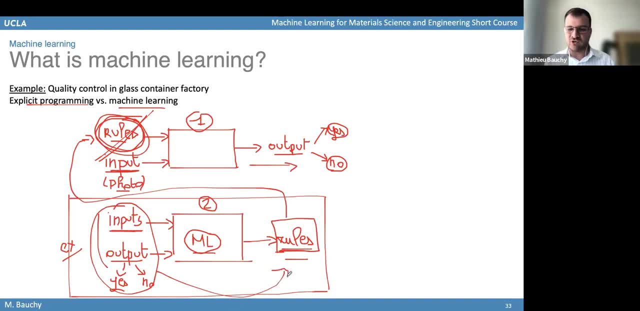 You use some example And based on that you can generate new knowledge, Or you can generate new rules that then you can use To inform your materials or discover new materials Or check if a material is satisfactory or not. So it's a completely reverse way of thinking about materials. 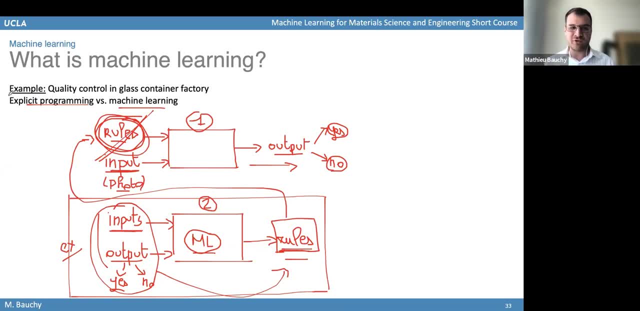 Do you have any questions regarding this, This difference between explicit programming versus machine learning here, Any questions about this, Those schematic here, Or any questions about this machine learning approach? Okay, So that was one example, So let's continue from there. 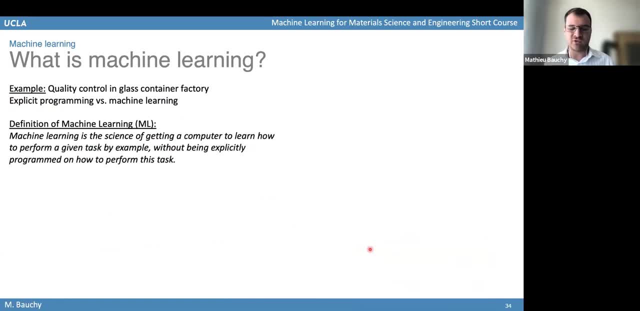 So based on this, So the way I would define machine learning. So I mean everybody can have a slightly different definition of machine learning. There's different way of defining what machine learning is, But the way I would define it is as follows. 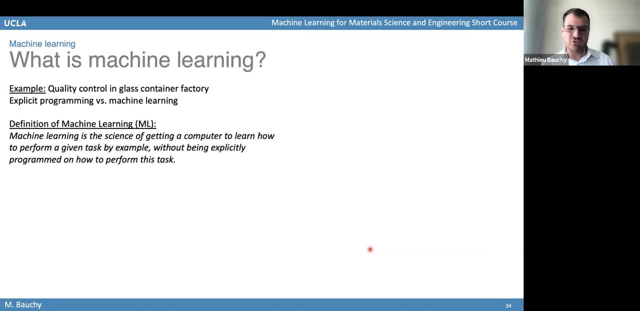 So I would define machine learning as the science of getting a computer to learn how to perform a given task by example, Without being explicitly programmed on how to perform this task. So, Just like many definitions, Like every word in this definition is important. 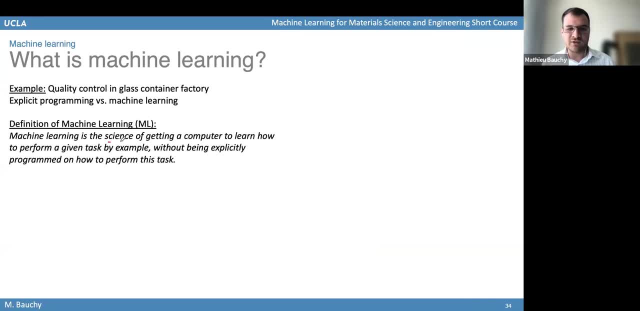 Right. So the first thing is that machine learning is a science. So that's one thing. And it requires computer. So machine learning will require a computer to be trained. So that's the first thing. The goal of machine learning is to perform a given task. 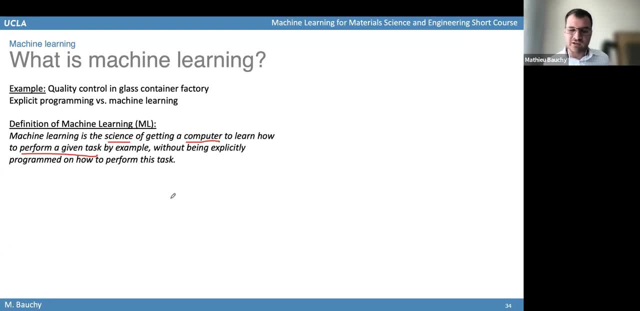 So, again based on the previous example, a given task can be based on a given photo of a given glass. Tell me if this glass meets quality requirement or not, So that could be an example of a given task, Or another task could be based on a given composition. 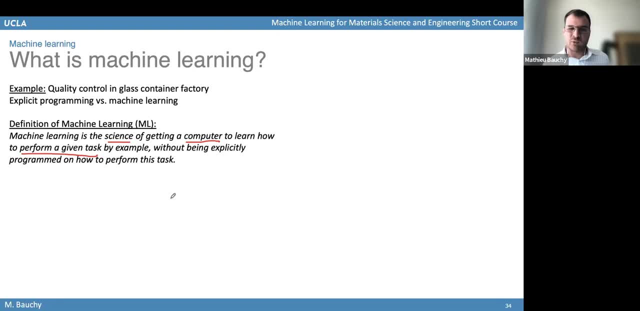 Predict what will be the property of this material, Predict what will be the density of this material, Predict what will be the modulus of this material, The toughness of this material, et cetera, So predicting a given priority, Or, it can be like, based on a certain condition of temperature and pressure. 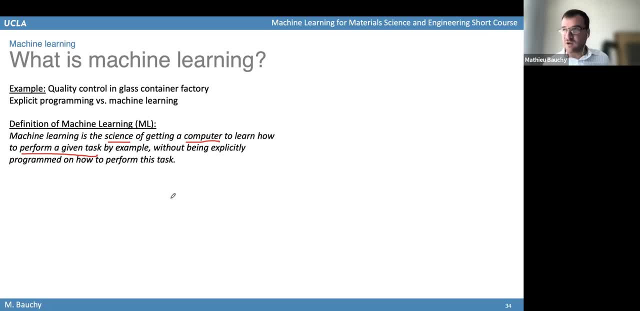 Predict if a material can be made or not. Is a given material going to be formed or not under a certain condition? So that would be some example of task that you would want your machine learning model to be able to do. So that's the next thing. 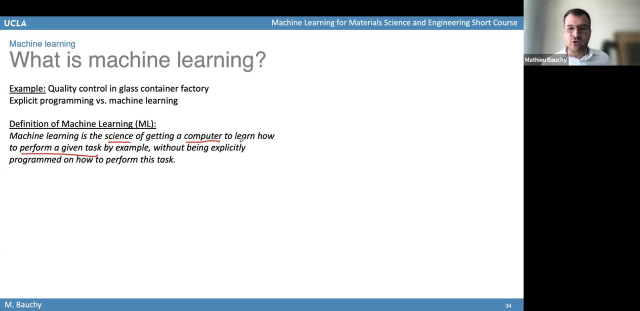 Now the question is: how do you learn how to perform this task? So what we said for explicit programming is that you, in that case, you would do this task based on explicitly putting some instruction. For example, if you know already, you have some physical knowledge about how the composition of a material is going to affect its priority. 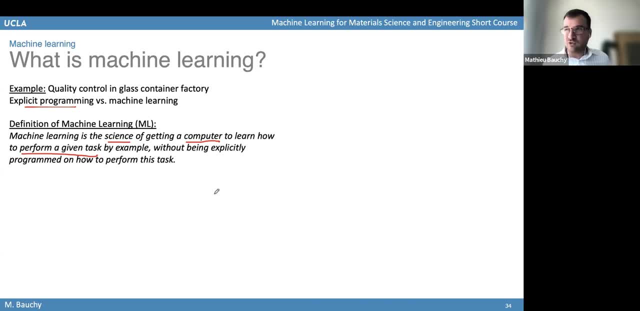 Then you are going to use this knowledge to build a model, like a recipe, where you will tell your software if the composition contains these oxides, Then the material will have this priority, Or if there is more than a given threshold, then the priority will be affected in a certain way. 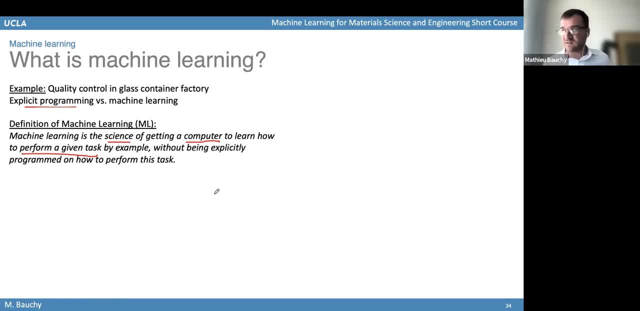 So in that case that would be an example of explicit programming. It's if you You know some knowledge about a given material, then you can achieve a given task. A computer can achieve a given task by you providing some instruction of what to do. what are the list of instructions on some conditions etc. 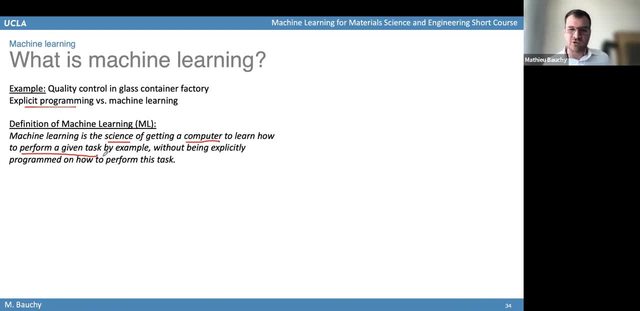 To achieve a given task, to make a prediction based on certain list of instruction. Here, in the case of machine learning, there is no instruction. The only way you will learn how to perform a task is By example, So without being explicitly programmed on how to perform this task. 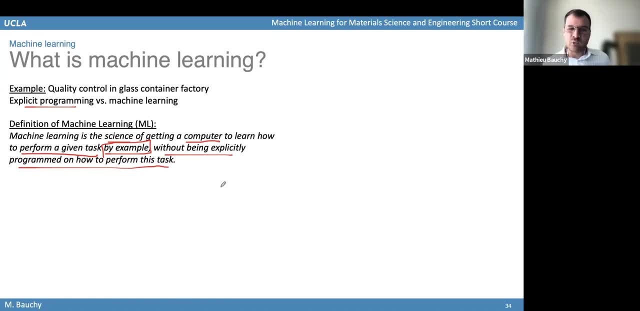 Here you won't tell the computer how to do this task. You will just provide some example of materials And the computer, in that case, will learn how to make a prediction simply by example, but without being explicitly programmed on how to do that. 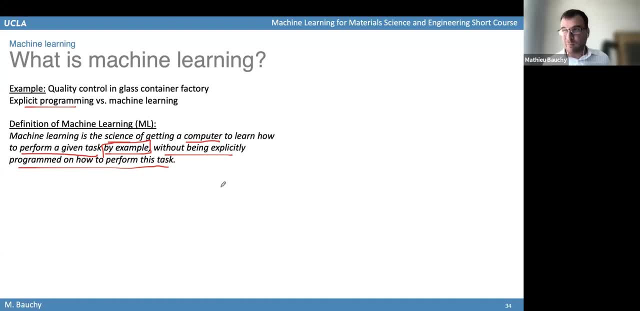 So, for example, you will provide a large number of examples of pictures of materials And then you will also tell the computer for this picture the material was satisfactory, Or for this picture the materials was not Is not satisfactory. And then you let the machine learning model learn by example how to recognize the satisfactory materials versus the non-satisfactory materials. 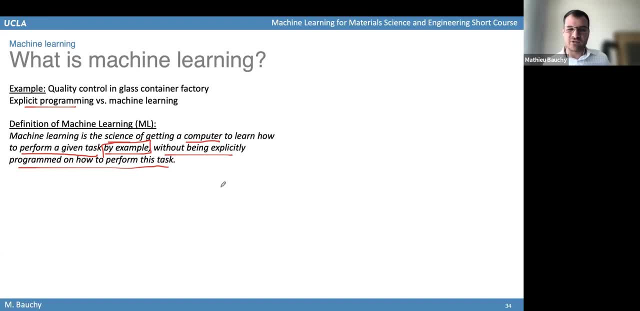 And in that case you don't tell anything to the computer on how to discover that, How to recognize the satisfactory materials versus the non-satisfactory materials. Just provide some example And you let the machine learning model recognize on its own what distinguishes satisfactory materials from non-satisfactory materials. 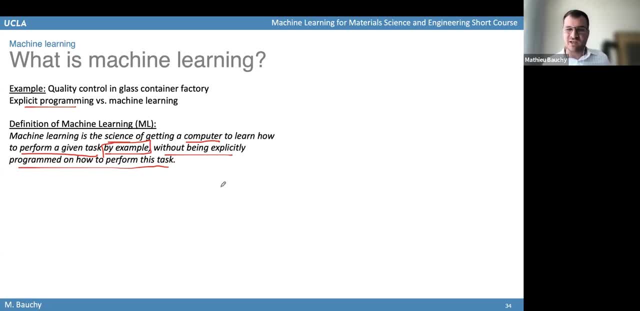 And that's something that computers are very good at doing, because they can find some patterns in data, Or they can find, like very subtle differences in pictures, for example, that as a human you would not necessarily be able to see, And then computers can use those patterns. 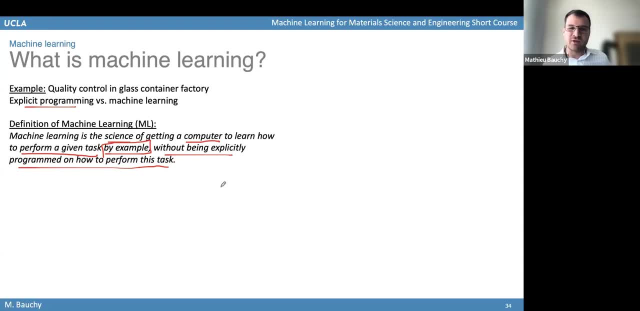 Or use those small differences to learn on their own how to distinguish the satisfactory materials from a non-satisfactory materials. So that's the way I would define machine learning. So again, it's the science of getting a computer to learn how to perform a given task. 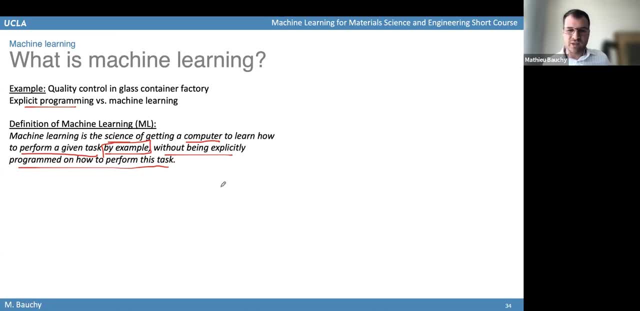 But learning this task only by example, without receiving some explicit instruction on how to perform this task. So that's really what machine learning is And that's really how it differs from the more traditional explicit programming. Any questions based on this definition so far? 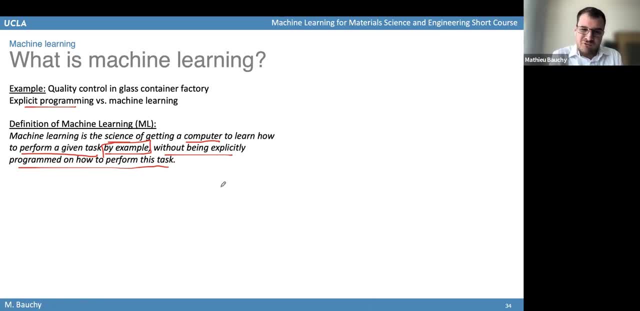 Then the next thing is: so, if this is the definition of machine learning, what is the definition of artificial intelligence? So, artificial intelligence, I would define it this way: So artificial intelligence is the science, The science of getting a computer to learn how to perform a task that usually requires human intelligence. 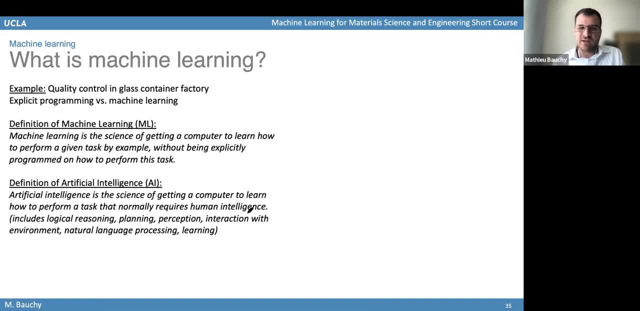 So that's the definition of artificial intelligence. It's actually pretty close to machine learning, but there is some differences. So in artificial intelligence again, you want to have a computer learn how to do a task. So that's still the same objective. 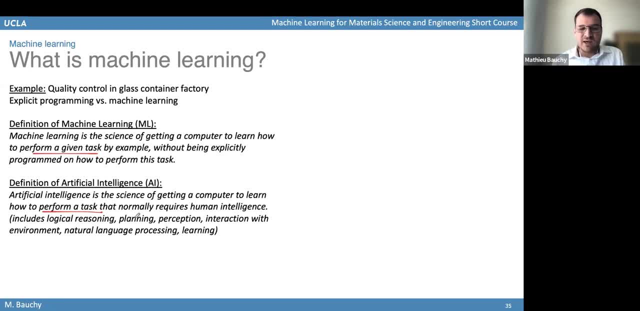 It's still about performing a given task, And this task is a task that typically requires intelligence. It's not something that can be done like. it's a task that typically would require some intelligence on how to perform this task. So the key difference here is that: artificial intelligence, the definition, as you can see here it's more general than machine learning. 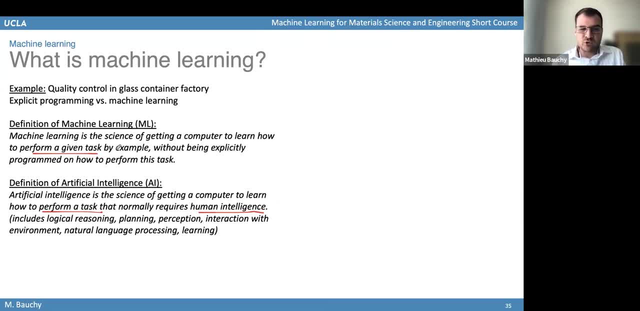 Machine learning, you will really learn how to perform this task. To perform this task by example. In the case of artificial intelligence, you teach a computer how to perform a given task, But there is no condition of how the computer will learn how to do this task. 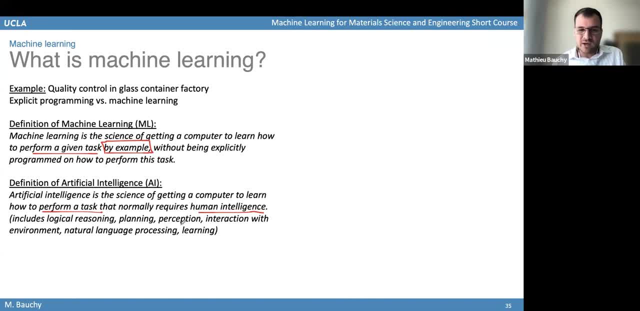 So in the case of artificial intelligence, one way to teach a computer how to perform a task could be by example, So that can be by machine learning, But it can also be by actually providing some instruction, Like that would be another way. You can just tell. if you are building a robot, for example, then you can tell the robot. if you see this thing in front of you, then you need to stop. 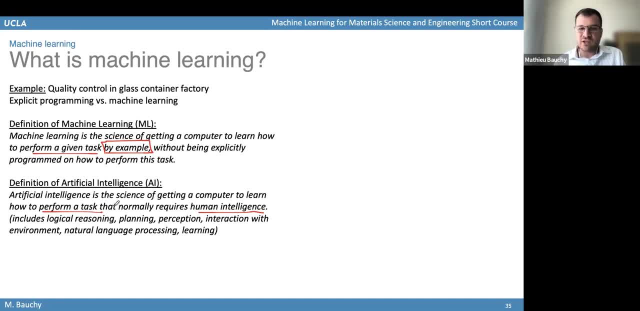 That would be an explicit condition of: if you see an object in front of you, then stop, Don't continue running towards this object, So to avoid a collision. So that would be, for example, an example of an explicit condition that you would provide. 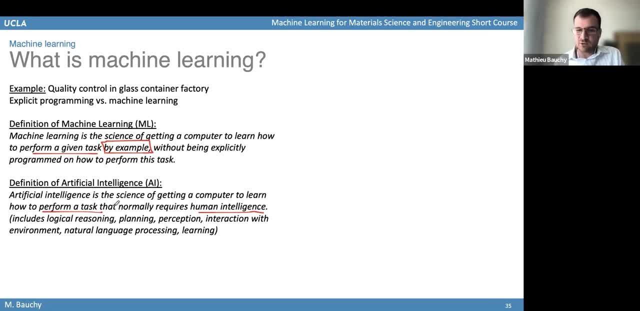 You would provide with a robot Like you, would teach the robot how to navigate in a given room And you would give them some instruction. If you see something in front of you, then you need to stop. So that would be an example of artificial intelligence, where you provide explicitly some instruction to the robot. 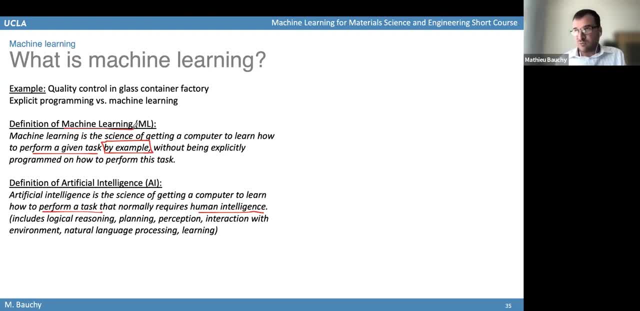 But another example: using machine learning, you would provide the robot with some example of motion that is safe Versus some example of motion that is unsafe, that led to some collision, And in that case the robot will just learn directly from those examples how to avoid collision. 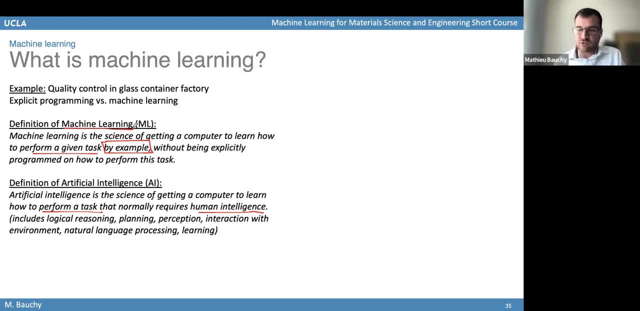 So the robot? you won't teach explicitly the robot that it needs to stop if it sees something in front of you, But it will. the robot in that case will just learn this on its own because it will have seen some example of a previous condition where the robot would have collided. 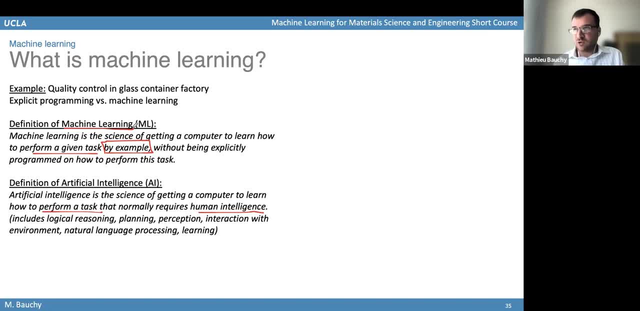 With something in front of him, And it will use those examples to learn how to avoid collision in the future. So, like this process of learning by example, it's very similar to the way babies learn, Like they learn by example if they do something that makes them feel painful or something like that. 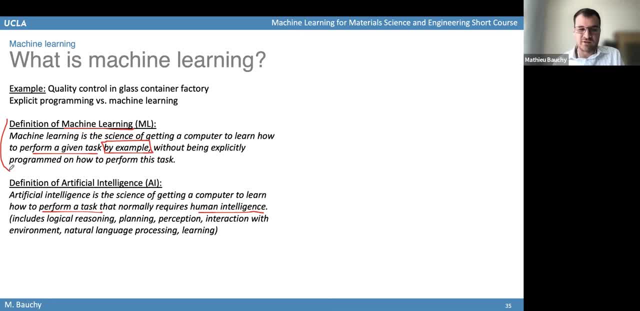 Or if they do something that and then an adult tells them that this was something bad, Then they will learn, based on this example, that they should not do this thing in the future. Or if they do something that leads to something happy at the end. 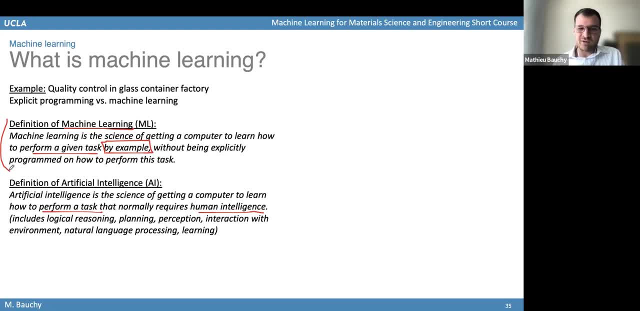 Like, if they eat something and something that tastes good, Then it's something that they will tend to do again and again, because it's something that they got rewarded for this. So this is the process of learning by example: doing something, And either you will receive a penalty. 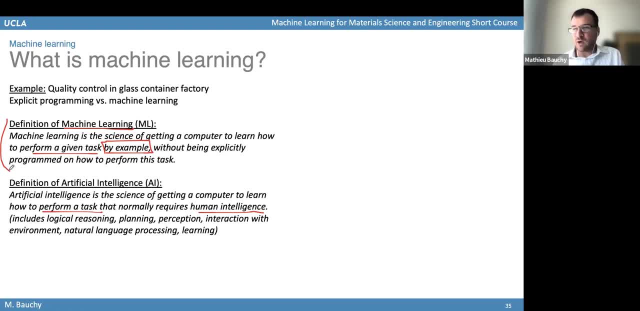 Based on what you did, Or you will receive a reward because you did something good, And then you will tend over and over to do things for which you receive a reward And you will tend to avoid things for which you receive a penalty. So this would be a process of learning by example. 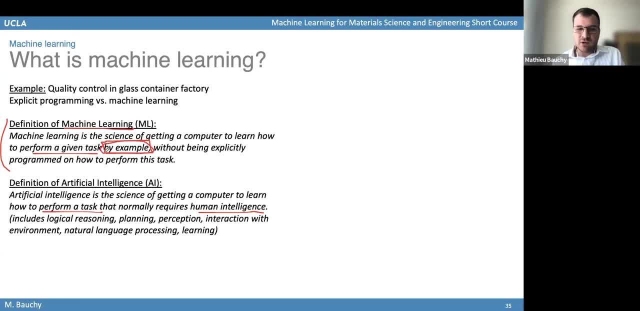 This is very often how kids learn, But artificial intelligence can be more general by that. You can also learn based on some condition. So artificial intelligence- This is more commonly abbreviated as AI- It includes more things than just machine learning. It includes logical reasoning. 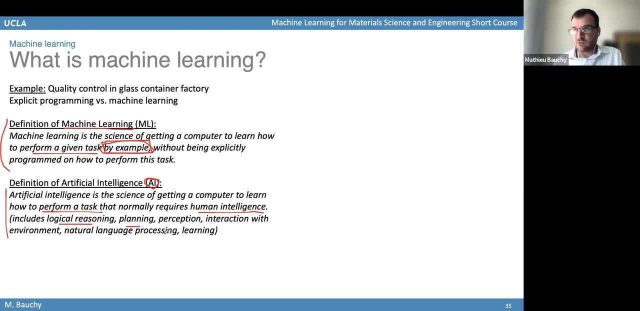 Like planning: How to plan different actions in a way to achieve a given task. Perception: How to perceive your environment, How to analyze what you see, How you analyze what you hear Or what you can feel, Like with all the five senses. 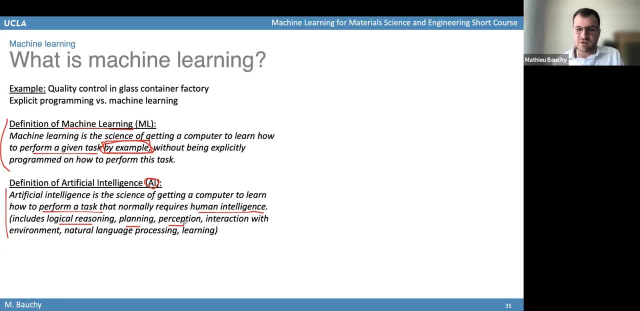 So the perceiving information About your environment. That's also a subfield of artificial intelligence Interacting with your environment Like taking some actions. Natural language processing. This is about understanding language, Understanding some written instruction Or some vocal instruction. 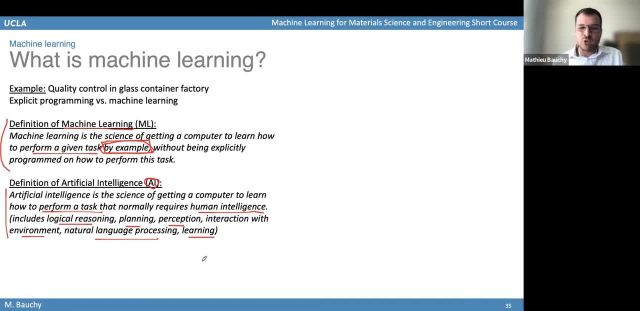 Or the process of learning in general. So those are all subfields of artificial intelligence. So again, artificial intelligence is something that is more general than machine learning. Machine learning is a more specific subfield within artificial intelligence. And then the last thing: another common term that is used is data science. 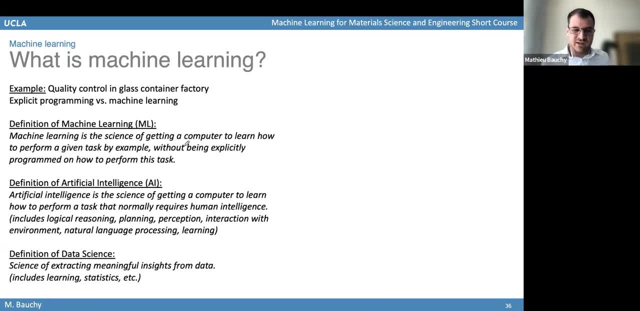 So data science- the way I would define this is- I would define it as the science of extracting meaningful insights from data. So in that case, that includes the process of learning from data. If you have some data, you want to learn something based on those data. 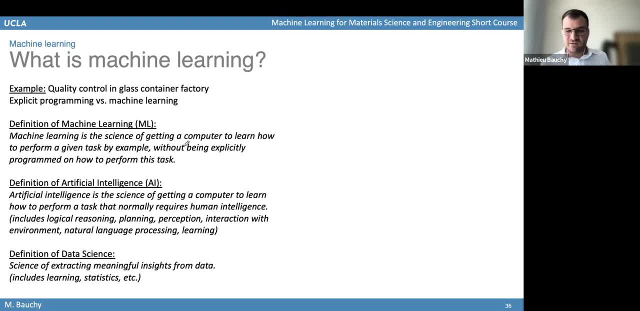 So that's data science. It also includes statistics, So generating some statistics based on some data, That's part also of data science. So those are three things: Machine learning, Artificial intelligence, Data science. Those are three fields that can be used for materials, informatics. 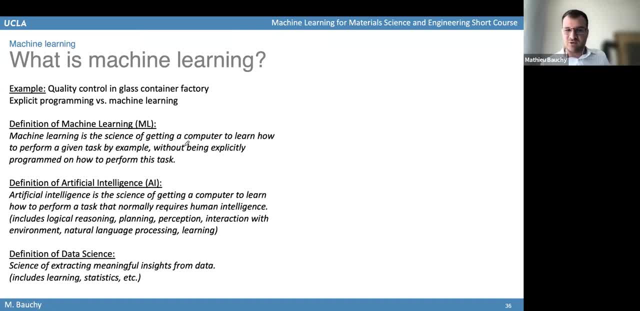 That can be used to discover materials or optimize materials, And so if we were to summarize this, So you have, Like, the field of AI, So we can represent it as a potato, like this. So that's the field of AI, And then you have the field of data science. 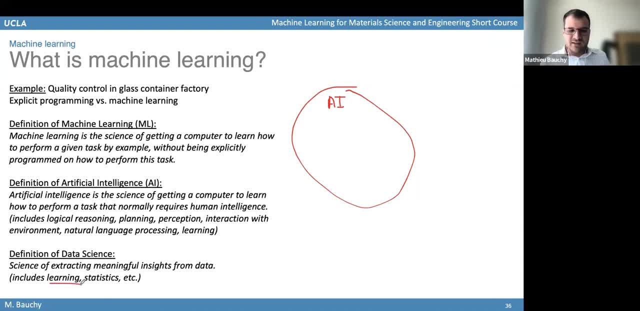 And so, if you see the definition here, data science includes learning from data And AI also includes learning from data. But data science it also includes other things, For example, statistics, The fact of coming up with some statistics based on some data. 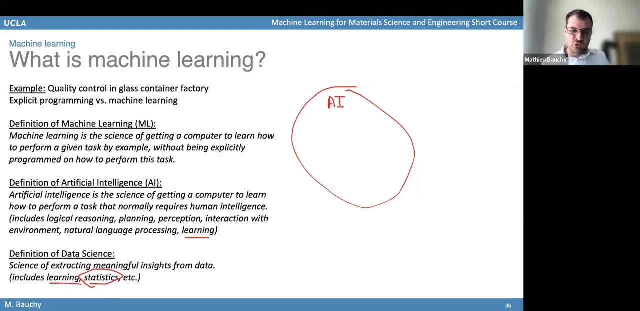 That's something that falls within the reach of data science, But it's not part of artificial intelligence. So, to summarize like we can represent this like this: You have AI, Then you have data science. They have some intersection. There is some intersection between data science. 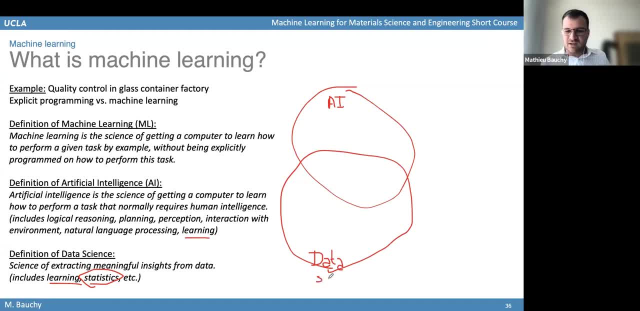 And AI, But it's two different things. So it's like two circles that have some intersection, like this, But it's not like a circle. It's like a circle. So it's not like a circle, But it's not like one is completely containing the other. 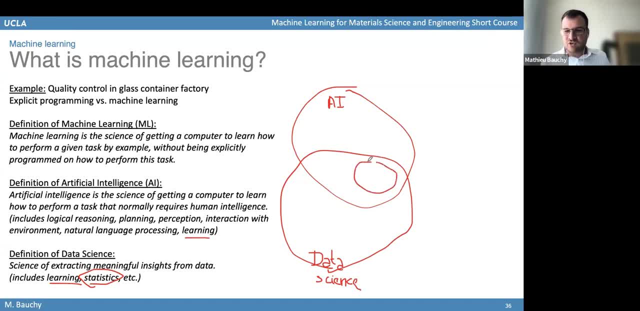 And then somewhere here at the intersection of AI and data science. this is where you have machine learning. Machine learning is a subfield of data science, because machine learning only deals with data, But machine learning is also a subfield of AI. So machine learning would be somewhere in the intersection of artificial intelligence and data science. 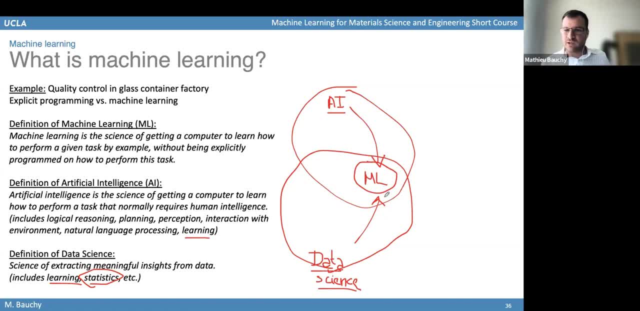 So this is what we are going to talk about specifically during the rest of today- is specifically about machine learning. We won't talk so much about all the application of artificial intelligence or all the application of data science. We're really going to focus on this machine learning, which is at the intersection of artificial intelligence and, specifically, the process of learning. 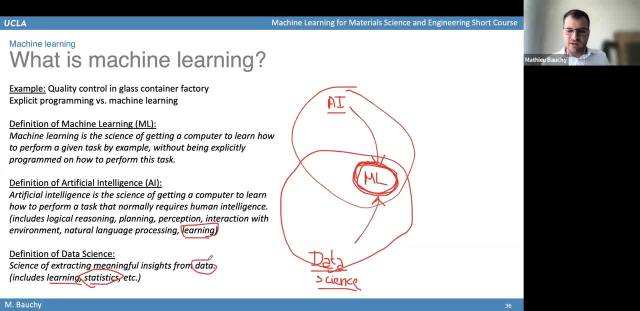 And to learn this based on data, based on getting some insights based on data. So that's it. That's really what machine learning is. It is at the intersection between learning, but learning based on data, learning based on example, not learning based on explicit instructions. 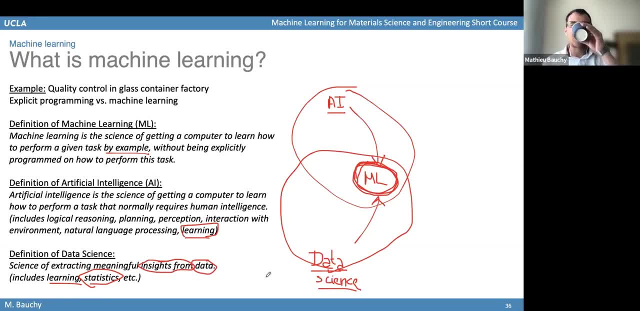 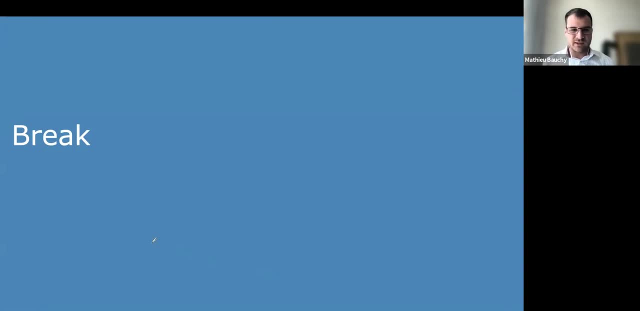 Do you have any questions regarding this so far? Okay, So I think maybe now is a good time for a short break So that we- you can relax a little bit before we continue. So just as a reminder. so this course is supposed to be about six hours. 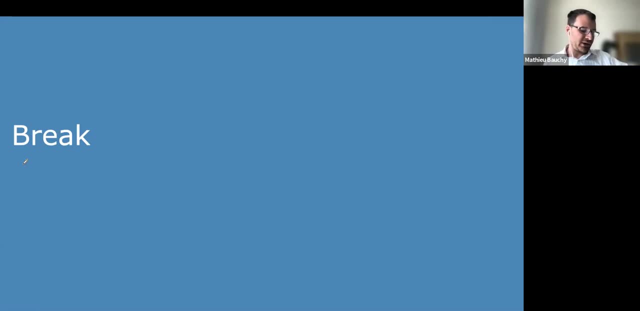 So I think we. so it's about two hours already now, So I think we can have a 15 minute break and we can restart in 15 minutes. So like at least for my time here, it will be noon 12 pm. 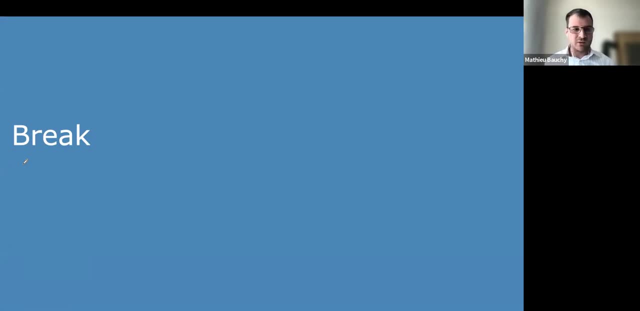 So we can restart that at 12 pm. Meanwhile, if you have any questions, let me know, otherwise I'll see you in 15 minutes. Okay, Thank you, Thank you. Okay, Welcome back. So we are going to to restart. 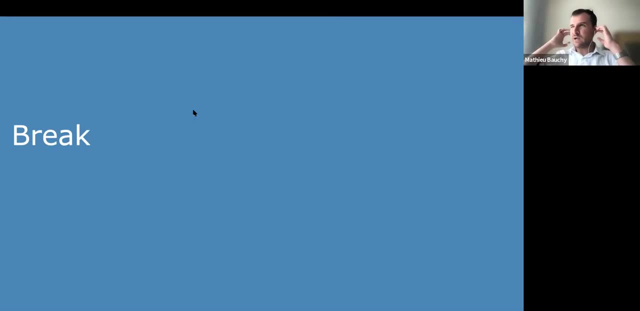 So what we are going to do in the in the following two hours is to start to see more technical detail of what our machine learning, what are the different types of machine learning approach And what are some example of how you can use those approaches to to solve problems involving materials. 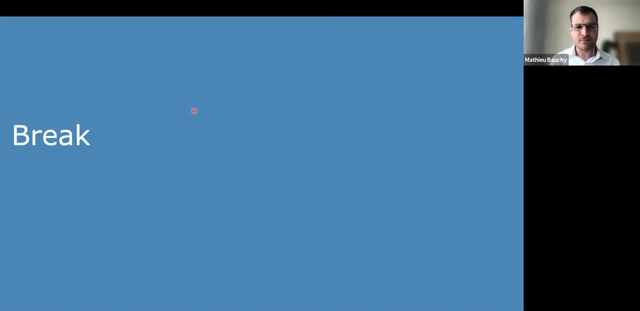 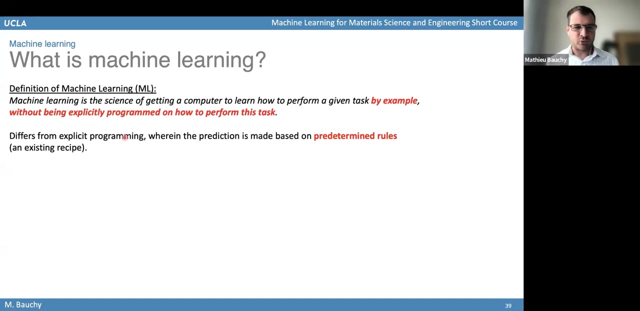 So let's, let's resume the course. Okay, So let's restart from where we stopped before the break. So as a reminder. So we define machine learning as the science of getting computer to learn how to use machine learning. Maybe it's a robot or maybe it's like a computer. 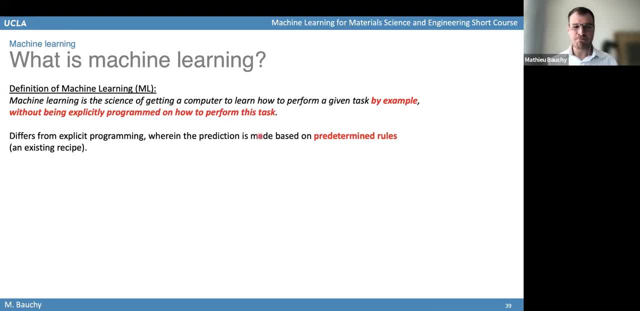 But I want to say that to a computer, the imagination begins with thinking. Okay, So machine learning, that have a computer to learn how to perform a given task by example, without being explicitly program on how to perform this task. So that's really the the. 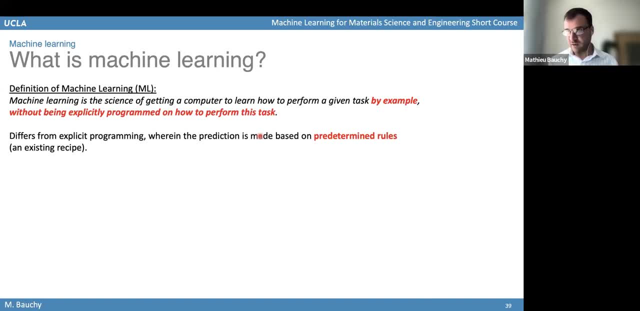 The key aspect of machine learning is that you don't have any predetermined rules, like you don't have any recipe that you can know to to to make a prediction, Like, for example, if you want to predict a property of a given materials based on its 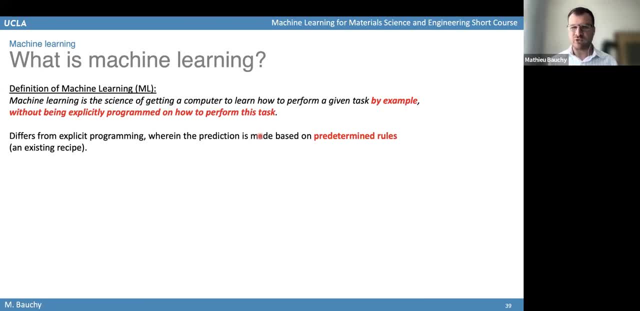 chemical composition. We don't have any rules how composition will affect the priority. you will just learn this by example, by by examining existing data. so that's the main difference between explicit programming, when you have some rules already, some knowledge, and machine learning, where you have no rules you want. 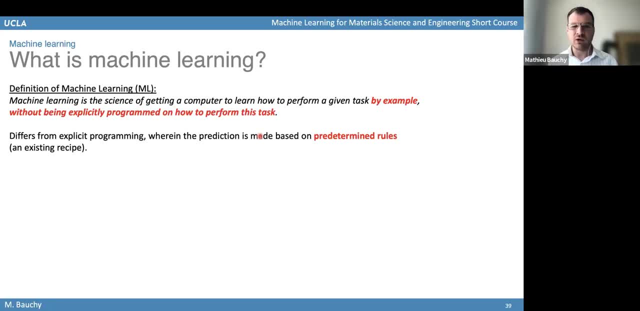 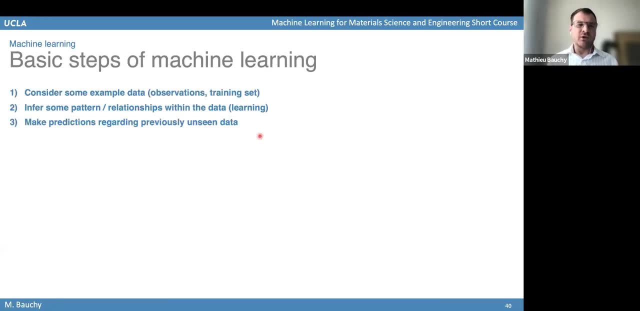 actually to generate those. you want machine learning to tell you what are the rules that you should use to convert a composition into a priority. so the the key steps of any machine learning approach will be those three steps. first, you need to have some data. the that's the first. 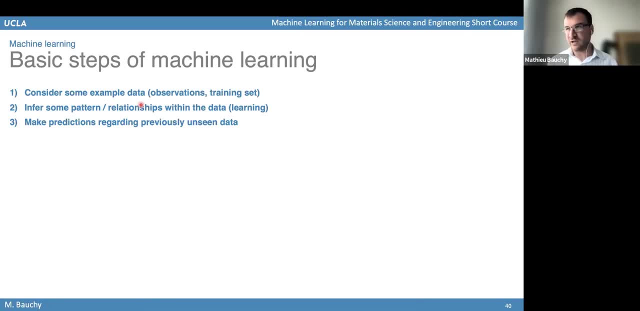 thing about machine learning. machine learning does not rely on knowledge, it relies on data. so if you don't have data and if you don't have good data, then you won't be able to use machine learning. so you need to have some data, so that can be some data about, some information about different materials, together with the the. 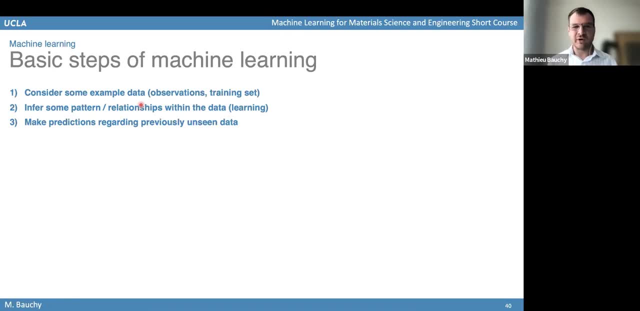 property that have been measured for those different materials, or it can be some data about the same materials subjected to different condition of temperature, different condition of pressure, different condition of irradiation, and then the knowledge of how those conditions have affected the performance of the material. so any any time you have some data about material. your machine learning application will be looking at that. you don't have a committee and you also need that data to do that machine learning application. machine learning is offer an opportunity to be taken as the common technique of manufacturing science and industry but beyond the common topics also. we 그러� is also useful when you are using machine learning. 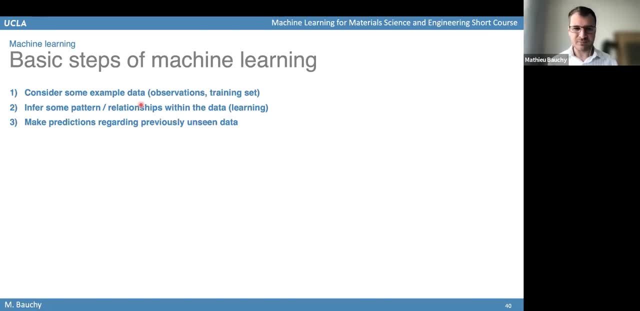 then this is where you can start to use machine learning. Then the second step is: once you have those data, then you will move to the learning process. So you will use a given machine learning method And what this machine learning method is going to do. 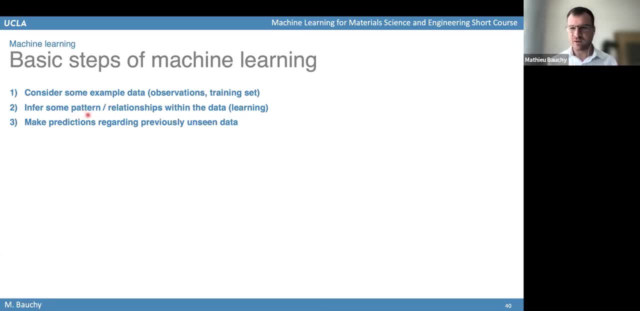 is to try to look at those data and infer some patterns. Do you mind muting yourself? if you, Let me see if I can see who it is now Okay. so again, the second step will be to find some patterns or some relationship within the data. 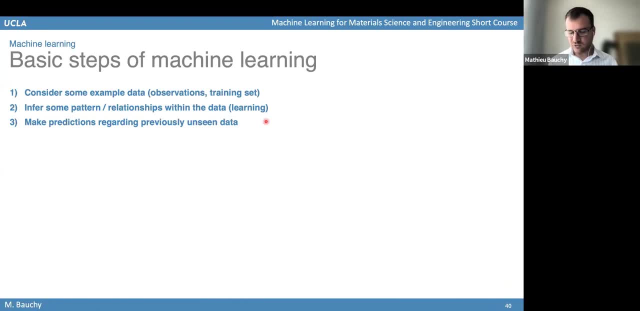 So that's the process of learning, is the process of using your machine learning algorithm to find some relationship between some inputs and some outputs, for example. So, for example, you will provide a lot of data with different materials, different composition and different properties. 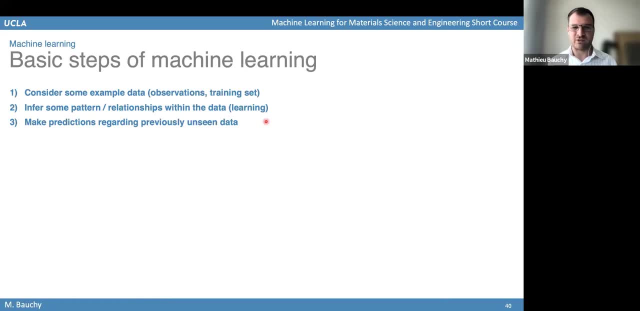 And the machine learning model will try to find some patterns, will try to infer a relationship between composition and priority. The next step is that once you have found those patterns, then the machine learning model, learning model, will give you some rules and then the next step is that you can use some rules to 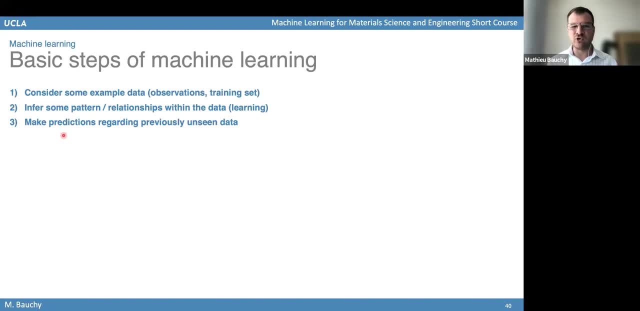 make some prediction about materials, new materials that you have never seen before. for example, if we come back to the example of the, the, the glass container that i gave previously you, you will take the step. one will be to to to gather a lot of pictures of glasses that are broken and a lot 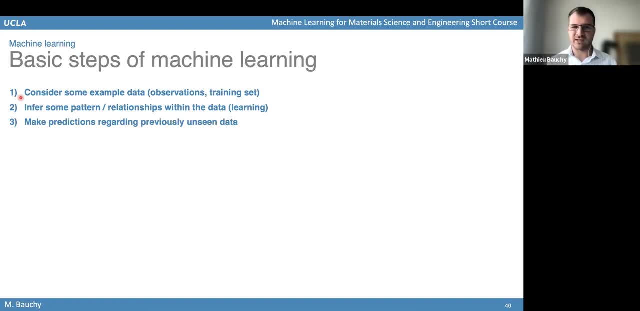 of pictures of glasses that are not broken. so that's going to be your, your data. then you will feed that to some machine learning and the machine learning model will learn how to recognize a glass that is broken from a glass that is not broken. so this is the process of learning: it will find. 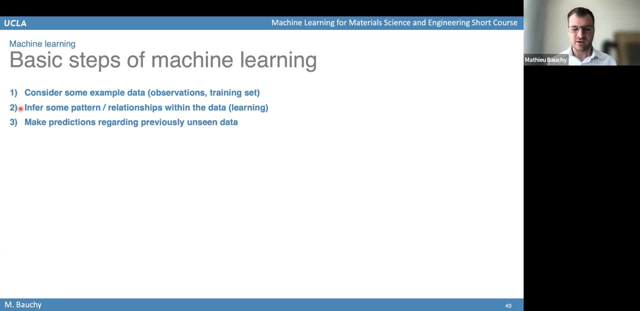 some patterns within the photos to recognize what distinguishes a broken glass from a non-broken glass. and then once you have- uh, once the model has learned, then it will have generated the rules that can be used to distinguish a glass that is broken from a glass that is not broken. and now the last step is you can use those, those rules, and now take a. 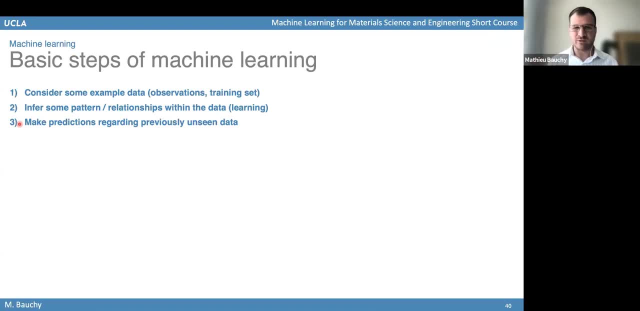 new picture of a glass, for which you don't know if this glass is broken or not, then and then you can apply those rules that the machine learning model has has learned and make a prediction for this glass. the model will predict: is this glass broken or not broken? so once you have used 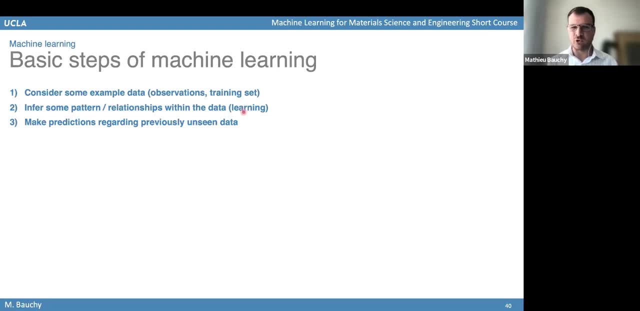 the data coming from the previous example to come up with the rules Now. after that, you can use those rules to make some prediction about new materials that you have never seen before. So that's the basic aspect of machine learning. That's what makes machine learning powerful. 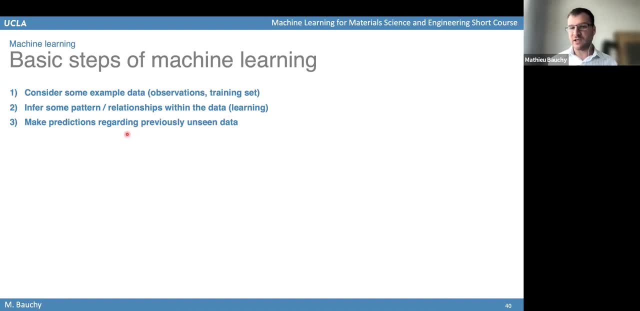 is that you start with some example. The machine learning learns some rules based on those examples And once you have done that, then you can use those rules to make some prediction for new material that you have never seen before. So you can make some prediction. 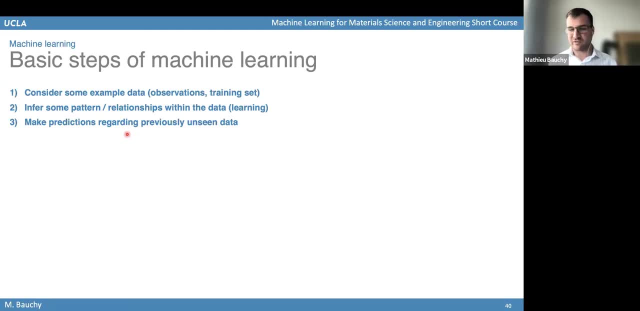 to predict the performance of future materials that you have never tested before, simply by learning from existing data. So an example for this. so, for example, like you would consider the asset of materials. So you have a list of materials for which something is changing. 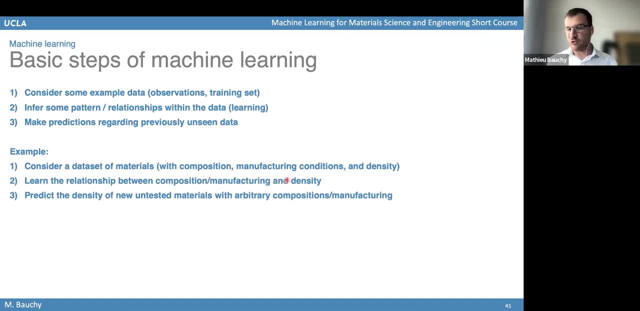 That can be. the composition is changing or the manufacturing condition is changing, like the temperature is changing, pressure is changing or relative humidity, Humidity is changing, something like that. Something is changing either in the material itself or in the condition, the environmental condition. 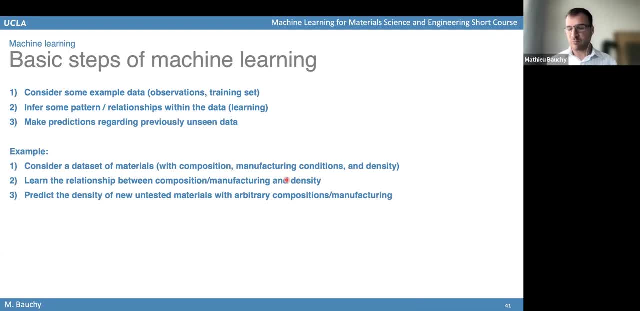 And so for this, you also have a property that you are measuring. For example, you are measuring the density of this material, And your goal is to try to predict how the composition of this material and the manufacturing condition, how does it affect the density of this material. 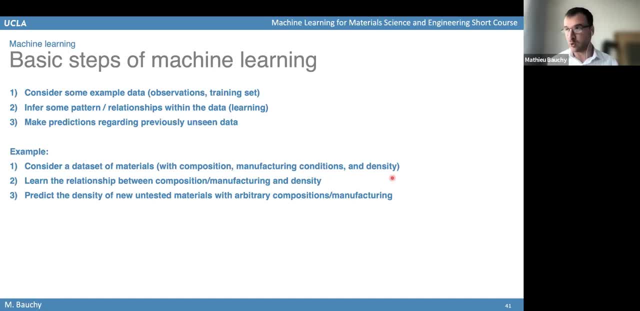 Maybe because you want to generate a new material that will have a very low density. So then, the second step is, once you have this data set, you will expose this data set to a machine learning algorithm, And this machine learning algorithm will gradually learn by looking at those data. 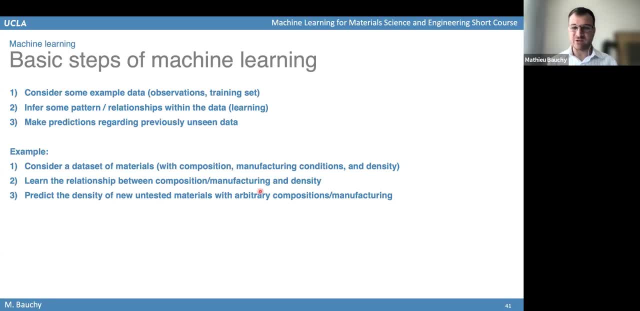 it will learn how to convert the composition and the manufacturing condition, how to use that to predict what will be the density. And once it has learned how to transform the composition and the manufacturing condition into a density, then you can use it to predict the density of new materials. 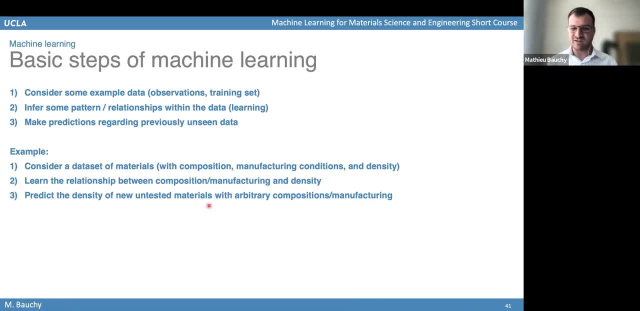 that you have not tested yet. So you can say that if I take this material and if I change its composition or if I change its manufacturing condition, then I predict that the new density will be equal to a given value, which will be the value predicted by the model. 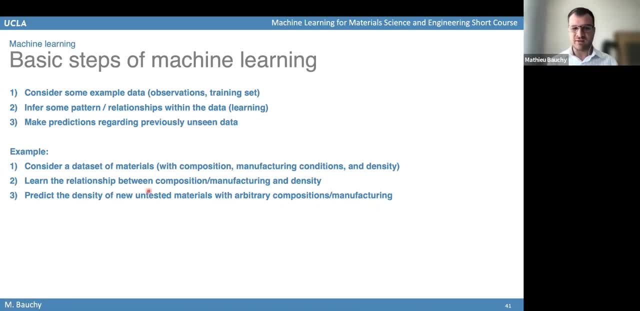 And so that's very powerful, because then it means that once you have this model that is trained, then you can directly predict if you change the design parameter of your model, how will that affect the performance of the model. So you can do that without having to actually make the material. 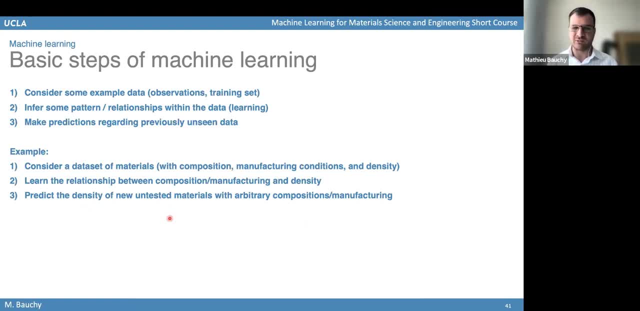 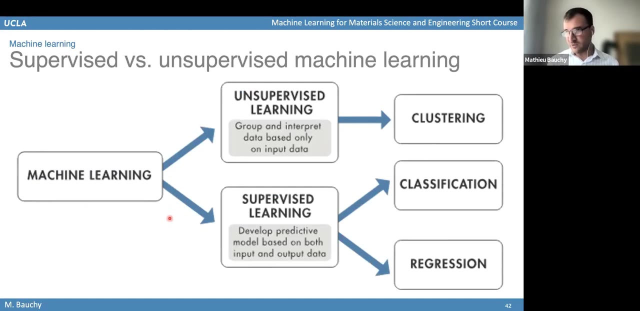 and having to test it. You can just simply use your machine learning model to quickly predict how each design parameter will affect the properties of the material. Okay, so now let's move more into the more detailed about machine learning and the different types of machine learning techniques. 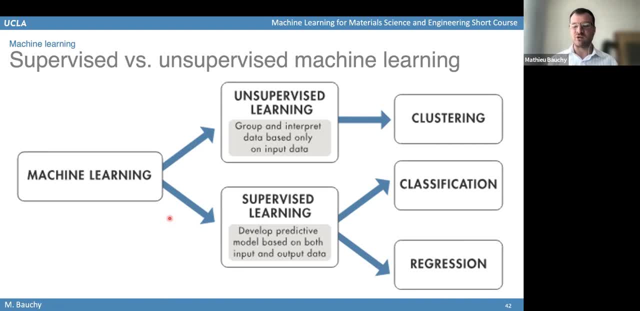 that are available and how you can classify those techniques into different groups of machine learning. So, when it comes to machine learning, there is really two main families of machine learning techniques. There is what we call unsupervised learning and what we call supervised learning. 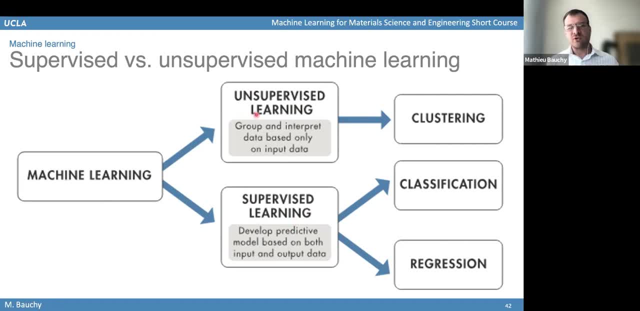 And so we're going to talk about the difference between those two. So, when it comes to unsupervised learning techniques, the idea of unsupervised learning techniques is when you have some data, but those data do not have any label. What I mean by that is: let's assume that you have. 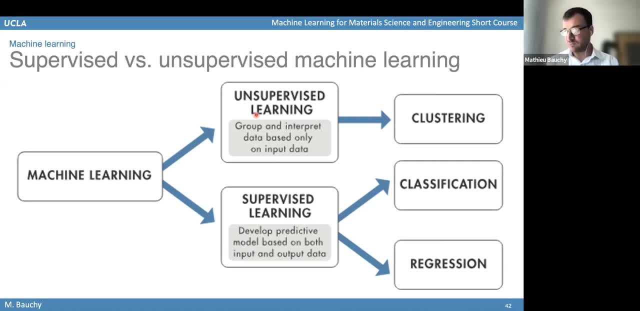 different types of materials, but you have not tested their property yet. You just have different types of material. You know some information about those materials. you know their composition, you know the temperature, you know the pressure that you use to synthesize these materials. 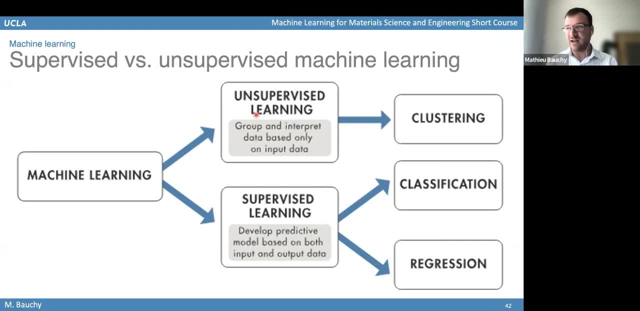 but you don't know any properties. You don't have any label attached to those materials, any property that have been measured. So in that case, if this is the information that you have, then the type of technique that you can use is unsupervised learning. 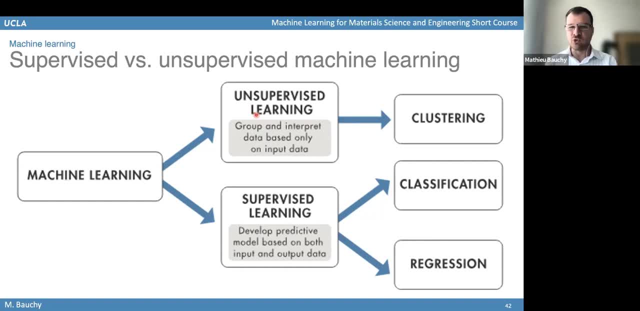 The types of action that you can do using unsupervised machine learning is to analyze those materials that you have and group them into clusters, into groups of different materials that have some similarity between each other. So I'll show you some example of that. 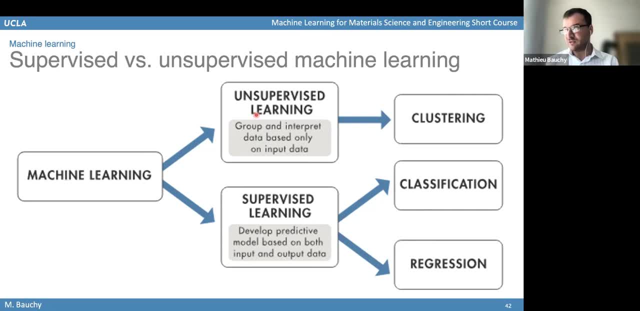 but you can think about this as, for example, if you have a list of different materials with different compositions, different processing temperature, pressure, et cetera, if you are interested in grouping those materials into different families or different groups of materials. 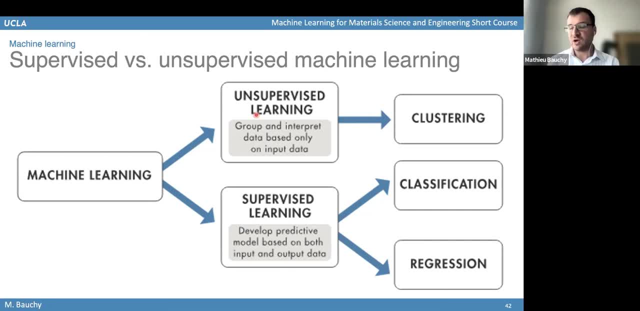 then you can use unsupervised machine learning. unsupervised machine learning in this case will analyze data and we'll try, for example, to find some similarity between groups of data, identify groups of materials that appears to be similar to each other. So that's one thing that you can do using 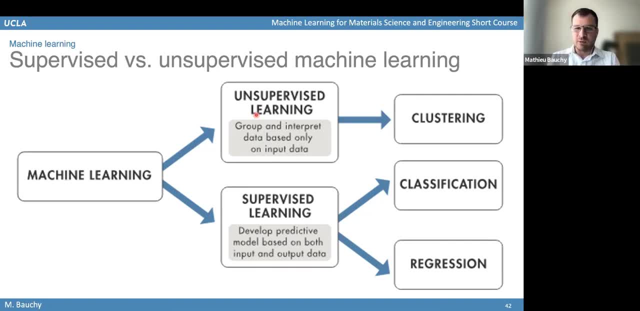 unsupervised machine learning. This is when you don't have any label attached to the material. you don't have any property that have been measured for those materials. Another example of this would be: if you have some pictures of materials, you just have a lot of pictures of. 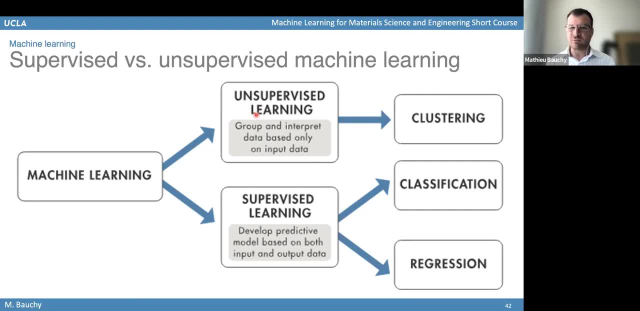 a lot of materials, but you don't know. you have not measured anything about this material or you don't know if this material is compliant or not. You just have the pictures of the material and that's it. You can use unsupervised machine learning to take those pictures and identify. 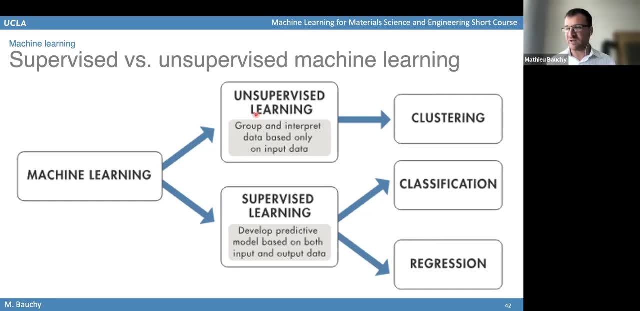 which pictures are the most similar to each other, to identify some groups of materials that appear to be similar to each other. So that's one thing that you can do using unsupervised machine learning similar to each other. So that would be one example of unsupervised machine learning, And 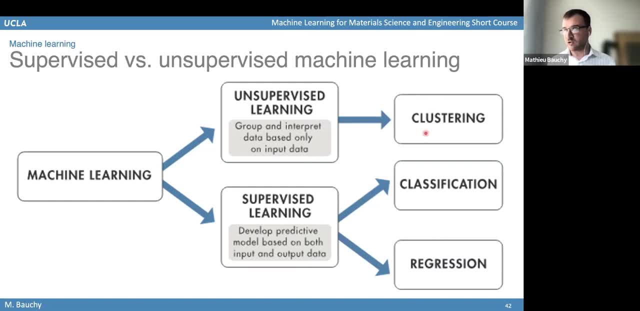 the main example of unsupervised machine learning is clustering. It's clustering algorithm that can identify groups of data points that are similar to each other. Another example of unsupervised learning would be to identify outliers. If you are producing materials and at some point there. 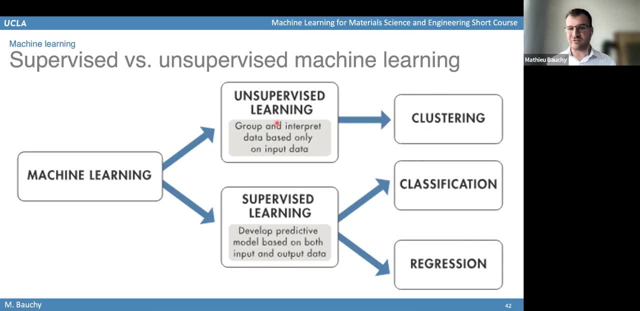 is one material that you produce that appears to behave very differently from all the other materials, either because there has been a mistake in the measurement or there has been some kind of think something went wrong in the synthesis of this material. In that case, this material is: 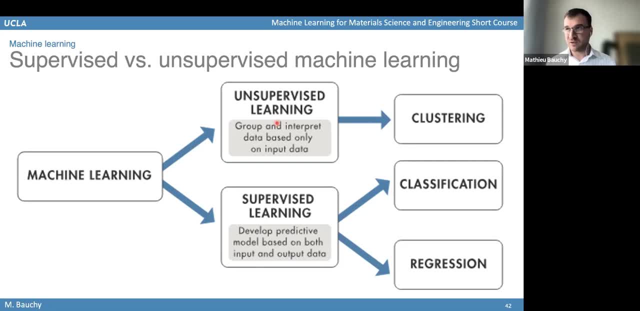 going to act as an outlier. It's going to act differently from all the other materials, And so usually it's due to some mistake by either in the synthesis of this material or in the outlier, And so usually it's due to some mistake by either in the synthesis of this material. 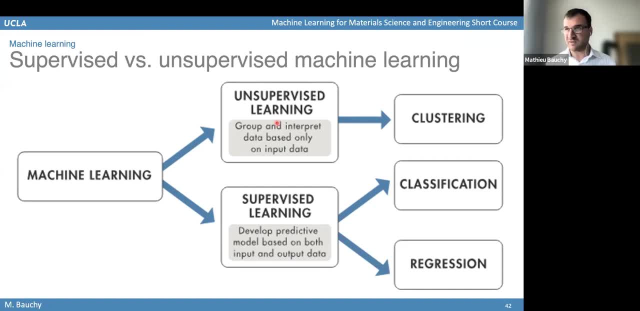 mistake in the measurement of the property of this material and, in that case, identifying outliers, identifying materials that appear to behave completely differently from all the other materials. that's something you can also achieve using unsupervised machine learning, because you don't have any label, yet you don't know what is the characteristic of an outlier or what is the 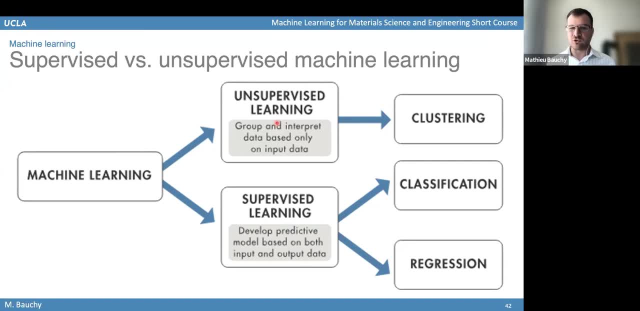 characteristic of a non-outlier. you just know that you have one point here, and this point, this material, appears to be very different from all the other materials, so that would be an example of unsupervised learning. and then you have the other example, which is supervised learning, which. 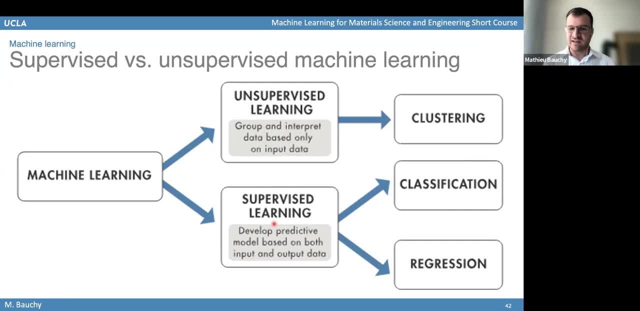 is kind of the opposite of unsupervised learning, in the sense that now you have some labels, it means that now you have some, some, a list of materials for which you know both the, the design parameters, so you know the, for example, the composition of the material, you know the, the processing condition, you know 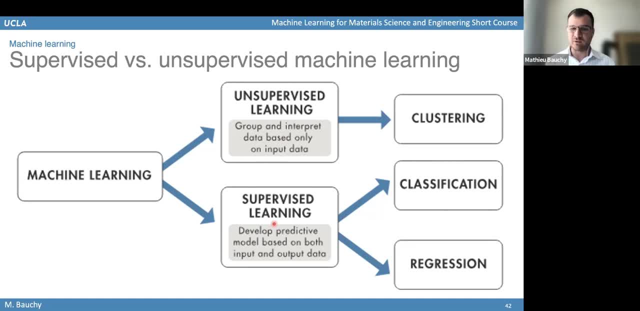 the temperature that was used to to make these materials. but you also know a label, you know an output, so you know a property that has been measured for this material. so, for example, you have measured the density, you have measured the elastic modulus, you have measured some mechanical 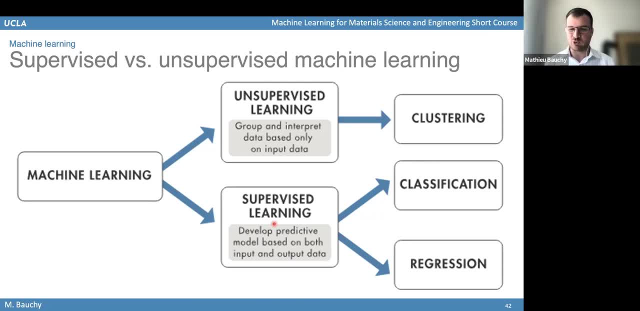 properties for these materials or any other types of property that has to be measured. and in that case, what you will want to do in this case is to build a machine learning model that can transform the input and use that to predict the output. so you will want to build a model that can take as input the composition, the processing, 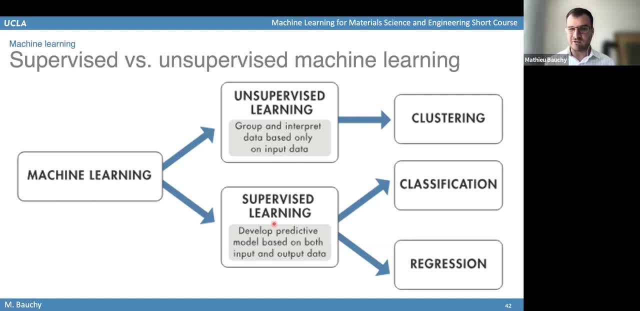 condition and use that to predict a given label, to predict a property that that you have been measuring. so in this case, when you want to predict something, predict an output, then that would be the the case of supervised learning. supervised learning where, in this case, you already have some example of materials for which you have both the input, the design parameter, and you also have, for the same example, the output that you want to predict. 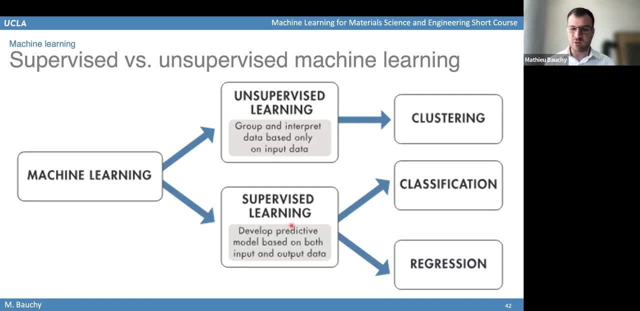 So in this case, when you have both in this information, that mean that in that case we call this a labeled data set as the data set for which you have the label, you have the output already. You will be able to use supervised learning in this case, and there is two main class of supervised learning. One is classification, One is regression. so we are going to talk more about what this is, but in the case of regression, typically it means that your goal is to 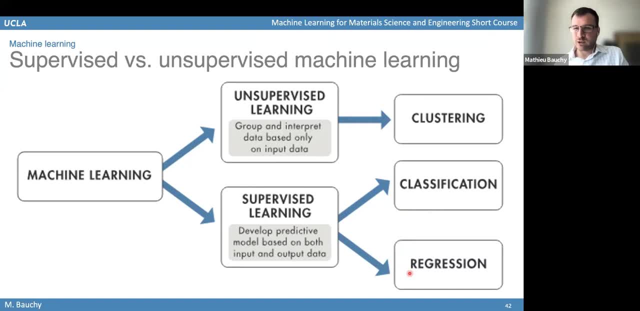 predict a property of this material that can continuously change. for example, if you are predicting the density of a material, density is a number that can continuously change, So that just a number that can have any value within a certain range. in that case you would use a regression techniques. But sometimes what you're trying to predict is not the number, it's more a class sample you can. what you want to predict is whether a material 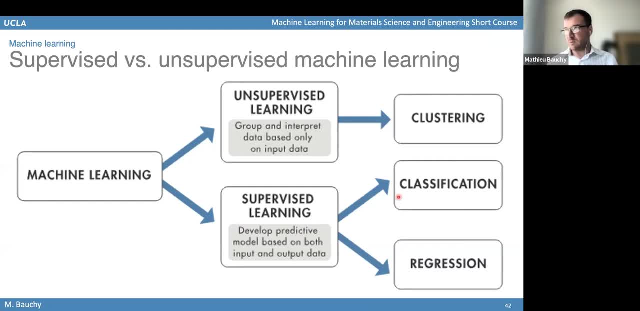 will form or not, or you will want to predict whether a material will be transparent or not, or whether material will break or not. in that case, you don't want to predict a number. You want to predict a number, You want to predict a class, you want to predict. 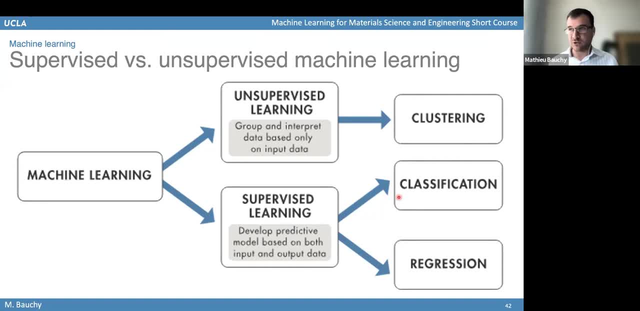 You want to predict a characteristics of this, of this metal. that won't be a number, that will be like more like a condition, something like a yes, no, it will be more like a classification level. you will say: I want to predict whether this material is transparent. 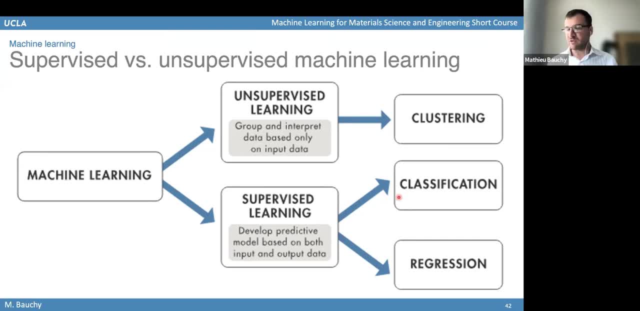 or not transparent, or I want to predict whether the the color of this material and the material will be either red, blue or green, And that's not something you can easily quantify with a number. you will just have different classes, the red material versus the blue material versus the green material versus the yellow material. 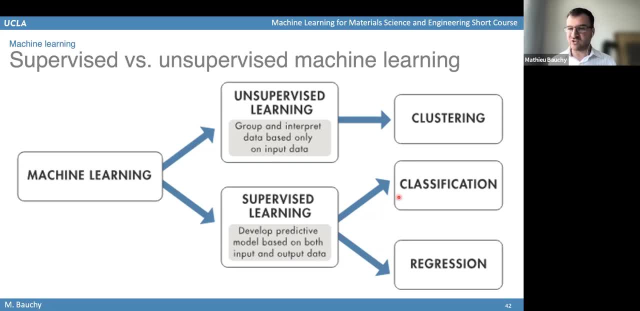 And in that case you want to just predict in which category This, this metal, is going to be. in that case that would be a classification problem. So those are the two types. classification: You want to predict the category regression. you want to predict a continuous number, a property of a material like it stands here. 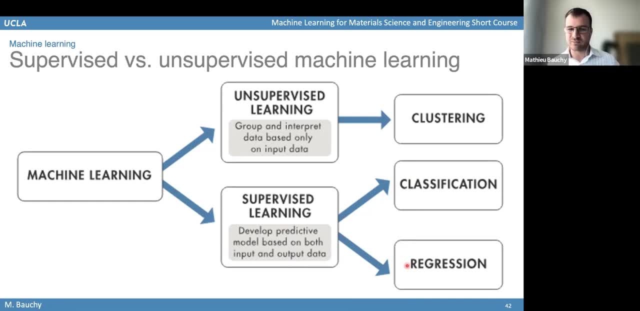 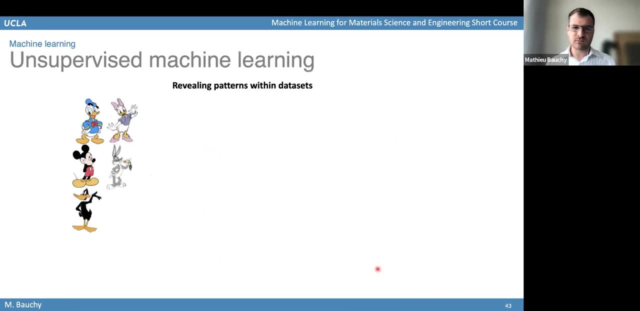 like its density, its models, et cetera. So those are the two types of supervised learning techniques that we are going to talk about. So let's start with the case of unsupervised learning. So here again, in this case, 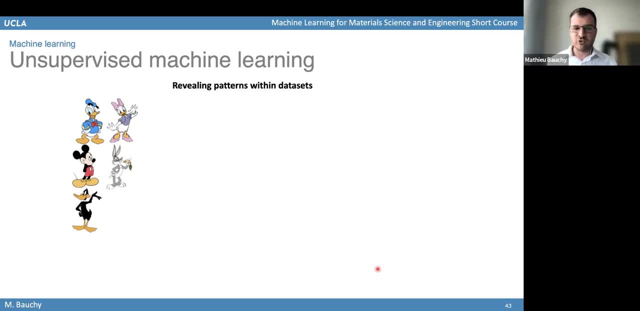 in the case of unsupervised learning, you have some data but you do not have any label associated to those data. You have not measured anything. So, for example, let's take those characters here. You can think of those characters as some pictures of some materials, for example. 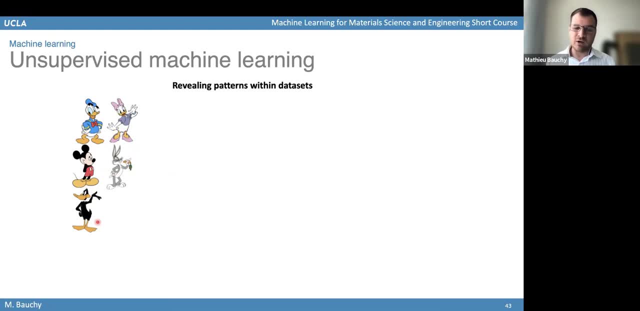 And so here you have a list of pictures of characters and what you want to do in this case. you don't know anything about those characters, You only have their pictures, and you want to group them into families of materials that appear to belong to the same family. 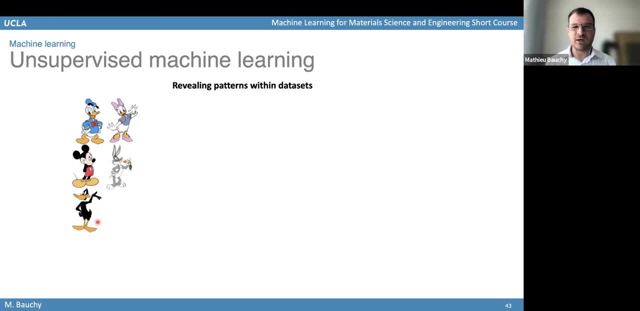 So you want to group them together. So the way the machine learning algorithm would do that is to follow an unsupervised approach and it will look at those pictures and it will try to identify some features in those pictures And we try to see which pictures appear to have. 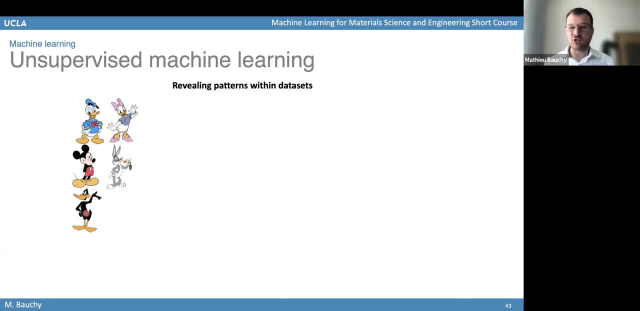 the similar features and which pictures do not. So, for example, if you look at those images, the first thing that you can look is maybe the color of the character, but in this case they all have a different color, So it's not a very useful thing. 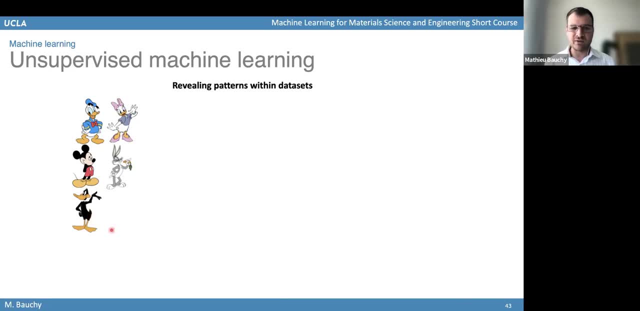 It's a useful feature to identify groups of character. Maybe something that can be more useful is to look at if those materials have ears or not, like, for example, like here: this Mickey Mouse has two ears, This rabbit also have two ears here. 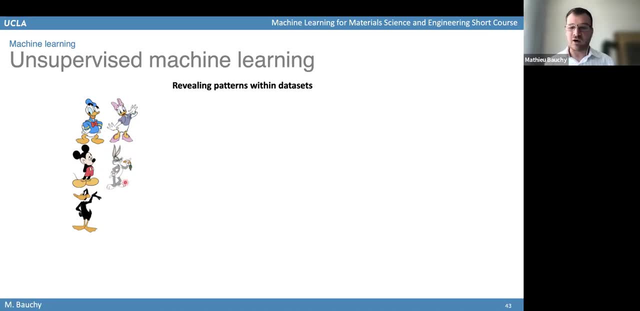 So that's, in this case, a common characteristics of those characters, but like most of them, in this case do not have ears. So that's not the most useful feature. if you look in more detail, maybe a better feature that appears to be more effective. 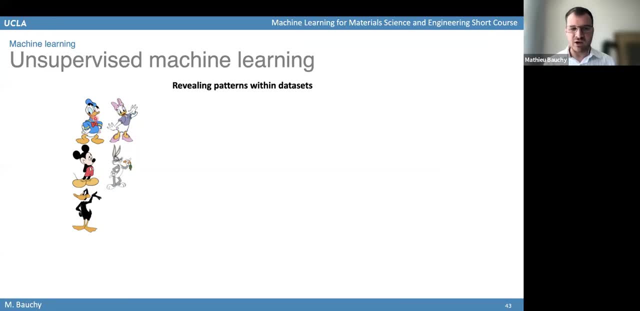 at distinguishing those characters is to check if they have like a beak, like the shape of their mouth Here. if you look at those three characters here, like this one, this one and this one, they all have a similarity: that they have this yellow beak here. 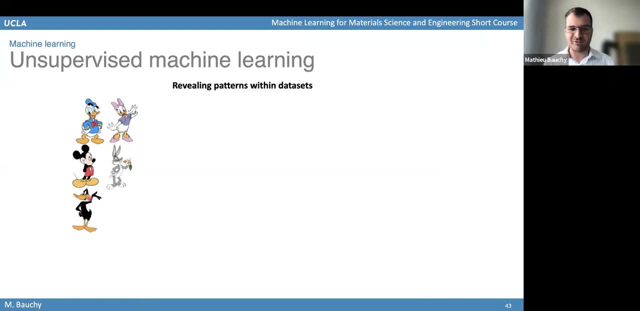 So they have, like, a very similar shape for their mouth, While on the other hand, like those two characters, they do not have these types of yellow beak, And so that would be, in this case, of features that the machine learning model will recognize. 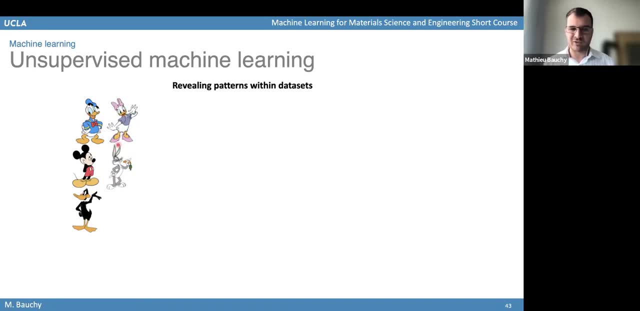 as being a feature that is very different for those two types of character. You have the character with the beak, that are most likely some kind of duck, And then you have the other characters which do not have a beak, which will be something else. 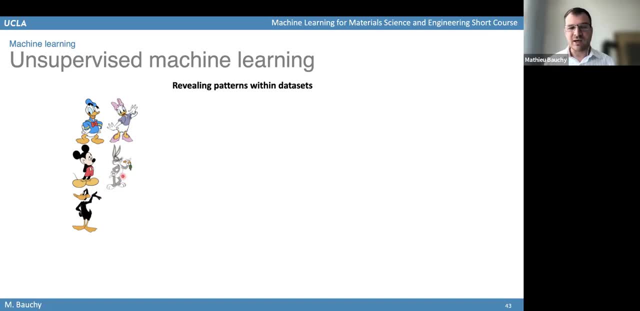 like either a mouth or a mouse or a rabbit, And so what the machine learning algorithm does in this case will do, is to look at those features and group those characters based on the one that have those similar features, like the yellow beak, and the one that do not. 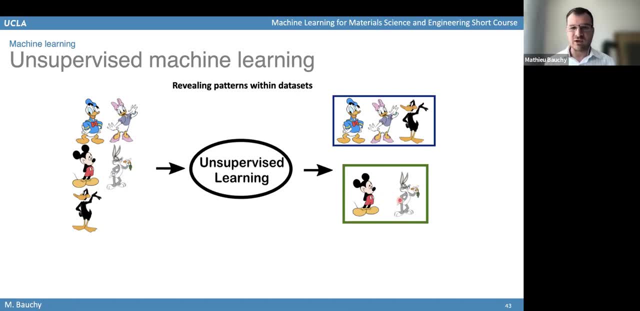 And so you can think of the same thing for materials. In that case, what this types of machine learning model will do is to analyze a lot of materials. You don't know anything about those materials, but you can just look at them and identify the one that looks similar to each other. 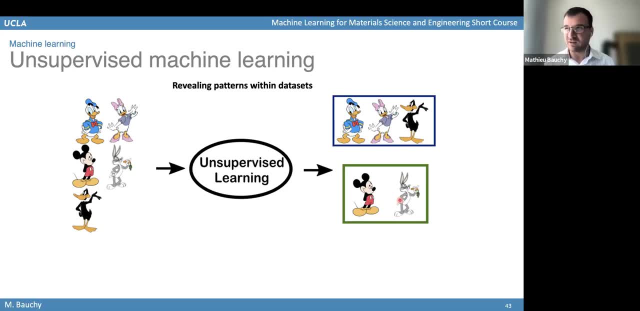 And so that's an efficient way to group material into different families: just by looking at some features of those materials and grouping them into materials that appear to have comparable features with respect to each other. So some example of application of this would be again: 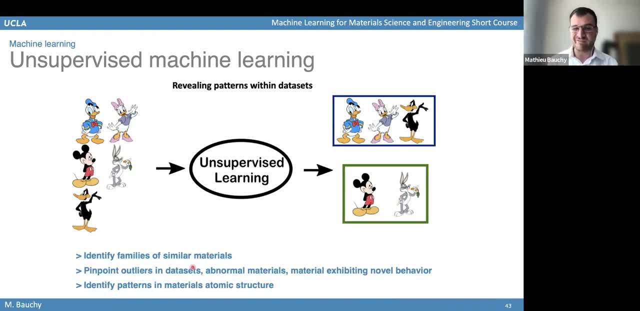 like you have different materials but you don't really know how to classify them into different families. So you can use these types of unsupervised learning to group materials together into several, several families of material. You can also use that to identify some outliers. 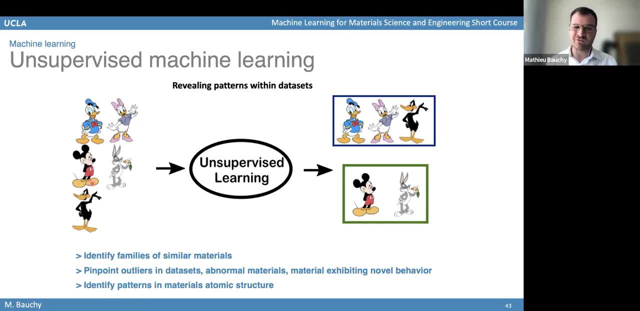 For example, like here, if you were to find a character that is completely different from the other. like for all of those characters here, they have two legs and two feet. If there was a character that has three legs, then that would be an outlier. 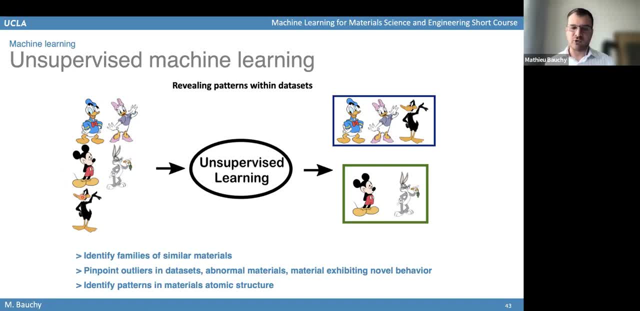 That would be a character that is completely different from the other, And you can use that to detect that. yeah, there is something abnormal, something unusual about this character, So that would be an outlier. something went wrong with this example. So in the case of materials, 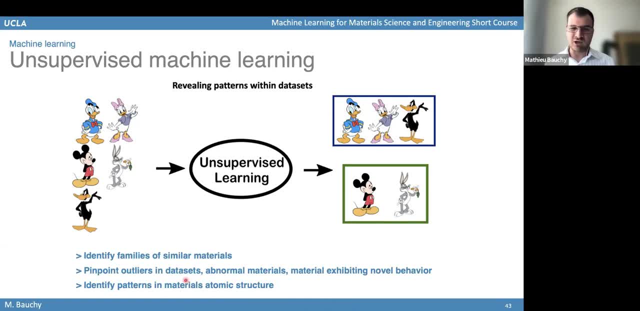 you can use that to identify. if a material is behaving completely differently from the others, then that would be an example of an outlier: a material that either something went wrong during in synthesis or something went wrong during the measurement of a property, And so this material either need to be checked. 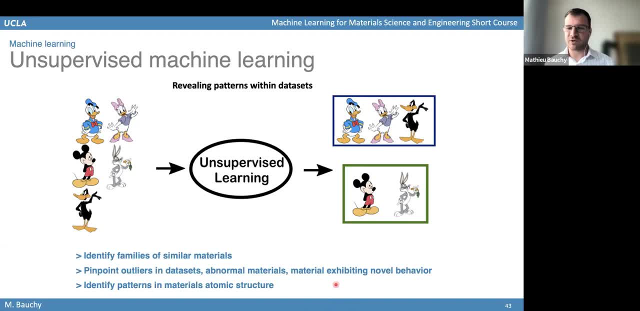 either needs to be retested, it's an outlier. So this is something you can achieve with unsupervised machine learning. The last thing that you can do is to: if you have some information about the atomic structure of those materials, then you can also use this information. 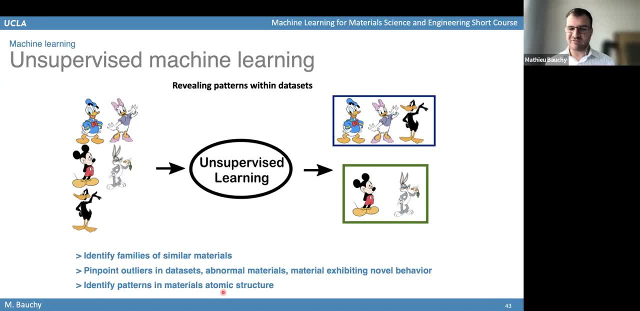 to identify groups of materials that appear to have similar atomic structure with respect to each other. So, again, that would be in that case an unsupervised learning process, because you don't know anything about those materials, except you know the atomic structure. 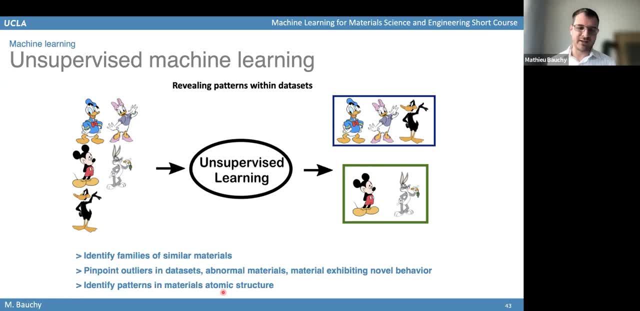 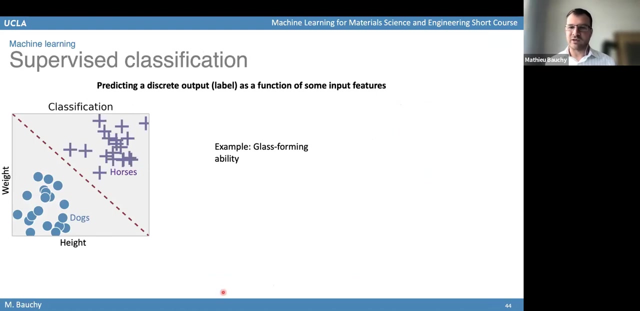 And in that case you will just use that to group material that appear to have similar atomic structure and separate them from others that have a different atomic structure. So that's about unsupervised learning. The second type of machine learning is supervised learning. 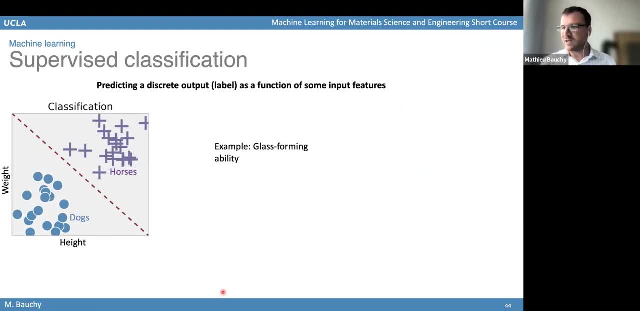 So in that case, that's the case where you have some label. So in that case you have something that you already know about this material. So you know you have some property that you want to predict, For example, in the case of the unsupervised learning. 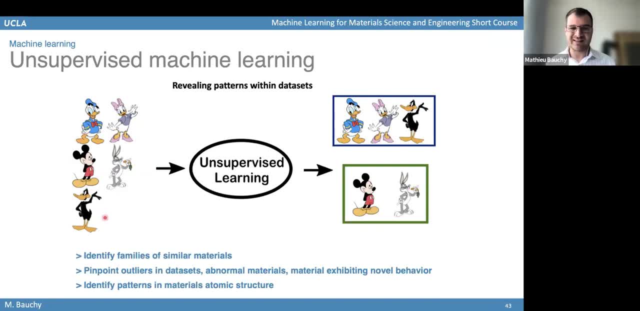 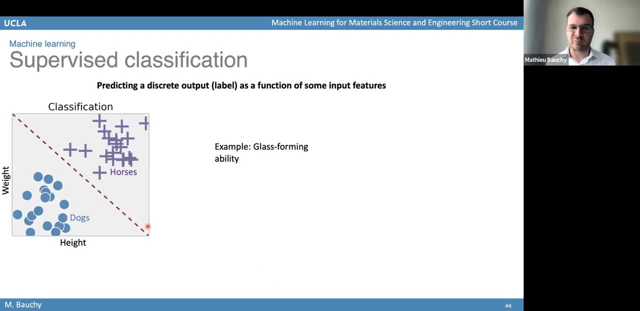 you just have the picture of those character, but you don't know what types of animal they are Like. you don't know that those are ducks, mouse or rabbit. Now, in the case of a supervised learning, you know, for example, what those characters are. You have a, for example, you have a wounds or wounds- You know you're this turns. those are clean, But these are kind of white spots from theanja so you can take a look and want to get the information signs or things running. So it's all really easy, depending on the exact quality And let's go to the grab feature for you. 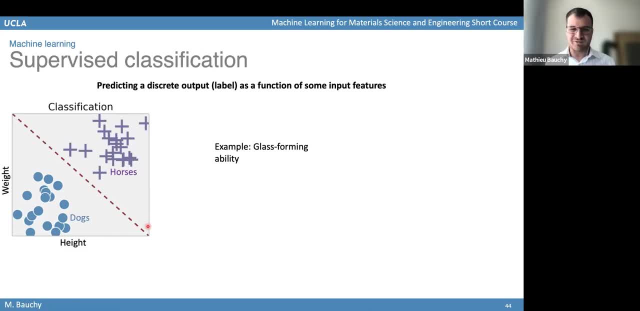 example, you have a list of pictures of animals and you know um what type of animal they are. so you have some example of pictures of of dogs, you have a some pictures of horses, and what you will do is based on those example of pictures. you will try to train a model that will recognize. 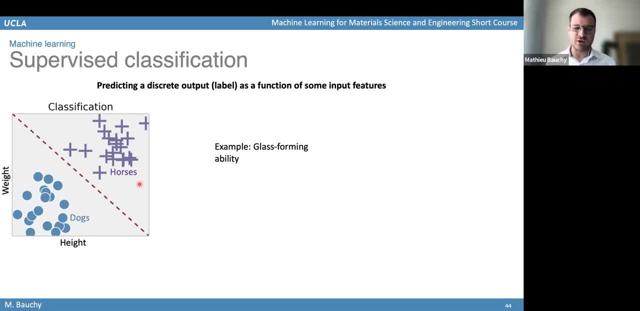 based on the picture to recognize whether it is a dog or a horse on the picture. so in that case that would be a classification problem, because you don't want to predict a continuous number. you just want to predict is it a dog or is it a horse, so that in that case it's just about. 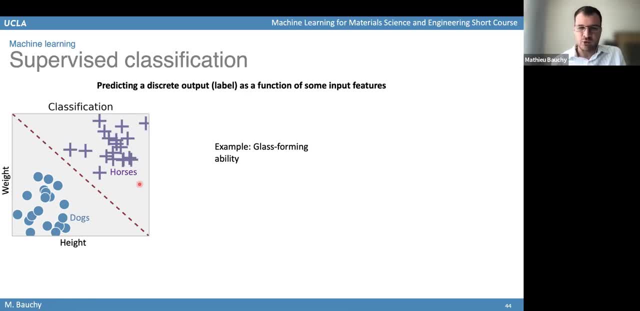 categorizing data. it's not about predicting a continuous number. so in that case, the way these types of classification machine learning would work is that you have some example of animals. those animals are already labeled, so they have two colors. you know whether it's a dog or whether it's a horse, and what the machine learning will do is it will try to. 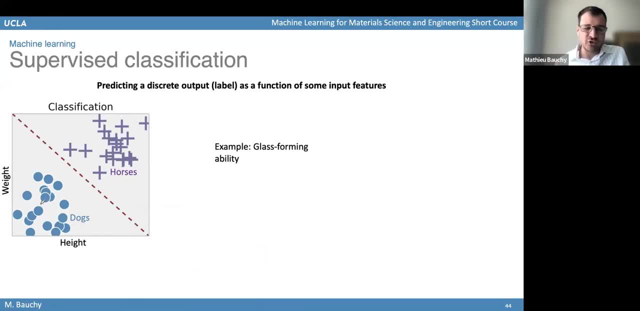 identify what are some useful features to distinguish those two types of animals. so, for example, you have the. if you know the weight and the height of those animals, then the machine learning model will recognize that if the weight is small or if the height is small, then it's very likely that 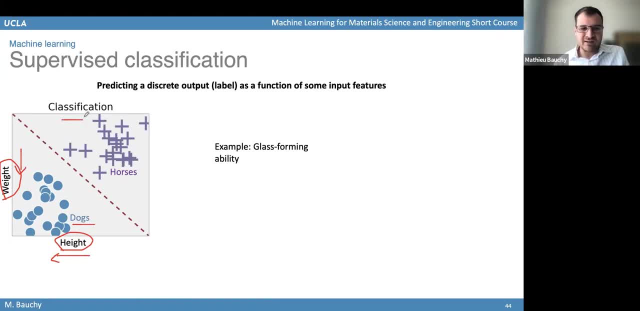 it is a dog. On the other hand, if the height is very high or if the weight is very high, then it's more likely that it is a horse. So in that case the machine learning model will identify those two features as being the very useful features. to find here a boundary, So it will find the 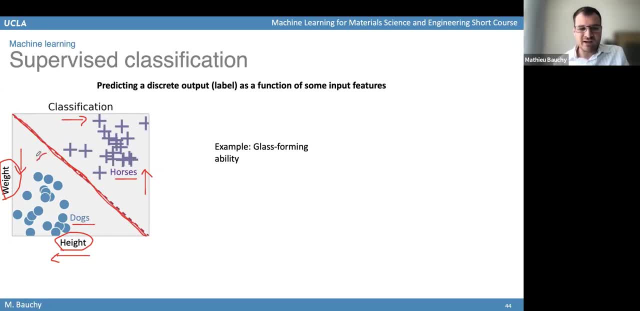 boundary that tells you that if you are on one side of this boundary, then you are most likely to be a dog, But if you are on the other side of this boundary, then you are more likely to be a horse. So in this case, this is an example of a classification problem where you have a 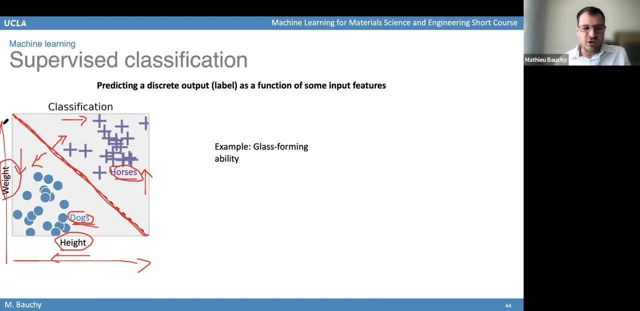 different features. Those features gives you a space, So you have different access. So here there is only two features, So it's a two-dimensional space. But for materials you can have much more features than that. You can have hundreds of features. So there are some features. 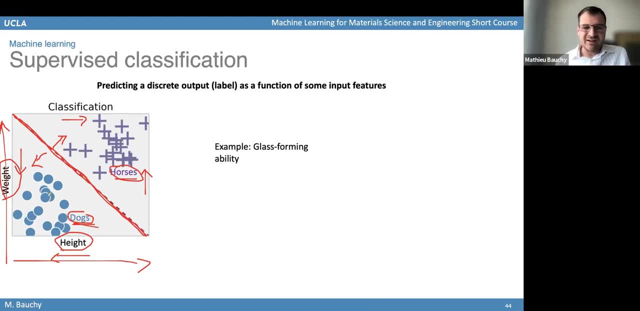 that describe your material And then you will have some example of materials. So each material will occupy one position within this feature space. So you will have a different example of materials that each of them occupies. So each material will occupy one position in this feature space, because they have one for each. 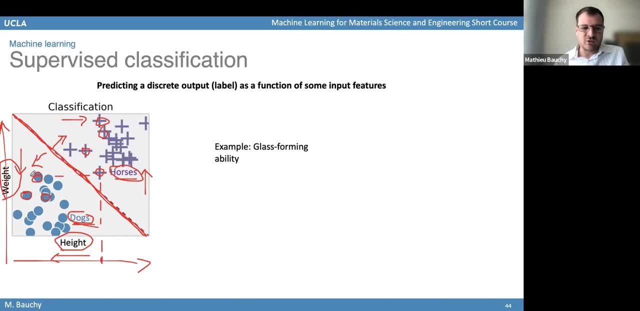 material, it will have a given value for each feature parameter, like in the same way that each material has each animal here has one weight and one height. So for each material you have the information of its weight or its height. So that would correspond for each animal or for each. 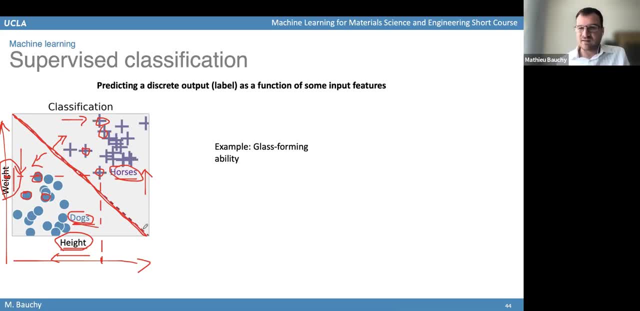 material that would correspond to one position inside this space. So that's what we have here, And then the machine learning model will learn how to find what is the best boundary here. So this boundary is called the decision boundary, And so this decision boundary. 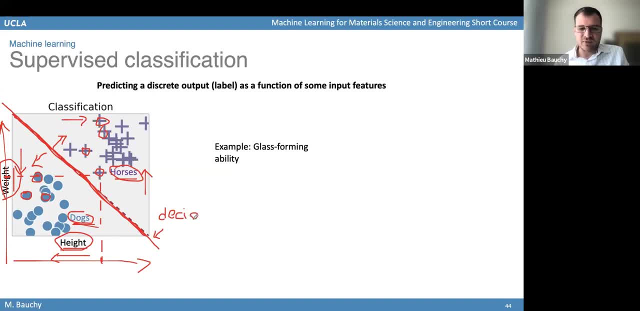 is like a hyperplane, or it's like either a line or a plane that separates the two classes of material or the two classes of animals, In this case. so the goal of this types of classification machine learning algorithm, in this case, is to 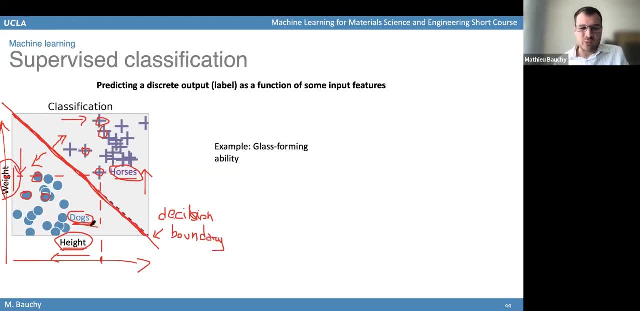 find what is the best boundary to separate different types of materials. So, by looking at various features of those materials, it will try to find what is the best boundary to distinguish, to classify those two materials into different families. And then, once you have this boundary, it 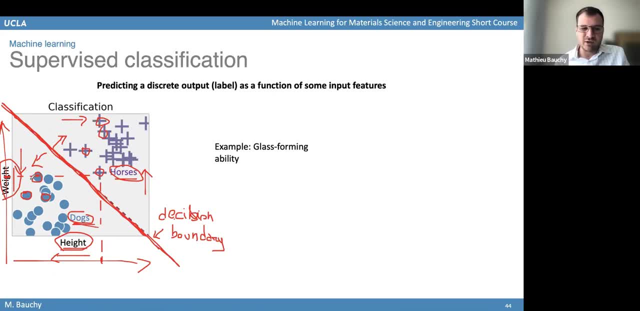 means that now, if you, if you, if you make another decision, you can measure the height of this material. And so, in this case, or if you, if you, if you encounter a new animal and if you don't know what this animal is, you will, you can measure the height. 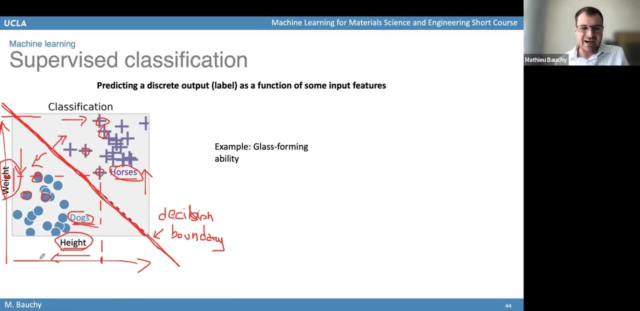 of this material, of this animal. you can measure the height of this material- So that gives you a new point here- And then you can check on which side of the decision boundary are you. If you are on the right side, then most likely it means that this animal is a horse. But on the other hand, if you 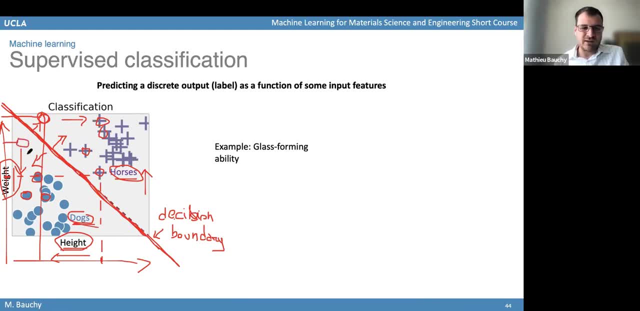 have another animal and you measure that this animal has a pretty high weight but a pretty low height, then it means that, on the other hand, this animal is very likely to be to be a dog. So once you have this decision boundary, this decision boundary gives you some rules that then you can. 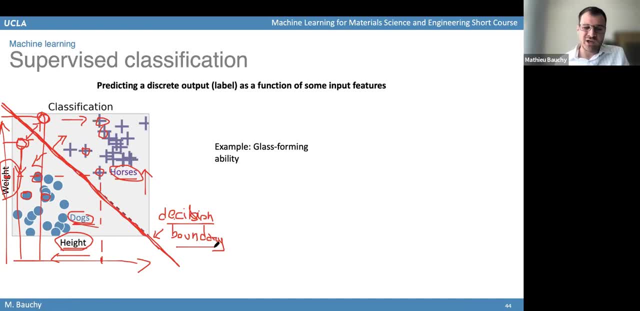 use on future animals and if you don't know what they are, you can, based on this decision boundary, predict if this material is going to. if this animal is to be a horse or a dog in this example, so it would be exactly the same for material if you have. 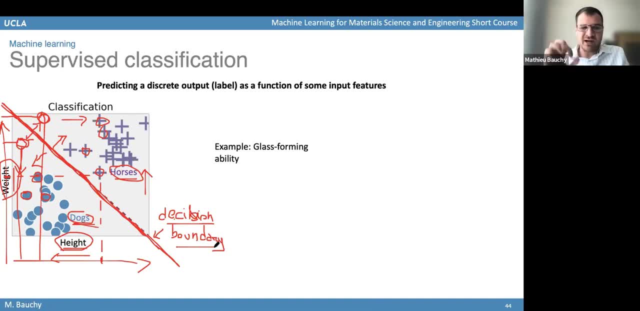 different classes of material. you will use the example that you have to determine with the machine learning algorithm what is the the decision boundary, and then, once you have this decision boundary, then every time you encounter a new material, then depending on which side of the decision boundary it is, then you can predict, uh, if this material belongs to category number one. 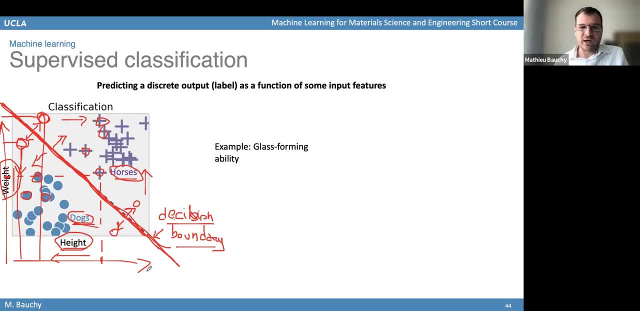 or to category number two. so that's an example where you take some, some example of data that you already have. you use this to train your machine learning model, and once your machine learning model is trained, then it gives you a set of rules that you can use in the future for new. 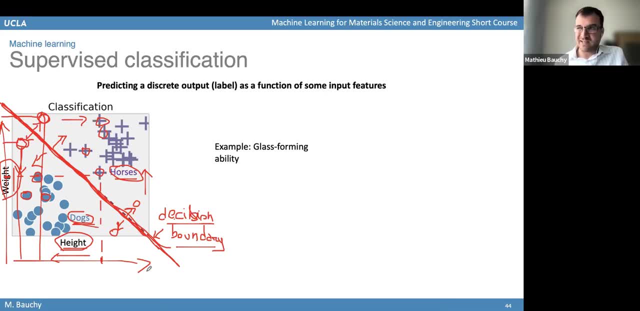 material that you have never seen before. your model will be able to predict which category this uh material belongs to. so one example of this would be, for example, the to predict the glass forming ability of various materials. so the glass forming ability tells you if you have a given material. 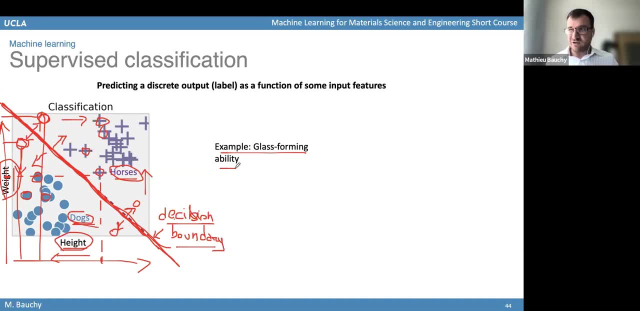 if you melt it and then if you quench it very fast, is it going to crystallize, form a crystal, or is it going to form a glass? does it mean is it going to to freeze without crystallizing and form like a frozen liquid, like a glass? so 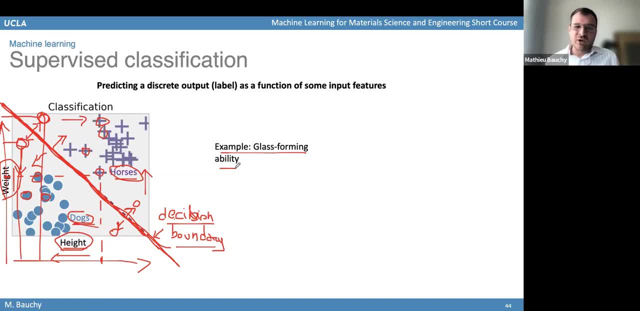 this. in this case, it would be an example of classification, because, uh, either a material will form a glass or it will crystallize, like so there's only like two possible categories. so that would. it's not in this case. you just want to predict: is it going to form a glass, or is it? 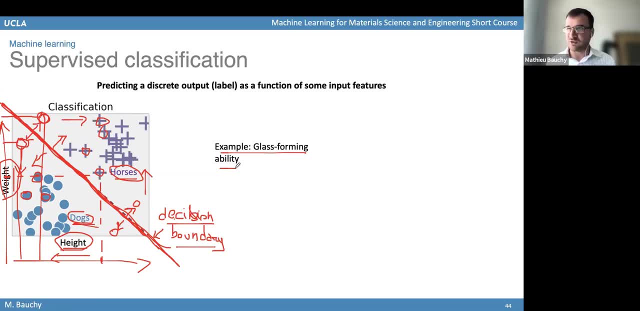 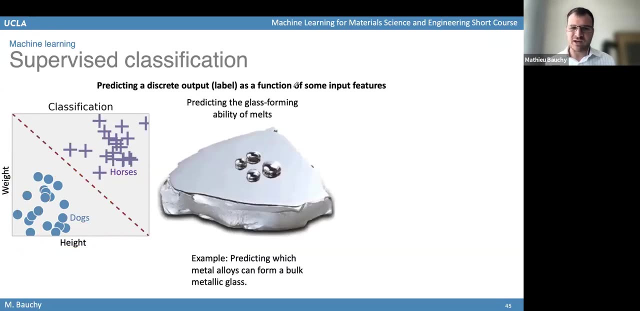 not going to form a glass. so that would be an example of classification. uh, because you are not trying to predict a number, you are trying to predict just between a forgiven material, which which class does it belong to. so an example of this, for example, is if you have um. 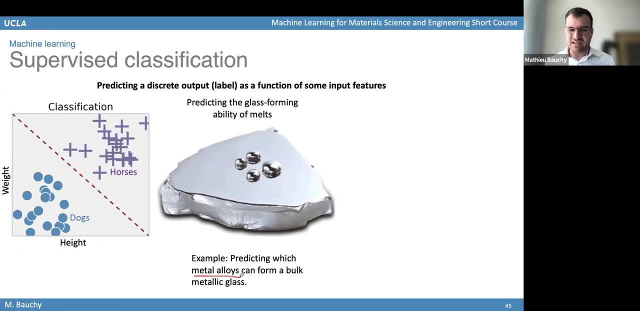 uh. if you are working with uh metallic alloys, you you can, for example, try to build a model where you will predict, based on the composition of this metallic alloy, based on the types of atom it contains, based on the concentration of those atoms, it will predict whether this metal 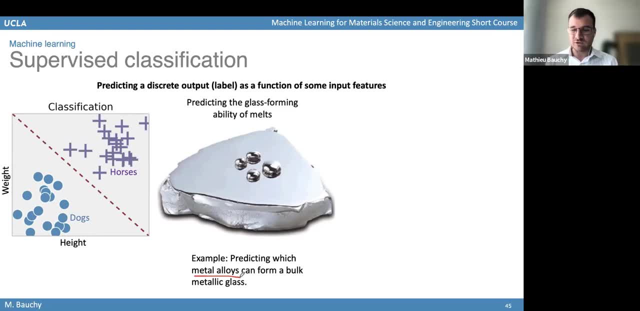 can form a glass. can it form a metallic glass or not? so in that case, that would be a supervised classification algorithm where you would use as many examples as you can of previous metallic alloys that can either form a glass or not, so you would have a data set that contains 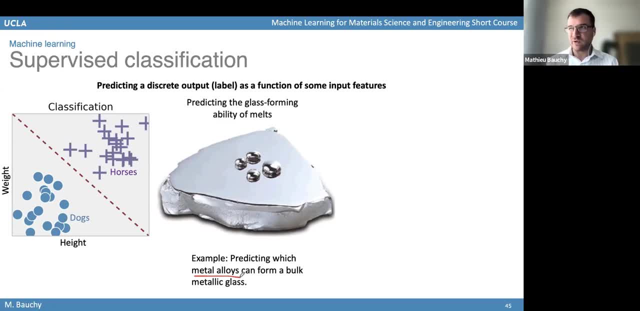 the metallic alloys with different composition, and you would also indicate in this asset either it can form a glass or it cannot form a glass, and then you would use those examples here to to come up with a machine learning model that can find the boundary between the alloys that can form a glass versus the alloy that cannot form a glass. 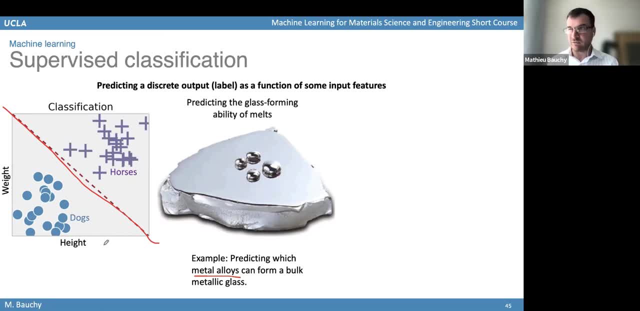 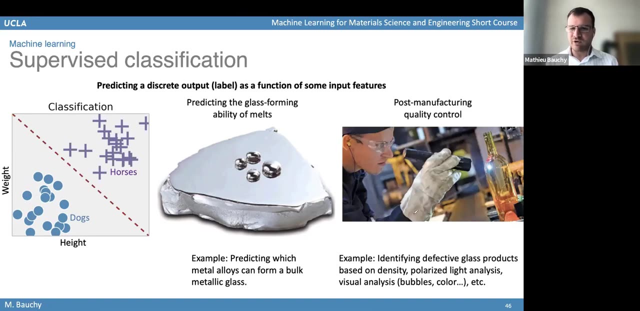 and then you, you will. you, once you have this model, then you can use this model for future metallic alloys that have different composition. you will be able to use that to predict if this alloy can form a glass or not. so that's an example of classification. another example is: uh would be um this uh types of quality control that we, that we talked about. 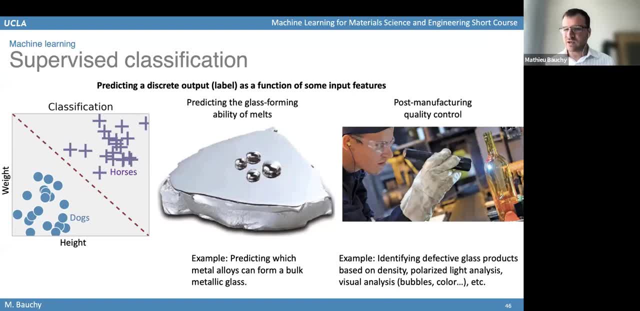 it's like, for example, if you, if you are building, if you have a factory, uh, to produce some, uh, some bottles, some glass bottles like this, then, uh, the question is how to recognize whether the glass has a defect or not. so in that case, that would be another example of 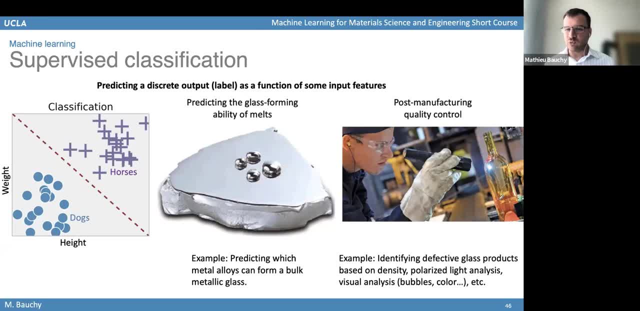 classification, supervised classification, where you would um, you would do uh, like you would consider for each bottle, like you would measure certain features of those bottles, like, for example, you can measure their weight or measure the density, you can do measure their transparency. you can look at what they look like on the picture, like: is there any specific? 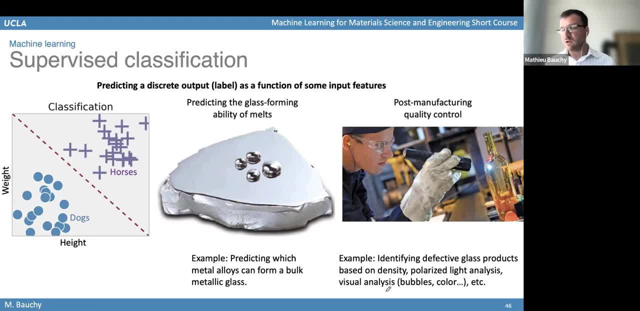 color or specific bubbles, so that that would be some features that you would measure about those bottles. and then, uh, what the the? you would also. you would also have some example of bottle that you know are defective and you would have measured all of those properties for the defective bottles. 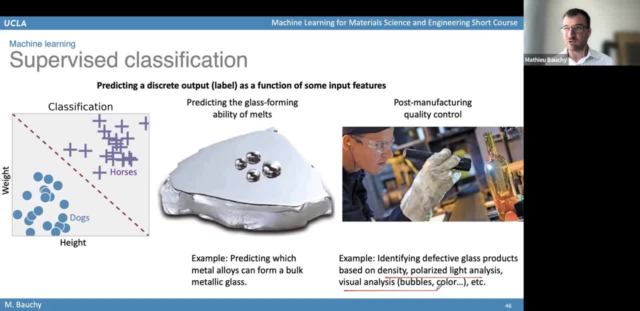 and you will also have some other uh example of bottles that you know are not defective and for which you would have measured all of those things, and then you will use that. you will provide all of those examples to your machine learning algorithm and the machine algorithm will um, will learn. 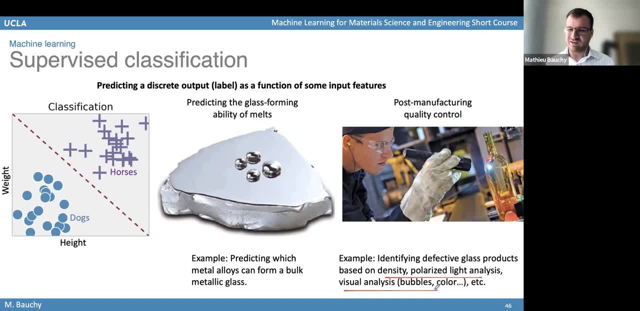 how to recognize a glass bottle that is defective versus a glass product that is not defective by by looking at all of those features, it will try to find the again, the boundary between the those features that differentiate a glass bottle that is defective from a glass bottle that is not defective. so that would be another example of 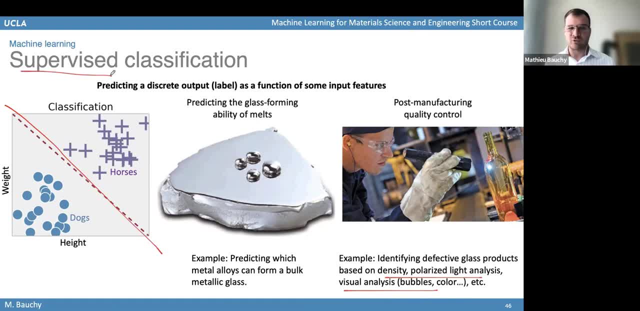 supervised classification. it is supervised because you provide some example of data where you already know what you want to predict. you already know for some example whether there's is defective or not, and it's a classification algorithm. because you don't- you only want to predict different categories. you don't want to predict a continuous number, because that would 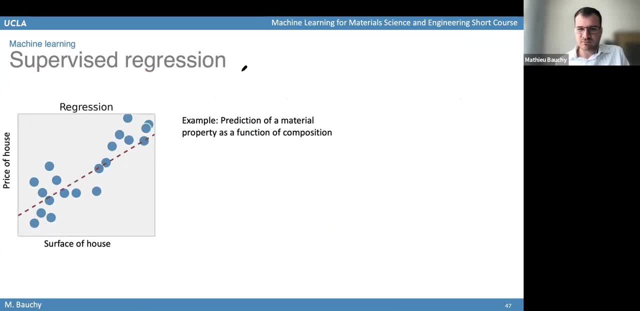 be an example of supervised classification, then the last example would be supervised regression. so it's still supervised. it means that you, you know already the the label for each data. so you know, for each material, you know something that has been measured about this material. that's what. 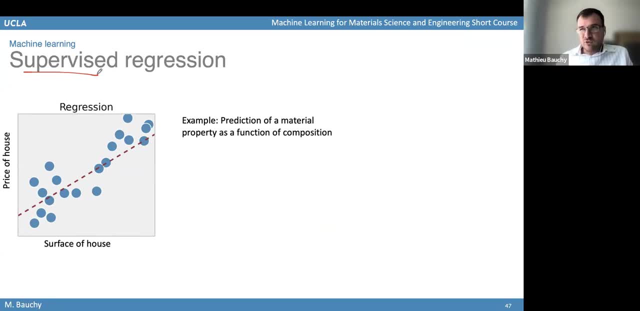 you want to predict, but in that case what you want to predict is not a class, you want to predict a number. so, for example, an example of supervised regression is if you want to predict the price of a house, and what you know about this house, for example, would be its size. you know the surface. 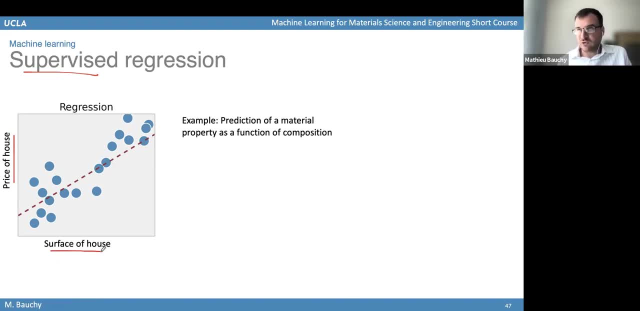 of this house. maybe you know some other things about this house. you know how many rooms it has, you know in which district it is located, if it's a good neighborhood or a bad neighborhood, you know if, if this, if this house like, how old this house is. so you know various features about. 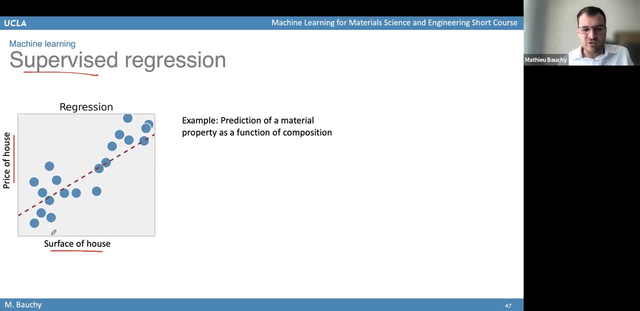 this house and in that case, what you want to use is to use those features that you know about this house and to build a model that can convert those features into something that you want to predict, which is the price of of this house, how expensive this price is. 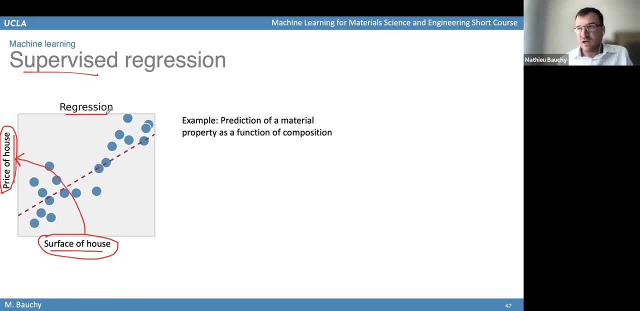 so in this case, that would be an example of regression uh problem, because what you want to predict is a continuous number, like you want to predict the, the price uh of this house, which is going to be a continuous number that can continuously change. so in that case that would: 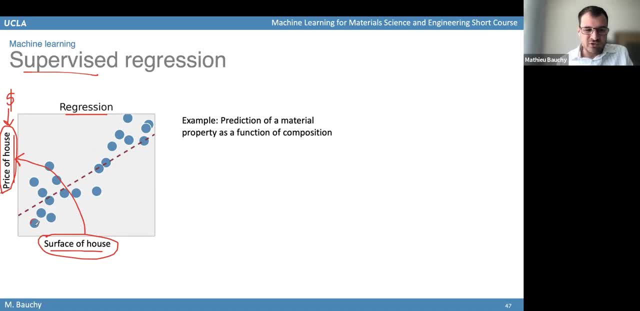 be an example of regression model where you would start with some example of how long it's going to be a continuous number and then you get a שלph and of course you can also just to convert a certain number and then convert it into a new one, so you can have. 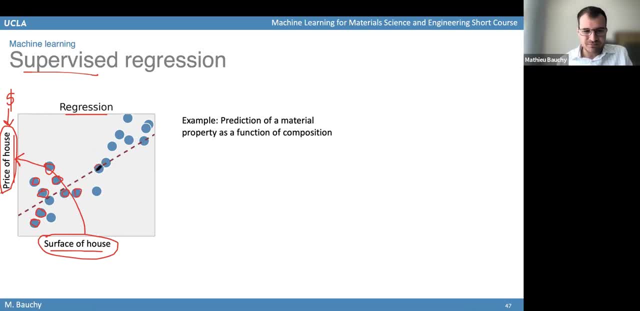 some kind of a unlucky number that can convert it into a new number or a new number, and that's what the machine learning algorithm is trying to do, and you know because the the machine learning algorithm can actuallylicitize the sources, for which you already know their price and you already 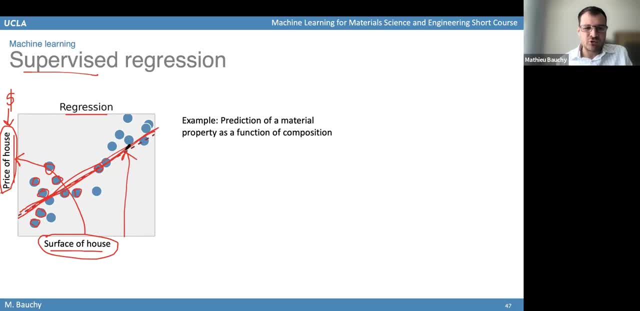 know their features, so you already know their surface in this case. but maybe you already know the surface into the price. so in this case the idea is that if you know the surface, which i can call x, that's the input- then once you have this, this model here, 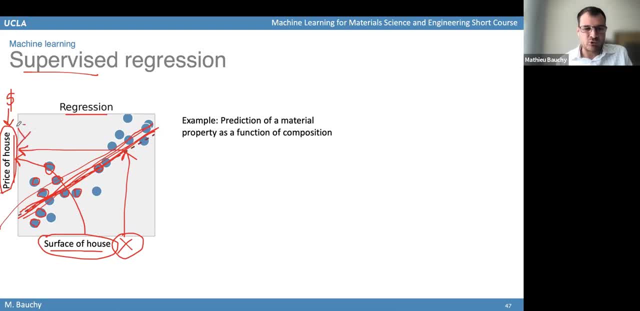 then you can use it to predict an output, an output y. so in the case of material, you can think about those inputs are going to be the composition of the material, or the temperature, or the pressure, etc. and based on that, the, the regression model will convert those inputs into an output which 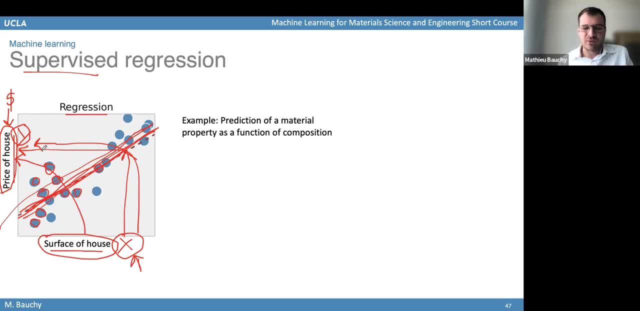 will be a property of this material, like, for example, density, modulus, etc. so in that case that would be some example of regression problem, because what you want to predict are not some classes, but you want to predict a continuous number, and it's going to be supervised, because 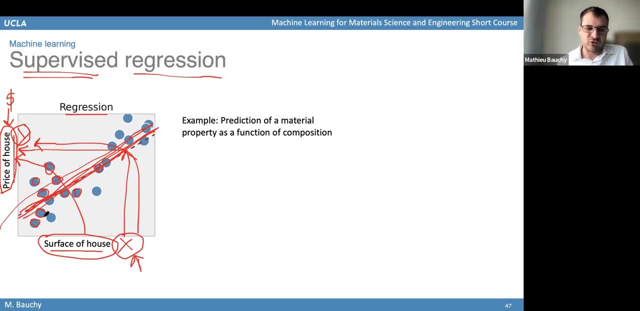 you are going to do that based on some example, like in this case. you have all of those examples of houses for which you already know their features and you already know their price. but it's going to be the same for materials. if you have already other sets of materials for which you 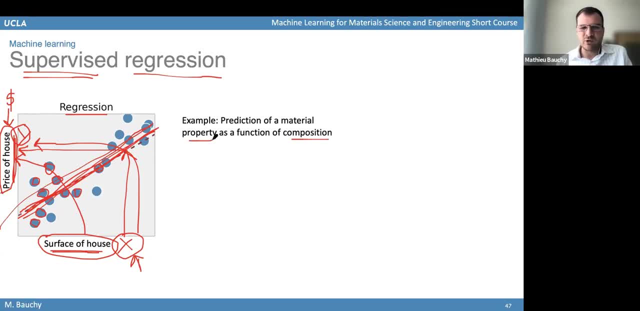 already know, for example, their composition, and you already know their priority, then in that case those data are already labeled, and so you can use that for a supervised regression. you already have some example of materials for which you already know the property that you want to predict, and 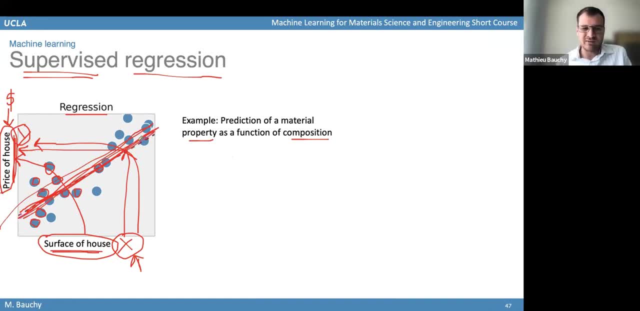 then in that case the machine learning model will try to find what is the best relationship, the best function that can be used to map the input into the output, to transform the input and to use this to predict the output. so it will try to find, for example, a mathematical 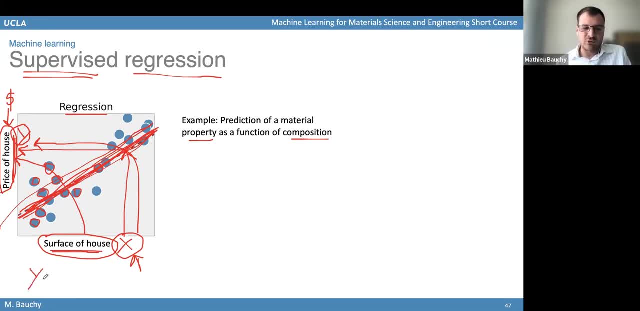 function that can be used to predict the output. so it's going to be. it will try to find a function where the variable of the function are going to be the input, x, and this function will transform into x, into y, so it will transform the input into the output. it will transform the, the composition. 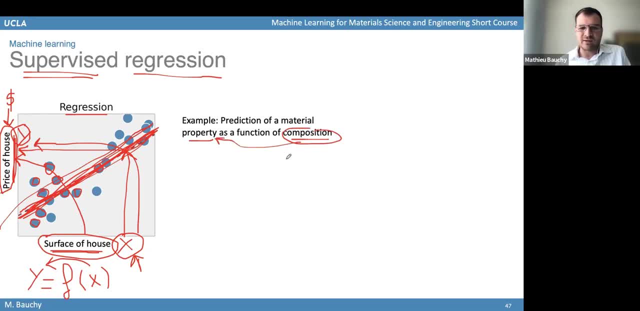 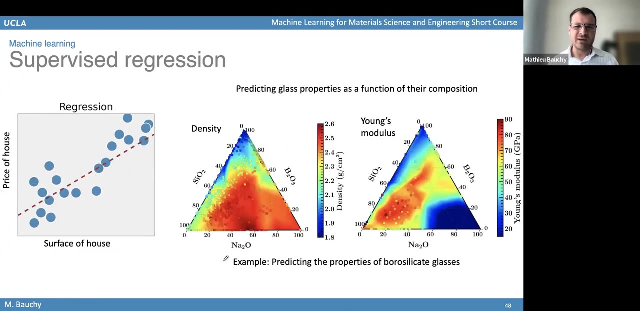 for all of the material into uh the priority. so composition would be the input x and the priority would be the output y. this is what you want to predict for this material. so that would be an example of regression problem in this case. so some example here would be the sample, if you. 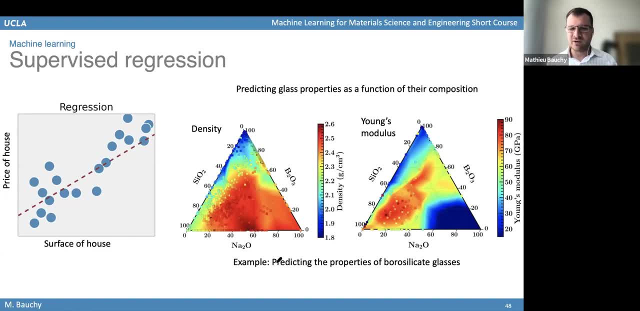 have some, some glasses or another types of material, and you would get aKS or you will see these in the. you want to predict how certain properties of these materials will depend on their composition. So in this case, those are two examples here of glasses, for which 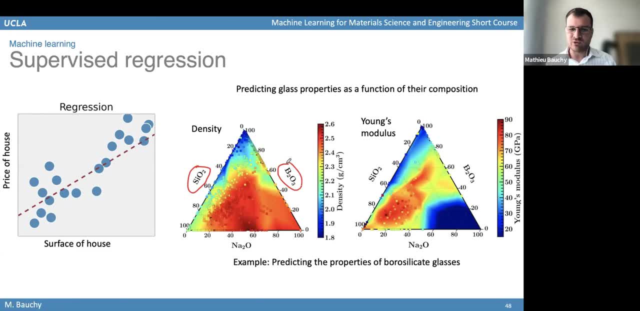 based on how much SiO2 or based on how much B2O3 or how much Na2O, like, based on the oxide, based on the concentration of the oxides that they contain, then the glass will have a different density of different Young's modulus. So in this case that would be a supervised regression problem. 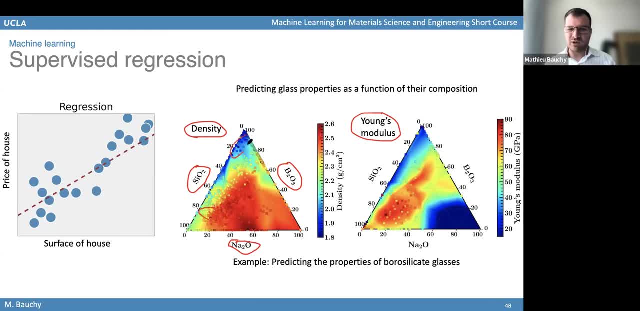 where you would start with some example here, like you have some example of different glasses for which you know their composition and you know their density or their Young's modulus, and so you will use those examples to train a supervised regression machine learning model, where now the model will be able to predict. 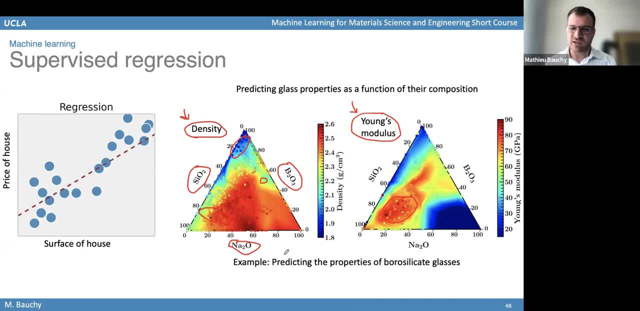 for any glass composition, even a composition that you have never seen before, the model will, would be able to predict what would be the density or the Young's modulus of those glasses, even if those are glasses that the model has never seen before. So that would be an example, in this case, of supervised regression, where its supervised 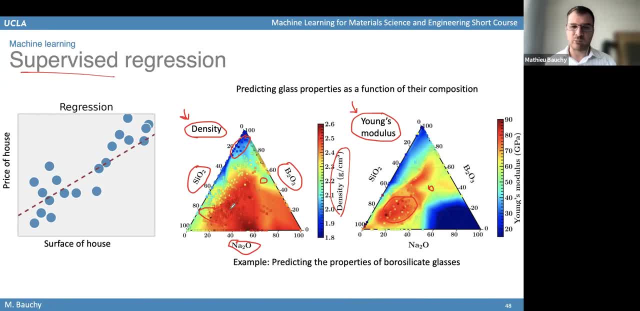 because you train your model by providing some example of previous glasses with where you know both the density of that glass, or you train data on them and providing these examples of the glasses where you know both their density of the glasses as well in terms of what you use. 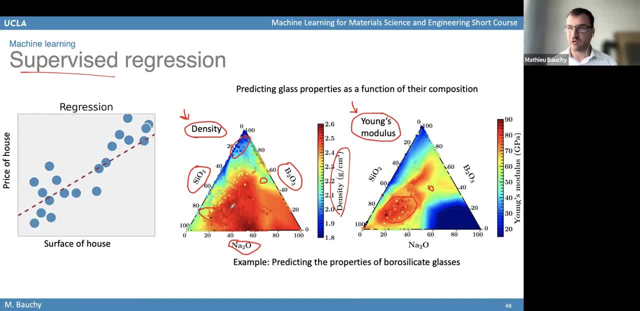 both the composition, the density or the modus, or whatever you want to predict about those glasses. And it's a regression problem because you are trying to predict a continuous number. You're trying to predict the density, which is not simply a category. 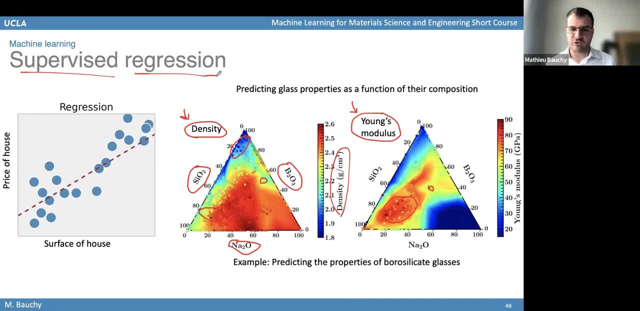 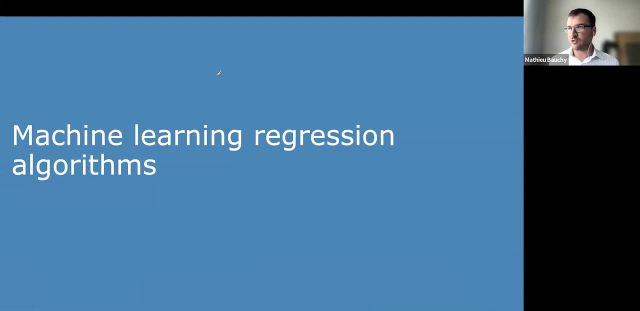 it's a number that can continuously change within a certain domain, So that would be an example of regression rather than a classification problem. Okay, do you have any questions regarding those differences between supervised versus unsupervised or between regression and classification? No, all is okay, thank you. 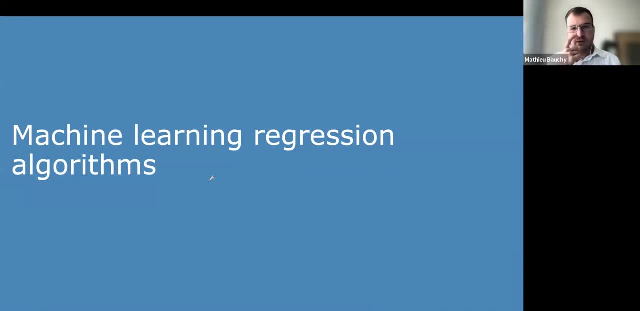 Thank you. Okay, so now we are going to focus more on regression algorithm. So regression is something that is typically very common in materials, because many commonly in materials you want to predict some kind of properties, So you want to predict the performance of those materials. 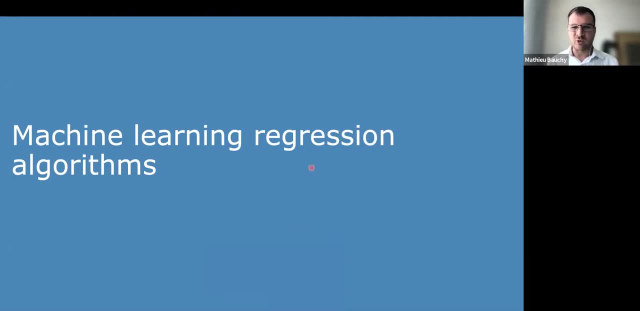 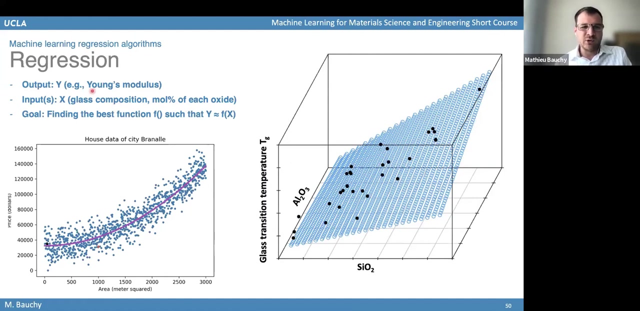 So in this case, that would be a regression problem, where you want to predict a property for this material, a performance metric that can continuously change. So in this case, in the case- so let's take an example where, for example, you want to, you have a list of materials. 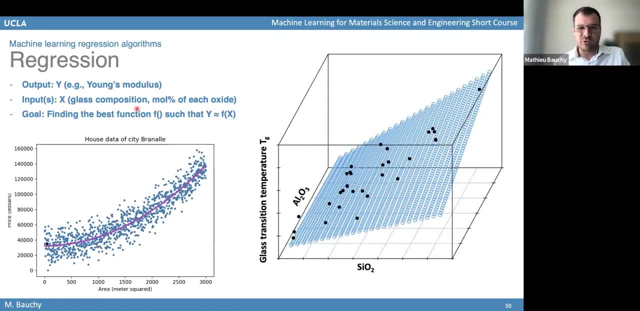 for which you know some features. So you know the composition, you know the temperature that was used to make these materials, you know the pressure, et cetera. So those are going to be the inputs. So that's what I call a capital X here. 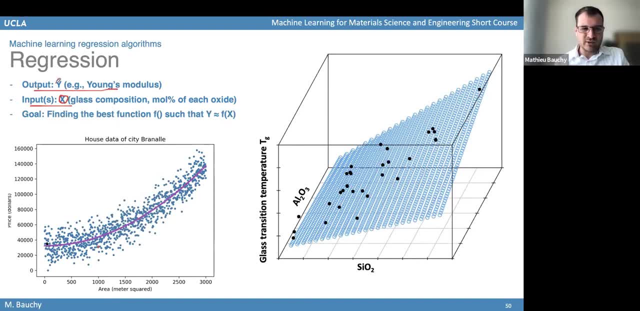 Those are the inputs, And then you have the output. So the output is what you want to predict, So for example the Young's modulus, some other properties of those materials. And so here the goal of a regression problem is to find: 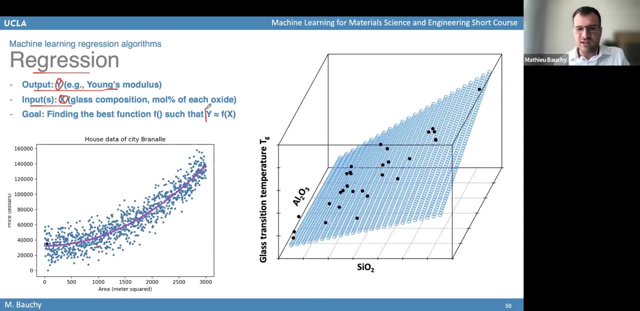 what is the best function that can transform the input into the output. So if you have, if you know, the input X, you want to find what is the best function F that will transform the input X into the output X. So you will try to define this function. 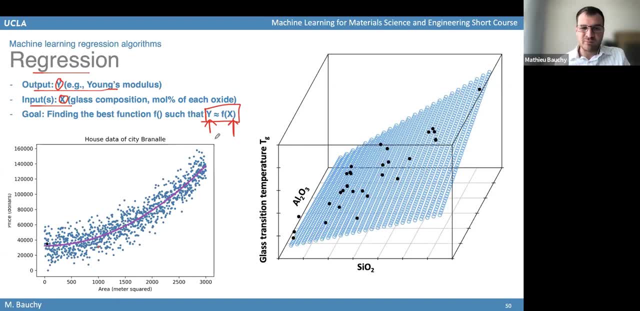 by looking at some example. If you have some previous example of materials for which you already know X, you already know the composition and you already know the Young's modulus Y, then you will try to learn, based on those example, what is the best function F. 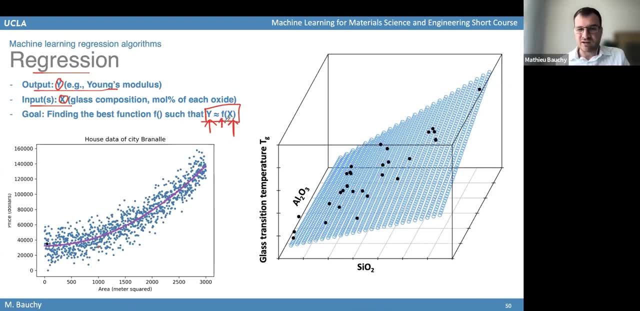 And once you have this function F, then you can use it for new materials that have new composition that you have never seen before. You can use it to predict what would be, for example, the Young's modulus. So, like an example for this, like would be like. 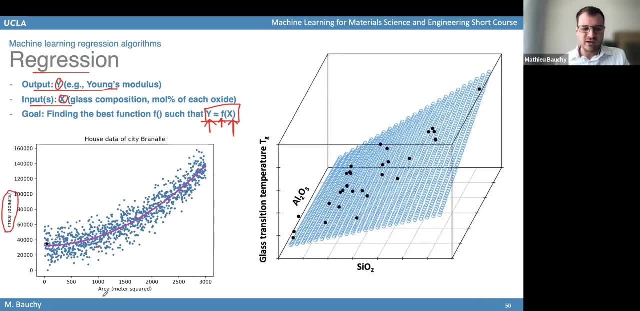 so what we just discussed- if we start with a simple example- is: you have a list of houses and for each of those house, you know they are area. So you have a list of houses and for each of those house you know they are area. 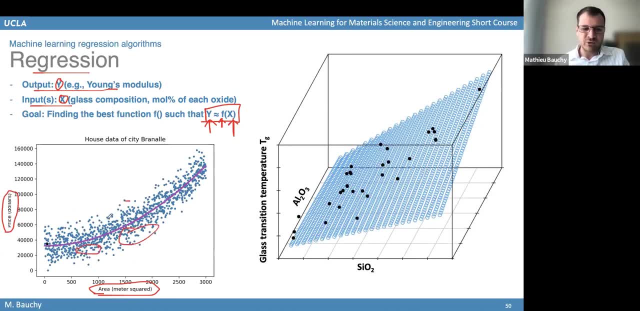 So you have a lot of example here of different houses and you know their corresponding price. So, and then you will use those data to try to come up with the best function, For example, in this case, like a quadratic function, like this: 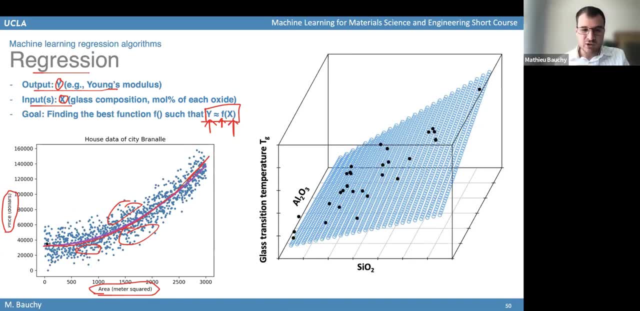 look like it could be the best function to transform the area of a house into its price. And once you have this, then you can say: now I have a new house here. It has a given surface. It has a given surface of, let's say, 2,700 square meter. 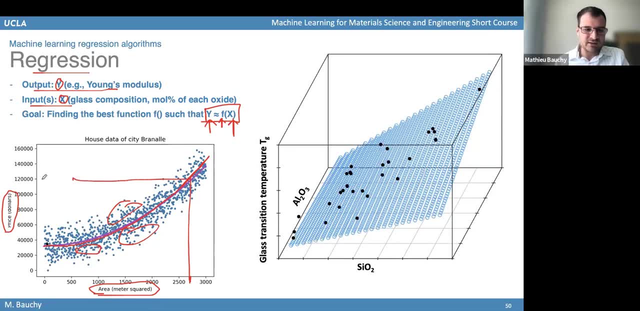 And then, based on that, you can say: I predict its price to be like $120,000 in this case. So in this case, that would be an example where you take those data, you know both their input and the output. 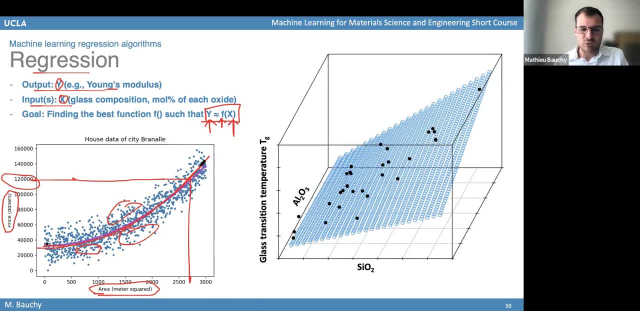 Based on this, you learn the relationship between input and output. You learn that this is gonna be a quadratic relationship And once you have this relationship then you can use it for every input. X- You can predict where it is gonna be the output- Y. 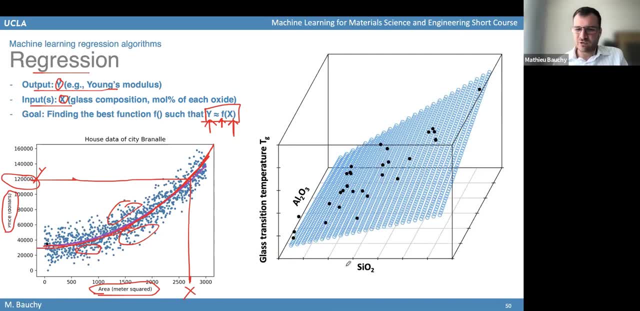 So in the case of material, let's take another example. So now let us assume that you have a glass for which you know how much silica, how much SiO2 this glass contain. You also know how much alumina, how much Al2O3 this glass contains. 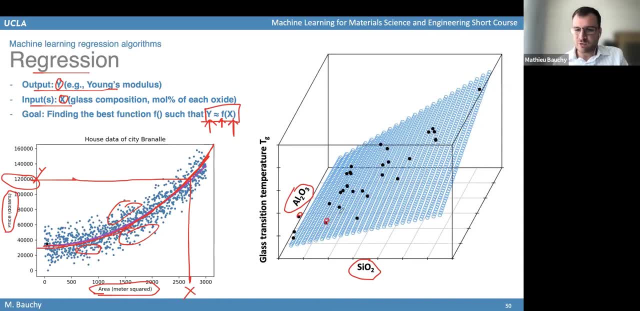 And so you have various example here of data points for which you know already how much SiO2 this glass contains, And so you have various examples here of data points for which you know already how much SiO2 this glass contains, And so you have various example here of data points for which you know already 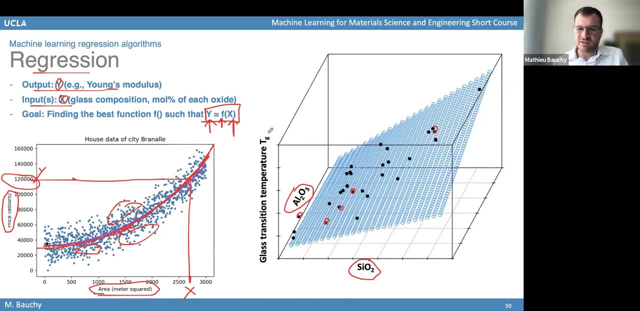 how much Al2O3 this glass contains And you know a property, for example, you know the glass transition temperature of this glass. So that would be, in this case, the third axis here. So you have two axis here and here. 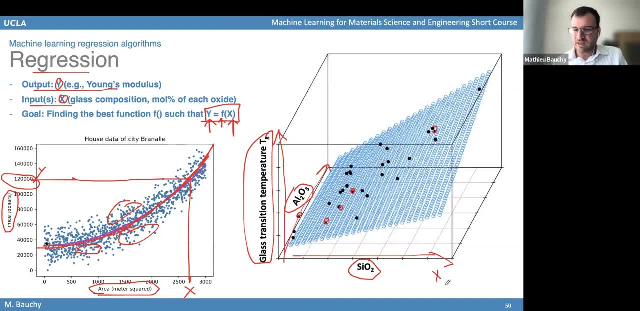 Those are some inputs, So that's gonna be input X1,, for example, Input X2, that's about how much silica or how much alumina they contain, And then you wanna predict the temperature at which the glass is going to melt. 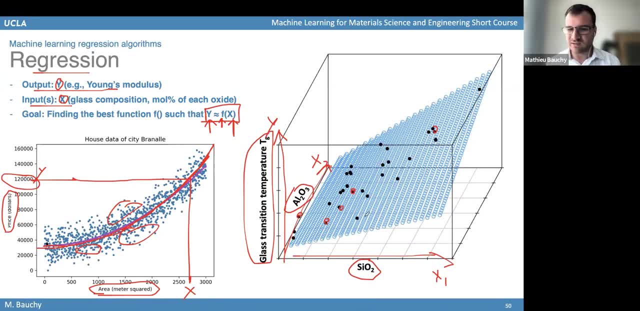 So the glass transition temperature. So what you do in this case is that you start with those example of data points, Then, based on that, you try to come up with the what is going to be the best function that can convert the input into the output. 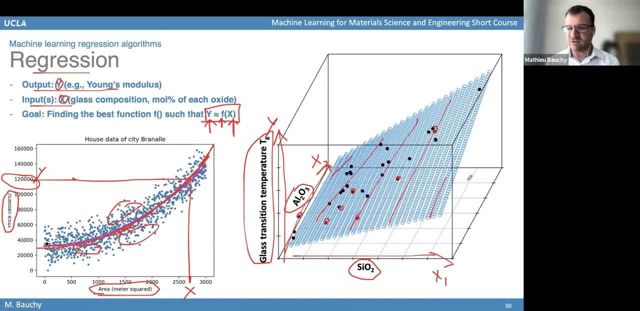 And then once you have a new glass- for example, you have a new glass here for which you know how much alumina it contains, how much silica it contains, And based on that, once you have the function, you can say that I predict. 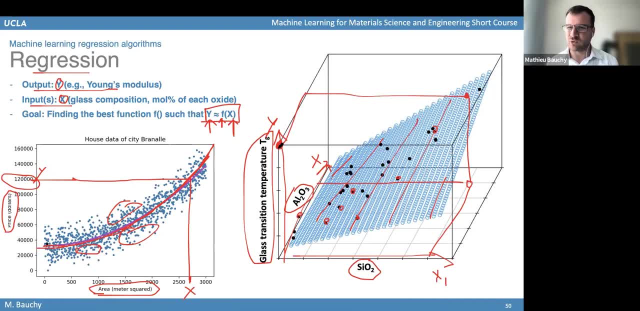 that this glass transition temperature will be equal to this number. So once you have this model that can map the input to the output, then you will be able to make some prediction for new materials that you have never tested before. You can predict what its property is going to be based on that. 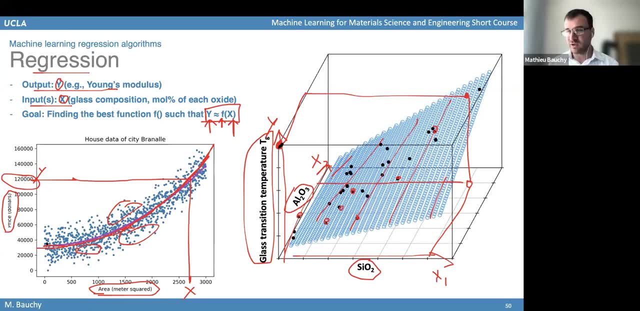 So that's the main idea of the regression model And that's very useful because if your goal, for example, is to find the glass that has the highest glass transition temperature, or maybe find the glass that has the lowest glass transition temperature, then once you have this model, 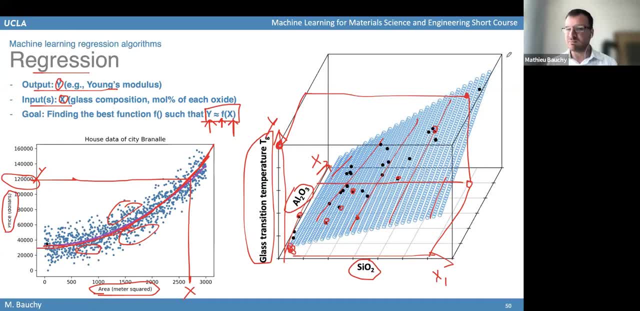 it's very quick to see where it's going to be minimum or where it's going to be maximum. So once you have this class of model, then you can use it to very quickly explore the design, the composition space that you have, explore the different composition that you can use. 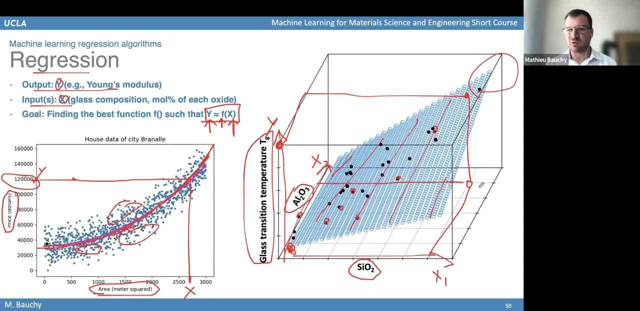 And, based on that, quickly pinpoint what is going to be the best condition, what is going to be the best composition for your glass, in order to achieve whatever you want to achieve. So now the next question is: the goal here for regression problem is: 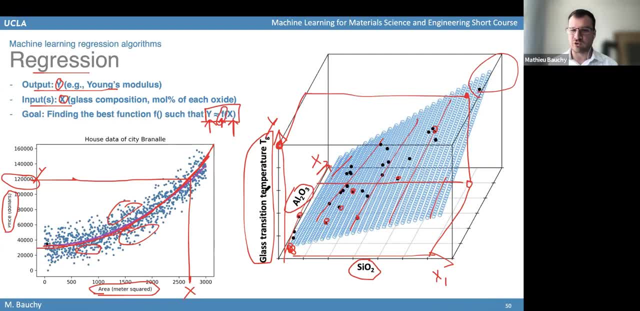 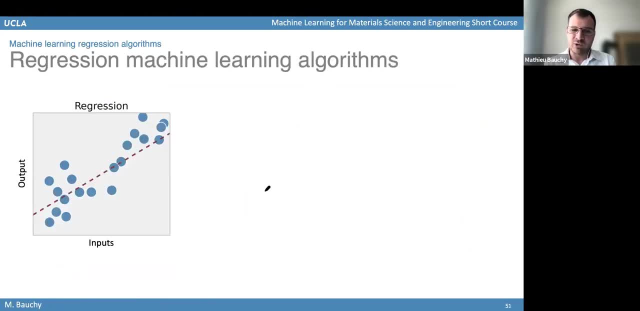 how to find the best function, how to find the best function that can be used to transform some inputs into the output. So, to find the best function that can be used to transform some inputs into the output情況 function, there is several algorithms that are available. so the question now is which algorithm? 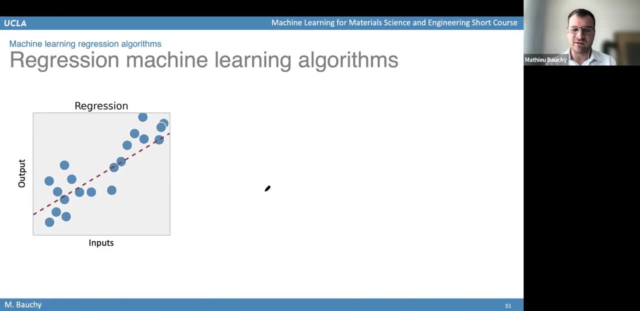 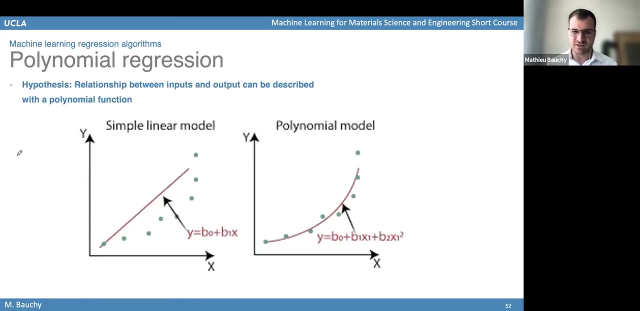 to use what are the different families of algorithm that you can use to find the best relationship between some input x and some output y? so for this you have various options, and we're going to briefly review what are the the possible options that you can use for this. 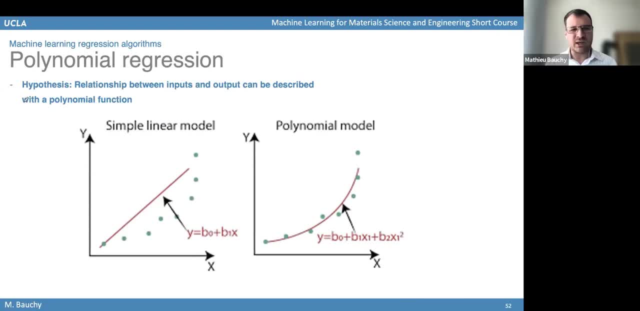 so a first option would be something that probably you have all done, which is polynomial regression. so in this case, the idea of polynomial regression is that you have some data for which you already know some inputs- x- and you want to predict some output- y. so, again, like the x could be maybe the 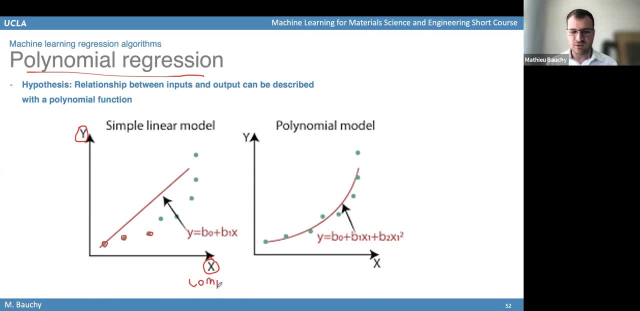 the composition of the material or something else, the temperature, and then you can have y, which is going to be a property that you want to predict. so then, in that case, uh, the, the, what you will do is first start with some data points of materials for which you know. 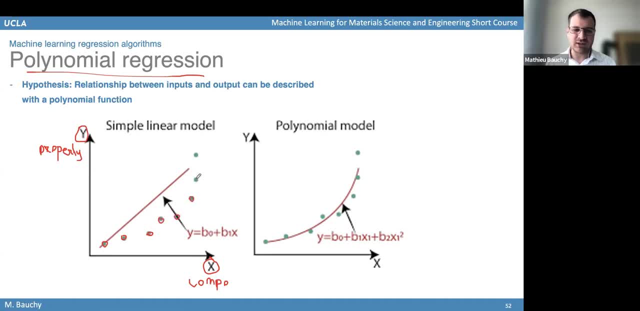 at the same time the composition x and the property y, and then, once you have those data points, your goal is to find what is the best function that i can use in order to transform the composition into a priority, and so, for one example here is that you can say: i'm going to 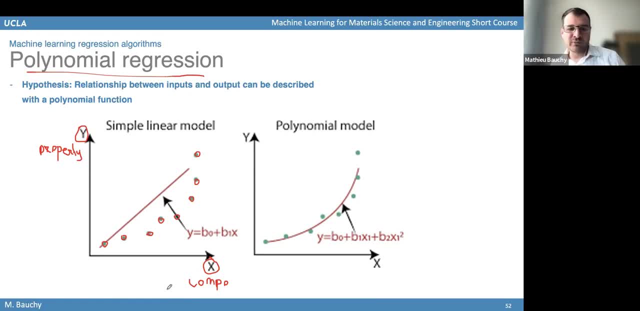 use polynomial regression, so i'm going to assume that the relationship between the input and the output is a polynomial. so for example, you can say: first i'm going to try a linear regression, so i'm going to try to fit those data by a linear function like this, so something that would look: 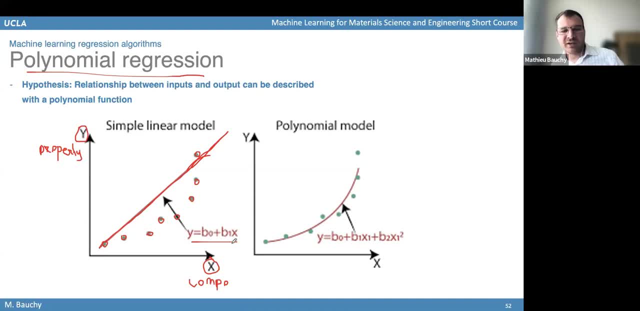 like that, like a linear function of x. but here, if you do that, you're going to see that you calculate for all. Okay, find that you cannot really describe the data by a linear function. A linear function is not really fitting very well the data. It's not interpolating the data very well. So in that case, in the case, 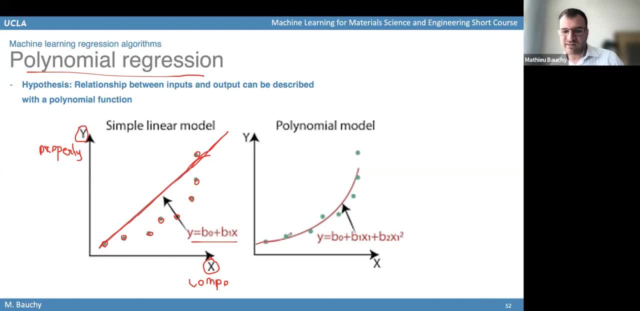 of those data. for example, you can describe the data much better by fitting those data with a quadratic function, something that depends also not simply on x, but also of the square of x. So in that case, using a polynomial of degree 2 would be a better choice to describe. 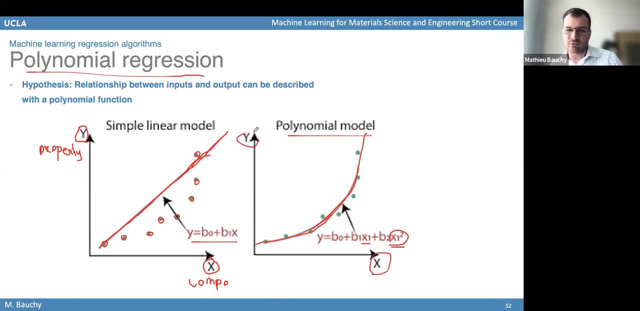 the relationship between the input and the output. So in this case, this is what you can do with polynomial regression. You have some inputs. You will assume that the output can be expressed as a polynomial function of the input with a given degree, Like, for example, if you use a degree 1, that's going to be a linear model. 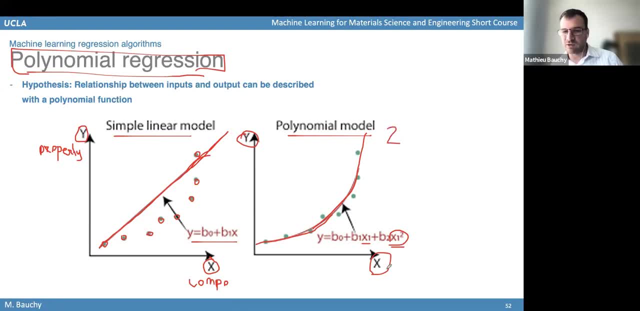 And if you use a degree 1, that's going to be a linear model. And if you use a degree 1, that's going to be a linear model. If you use a degree 2, then that's going to be a quadratic model. You could also say: 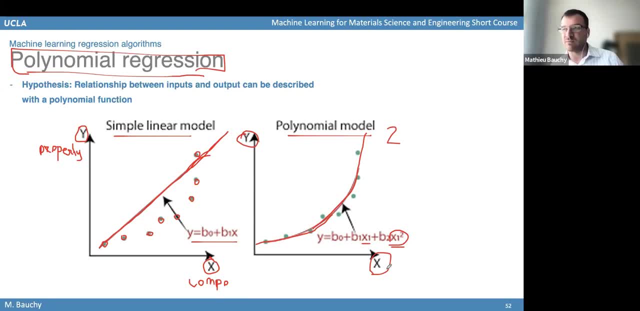 I'm going to use a degree 3.. So that's going to be now a cubic model, et cetera. So you can assume a given degree for your polynomial And then, based on that, you will find what is the best polynomial that can fit the data. So the polynomial function that can 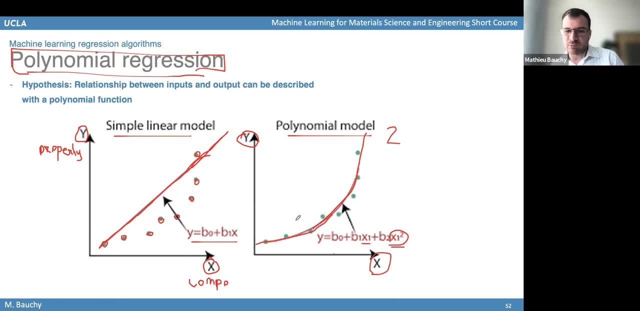 best represent the relationship between the input and the output. And again, like once you have this polynomial and once you have found that it describes well the relationship between input and output, that means that if you have a new material that has never been tested, with a new input x, then you can use that and predict what would be. 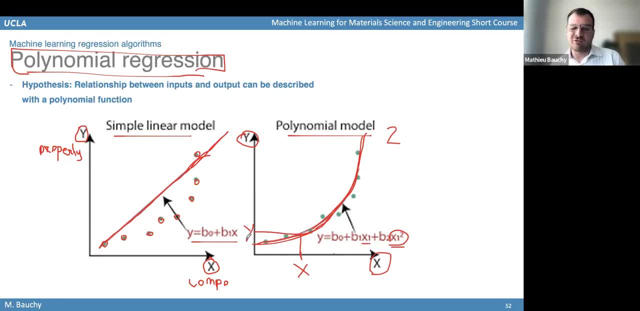 the corresponding output. So you can make some prediction for material that you have never seen before: to predict what would be their priority, based on their composition, based on the polynomial model that you have been fitting. So that's the polynomial function that you can use to predict. 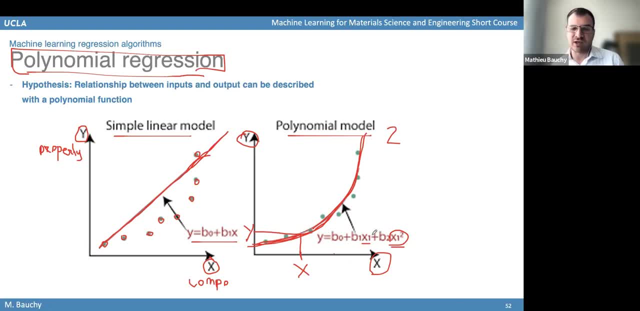 Based on the data that you already have. So that would be an example here of a regression, a supervised regression model, because you want to predict a property that can continuously change. the priority y can continuously change, And you want to. for this you will need some. 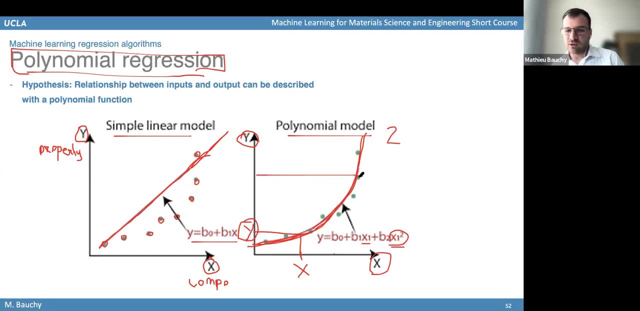 example of previous data for which you already know both the input and the output. So those are in this case. this is a. this is a, a supervised approach, because you have already the input and the output. You have some example of of data for which you already have the label. you already have the output. 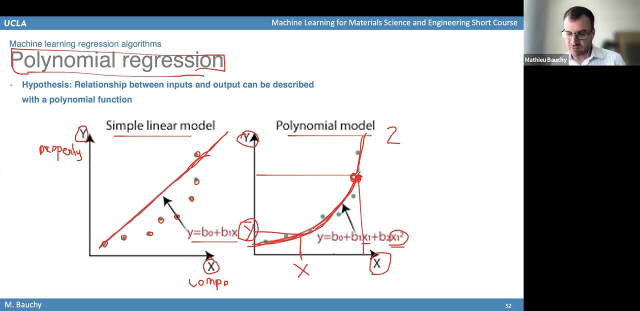 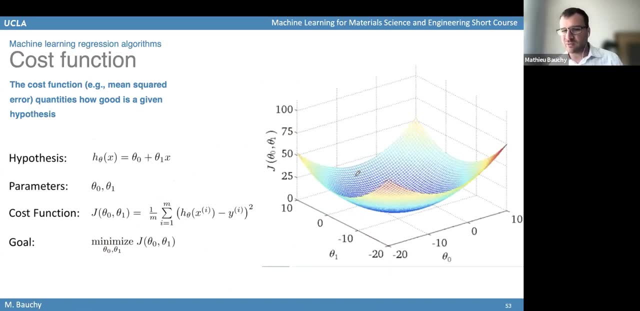 and you will use that to train your polynomial regression model. So then the question is: how do we do that? So if you have some data, so let's assume that you have, for example, some data here for which you know the input x, and you have some output y that you want to predict, and you have some 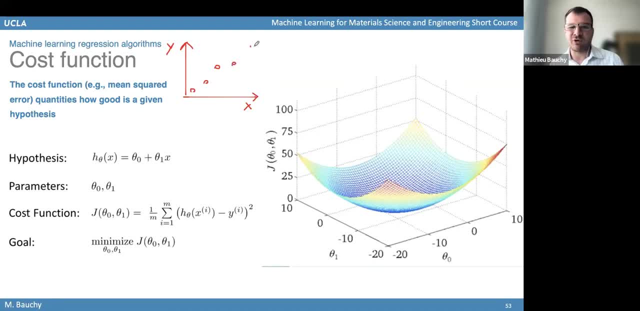 example of measurement that you have been doing for different materials with different composition- x, for which you already know the output, y- Then the question is, if you, if you think that those data can be described by a linear relationship, is: how do you find the best linear relationship? 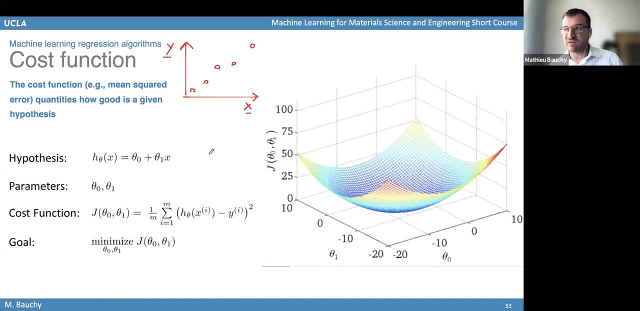 So in this case it's. it's very simple, Like you can just do a linear fit of the data, but in some cases, if your model is more complicated than a linear relationship, then it becomes more. it becomes harder to find how. what is the best relationship? 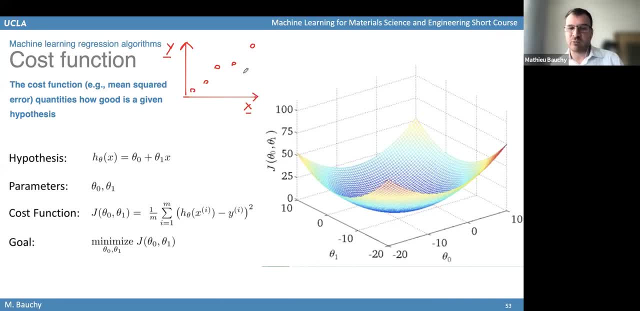 What is the best function that is going to transform the input x into the output y? What is the best function here, For example, if, if you are just assuming that it's going to be a linear fit of the data, then you can just do a linear fit of the data. 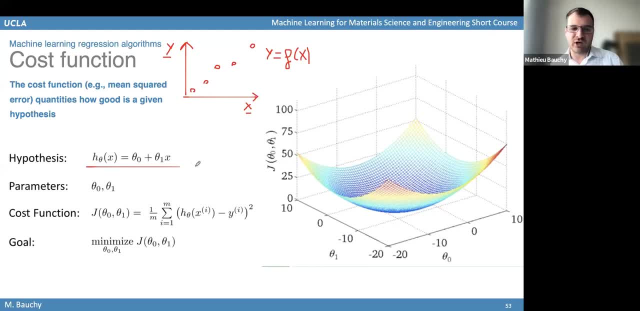 Assuming that it's going to be a linear model. So let's assume that your hypothesis is this one. You hypothesize that your, your function, your, your output, y, can be described as a function that is a linear function of x. So in this case, you assume that it's a linear function, So it's a. 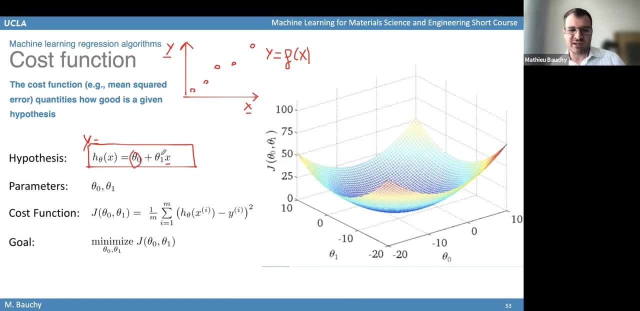 linear function of x and you have two parameters. So you have the intercept and you have the slope of this function. And the question here is: how do you find the optimal value for those two parameters, for theta one and theta zero, for the intercept and for the slope that will best describe the relationship between the input? 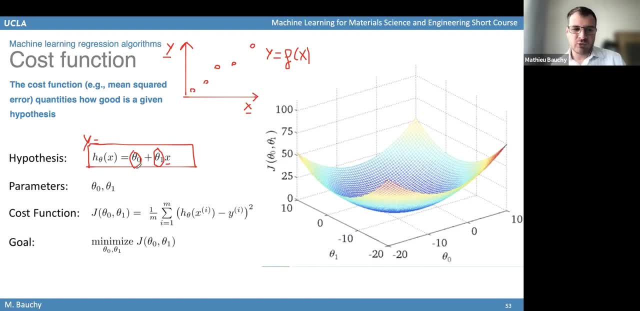 and the output. So, for example, if you don't know what is the best choice for the slope- theta one- and the intercept, theta zero, then you can say: well, I'm going to start with that. That's, that's my initial assumption that this, this, function. here, where 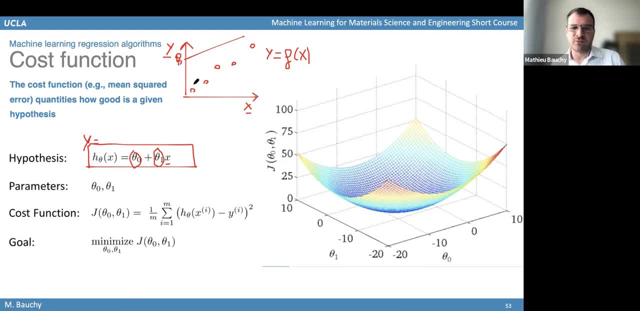 here this is theta, not, that's the intercept, That's the value of the function when x equals zero. And then you have the slope. here the slope would be, uh, theta one, That's the, the slope or the derivative number. So here, if you take those value of theta one and theta not, 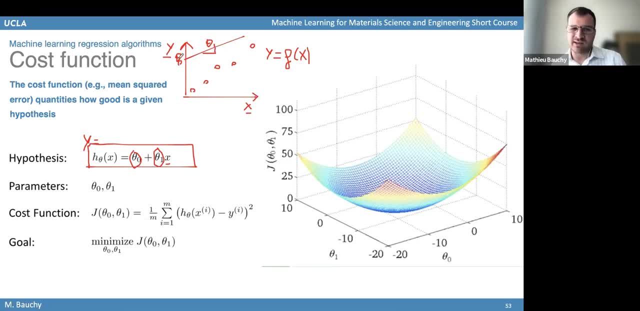 then those parameters here. they are not the correct one. Like theta not is too high, Like we would need. the right function that we would need is is this: we would need to decrease theta not, And we would need to decrease theta not, And we would need to decrease theta not And we would. 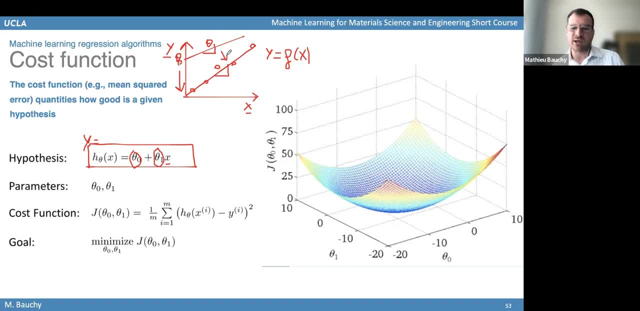 need to also increase theta one to increase the slope here. So the question is: how do you find the best parameter? And that's always going to be the case in uh, in in uh regression machine learning problem is that you have some parameters that uh describe the relationship between the 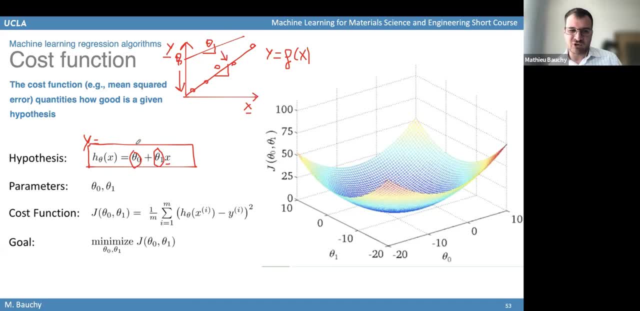 input and the output. So in the case of linear regression, the parameter are just the intercept and the slope. But if you have a more complicated uh model, that is uh quadratic or cubic, then you will have more parameters. Or if you are using 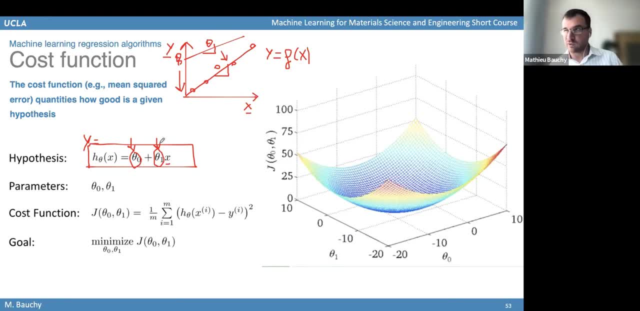 an even more complicated model like an artificial neural network, like we are going to talk in a in a few minutes. then you you can have hundreds of parameters and you need to find what is the best value for those parameters, And usually you don't know what is the value for those parameters. 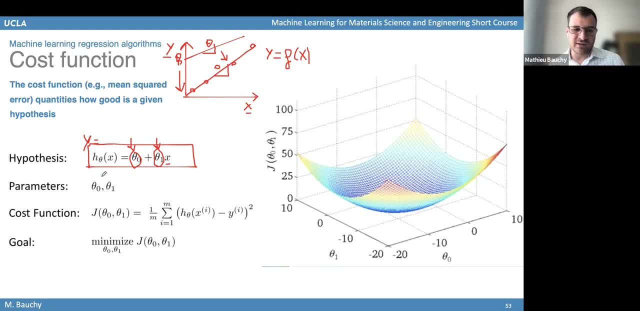 but you need to optimize them. So the goal in this case is: you have some parameters here. It's only two, but in general you will have, Uh, potentially hundreds of parameters and you want to find what is the best value for those parameters. that will give you, like, a good description of the relationship between input. 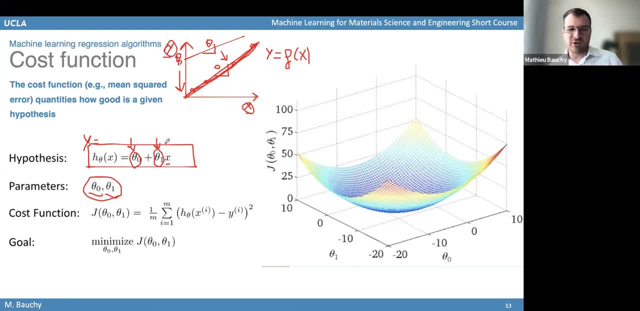 and output. So the way that we are always going to do this is to define a cost function. So the cost function is a function, and this function depends on the parameter. So, uh, this function is a function that will determine how, uh that the input is going to be used for each parameter. 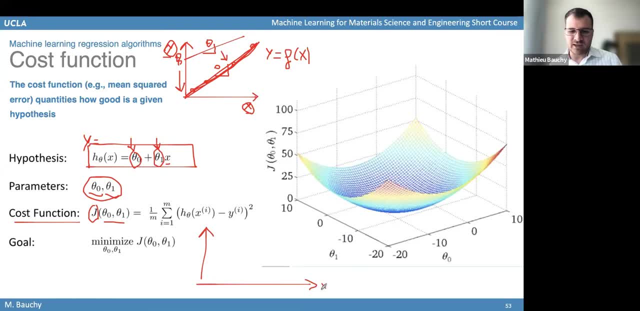 How good is your model? So, for example, if you have um, uh, some data points here, so you know the input X, you want to predict the output Y. you have some, um, some example of data points. 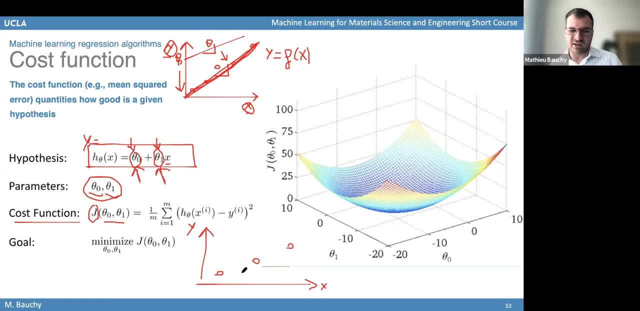 Then you are going to start by making an assumption, making a hypothesis of what you think are good values for theta one and theta zero, like for the parameters. So that's even that you start good initial guess. so to check how good this guess here is, we are going to define the cost function. 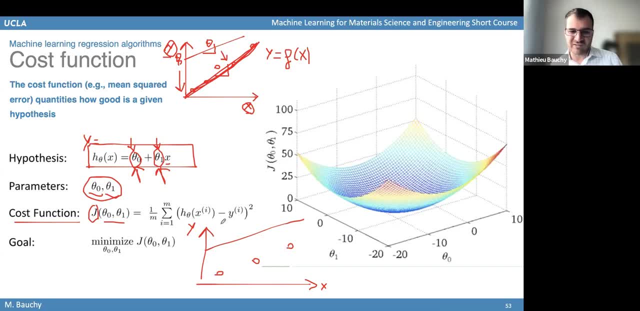 the to define the cost function. what you are going to do is to measure the distance between the actual data points that you have and your model. so in this case, for example, you are going to measure for each data point i that you have. so this would be: i equal one. uh, i equal two. 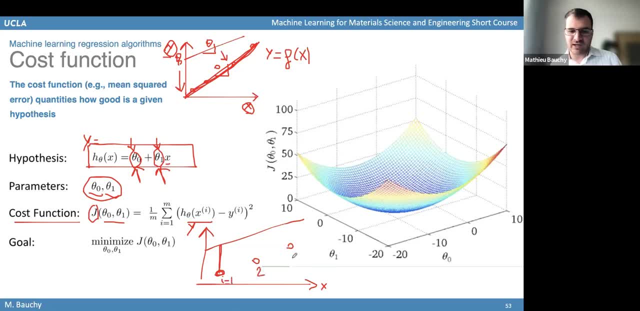 so that would be the, the different data points that you have. so for each other point, you will measure the difference between the true data point that you have. so that would be uh, why this is the true data point that you already know- and the you measure the how different it is from the. 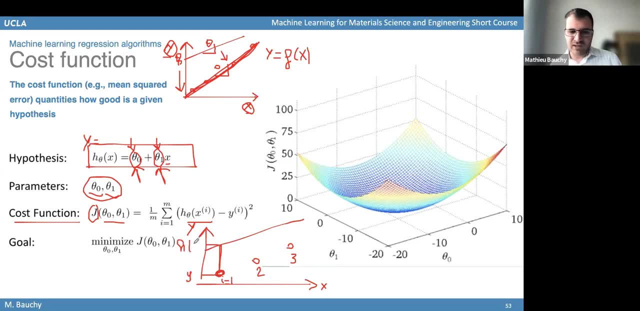 prediction of your model, where your model would be this: um h, h of x. so uh, h of x is this is: uh. this is what your model predict. like for given x, here your model predict uh, h of x. so what you do is that you measure the difference here. 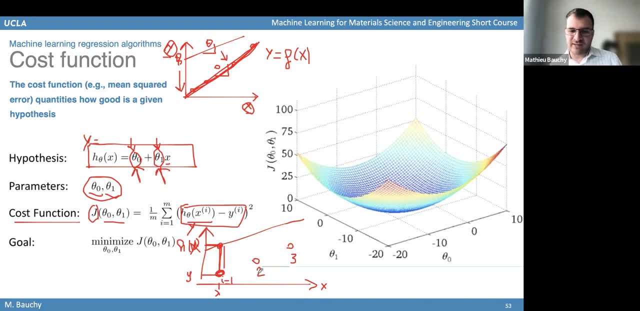 between the, the prediction from your model, and the actual data points, and you will measure this for all the data points. so you will get all the differences here between your model and the, the actual data points. then you you put everything to the square so that it doesn't matter if the 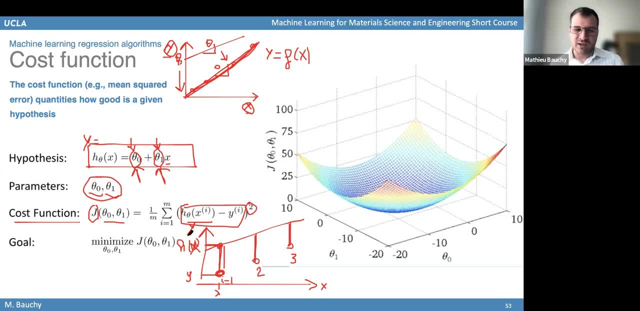 you are making a positive or negative error, and then you take the sum over all the data points and, if you want, you can divide by the number of data points, although it doesn't really matter- and so this will give you a cost function. this cost function is a number and the smaller this 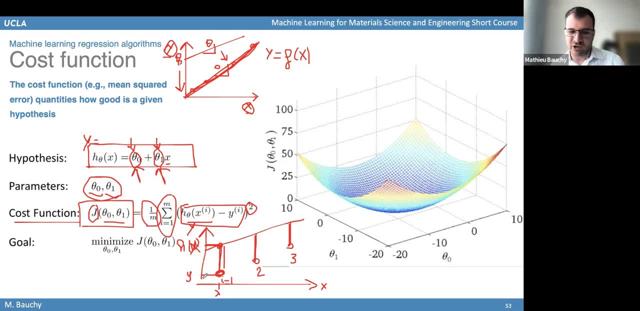 number here is, the better is your model, for example, if your model was like this, then the difference between your model and, yeah, the data points would be very small, so that would be a very small uh j for this, for this choice of theta one and theta not. 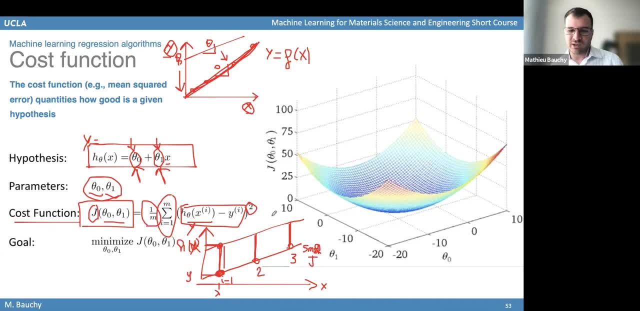 you would have a very small uh cost function. but if you use the wrong uh theta naught and the wrong uh theta one, then you will have a very large cost function j. so uh this, this cost function j here, by calculating the difference between the prediction from your model. 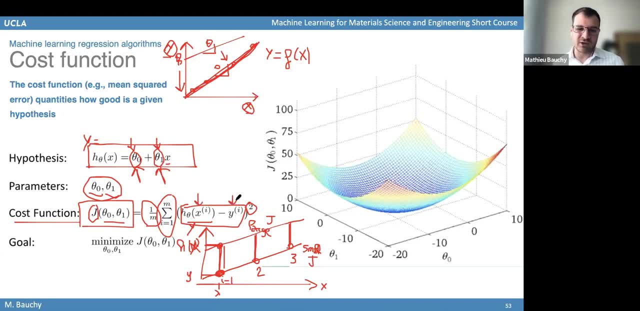 and the actual data points. it's telling you how good your model is. it's telling you for those parameters- theta naught and theta one- it's telling you how good those guests are, and so your goal here will be to find what are the best value for theta 1 and theta naught. 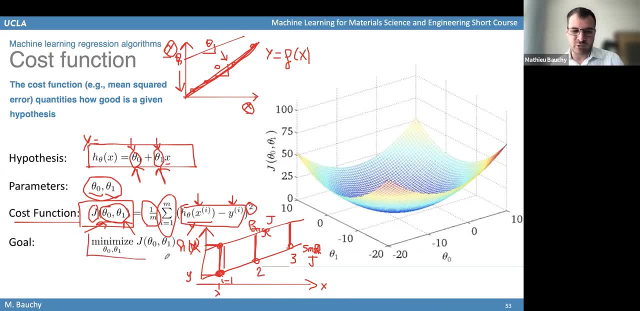 that will minimize this cost function. so you can summarize this like this: you want to find the parameters for your model, theta 1 and theta naught that will minimize the the cost function. You want to minimize the cost function as much as possible. So this can be represented like this: 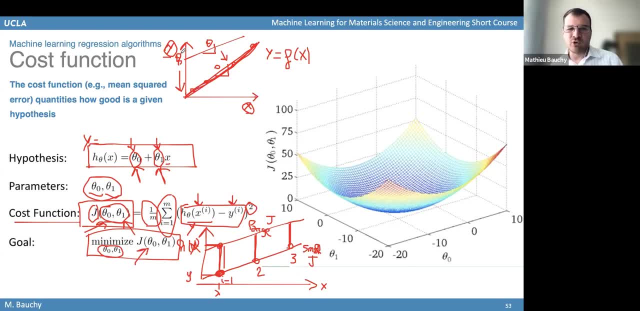 So you have your data points. You will try different combination of theta one and theta naught. For each combination of theta one and theta naught you will get a given value for the cost function. So now you can represent things like this: 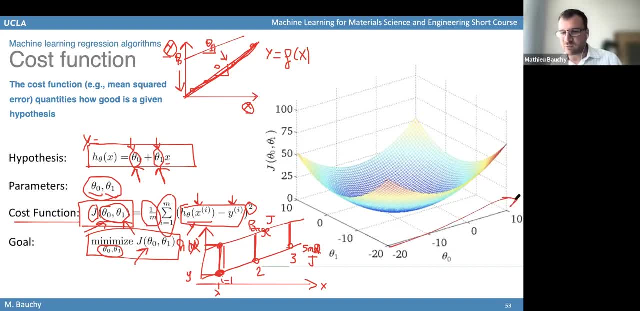 So you have one parameters here which is theta naught. You have another parameter which is theta one here, And then if those parameter change, then your error is going to change. So this axis here will be the cost function. This is the error made by your model. 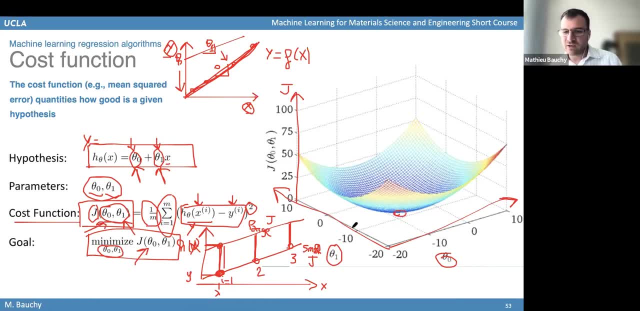 And your goal here is to find this. It's to find the combination of the parameter theta one and theta naught. that will give you the minimum cost function. So you want to find the parameter- This is the number of parameters for your model- that will give you the model that has the lowest distance. 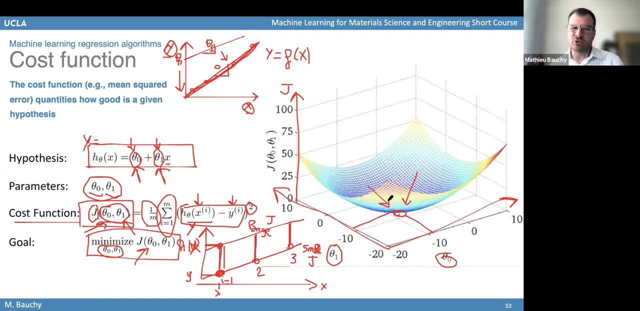 from the actual data points, the model that fits the data point the best. So this is what will be the base of most machine learning algorithm. most regression machine learning algorithm is that you have some parameters and you will need to adjust those parameters in order to minimize a given cost function. 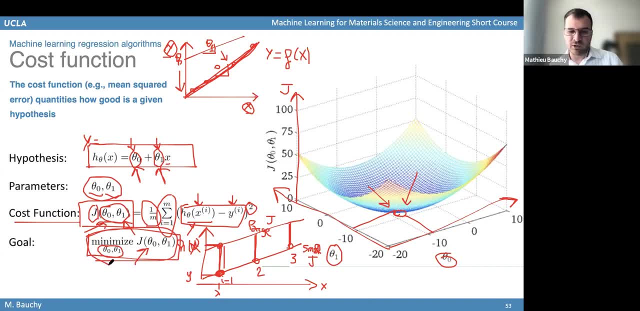 So you will want to minimize the, the given cost. function J to understand that. So you want to make sure that your model is as close as possible to the actual data points that you have. So that's the main idea of how you train a model. 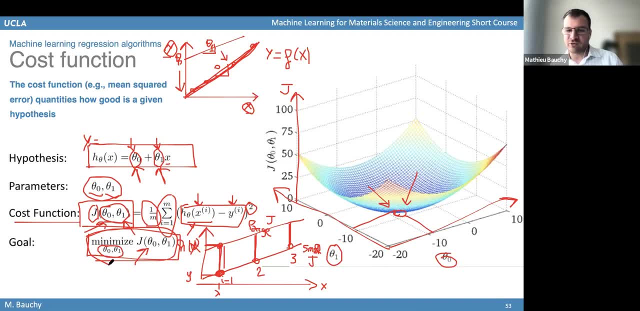 Training a model means you adjust the parameter to try to fit the data as well as possible. So there is various algorithm that you can use for this to find what are the best parameter that will minimize a given cost function. So we're going to talk about one here. 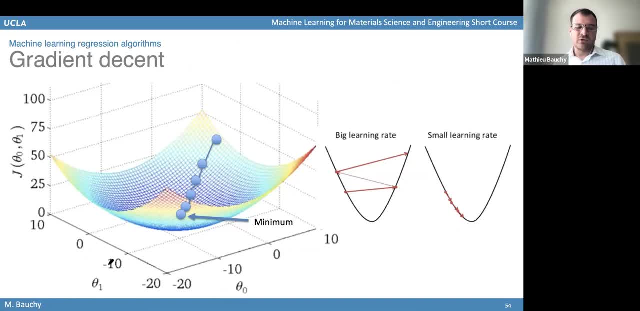 And so this algorithm is the gradient. This sense, So the idea of the gradient descent is as follow. So you want again. your goal is to find what are the best parameter: theta one and theta not. that will give you the access. 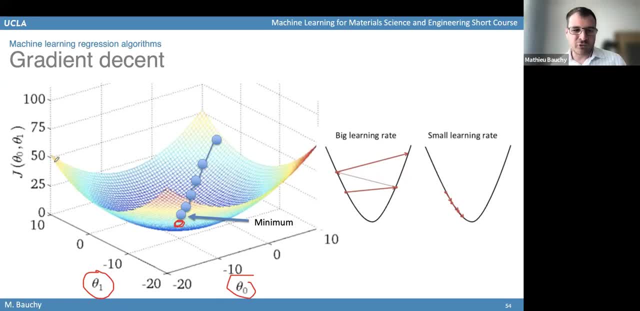 to the minimum of the cost function. So, of course, if you had this plot in front of you, then it's very easy to quickly see where the minimum is. You can just see that the minimum of the cost function is here. So if you have the 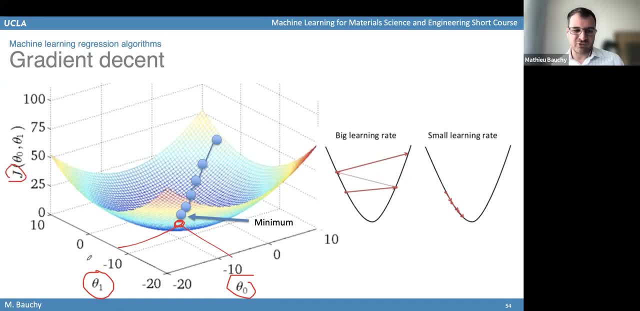 the evolution of the cost function as a function of the model parameter, then it's very easy to do. But in practice you will never know that because you cannot test all the possible values of theta one and all the possible values of theta not. 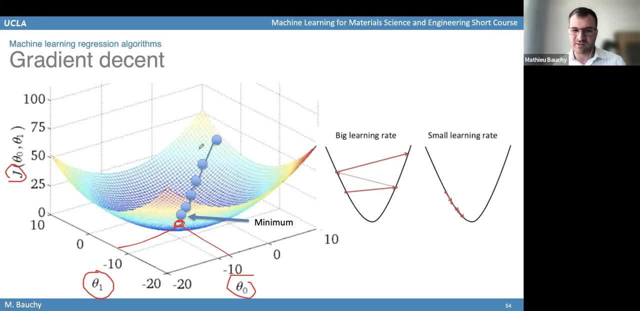 You cannot try everything to build this entire plot here. What you can do is try initially with a given combination of theta one and theta, not measure what is the corresponding value, What is the corresponding error, And then, based on that, you need to decide. 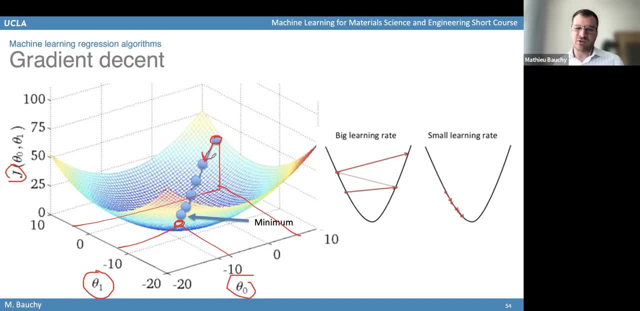 how are you going to change the value of those parameters? How are you going to adjust, How are you going to change theta one and theta not to try to make your model becoming better? But you don't know initially where the minimum is, If you knew already where the minimum is. 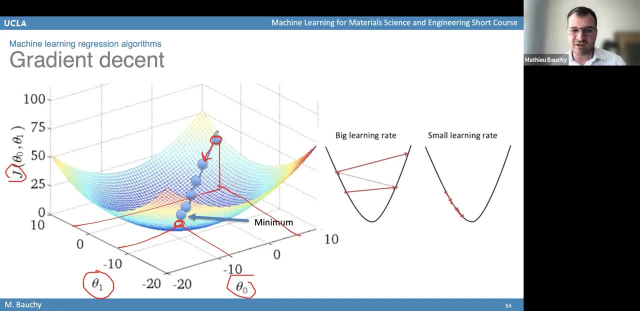 then that would be a very simple problem. But initially all you have is just this point here. So you know. this is the first point for which you know the value of the cost function for a given choice of the parameter: theta not and theta one. 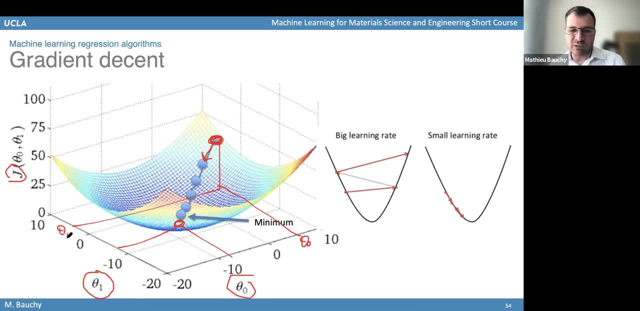 And, based on this point, you want to decide what should be the new theta one and the new theta, not that you should be trying next. So, for example, in this case, what you want most likely is to decrease theta one and you also want to decrease theta not. 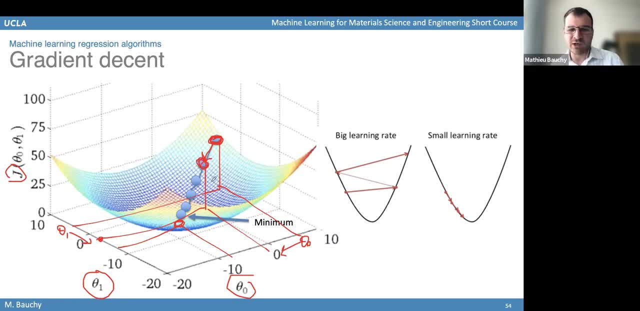 because it's going to give you a new cost function that would be lower. You're going down, you're going towards a more, lower and lower cost function. So here the idea is: how can we decide in which direction should we change? theta one and theta not? 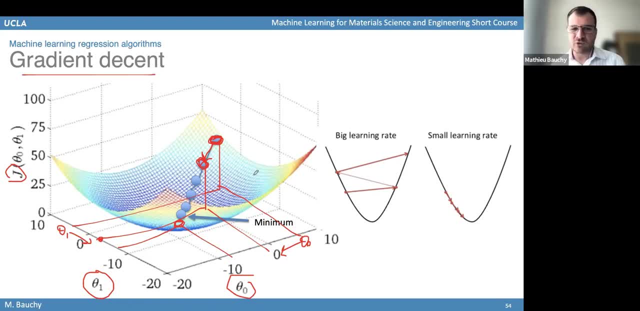 So this is what you can do with gradient descent. So here the idea is that it's the same as if you were walking in some like mountain area and you start from there And your goal is to find where is the lowest possible point. 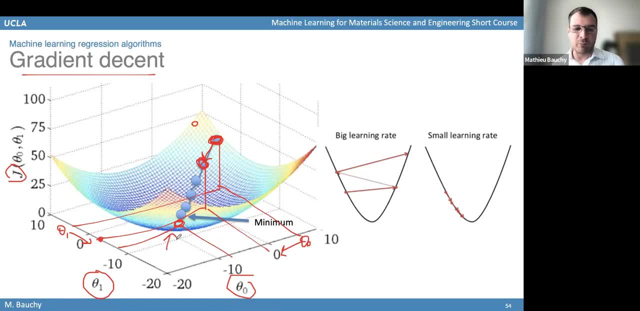 Like you want to find where is the valley here? What is the point with the lowest altitude? So again, if you can see around you and you can see where the point with the lowest altitude is, then that's a very easy problem. You will just directly go there. 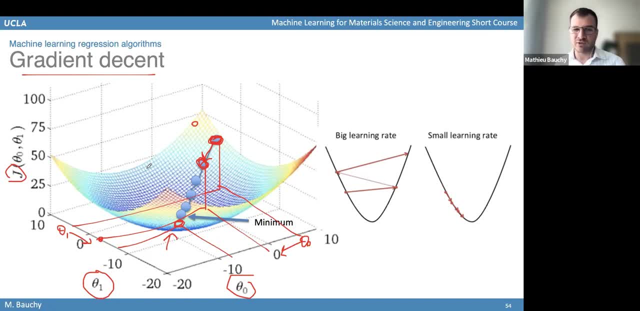 But if there is some fog, for example, if you cannot see around you, then the question is: if you are here, in which direction should you be moving? in which direction are you the most likely to find the minimum? And so the idea of the gradient descent algorithm. 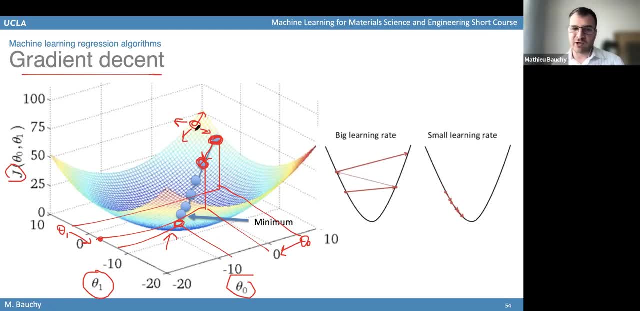 is that you will calculate the gradient of where you are. You will calculate in which direction does the altitude decreases the most. You will try to look towards the direction where the altitude decreases the most And then you will move towards this direction where the altitude decreases the most. 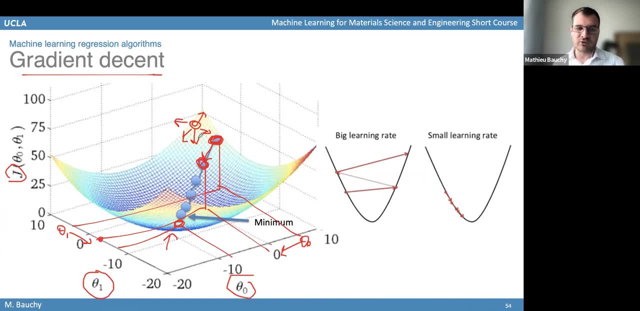 because that's the direction that is the most likely to bring you towards the minimum, to bring you towards the valley where the altitude is the lowest. So here it's gonna be the same idea: You start with a given data point and then you need to find in which direction. 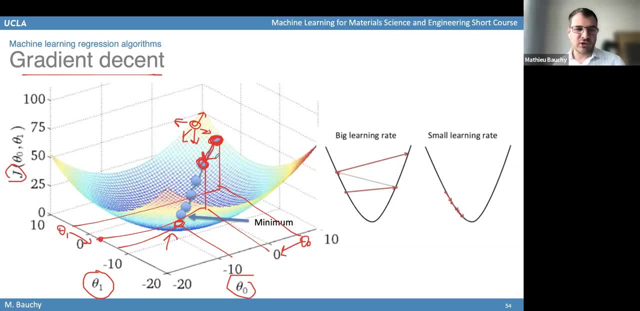 how to change the value of theta one and theta naught. What is the direction of theta one and theta naught towards which the cost function J is going to decrease the most? And so one way to do that is to calculate the gradient. 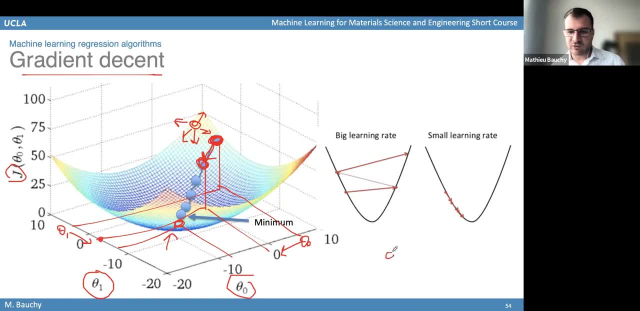 Why? Because if you calculate the gradient, so you calculate the derivative of the cost function with respect to theta naught, and you also calculate the derivative of the cost function with respect to theta one. So if you do that, so you calculate the partial derivative. 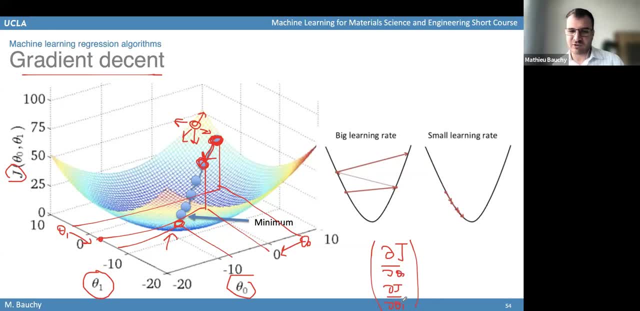 of the cost function with respect to theta naught, the partial derivative of the cost function with respect to theta one. this is the gradient. This is the gradient of the cost function with respect to theta one and with respect to theta naught. 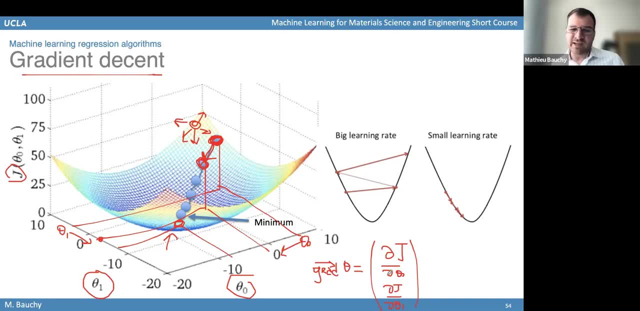 This gradient gives you the direction towards which the cost function increases the most. So if you calculate the gradient of this cost function, it's gonna tell you that this cost function increases the most towards this direction. And then what you will want to do is: 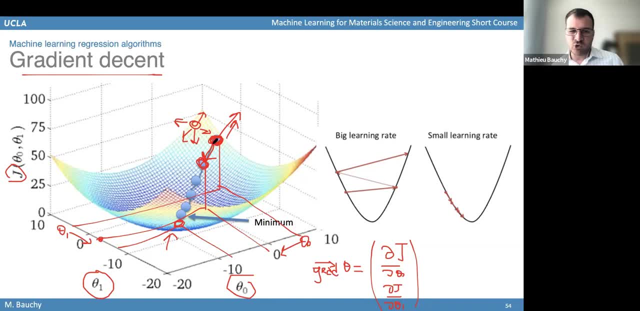 if the gradient is pointing towards this direction, then you will want to go exactly in the opposite direction. You will want to go towards the direction where the gradient is the lowest, because that's the direction towards which the cost function is going to decrease the most. 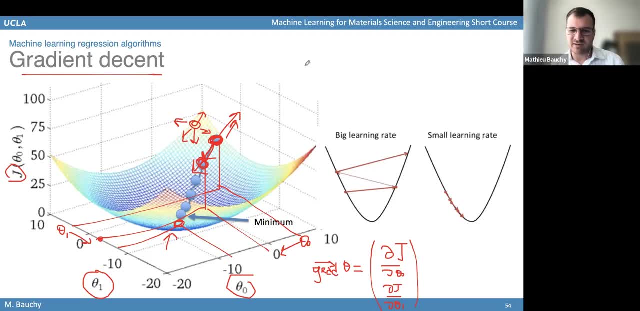 So here, the main idea of the gradient descent algorithm is that you will calculate the gradient of your cost function with respect to the parameter theta one, theta naught, et cetera. Then you know that if you are going to, if you want to change those parameter, 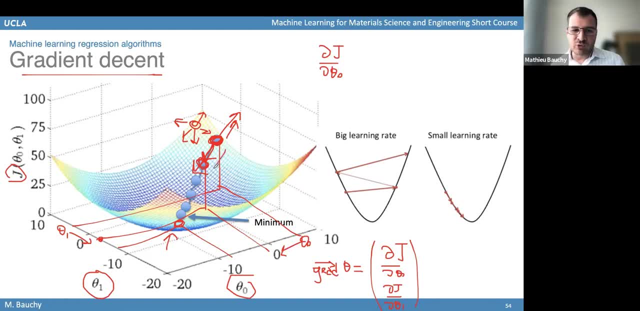 in a way that will minimize the cost function. you need to move towards the direction that is opposite to this gradient, so you will need to to add a negative sign here. If you add the negative sign now, it means that you will be moving. 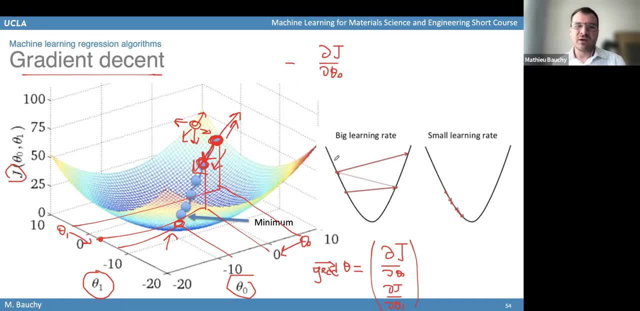 towards the negative gradient, towards the direction where the parameters are decreasing the most, Then. so what you will do is that you will say that initially I had a parameter, theta naught. that was your initial choice of parameter, So I'm gonna call it theta naught one. 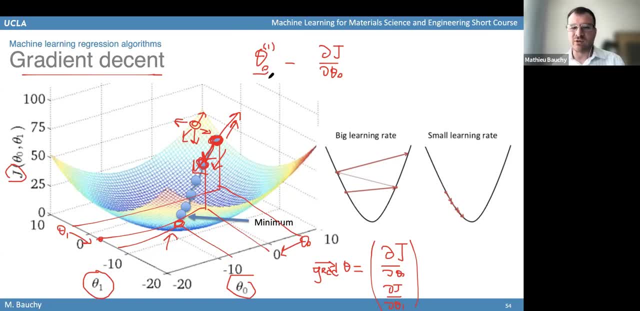 that's your initial choice of parameter And what you will do is that you are going to change, to adjust this parameter, theta naught. So, for example, in this case you find that you can decrease the cost function by decreasing theta naught. 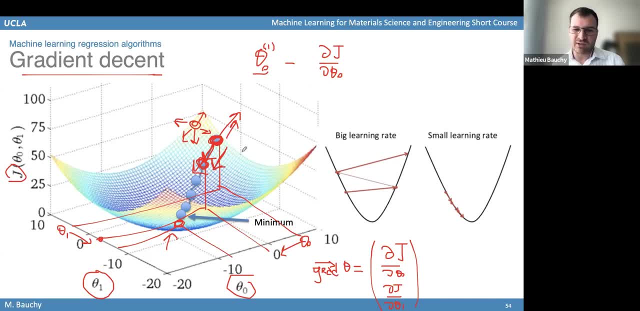 Why? Because the derivative of J with respect to theta naught is positive. if you go towards the right, So it means that you should go towards the left. So what you can do is here you calculate the gradient of the cost function with respect to theta naught. 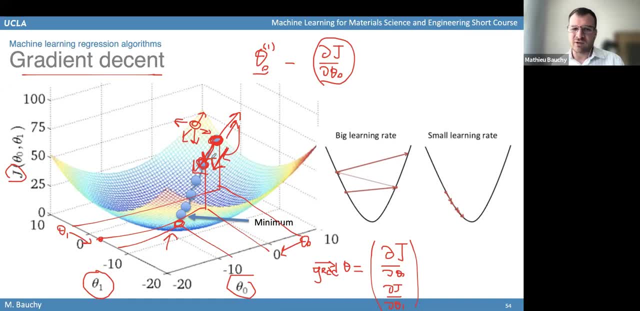 If the gradient is positive, then it means that the cost function J is increasing. as you are increasing theta naught, It means you should be moving towards the left. On the other hand, if you were here, then the gradient would be negative. 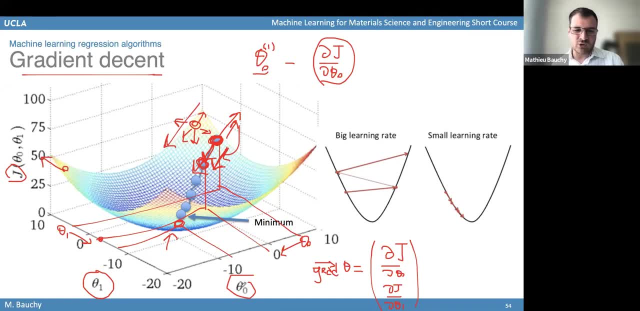 In that case the cost function is decreasing when you increase theta naught. So in this case, if the gradient is negative, then it means that you need to move towards the right. So you always need to change the value of the parameter in the direction that is opposite to the gradient. 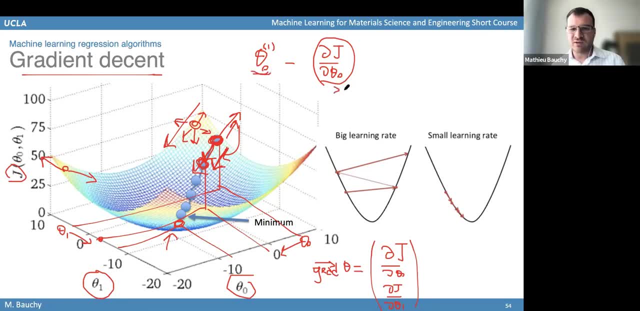 So if your gradient is positive, then you will want to decrease theta naught, So you will do minus the gradient. But on the other hand, if the gradient is negative, then you will do minus a negative gradient, so that will actually increase theta naught. 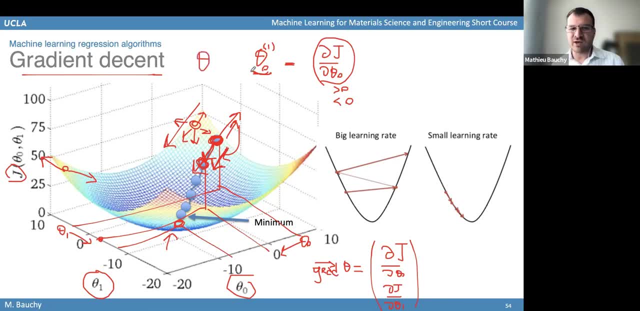 So here, what you will do is that if you have a given initial value of theta naught, you want to predict what should be the next value that you should try. What you will do is to take the initial value of theta naught and either you will increase this theta naught. 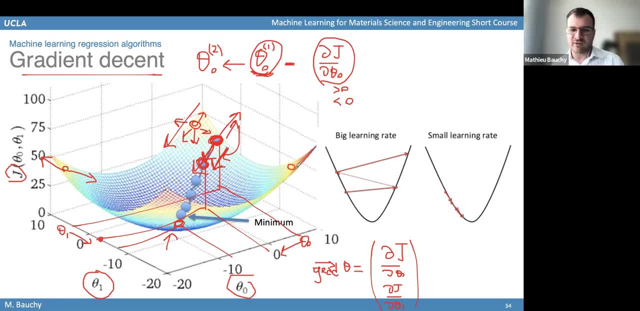 or you will decrease this theta naught. If the gradient is positive, then you will decrease theta naught. If the gradient is negative, then you will increase theta naught. So you will always move towards the direction of the negative gradient. 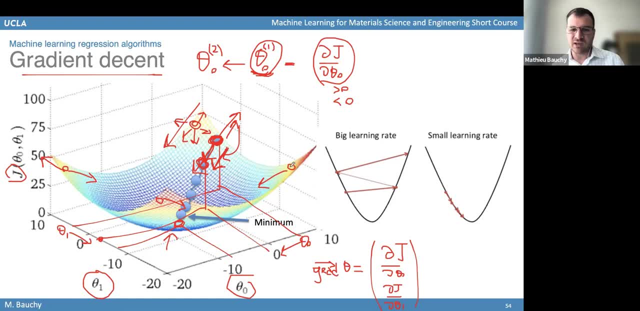 Then the next question is: how much do you move Like? if you realize that theta naught is too high or theta naught is too low, then you will need to increase or decrease theta naught, But you cannot increase it too much. 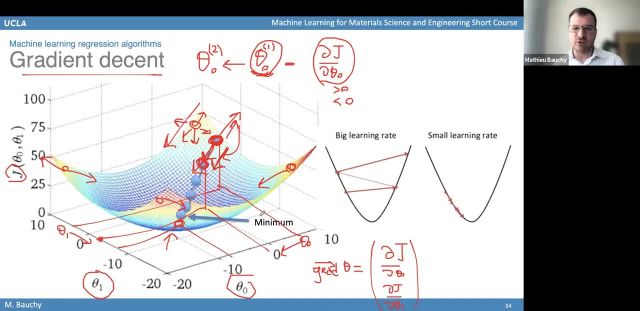 or you cannot increase it too little. So you need to decide how much are you going to change theta naught if you realize that the gradient is positive Or the gradient is negative, And so for this, what you are going to use is to add a parameter here. 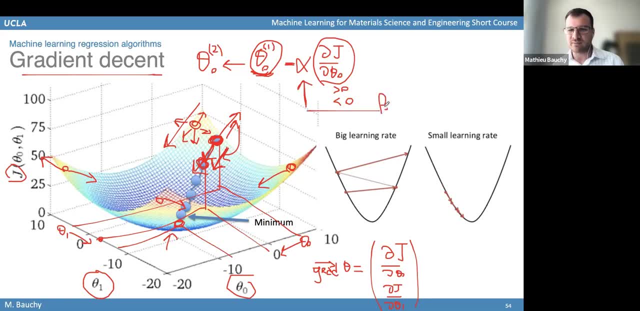 This parameter alpha- it's called the learning rate- And this parameter alpha tells you how much you are going to change the value of the parameter of your model if you realize that the gradient is either positive or negative. So here the idea is as follows: 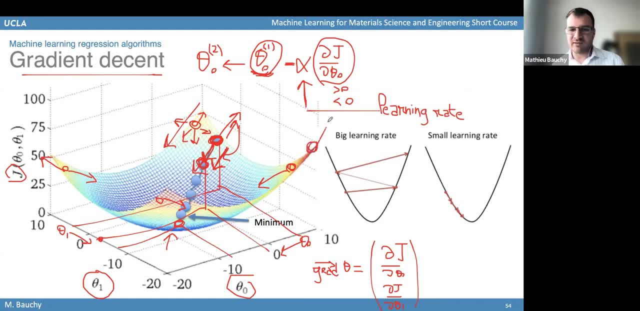 If you are here, for example. so here your model is increasing a lot, Like the error of your model J is increasing a lot. It has a very large gradient, So in that case this gradient here is going to be very large. 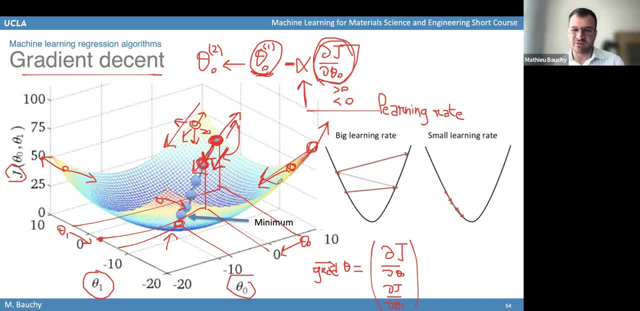 So you will want to move a lot because you know that the gradient is very large. It means that most likely you are very far from the minimum, But on the other hand, if now you are at this point, you are very close to the minimum. 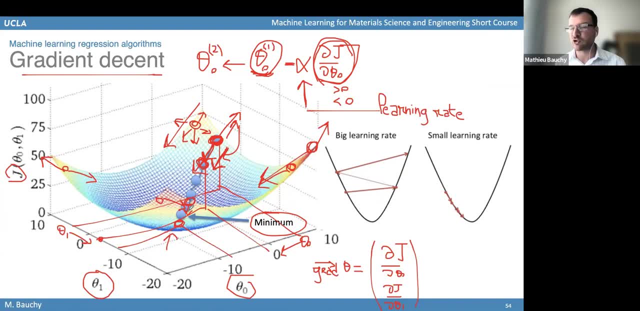 The gradient is much lower- lower because you are closer to the minimum. the slope is much lower, so you will want to move less. so when the gradient is very high you will move a lot. but when the gradient is very low, then you will move a little bit. so the change in delta is going to be proportional to the gradient. 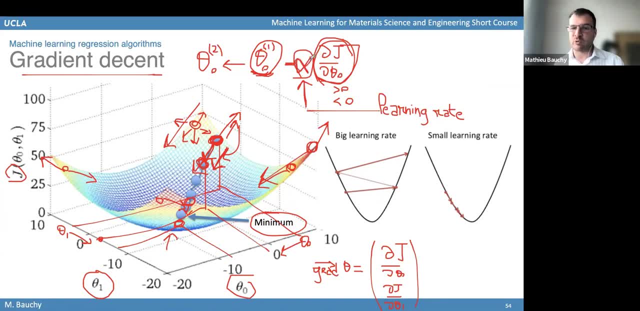 so you will have a number here. this learning rate is a proportionality constant and if you start with a given choice for your parameter- theta one or theta naught- you will change this parameter proportionality to the value of the gradient. if the gradient is very large, it means that you are 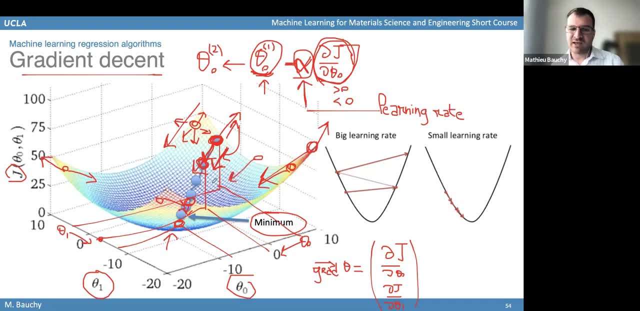 very far from your minimum. so you will move a lot and as you get closer and closer to the minimum, then the gradient decrease, decrease, decrease. so your, your steps, you will change the, the parameters, with smaller steps as you become closer, closer to the, to the to the minimum. so that's the main idea of the gradient descent. you start at a 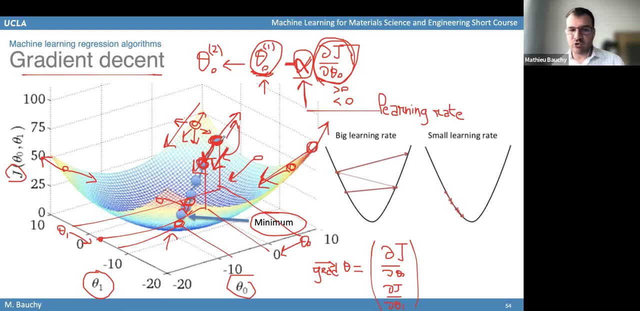 given point. you look at what is the gradient, then you move towards the, the direction opposite to the gradient, to find what are going to be the best parameter, theta that will minimize the error of your model. now the next question is: if you do that like, how do you choose the optimal learning rate? 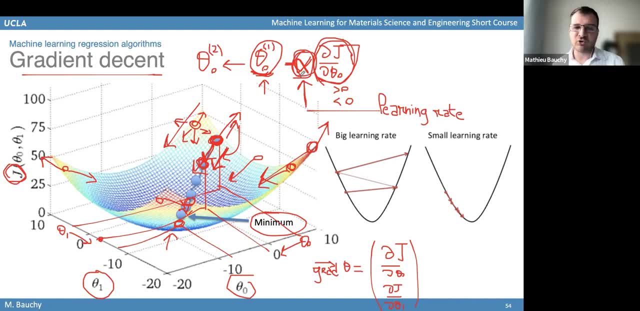 how do you choose what should be the? how much do you want to move, if the, the gradient is positive or negative? you know that if you are exactly at the minimum, then by definition of the minimum, like, the derivative of the cost function would be zero at the. at the minimum, the gradient would be zero. 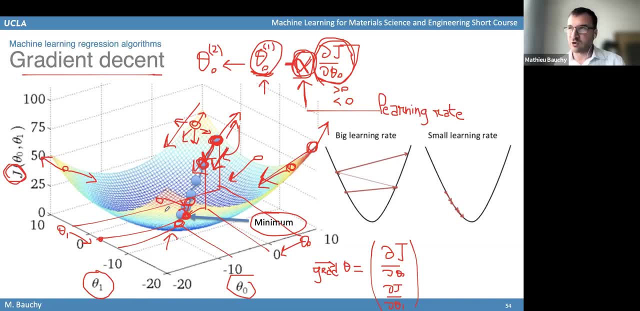 which means that once you reach the minimum, you you won't move anymore. your gradient is zero. you have found the minimum, so you don't need to move anymore. you have, uh, found the best parameter, alpha, and you can minimize the error, minimize the cost function, so you have found the best possible. 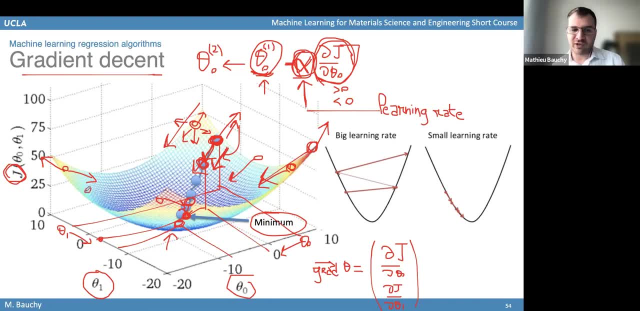 model. but if you are still not there, so if you, if your gradient is either negative or either positive, then you need to decide how much are you going to change the parameter of your model, and this depends on your choice of the learning rate alpha here, and so for this you will need to 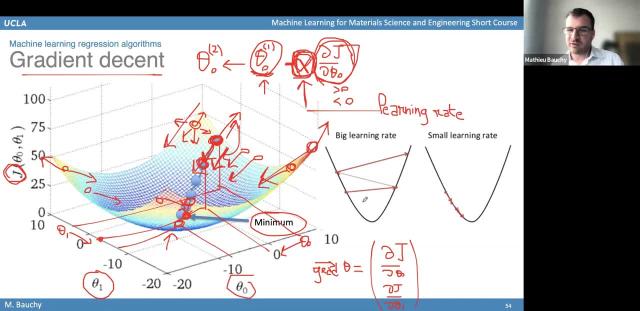 decide: do i want to use a small learning rate or a large learning rate? and usually, uh, the way you will do that is that you will need to choose a learning rate that is not too small, but also not too large. so the reason for this is, if you choose, 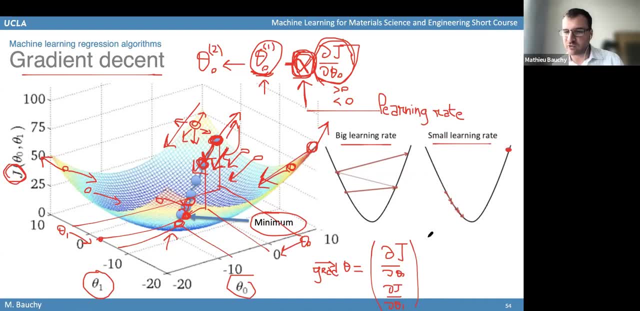 a learning rate that is very small. it means that, for example, you will start here. so what this plot shows here is you have the, the cost function, on the, the y-axis. it tells you how good your model is. and then you have the, the parameter of your model, on the x-axis, which tells you the parameter of your model. 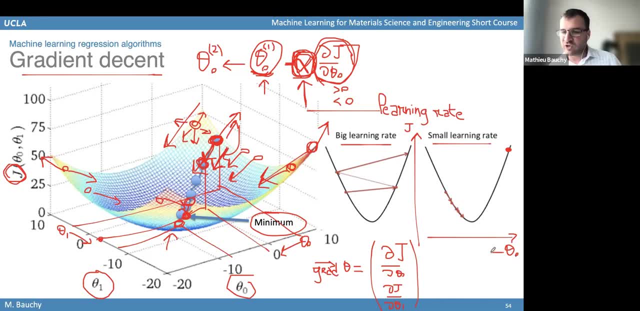 and your goal is to find what is how to change the parameter in order to find the best parameter that will minimize your, your, the error of your model, minimize the cost function. so let's assume that initially you start with: uh, with this point here, you start with this parameter, and if you 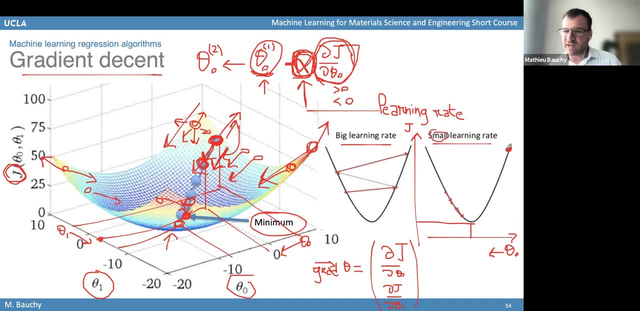 choose a very small learning rate. so here you will calculate it: the gradient, so, in this case, the gradient of the cost function with respect to the, the parameter. this gradient is in this case positive. so since the, the gradient is positive, then you will go towards the negative data, you will go towards the, uh, the direction that is, uh, towards the. 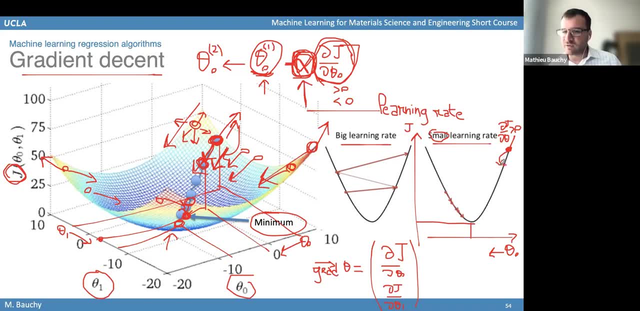 negative gradient, but if your learning rate is very small, then it's going to take you a lot of steps before you can reach the minimum. it's going to take you many, many steps before you can find the minimum. so it's eventually you will find the minimum. you will. 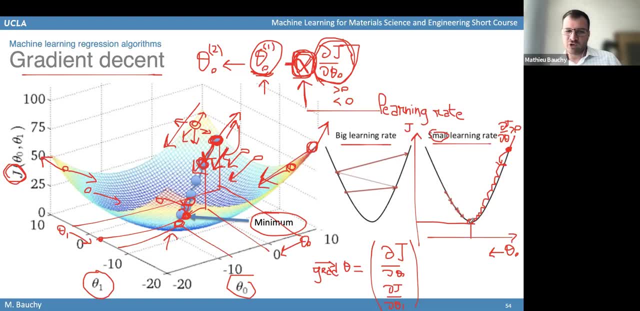 find the best parameter that minimizes the cost function. but it's going to take a very long time because your learning rate is very small, so it's going to take a lot of iteration before you find the minimum, before you find the best parameter. so that would be the problem if your 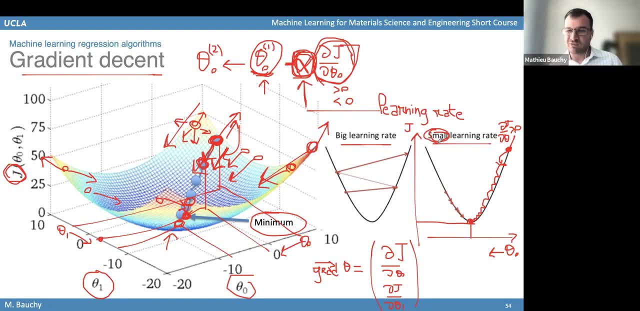 learning rate is too small, it takes you a lot of iteration before you can find the the best model. on the other hand, if, if the, if the learning rate is too high, then that's even worse, because it means that you you will change the parameter too much, for example, here, if you start from there. 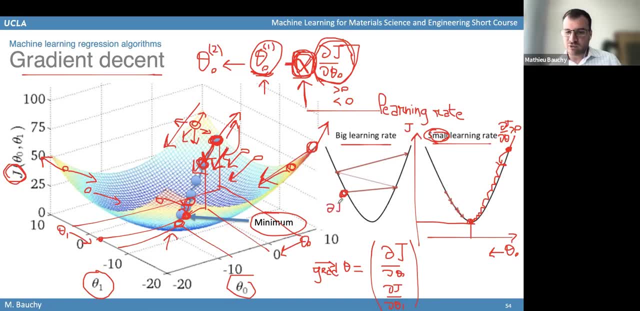 the initially. here the gradient is negative, so the cost function is decreasing with respect to theta. so that's an example of negative gradient, which means that you will move towards the positive theta. you will move towards the right since the gradient is negative. but if you are learning rate is too large, then you will move too much. you will move so much that you actually 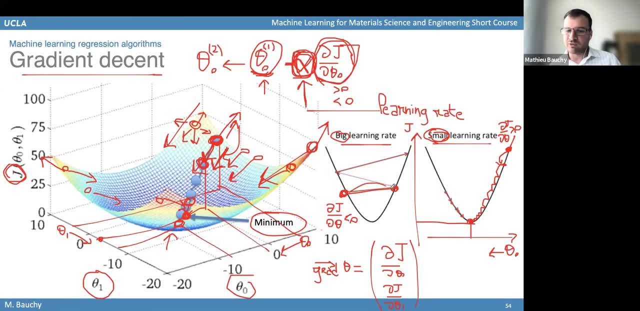 increase the, the, the cost function even more. like you, you move directly towards there because you want to move a lot. so now you reach a point where now the, the gradient now becomes positive. so it means that, um, you will want to move now towards the, the left, so you will move. 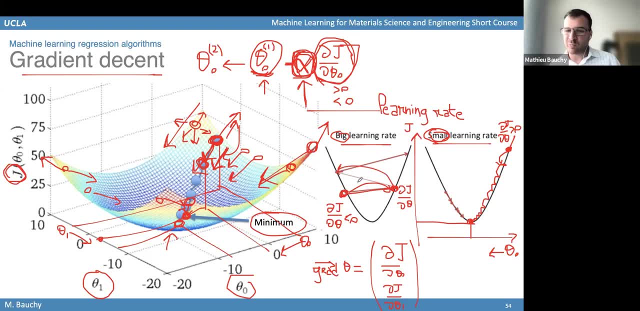 and again you will move a lot, so you will really overcompensate. now you're back to a region where the, the, the cost function, has a negative gradient. so you will move towards the right and again you will move too much. and the more you go towards the right or towards the left, the gradient becomes. 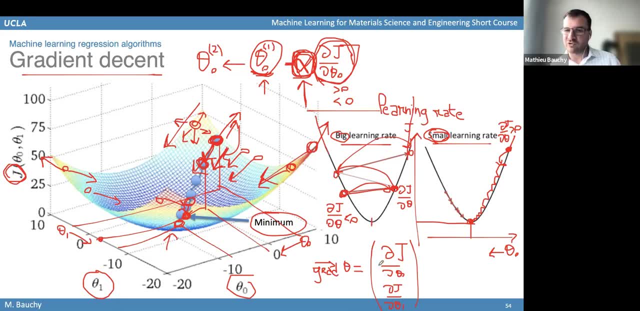 larger and larger because you go far away from the minimum position. so since the gradient becomes larger and larger, then you will move more and more. so you keep getting going. you keep going further and further from the the minimum position. so this would be an example where your learning rate is um, is too high and you, you, um, you, you keep overcompensating. if, if you. 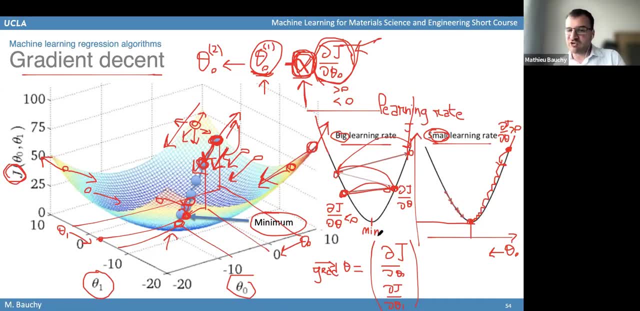 make um a given error. you keep changing the parameters too much, so that you actually go further and further away from the optimal value of those parameters. so ideally, the way that you should do it is that you should choose a learning rate that is going to be in between those two. 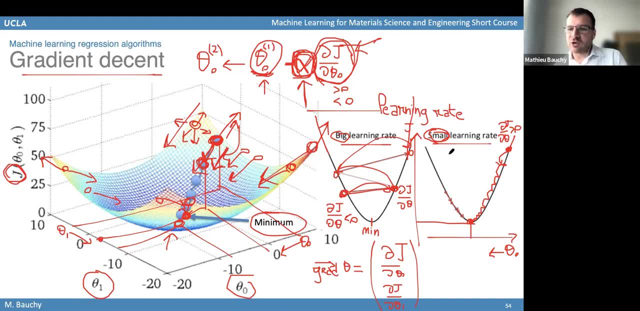 extreme, a learning rate that is going to be not too small so that, uh, you will still um find the answer without too many iterations, but also not too large so that your, your, your optimization, is not unstable, that you can actually decrease the, the, the cost function so, like typically, what you should do for this is, if you're trying to 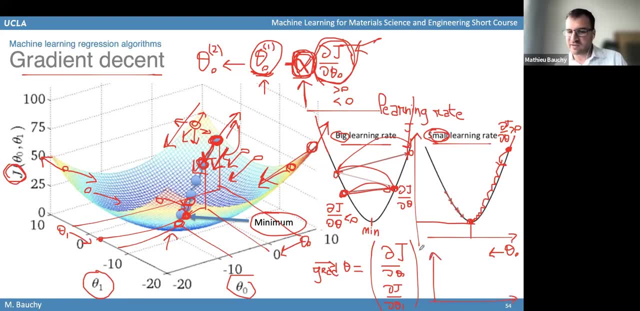 train a machine learning model. so it's going to take several iterations where you try you start with a given choice for the initial parameter, then you are going to slightly change those parameters, step by step, using this gradient descent technique. you're going to try to increase or decrease the value of the parameter, and so you will do that iteration by iteration. 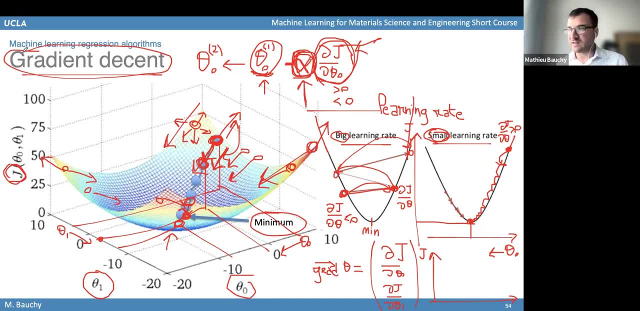 and what you hope is that gradually the cost function will decrease. so if, if you start initially at iteration uh, number number one, your cost function is going to be initially like this: if your learning rate is too small, then your cost function will slowly decrease, but it's going to take a lot of time before the the cost function. 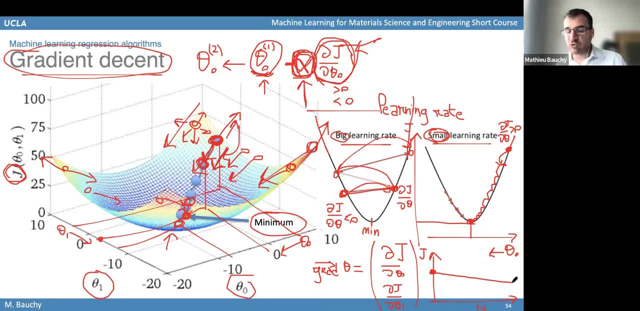 becomes close to zero. so it's- uh, it's going to work. we're just going to take a very, very long time. so this would be: if your learning rate is- um is too small. on the other hand, if your learning rate is too high, then you will be in this situation. 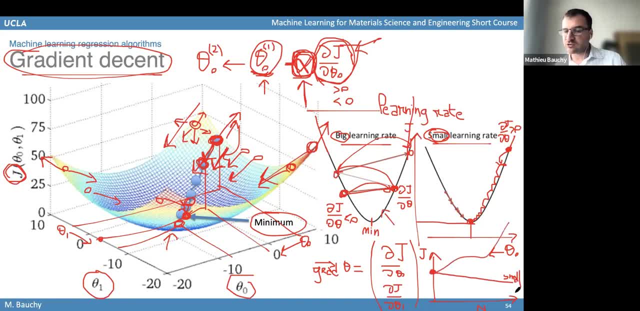 in this case here, where your cost function is actually, uh, increasing, keeps increasing. so in that case your model becoming worse and worse. so that would be a case where your learning rate is is too large. so what you want, ideally, is to find the optimal learning rate that would give you. 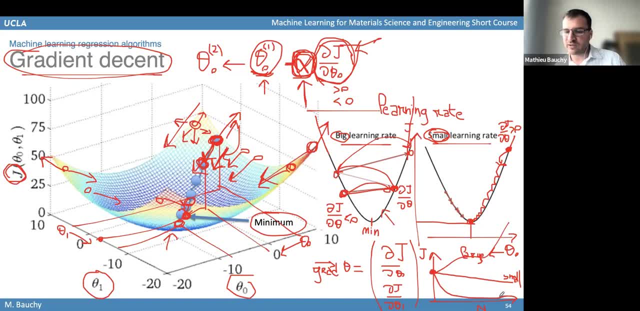 something like that, where your cost function quickly decrease and then converges towards a cost function that is very close to zero. so that would be the case where you have, in this case, an ideal learning rate that is not too high, not too low. so the idea here is, if you want to find the best learning rate initially, 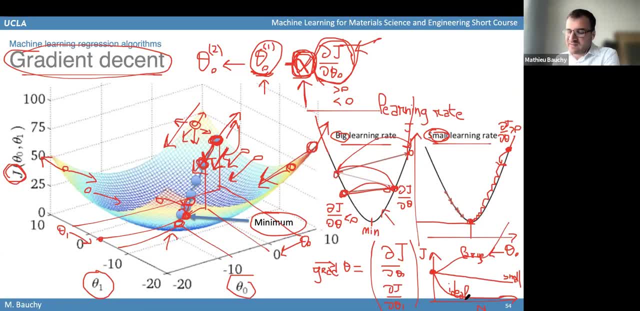 you won't know what is the best learning rate. so you and you need to try several learning rates to and to track how the cost function decreases as a function of the iteration, and to check that first, your, your cost function, your learning rate, is not too large that your cost function would. 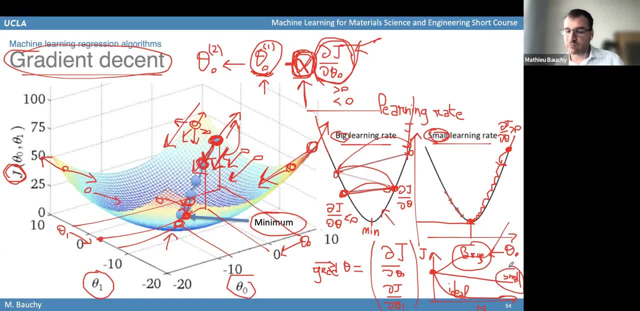 actually increase over time, or that it's not too small that it takes forever for the model to find the best parameters. so you want to find the ideal learning rate is going to be the one in between those two extreme cases where your cost function decrease as quickly as possible and then converge. 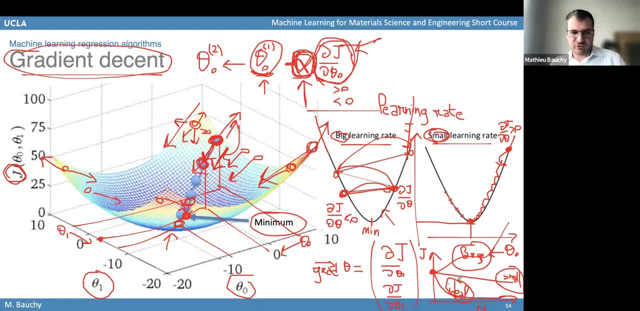 towards a low value for the, for the cost function, for the cost function- j- do you have any question about this? like this. so this is an important point because this is going to be the base of any kind of training, a machine learning model. you will start with a model and then you will need to train to adjust the parameters of this model. 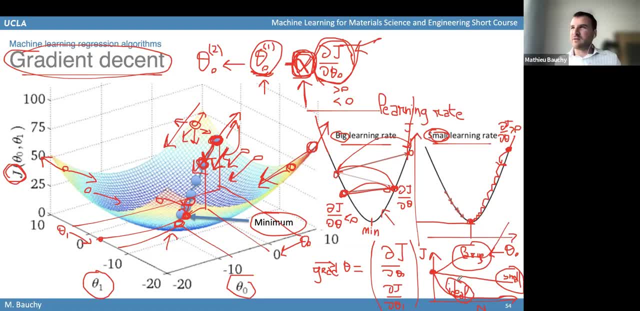 so as to decrease the difference between the model and the, the actual data point. so this is always going to be the idea of any machine learning model. you will define the cost function j. then you will need to adjust the parameters of your model to decrease j as much as you. 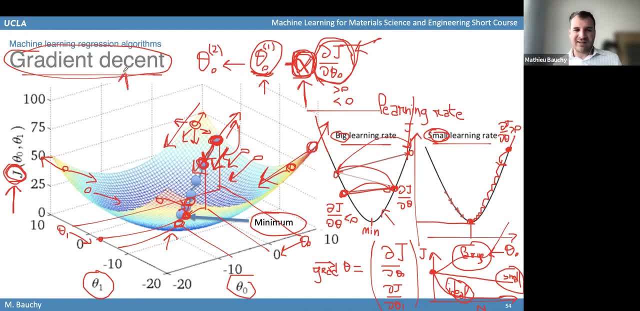 can, and typically you will do this using this gradient descent algorithm here, where you adjust step by step the parameters in order to decrease j, and for this you will very often need to use these types of learning rate where you decide if the, if the gradient of the, the cost function. 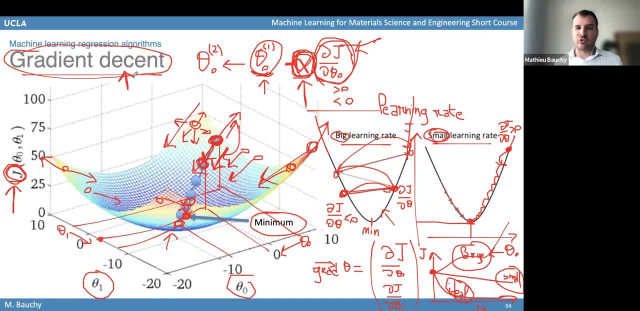 respect to the parameter is not zero, then how much are you going to change the parameter? are you going to change the parameter very quickly or are you going to change the parameter more slowly? and for this you will need to find what is the optimal value of the learning. 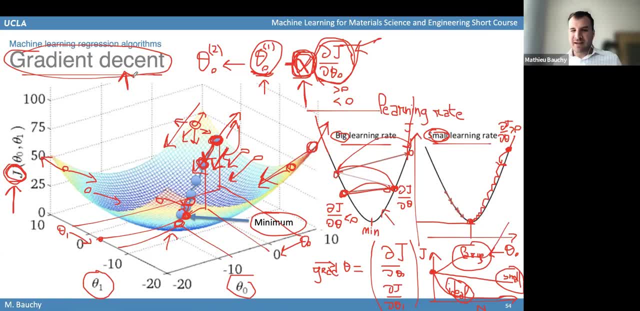 rate, so that you have a model that can learn as fast as possible what are the right parameters, without taking forever or without being unstable, where your model becomes worse and worse at each iteration. is there any questions regarding this? yes, i have a question for you. okay, your simulation. 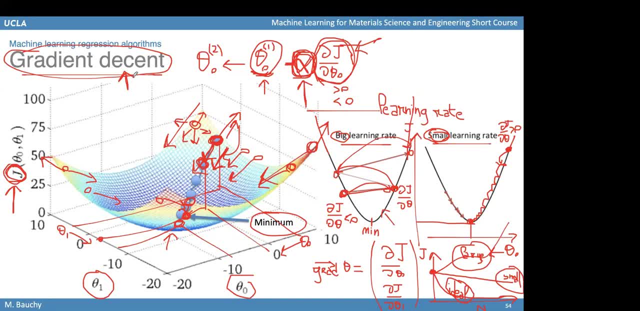 is: uh, when you modify the promotional instance, uh for one thing, and then change the model, is it possible to do this with? with the existingsolve model in in lab programs or what is? it can be anything right, so the you can do it in matlab or you can write it, so you will need to um. 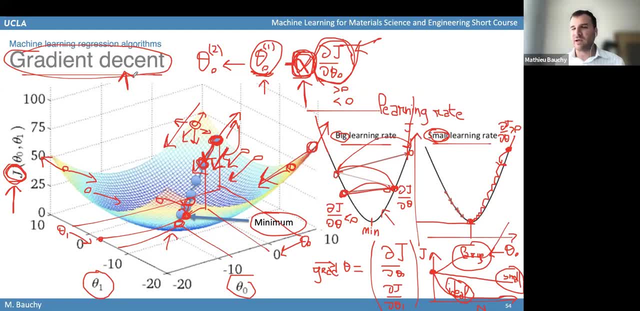 to to use some kind of language right, so you can. many machine learning people use the, the python. it will already come with some function that you can use to do these types of gradient descent. So in MATLAB you already have some optimization technique that you can already use to optimize some parameters. 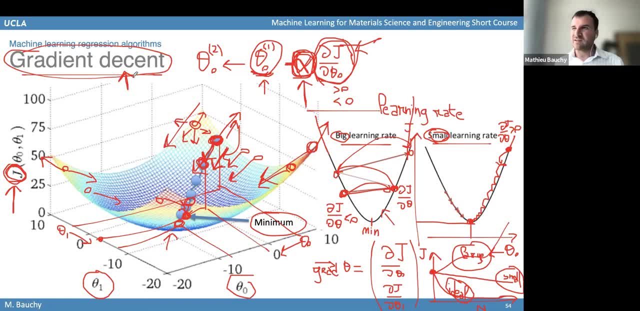 of a function in order to decrease a cost. function like this. So if you are using MATLAB, for example, then you can already. these types of algorithm will be already implemented so you can directly use it, But it can be done with any programming language. 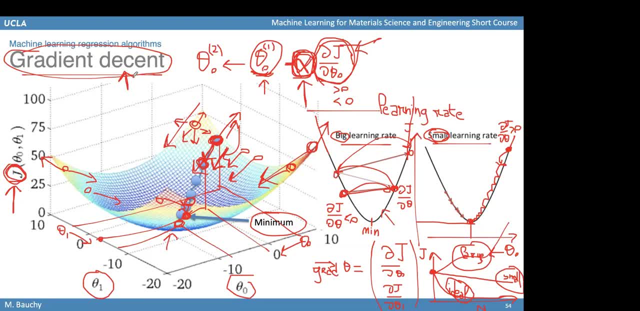 MATLAB or something else. Okay, thank you. Another question, Anne. in your experience you recommend that you use could be in MATLAB for machine learning. I would recommend you to use whatever you are already comfortable with, Like you can. I don't think there is necessarily a language or software. that is, you know, you can you know, you can you know. I don't think there is necessarily a language or software that is: you know, you, can you know, you can you know. it's much better than another one. 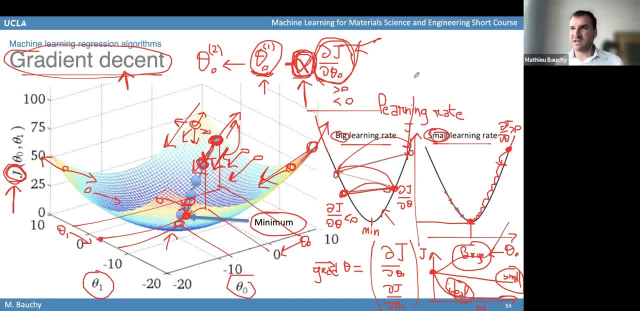 Like, because, like, you can do almost everything with MATLAB, or you can do almost everything with Python, or you can do almost everything in R, for example, which is another language that is used for machine learning. So I think the premise is not how to choose the best package. 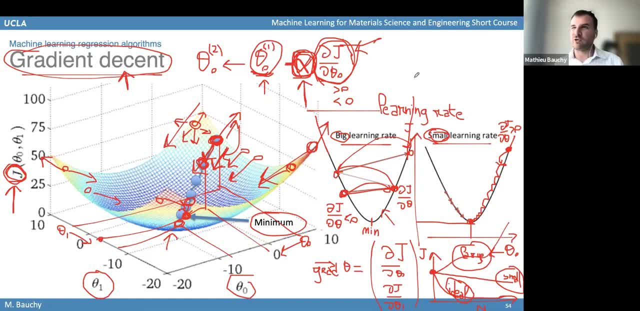 It's just you should use the software or the language that you are already familiar with, because that's gonna make it easier for you to use it quickly without having to learn everything from scratch. So I would recommend, if you already know, MATLAB. 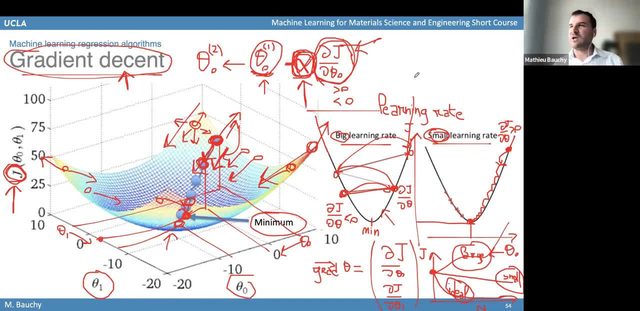 then you should just use MATLAB. If you already know Python, then you can use Python. I mean, if you don't know anything, if you're not familiar with any programming language, then maybe I would say if you have more an engineering background. 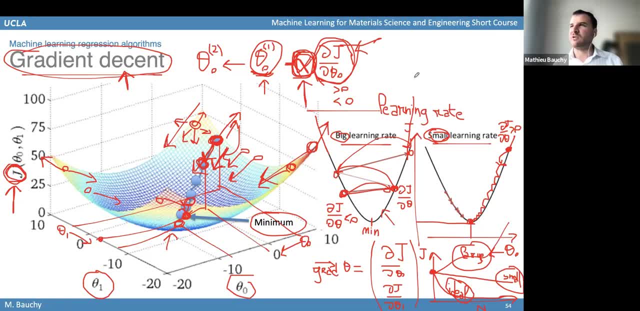 then MATLAB is gonna be maybe the easiest for you. If you are more, like I would say, a computer scientist, maybe a computer science background, maybe Python would be the best choice. So if really you're starting from scratch, then you can choose either MATLAB either Python. 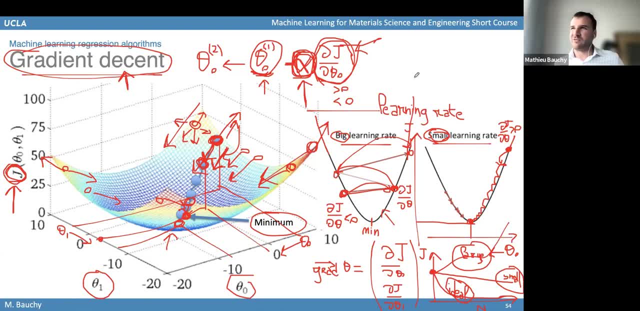 But if you already know something, if you know MATLAB already or another types of language like this, then I would recommend to just use the one you know, because that's just gonna make it easier for you to get started And again, there's no big difference. 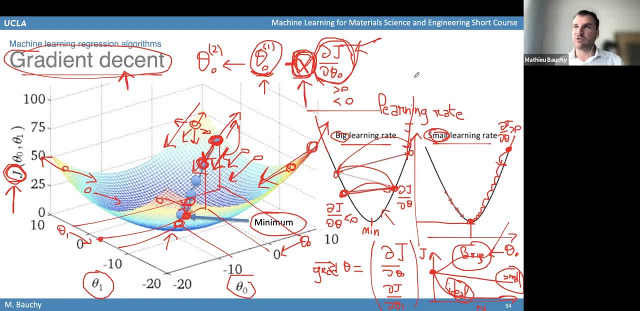 between what you can do with MATLAB. with Python You can do most of the machine learning model. You can do them with any language, So you should just use the one that you prefer. Okay, Fen doctor. Thank you. Any other questions regarding that? 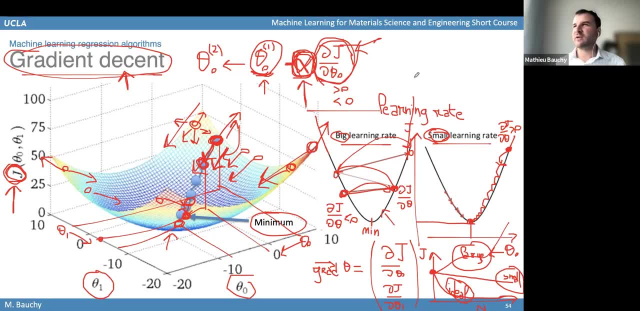 Okay, Just one thing. So in this course here, since it's a little bit short, like we don't really have time to actually see some examples of how we would do that in MATLAB, like with some actual coding, But if you're interested, 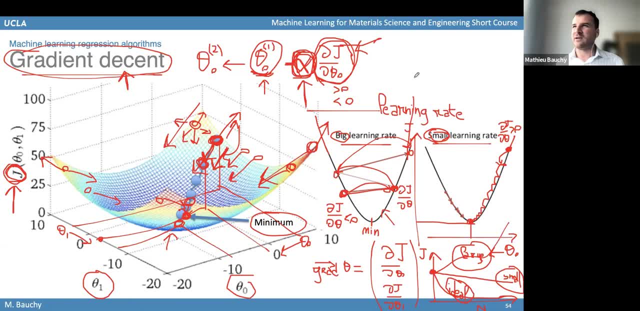 I have some other videos online where I have some actual example on how you would do that in MATLAB, the actual function and the actual code that you would be using. So at the end I can send those videos to you if you want to actually see some example. 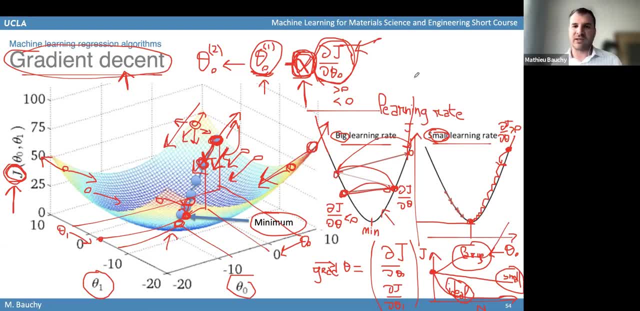 of how you would do that in practice in MATLAB. But in this course I'll focus more the ideas and the theory behind machine learning but like to use it in practice. I would refer you to some other videos where you can see step by step or line by line how how to do that in practice. 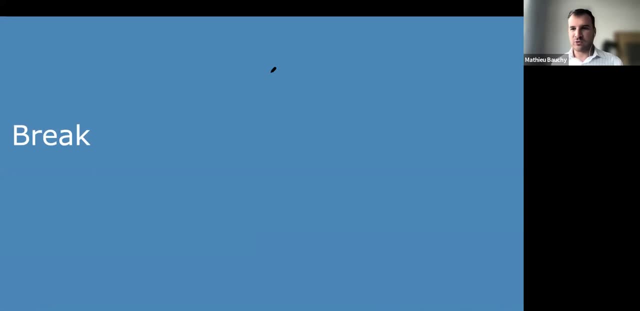 okay. so I suggest we do another short break, so we can do another 15 minute break, if that's okay for you here. and so what we're going to do after we come back from the break is now to see a complete pipeline, like to see if you want to solve a given problem in material, like what would be step one. 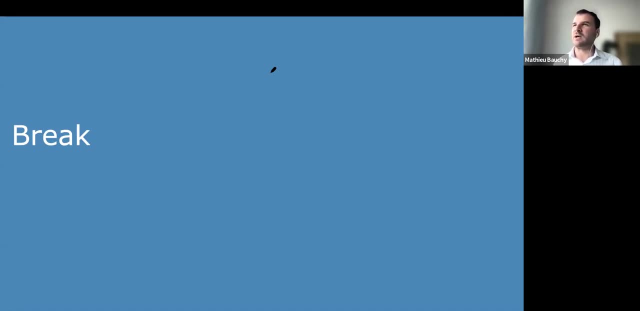 step two, step three, etc. so, like, what would be all the, the, the different steps that would be needed in order to, to, to achieve the, to, to create a machine learning model and to use it in practice. so we will see, with all the, the different steps, that that you should be, that you should be doing in. 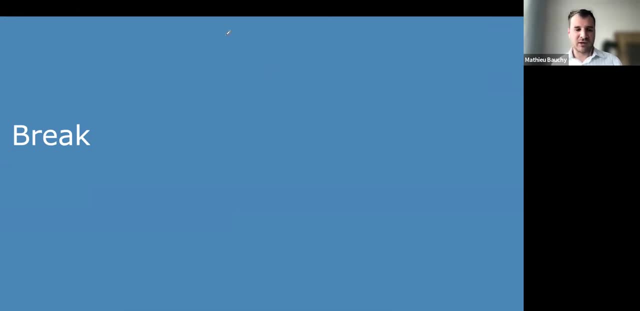 practice. so we'll see that after the break. so again, like so, I think we can take a 15 minute break and come back in in 15 minutes again. if you have any questions meanwhile, let me know, otherwise I'll see you in 15 minutes. thank you, welcome back. so we're gonna restart like the, the further and. 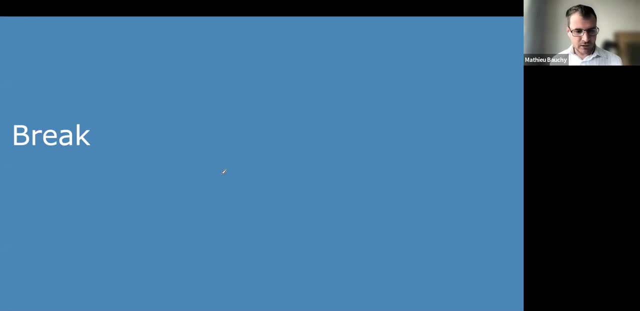 last part of this, of this course. again, if you have questions, feel free to to stop me as we go. so, so now what we are going to talk about is how to, in practice, what would be the different steps from the very beginning to the very end of if you want to develop and deploy a machine. 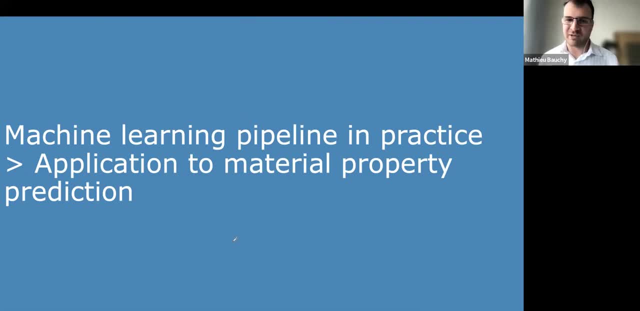 learning model, to to predict from all the properties of a given material. so we're going to see like what would be the, so what we call the, the pipeline. so the pipeline would be the different steps that are needed in order to get there, from the very early stage to the, to the later stage. 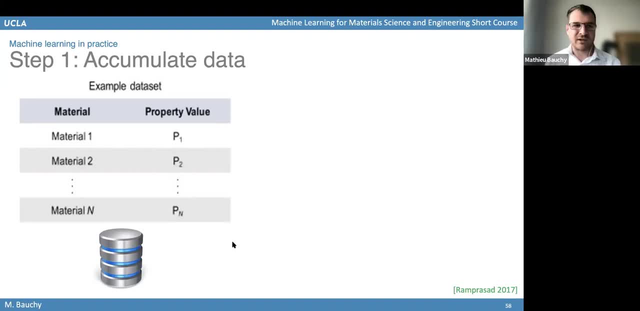 okay, so there, in total there's going to be like I think, eight to nine steps, something like that. so like, in each step is can be important, but but some to some extent can be more important than other and to some extent, like the most important step- because it really enables machine learning- is to accumulate data. so if you don't have data, then 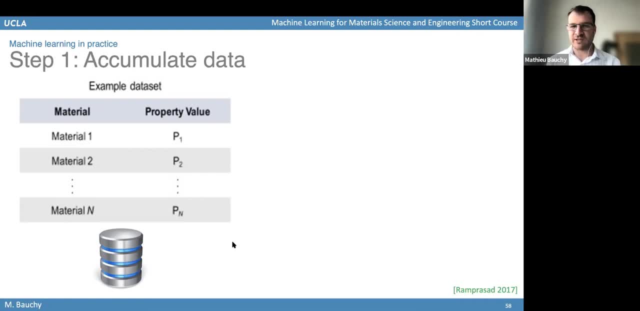 you, you won't be able to um to do any kind of machine learning analysis, so that that's really, to some extent, the most important step. it's to accumulate data, and so accumulating data about materials means that you need to create some kind of data set that contains. 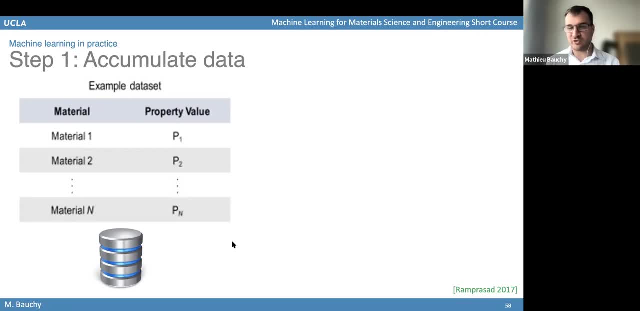 for a list of different materials or for a list of different conditions, to to contain, like, for those condition or for those materials, what is the corresponding property. So it needs to be like a data set where you have different materials for different composition, for example. 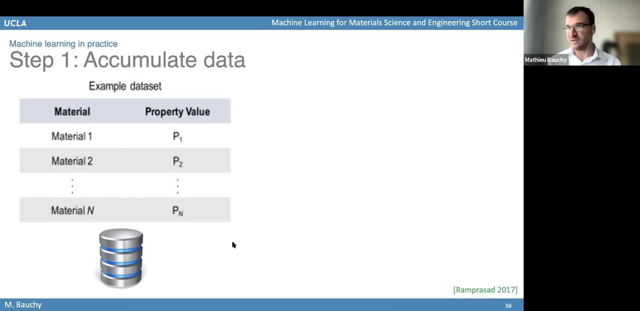 and the associated measure, property or a different material under different condition of temperature, pressure, et cetera, together with this property. So that's gonna be the first step, And so gathering those data means that either you are going to do the experiments yourself, 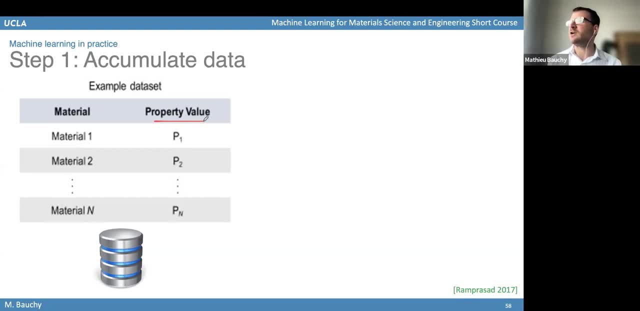 so generate your data yourself, in your group, by doing some experiments on different materials with different condition, et cetera. or you are going to gather those data from the literature to source and to mine different publication, or you can use some libraries or some database. 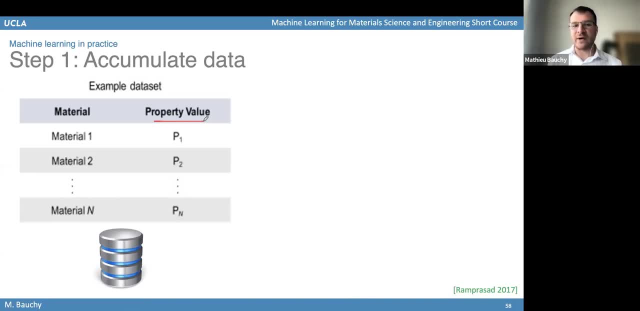 some database of material properties that have been curated already, And so that's the first step, And so the main aspect behind this is that you need to make sure that, since machine learning only rely on data, you need to make sure that your data set. 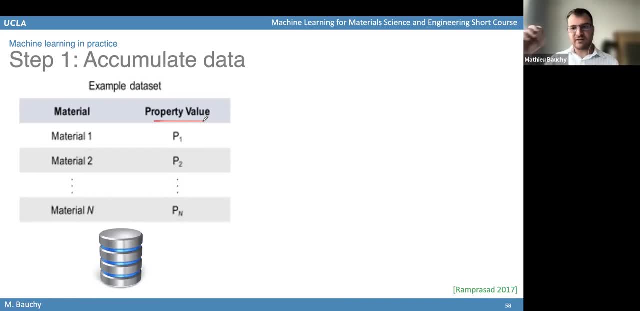 will contain good data. If your data set contains bad data, then your machine learning model will be bad as well, So everything will rely on that. So you need- this is gonna be a very important step, which is to ensure that your data set is of good quality. 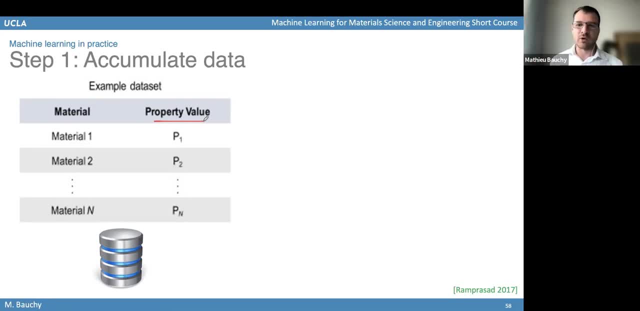 If your data set is of bad quality, then all of your subsequent machine learning analysis will also be of bad quality. Then the next question is: what do we call good data? So like, a good data would satisfy several condition. So the first thing about data. 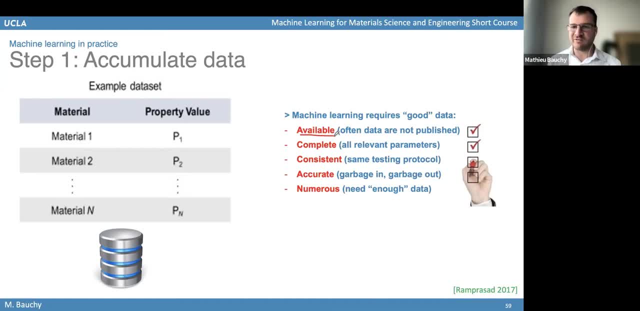 which is sometimes the main bottleneck, is that it needs to be available. So if the data is not available, then you cannot use it. For example, if you find a publication that reports some result, but if you have, if the data are not provided. 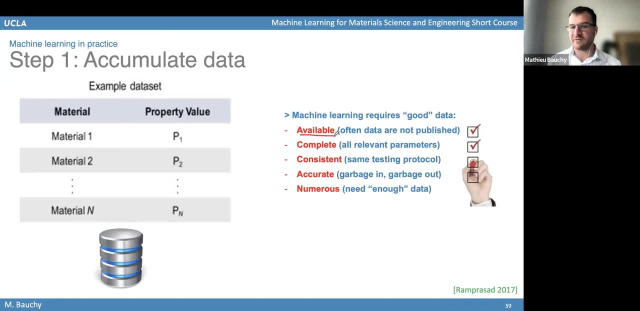 as part of this paper, then you will not be able to use it unless you contact the author and they are willing to share this data. Or sometimes company would not be willing to disclose their data Like, so they would keep the data private, proprietary. 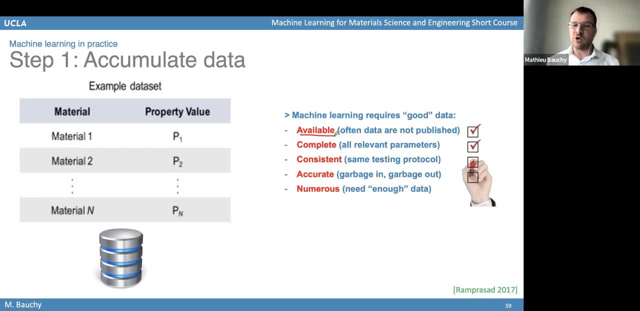 So in that case that would be very difficult to use To access them. So the first attribute that is needed is that this data you need to be able to access it, So it needs to be available. So that's one thing. 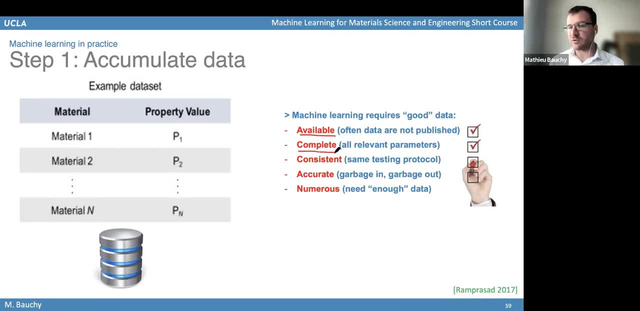 The second thing is that the data needs to be complete. So what it means to be complete is that you need to know all the relevant features that fully describe a material, For example, if you have different material that are tested and you know the property that are measured. 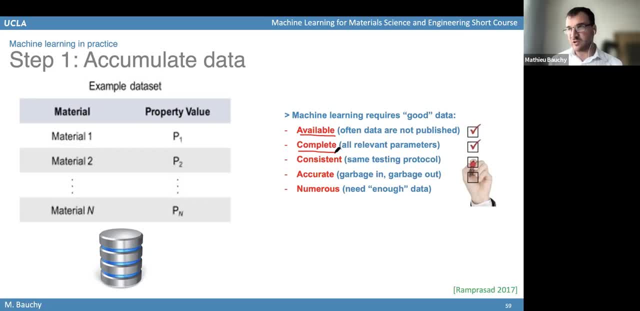 for this material and you have access to this, this data set. But if there are some information missing about, for example, what was the temperature during the test or what was the relative humidity, and if those features are missing, if they turn out to be important, 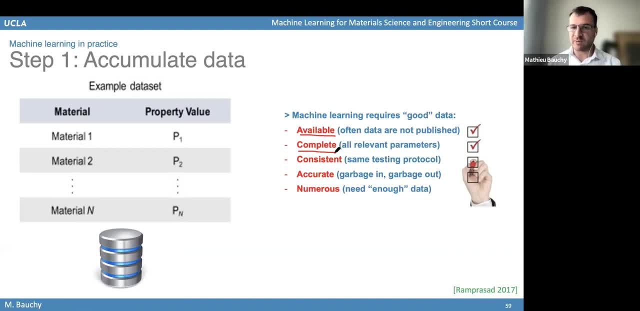 if those features are also influencing the properties of the material, if they are influencing the results, then if you don't have access to those details, then you would not be able to develop a model that can predict properties, Because if this property depends on temperature, 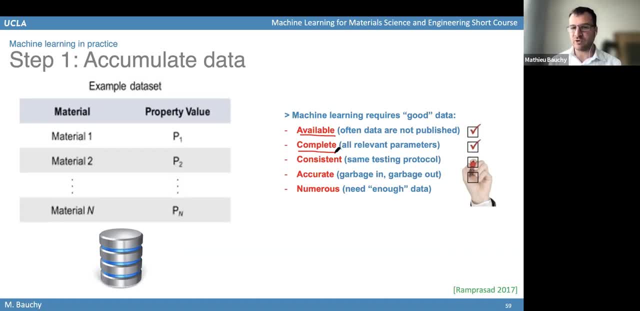 and if you don't know what was the temperature that was recorded when then this property was measured, then you won't be able to teach the model how to predict the value of disparity if it didn't know what was the temperature during the measurement. So the data needs to be complete. 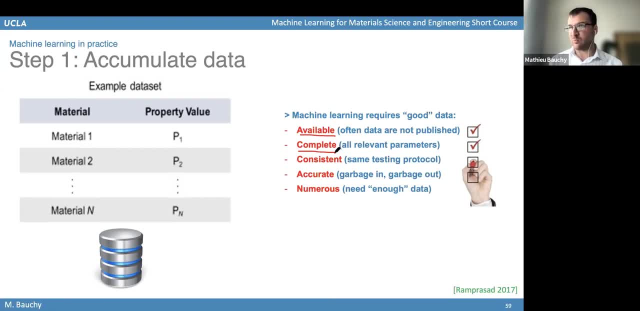 And so when I said by data needs to be complete, it means that you should need to know all the information that you need In order to make the prediction. So if you don't know the composition of the material, if you don't know the temperature, 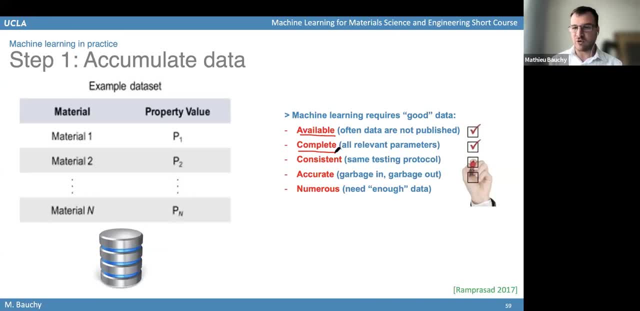 if you don't know the relative humidity or if you don't know other parameters that are influential, then you will not be able to train a machine learning model. You don't always need to know all those details, For example, if temperature does not really matter. 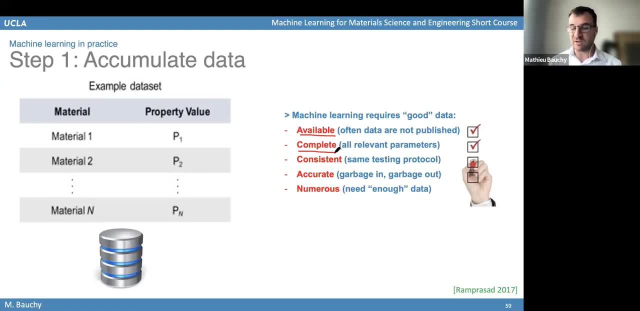 if relative humidity does not matter, then you don't need to know it, But if it's something that matters, then you need to have this information as part of the list of input so that your machine learning model can learn how to relate the input to the measure of priority. 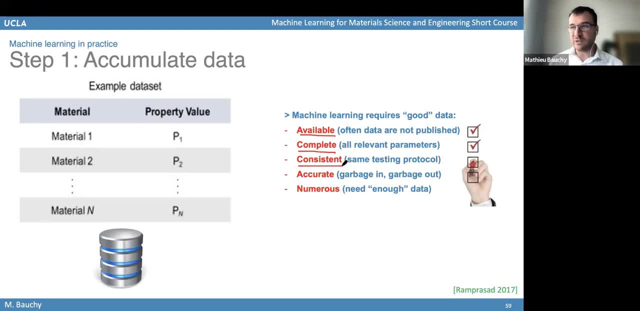 Another thing that is pretty important is the data needs to be consistent. So consistent means that the data that you get, they need to be obtained using the same protocol, And that's a problem if you, for example, are going to gather data based on the literature. 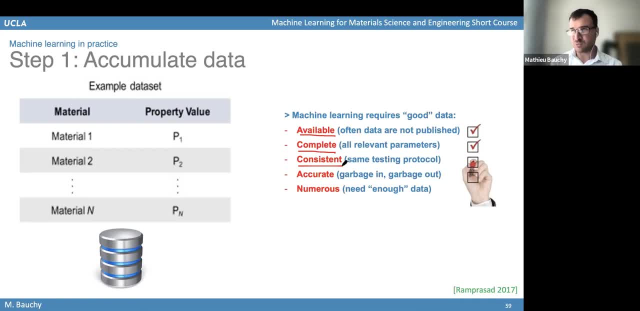 and you're going to use the data, And you're going to use the data prepared by different groups, then there is a risk that those data might not be consistent, because maybe different groups are not using the same protocol to test material, Maybe they are not using the same equipment. 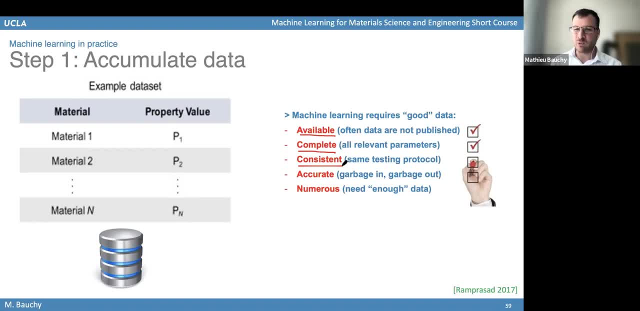 And sometimes maybe, even if it's not the same operator, even if it's the same group, but it's a different person doing the experiments, like they might get different result out of this. So, ideally, since you are using those data to train the machine learning, 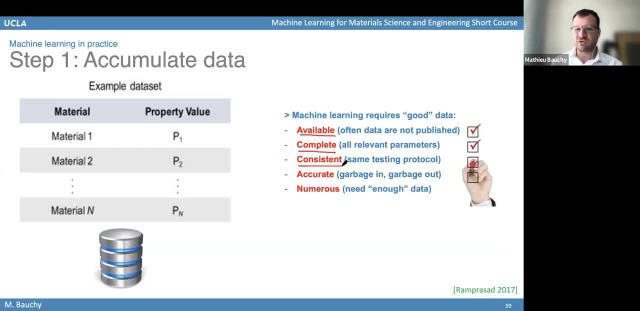 model, all those data needs to be fully consistent with each other, tested exactly in the same way. So if they are not consistent then that's going to be very difficult for the machine learning model to find a universal pattern that can dictate how to predict the priority that you are trying to measure. 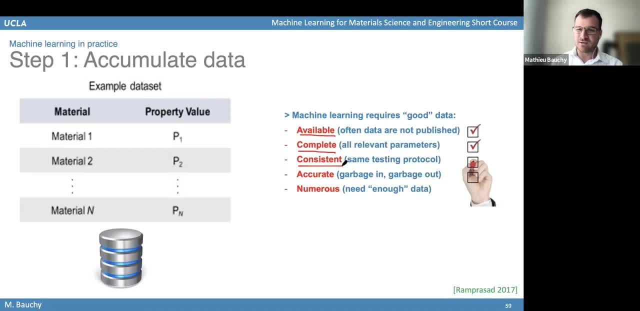 If the priority that is measured is going to be different based on who is measuring this data, then that's going to be very difficult. It's going to be very difficult to find a universal pattern. So when you gather data, you need to make sure that they are as consistent as possible. 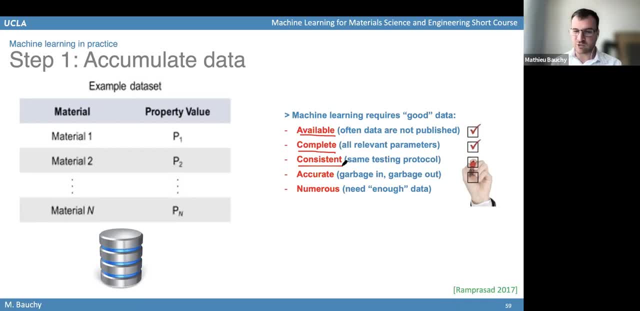 The best way, of course, is if you just generate all of those data yourself, then that way you know it's exactly, fully consistent. But sometimes we cannot generate enough data just ourselves, so we need to gather data from other groups as well. 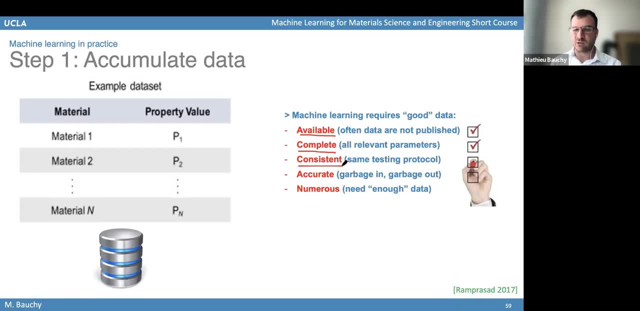 But in that case we really need to make sure that those data are as comparable as possible, That they are tested using the same protocol, the same type of equipment, the same condition. Otherwise that might be very difficult to merge data that are not consistent with each other into the same data set. 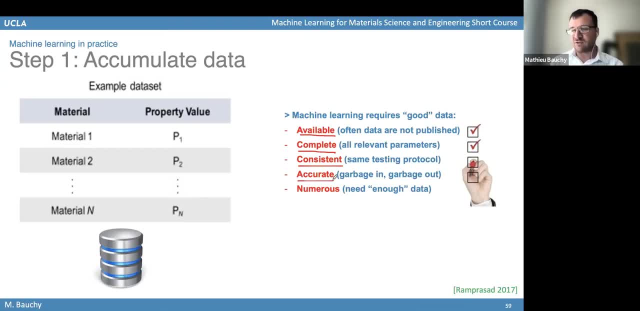 The next thing is that the data needs to be accurate. So, of course, since everything in machine learning relies on data, if you use data that are not accurate, like the data that have been measured improperly, or if there is some kind of mistake, 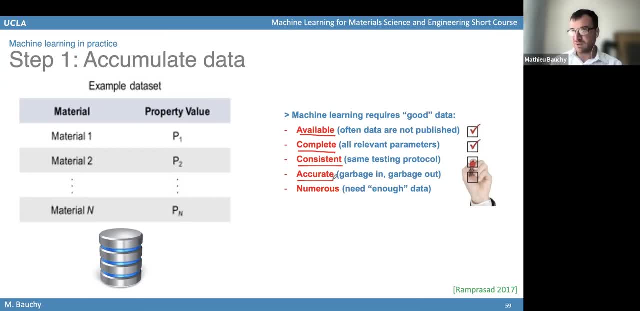 sometimes a typo in the data, then that's going to be an issue. So there will probably always be some inaccuracy in the data, Like no data can be perfectly measured, So that's fine. That's something that machine learning algorithm can deal with. 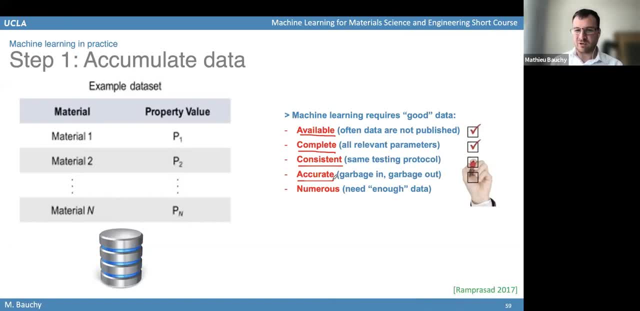 And sometimes there will be typos. There might be some outliers, So it's OK as long as the fraction of those outliers is very small. But if you have a lot of variation, very noisy data, a lot of outliers, a lot of experimental mistake, then the machine learning. 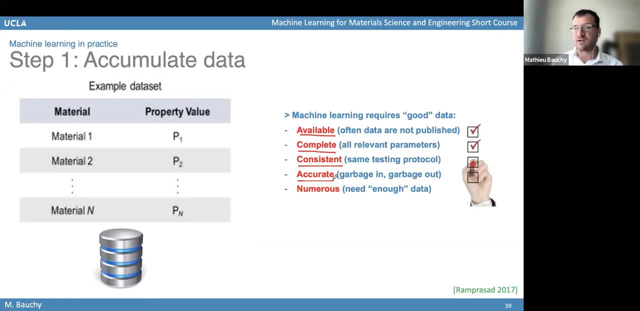 model will learn from those mistakes as well, since it only learns from the data. If the data themselves are not accurate, then the model will also learn something that is not accurate. So you need to make sure that the data are as accurate as possible. 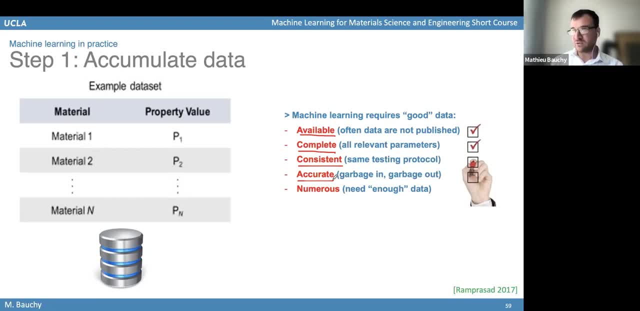 And sometimes this requires some experience to figure out if this data appears to make sense or not. All we need to do is make sure that the data is accurate, So we can also use some algorithm to clean data to remove outliers. So that's something we will talk about in the next few steps. 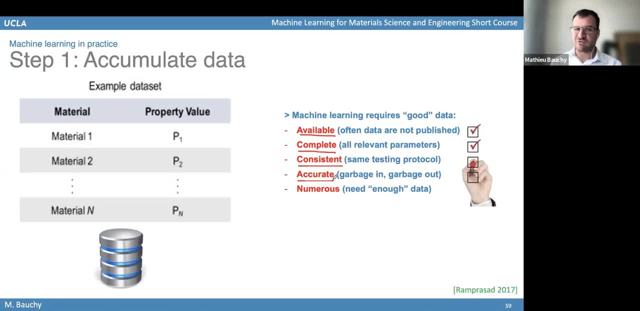 So that's something like: if you don't have a good intuition of what is a good data point and what is a bad data point, then there are some techniques to identify outliers using unsupervised machine learning, And the last thing is that data that I said that you need to use. 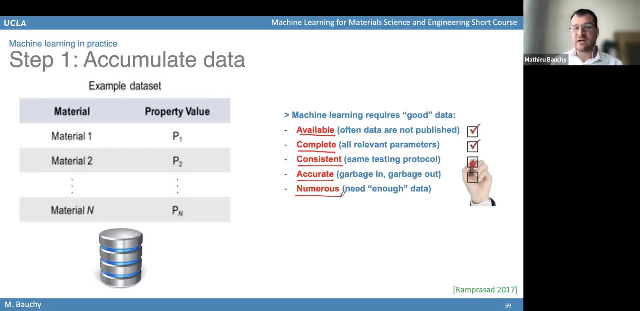 they need to be as big as possible. So that's a key aspect that we haven't really talked about. But for machine learning to work, you need to have as much data as possible, So there is not like a magic number of data points. 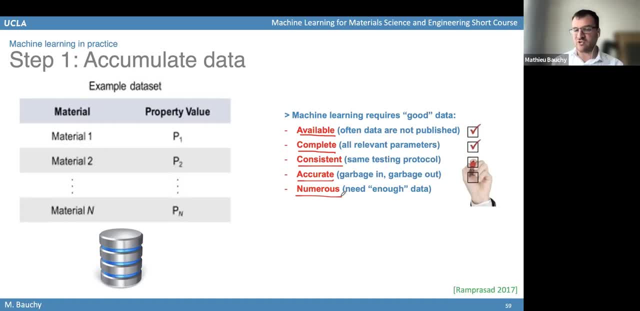 that will be like: OK, if you exceed this magic number then you can use machine learning, And below this magic number you cannot use machine learning. So there is no clear magic number, But for sure you need to have as much data. 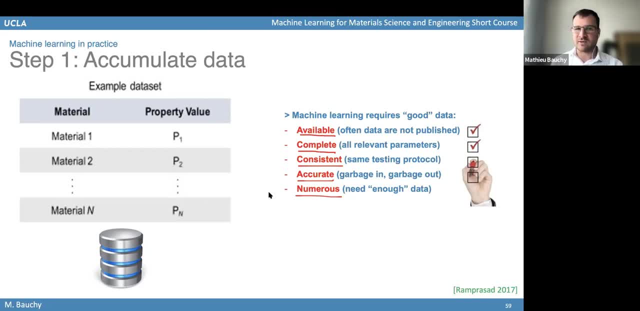 as possible. The more data you have, the more accurate your machine learning model is going to be. So if you are going to solve a problem using machine learning, then you need to make sure you have as much data as possible. The number of data points that you need. 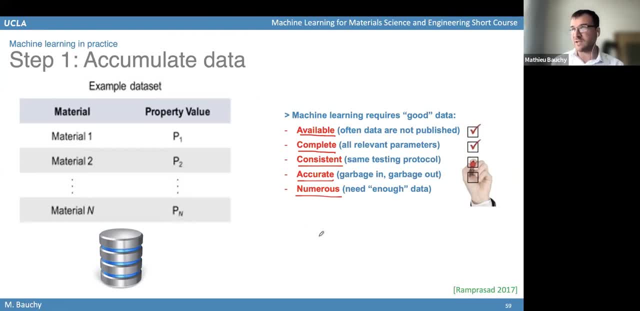 it really depends on the problem that you are trying to solve. For example, it depends on mainly two things. It depends on first: How many variables do you have? For example, if you're trying to train a machine learning model, where you have a material and there 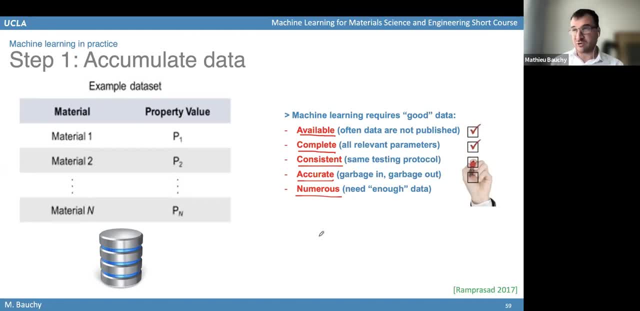 is only two or three parameters that can change in this material. For example, you can change the temperature according to which this material is prepared, You can change the pressure, And that's it. Those are the only two parameters, And then, based on those two parameters, 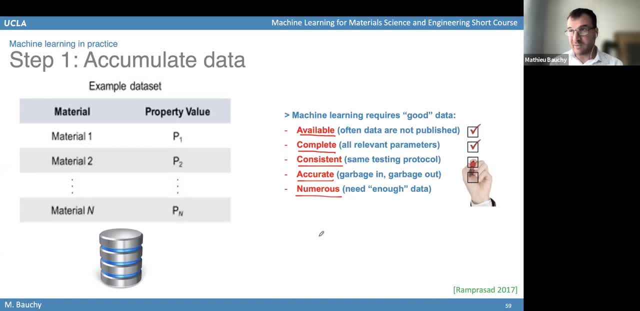 the priority of the material is going to change. If you have only two parameters, then having just maybe something as low as 20 data points might be enough to start training a machine learning model, because the number of variables is very low, So it's OK to have few data points. 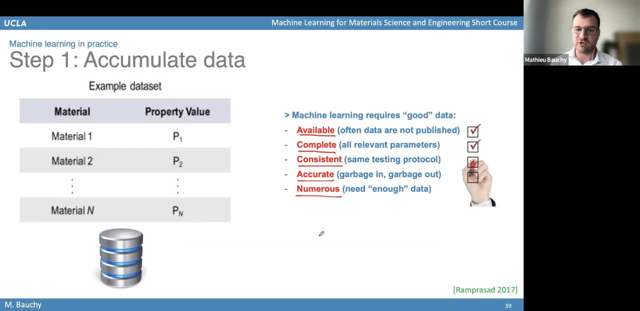 And the machine learning model will still be able to find a relationship between the parameters like temperature, pressure and the priority. Typically- I would say ideally- you need at least six data points per dimension. Per dimension I mean per parameter that can change. 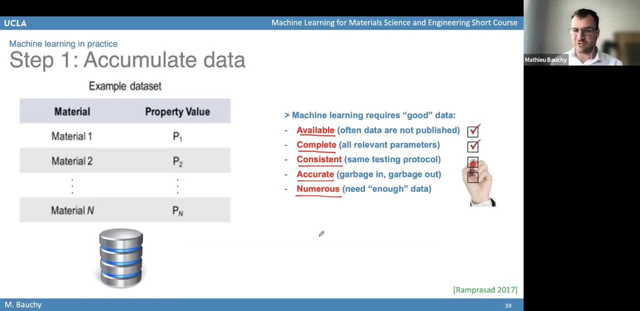 If the priority of the material can change as a function of temperature, as a function of pressure, as a function of how much of a certain element it contains, as a function of the annealing time or as a function of the irradiation time. 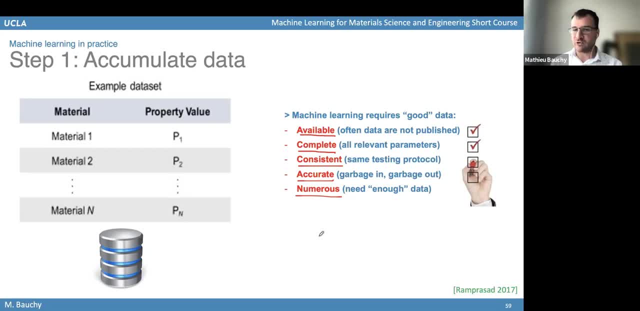 So those are all parameters, And the more parameters you have, the more data points you need in return to be able to train a machine learning algorithm. So ideally, every time you have one parameter you need to have at least, I would say. 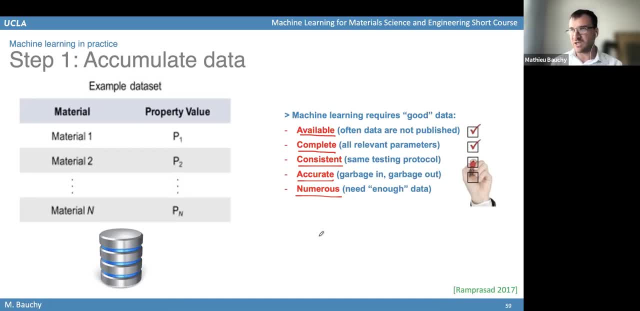 six data points with different values for this parameter. So the more parameters you have, you will need more and more data points in return for the model to be able to find a pattern between the variable, the input variable, the design parameter and the corresponding material priority. 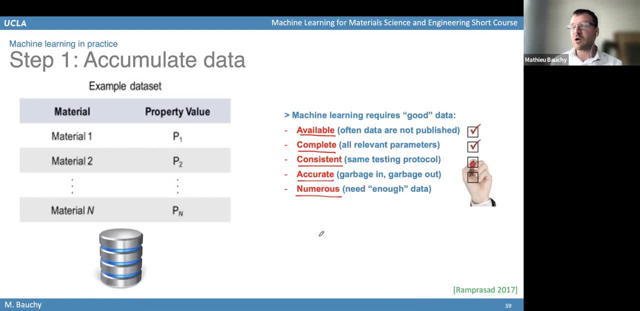 Another aspect also that can play a role is how complex is the relationship between the parameters of your material and the priority. If, for example, you are trying to predict the density of a material as a function of its composition, then very often this type of relationship is very simple. 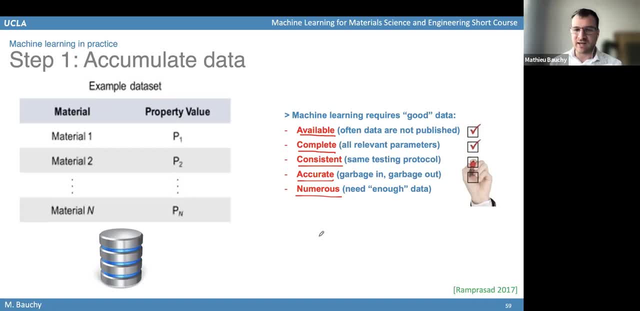 Like usually, the density is going to change linearly with the composition, the chemical composition of the material. So since it's going to be a very simple linear relationship, it might be enough to just have a few data points. That's going to be enough to train your model. 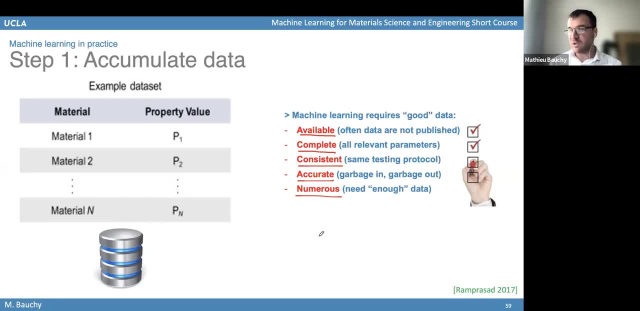 because it's a very simple linear relationship. But if you have a very complex relationship where you have a given input x and then the way this input x is affecting the variable y is very complex, like a very complex relationship like this. that is non-monotonic. 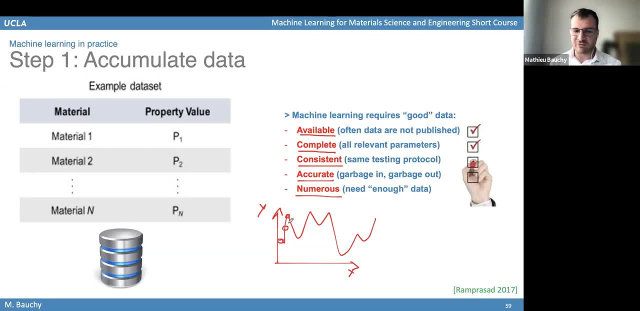 then you will need probably a lot more data points in order for the machine learning model to be able to learn this relationship. If you have just a few data points, like one data point here, one data point here and one data point here, 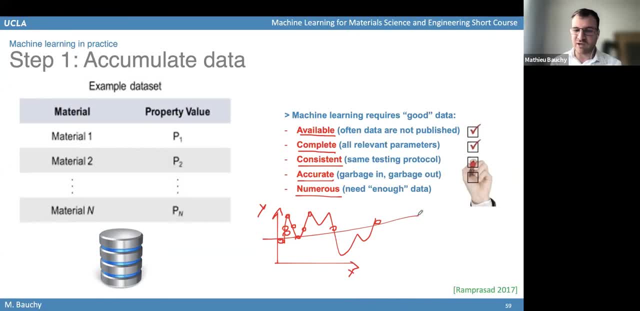 then your model will think that it just should be a linear relationship. Your model will not be able to guess some complex relationship if it doesn't have enough data points to be able to be exposed to the complexity of the relationship between the parameters of your material and its properties. 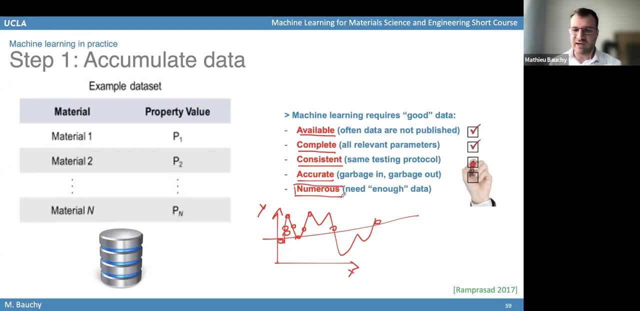 So a very important aspect is to have as much data as possible, to have a data set that is large enough to really be able for the model to learn the complexity of the relationship between the input and the output. Do you have any questions regarding this so far? 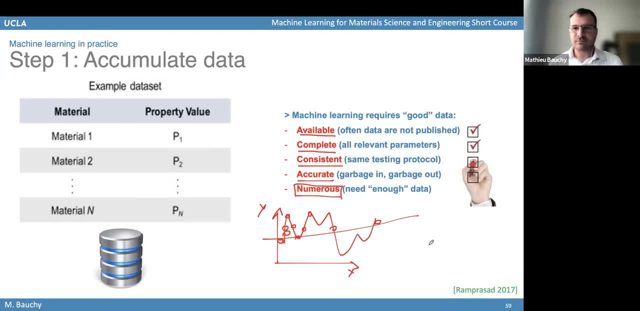 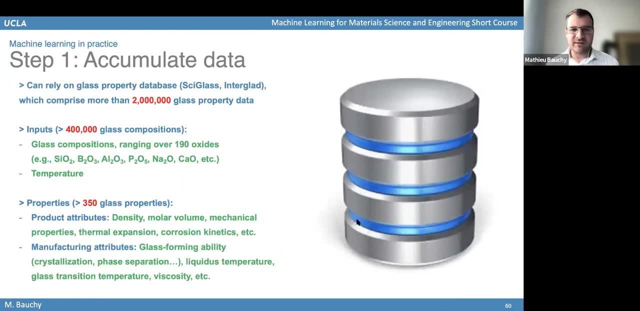 Yes, OK, So let's continue. So when you accumulate data. so again, like something that is, if possible, depending on the types of material that you are using, there might already be some data sets that are already available where people have already. 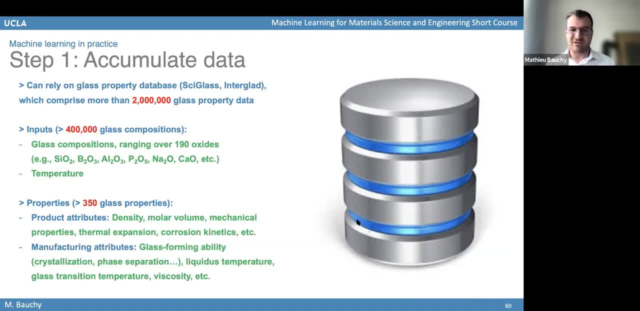 spent some time and some effort compiling data from different sources And group them together into some database. So, especially since machine learning is becoming more popular every day, it's very likely that there exists such data sets already for the material that you're interested in. 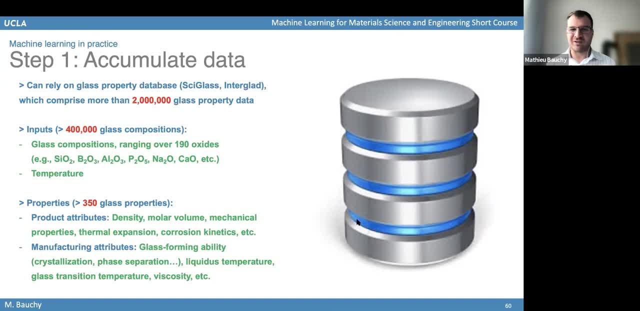 So this is here one example. In the case of glasses, there are some data sets that contain a large number of glasses, together with their properties. So, but like even for other types of glasses, there are some data sets that contain a large number of glasses. 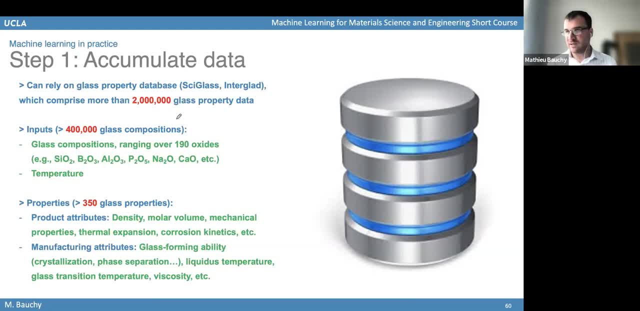 together with their properties. So, for example, if you have, for example, a pair of glasses with different types of materials, whether it's semiconductors, whether it's, like I don't know, types of polymers, things like that- 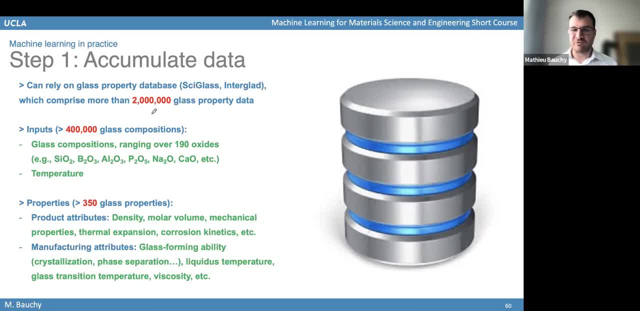 there exists already some data sets that will contain large number of data, for which you would have, for example, different semiconductors with different their corresponding band gap, for example. So you should try to take advantage of those database, the data sets that are already being populated by people. 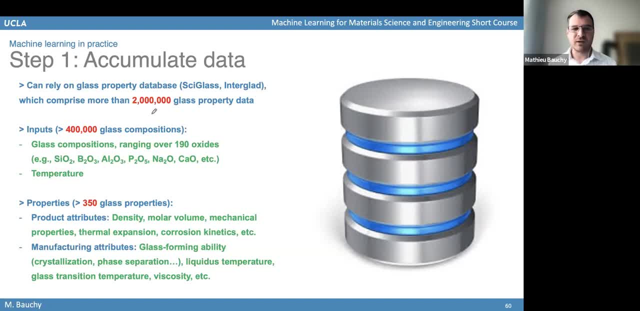 that the data have already been cleaned. So the data are pretty consistent, pretty accurate. So it's good to use those data sets when they exist, But sometimes for material that are a bit less studied or more exotic or more news, those data sets 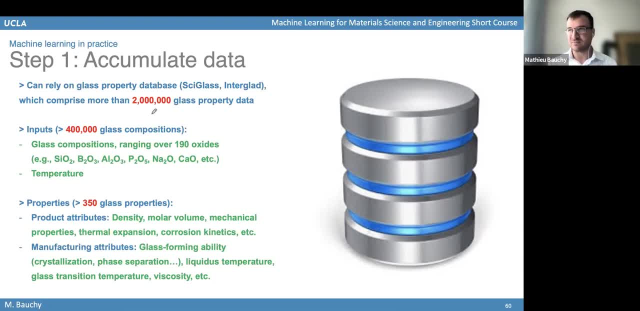 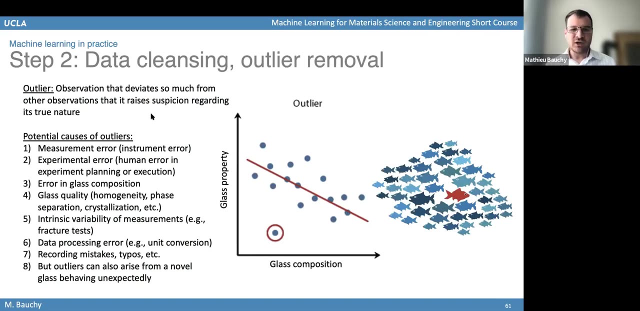 might not be available yet, So in that case you would need to create yourself the data set by compiling different publication or by doing the same thing yourself. Then step two is: once you have the data set, then you need to make sure that the data points that you have. 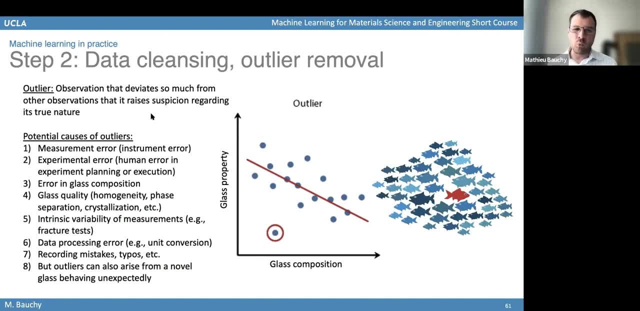 in this data set need to be accurate, And so one problem that can really affect the quality of machine learning is when you have an outlier like this, For example, like here. this is an example where you have glasses with different composition and you measure the corresponding property. 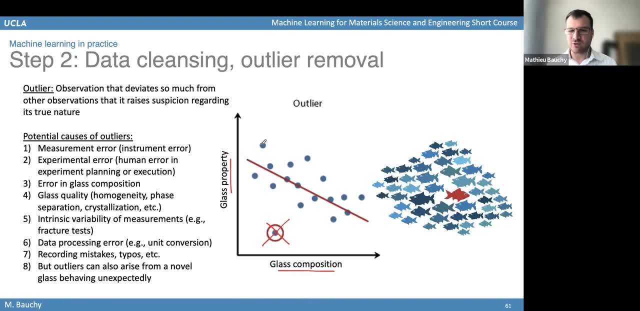 of the glass. And so here, when you do that, you realize that most of the glasses are following one trend. But then here there is one data point that is completely different from the other. So if you have something like this, it means that either here there, 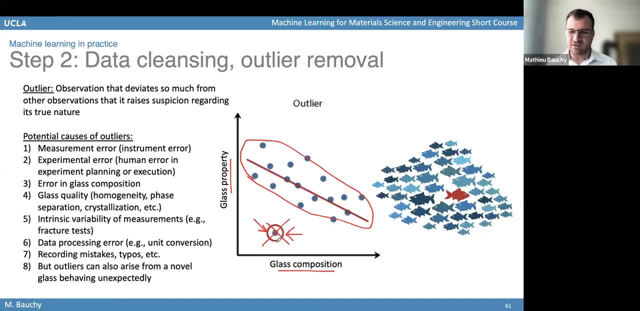 was a mistake, like either a mistake in the glass composition, that maybe this glass actually had a composition like this and it should be here. OK, OK, Yeah, or maybe the completion is correct, but it's more like the property, that that should be much higher. 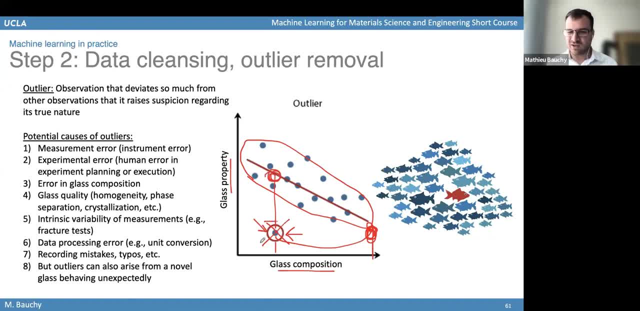 it was not properly measured, or maybe there is something, uh, very special about this glass that makes it have a different property, but we don't really know what. maybe the temperature was different during the measurement, or maybe this class, this glass, was not properly annealed, or there was something broken in this glass. so it's, it's. it's hard to say sometimes, but like sometimes. 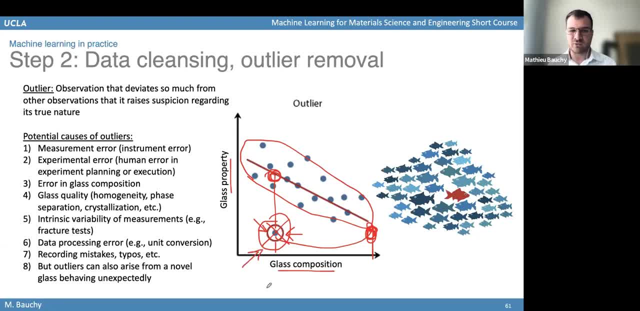 you will get those outliers. you will always get some outliers when you do some experiments, like sometimes something can go wrong. so in that case, either this is a real point that can be very interesting, because it's a metal that behave very differently from all the other, but it's also 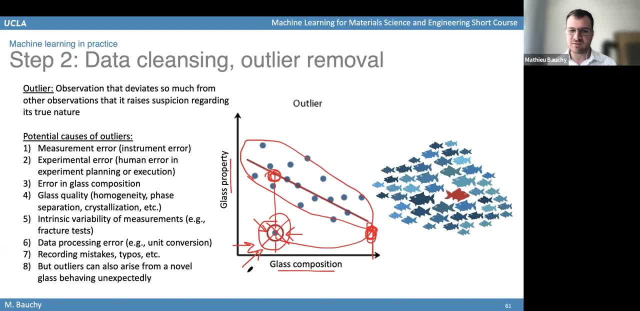 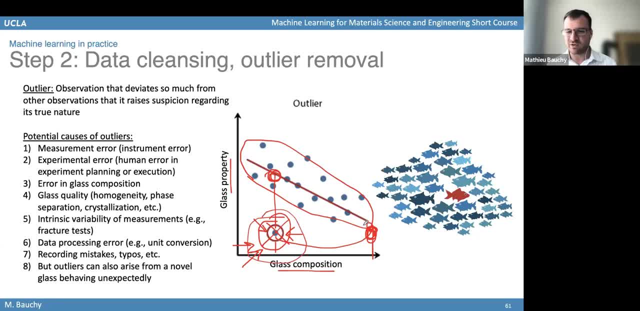 and what you're doing, and what you're doing, and what you're doing and what to do with this point, it it will, it will not be able to understand the true relationship between the, the glass composition and the glass priority, for example. so you would need to remove outlier. if, if, if, those are true outliers. 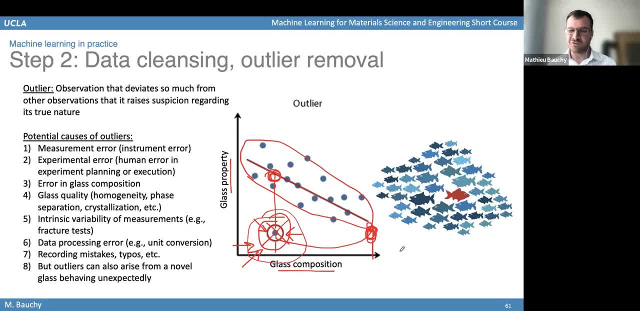 if they correspond to an experimental mistake or if um, if if it's something that you cannot really understand, or it's a, it's um, if it's something that went wrong in the synthesis of the material. so for this the the question is: how can we recognize outliers like you? you cannot necessarily, if sometimes you would have. 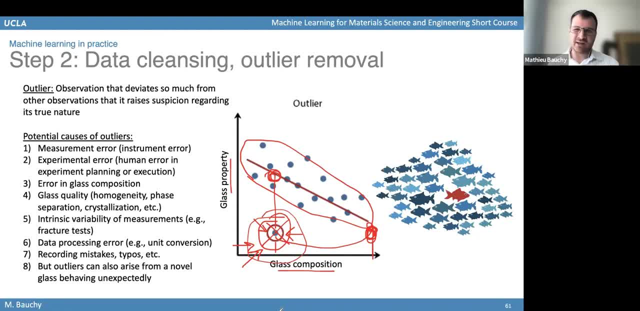 millions of data points in your asset so you cannot look at them one by one and decide if you think those are outliers or not, like in this case on this plot. it's pretty easy because there is only one input and in that case it's easy to just see what seems to behave as an outlier. 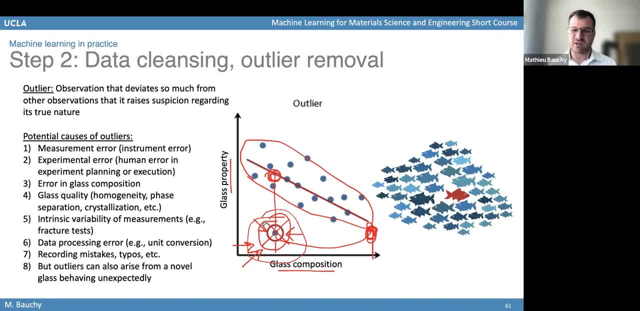 but when you have many dimensions and millions of data points, then it's almost impossible to look at them one by one. so you need, in that case, some other techniques that you can use to identify outliers, or at least to flag outliers. and once you have flagged outliers, then you can. 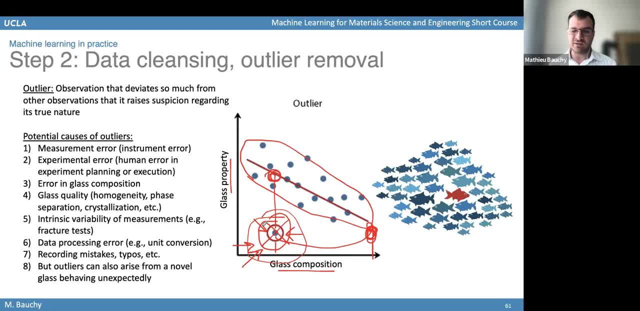 look at it more carefully to decide yourself if you think this is a legitimate point or if it's really a suspicious point that needs to be, for which you need to redo the experiments, for example. so the way i would define outlier is like this: it's an observation that deviates so much from the other observation that it raises suspicion. 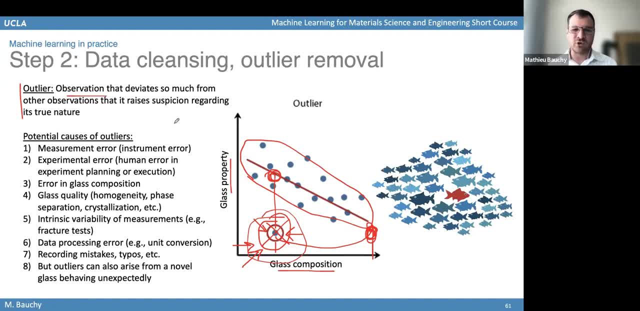 regarding the the true nature of these data points. so again, like when you do experiments, you always get some fluctuations. so like, for example, like here you you will get some noise. anytime you do an experiment, there is an uncertainty associated to this experiment. so it's okay to have some deviation between data points, but when this deviation is so large, 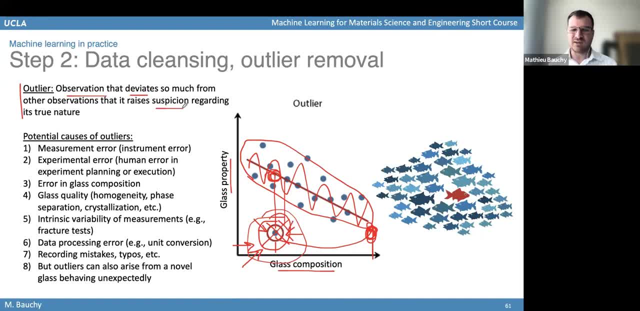 that you, that you that it really becomes suspicious that that something went wrong, then it's. it's that would be the case of an outlier. it's a point that is so far away from the other point that you can be very suspicious that something might have gone wrong with these. 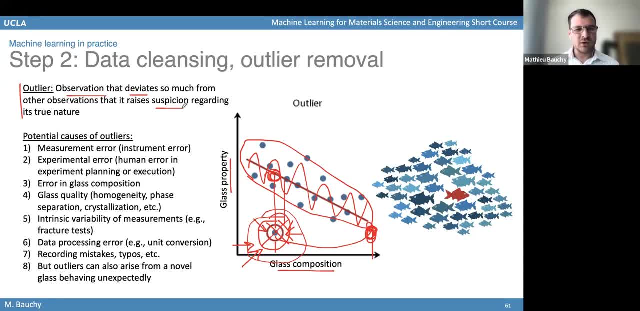 data points, so in that case it needs to be checked or removed. so the different thing that can cause outliers, so that could be like an experimental error, like maybe, uh, there was a mistake in the of the, the equipment or something like that. so it can be an error like, uh, during the, maybe the 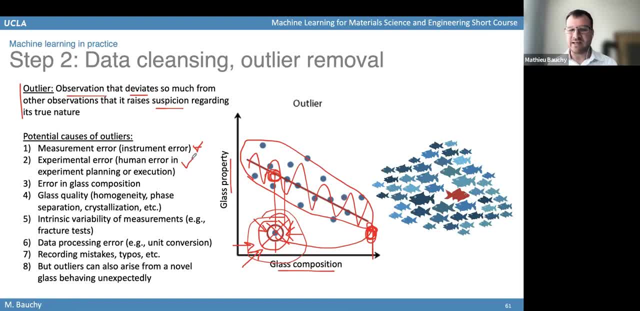 synthesis of the material, or, like the, the planning of the experiment, or the. uh like the, the the human execution of the material was not conducted properly, so that can be another thing. uh, like the. the composition of the material might not be the the one you think so there. 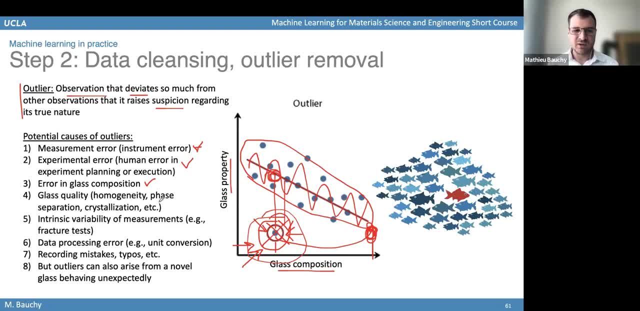 might be some impurities in your material, something like that. there can be some, uh, some issue like some, uh, your material is not homogeneous, so it can be face separated, partially crystalline, so this can be an issue about the quality of the material, so that that's. 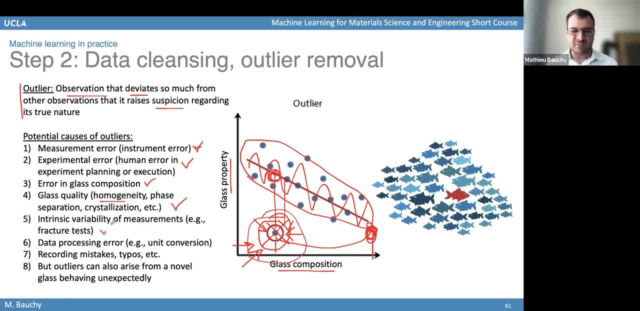 another potential source of error. sometimes there is just some intrinsic. some measurements include some kind of randomness. for example, if you test the fracture of a material, the fracture of glass for example, uh sometimes like you need to do the the same experiment several times and uh take some. 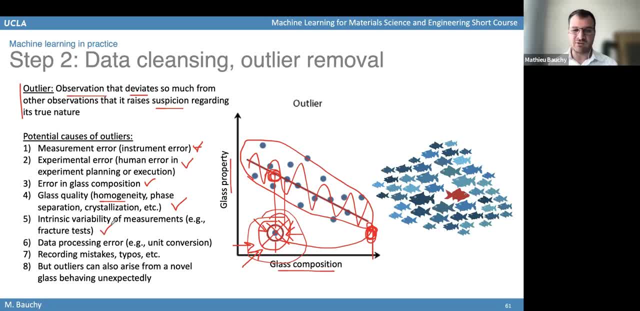 like uh similar uh decades and uh uh average, because each experiment individually might give you a very different answer. because i'm some uh intrinsic variability of the measurement, so if it's very sensitive to small detail of the material, so in that case it might just be like a. 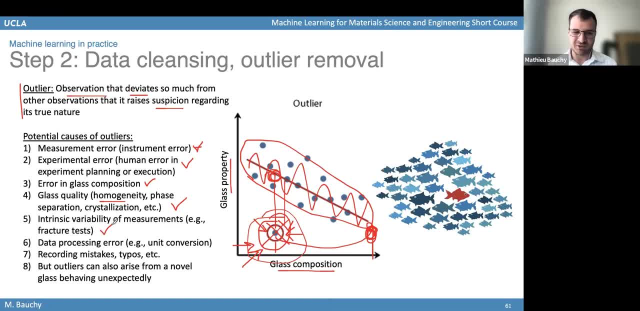 random deviation, uh, due to the variability or the sensitivity of a given measurement. so, uh, of course, another potential mistake is just like a human mistake. for example, if somebody did a in the converting one unit to another or something like that, so that would be like a mistake from the. 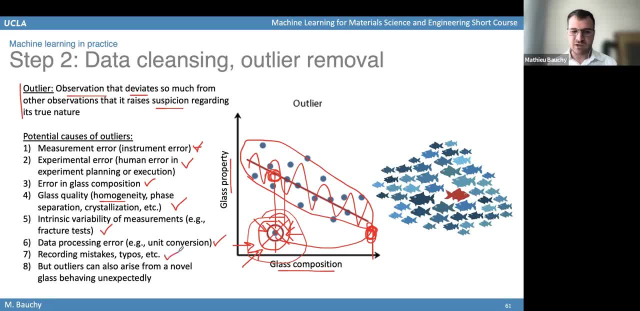 during the processing of the of the data. something that is actually very common is just typos. like you, just if you, if you write a given measurement on a piece of paper and then somebody else will read the number but cannot exactly see the based on the handwriting, will think one figure is another. 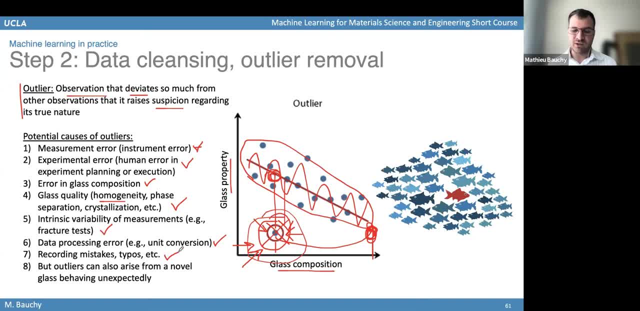 figure something like that, or you enter data on the computer and you forget the point, so you forget the decimal point, so that would be like a typo. so, uh, those mistakes can can always occur. so it's um, something that is going to be part of that. i said there's always going to be a small fraction. 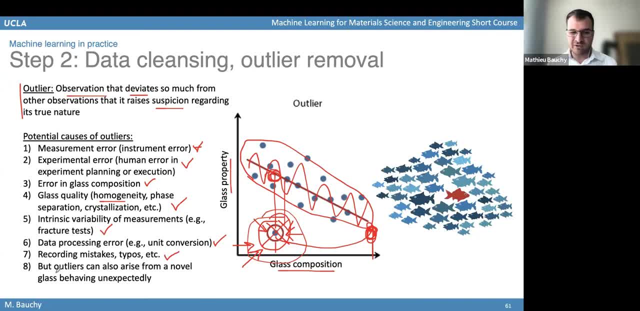 of typos like this: uh, of course, there's also um the possibility that something that looks like an outlier might not actually be an outlier like it. it might be just that there is uh, for example, in the case of a glass, there might be a very special composition for which. 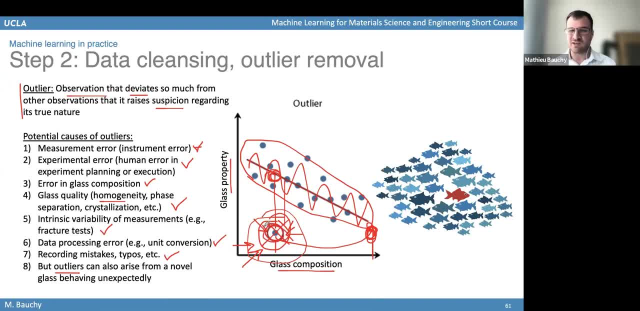 the glass will suddenly behave very differently than if the composition is different. so for this, the only way to make sure of that- whether it's an outlier or actually a very special material- is to, uh, to repeat the experiments, like to do the experiment again and see if it's. 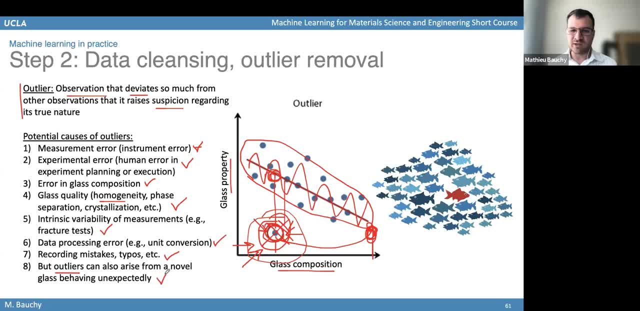 if this measurement is repeatable, if, if you redo it and you you find out that actually the, the, the new measurement, is now in line with the other measurements, then it means that it was probably an experimental error, like some, something like based on those reason one to seven. but if you 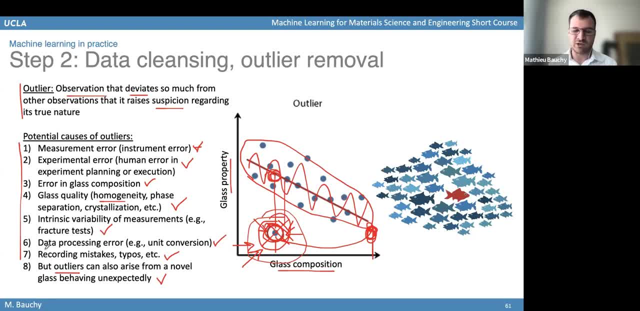 keep getting the same measurement over and over, then it might not be an outlier. it might just be a point, a material that that suddenly have very different properties and something that can happen like there can be some very specific condition where material will perform very differently uh than for all of them. 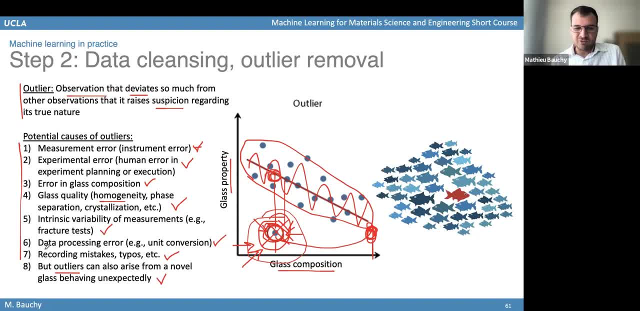 it's very difficult to get a better judgment because that's the same kind of scale that you have in your view of the condition. so sometimes you need to be careful. when you see outliers, you you should not always say, okay, i'm going to delete it. uh, you should really carefully check, like is. 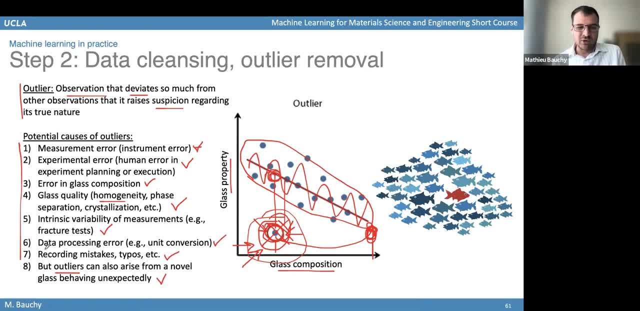 there a good reason that it's an outlier, or can i redo the experiments to confirm to, to really see if if it's a good reason, a good uh uh, if there is a good reason to delete this outlier, or if it's actually something that's check, if it could actually be a very unusual material that that deserves to be kept in the. 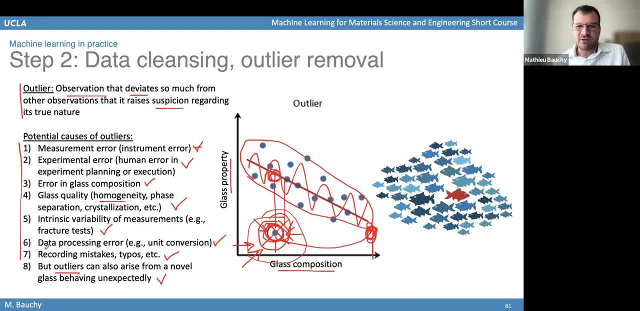 data set. that's step two. that's what we call the, the data cleansing, uh, removing the outliers. so now the question is: how do you do that in practice? how do you detect which data point is an outlier and which outlier, which data point is not an outlier? so for this we need to use unsupervised 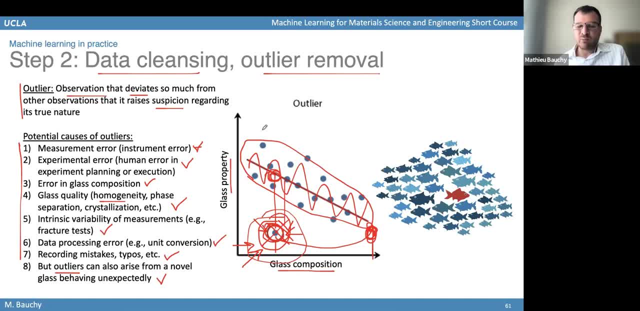 machine learning, because we don't know, we don't have some example of data that are outliers or data that are not outliers. we, we, we don't have any label for that. we just have some data points. some of them are going to be different than others. those are the one that we want to to flag as. 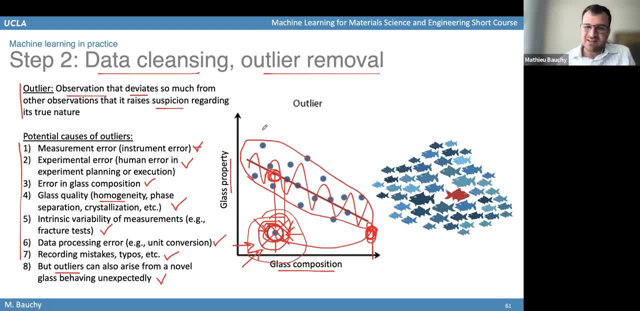 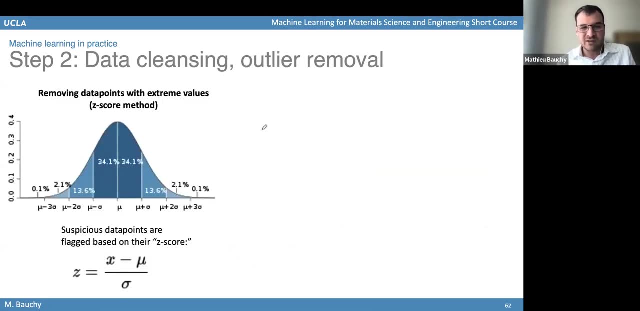 outlier, but we don't have previous example of data points that are outliers and previous data points of uh that are not outliers. so we need to do, since we don't have any label, we need to use unsupervised machine learning for this. so uh first. so we'll see here different methods. some are very simple, some are more. 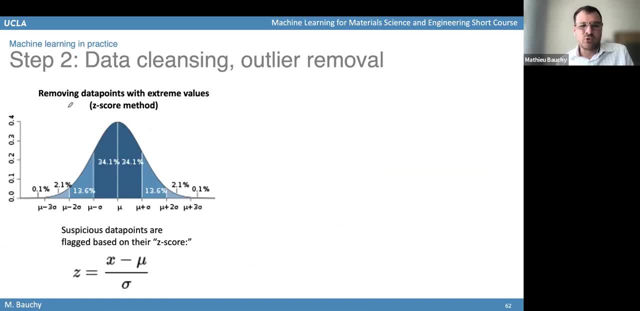 complex. a first common method to remove outlier is to just look at, um, how far those data points are from the average. so that's a very simple method, but typically that's not a very good idea to use that. uh because, um, it's not necessarily because the data point is far from its average. 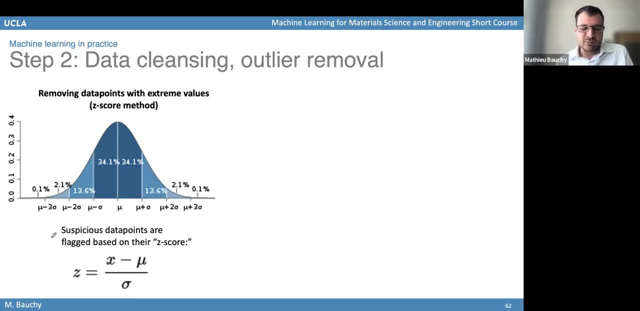 value that it's necessarily an outlier, but still, in some cases this method can at least help you to to quickly identify points that are more suspicious than other. so here the idea, for example, is that you have some data points and um, so those correspond to different materials, and for those, 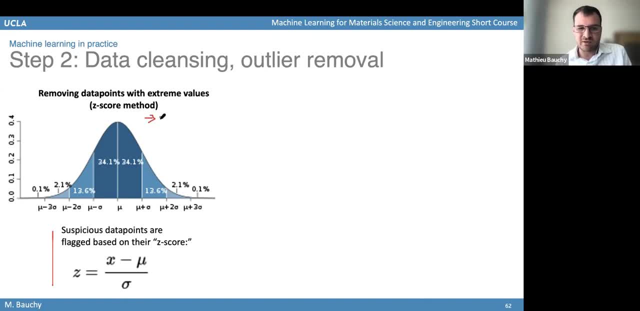 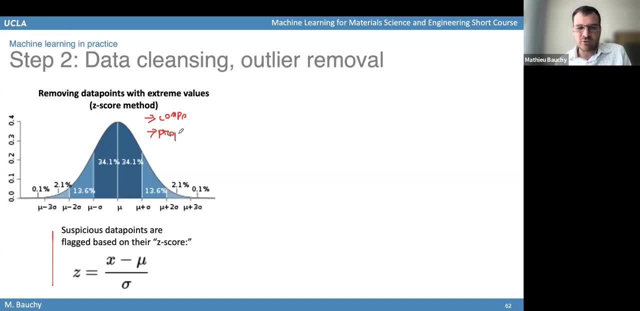 you have different, different uh thing that can either be an input or an output for your machine learning model, then what you can do is to look at all those features of the materials, all of those features like its composition etc. or the property that are measured, and you can calculate the average of those uh, of those features, over the 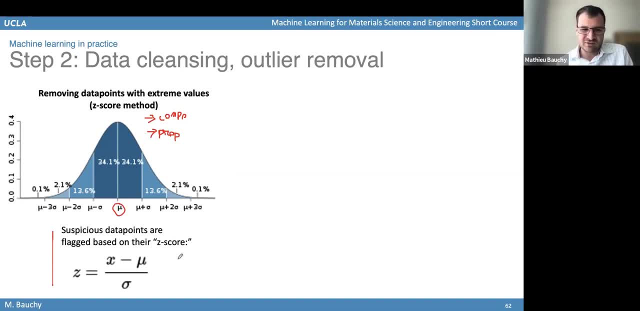 entire data set that you have. so you take all the material that you have and you calculate the average composition or the average property. so that's going to give you the average mu. so this is the average, the average value of this property over the entire data set. 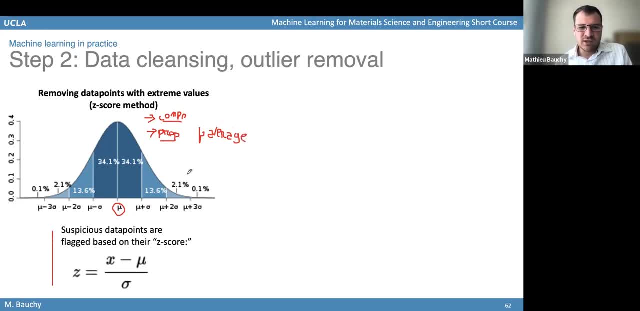 that you have. then the second thing that you can do is to calculate now sigma, the, the standard deviation. so this you calculate like: what is the average deviation of the points from the average? you calculate the average and the standard deviation and then what you can do is, if you look now at the distribution, 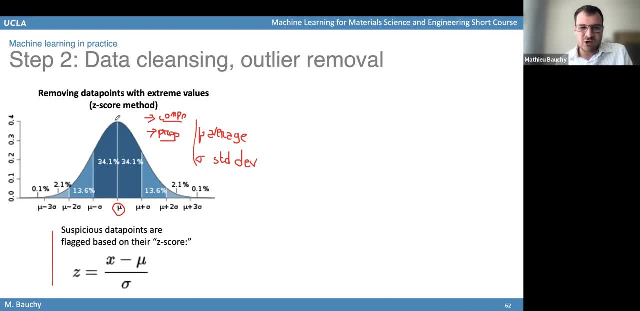 of the data points. so you will have probably a lot of data points that are for which the value of this feature is close to the average, and then as you go further away from the average, then you should have a less and less data point. so this is assuming that your your the feature like follows: 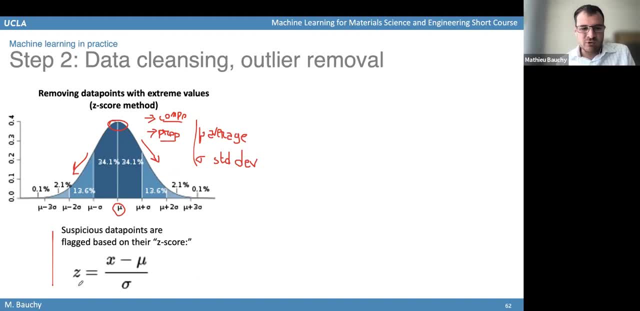 some kind of normal distribution like this, and then what you can do is to calculate, then the z score. so the z score, you would calculate it as you take the value of the, the feature of the material. so you, for a given material, for example, you will calculate its, its composition. so this is the. 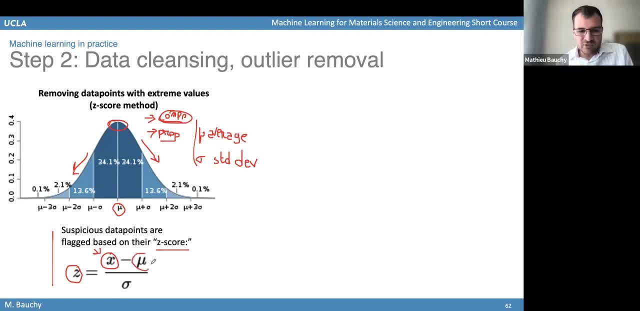 actual composition that was measured. you compare this composition to the average. so when you have x minus mu, this will tell you how far are you from the average. and then you divide this by the standard deviation, so this will tell you then a z score that tells you that for a given material you are one standard deviation away from. 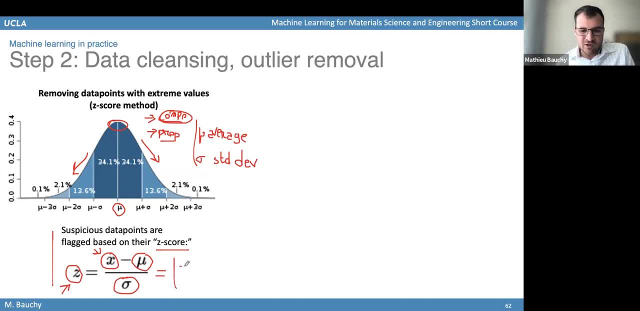 the average. so this is if you have a z score, or of plus one or minus one, for example. so that means that in this case you are one standard deviation away from the average, or you can be. if you are here or here, then you are two standard deviation away from the average, or three standard deviation away from the. 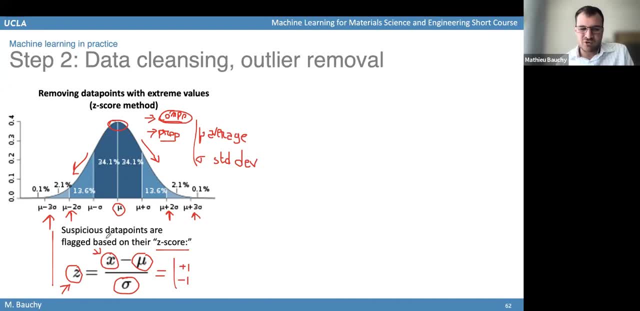 average, and then you can define a threshold. you can say that if i have one data point for which one feature is more than, for example, a free deviation away from the average, then i'm going to consider this point to be very suspicious and i'm going to flag it as an outlier, so that that's. 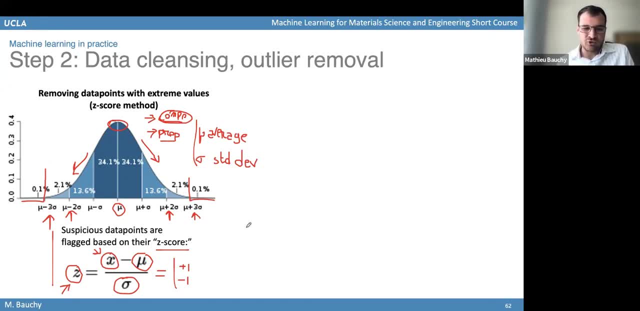 one common way: you look at the value of all the features, you compare the value of all the features and you can see that the value of all the features, you compare it to the, to the average. you check how many standard deviation away from the average is it and if a data point is too far away, it is if it is several standard deviation away from the. 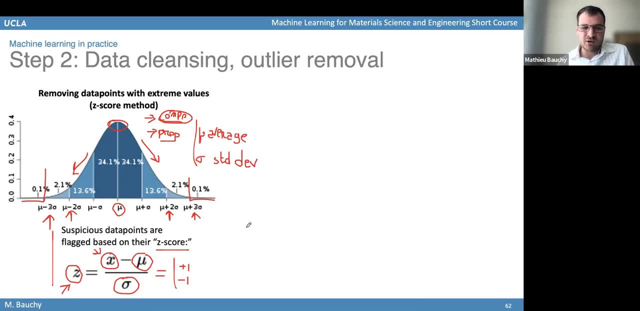 average, then you will either remove it, either carefully look again at these data points to see if something went wrong. so that's the idea of the z score. you calculate this z score to see how many standard deviation away you are from the average, and if it is far from the average then you remove. 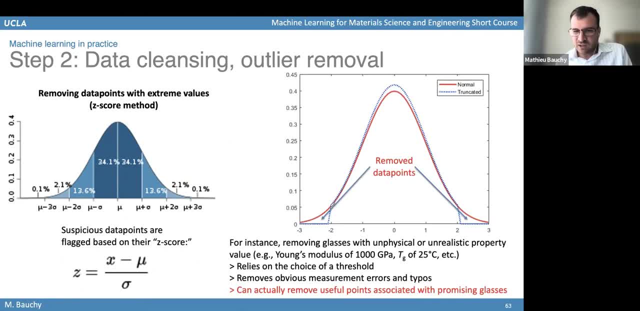 it. so that would be like, for example: in this case, if you take the, the red would be the distribution of the material that you have been measuring, and then if you say, i'm going to remove everything that is more than two standard deviation away from the average, i just remove it because you are too far. 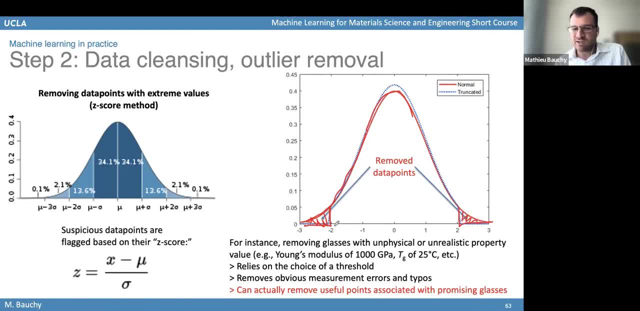 away from the average. it looks suspicious, so i remove it. and then you are left with only the rest of the data point. that would be not more than two standard deviation away from the average. so that's a common way to um clean that asset, but it's not always, uh, necessarily the the best method, because 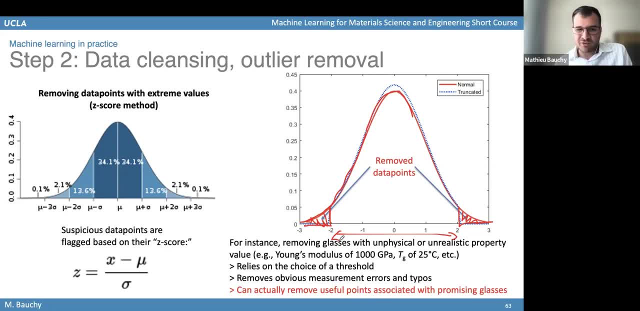 sometimes um, for example. if you are testing materials with different um composition, sometimes you will have a material that has a very different composition, and that's not necessarily a bad thing. it's just going to be a composition that is very different from the average, but it doesn't mean. 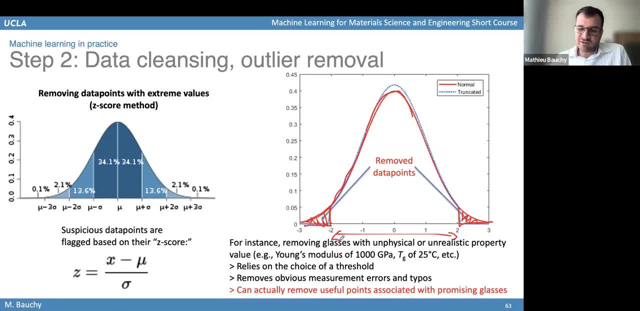 it's an outlier. It might just be that it's a different types of material that you have in your dataset, And in that case you should not remove these data points. So this is a method that can work in some cases, but you need to use it very carefully to avoid. 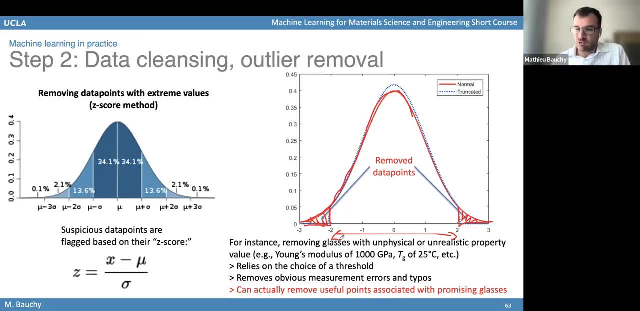 removing that point. that would actually be real data points. So one example for this is like, for example, let's assume that you have a database of different glasses with different composition and you measure their Young's modulus. you've measured their elasticity. So if you really see a very high value, like for example, in the case of glasses, 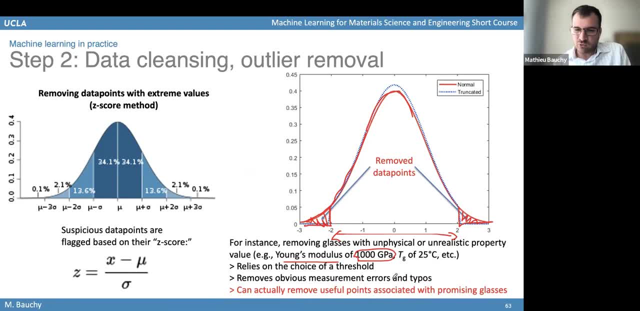 the Young's modulus should be somewhere between 50 to 100 giga Pascal. So if you have something that is really wide, for example a height somewhere between 54 and 400 giga Pascal for this responsibility, so they should measure that exactly And be careful when improvement is made. 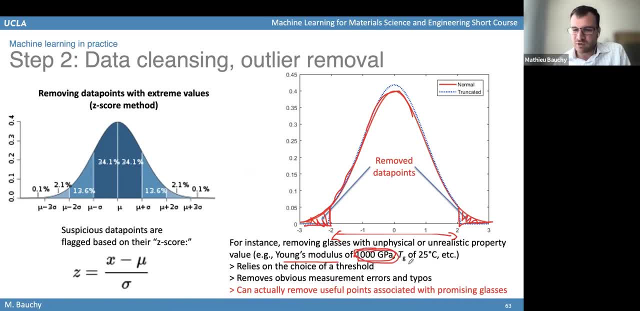 like one order of magnitude larger or smaller. like, for example, you find 1,000 gigapascal as the Young's modulus, then you know it's very unrealistic. Your z-score in this case would be very high because you would be very far from the average. 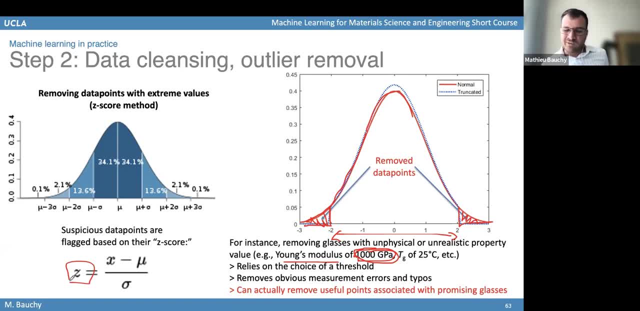 So in that case you can probably assume with a high degree of confidence that something went wrong in the experiments and that you should not have such a large Young's modulus in this case. So by calculating the z-score, at least you can pinpoint those points. 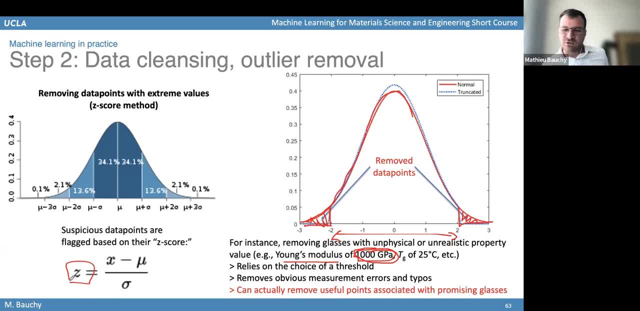 that are really the most that looks the further away from the average And those points. then you can look at them more carefully to see if there is something that looks really suspicious. So the one drawback of this method is that you still have to choose. 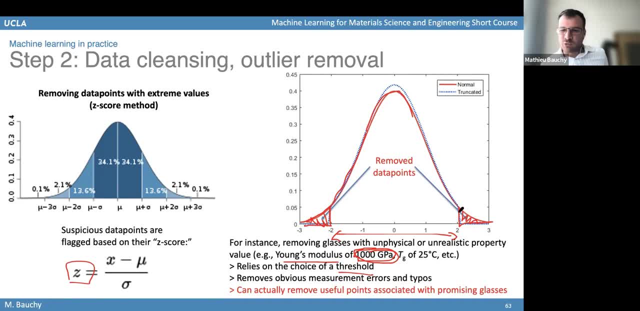 what is gonna be the threshold Like? if you decide- I'm gonna remove the point- that are more than Tucson aviation away from the average, or maybe you're going to decide to remove the point that are more than three sun aviation away from the average? 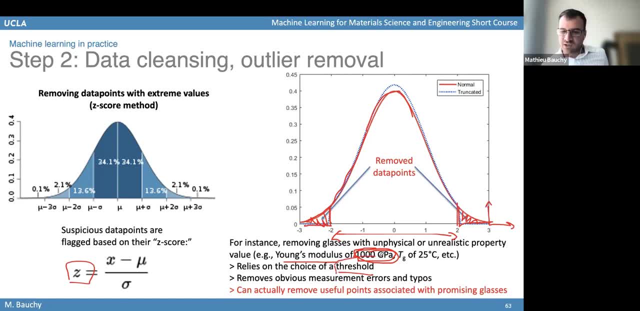 So you need to decide of a threshold here, and there's not necessarily a good choice on which threshold to use, So this depends on your intuition. This depends on what type of priority you are measuring, So this depends on how noisy the experiments are. 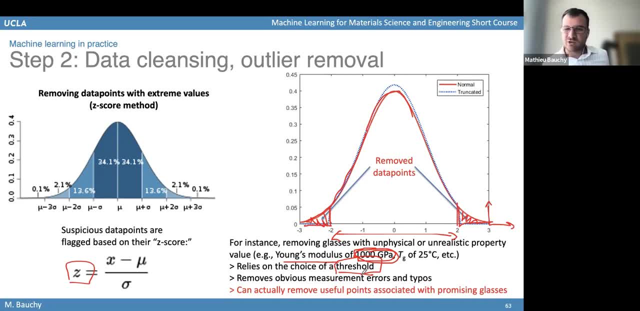 So you need to choose the threshold based on your intuition of what is a reasonable and what is an unreasonable value for each of the priorities that you are considering. So the advantage of this is that it's gonna remove, like, the very obvious error, Like if you have something that is 10 times too large. 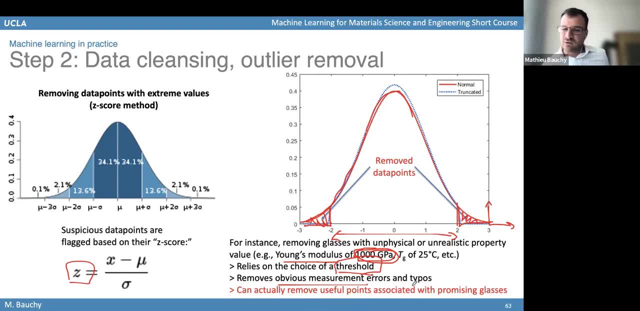 or 10 times too small, then it's gonna be like removed because it's gonna be a very obvious difference with the rest of the data points. But again, like it's also possible that this method can remove point that are actually real points. 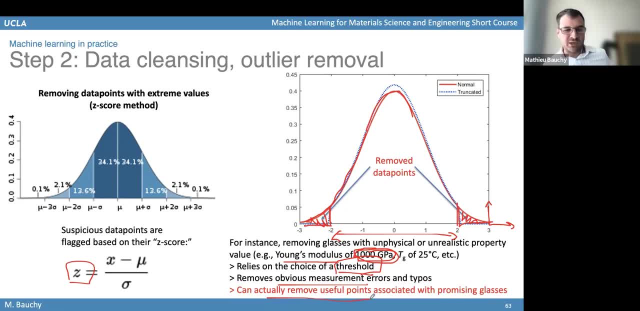 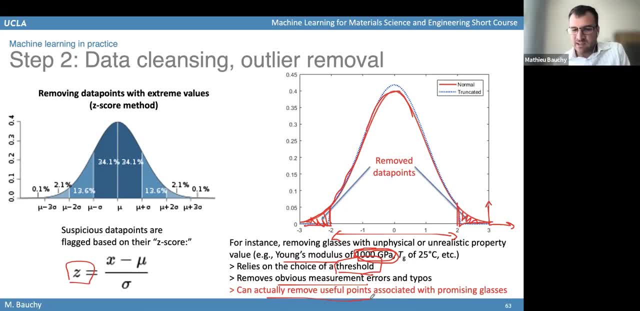 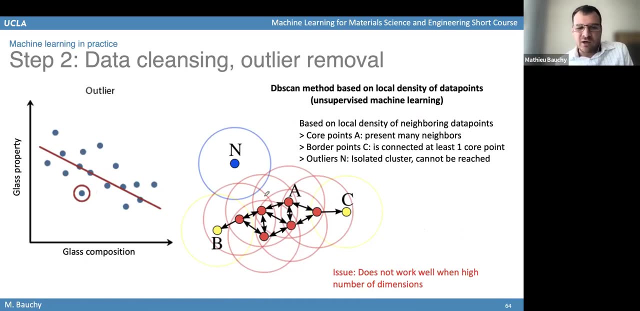 to avoid removing points that are actually legitimate data points. So this is like the most simple method, but in practice, like there are some better methods that you can use for data cleansing, So let's talk about this. Another method that is better is to use the dbScan method. 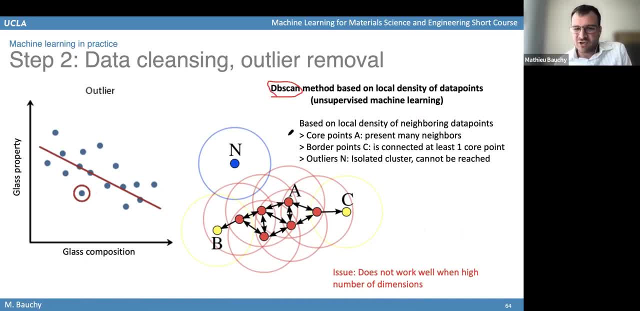 So that's an unsupervised machine learning method that is used to identify data points that are behaving differently from the others, And in this case the idea is to look at the local density of data points. So the idea is as follow in this case, 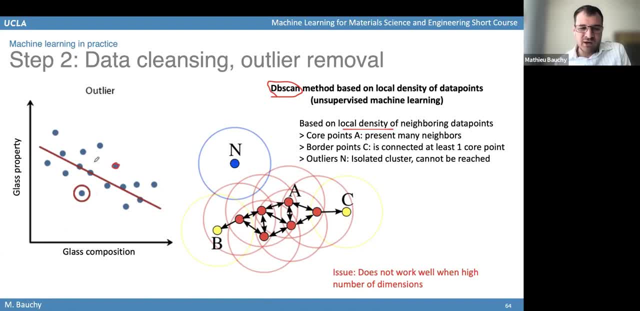 is that if you have a data point here, what you will do is to look around this data point. So you will take a sphere around this data point and you will check: do I have some neighbors? Do I have some other data points that are neighbors of these data points? 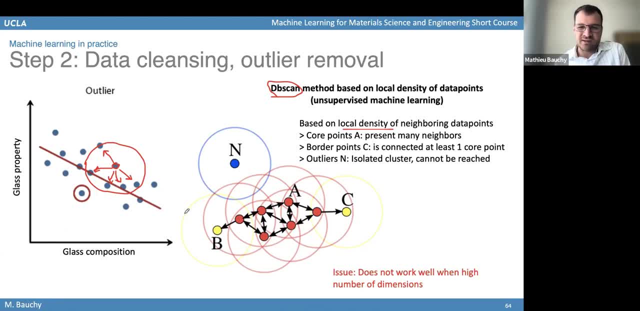 Do I have what is the local density of neighbors around this data point? And then, if you do that, you can classify data point into three categories. For example, if you take this data point here, you take a sphere around this data point. 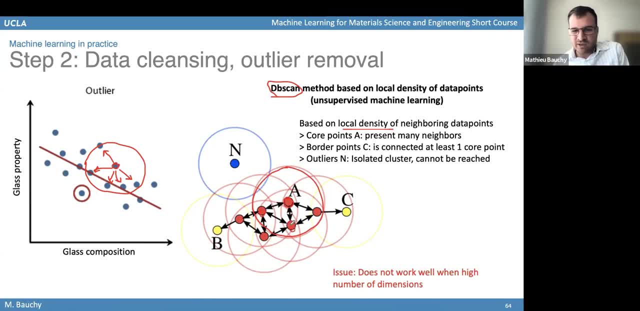 Here you find that it has three neighbors. So that's a point that has a high density of neighbors. So that's what you will call a core point. That's a point that has many neighbor And a point that has very a lot of neighbors. 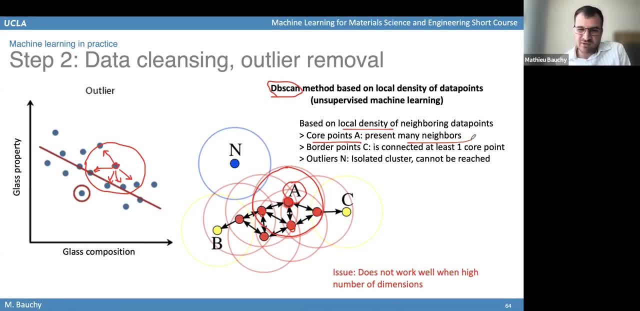 it's a point that you can be really confident about because it has some neighbors. It means that it's a point that behave similarly to all the other points, So it's a point that is unlikely to be an outlier. It's behaving similarly than its neighbors. 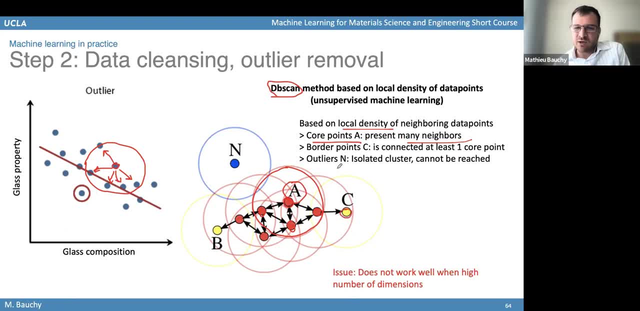 Then sometimes you will find points like this, that are what we call border points. That's a point that when you look, when you look at a sphere, you look at their neighbor. it doesn't have a very high density of neighbor, but it's because it's at the edges. 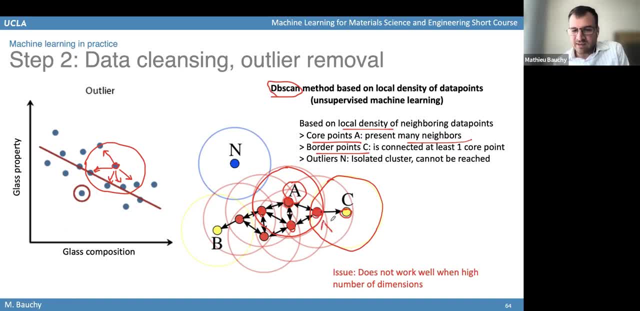 At least it has at least one point, And this point itself is a core point. So if you have one point and it's connected to at least another core point, then you can assume that this point C here, despite the fact that it has only one neighbor. 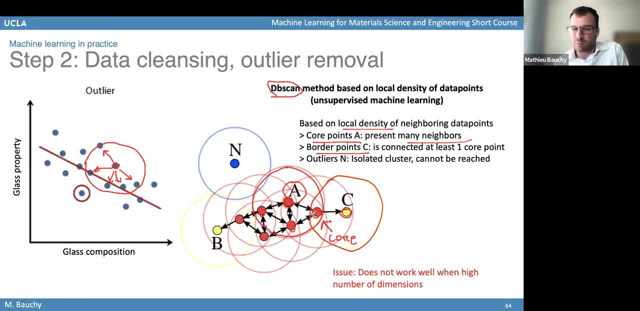 it's still a very reasonable data point connected to another core point, So it means that it's a point that still does not behave differently from its neighbors. But then sometimes you will find points like this where you take the sphere around them, you look at how many neighbors there is. 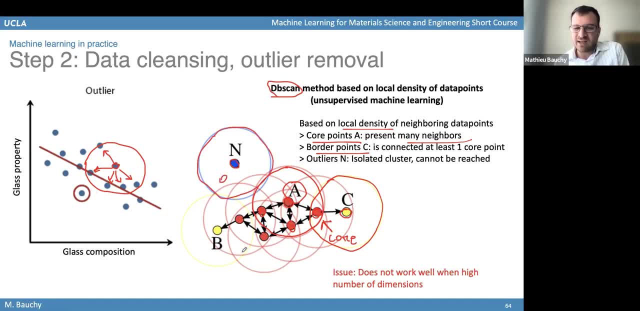 and you find that there would be zero neighbors. It's not connected to any core point. So in that case, that's a point that is very behave, that is isolated from the other data point. That's the point that is very suspicious, because it appears to be disconnected. 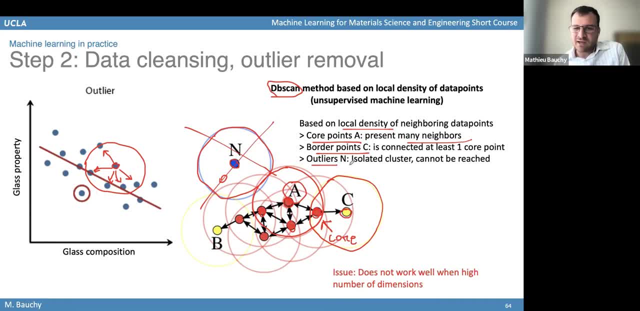 from all the other data points. It's a point that is an outlier. It's an isolated point that is not connected to any other core point. So in that case, that's a point that has a very high chance of being an outlier and that you should confirm. 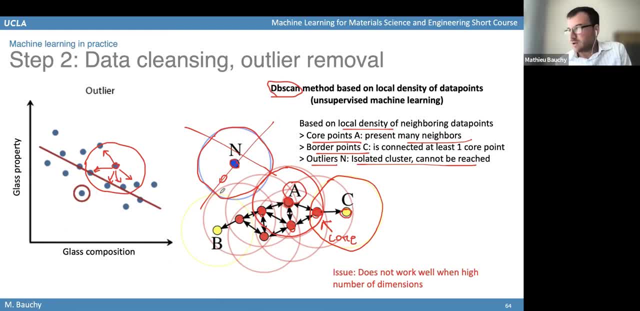 or try to check or redo the experiments for this data point. So that's a pretty powerful way to identify outliers. It's not perfect though, because you could, for example, if you take this plot here, you could very well have, for example, a point here: 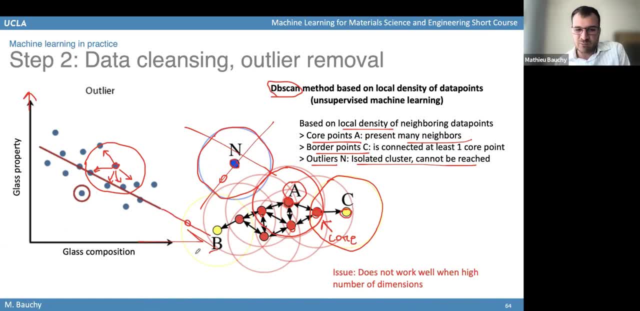 And this point would be pretty reasonable because it's actually on the same trend. But still, when you look around this point you don't find any neighbors, So this point would still be classified as an outlier, despite the fact that actually this point looks pretty good. 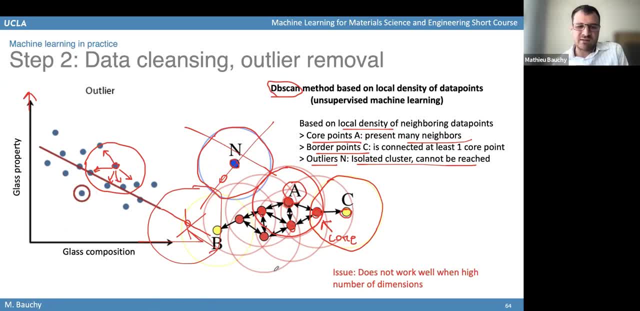 So this method is not perfect, because it can still classify some points as being outlier just because they are far away from the other points, But it doesn't really. it might not necessarily tell you if it's on the same trend or not- A typical case where this method doesn't work very well. 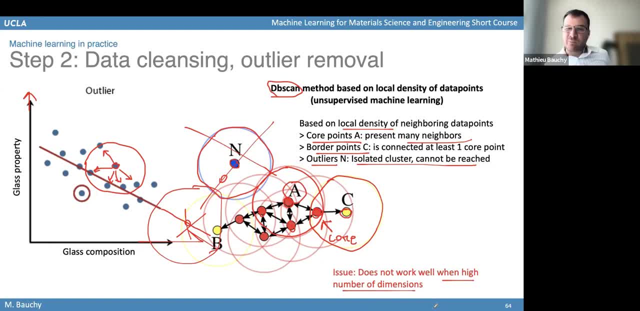 is when you have a very high number of dimensions. So when you have a lot of parameters, like if the composition can change, the temperature can change, the pressure can change, humidity can change, If all of those things can change at the same time. 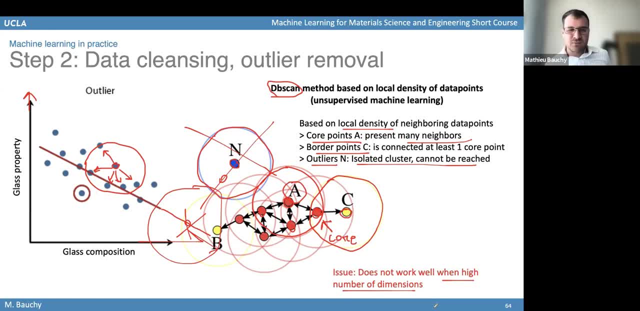 then you have a lot of dimension And in that case it becomes very hard to use this method, because there are so many dimensions that each point appears to be pretty isolated. The more dimension you have, the more the database will look sparse, The more the points will look very far away from each other. 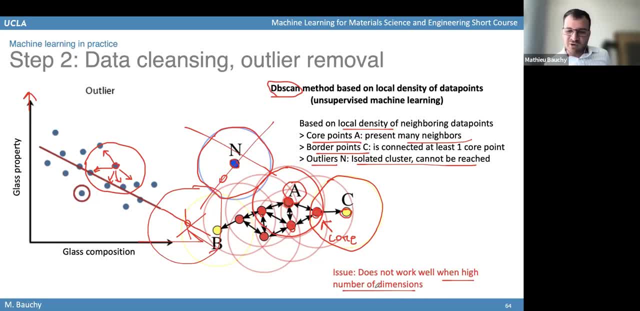 because you have so many dimension. So if you have a very high number of dimension and if you use this dbScan technique, it's possible that really a lot of data points will be classified as outliers just because there is so many dimensions. So that's one drawback. 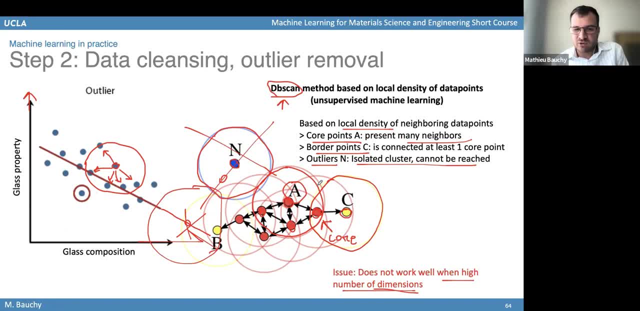 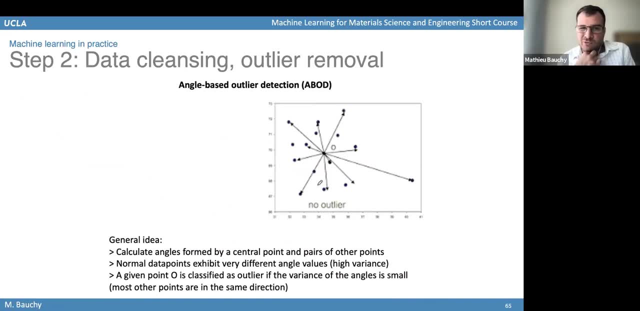 that when you really have a lot of dimension, like the dbScan method, does not work very well. Another method that is probably one of the most powerful method to detect outlier is what we call the angle-based outlier detection or this ABOD technique. 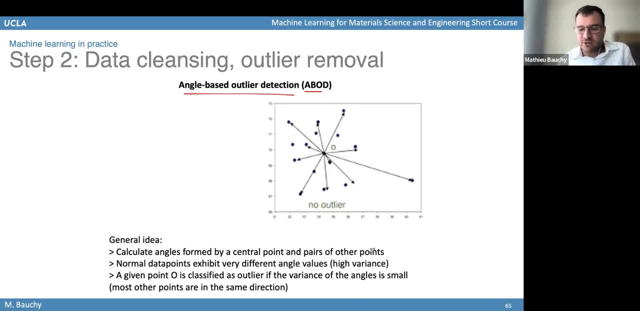 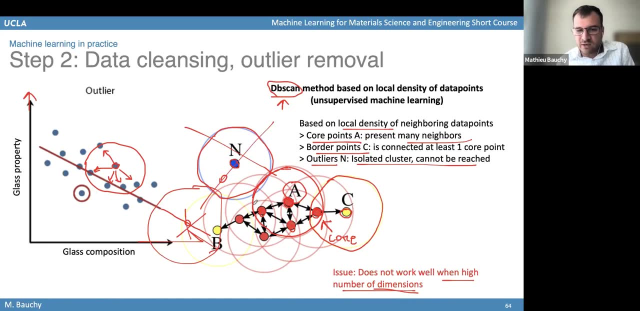 And so here the idea is that rather than looking at the density of the points like, rather than looking here at taking one data point and looking at what is the density of neighbors around this data point- here it's not based on density. 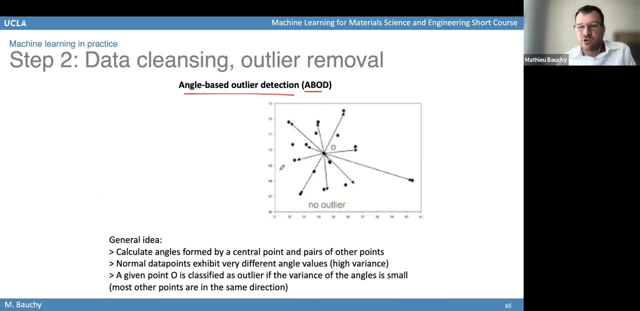 It's based on looking at angles, And so the good thing is that if you look at angles rather than density, it's gonna work better when you have a high number of dimension. So here, the idea of this method is that you're gonna take one data point here. 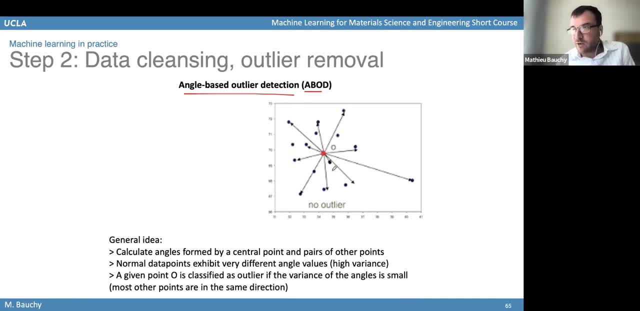 and you wanna know if this data point is likely to be an outlier or not. And so, for this, what you're going to do is you are going to look at all the neighbors of this data point. So you're going to take all the neighbors, like this. 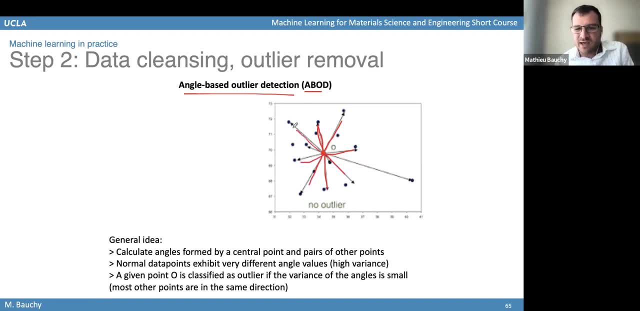 and then you're going to calculate the angle formed by the neighbor, So you will define some angles which, again, like I said, which is the one neighbor, the central point that you are looking at, and another neighbor, So that's going to define one angle. 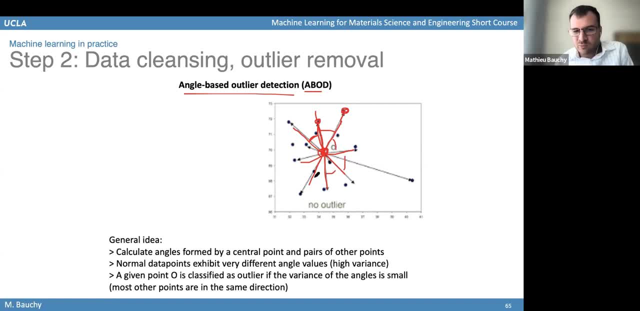 And so you can define all of those angles here between the central that you're looking at and two of its neighbors, And then what you're going to do then is to look at all of those angles, So including, for example, this would be another angle here. 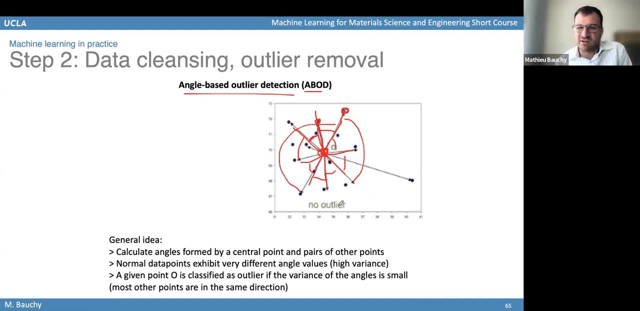 or this would be another angle here. Those are the list of all the angles that you can form with the central points and at least two of its neighbors, And then you're going to calculate the standard deviation of those angles. So if you have something like this: 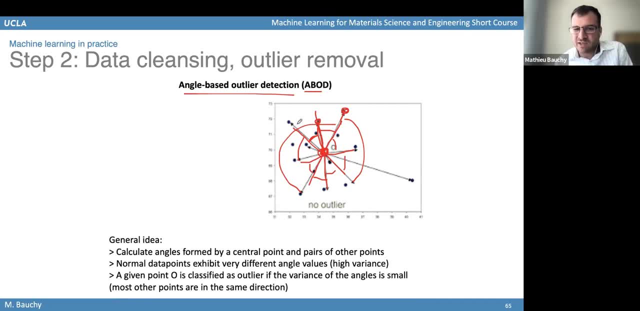 so here, if you calculate the angles, you have very different angles, Like some of the angles are very small, but some of the angles are very large. You can find some very large angle like this. So here it's a point, it's an example of a point that has 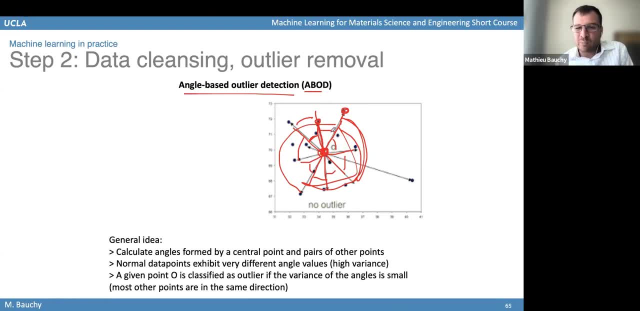 if you look at the angle around this data point, you have a combination of small angles, medium angles and large angles. So that would be a case where you have a high variance of the angle. So that's going to be a case where the angles 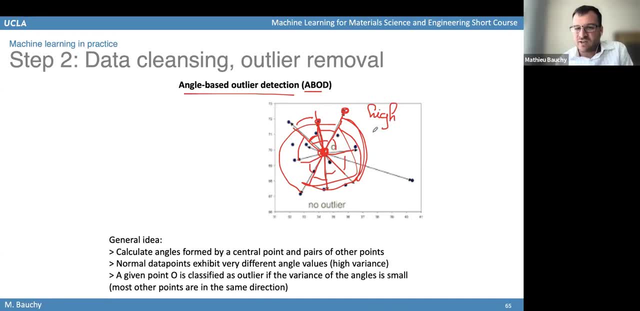 can be small, large, et cetera. It can be. it will have a high standard deviation or a high variance. So in that case, when you have a data points for which the angle around it has a high variance, that's a good sign that this data points. 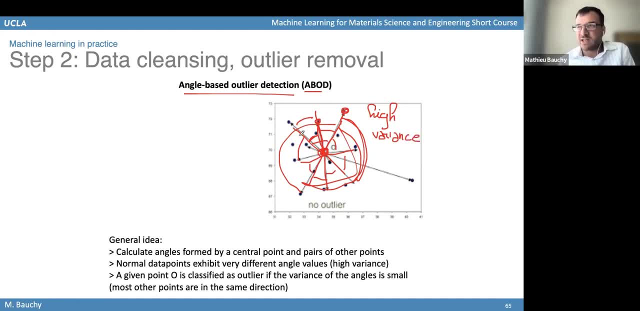 is not an outlier. It means that it's surrounded by all the data points in many direction around it, So it's a good sign that this data point is actually behaving as expected. It has some other neighbors in a direction all around it, So it's surrounded by some other data points. 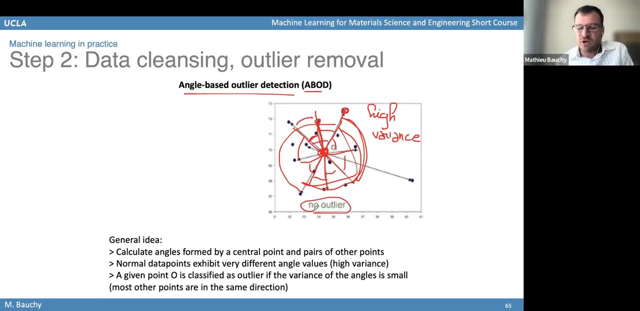 So that's a good sign that it's not an outlier. But, on the other hand, if you have something like this, where now you look at this data point and again you will take all the the neighbor of these data points, 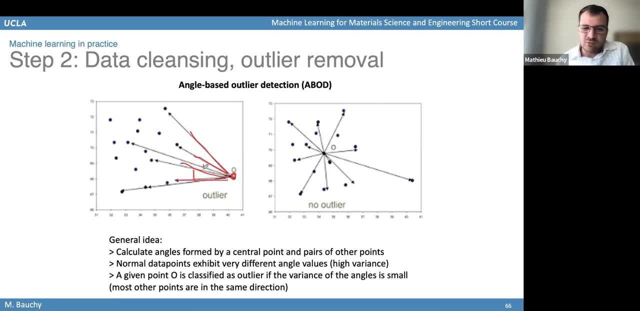 and you will calculate all the angle with the neighbor with respect to the central data point here. Now, all those angles, they are always small, So in this case it means that those angles, if you calculate all the angles between the central data, 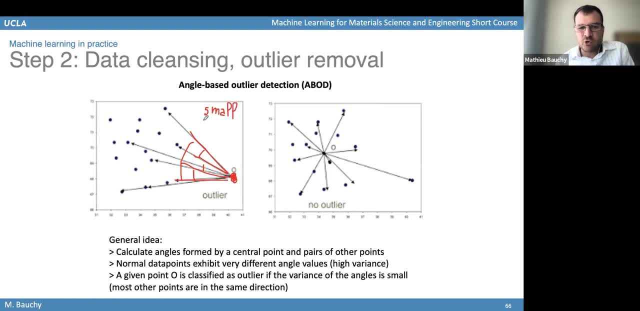 points and the neighbor, you will find a smaller variance because the angle will be always the same. It's always going to be small angle And in that case, when you have some angles like this with a small variance, that's a sign that it's very likely an outlier. 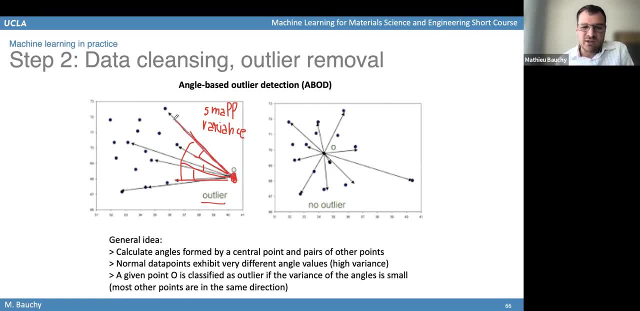 Because it means that it's far away from all the other neighbor, and all the other neighbors are all pointing towards the same direction, like this. So in that case, that's a sign that this is an outlier. It's far away from the other points. 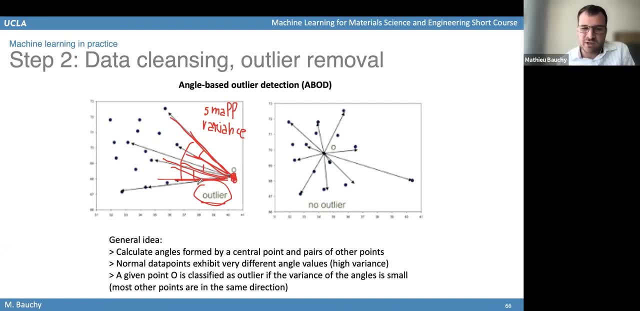 And the angles are all pointing in the same direction. So that's a sign, Where you have a small variance for the angle, that it might be an outlier, And so these types of techniques works better in high dimensional space because it's not based on the density of data points. 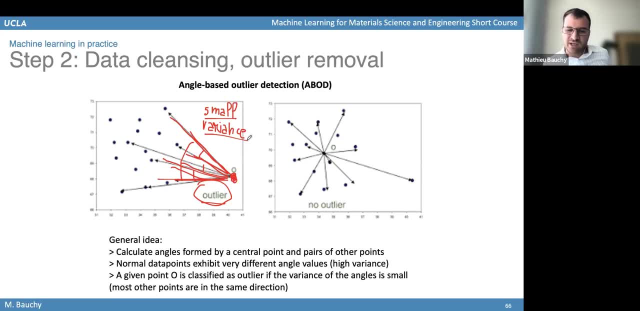 It's only based on the angle around a given data point, So it's a good way to distinguish point that behave as outlier from point that behave more expectedly as point that appear to be more legitimate. So what you would do in this case is look at all the data points that 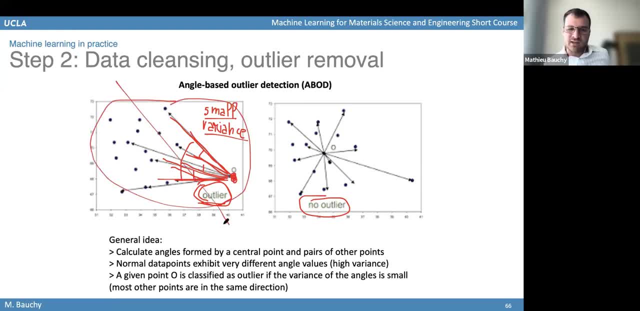 have a small variance in their angles And then either you remove them or you need to double check them or redo the experiments to check what could have gone wrong with these data points. But at least it gives you a fast method that is pretty powerful to detect. 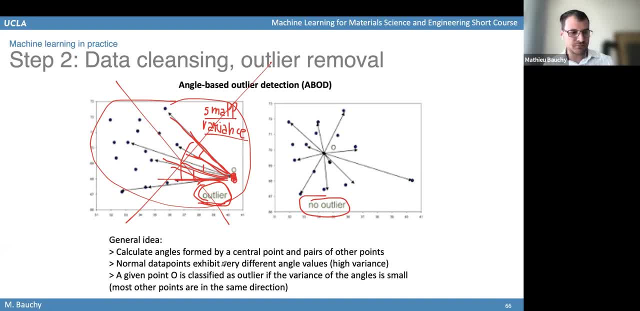 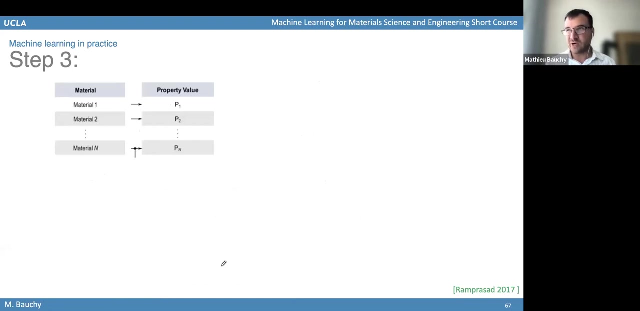 those points that behave very differently from the others. Do you have any questions regarding this data cleaning? step OK, So let's go to the next step, So step three. So now, step one: you have the data set. Step two: you have cleaned the data set. 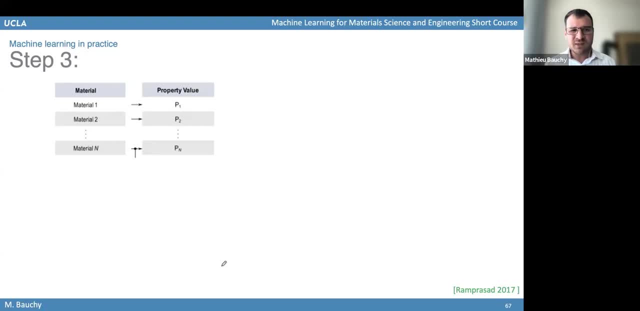 by removing the outliers. Step three. step three- is going to be about creating a fingerprint for your material. So let me explain what I mean. What I mean by fingerprint? So, initially, what you have in your data set is a list of materials. 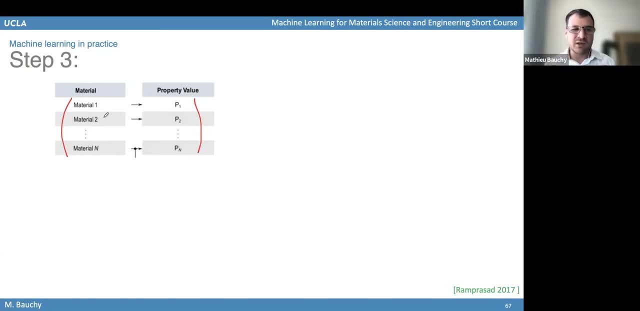 And you have the corresponding measured properties. If you do that, it's going to be very hard for the model to find a direct relationship between those materials and the property. Because you need to find, you need to describe those materials in a way that 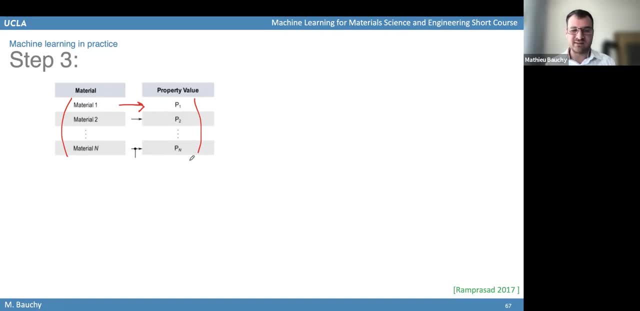 is going to make it easy for the model to predict the property. So what I mean by that is that, for example, when you test this material one, this material two or this material n, you need to describe, You need to find some features to describe those materials. 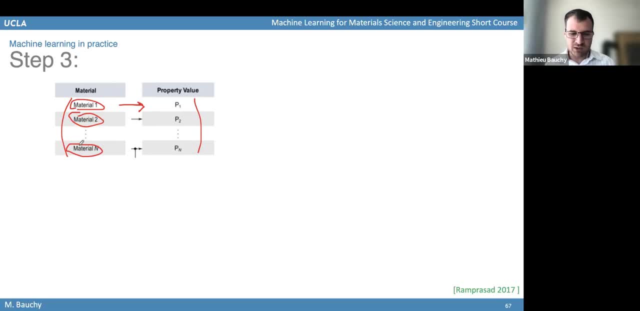 You need to describe them with a list of numbers, And those numbers are then what you are going to use as input for your model to try to see how you can predict the output property. So this is going to be about creating, and we're going to do that today. 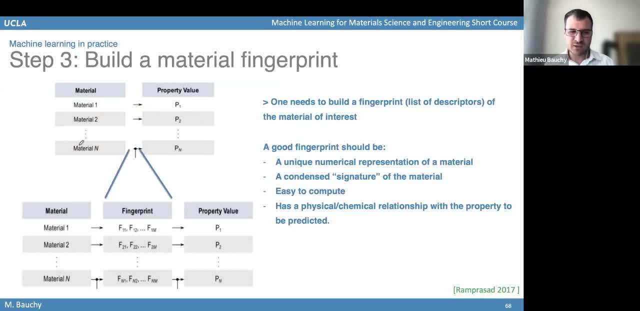 OK, about creating a fingerprint for the material, and the idea is going to be like: you start with your material, like material one, material two, material n, then you will create a fingerprint so you will find a list of features that describe this material. so that's going to be feature one. 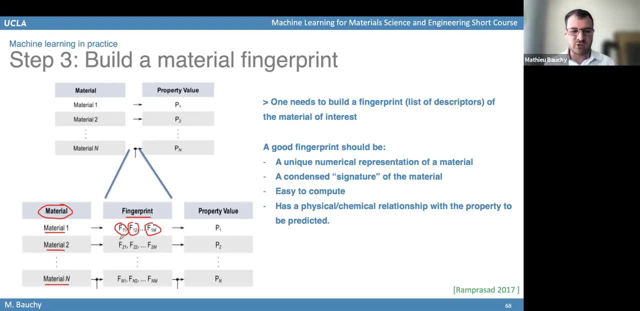 feature two, feature m, and then you are going to look at what is the value of these features for each of the material. and this, the value of those features for each material, is what we will call the fingerprint. so let me tell you some example of fingerprint to make it clearer. so 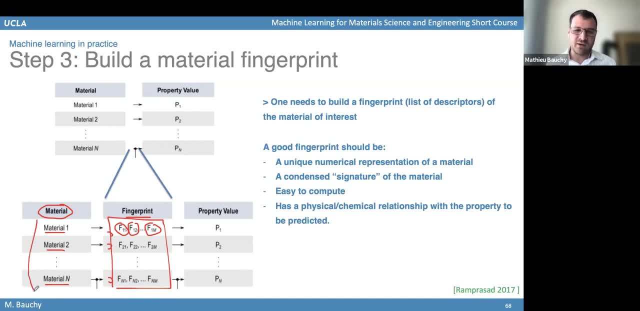 for example, if you have a material, you need to find a fingerprint that you will be that will be able to describe these materials. so, for example, the fingerprint of a material can be its chemical composition. it can be: what was the temperature that was used, uh, when you made this matter. it can be: what was the ph of the solution that you use? what was the? 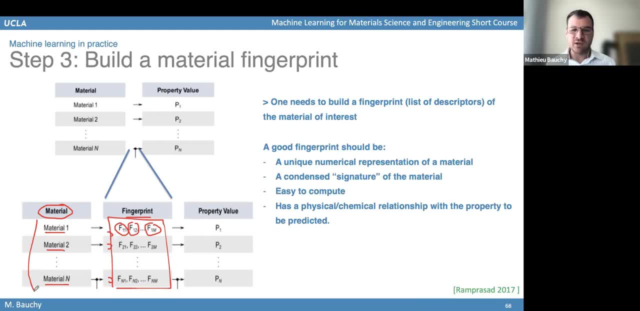 the pressure? what was the? the relative humidity? those are all parameters that can act as the fingerprint of a given material, because it's a list of parameters that can describe a given uh material. so this idea of the fingerprint, it's the same idea as if you have an individual, like a. 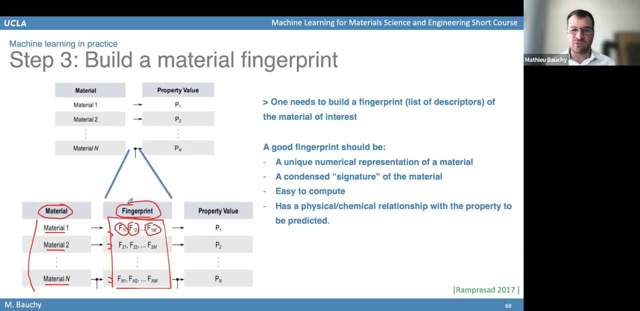 human and you want to, um, to, to, to figure out like which, uh, human is that? so, like how to describe a given human. so if, if you have this, like, you can look at the human, take a picture of this human and um, and look at all the. 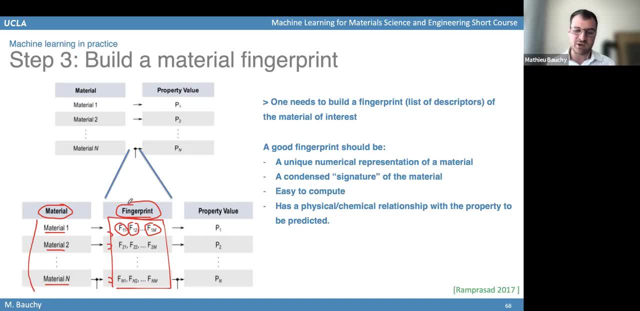 details of of this human. but then, if you do that, you're really gonna have a lot of features like the color of the eyes, the, the color of the hair, the size of the hair, like the weight, the height, etc. so those are a lot of features. what is more efficient is to find a more. 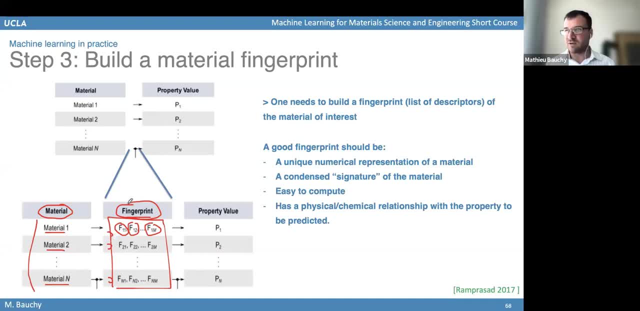 condensed way to represent an individual and, for example, if you, um, if you are a human, a very simple way to identify one human and to separate it from another is to use, like, the, the fingerprint, like, like the actual fingerprint in the, in your, in your, in your fingers, and it's a good way because, like, uh, it's a, there is a very low. 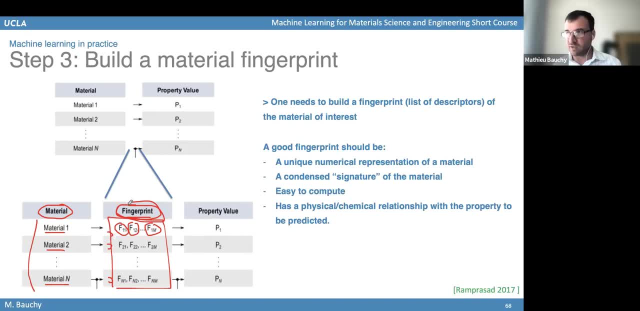 chance that two different individuals will have the same fingerprints. so and the fingerprint is a very small representation, it's just like a small part of your body. so it's a very condensed representation of of a human, but still it's. despite the fact that it's small, it's enough. 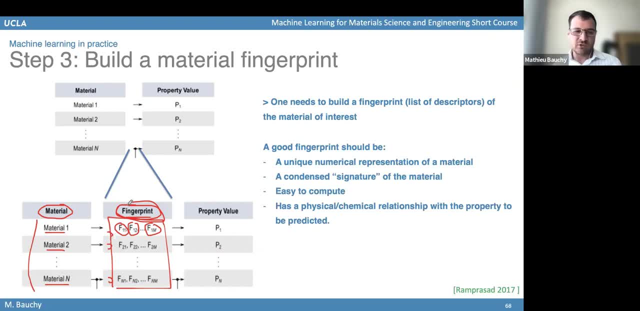 to separate different individuals from each other, so that should be the same idea for materials. if you want to develop a machine learning model, you will need to find what is the right fingerprint to describe your material. so ideally so the fingerprint should be a list of descriptors, a list of features that describe your material. so a good fingerprint ideally should have a various. 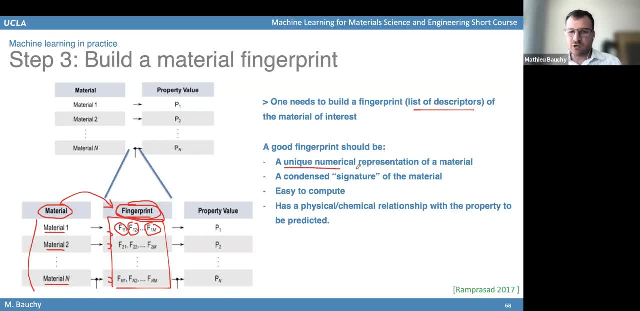 characteristics. so first it should be a unique numerical representation of a material. so unique means that two materials that are different should have two different values for the for the fingerprint. like if if you define your fingerprint in a way that two materials that are different can still have the same values for the fingerprint, then your model will not be able to distinguish those. 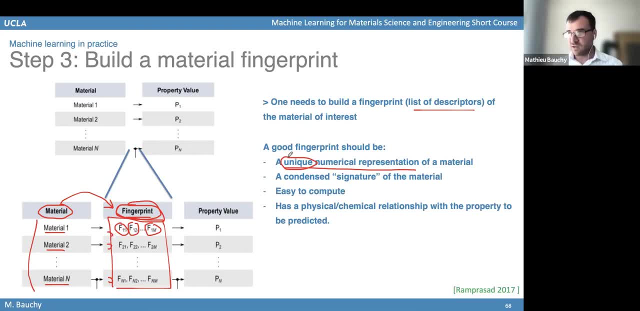 two materials. so you need to have a fingerprint that is precise enough that each material that is unique. if two materials are different from each other, then they should have different values for the fingerprints. for example, if you, if you um, if you define your fingerprint as being the composition of the material, a chemical composition, then if two materials have 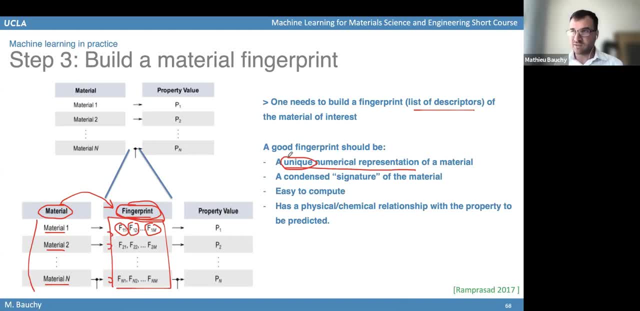 two different composition, then they will have two different values for the fingerprint. so that would be a good fingerprint. but if you just take a material and use its density and, uh, you'd say the density of this material is it's what i'm going to use as its fingerprint, then it's possible. 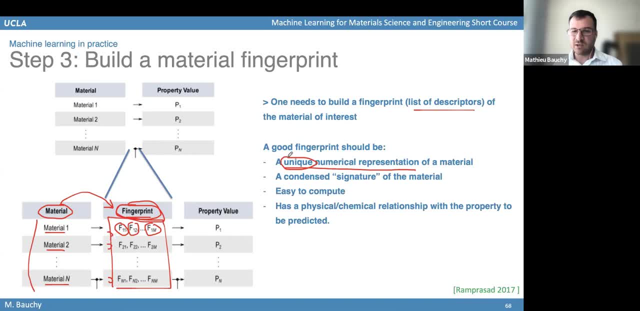 that you can have two different materials that have the same density, but still those are two different materials that are different from each other, two different chemical composition, etc. so in that case that would not be a good fingerprint, because it's a fingerprint that would not distinguish materials that are actually different from each other. so it should be unique. 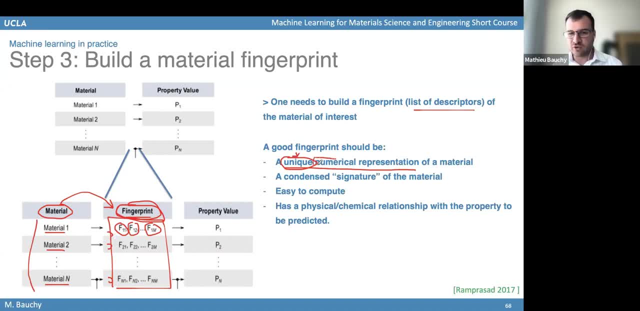 that's the first characteristic of a fingerprint. it should also be numerical, like you need to be able to put some numbers, like if you have a material, you cannot just say this is material one, material two, material three. you need to be able to come up with some numbers, uh, for example. 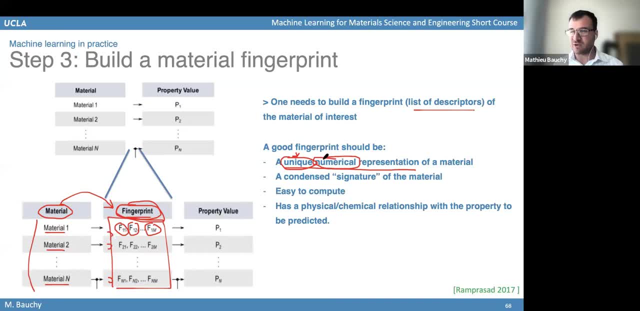 you can say: how much carbon do you have in this material, what's the, the concentration of carbon or what was the temperature that was used to create this material. so these are going to be some numbers, so it's going to be a numerical representation, with a number that can change. 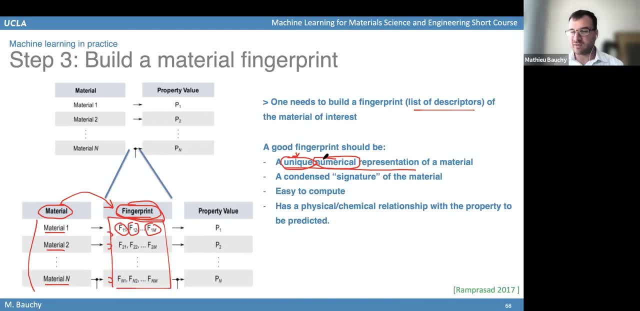 for each material. so that that's going to be a good fingerprint if it, if it can be quantified by some numbers. the second thing is that the the fingerprint should be condensed. it should be a vagable. it's good if you have a very large, wow. 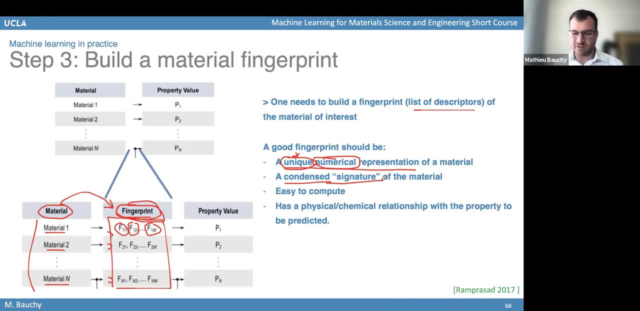 as you very like. you have 100 000 signatures, so it really depends quite on how much you know looked like. so the important thing is: is that no life history I'm very passionate about Сейчас? очень ouvelländ 수도 details in这有很多. 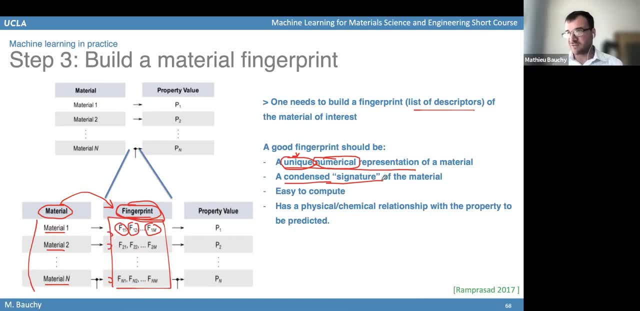 But a lot of fun fact is this is not that it's so, it's only that I think it's very important, and so you think if I want a big feature of a material, it's too blue. or you think it's no. find a very condensed way to represent your material. for example, if you have a list of. 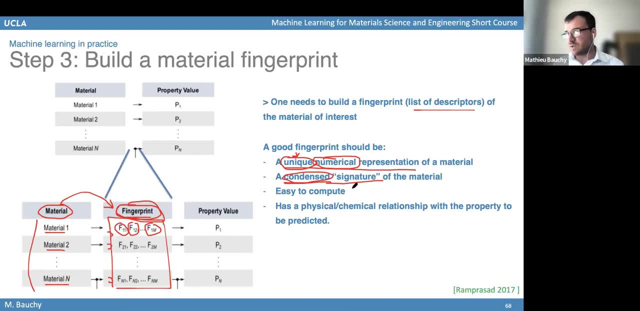 different materials and you. the only thing that is changing for these materials is the temperature that is used during the processing of these materials. then probably you should not use the pressure, or you should not use the relative humidity as being part of the fingerprint, because it's not really changing, it's not really influential, so you should really focus. 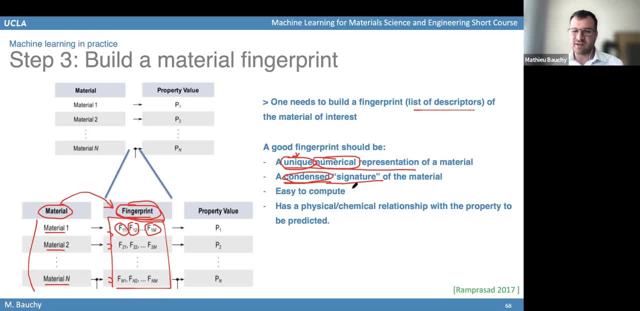 on the, the properties, like the features of your material that are the most important and remove the one that are not very influential. so it means that your, your fingerprint, needs to be precise enough so that it can distinguish material that are different from each other, but it also needs 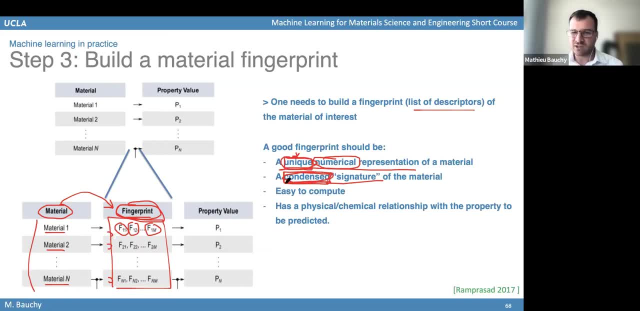 to be condensed enough, because if it's too large, then your you will have too many different dimensions. that's going to be bad for your machine learning model. you will need a lot of data, so it needs to be still as condensed as possible that you need to describe your material. 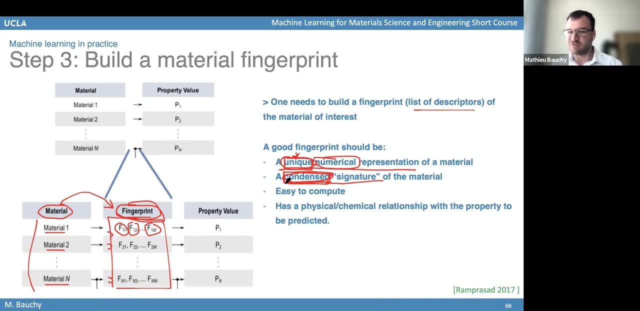 with a small number of, um of, uh, different features. so the the next thing is that your fingerprint needs to be easy to to compute, easy to calculate or easy to measure, like, for example, if you have a given material and if you are going to say, i want to use. 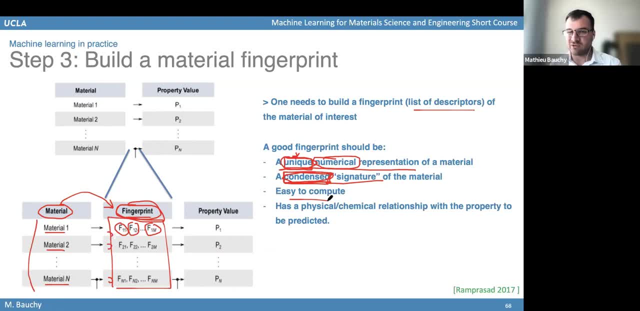 the the melting temperature of this material as a fingerprint, or i want to use the band gap of this material as the fingerprint. maybe that's a very good choice if the melting temperature or the band gap is an influential feature of this material, but then it means that you will need to. 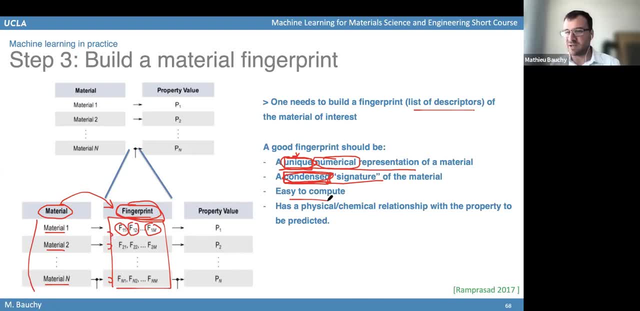 be able to. for all the materials you have, you will need to measure them, their melting temperature, or you will need to measure their, their, their band gap. so that's something that uh might be hard to to get, if it's something that is hard to measure, or how to how to compute. so, uh, ideally the good. 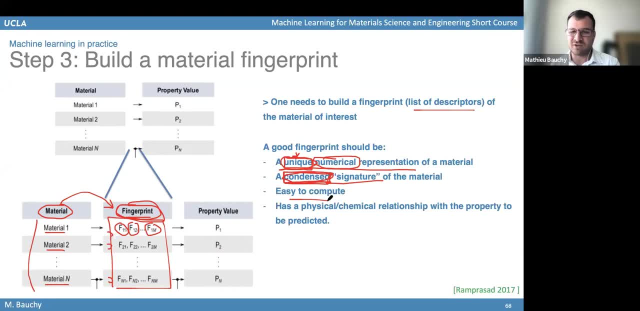 fingerprint should be something that is, uh, not too difficult to access, because otherwise it's going to take you a lot of effort, a lot of time to measure the value for the, for this fingerprint, for all the materials that you have, the. the next thing is that, ideally, your fingerprint- 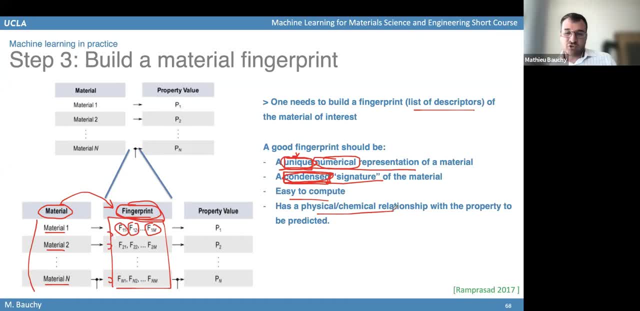 it should be based on some, um, some features of materials that are likely to have a physical or chemical relationship with the priority that you're trying to predict. for example, if you're trying to predict the, the density of a material, then, uh, most likely you just need to know. for. 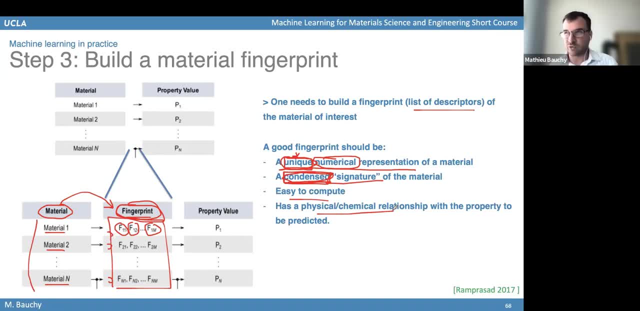 example, the, the composition of the material. maybe you, you should know also the porosity of the material, and that's going to be enough to predict its porosity, because, to predict its, its density, sorry, because the density is going to be, uh, very influenced by the, the porosity. 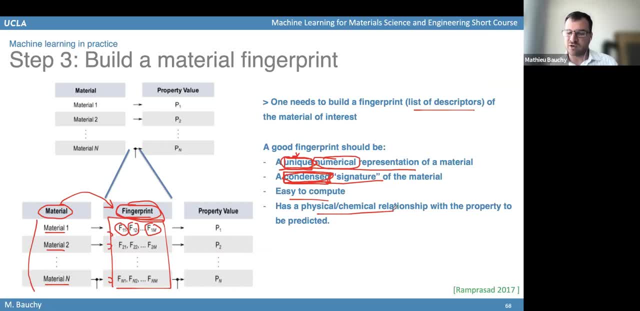 of the material and by the, the composition, uh, of the, the element that are that this material is made of. but in that case, maybe it's not that useful to know the, the band gap of this material like, because, um, the the band gap of a given material is, uh, maybe it has nothing to do with its density. so 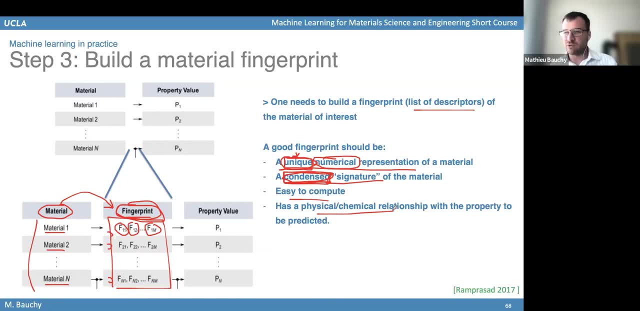 even if you know the band gap, that's not going to be so helpful to be able to predict its density. so when you, um, when you select the various features that you're going to use in the, the fingerprint, ideally you should choose the one that are the most. 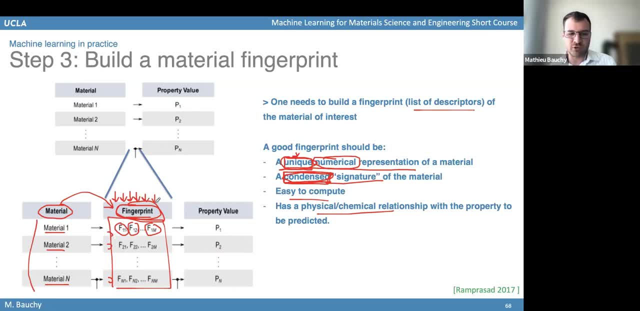 actually the the most likely to be influential, the the features that are the most likely to be actually related to the priority that you are trying to predict. so that that's another thing, like if you have some intuition that this property should be influential or this property should not. 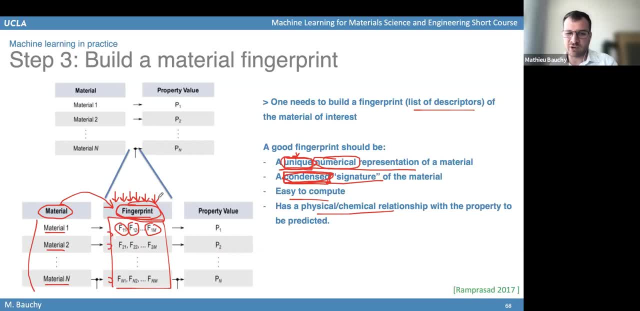 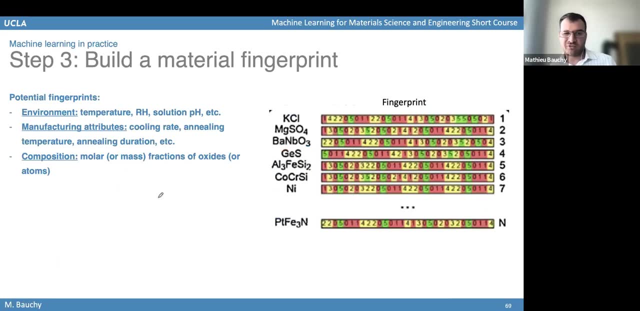 be influential, then you can use that to inform your choice of the of the fingerprint. so like a example of potential fingerprints, so some fingerprint can be about the environment itself. so either the environment during the synthesis of the material or during the, the condition uh, during which the material is being tested. so the temperature, the relative humidity. 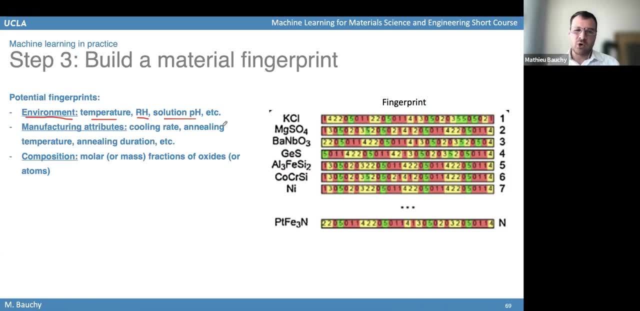 the solution, ph, etc. so those are all potential um information that can potentially influence the, the property that are being measured, and so in that case it's important to include them in your fingerprint. then you have the, the manufacturing attribute, like, for example, if you form a glass. 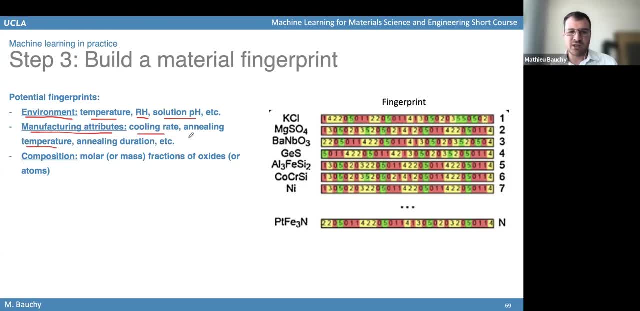 what is the cooling rate? what was the, the temperature at which you anneal your material? in which direction? how long did you anneal your material? like all of those things, it's about the manufacturing. it can influence the property of the material. so in in that case, if it's something, 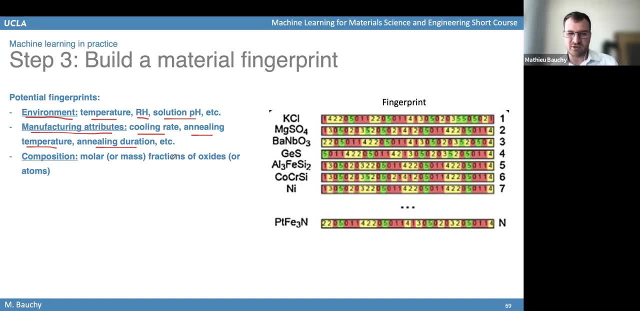 important. it needs to be included in the fingerprint as well. and then you have some information about the material itself, like about its um, its, its composition, its chemical composition, like what type of oxide is it made of, etc. so, like the, this is some information about the material itself. maybe you could also have the porosity. 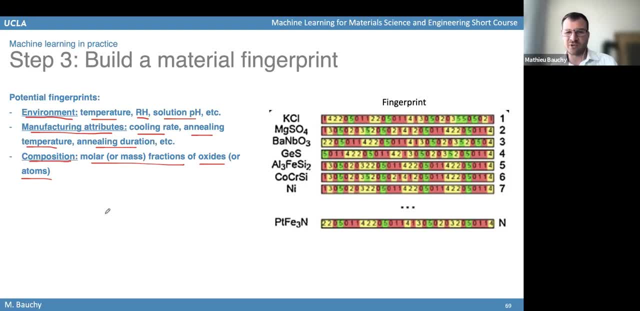 the degree of impurity, etc. so those are some, all, some, some fingerprints. that uh is going to be about the the material itself, and in that case it should also be um, uh included in your, in your fingerprint. so then your fingerprint is going to look like this, like: 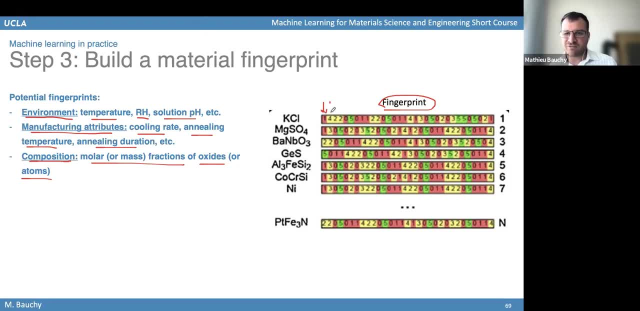 uh, you will have a list of features that you are going to determine. so each feature, in this case, here would be one column of this table. so for each uh, each feature. for example, for example, you will want to have the- the temperature- that's going to be column one. you will want to have the 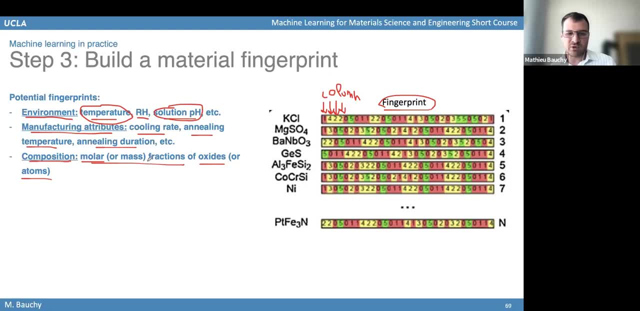 the solution ph, that's going to be column two. or you will want to have the, the composition of different oxide, that's going to be column three, four, five, etc. and then you will have different lines. those lines are going to be the different materials that you are testing. so here, for example, 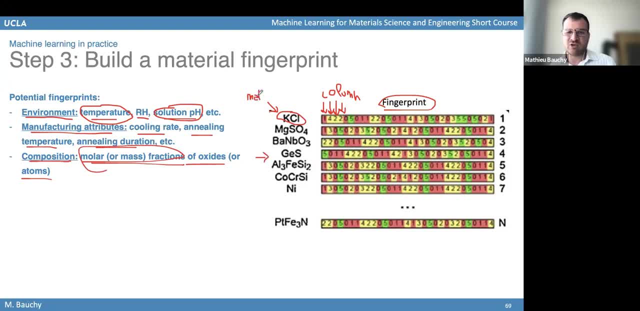 if those are different materials that you are testing, each material will be a given line. so you have the- the feature as a as columns. so this is the features according to which you are describing your material: as different columns and then as different lines, you have the- the materials. 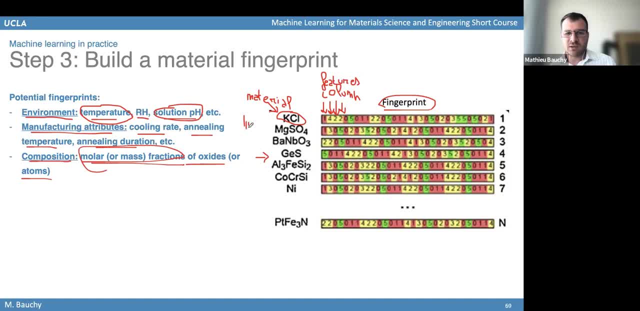 that are going to be different lines here, and so this then gives you a fingerprint for each material. you need to know the value of the feature. so that gives you a table here where, for each material, you have this fingerprint, with this fingerprint is going to be a list of values here you will need. 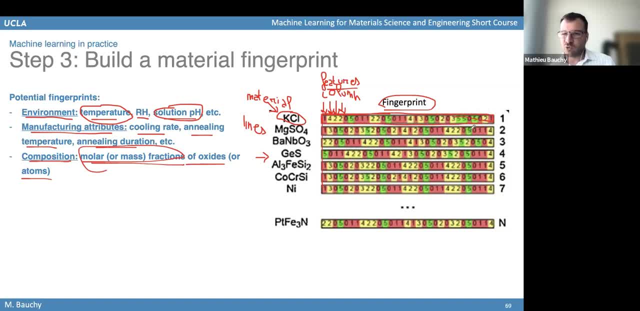 you will know, for each material, what is the value of all the features for this material, and so for each material it will have one fingerprint which is like the list of all those values here. so you can think about this like some kind as a as a barcode, where for each material there is like 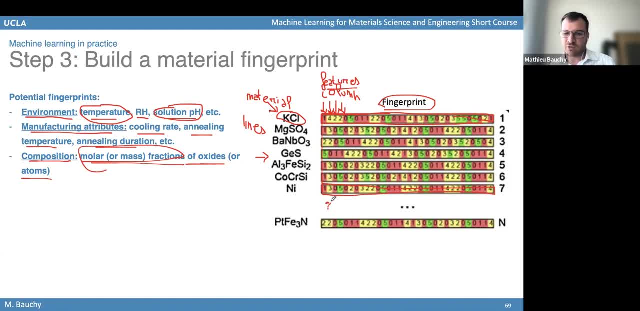 one barcode, which is the the value of all those things, or, like you can think of this as a QR code if you want, where, each for each material, it comes with one list of values like this, which is the value of all the features in the fingerprint, and this is really what is going to be capturing a. 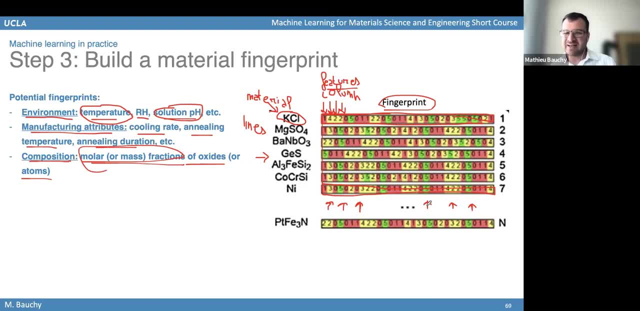 representation of your material. this is what is going to be used as input for the machine learning model. Do you have any questions about this? about the this step of building a fingerprint for the for the material. Okay, so let's go to the next step. so now, so you have the data set, you have removed the outlier. 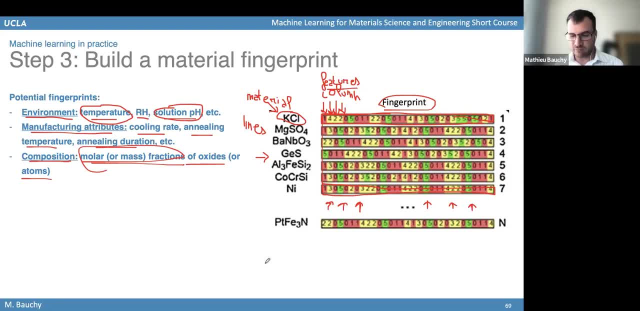 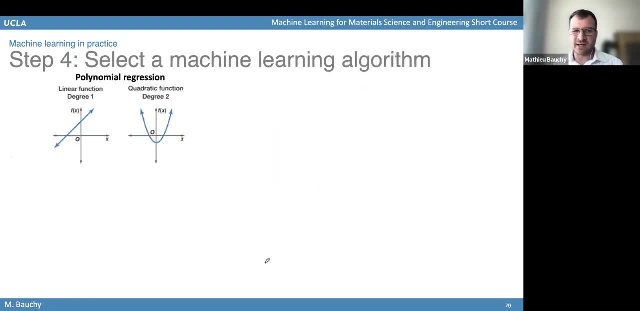 as step two, and now you have a fingerprint as step three. so the next step is that you will need to select a machine learning algorithm. so we talked already about polynomial regression, but there can be some other algorithms that are more complex, because polymer regression it's it's pretty limited, like 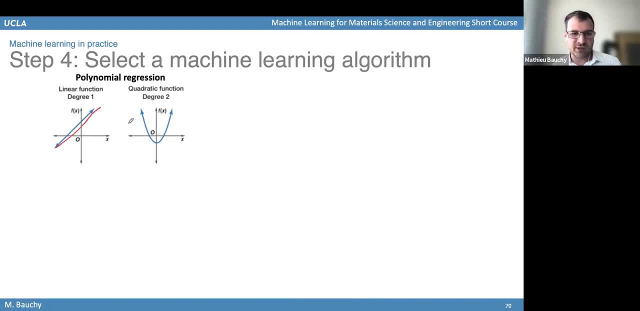 it's. you can have something that is linear, or you can have something that is quadratic, you can have something that is cubic, etc. but the the number of potential types of relationship that you can have it's going to be limited by the, the polynomial nature of the function that you are. 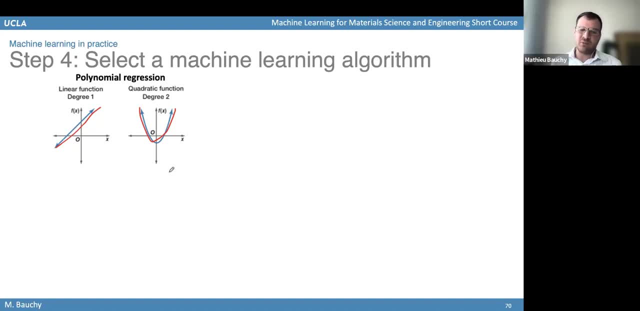 using. so there are some other machine learning algorithms where you have more freedom and you don't need to know in advance if the relationship between the input and the output is going to be linear, cubic, quadratic, etc. so a very common types of machine learning model is the artificial. 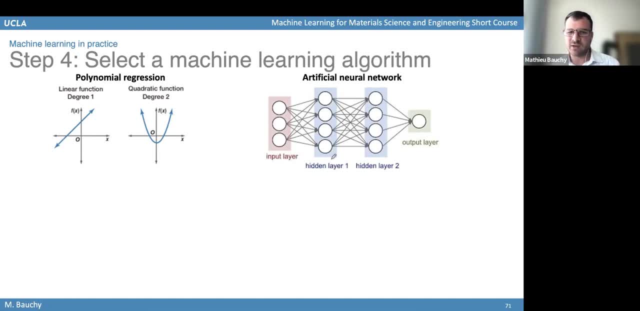 neural network. we will talk more about this in a few slides. the idea in this case is that you will use the fingerprint of your material. that's going to be the input and then, on the other side of the, the artificial neural network, you have the output that you want. 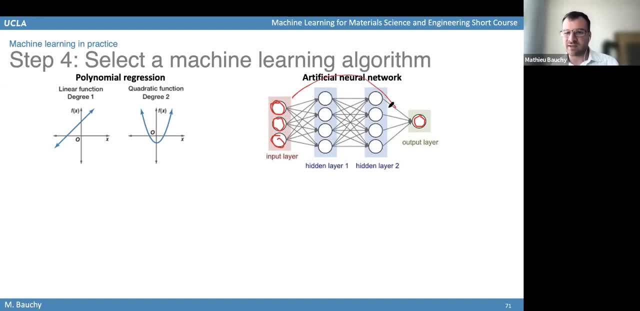 to predict. and then the way you're going to connect the input to the output is by this kind of network where the inputs are going to be connected to some uh, what we call some neurons like this, which are going to be- uh- i will talk more about what this is, but so there are going. 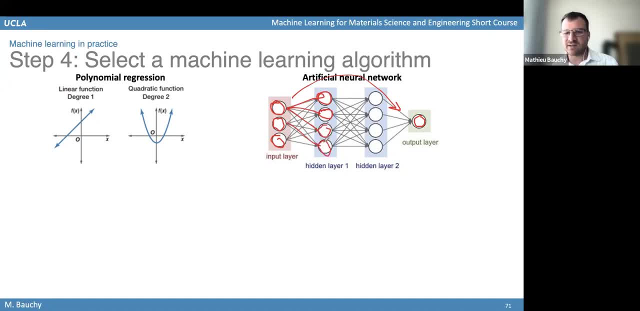 to be some intermediate nodes that are connected to each other. those neurons can be all connected to some others, or there are also connected to some other neurons, like this, and at the end those neurons are going to be connected to uh, to the output, and then what you will need is to to. 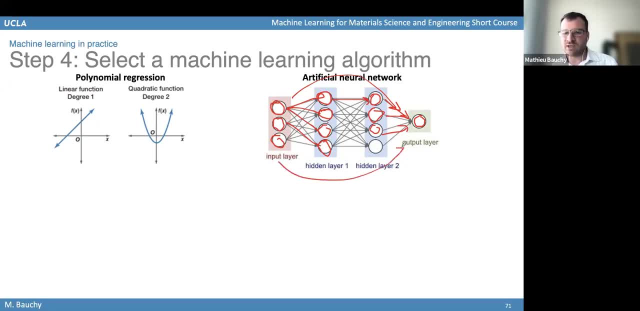 find what is the the best network like this that can transform the input into the output. so it's going to be made of different layers, so you will have: uh, this is the first layer, this is the second layer here, going to be connected to the output through different layers like this, which are going to 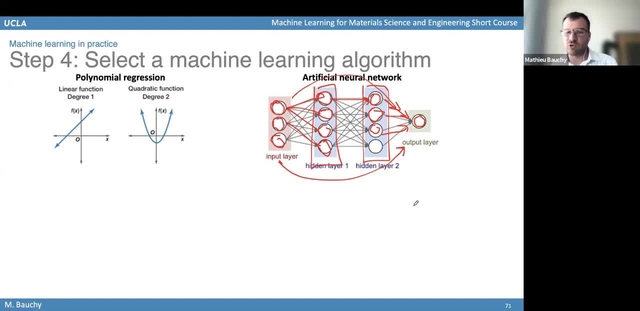 gradually transform the input into the output. So we'll talk more about this. So this is the artificial neural network, or usually we write it ANN, like this. And so this is a very powerful method because it can find very complex relationship between input and output And you don't have to. 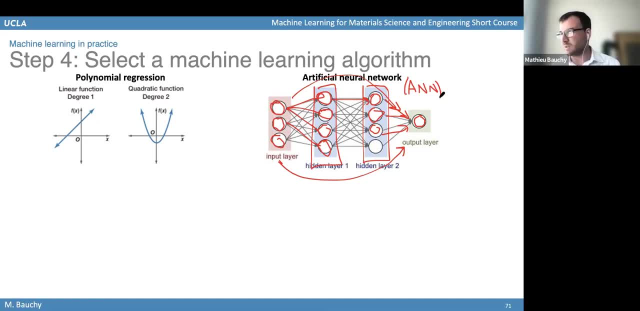 make any assumption regarding whether the model is going to be linear or quadratic or cubic or anything like that. So these types of artificial neural network can learn very complex function, very complex relationship between input and output. So we'll talk more about this, because this is one of the most commonly used method. Another example would be a decision tree. 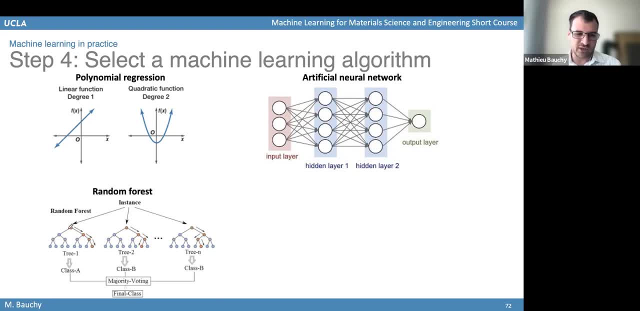 In a decision tree. it works like this: You start with a, a, a, a first node, like this, And then you will ask one question. For example, you will ask: is the temperature lower or higher than a given threshold? And depending on that, 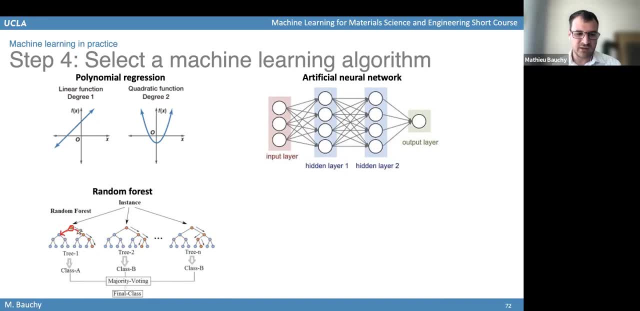 depending on which one of those two cases is it, you will have two different branches, And so if the temperature is lower than the threshold, you will go to this branch, And if the temperature is higher, you will go to this branch, And then you will keep asking more and 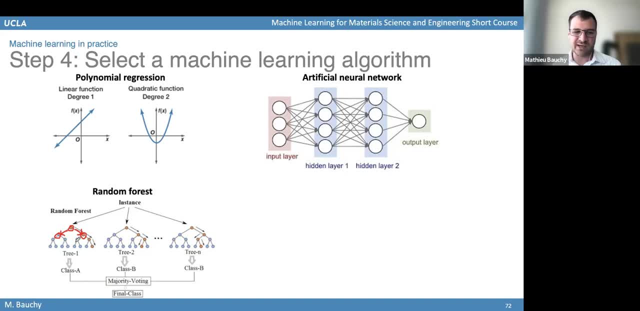 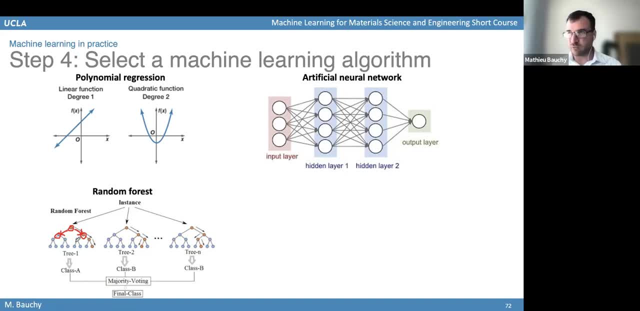 based on the value of the fingerprint. So, for example, if your fingerprint contains the temperature of the material and if it contains also the composition of the materials, you will have a different branch, where the branch that you will follow will depend on the value of the temperature. 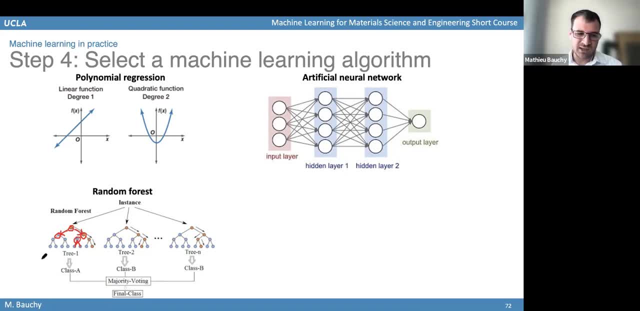 or will depend on the value of the composition, And I will say that And at the end, at the end of each branch, this decision tree will say that I think the property is going to be equal to that. So every time you have one material, depending on the value of the fingerprint, you will. 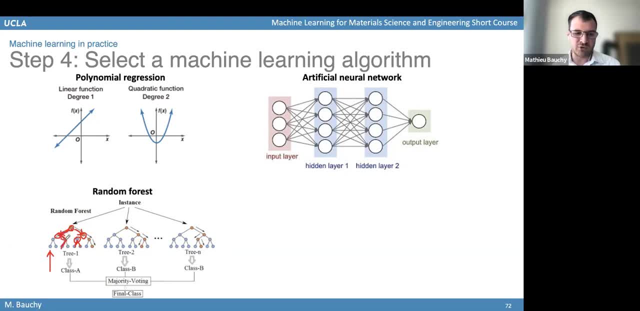 have a given path. You will follow certain branches and at the end you will reach a final node. here that will say: I predict that the property will be equal to a given value. So this would be a decision tree where you make a prediction by a list of conditions. 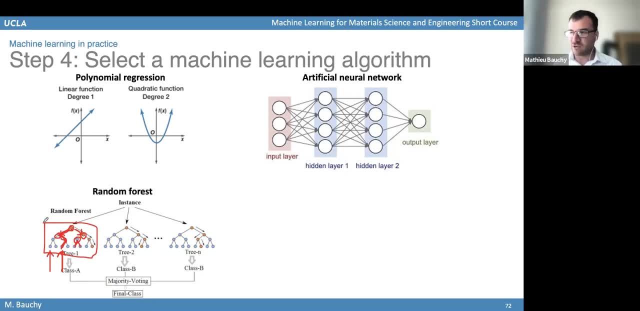 that look at the value of the features And, depending on the value of the features, you select a different branch until you reach the final branch of this decision tree, And in that case each final branch will be associated. So it's going to be equal to one prediction for the property. 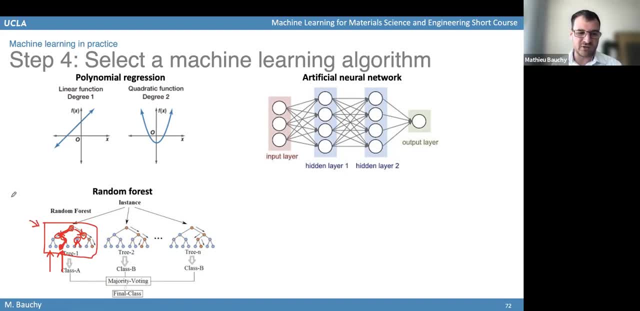 Another common method is not to use a single decision tree. So that would be a decision tree, Like. the reason we call it a tree is because it's made of branches like this, just like a tree. But something that is commonly do is, rather than using one single tree, you will use an. 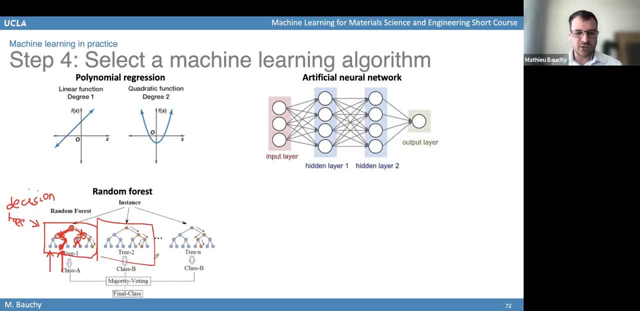 ensemble of trees. So you will use a tree, number two, tree number three, et cetera, And so you will have this ensemble of trees that we call a forest. The forest is going to be a large ensemble of different trees, And then what you will do is that each tree will be slightly different from each other. 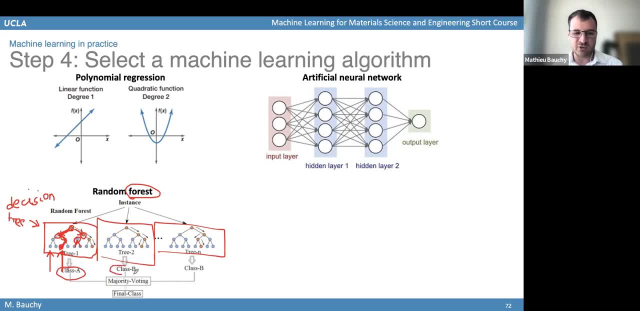 And each tree will make a prediction, like about the value of the property. Each tree will predict something And then you will look at all those trees and you will consider that each tree is voting for one value. So, for example, this tree is going to think: 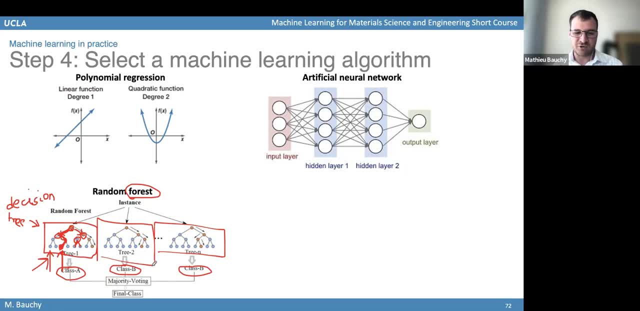 This one is going to think that the use models of a given material is 40 gigapascal. This one is going to think that it's 40 gigapascal. This one is going to think it's also 40 gigapascal. 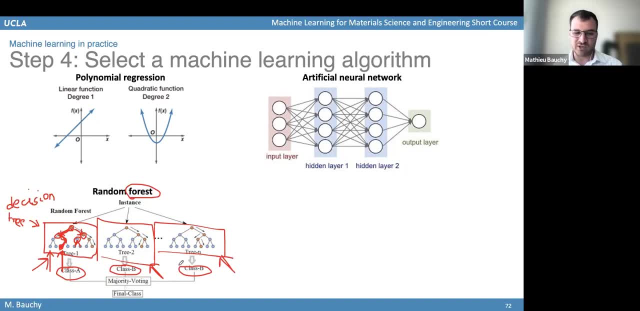 So all of those trees will be voting for a given prediction, And then you will look at what is the majority, What does the majority of those trees think, And that you will select the choice. whatever is the choice, that is, the most trees are voting. 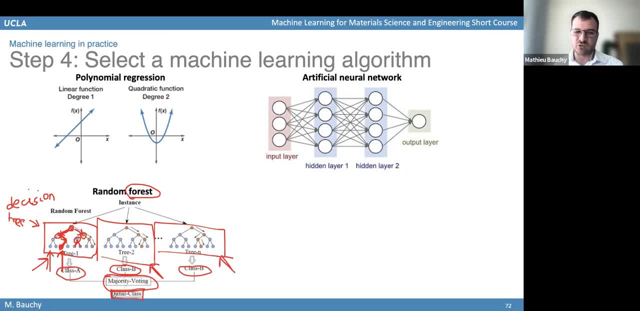 for this choice. That's what you will use for your final prediction. So sometimes, just, rather than using a single tree, you use this forest, this random forest, this ensemble of trees, And then each tree makes a vote, And then you look at what is the overall consensus. 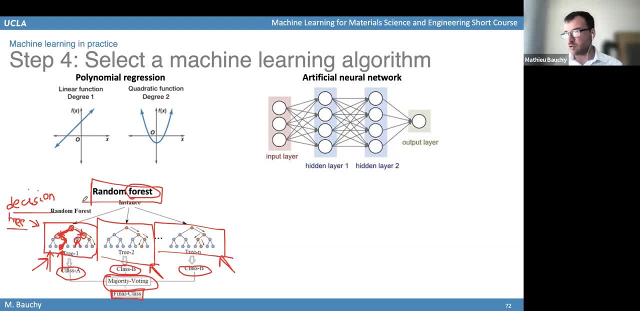 What is the vote? that is the most popular vote among all those trees And that's going to be the prediction from your random forest model. Another example Of model would be the Gaussian process regression. So random forest it's typically we write it RF and the Gaussian process regression. 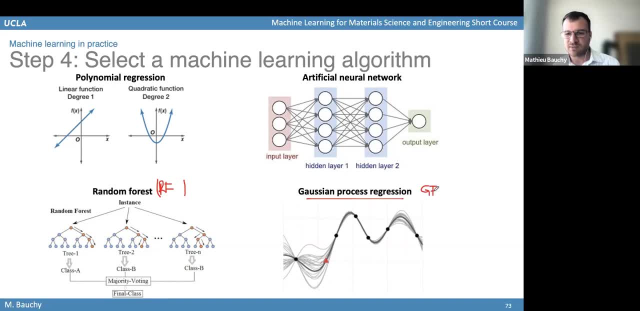 that's typically abbreviated as GPR, And so in this case, the idea is that you have some data points here and you are going to try to describe those data points with different Gaussian processes, So you would have a- you will describe this- with different types of process: Gaussian. 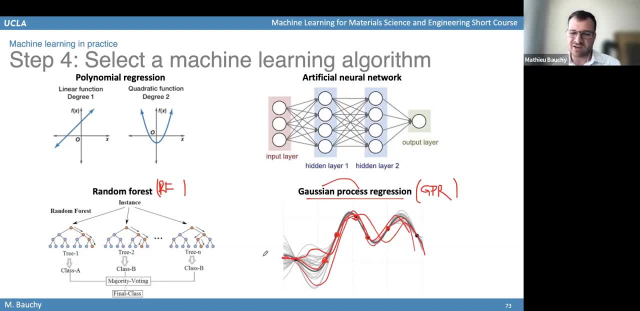 processes. And the good thing about this is, once you have described those data points with different Gaussian process like this, it's going to give you a model that you can use to predict, For example, if this is the input X and this is the output Y. then once you have this model, 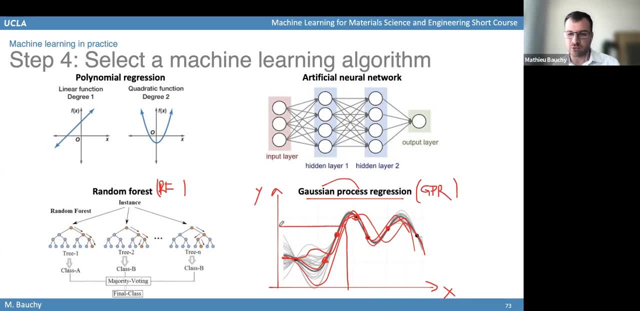 you can say: for given X, I predict that the output will be Y. But this step model- the big advantage- it's also going to give you a prediction of the confidence interval, For example, like here, if you have a point X. this model is very not confident in this. 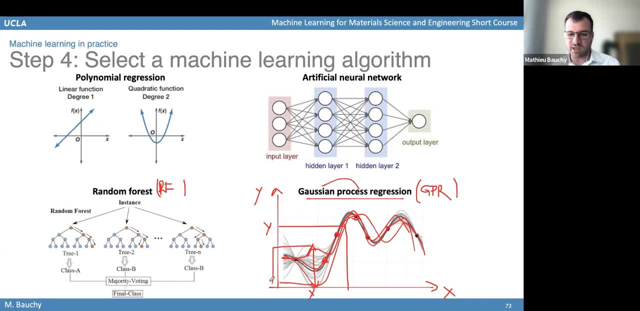 It cannot be sure, like, of the value Y. Y can be anywhere within this interval here. So the idea in this case is that this types of method not only it's going to give you a prediction of what it thinks the value of a property should be, but it's also going 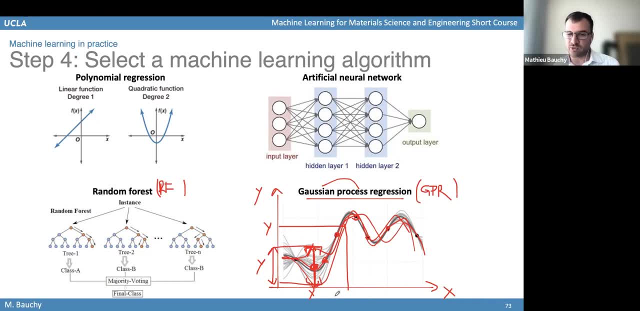 to give you a prediction of the uncertainty of the prediction. It's going to give you the confidence interval of the prediction which other method typically cannot do. other method will give you for given material is going to predict one property, but it won't tell you how confident the model is in predicting that property. 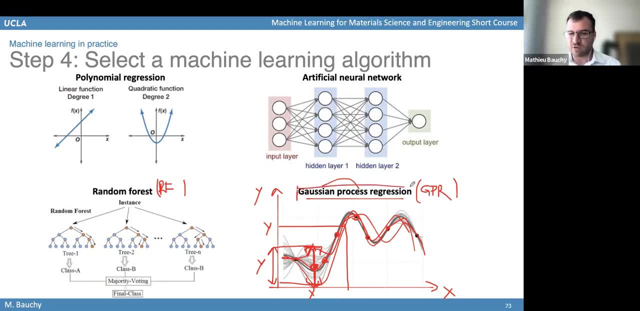 So that's one of the advantage of this. Okay, So now let's we're going to talk more specifically about maybe the one of the most popular models that we've seen in the last few years, which is the Gaussian process regression model. 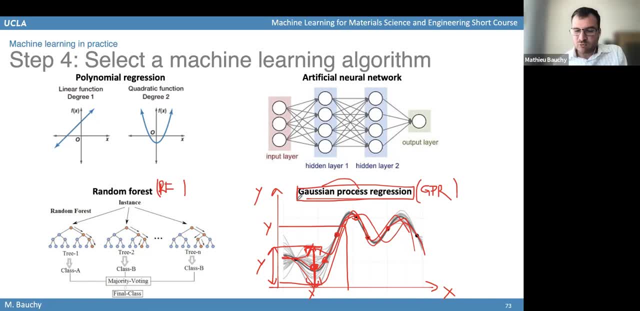 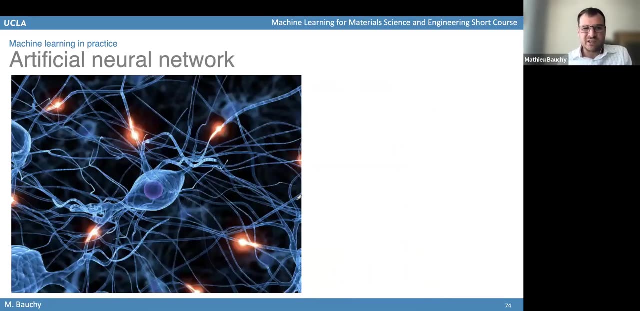 So the Gaussian process regression model is a model that gives you a prediction, but it also gives you the uncertainty. It gives you how confident the model is when predicting this, this priority. So that's a big advantage if you want to know also how confident like, how confident should. 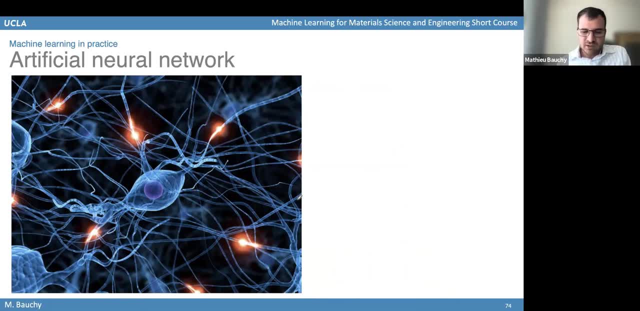 you be about this prediction, Okay, So the Gaussian process regression model is the most popular model in machine learning, which is the, the artificial neural network, And the reason this, this model, is pretty popular is because it mimics the way the brain. 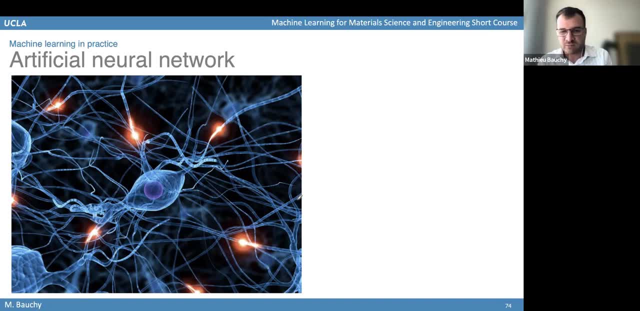 works. It's an approximate representation of how the brain works, at least, and how the brain learns how to perform certain tasks. So the idea of the artificial neural network is that it tries to mimic the way in the brain you have some neurons that transmit some information to each other. 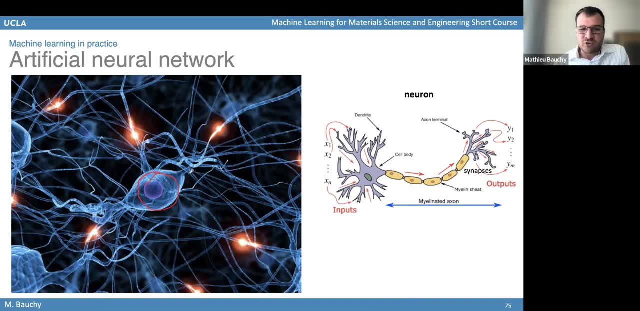 So if you look at the brains, it's made of different neurons like this, and those neurons are going to transmit some information that are going to be transmitted to other neurons, And those neurons are connected to each other and they transmit some information to each. 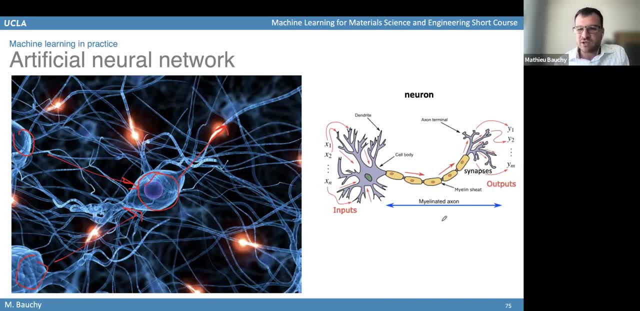 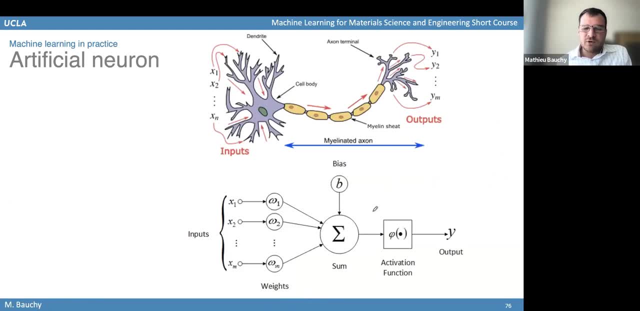 other. So that's the same idea. in an artificial neural network It's also going to be made of different neurons that are connected to each other. Okay, So like, the basic unit in the artificial neural network is this neuron thing, the neuron. 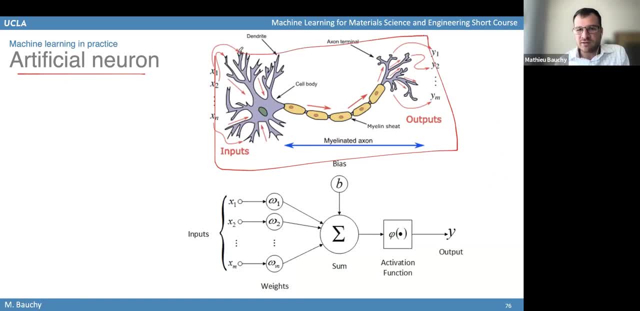 So this would be here like one neuron. This is the what the neuron would look like in the in the brain. And now this is the way a neuron looks in a. an artificial neural network Like this entire thing would be one neuron. 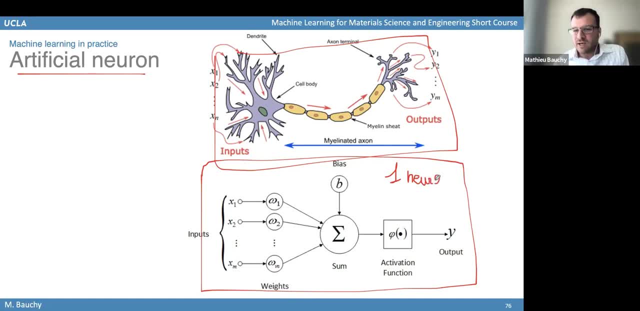 So the idea in in, in the brain, of the brain, What the neuron is, is that you have some, some, what we call some dendrites, dendrites, dendrites- I'm not sure how to pronounce it- which- which is the, the, the beginning. 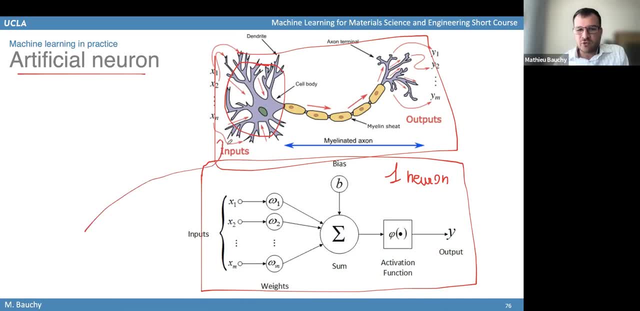 of the neuron. So here, this is where the, the other neurons will be connected to to this neuron and they will be connected to the to the beginning the dendrites of the of this neuron. So this is where some information will be received from the other neurons. 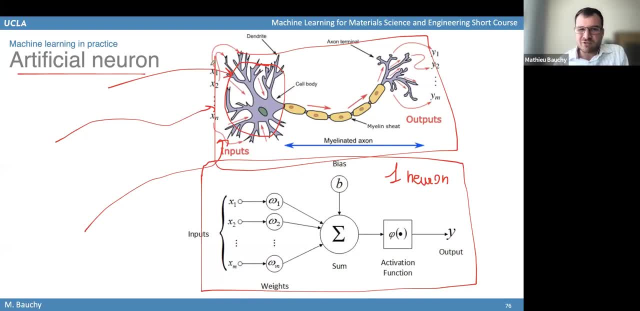 So this is the entry to the neuron. Okay, So you will have different message. X1,, X2, Xn. Those are going to be some electrical signals that are being sent by the other neurons in in the brain, Like the, the. the way neurons transmit information to each other is through some small electrical 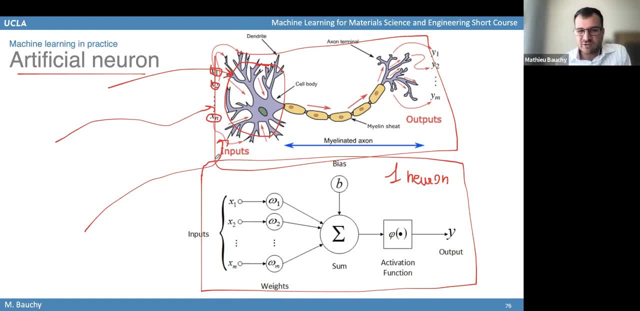 signals, And so some, some electrical signals are going to be transmitted by each neuron to another neuron in here. So that's the, the area where, Where those message are received, Then the way it works is that the this neuron is going to receive those input electrical. 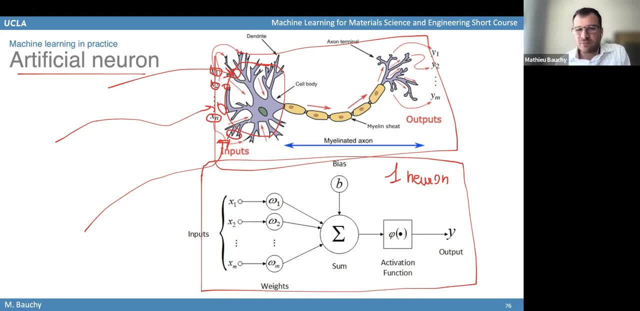 message from the other neurons And then it's going to either transmit the message to through the neurons or the this neuron is going to be stopped. It depends on the value of those input signal. If those electrical signal X1, X2, Xn are very small, not so intense, then they are. 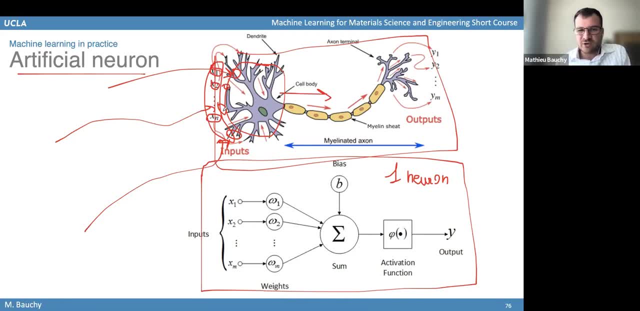 not going to be transmitted to the next neuron, But if those electrical signal are very intense, then they are going to activate, like those dendrites here are going to be activated, and they are going to create their own electrical signal which again is going to be transmitted to the next neuron. 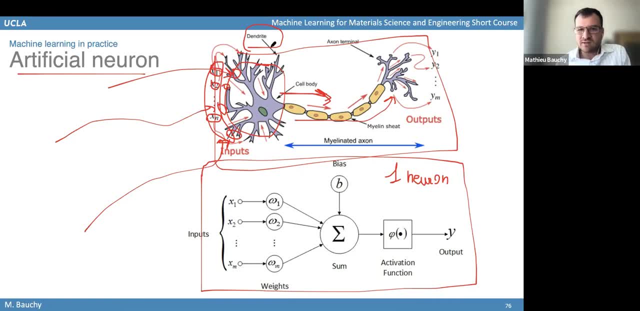 So that that's the base idea of a neuron. It's a unit, It's like a processing unit that is going to receive some inputs, And if those inputs are intense enough, then an output is going to be generated, And this output is then going to be transmitted to the next neuron. 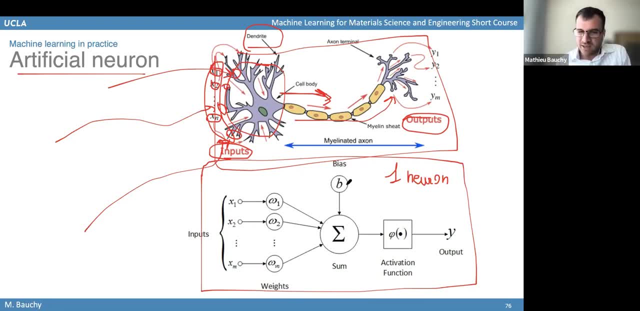 So that's the basic idea of a neuron in a in a brain, Now a neuron in an artificial neural network. It's fairly similar, not exactly the same, but still fairly similar. So the idea is still the same. You have different inputs. 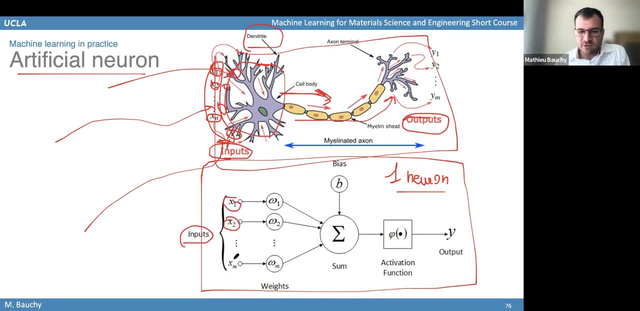 Those are going to be some inputs that are going to be transmitted by the previous neuron. So each- this is going to be a previous neuron here is going to be transmitting different information, And so this neuron here is going to be receiving various information from several other neurons. 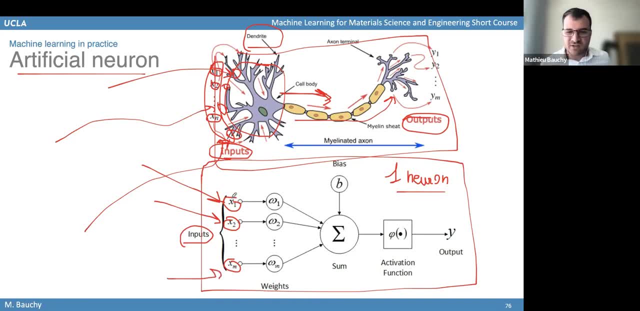 before it. Then what this neuron is going to do is that it's going to take the signal From each of the neurons, And the first thing is that it's going to attribute a weight to each neuron, So it's going to take the signal. 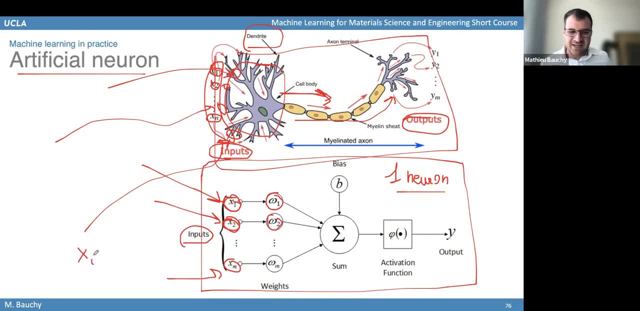 It's going to take all the signal, X, I, where I is equal to one, two, three, et cetera. It's going to multiply this by a given weight. So it's going to multiply this signal by a weight where each, each input signal will. 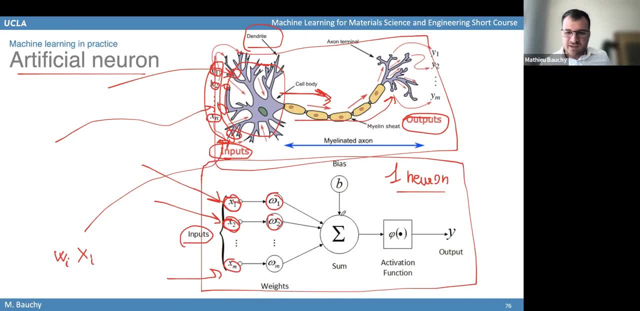 have a different weight, Then it's going to take the sum of all those weighted signals And then you take the sum of all those things where you sum from a I equal one to M, where M is the number of input neurons. So here it takes the sum of all the input neurons after they have been multiplied by. 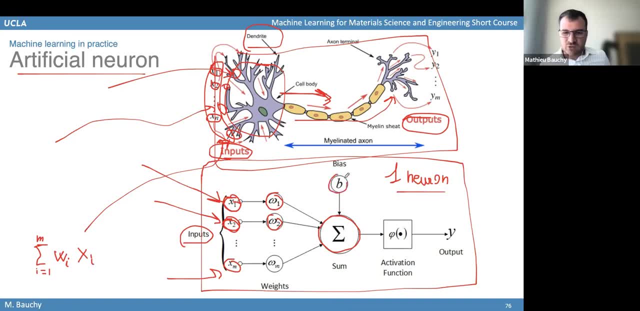 the weight. Then the next thing is that you, you are going to add a bias, So you add a parameter B, which is the, the bias. I will take more about what is this bias- And so this is now going to give you like an output that we can write, H, for example. 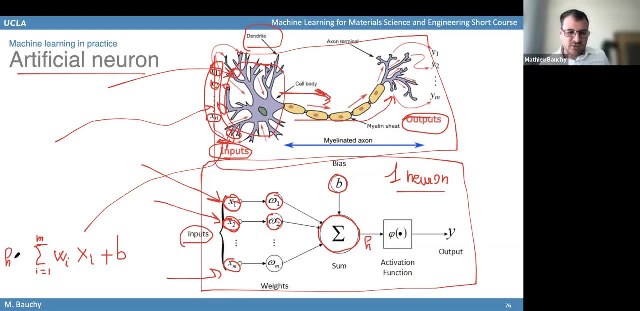 here. So this H is going to be? what is the the? what you get after summing the weighted the uh signal X and adding the bias. So at this point you just have like a weighted sum of the different uh inputs after you. 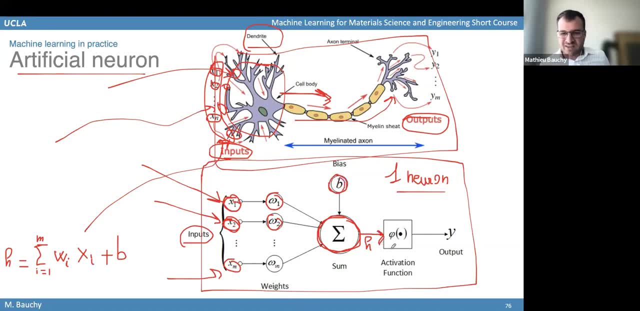 add the bias. Next, once you have this, you will feed that to an activation function. So this activation function will play the role of the dendrites here. This activation function is going to be what? uh, it's going to be a function that decides. 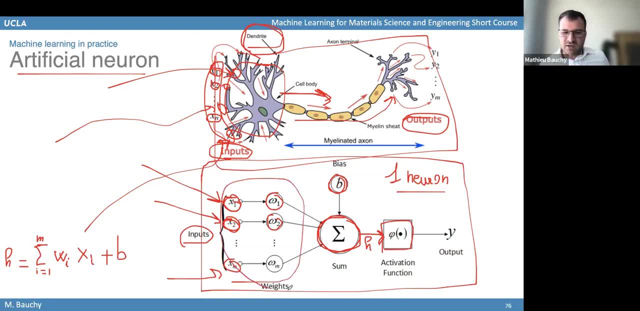 whether this input signal here Is it intense enough that it deserves to be- uh uh propagated to the output, or is it too small so that it should be blocked? So this activation function typically will look like this. So it's going to be a function that we can write five. 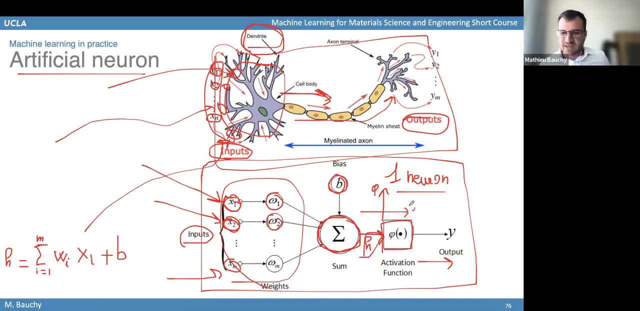 It's going to take as input this uh, viable H that comes after you sum all the signal and add the bias, And then the activation function can be, for example, something, something like this, Something, something like that, where if H is large enough, then uh, the this function. 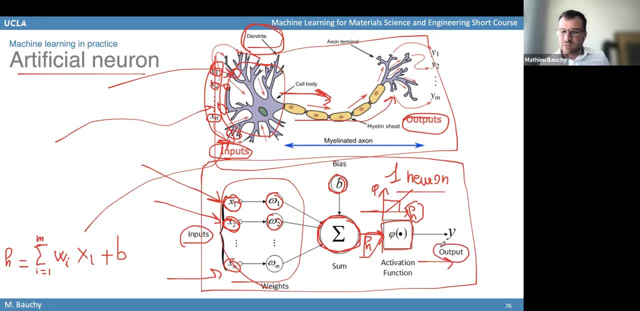 is going to be activated and an output will be generated, But if H is too small, then uh, five is just going to be equal to zero. It means that this neuron is not going to transmit anything. So what this means here is that, um, one way to understand this is that here, this is the 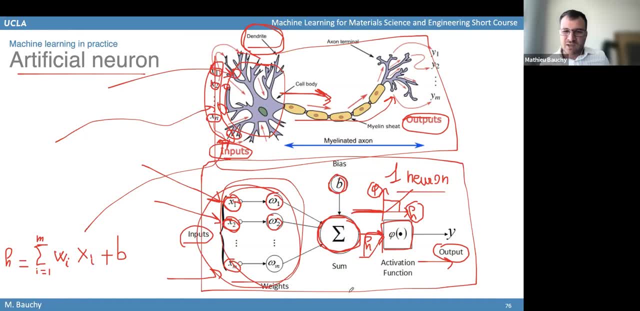 message that you receive from the neuron, The previous neurons, And then uh, you will add a bias to this And then, based on this bias, after you do the, you calculate the sum of all the weighted uh message from the previous neuron. 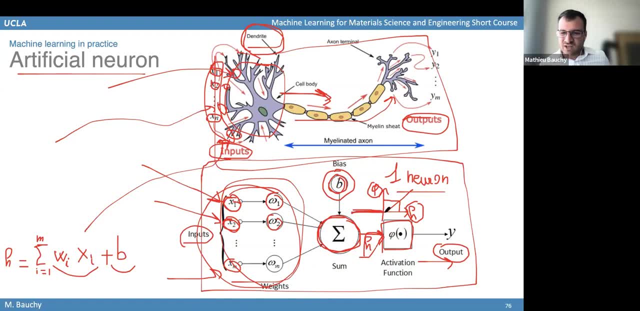 And after you you add the bias, then you will check: is this property, uh H, going to be large enough to activate this neuron? If this neuron is activated, then it's going to generate uh, an output which is going: 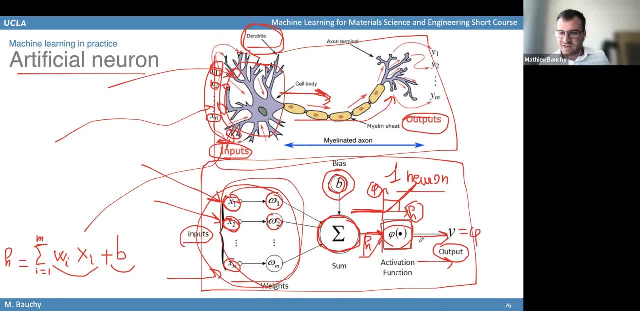 to be the. the value of uh of five is going to be the value provided by the activation function. But if uh H is so small uh that the, the neuron is not activated, then then five is just going to be equal to zero in this case. 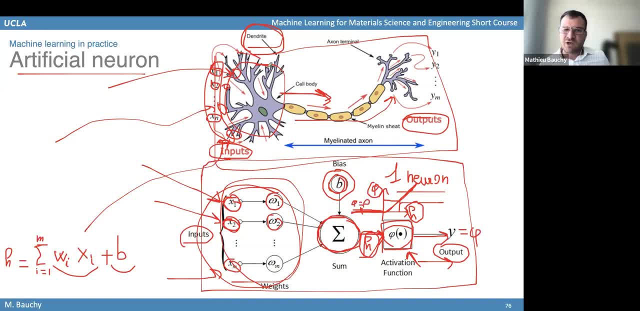 So this mimics the behavior of uh, an actual neuron in the brain where, depending on the value of those electrical signal, either it's going to activate those neurons, It's going to activate those dendrites, or it's going to not going to activate the neurons. 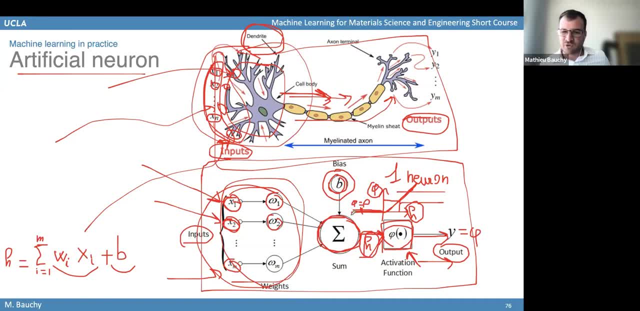 And in that case either it's going to transmit an output, either it's not going to transmit an output. So here the ability for a neuron uh to transmit an output on it. it depends a lot on the bias. For example, if your bias is very large, then even if your inputs here are very small, when 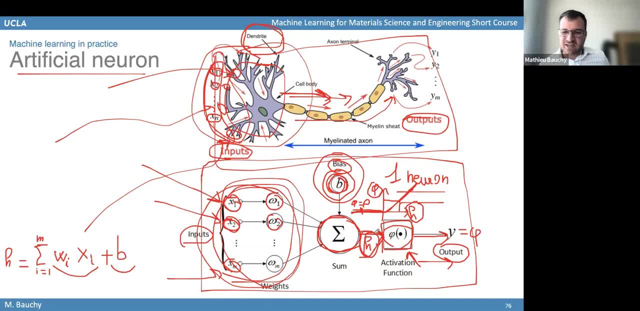 you add the bias, then H is very likely to still become small. Okay, So it becomes pretty large, so that it's it's very likely your uh neurons is going to be activated. But if you have a bias that is very negative then it's going to be very hard to activate. 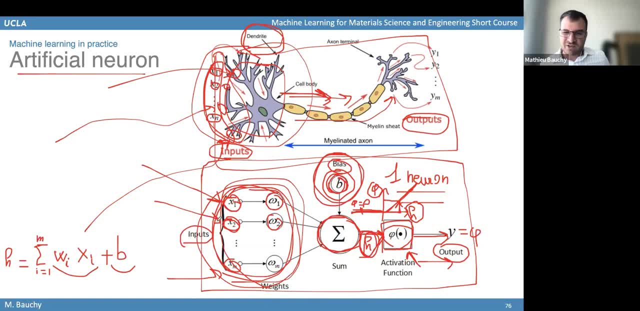 this yours, Even if the input signal are very large, then when you add the bias, if the bias is very negative, you are very likely that your property H is still going to be negative or it's going to be very small, So it's not going to activate the neuron. 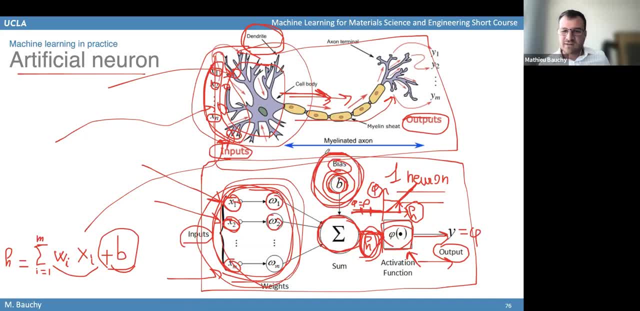 So the bias here uh dictates how easy it is to activate this neuron, Like how big, how intense this um uh input uh message needs to be for this neurons to be activated. So this bias captures, like how sensitive this neuron is going to be. 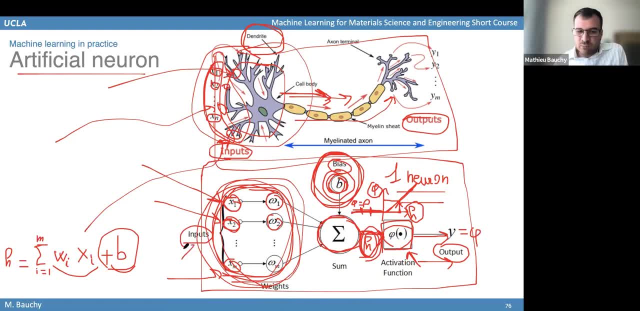 Is it going to be activated even if the input message is very small, or is it going to really, uh, be a very uh, Uh, non-sensitive, uh neuron that really requires a very intense input message to be activated? So this, this neuron is, um the the the sensitivity of this neurons to the input message. 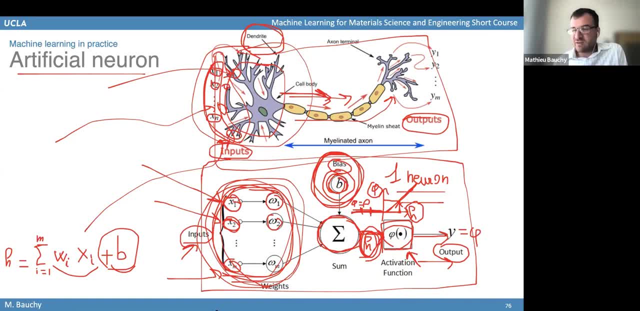 whether it's going to be likely to block the message or whether it has a very high chance to transmit the message. this is going to be dictated by the bias, And then And then the. the advantage of this is that, since this neuron can either block the message, 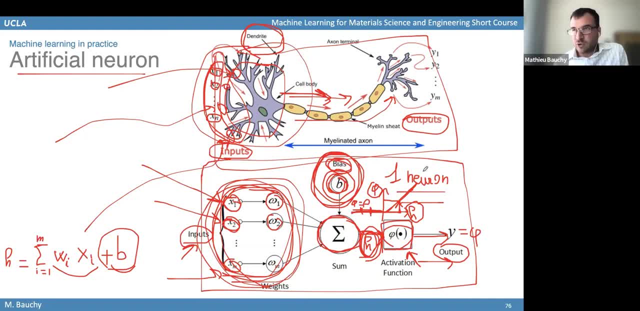 or transmit the message, then you can get some nonlinear response. because if, um, if you were simply taking the inputs here, multiplying them by some weight, I think, some bias, then what you would get is something like this: which is the same as a linear, uh, linear. 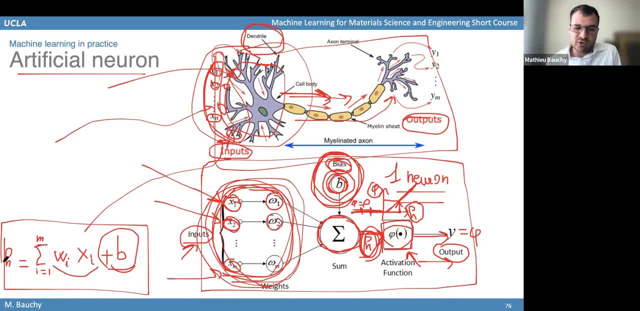 model where you just take a linear combination of the inputs, Put some weights, add a bias. that would be a purely linear model, So that would be the same as a linear regression. But since now you have this activation function that can either let- uh, that can either block. 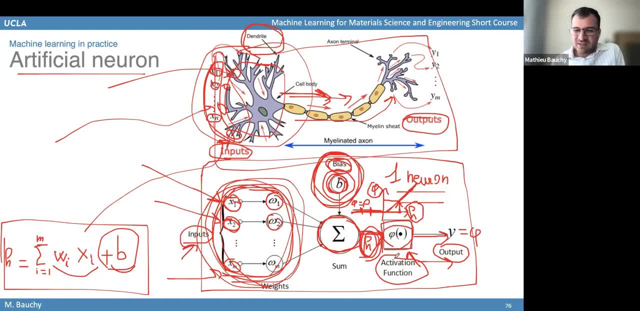 the message or let the message go through. this is where you can now have some nonlinearity and you can end up with a nonlinear model where the, the output, will not simply be a linear combination of the input, So altogether like w. with this combination, like each neurons will be able to take some 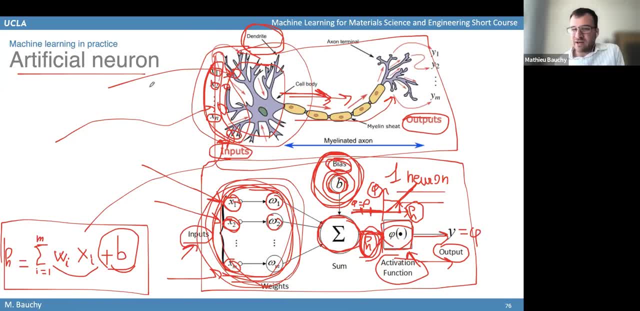 inputs. then uh analyze those inputs, combine them with each other with some weights, add the bias, then um uh feed that to the activation function and check, based on the activation function, If this uh neuron is going to transmit uh another signal or if it's going to block. 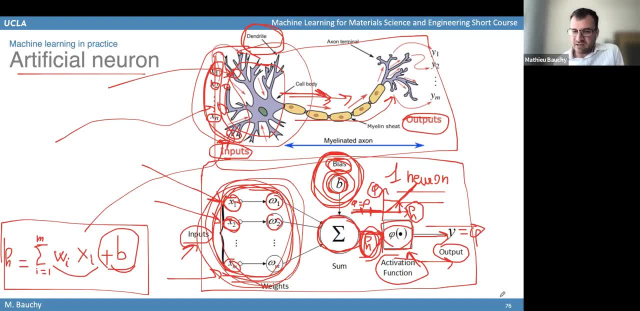 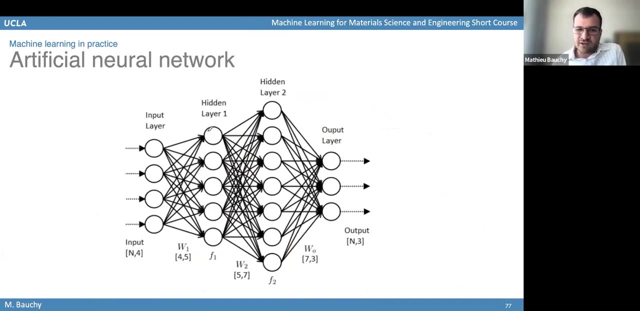 this signal And this is what is going to be the basic idea of the, the neuron. So the base idea is that you will take those neurons and you will combine a lot of neurons together inside a network. So now the, the base idea of a neural network is that you are going to, uh, use a large 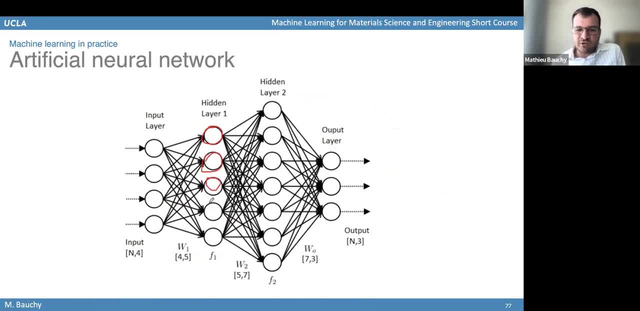 number of those neurons where each neuron is going to behave slightly differently, with different weights, different bias, et cetera, And you will have a combination of, uh, a network of all those neurons, And this is what is going to be used to transmit the input to the output. 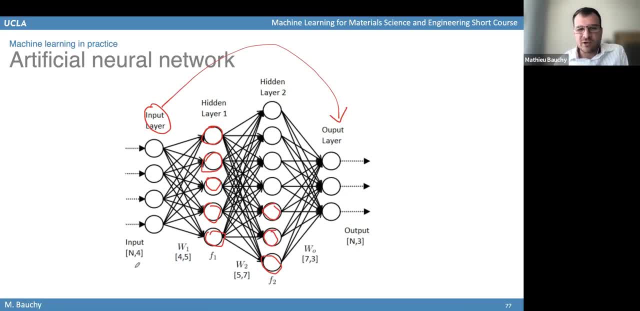 So here. so when you look at this types of network, there is uh, it's organized within layer, So you have a uh, a first layer here, second layer here, third layer here. So the, the, the first layer is going to be what we call the uh, the input layer. 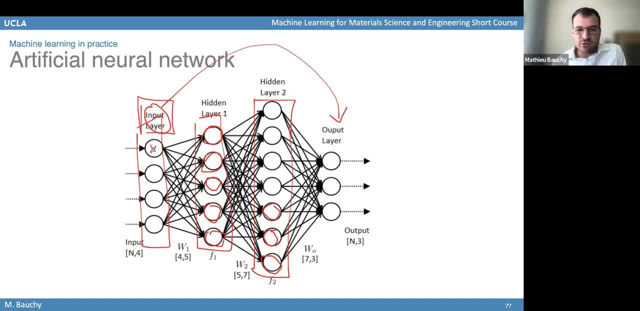 So this is where you will have the um, the value, Okay, Of the, the fingerprint. So if you have the, the fingerprint of your material, so you have the the different features. this is what you will put here for each material. 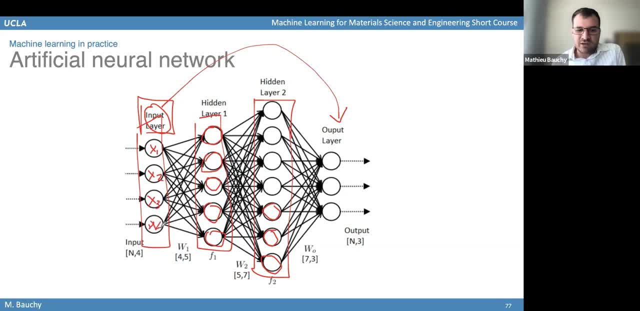 You will have the value of this uh material, Uh, you will have the value of the features for each material. So this is where you have the, the fingerprint. Then each of those um input layer. they will be connected to some other neurons. 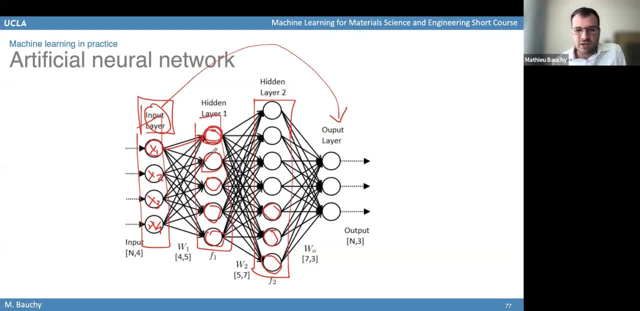 So this is where you start to have some um, some neurons. Okay, So each of the neurons, it's connected to all the um, the uh inputs of the fingerprints, And so each of those neurons here will attribute some weights to the each of the inputs. and 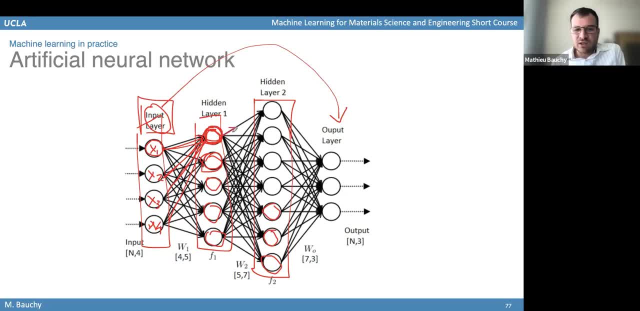 we'll have a bias And based on that, it will um uh, transmit a signal to the to the following uh neurons, Then this information is going to be transmitted to some, all the neurons here, Uh, neurons of the second layer. 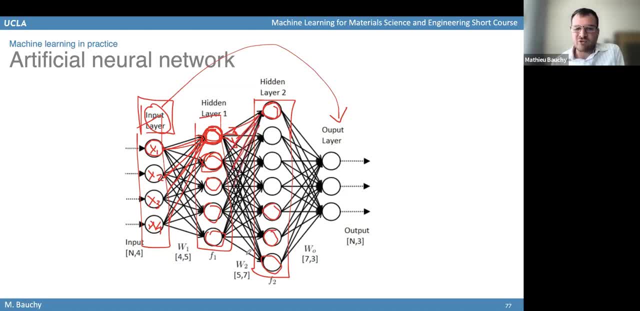 And so those neurons, again, they're going to receive the information from all the previous neurons. They are going to combine those information at some weight at the bias and then themselves they are going to decide if they are going to um transmit the information to the next. 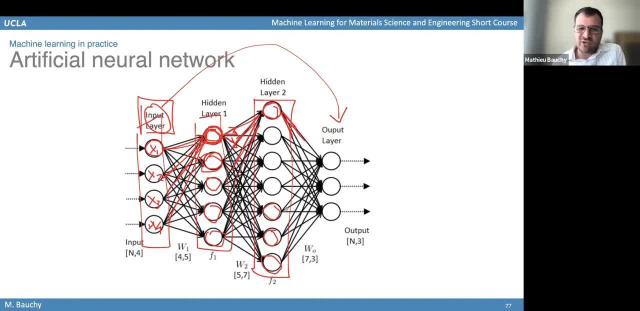 neuron And then. so what you have altogether is a series of neuron like this, where each neuron can decide to either transmit the information or block the information, And at the end, what you get here is the- uh, the output layer. 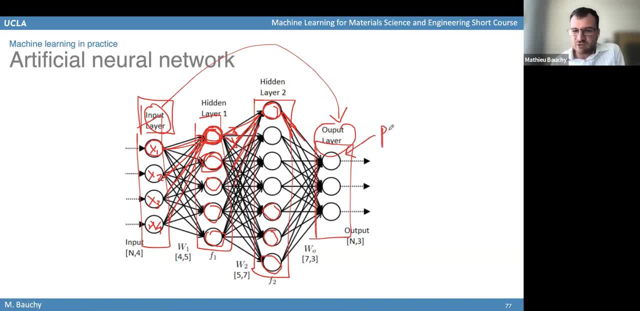 So this is going to be the list of the properties that you want to predict. So that's going to be property number one, or a property number two, property number three, et cetera. So that's that's going to be the final um layer that contains the priority that you. 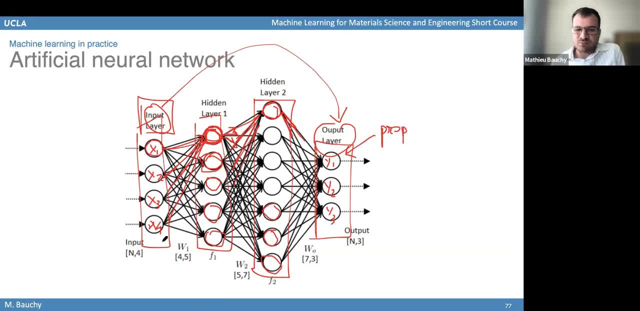 want to predict. So this is, this is, um, how it's going to work. You provide as input- Okay, So this input, the value of the fingerprint for each material. this input is going to be transmitted neuron by neurons, through layer one, layer two, et cetera, until eventually. 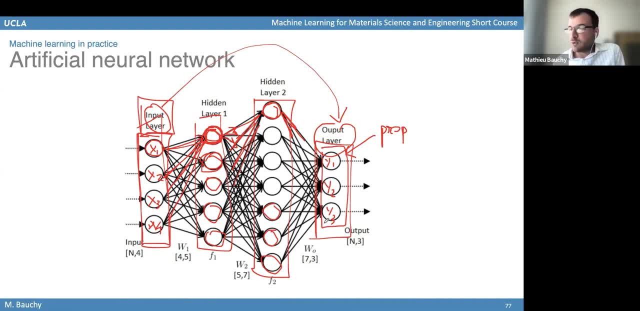 this gets converted into the um, the final output, which is going to be the, the value of the priority that are predicted for each material. So, for each material, it has one value for the fingerprint. So it's going to give you one value of the, the predicted priority. 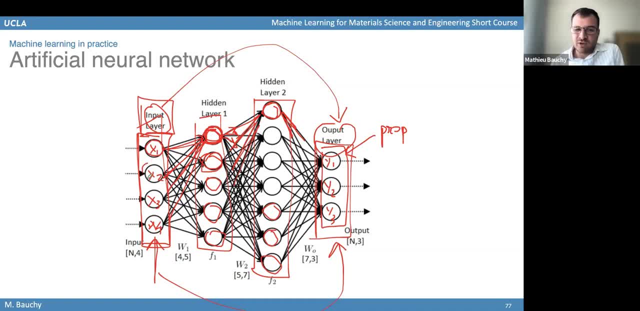 And every time you have a different material for which The value of the fingerprint changes, then it's going to change also the, the predicted property, in return, since the signal goes from the left to the right here, So it's it goes. if you change the, the entry signal here, then it's going to change the. 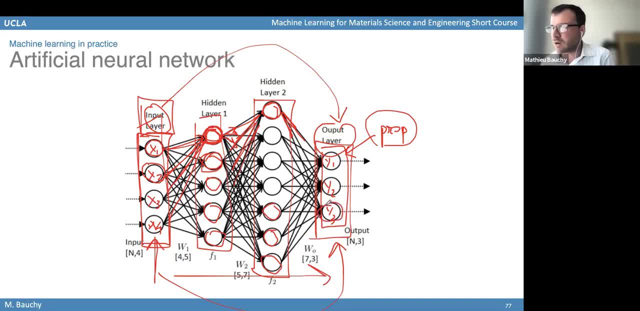 uh, the output signal on the right- So that's the main idea of how a neural network works- is just: you start with the fingerprint on the left, Then you connect that to a large number of neurons, Just like you would have in the brain. 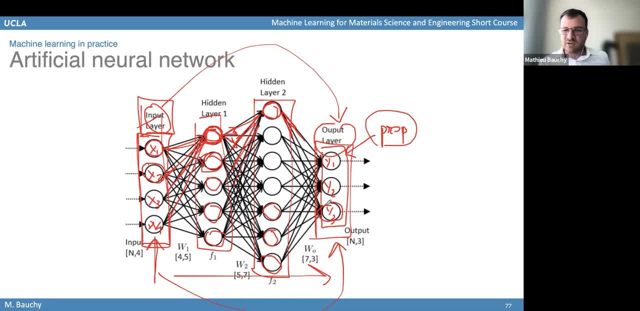 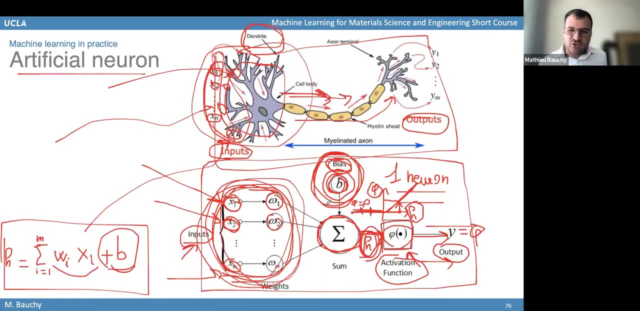 And, at the end, what you get as an output is the priority that is predicted by this network. Do you have any questions regarding that? So then, if you look at each um, each neuron, so here you have some parameters you have. 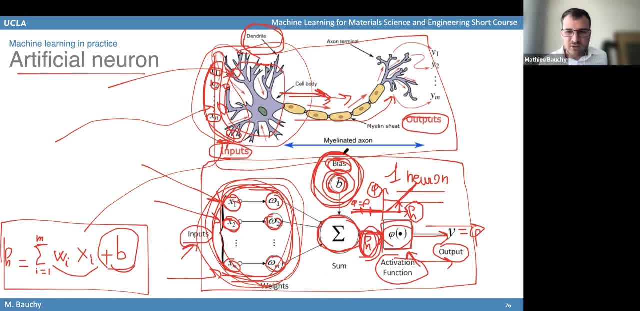 the weight associated to each signal and you have the bias. Okay, That those are going to be the parameter of the model. in the very same way that in a linear model you need to adjust the slope and the intercept. You have two, two parameters that you need to adjust in a linear model. here in a neuron, 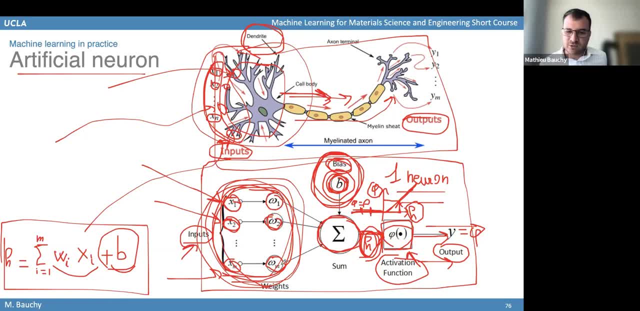 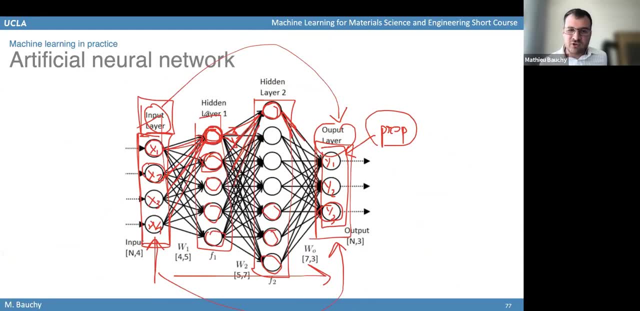 you have all of those parameters like W1, W2, WN and the bias, And you need to. you have this for each neuron. So for each of those neurons, you will have, um, uh, some parameters to obtain. 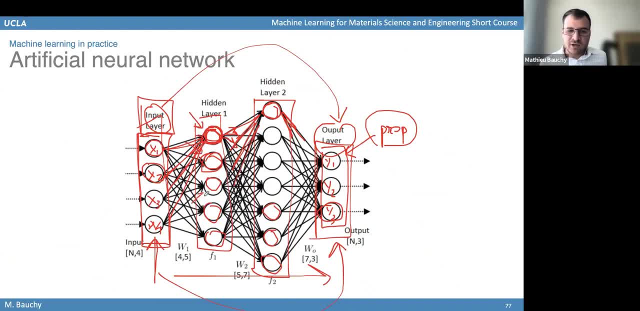 Okay, So here in an artificial neural network, you have a lot of parameters. You can have a hundred thousand or maybe millions of parameter. that needs to be optimized And that's the process of training, um, uh, a neural network. When you, when your neural network is going to stop learning how to transform the input. 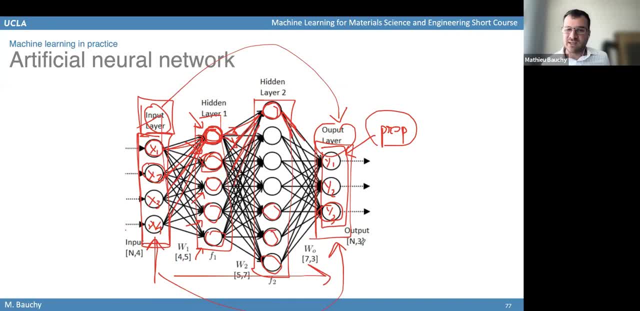 fingerprint into the output priority that it wants to predict this process. you need to train the model, You need to adjust The parameters, uh the weights between the neurons in order to teach this network how to convert the input, uh fingerprint, into the output property that you want to predict. 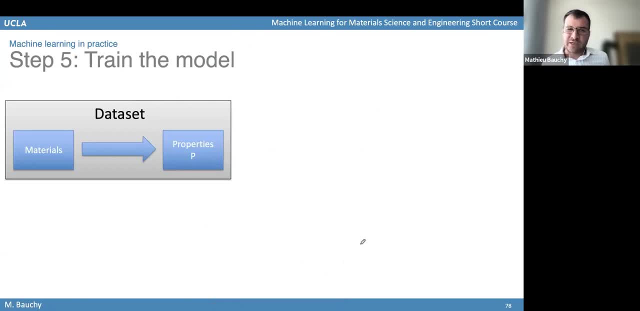 So that's going to be step five, Like: once you have chosen your algorithm, then you need to train it, and training the model needs that. you need to adjust the value of the parameters of the model so that that's what it is. So the idea is that you have your data set where you have the material as input and 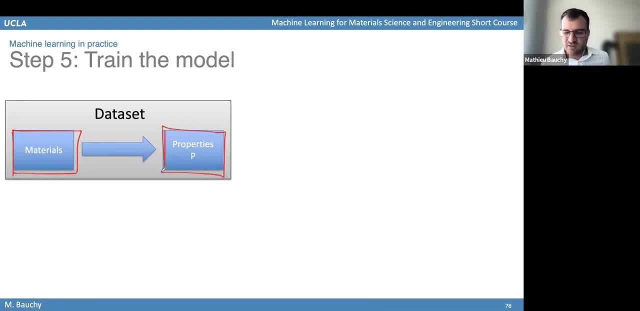 you want to predict the properties, uh, of those materials that output. So the way it works is that, starting from the material, you determine what is the fingerprint. So this is the fingerprint that described the material, And then you have your machine learning model that converts the fingerprint into the property. 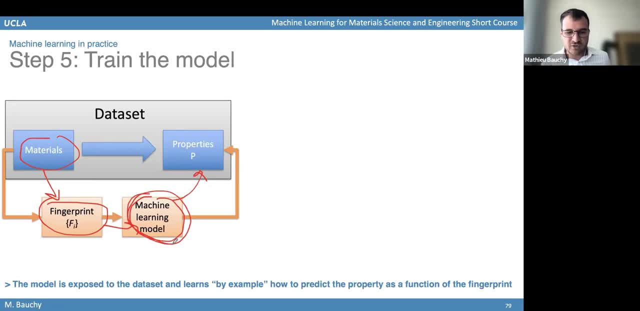 And this is what you need to train. You need to adjust this machine learning model so that it can successfully map, uh, the, the fingerprint, into the, the priority. So, if, if you are, your machine learning model is simply a linear regression and it means 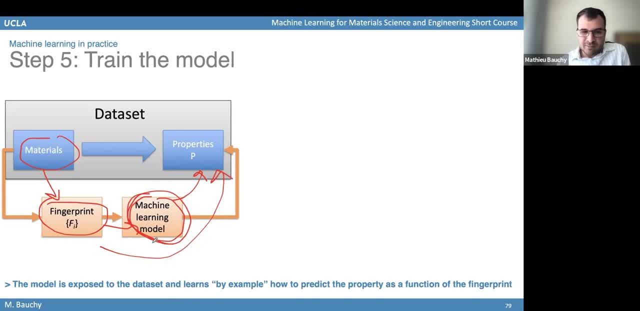 that now you need to find what is the best value of the slope or what is the best value of the intercept that you need to use to convert the input fingerprint into the output properties. If you are using an artificial neural network, then it means that you have your features. 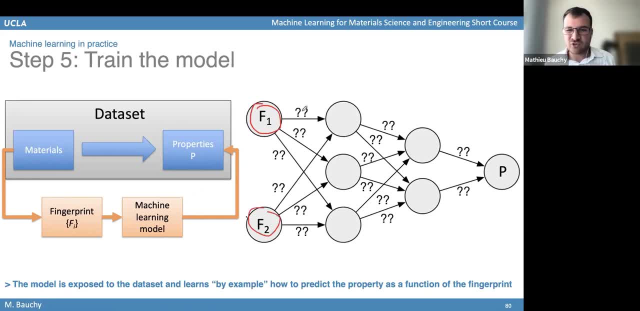 here And uh, you need to uh adjust the weight associated to each neuron. Like every time, you have some neurons that are connected to each other and you need to uh adjust all those weights here. So that's the. the model gradually learns how to convert the the the input features. 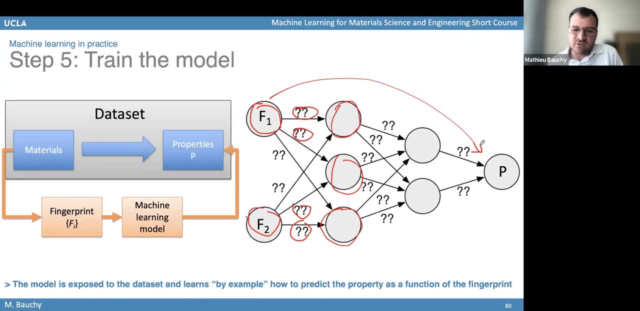 into the um output features. So that's what that's the process, That's what a process is of training a neural network, is that you are going to gradually adjust all of those um weights here, all of those parameters, in order to find uh. 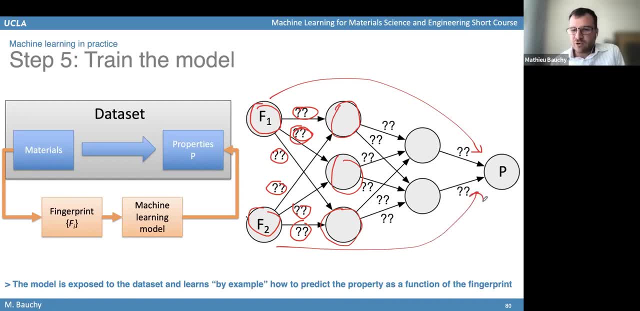 an, an ideal network that can convert the, the input, into the- uh, the output. So that's the process of learning And, again, the way it's going to work. Okay, So the way it's going to work is: uh, you're going to learn by example. 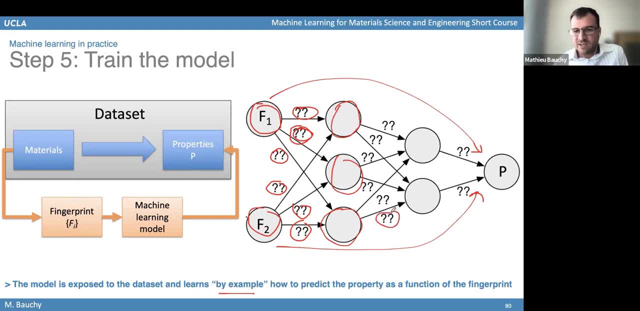 It means that initially, you will make some initial choice about those parameters and then you are going to define um a cost function, just like what we said before, like a cost function that describes how good your model is, And then you're going to start adjusting all of those parameters here in order to def. 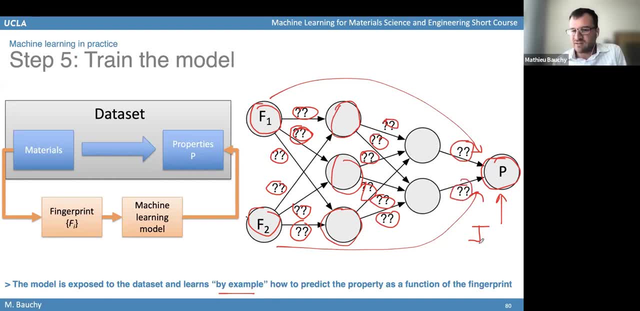 to decrease your cost function. So you have your cost function that characterize How close your model is to the actual data points that you have, And then each of those uh parameters here is going to be adjusted so that the the prediction for your model is as close as possible to the actual data points that you have. 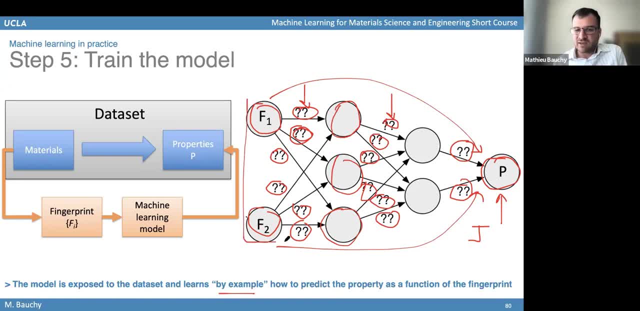 So, for it means that, based on the example of the metal that you have, you have their fingerprint, You also have the corresponding property for those materials. So then you are going to try to, Then you are going to try to find what are the best value of the parameters that make 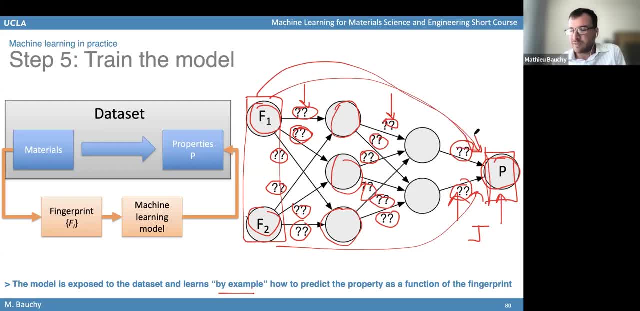 it possible to convert the fingerprint into the property based on the, the, the data points that you already have, And so this process of adjusting the um, the parameter, this is called the, the training uh of the of the model. 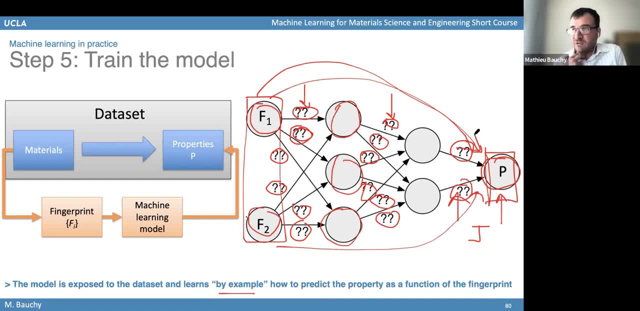 So this is where you adjust the, the, the, the, all the parameters, and, and the way you would adjust those parameters, Exactly what we described before. using the conjugate gradient method, you calculate the cost function. calculate the cost function, that, um uh, describe how good your model. 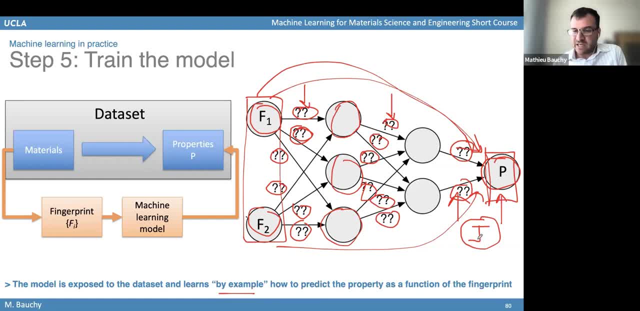 is, And then you are going to calculate the derivative of the cost function with respect to all of those parameters And then you will start adjusting the um, those parameters, to decrease, uh, the cost function. So you would calculate the derivative of the cost function with respect to each of the 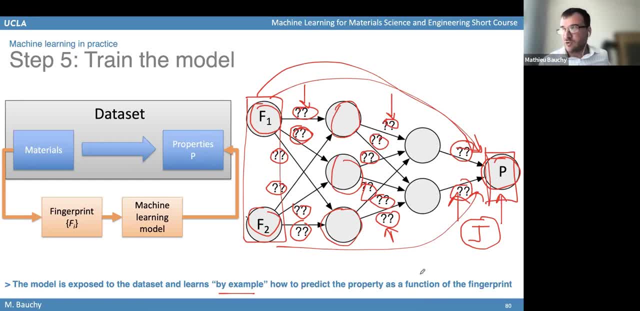 cost function with respect to each coefficient And then you gradually adjust those coefficients towards the the negative gradient direction. You calculate the gradient and then you adjust the parameters towards the negative gradient direction to try to decrease as much as possible the cost function, to decrease as much as. 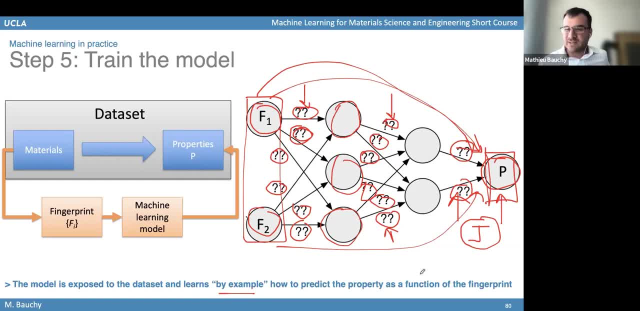 possible the difference between the, the predicted, the property that is predicted by the model, and the property that you that are, uh um, the, the, the real cost function, The, the- the real property that that are in the, in the data set that you are using? 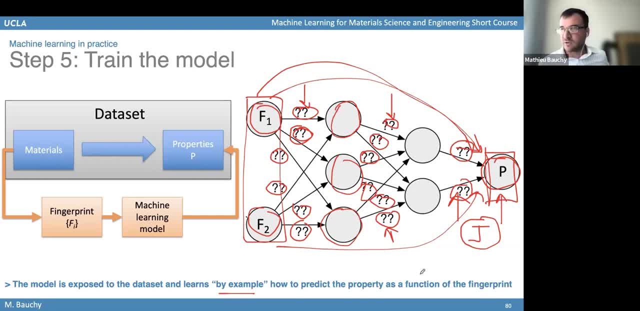 to train this, this model. So this is the process of training a model. In every model- machine learning model- you have some parameters and you just need to change those parameters in a way for your model to be as close as possible to the data. 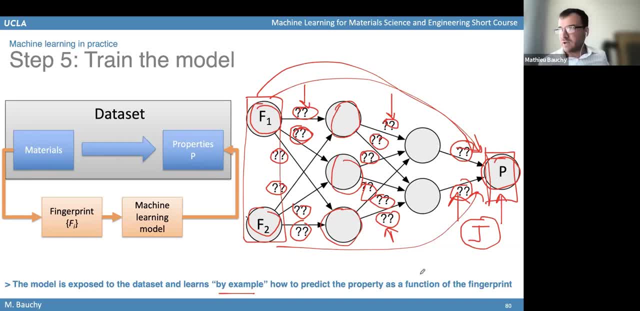 points that you have in your data set. So that's what it takes to to train a machine learning model. This is about adjusting parameters. Do you have any questions regarding this step five, which is about training your, your machine learning model? 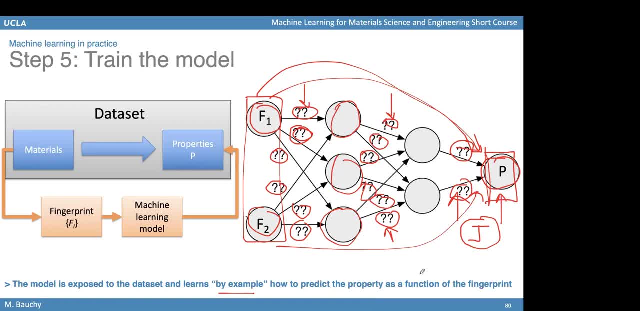 Professor Mathieu: Yeah, What are? what does the number of hidden layers depend on? So, yeah, so this, this is going to be, I think, uh, the the next step. So let's, um, I'll talk about this in, um, in, uh, in a few, uh, a few slides, but basically, 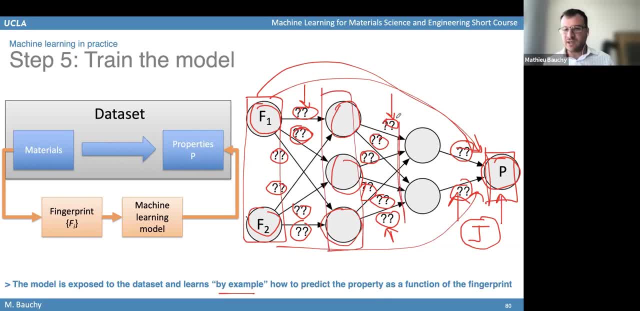 here There's two things that matters. There is how many layers are going are you going to choose? And then a second thing is: how many neurons per layer are you going to choose, And this is something that that needs to be optimized. 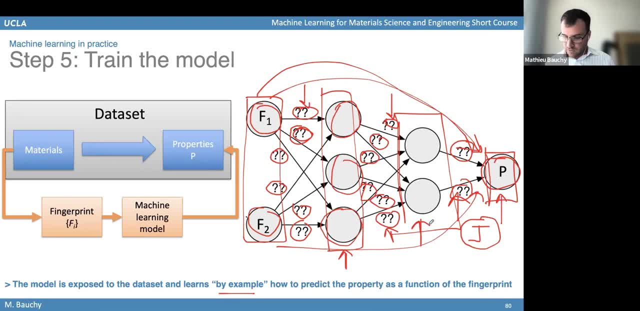 Like when you, once you have chosen uh, a given uh learning algorithm like artificial neural network or random forest, then you will need to adjust some additional parameters that those are what we call a hyper parameter, Um the uh. this is to differentiate the parameters from the model that are, for example, 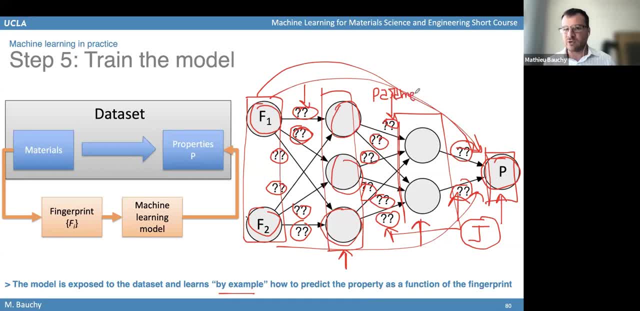 the, um, the, the weights, like the weights between the neurons. This is what we call the parameters. And then you have something else, which is the hyper parameter. The hyper parameter are not parameters that are going to be trained, uh, during the training. 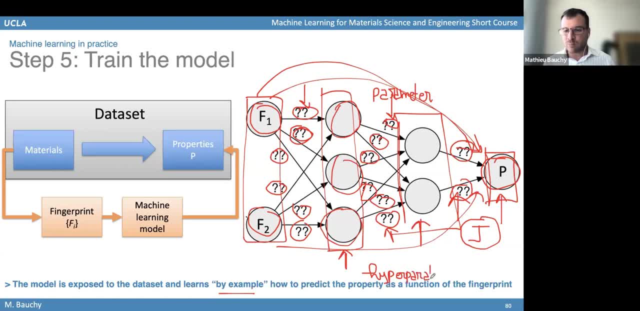 of the model, but there are some parameters that dictates how complex your model is. For example, one hyper parameter would be: how many layers do you have? Another parameter would be: how many neurons per layer do you have? So those are some parameters that describe the the complexity of your model, and they 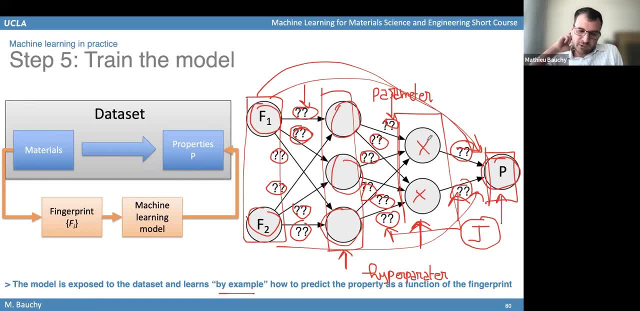 also need to be optimized, And so we're. we're going to talk in a few slides on how you would do that. How do you select the best uh value for those hyper parameter, But the basic idea is that when you train these types of model, 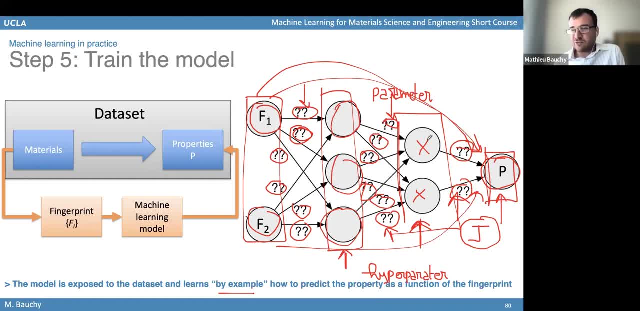 You want your model to be complex enough so that it can capture the relationship between the input and the output, but you don't want this, this model, to be too complex. If you use too many layers here, or too many neurons per layer, then your model will become. 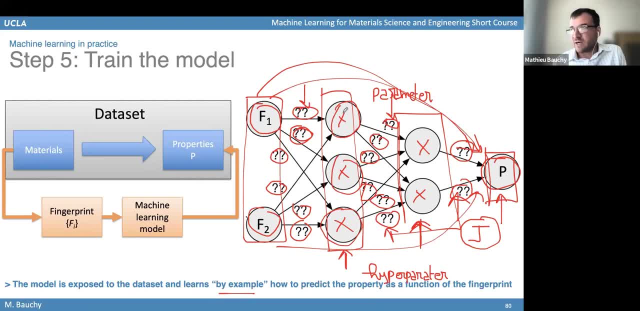 too complicated And that's going to be very hard to train. such a complicated model- And a very complicated model- is also going to be likely to give sometimes very crazy predictions. I'll talk about this and explain why in a in a few slides, but but basically when 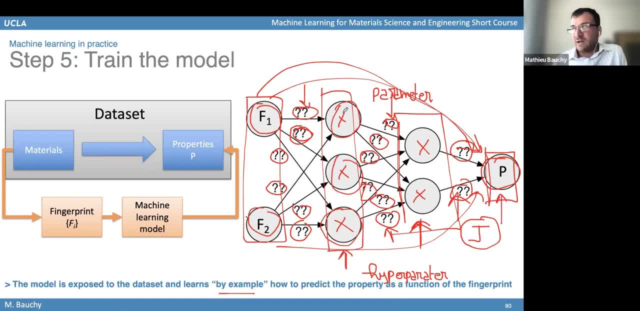 you come up with a new model, you will always try to find what is the right model: complexity, to have a model that is not too simple but also not too complex. And this is going to be about, uh, optimizing the, the hyper parameter, which is going to 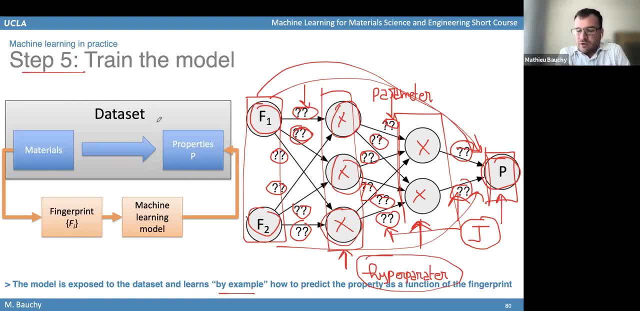 be, uh, an extra step after training the model. So, uh, let me know, uh, I'm going to talk about this in a few slides And, if it, If it did not answer your question, uh, feel free to ask again, and, um, we can talk more. 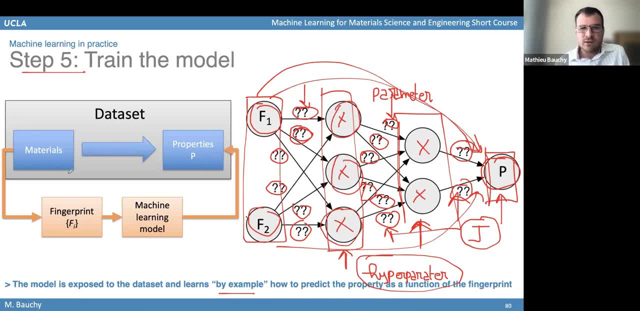 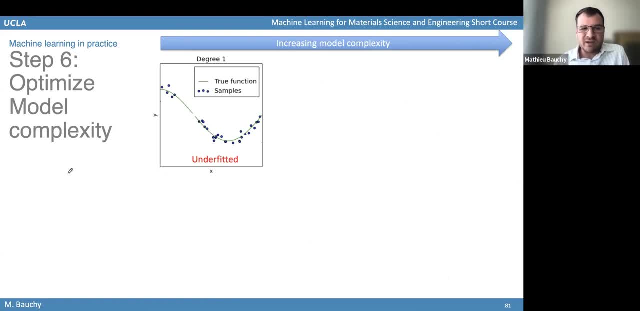 about this, Okay, So there, so let's talk about the. so this is the next step. So this is step six. Now it's about optimizing the model complexity. Optimizing the model complexity can mean different things. For example, if you are using polynomial regression, you have to choose whether you want a linear 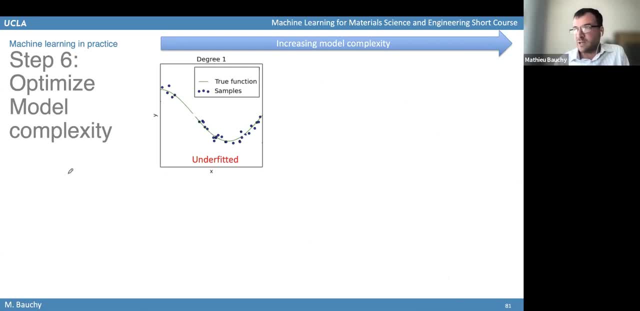 model, or a quadratic model or a cubic model. So this is different degree of complexity. If you are uh dealing with a neural network, then you need to choose how many layers do you want and how many neurons per layer do you want? 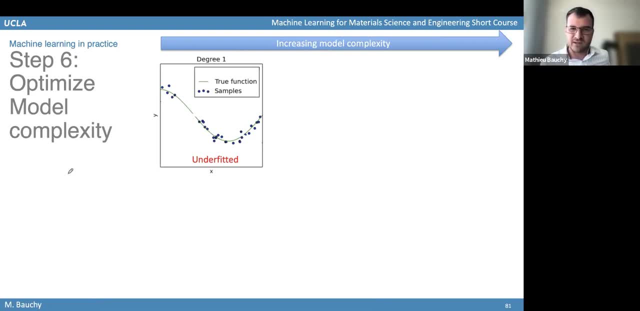 That's also something that dictates the complexity of the model. So, uh, this step six is very important because it's about deciding what is the right degree of complexity that you need for your model. So let me show you an example to illustrate. 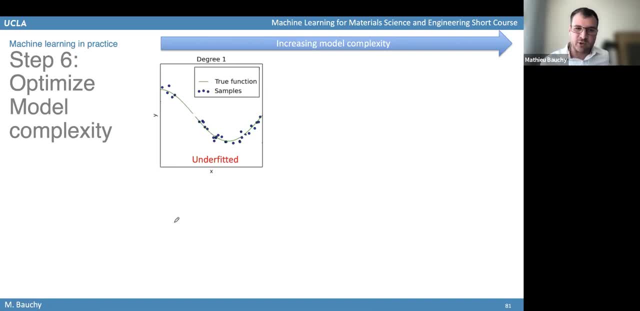 Uh, why the complexity of the model is important and how, in practice, we would determine the optimal complexity to use for a given uh model. So here, what I'm representing is, you have this, this green line here. This green line is the true function. 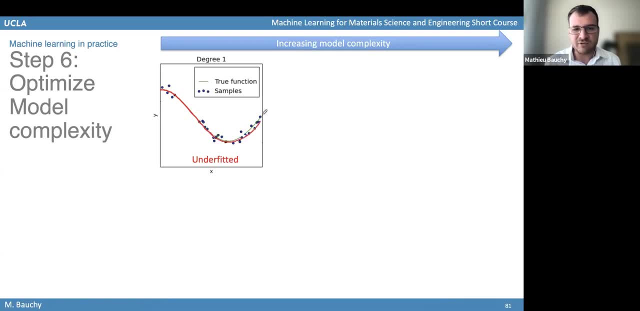 By the true function I mean that if you have um some input, X, so that's the, the fingerprint of your material, Like it's composition, Then, uh, there is a true function that tells you how the composition, uh, of the material. 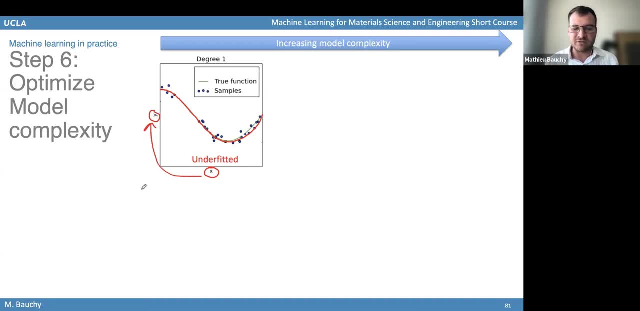 X is governing the property of this material. So there is a true function, which is the true physical or the true chemical law that relates the composition of a material to its property, The premise that we don't know what this function is. So this, this green function, we never know what it is. that that's what we want to find. 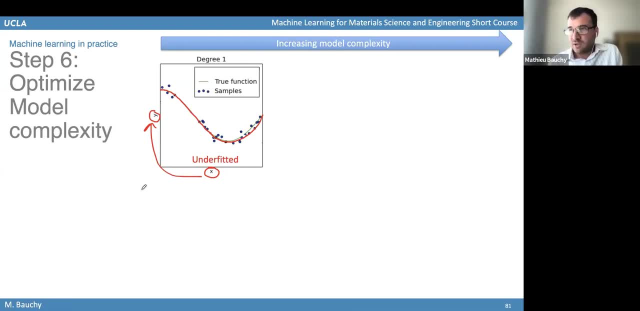 using machine learning. So this true function, uh, we, we don't know what it is because we don't have, uh, any physical or chemical knowledge about the relationship between input and output. So this is what we want to find. Our goal is to find this green function. 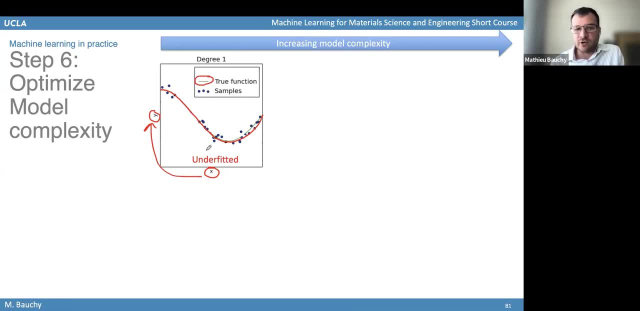 This is the true function. This is what we want to find, but we don't know what it is. All we know is we have some example. We have some data points here. Those are the blue data points. Those are the points here. 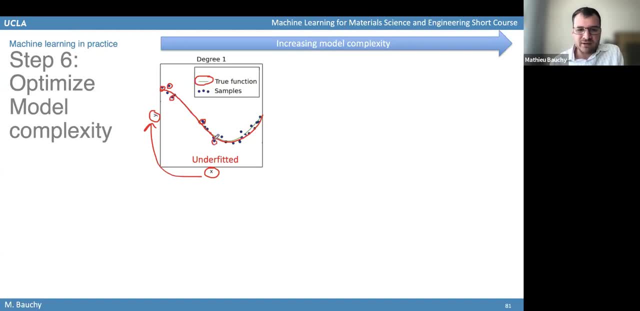 Those are some measurements where, for example, materials with different composition or different process, uh, different manufacturing method, What you did is that you took those materials with different composition and you measured their property, Why. And so when you do a measurement, you will not get the true function because, like every, 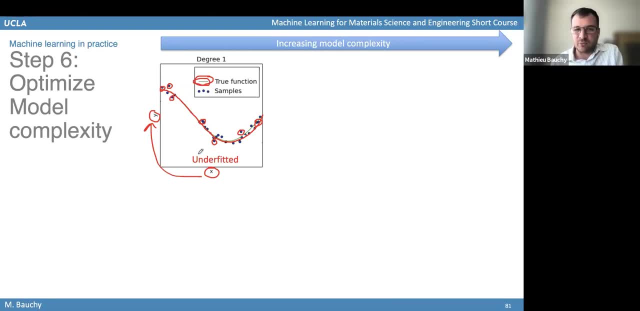 time you do an experiment, you get some- uh, you will get necessarily some, some noise. So, uh, uh, a measurement can never Be 1% accurate, So you always get a little bit of noise every time you do a measurement. 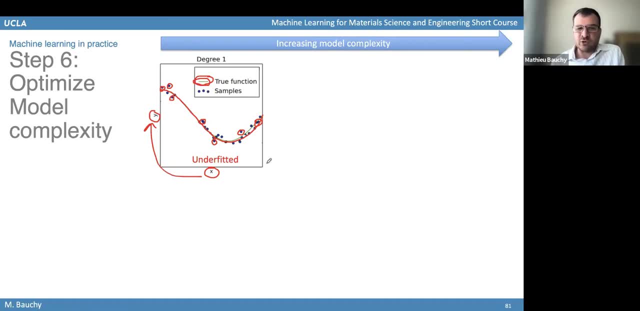 So what you get, uh, as information that you can use for machine learning, is never the true function. You just get some, some samples, some experiments, some measurements, that is, uh, an approximation of the true function, And so, based on this, your goal is to find what is this green true function and how complex. 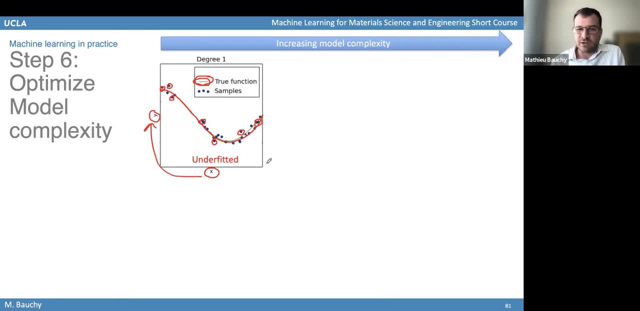 should it be? Do I need a very complex model? Or, uh, do I? can I represent this with a very simple model? So, for example: uh, here let's assume that we are going to use polynomial regression, just because it's easier to understand. 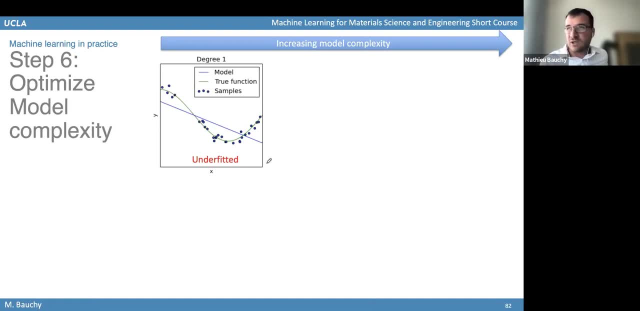 So initially maybe you will think that, um, uh, a linear model with degree one, uh, is good enough to represent this, uh, this information, to represent the relationship between input and output. So, or an equivalent for this would be to choose uh in your artificial neural network. 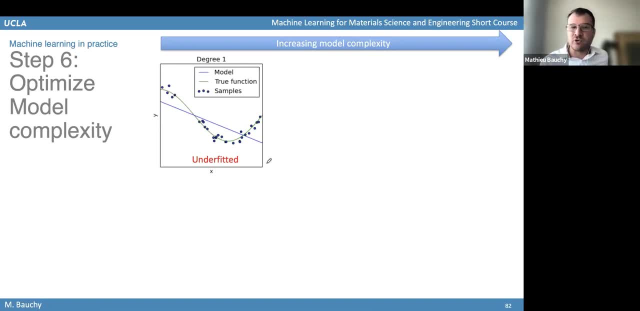 you would choose maybe only one layer and you would choose a very small number of neurons in this layer. So that would be an example of a very simple model. A very simple model will typically look like this: It's just going to assume a linear relationship between the input and the output. 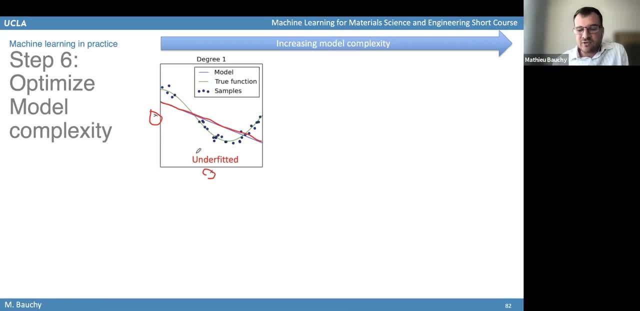 So here, if you look at this model it, it looks like it's too simple. It doesn't really capture the detail of how the, the property of material, is changing as a function of the input. And I mean it's, it's not. it's, it's not the same as the true uh green, uh function. 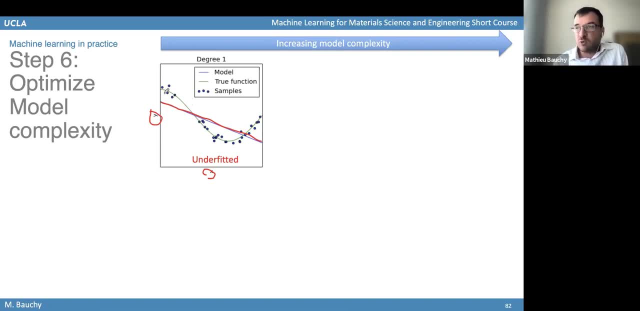 here. But again, we, we have no way to know that because we don't know what the green function is Like, we don't know what the true relationship is. If we knew that then we would not need machine learning, but still like here. uh, this is. 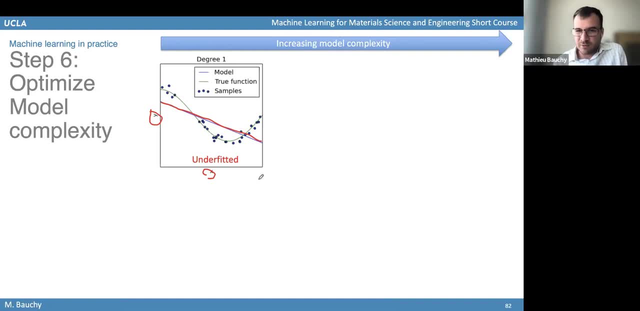 not going to be a very good model because it's too simple. On the other hand, you could also use a very complex model, Like: if you use a very complex model like here- that's an example of a polynomial regression with a degree 15, then this model is going to be like very accurate. 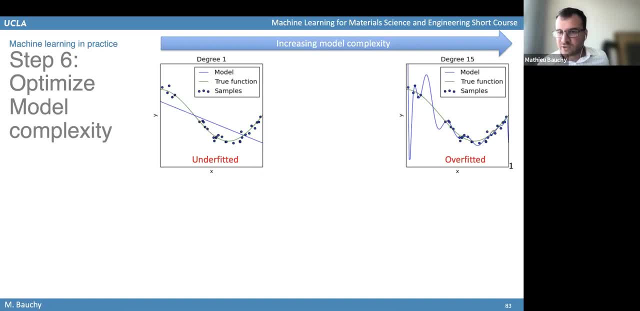 Like it's going to be, like really going through each of the of the data points very perfectly, because it has a very high number of parameters. So you will adjust all of those parameters in order to really minimize the difference between your model and the experimental data points. 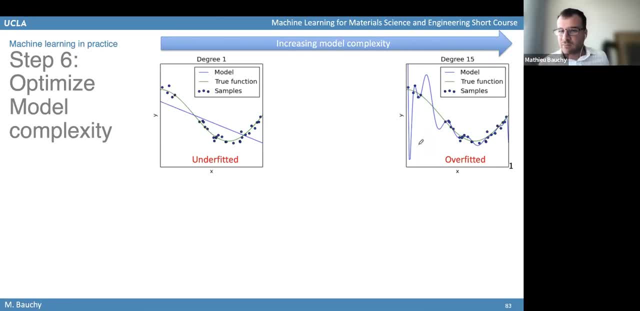 And that's going to give you something like this, where your model goes very accurately through all of the data points, which is not surprising because, again, in machine learning, this is really what you're trying to do: You're trying to minimize the cost function. 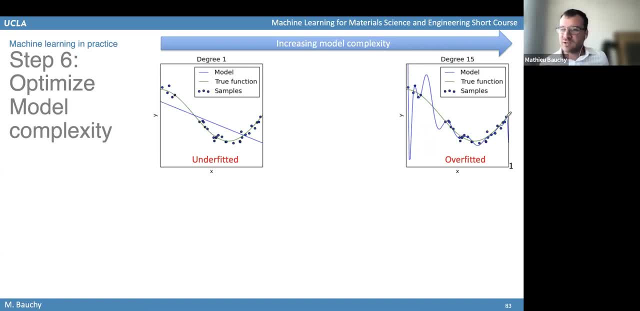 You are trying to minimize the distance between your model and the data points. So here this is the function that uh, uh really minimizes The distance between the um, your model in blue, and the experimental that I point in uh in blue here. 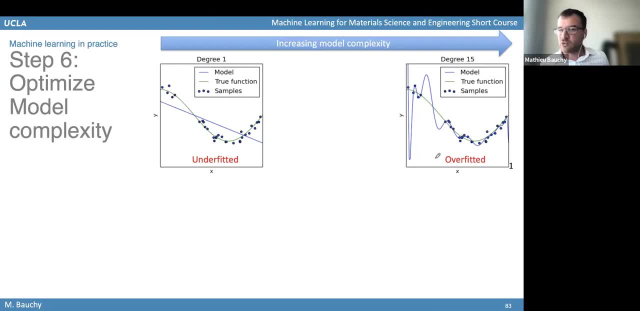 So but like, if you look at this model, it's, it's, it looks like it's too complex, Like it's fluctuating a lot, So it's not. also, it's not a good representation of the um, the, the, the true green function. 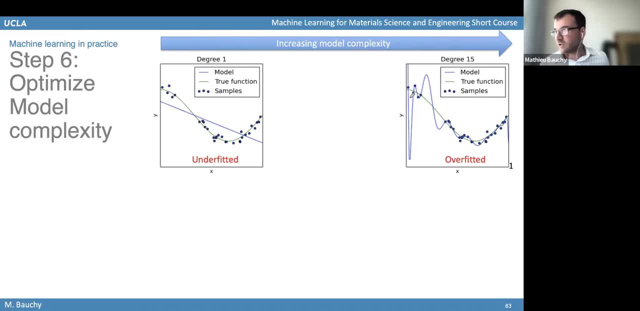 But again, we don't know that because this green function is is hidden, Like we, we don't know what this is, What this green function is, So, uh, but the the only thing that we can know is that if we look at this model, it looks too complex. 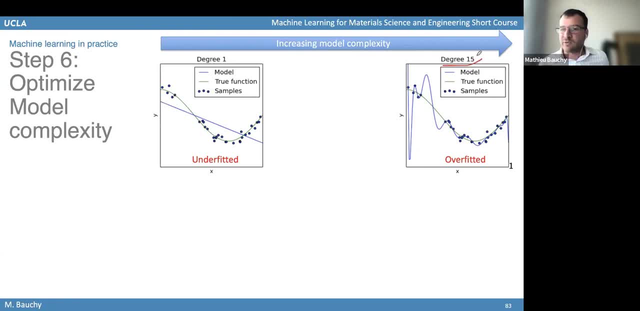 So this is what you would get if you use- uh, polynomial regression with a degree that is too high, Or this is what also what you would get if you use an artificial neural network with too many layers or too many neurons per layer. then you will tend to have a very complex model like this. 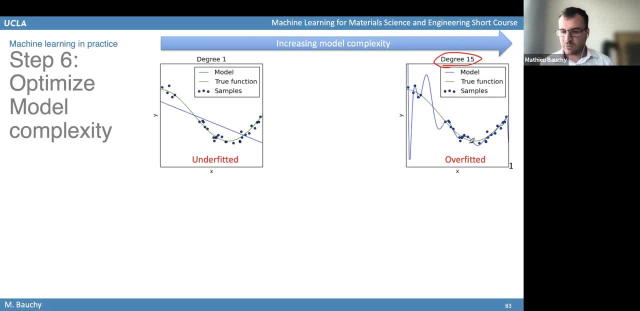 So what you want here? You want to find the optimal model that is not too simple but not too complex. So, for example, in this case, a good model would be this: That's a model that would be smoothly interpolating the data points, but without, uh, trying too hard to to really go through each of the data points individually. 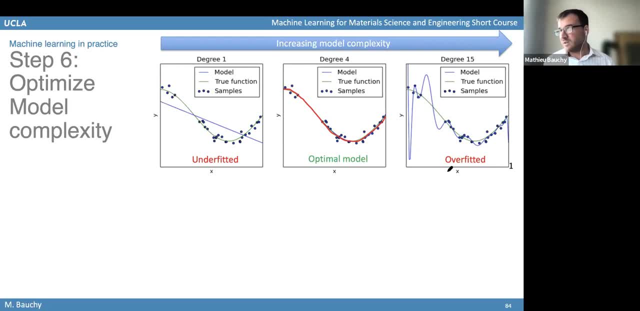 Remember that those data points. they are noisy because, like the um, the experimental data, when you get them, any experiments comes with some noise, So it's um. we should not try to fit all the details of the um, of the of those points here. 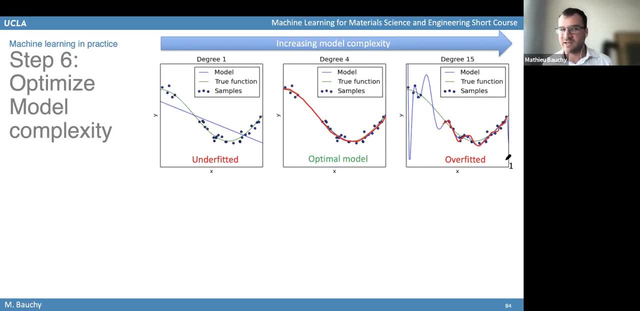 because at some point what you are doing is that you are fitting the noise of the data. You are not just simply trying to find um the best relationship. that dictates the relationship between the um, the input and the output. You are starting when you have a very complex model. 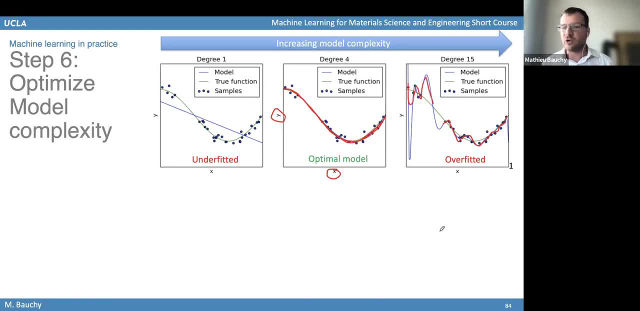 you are starting to really fit the noise of the data, which which means that it's not going to be an accurate representation of the true function. So here, in this case, you see that your model is ideal because it's it's um, describing the relationship between the input and the output. 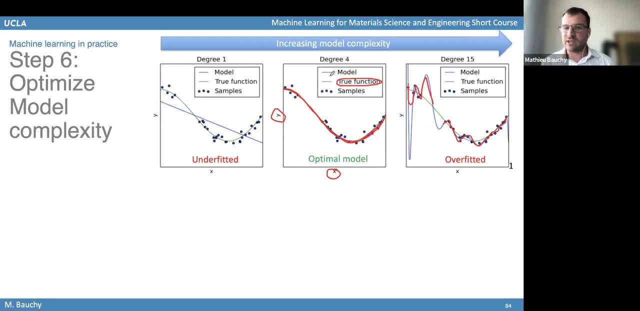 but without being overly complex. And actually this model is is very close to the what the true function is Like. the blue line of your model is in this case very close To the um, the true relationship in green. So this model here would be too simple. 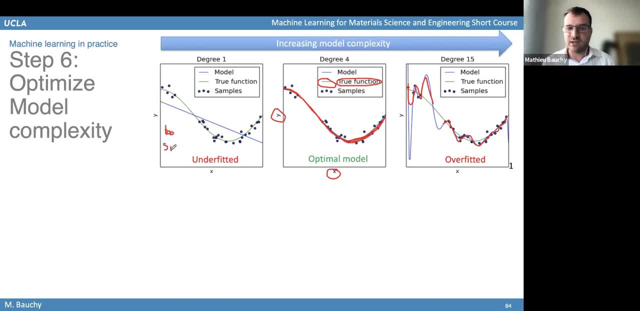 So this one is too simple, So it doesn't fit the data well enough. So when your model is too simple, we call this model, uh, underfitted, So that this is. when the model is too simple. It means, like the the degree in polynomial regression is too low. 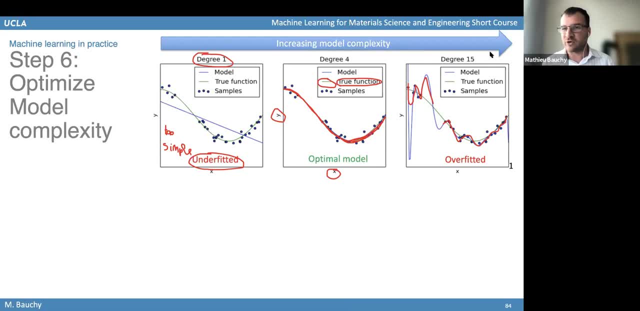 or it means that you are not using enough layers or enough uh neurons in your artificial neural network. On the other hand, here this model here is too complex. It's too complex that it it's. it's really trying too hard to agree perfectly with uh the data points in your data sets. 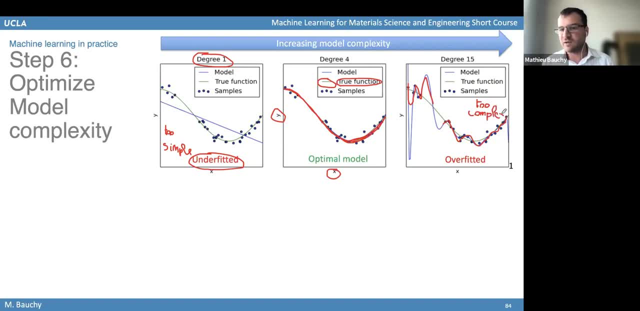 but it's agreeing so well that it actually fit the noise in your data. So in this case this model is too complex. That means the the degree in polynomial regression is too high, or that means that the number of layers, of the number of neurons in the artificial neural network is too high. 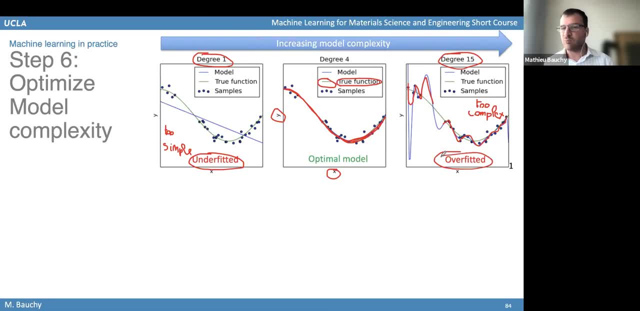 So in this case, that's what we would call uh an overfitted model. It's a model that is too complex And uh, in between, you have the optimal model. That's the model that is the best at uh learning the true relationship between the input and the output. 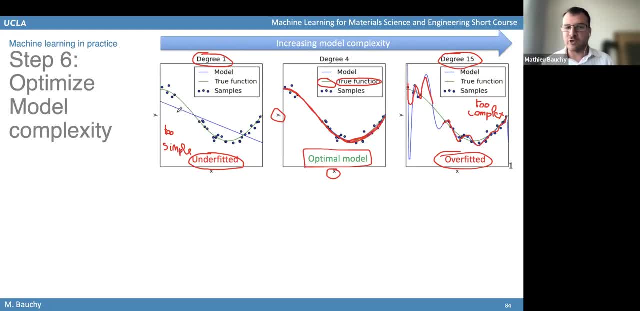 So like, if you think about this uh underfitted model, like why is it bad? It's bad because it's too simple. It means that then if in the future you have a new uh material here and if you want to predict what is going to be the output for this material, 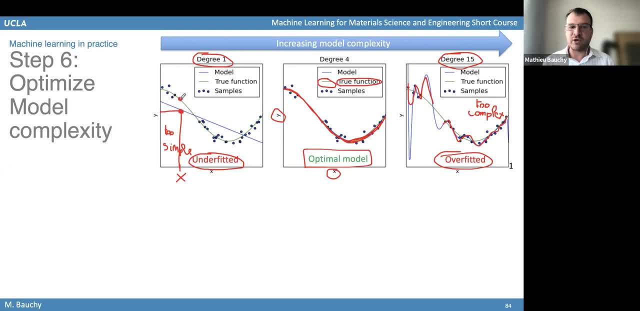 it's going to be something that is far from uh what should be the true uh, the true output, the true property of this material. It's because the your blue model here is too simple. It doesn't really capture the complexity of the relationship between 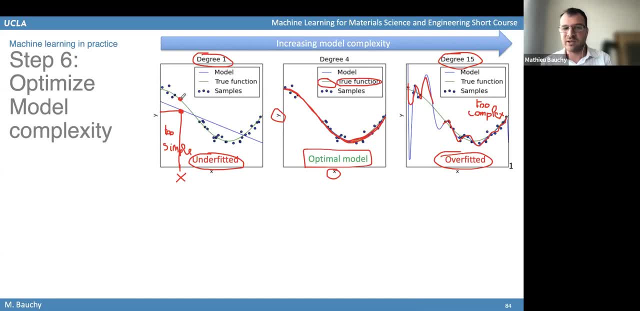 uh, the input, like the material composition, for example, and the property of this material. But on the other hand, having an overfitted model is also bad because, again, like here, if I look at for a given material composition, 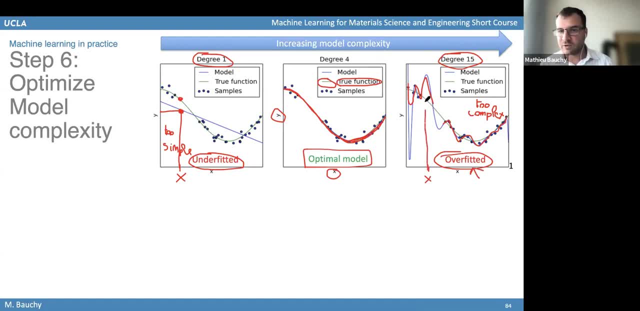 I look at what my uh, the the model is predicting Again. it might predict something completely crazy here. It's something that is very different from what should be the true property for this material. So for both underfitted and overfitted model, 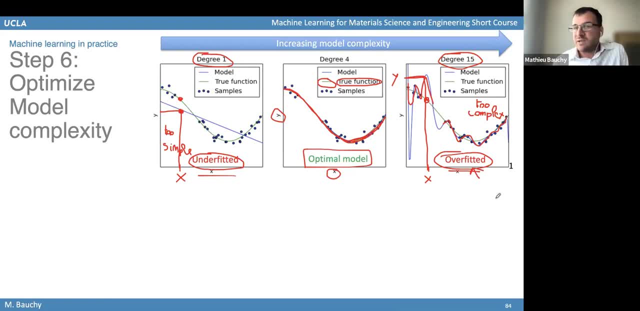 they are both bad because in both cases, uh, even though the overfitted model fit perfectly the the point that you have in your asset, it's actually bad because it means that when you will use this model in the future for some new materials that the model has never seen, 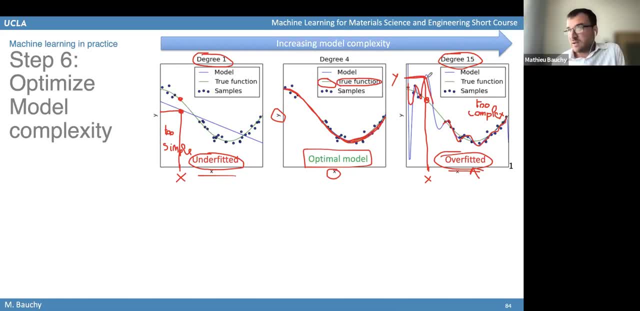 this model will not be able to generalize very well It's. it's going to be good uh at uh manipulating the points that were in the data set, But every time you will use this model to predict, to make a prediction for a new model. 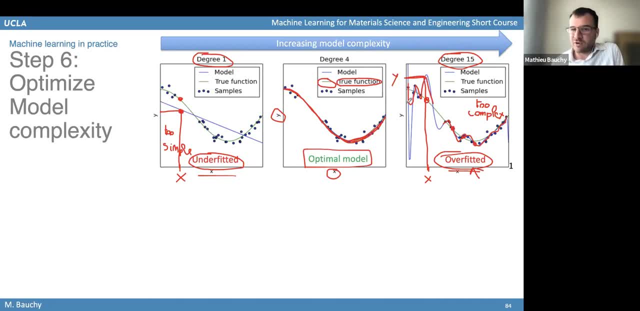 for a new material that the model has never seen before you. you will have potentially this big uh difference here between the prediction and what should be the the true property for this uh, for this material. So both under underfitted and overfitted. 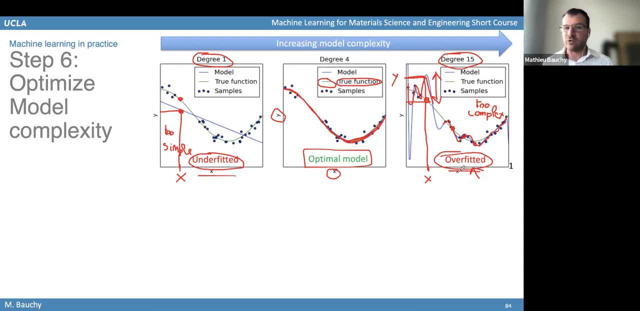 they are both bad, uh, when you want to to to to build a machine learning model. So for this, if you want to find the optimal model, you need to find a model that is not too complex but also not too uh, too simple. 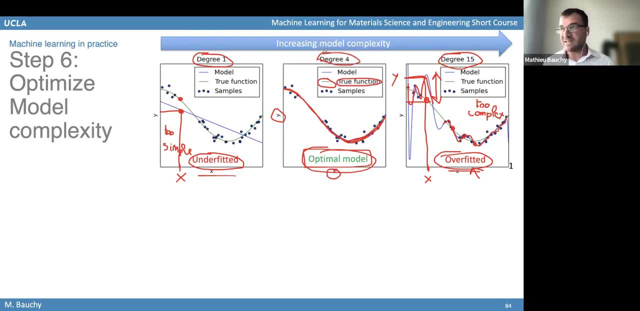 So in this case I'll pull a degree four would be the best, uh, optimal combination. So the question here is: how do we find this optimal model? complexity, How can we be sure that we have found a model that is not too simple? 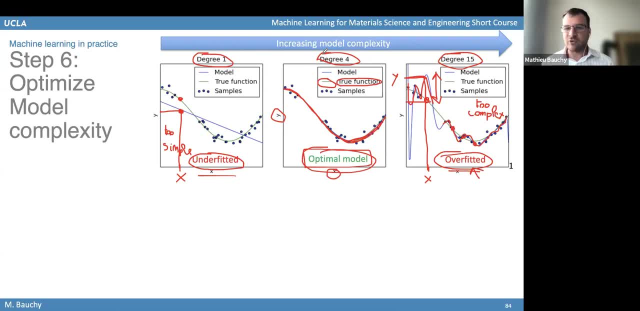 but also not too complex, And so the way that we are going to do this is that we are going to use what we call a validation set. So the main idea of the validation set here is that, when you have your, your data set, 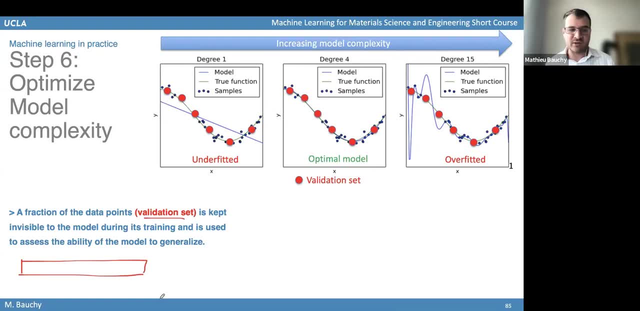 So if this is your data set that you have, this is the ensemble of all the material that you have, together with the priority. You cannot use all those data points to train your machine learning model. You need to hold down on a fraction of those data points. 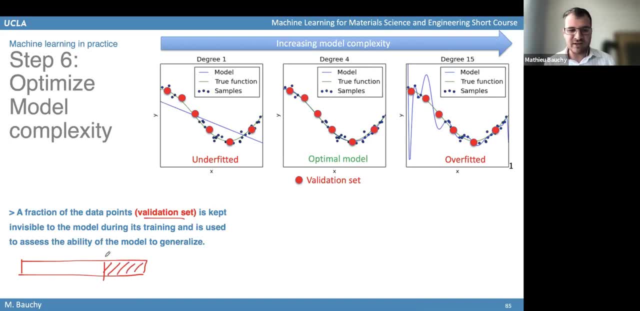 And this is what we call the validation set. The validation set is going to be a fraction of the data points that you have in your data set that you will keep hidden to the model. You will not use those data points when you train your model. 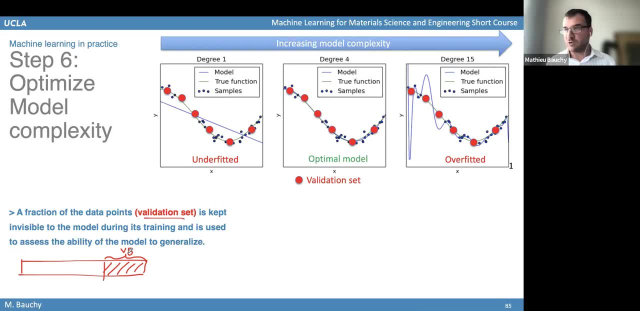 So when you try to adjust the weight of your model in order to find the relationship between inputs and outputs, you will keep those data points in stock, and you will keep it until the very end. So let's see why we need to do that. 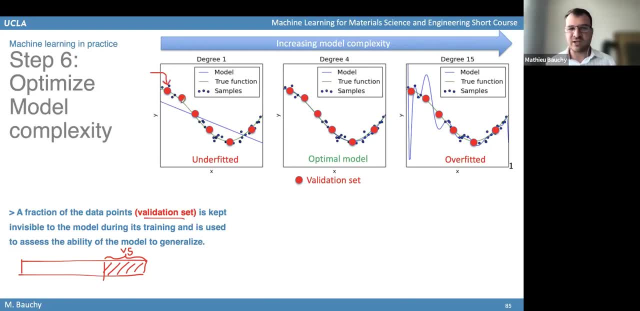 So here, this validation set is going to be the red points that I have here. This is a series of points that you will keep hidden, that you will not include in the model when you train it, And so the reason you do that is that now, what you can do is two things. 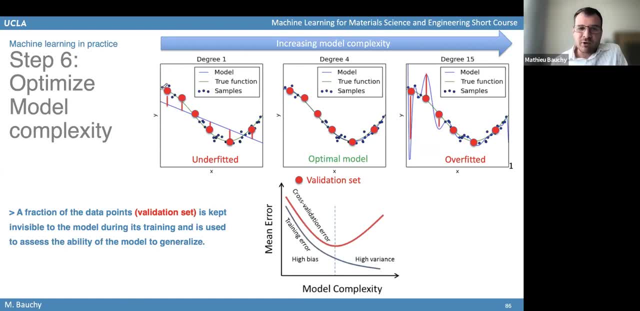 You can calculate how much error your model is making when predicting the points that we are used to train the model. So, for example, like here, your model is this blue line. So if you look at how far are the points that we are used to train the model, 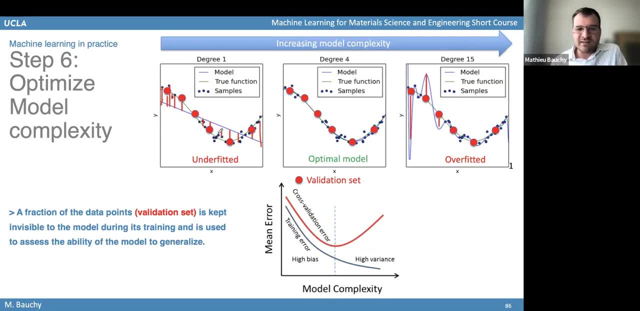 you can calculate, like how good your model is at predicting the blue point that you used to train the model. So this is what we call the training error. So this is how far is the model from the point that you used to train it. 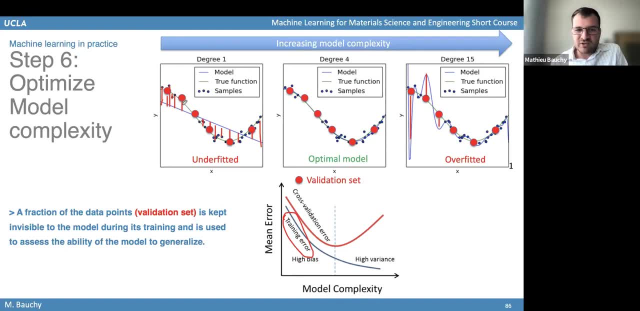 And now you can also have a second error, which is here: the distance between the points in your validation set. So those points that you did not include, that the model did not see during its training. Now you can use that to calculate how good is your model at predicting those points. 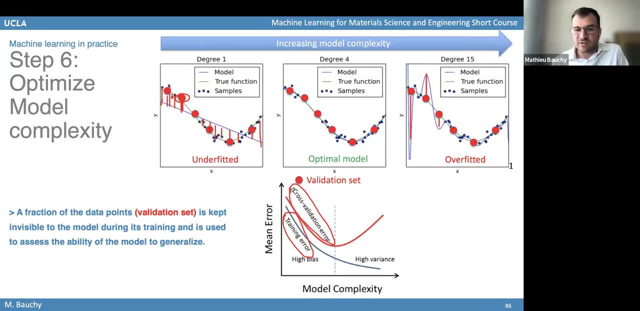 in the training set, in the validation set, sorry. So this is going to be a second error, which we call the validation error or the cross validation error. So now you have those two errors. You have the errors for the points that we are used to train the model. 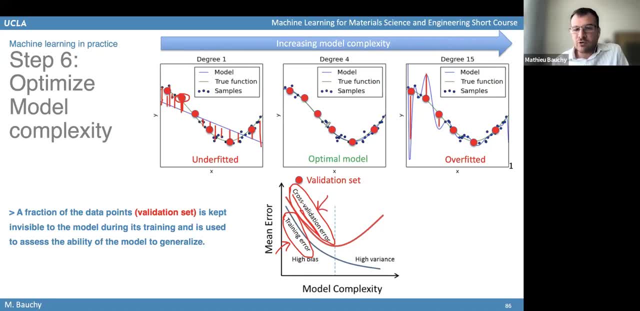 And you have now a second error, which is how good your model can predict those red points, And so this is what you're going to use to determine the ideal complexity for your model. Why? Because if you look at the training error, which is the blue here, 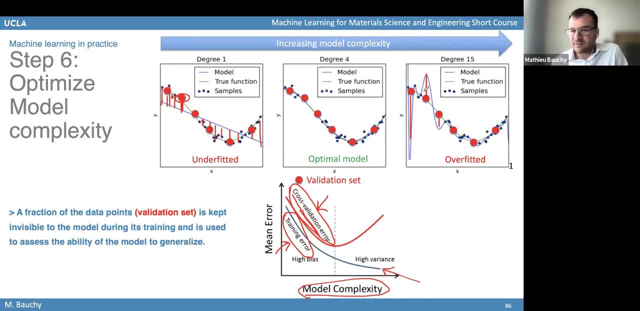 then it's very easy because, like, the more complex your model becomes, the more it will really try to go through each point of your data set. So the more complex your model is, the lower the training error will be. So this blue error here. 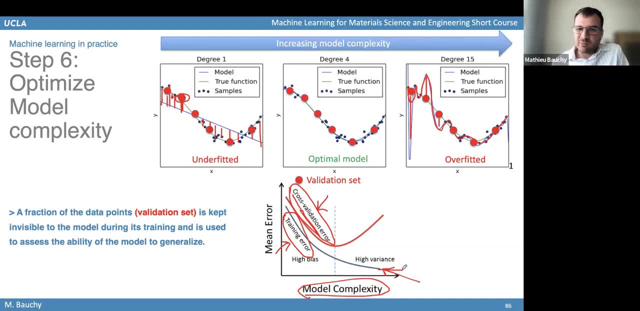 it will always decrease if your model becomes more complex Because, like the model is more complex, so it can really go through every single point of your data set, So the training error is going to become smaller and smaller, which means that you cannot use the training error to decide if your model is overfitted or not. 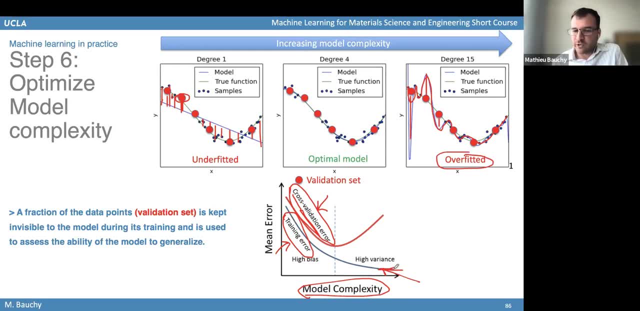 Because, like this model will just keep becoming lower and lower, So it will look like a more complex model is better, but you won't be able to see when it becomes overfitted. On the other hand, if you now calculate the error for the validation error, 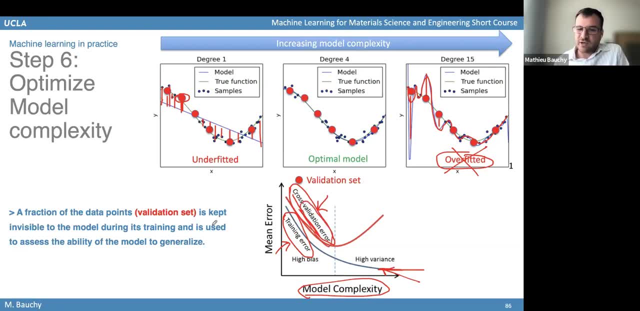 like the error of the points in the validation set. you calculate how good is your model at predicting those points in the validation set. Those are some points that were not included during the training of the model, So the model doesn't know that those data points exist. 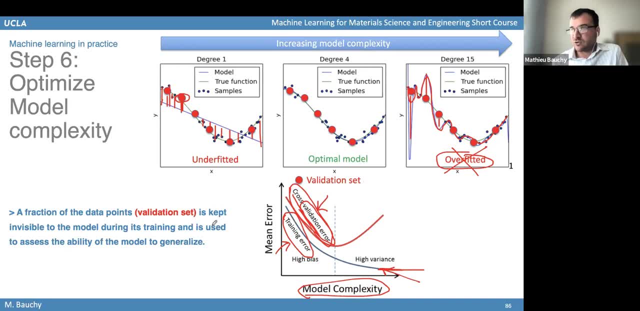 So the model did not try to fit those points, And now you can use those points to see how well your model generalize to material that it has never seen before. So, for example, in this case your model is too simple anyway, So it's pretty bad. 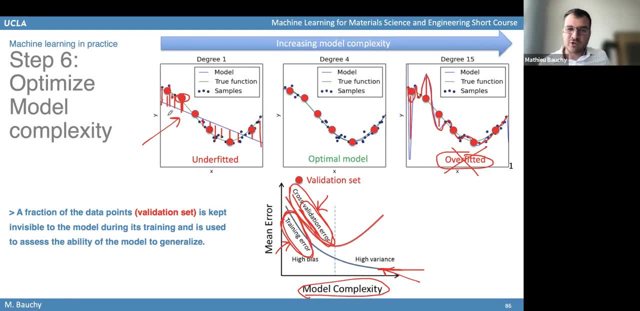 It's making a bad error to predict the point that we are used in your training set, The point that we are used to train the model. they are associated with a high error. But it's also bad to predict the point that are used in the validation set. 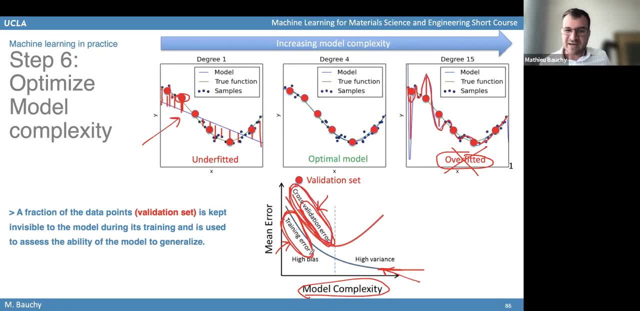 It's bad for both. So when your model is bad both at predicting the points that we are used to train- the model that's the training set- And it's also bad to predict the points in the validation set, like to predict those. 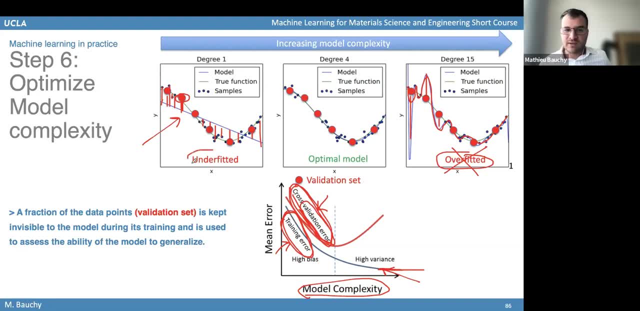 the priority of the material that it has never seen before, Then that's a sign that your model is underfitted. On the other hand, here, when you have a material that is overfitted, the material- the model in this case- is very good at predicting. 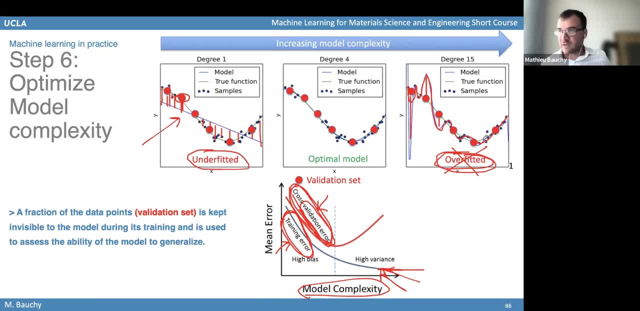 the points, the blue points. It's very good at predicting the properties for the material that it has seen during its training, but it becomes very bad at predicting the properties of the material that it has never seen before. So it's going to be very bad at predicting. 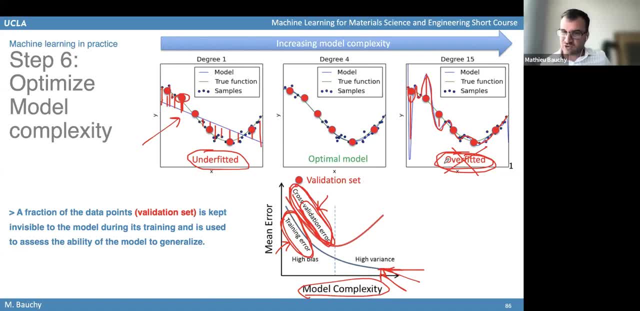 the properties for the materials that are in the validation set here, because it's trying so hard to go through each of the blue point that it starts to fluctuate a lot, And so you will get a big error between the points, the actual points in the training set. 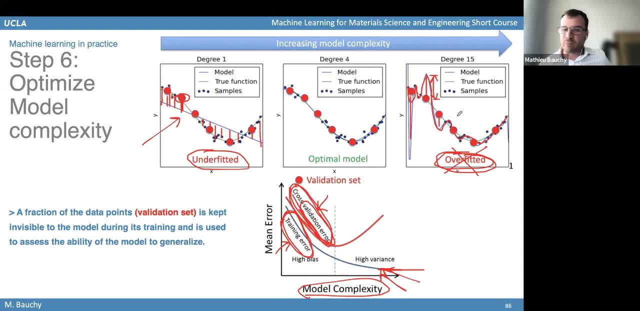 and the sorry, you will get a big error for the red points that are in the validation set here. It's not going to be able to predict the validation set very well because it fluctuates too much. It's not able to really generalize well. 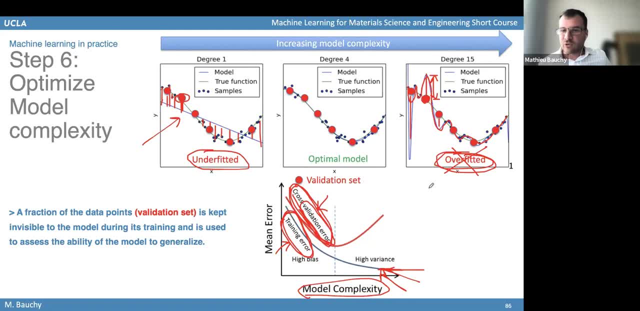 to new material that it has never seen before. So when you have an overfitted model, it means that in this case the error associated to the training set, like the training material that's used to train the model, will become very low. 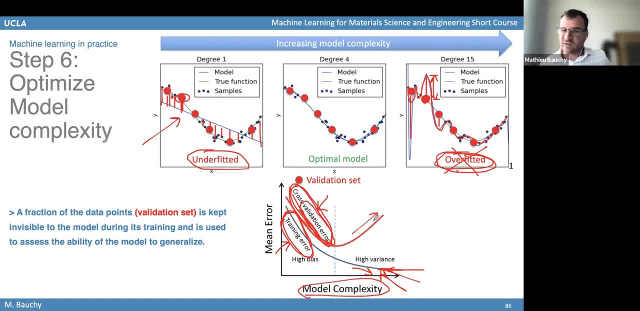 but the error associated to the validation set will now start to increase again, because your model will not be able to really generalize well to material that it has never seen before. So this is going to be a sign now that you have an overfitted model. 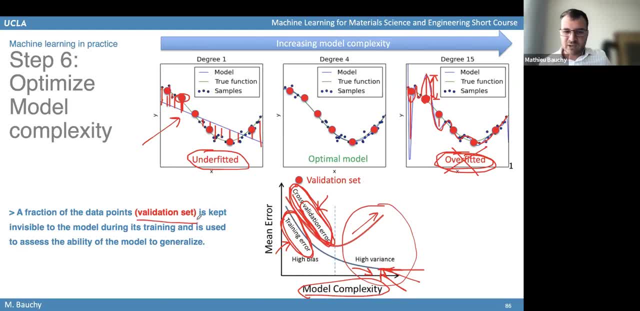 So that's why, when you train a machine learning model in order to check if your model is overfitted, you can never use all the points that you have to train your model, because if you do that, you have no way to detect if the model is overfitted or not. 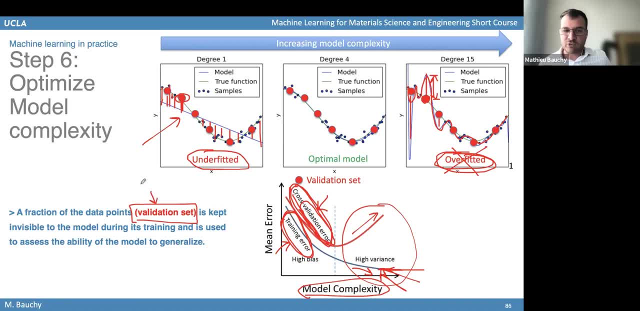 You always need to keep a fraction of the data points, So typically that can be about 20% that you keep until the end and you keep those data points hidden to the model. You keep it as a validation set so that you can see how good your model is at predicting those points. 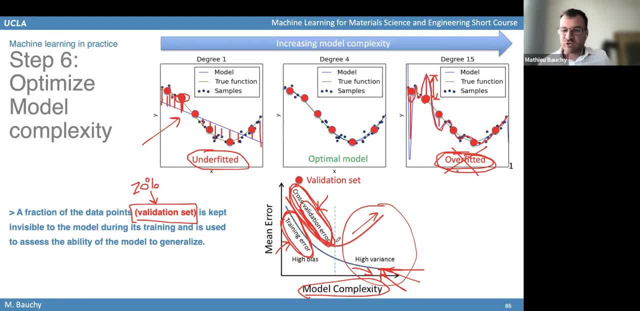 And then, based on that, what you will want is to select this ideal complexity here, Like if you select this level of complexity for which the error of the training error is low, but also the validation error is low, it means that your model is good. 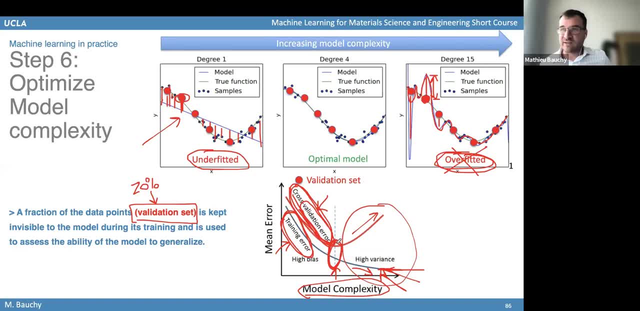 not only at predicting the points that it was used during- that was used during the training of the material- but, even more importantly, this model is good at predicting properties for new material that it has never seen before. So in this case, this will be the sign. 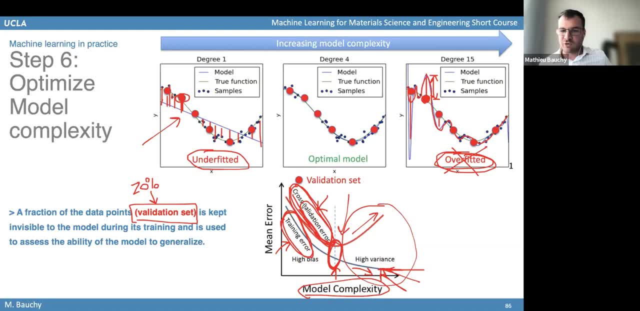 when you see like there is this minimum of the validation error, this is going to be the sign that you have found like the best model with the ideal level of complexity: not too complex, not too simple. So this is the how we would do in practice. 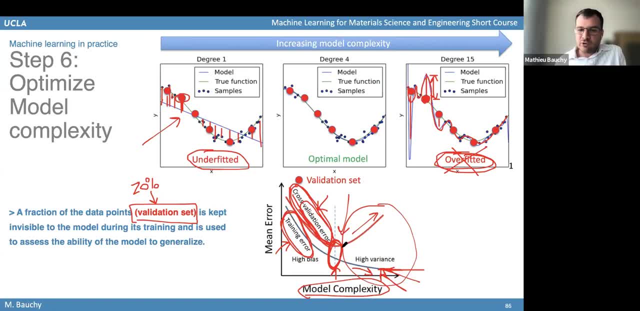 for example, if you have a neural network, you will try to train your neural network with different number of layers or different number of neurons And then you will track the validation error of your model for different number of neurons, different number of layers. 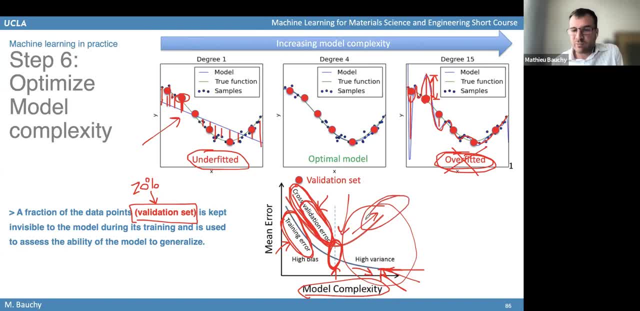 And you will see, if your model is too complex, too many layers, too many neurons, then it's going to be overfitted, So it's not gonna be generalizing very well, And, on the other hand, if your model is too simple, 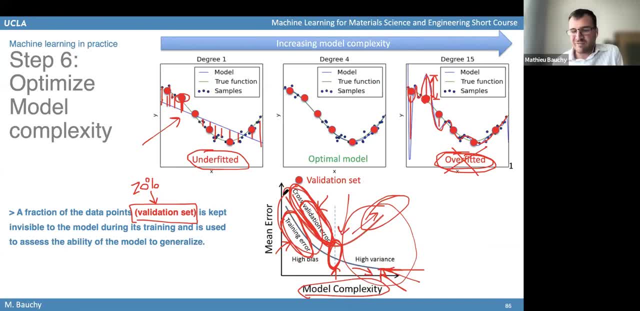 then it's gonna be underfitted and it's not gonna be fitting your other points very well. And so whenever you have this minimum here in the validation set error, it means that you have found the ideal degree of complexity that is not overfitted and not underfitted. 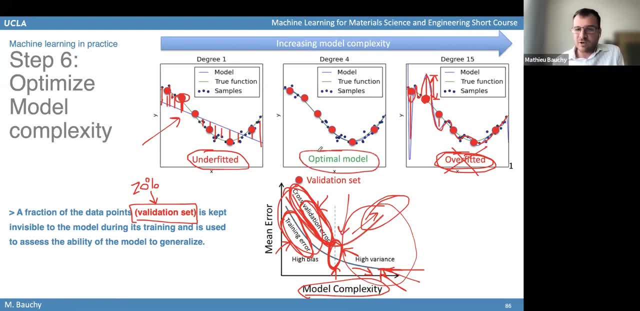 So this is the what will give you the optimal model that is the most likely to really give you a good prediction of the true relationship between the input and the output. Does it make sense to everybody Like? do you have any questions regarding this? step six: 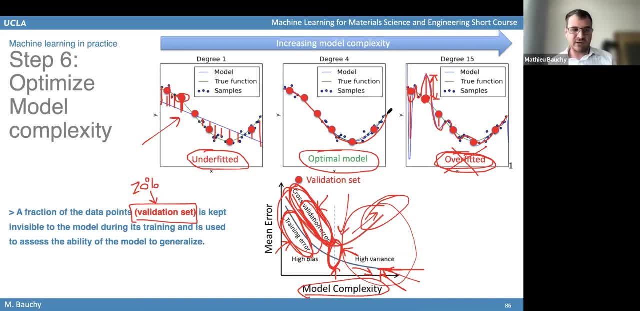 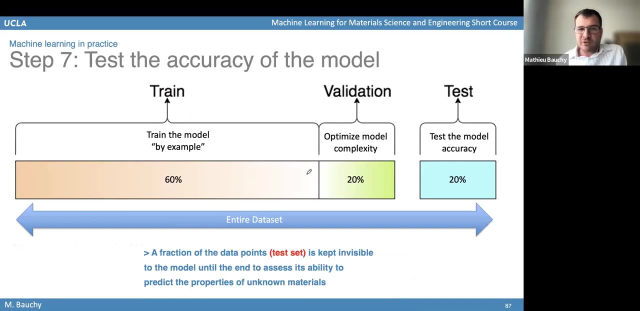 on how you would optimize the complexity of your model. Okay, so let's go to the next step. So the next step is about testing the model. So for this, the idea is that you used a fraction of the points. you use them to train the model. 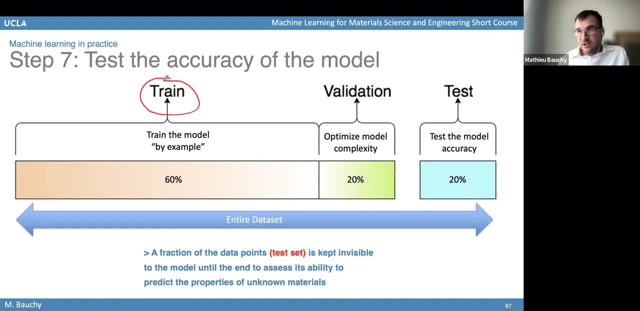 So you some of the points. you use them to adjust the parameter of the model. So this is the training set. So those are the points that you used to adjust the parameter of the model. So this is the training set. So typically this 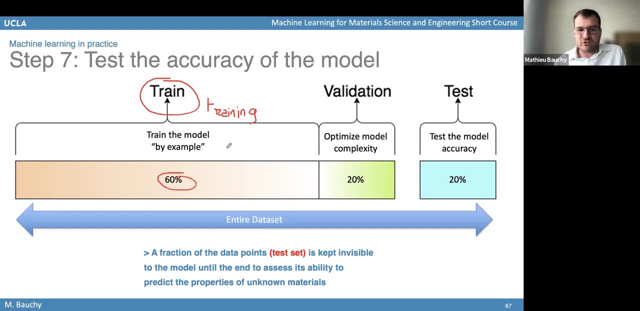 those points can be about 60% of the data set. So if you have a data set of, let's say, 100 points, you will use 60 of those points to train the parameters of the model. Then you have your the second step. 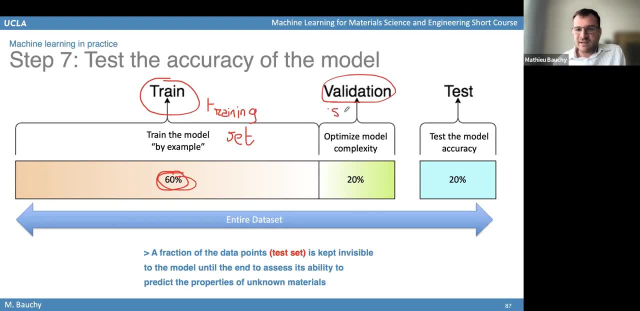 which is your validation set. So this is the validation set. This is a fraction of the points that you have kept hidden to the model, And now you will use those model to optimize the complexity of the model. So you will use this to decide. 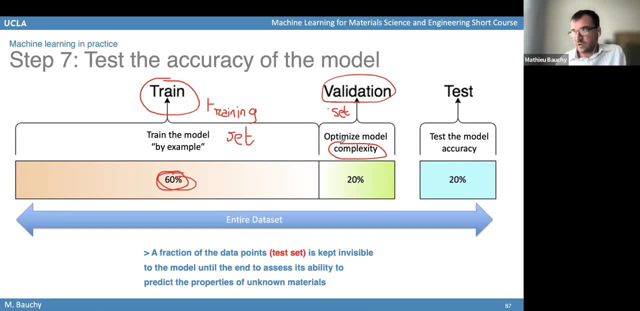 how many layers should I use, How many neurons should I use, Which degree should I use in polynomial regression, et cetera. This is gonna be typically an over 20% of the data set. But now, once you have this, 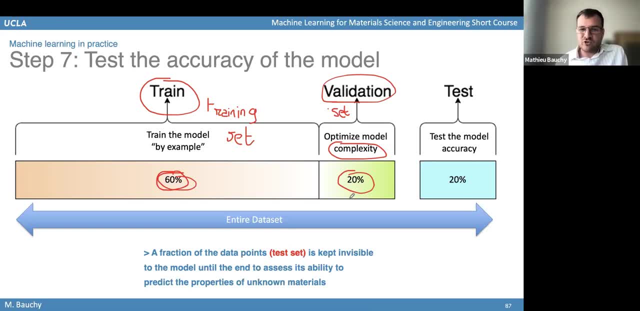 you still need to test, have a final evaluation of how- not only how well the parameters have been trained, but also how well have you optimized the complexity of the model. So if you want a final evaluation of how good your model is, then you need to have another fraction of the data. 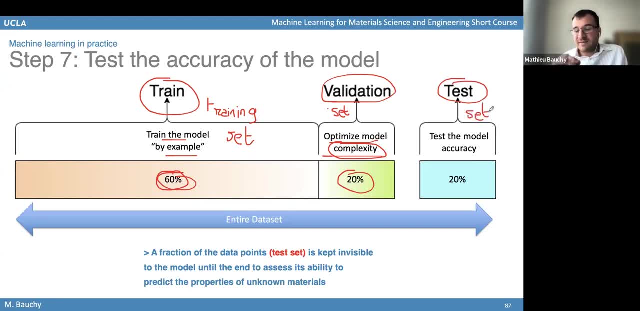 that we call the test set. So the test set is another- for example, 20%- of the data that you will use to see how good your model is. You will train the model and then you will use your model to predict some probability. 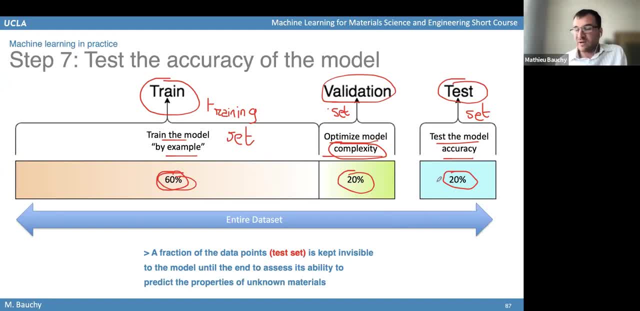 for the remaining 20% of the materials And you will see how far is your model from the actual data points that you have in your test set. here You will see how good is your model at predicting the test set, The reason it's good to have. 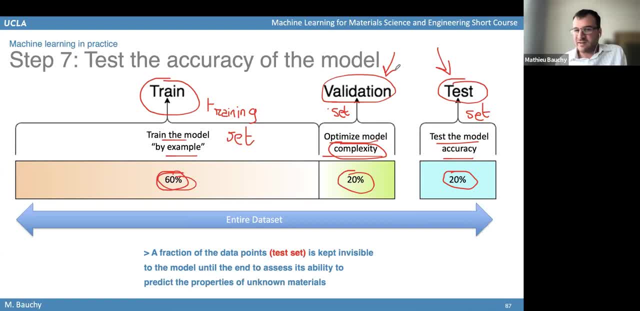 not only a validation set, but also a test set is because, like each of those data points, they have a specific purpose. The training set, this is to train the parameters. So this is to train the parameters of your model, like the weights in the neurons. 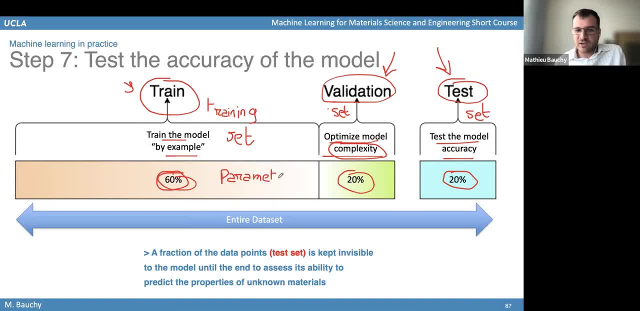 or the parameters of your polynomial regression, The validation set. this is to train what we call the hyperparameter. So this is to decide how many layers should you use, How many neurons should you use, Which degree should you use in a polynomial regression. 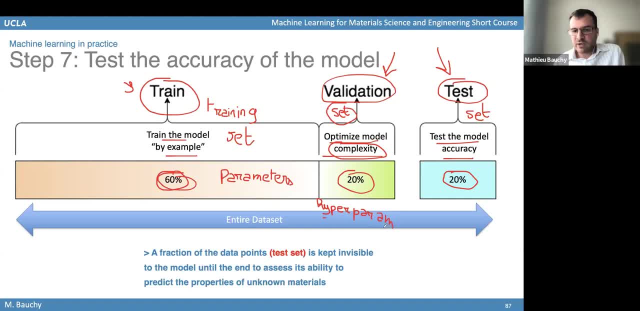 So those are the hyperparameter. This is the parameter that dictate how complex the model is, And you use the point in the validation set to decide which hyperparameter to use. So then the last set of point, the test set. it has only one purpose. 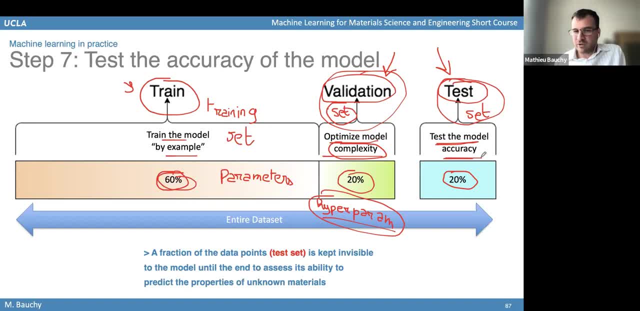 which is to test how accurate the model is, And ideally, you should not use the same point to both optimize the complexity of the model and also test the model, because that would not be, in that case, a fair assessment of the model, If you want to. 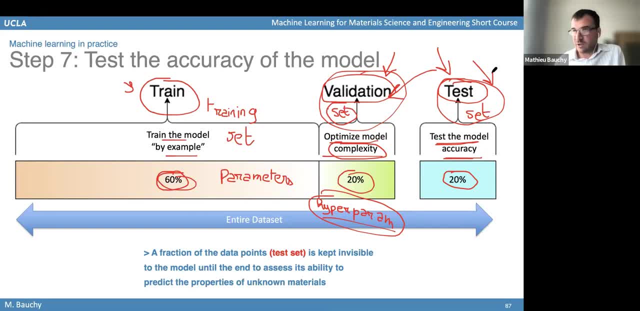 if you want to have a fair assessment of how accurate the model is, you need to use some model, some points that the model has never seen before. It needs to be some point that we are not used to optimize the hyperparameter, or some point that we are not used. 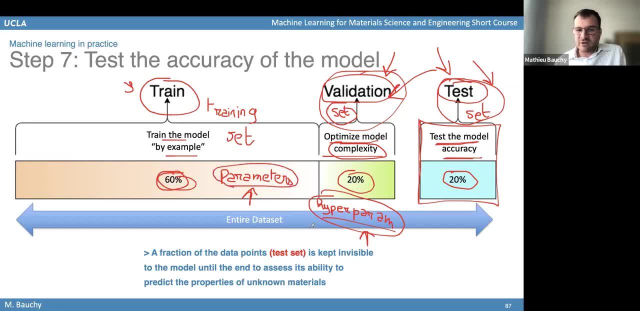 to optimize the parameters. So some of the points are used to optimize the hyperparameter, Some of the points are used to optimize the parameters And then you keep a remaining fraction of the point that is not used to optimize anything. It's just used to see how accurate the model is. 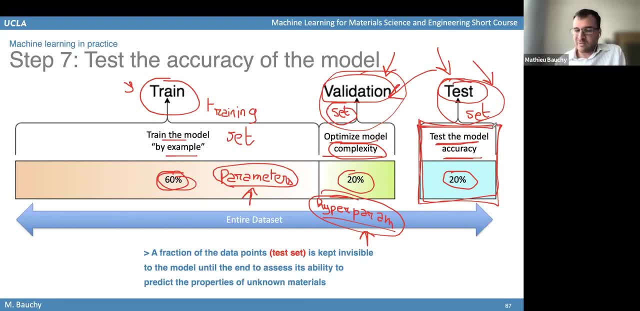 when it's trying to predict the properties of new material that it has never seen before. So in practice it's a good practice just to keep about 60% of the data set to train the model: 60%, another 20% of the data set. 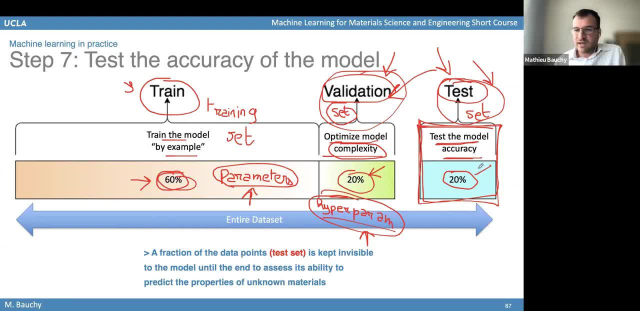 to train the hyperparameter to optimize the complexity, and another 20% to just test how accurate the model is. So those are the. when you have a data set, you want to, you will need to randomly split this data set into 60% for the training. 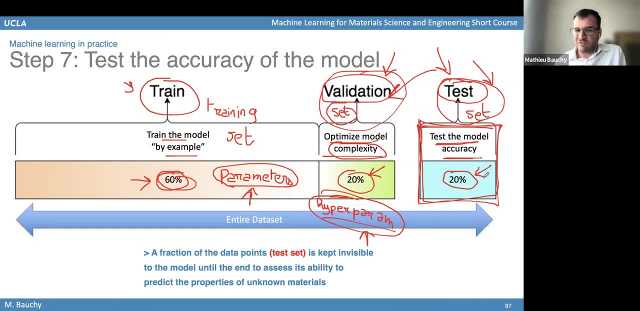 20% for the validation and another 20% for the test set. So that's typically a good practice when you train your model, And that's gonna be one of the final step, which is, like you test how accurate the model is. 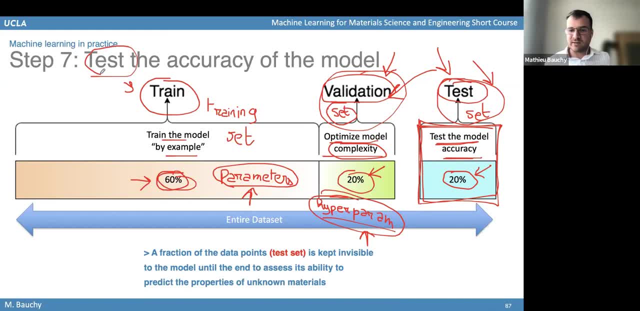 And based on that you can see like. well, my model can predict the properties of this material with an accuracy of a plus minus 10%, or plus minus 5%, or plus minus 20%. So, based on that, by testing your model, 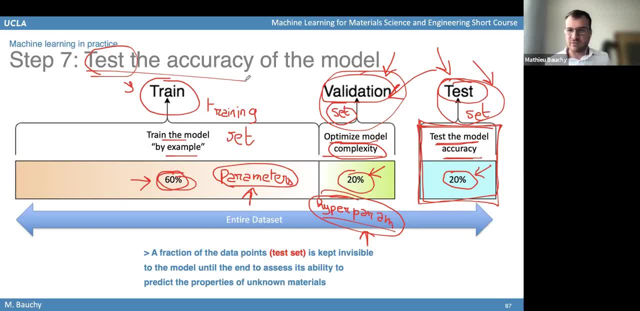 you can determine how accurate the model is, to see if it can be used in practice or if it doesn't have enough accuracy to be really useful in practice. Any questions about this step seven? Yes, professor, I have a question. What if you? 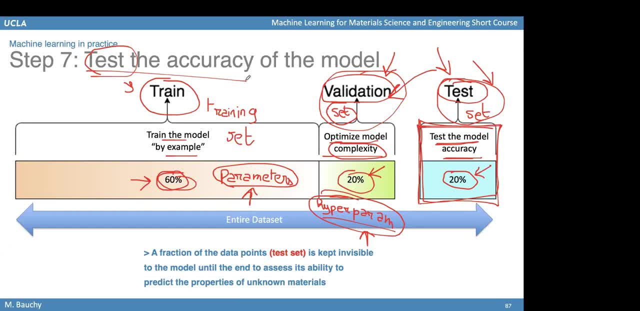 what if your train is not the same? 60% in train. Yes, Yeah, So the here the numbers. I'm saying it's like those are some recommendation. Sometimes maybe you will want to use like 80% of the data for the training set. 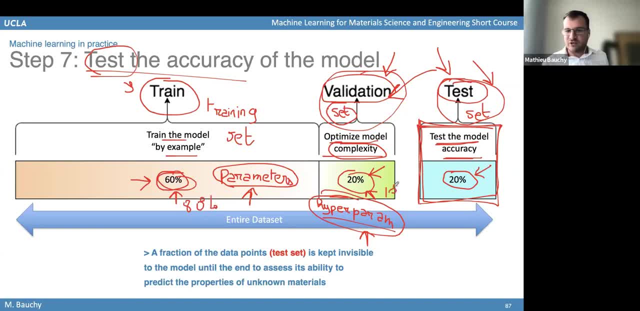 and only 10% for the validation and 10% for the testing. I think it's also fine, Like there is no universal rule of how many points you should use for training, how many points you should use for validation. I think it also depends on the size of your data set. 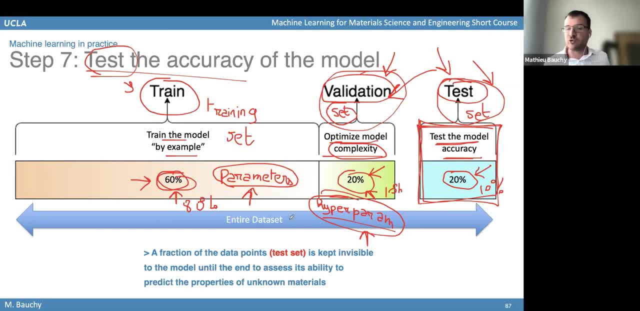 Like, if you have a very small data set of just a few hundred points, then you will typically want to use a pretty large training set. Otherwise you won't have enough points to really train your machine learning model, So in this case it's better to use a smaller validation set. 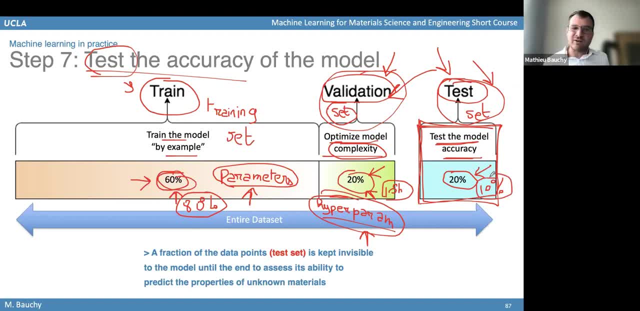 and a smaller test set. But if you have a lot of points, then you can afford to have a larger validation set and a larger test set. So I think it really depends on how many data points do you have. but those numbers, those are recommendation later. 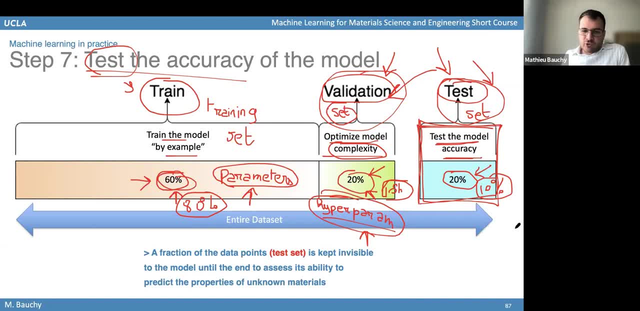 Like there is no really universal rule of that it should be 60% or 70% or 80%, So that depends on, really, the size of your data set. That depends on how strongly you want to test your model Or if you really have. 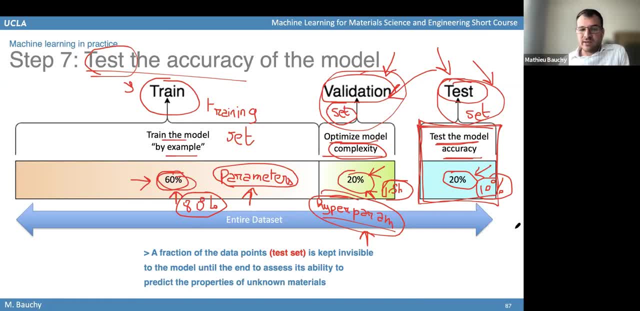 a very small data set, then you really need to use a large fraction from the training set. So there is no clear universal rule from that, But typically still it should be around like those numbers, like from 60% to 80% for the training set. 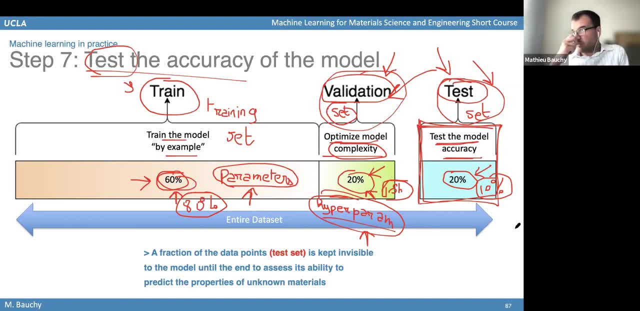 and from 20% to 10% for the validation set And 20% to 10% for the test set. Those are the typical orders of magnitude that you should use in practice. Does it answer your question? Okay, thank you. 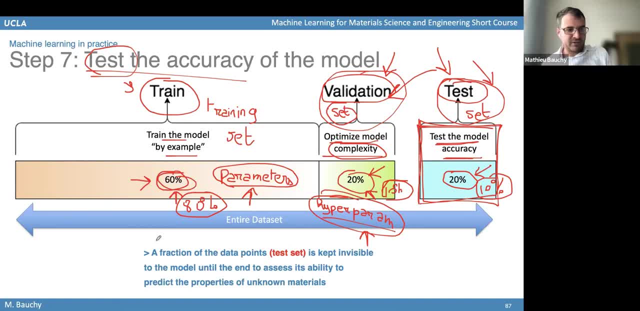 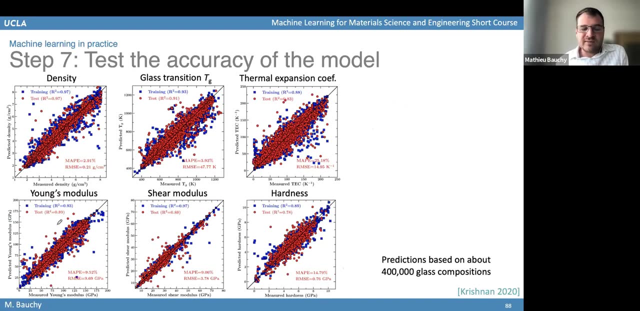 Any other questions regarding this step seven? Okay, so let's go to the. Okay, so there's still step seven. So one of the common ways to test how accurate a model is is to do those kind of plots here. So what those plots show is: 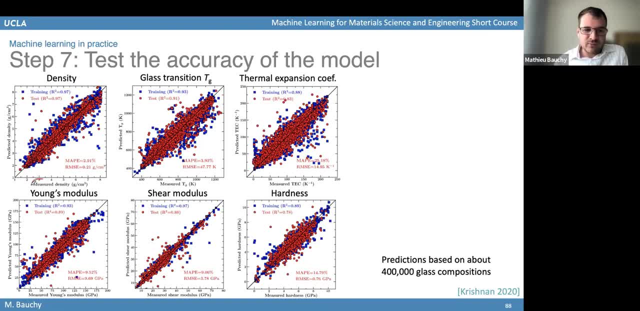 you show on the x-axis the true value of the property that you are trying to predict. So, for example, this is here some example of some machine learning model that we are used to predict various property of glasses, For example the density, the glass transition temperature. 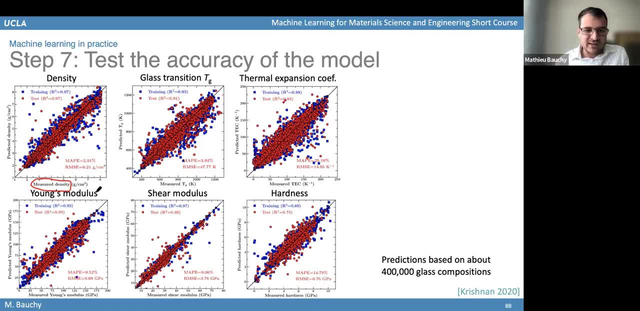 the coefficient of thermal expansion, et cetera. So in that case, on the x-axis, here you would put the true value of the measured property, And on the y-axis you will put the value that is predicted by your model. 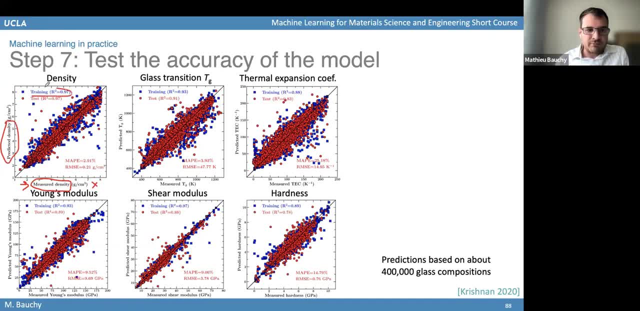 And then you can do that both for the point that you used to train your model, like the training set, and also for the point that I used to test the model, like the test set. So if your model was predicted to be perfect, 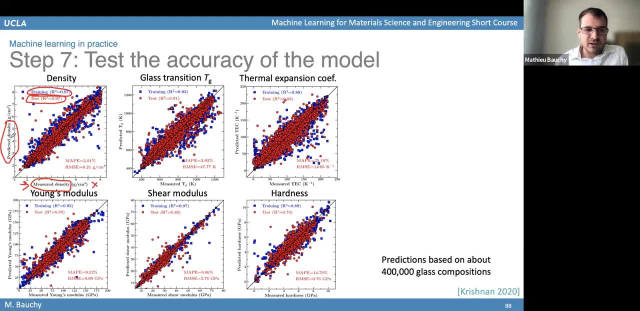 then you would get a perfect agreement between the measured property and the predicted property. So everything would be very close to this: y equals x line. like this: y equals x line. Here is the line of equity. This is the line that corresponds to when the predicted property 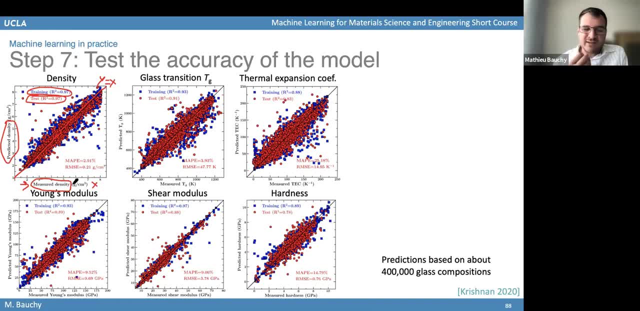 is exactly equal to the measured property. In practice you can never have a perfect agreement between predicted and measured property because there is always some noise in the measurement, So you cannot have a perfect prediction. The noise is always going to induce some small fluctuation. 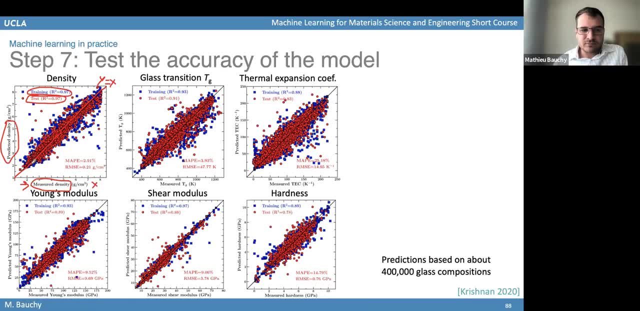 So in practice, the points that you have, they will ideally be close to this line of equity. But if you have some points that here are very far from this- y equals x line- it means that those points are not very well predicted by your model. 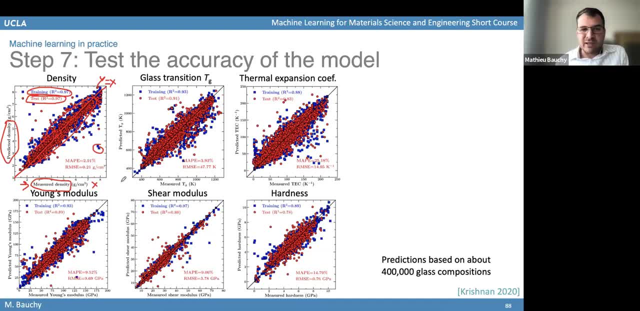 So then, if you want to determine, put a number to determine how good your model is, then you can use those plots and calculate either the coefficient of determination, r squared, which is going to give you a score, and the closer r squared is to one. 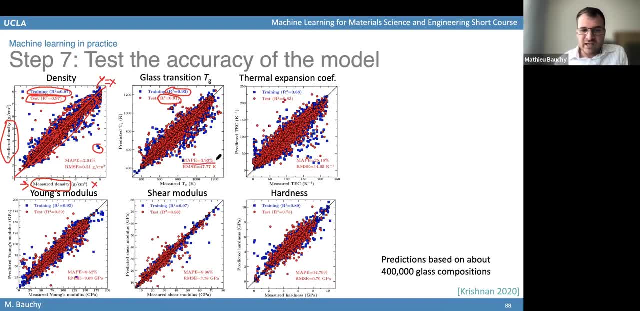 the more accurate your model is. Or you can use the MAPE. MAPE is the mean average percentage error. You calculate for each point. you calculate the percentage error between the predicted and the true measured. Or you can use the RMSE. 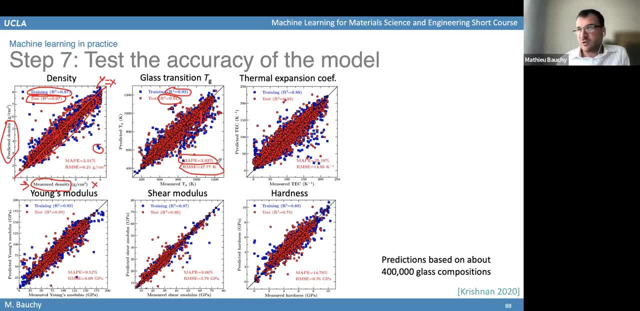 This is the root mean square error. So this is another metric that you can use to see, on average, how much error do you have, how much difference do you have between your predicted probability and the true probability? So, in this case, r squared, ideally. 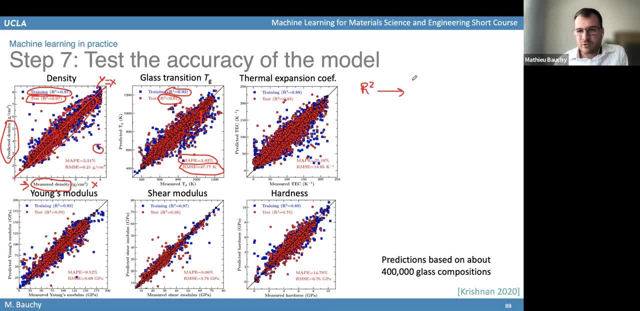 needs to be as close as possible to one where one would be a perfect model For the MAPE, the mean average percentage error. ideally, you want this MAPE to be as close as possible to 0%. Like in practice, you can never have 0%. 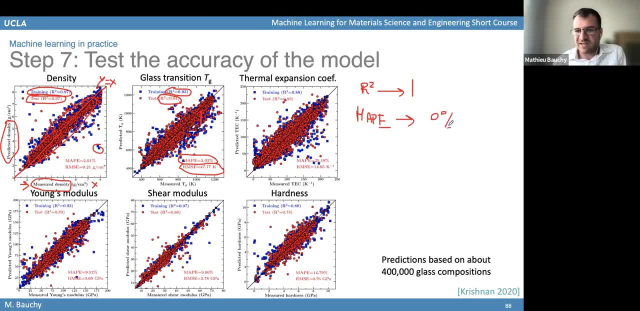 but you want to be as close as possible to that. You want to have an error that is typically less than 10%, for example, And the RMSE? well, you also want the RMSE to be as close as possible. The RMSE is the root, mean square error. 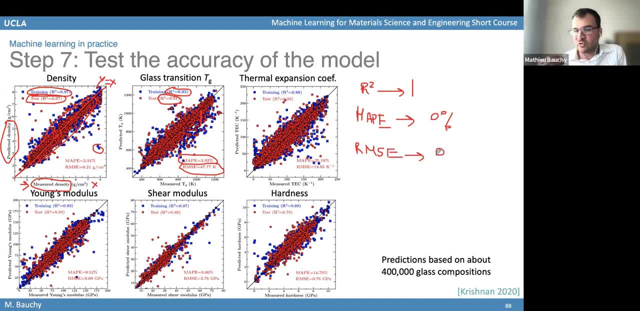 Typically you want this to be also as close as possible to 0,, which means that your model is making a low error on average. So that's typically how you would test and quantify how good the model is. You would calculate specifically the r squared. 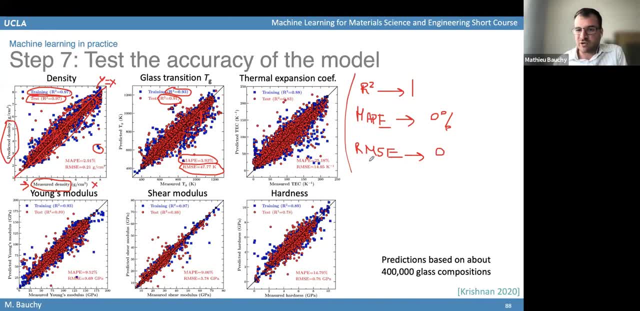 the coefficient of determination, the MAPE, the mean average percentage error, or the RMSE, the root mean square error. You calculate that both for the training set but also for the test set, And that's going to allow you to see. 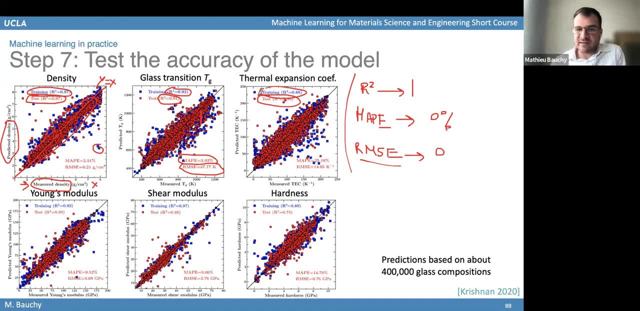 how good your model is at predicting the properties of glasses that it has never seen before in the test set, And that's going to be a good test to see how accurate your model is. So this is typically one of the final steps when you train a model. 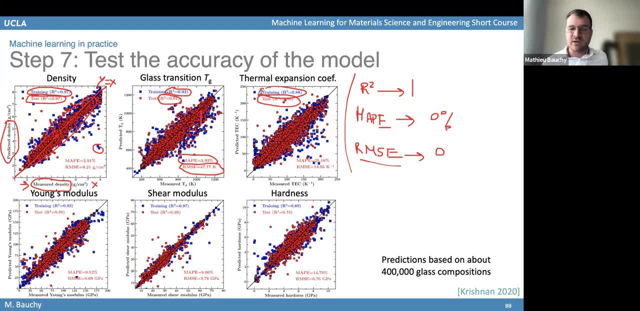 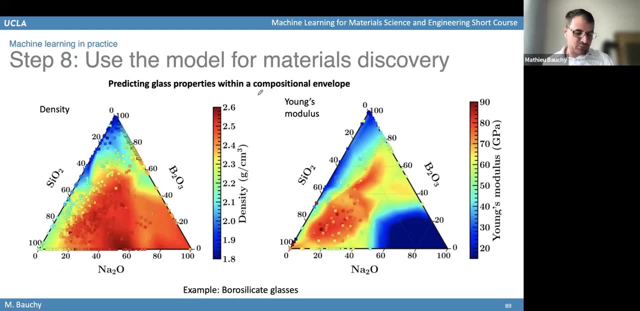 This is to test how accurate it is by calculating one of those three metrics here. Then the last step is: once you have the model, then you need to use it. You can use it to, for example, discover new materials. So here the idea is: 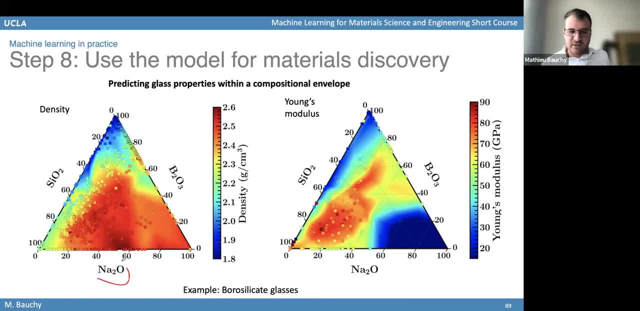 for example, you have trained a model that takes as input the composition. So you have three oxides here And as a function of those three oxides, your model can predict what would be the density or what would be in this case. 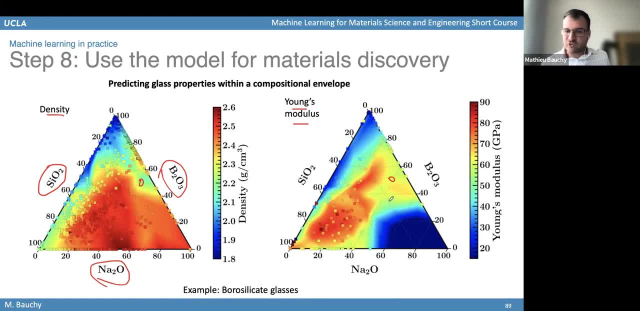 the Young's modulus of this glass As a function of its composition. So this is going to give you a prediction. So it means that if your goal is to find the best glass that has, for example, the highest Young's modulus, then you can directly 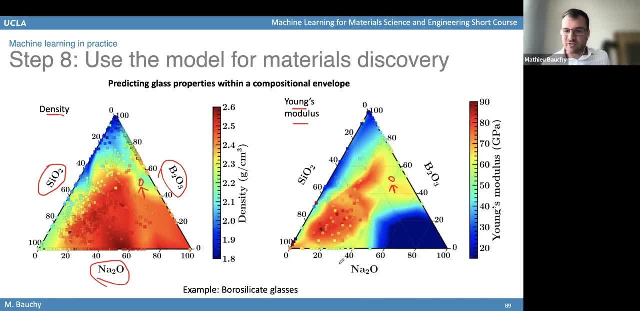 look into that and see what your model predicts for every single composition and directly see that here the best Young's modulus is going to be somewhere in this area here, where you have the highest possible Young's modulus Or, if you want to have the lowest possible density. 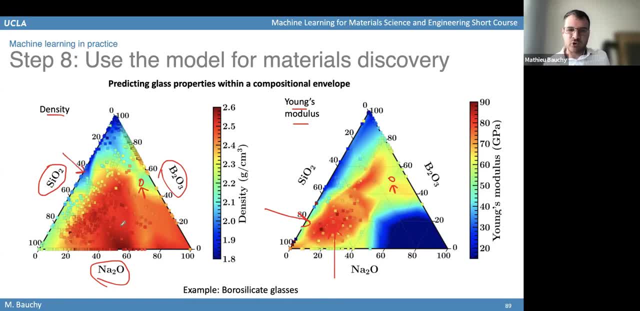 then it's going to tell you that this is where you have the lowest possible density. So you can use this- those models here- to directly make some prediction for any glass composition and directly pinpoint the glasses that will have the best properties. So this is something. 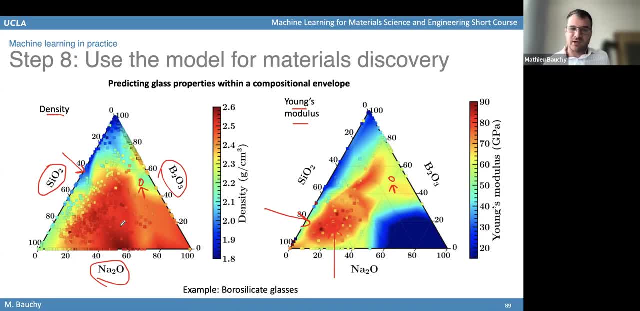 that you can use when you have your model, when it's trained, And once you have the model that is tested, then you can use it in practice to make some prediction. So this is another example here where, once you have those models and you can directly predict, 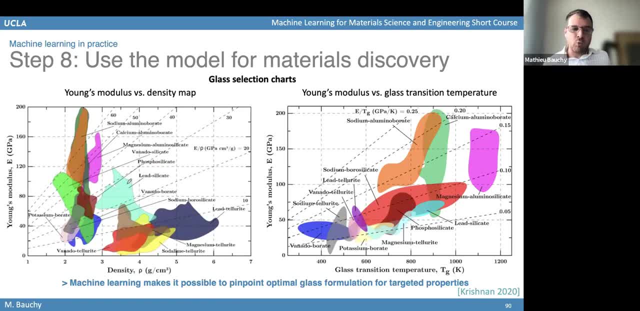 for every families of material what would be, for example, their Young's modulus or what would be their density. So this is going to give you some maps where you have some domains here where for one family of material, you can determine what are all the possible Young's modulus. 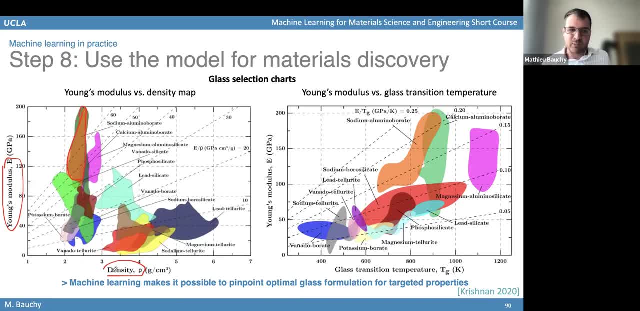 that they can have all the possible density that they can have. So for example here: if your goal is to find some material that have the density that is as low as possible, but the Young's modulus as high as possible, then you can use that. 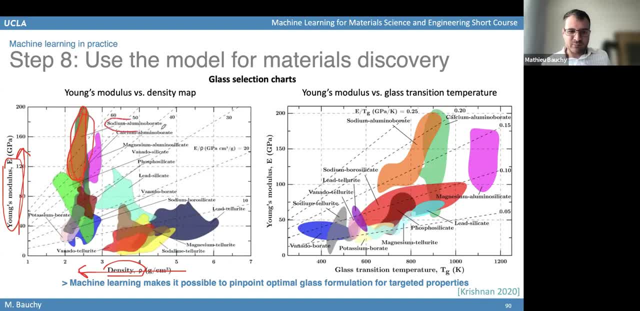 to directly predict that these types of material are going to be the one that has the highest Young's modulus while having the lowest density, And this is because you have a machine learning model that you can use to directly predict what will be the priorities of any material. 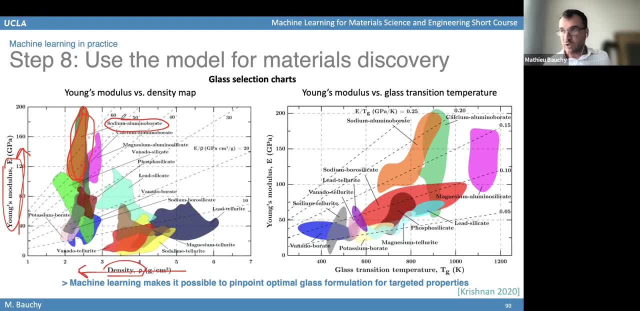 that you can use that to directly select what will be the most promising type of material based on what you want to achieve. So that is the kind of map that you can build once you have a machine learning model, once you have ensured that your machine learning model is accurate. 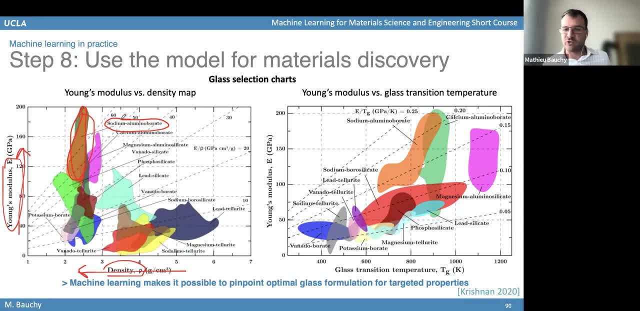 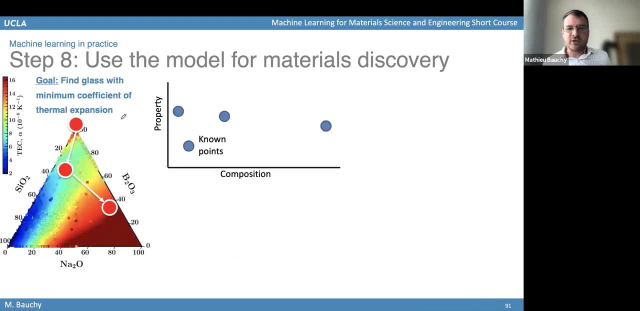 then you can use it in practice to discover new materials that have the right properties that you are interested in. Then the last thing that I want to talk about is how do you use that to try to discover the best material that will satisfy certain requirements while having the lowest number? 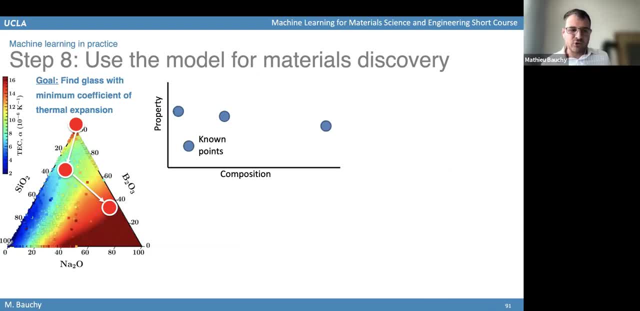 of iterations, for example here. let's assume that you have this ternary domain here and your goal here is to find what is the glass that has the lowest coefficient of thermal expansion, for example. So that is your objective and you want to find this glass here. 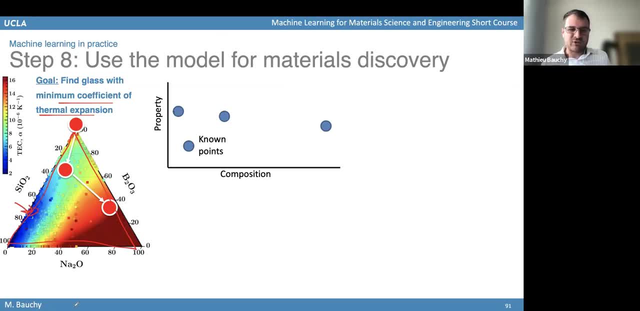 that would have the lowest possible coefficient of thermal expansion. but you want to find this without trying every single glass. you want to just minimize the number of times you actually synthesize the glass and measure its properties. So the way you can do that is to use something called 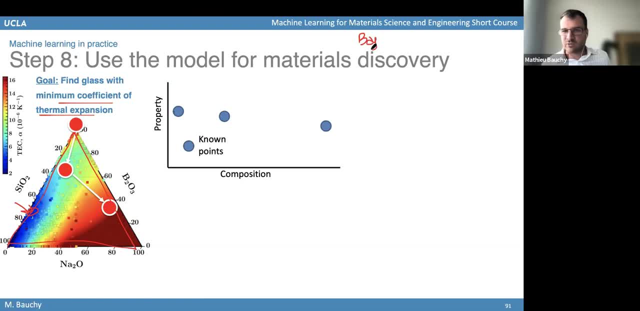 Bayesian optimization, and so that's what I'm going to talk about in the coming slides. So this is the Bayesian optimization process, where it allows you to discover new materials by minimizing the number of trials that are needed. So the idea is, for example, 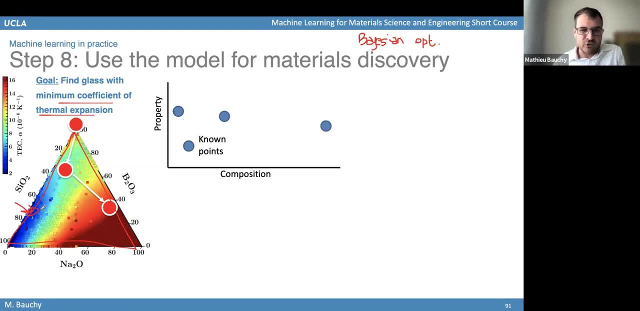 again, your goal here is to find what is the glass that has the lowest coefficient of thermal expansion. So here, what you have so far is: you have three points. you have three glasses with different composition, for which you measured both the composition of those three glasses. 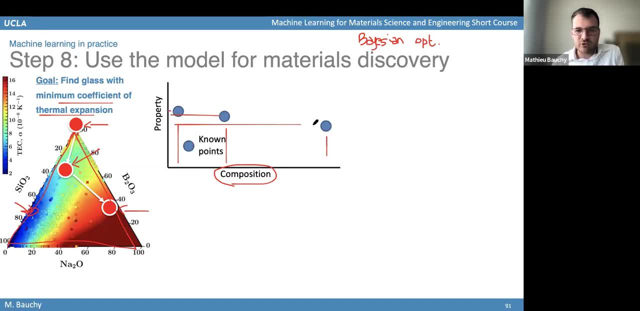 and you also measured the priority, So you also measured the coefficient of thermal expansion for those three glasses. So, then, what you are going to do, based on that, is try to, based on those three points, determine what should be the composition of the glass. 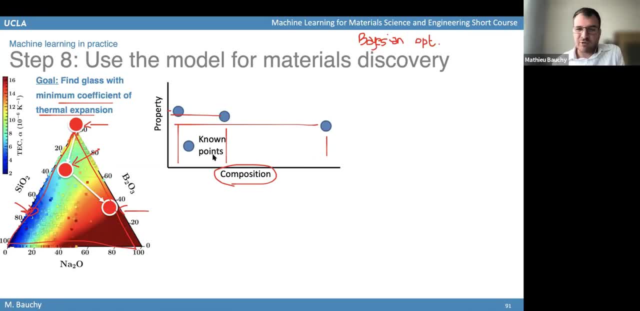 that will give you a minimum in the coefficient of thermal expansion. So the step one that you are going to do here is to try to find a machine learning model that can fit those data points And ideally, here for these types of techniques you will also want. 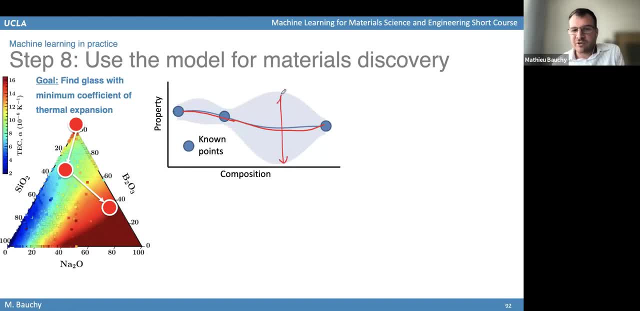 a technique that can also give you the confidence interval, like how confident the model is at making a given prediction. So this blue line here is the prediction from the machine learning model and this shaded area here is how confident the model is at making each prediction. 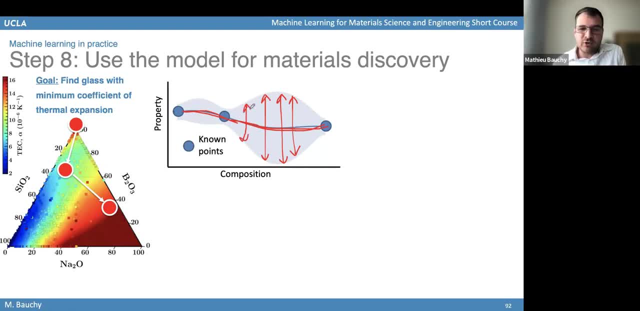 So then, the next step is, once you have this, then you want to use this information to find the glass that will give you the minimum value for this property, the minimum value for the coefficient of thermal expansion, And so there is really two things that matter here. 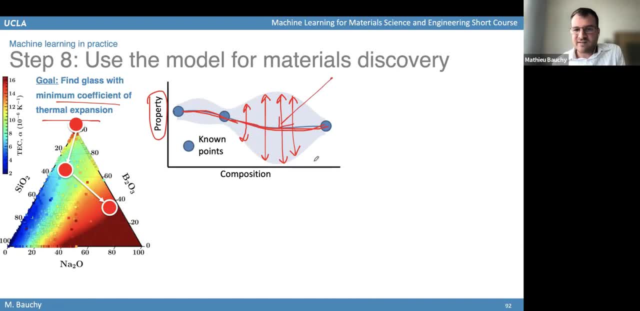 The first thing is that your model here predicts that there is a minimum here. Like your model says, this property is going to reach a minimum here. So that's one information that is useful. But there is also the fact that here your model has a very high uncertainty. 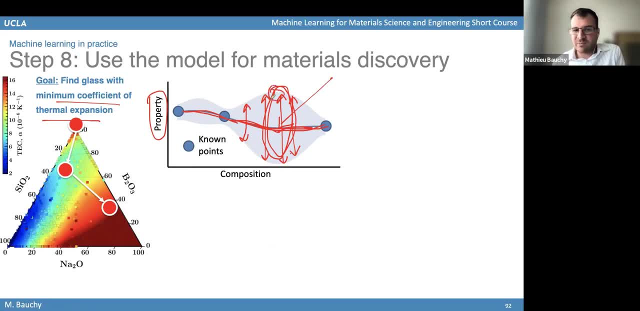 It means that your model. it's possible that here maybe the actual coefficient of thermal expansion might be very high, but it could also be very low. Here you have another area where you have a pretty high uncertainty, which means that potentially it's possible you could have 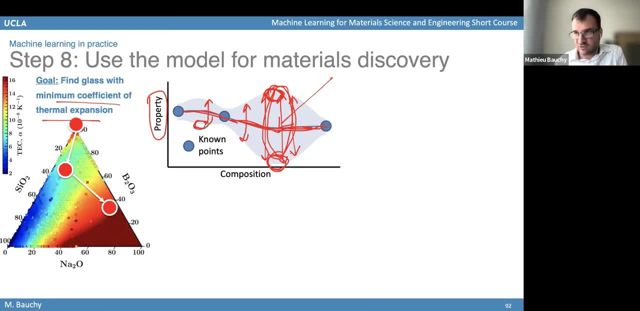 a minimum here that you are missing because your model has such a low confidence. So when you need to, when you want to determine what is the next glass, that you should try the next composition, that you should try to try to find the minimum of coefficient of thermal expansion. 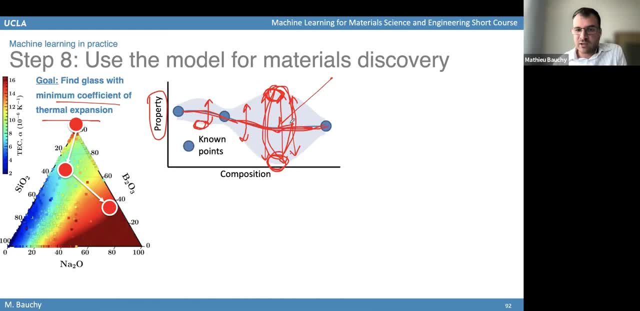 you should try two things. First, you should try to check, to explore the domain that your model is predicting a minimum. If your model is predicting a minimum here, then it's a good sign that you should go explore this area. But you should also explore: 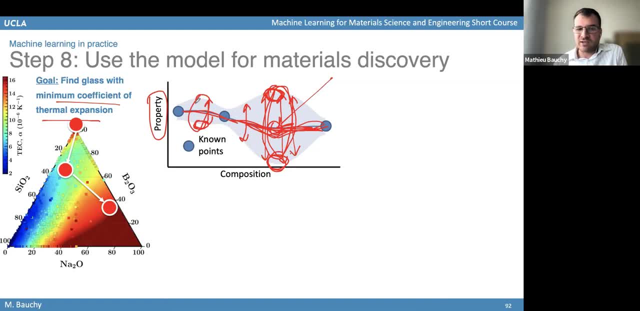 the area that have a high uncertainty, because it's possible that in those domains that have a high uncertainty it's possible that there might be a minimum there that you are missing because your model has a confidence that is too low. So the way you can find 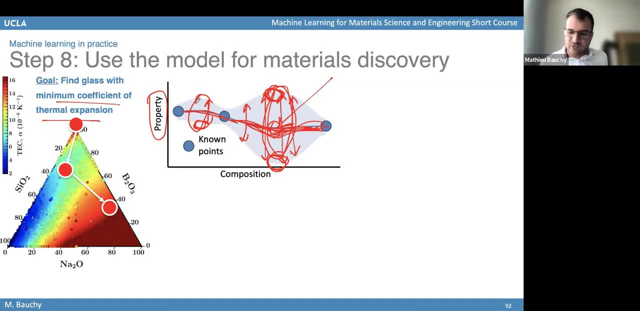 the best balance between trying to test the material for which your model has the high uncertainty and where your model predicts a minimum, is that you can calculate a function which is called the expected improvement. The expected improvement function is a function that takes into account two things. 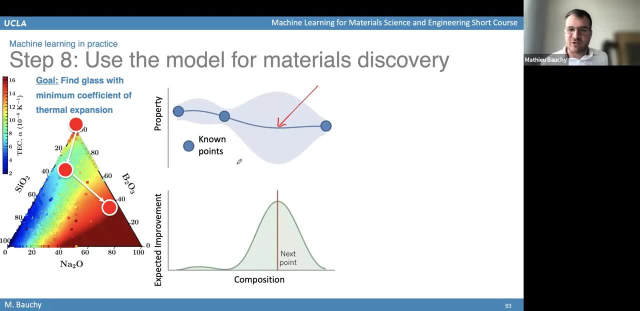 It takes into account the prediction from the model, but it also takes into account the uncertainty And it tries to find the best balance between exploiting the region that the model is predicting to give you a minimum coefficient of thermal expansion, but also exploring the region. 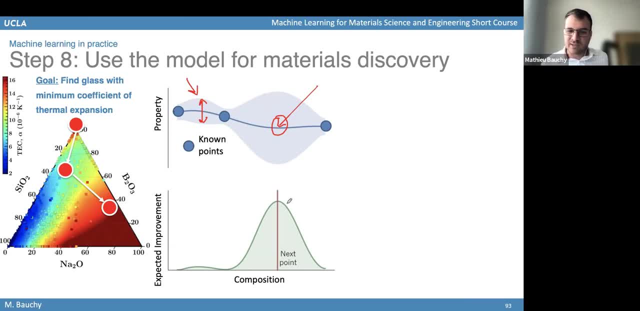 for which the uncertainty is pretty high, Like, for example, here. you have a very high value for this expected improvement function because this region- here not only your model predicts a minimum, but it also has a pretty high uncertainty. So this is going to be. 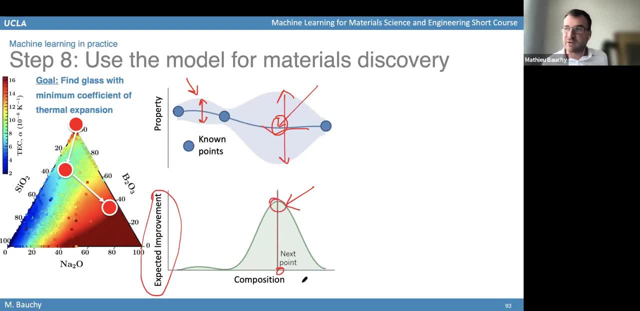 what should be the next material that you should try. But, like for example here, your model does not predict a minimum. It actually predicts a maximum here, but there is a pretty high uncertainty. So your model- the expected improvement function- also thinks. 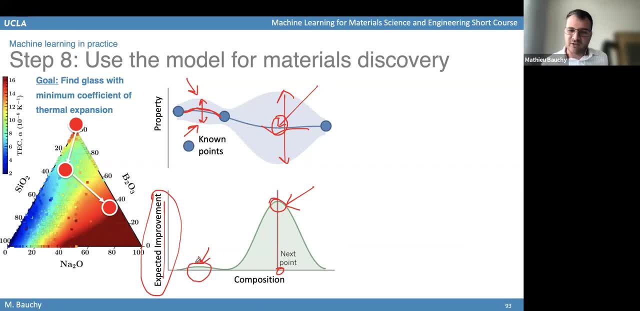 that this area should be explored as well, But at least in this case it's preferential to start with this data point first, because not only your model thinks there is a minimum, but it also corresponds to a very high area. So then, what you're going? 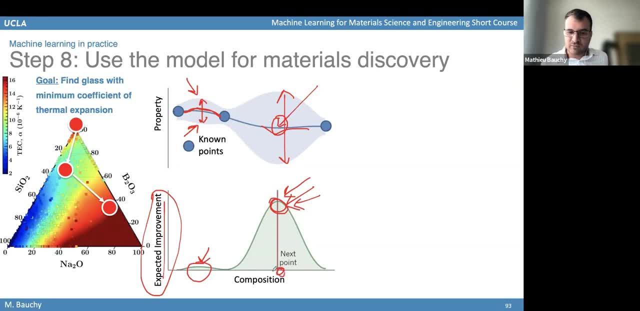 to do is to take this composition, make a glass with this composition and then measure the coefficient of thermal expansion for this glass. So now that gives you a new point. Now you have a new point here, which is a new point that you can now add. 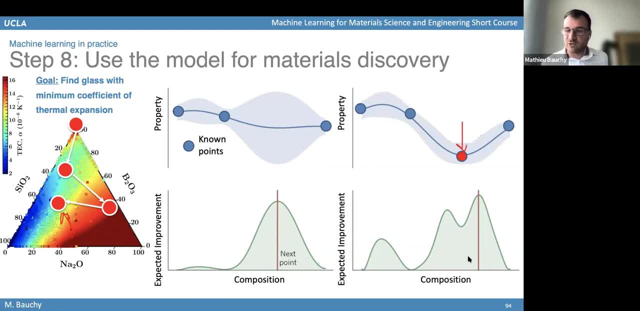 to your data set. So that's a new point that you can reuse to retrain your machine learning model. That's a new information that you have now, And so, now that you have this new information, you can again try to optimize your machine learning model here. 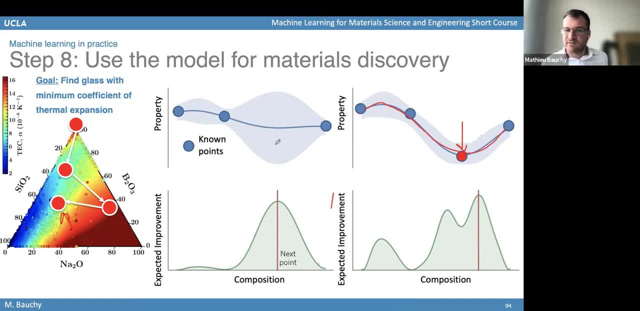 So now it will have changed, because now it is aware of a new point here: The uncertainty. the confidence interval is also going to change And again you can calculate the new expected improvement function which will tell you again what is the best balance. 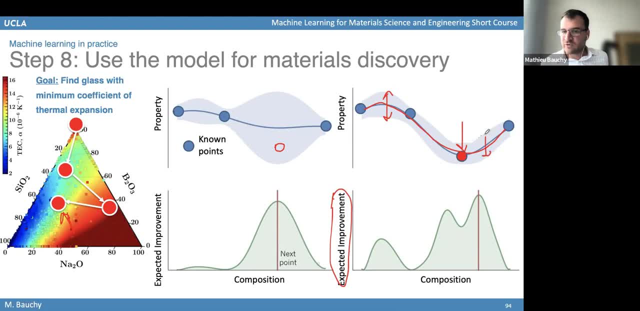 between trying to reduce the uncertainty of the model, but also exploiting what the model thinks should be the minimum. And so now, what the model thinks, what the expected improvement function thinks, is that this point here should be the next composition that you try, because it's possible. 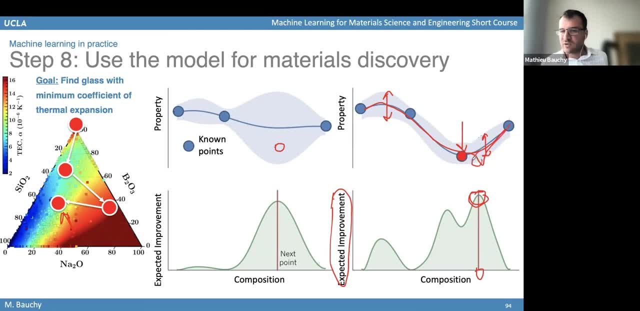 that your model continues to dig freeze here, So this composition could be the best choice to try next. So what you're going to do is to try it again And again. you're going to get, you're going to synthesize this glass. 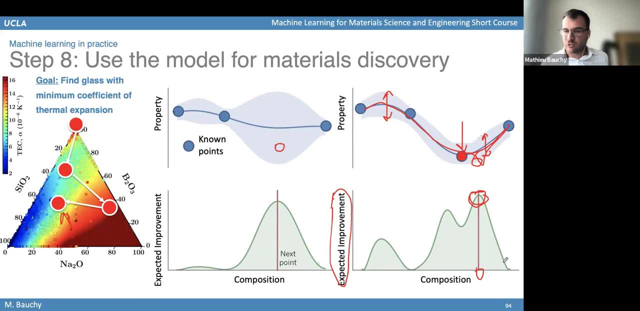 with this new composition and add it to your training set, retrain the model, et cetera, And you're going to continue this iteratively until you find that you have found the minimum possible value. So at this point, at some point, 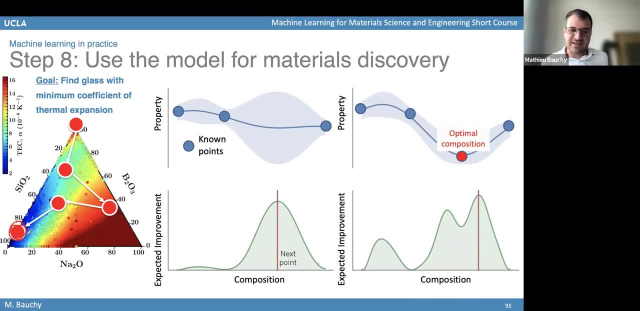 you will have found the glass that has the minimum value for the coefficient of thermal expansion, And at this point you know that you have converged. you have discovered the new glasses and you have been able to discover these glasses with a very limited number of trials. 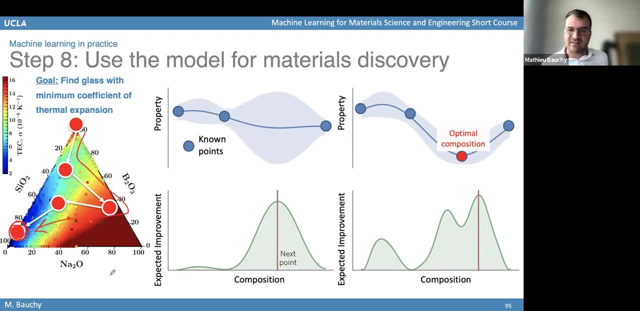 because you always try. the next glass that you always try is always the best possible glass. It's the glass that the machine learning model think is going to be the most promising to try next. So this allows you to discover new materials very efficiently without trying too many. 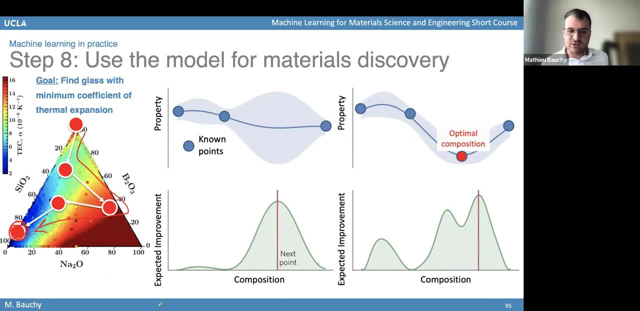 trial and error, by just always using the glass that is or the material that is predicted by this expected improvement function to be the most promising, to be the next glass to try, That is, to be the most promising based on the objective that you have. 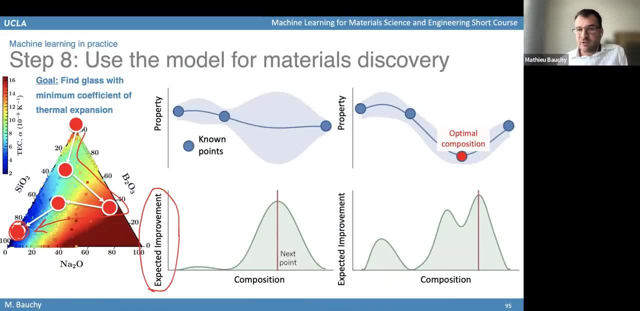 Okay, so that's pretty much all I wanted to talk about for this course. So sorry for being a little bit late. So now I think if you have some questions about any content of this class, or if you have any questions about like machine learning, 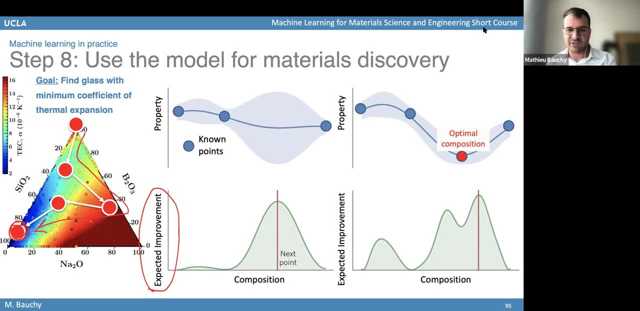 in general, feel free to ask. We can save a little bit of time to answer some questions. So, yeah, if you have any questions, feel free to ask, And if you don't have any questions, then I'll just thank you for attending this course. 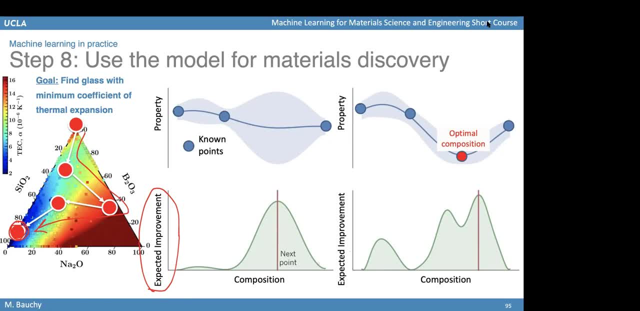 Hello For have more examples for the machine learning. you say you have videos, but you say it was in Matlab. but I was thinking you have videos in Python. Yeah, I mean, I don't have any videos that I made myself using Python. 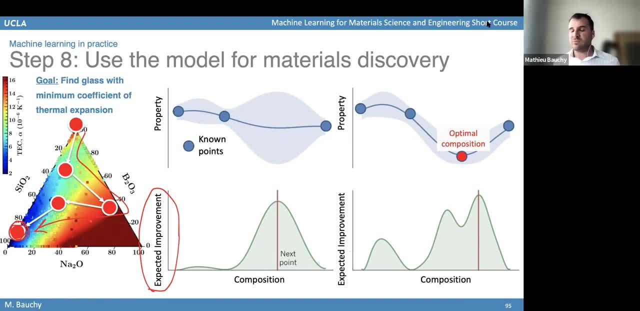 like all my videos are using Matlab. That being said, I'm sure you can find some other example of videos in Python. I think actually it's. there's probably more videos using Python as an example than Matlab. So, because Python is really the most, 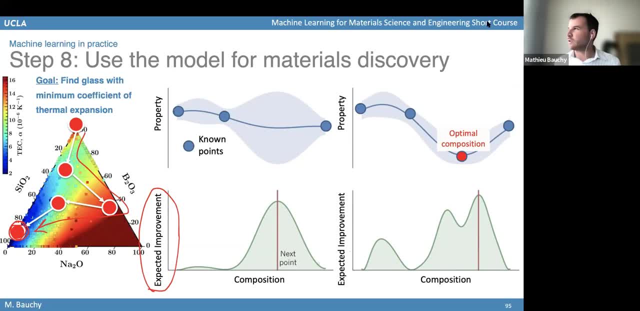 popular language when it comes to machine learning. So yeah, unfortunately, all the examples I have are all in Matlab, but I think you should be able to find a lot of examples in Python as well, either on YouTube, either by looking at some courses. 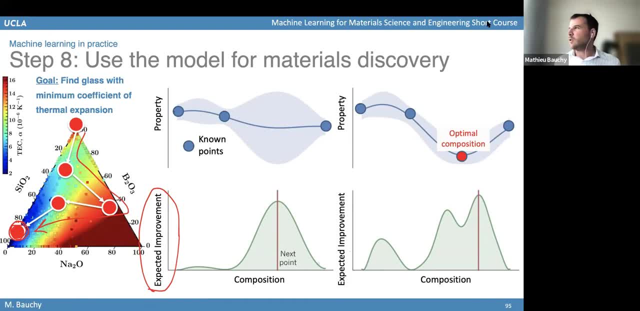 on Coursera or other websites that have some courses to teach machine learning. Most of the examples here are going to be likely in Python, just because it's the most popular language for machine learning, So I think you should be able to find some. 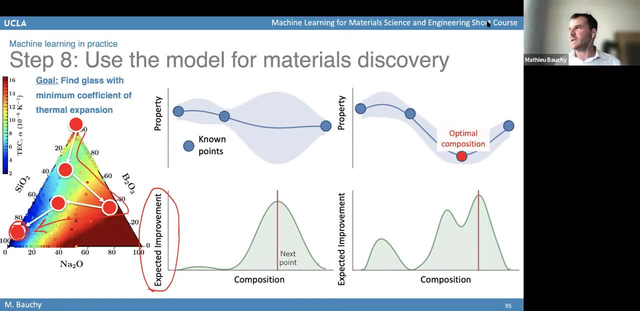 If you need some recommendation, let me know and I can point you towards specific video in Python. But otherwise I think it should be probably even easier to find videos using Python than using Matlab. Thank you. Any other questions, Doctor, before you officially finished? 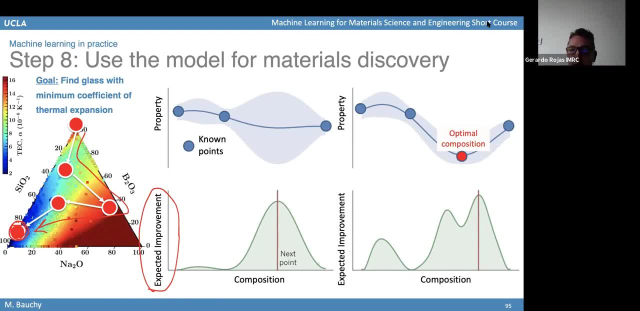 let me tell you that, on behalf of International Materials Research Congress and Sociedad Mexicana de Materiales, President Patricia Zambrano, we want to thank you so much for providing such a great tutorial And please let me share my screen for a while. 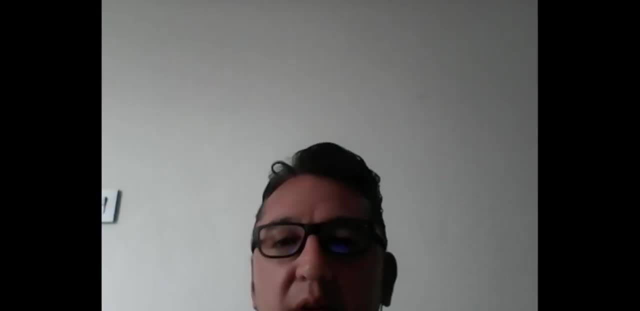 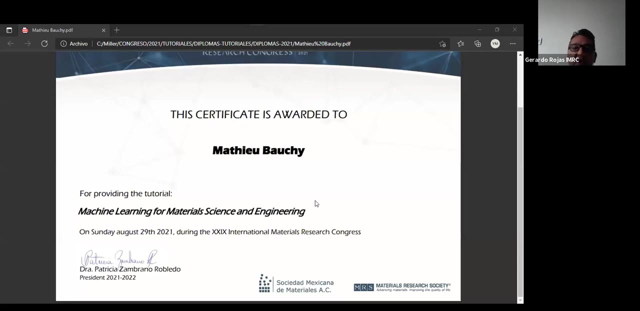 Thank you, Doctor, And I'm going to read it. It says: this certificate is awarded to Matthew Bauchi for providing the tutorial Machine Learning for Materials Science and Engineering on Sunday, August 29th 2021,. during the 29th. 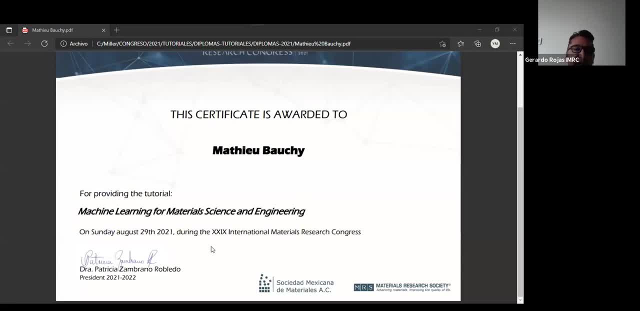 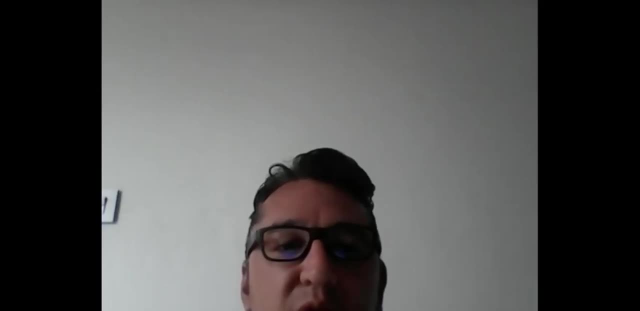 International Materials Research Congress and signed by Doctor Patricia Zambrano-Rovell, President 2021-2022.. Congratulations, Congratulations, Doctor Matthew. Thank you, And also I'd like to. I want you to turn your camera on. 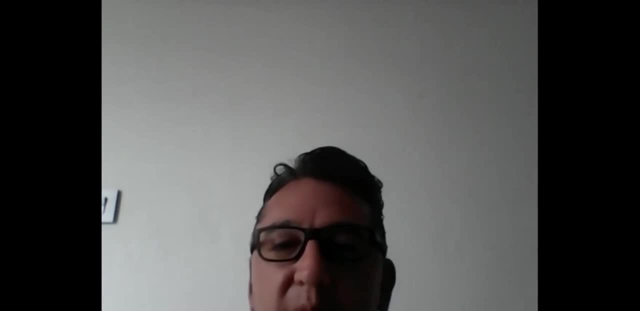 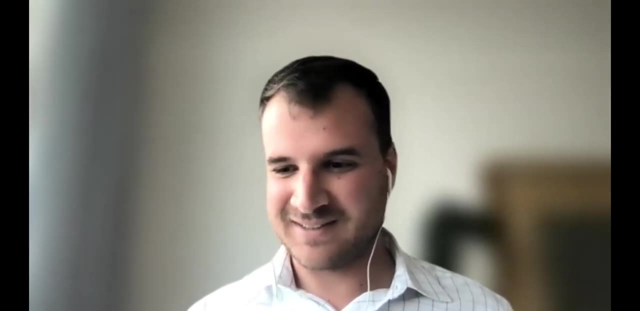 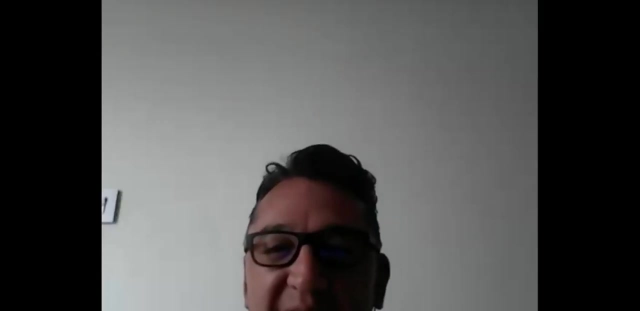 please, in order to take a screenshot. Thank you so much. Oh, I can finally see the way you look like. I'm sorry. Well, it's good to finally see how everybody looks like. Yeah, of course, Everybody try to make.